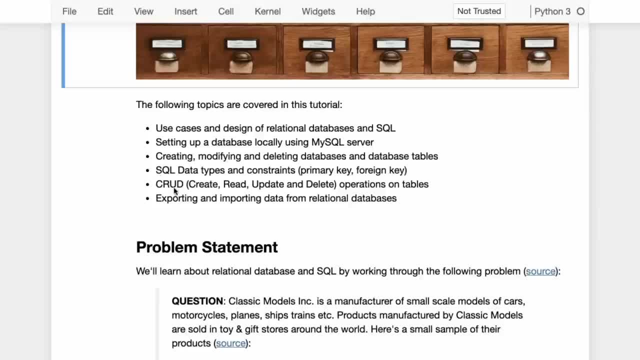 at crowd operations. You will see this term a lot in relation to databases. So create, read, update and delete operations on data stored in tables, And then we'd also look at how data can be exported and imported from relational databases. This is part one of 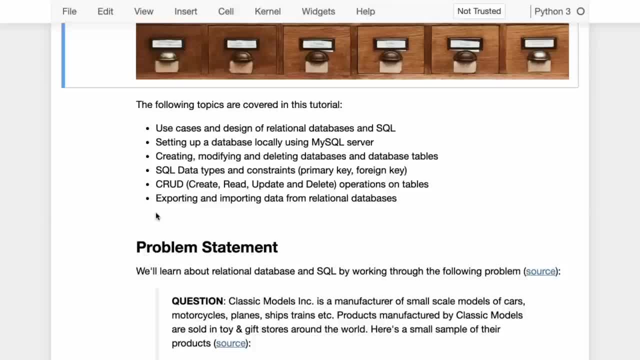 two lessons On SQL. So the next week will be an advanced lesson where we will look at aggregations, We look at joins, we look at indexes and we will also see how to use, how to use Jupiter to get data out of a SQL database and how to work with it in Python. So maybe how to 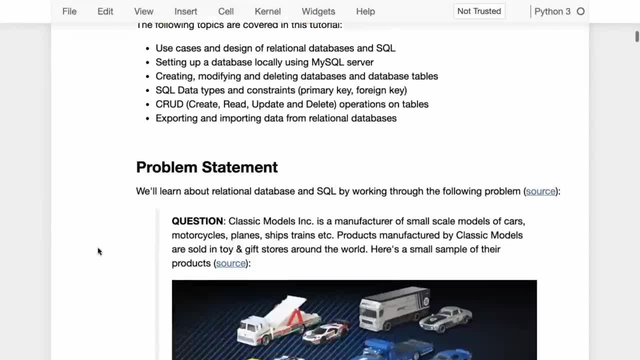 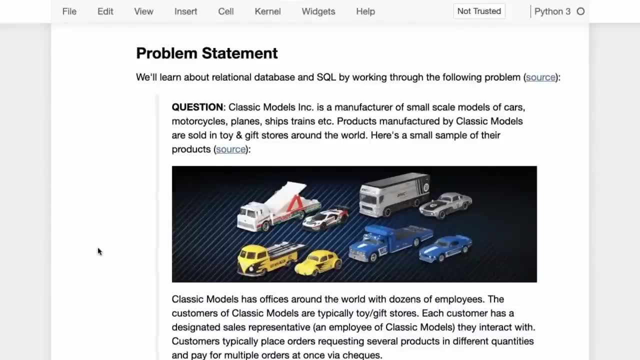 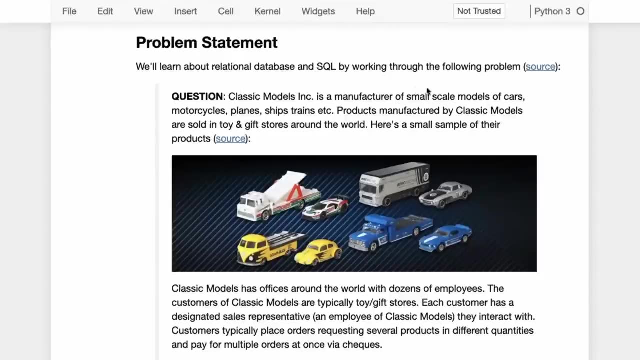 do some analysis and how to do some visualization. But today we are going to work in a more traditional setting where we are going to use some Commonly use software like a my SQL server for working with SQL databases. Now we learn about relation databases and SQL by working through this problem. 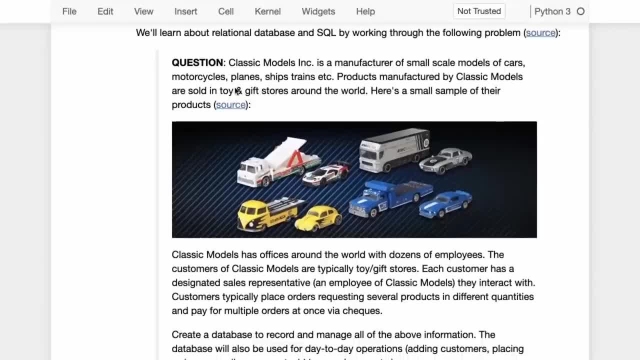 This is a hypothetical scenario that we've set up and we try and understand, in the context of this problem, why we want to use a relational database and how SQL is helpful. So, classic models and cooperated is a manufacturer of manufacturer of small scale models of car. 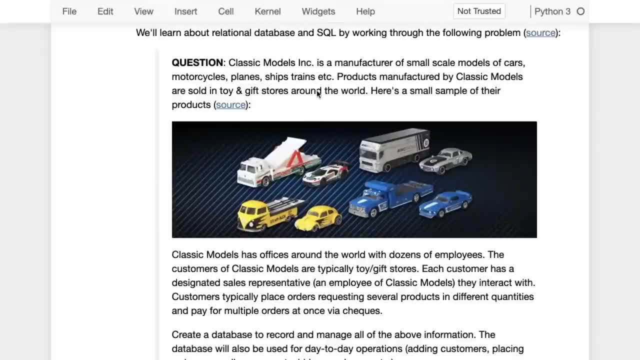 models- cars, motorcycles, planes, ships, trains, et cetera- and products manufactured by classic models are sold in toy and gift stores around the world. So this is what some of their products look like. They are small scale models of various types of vehicles, and classic models has offices. 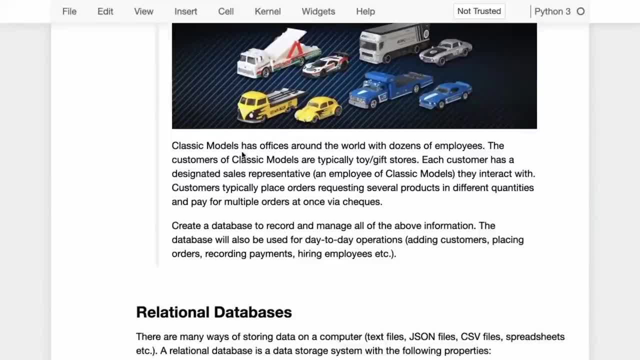 around the world with dozens of employees, And these are primarily sales offices. So the customers of classic models are typically toy or gift stores, And each customer typically has a designated sales representative in the same region who's also an employee of classic models. 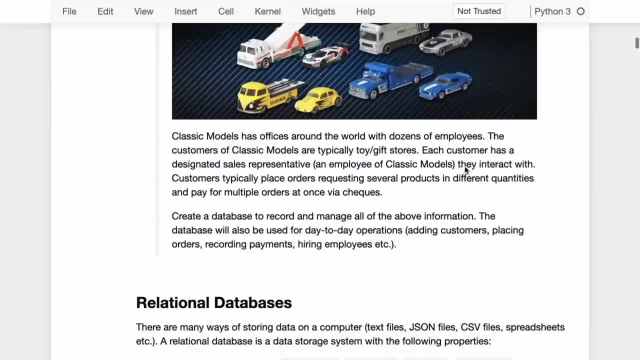 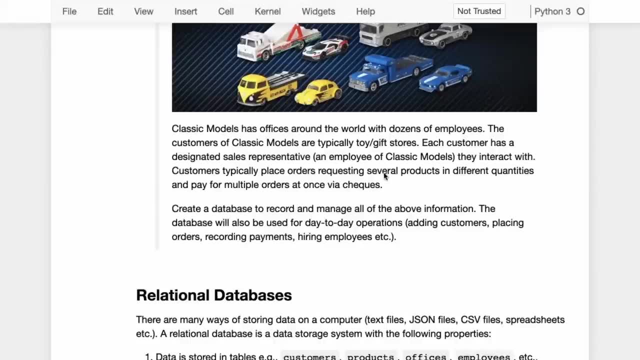 And they interact with that sales representative directly. Then customers typically place orders requesting several products in different quantities, and then they pay for multiple orders at once via checks. So this is typically how a business works. You have, You manufacture some products, and then you have offices and then you sell your products. 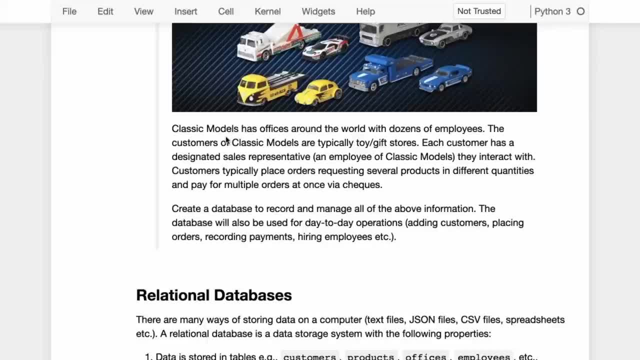 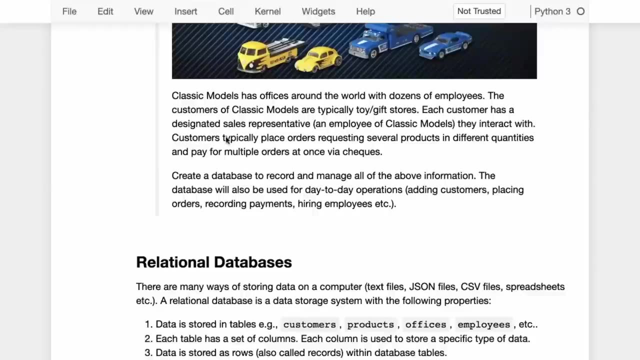 to people and you have transactions with them, And then you have employees involved who are involved in managing these relationships and managing the offices that you run right now. for an international organization like this, it is important to record all of this information, all of the activities. 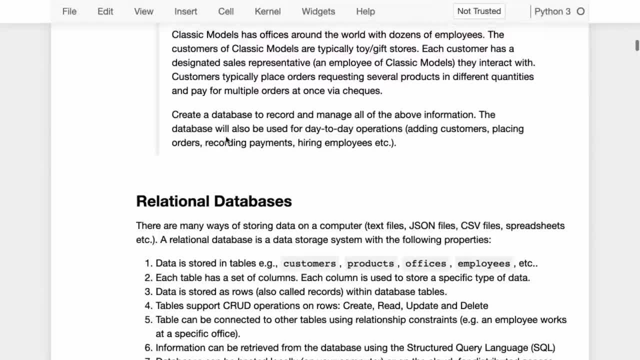 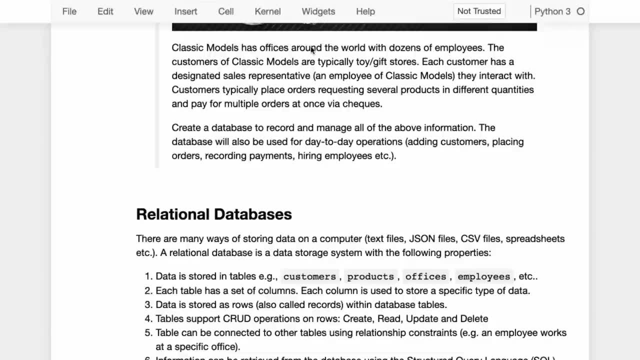 In a single central place, right? So your task is to create A database, some sort of a system where you can record and manage all of this above information. So where do we have our offices? who works at these different offices? Who are our customers? how? who is the sales representative for every customer? 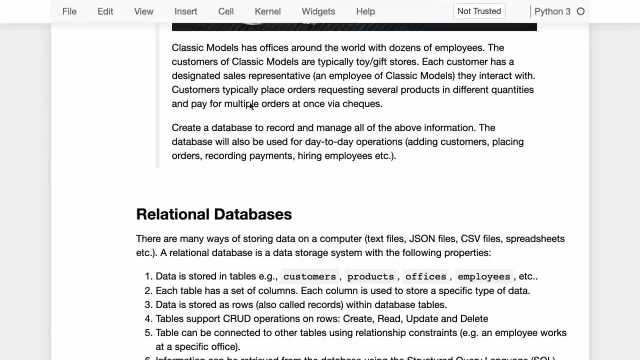 What kind of orders are customer placing and what are the payments from them. What do the payments from them look like? So we want to record and manage all of this information in a database in a central location, And this database Can also be used for day-to-day operations. 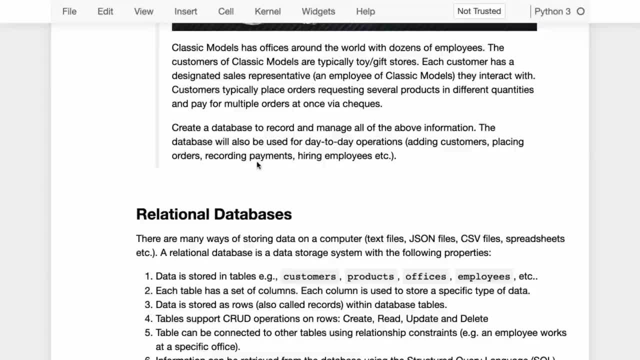 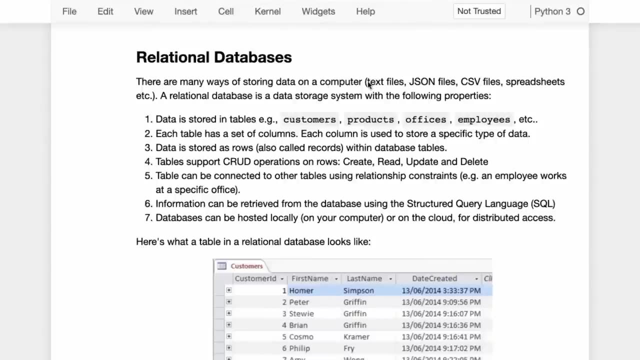 For example, adding new customers, placing orders, recording payments, hiring employees and things like that, And also just querying information and getting analytics about how the business is doing. So, while there are many ways of storing data on a computer, for example, we could put this: 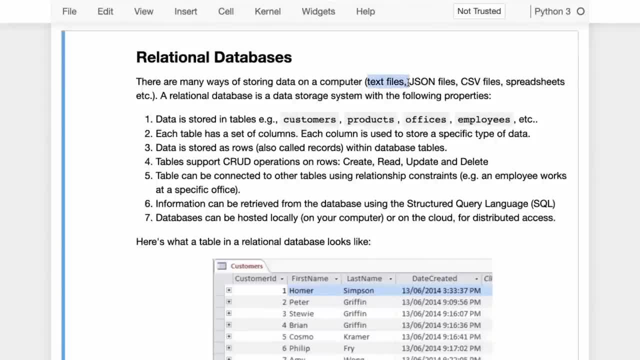 into a bunch of text files. We could maybe open notepad, create a few files and put in all this information there, but looking it up is going to be very difficult, Are we So? we could use JSON files. We could use CSV files. 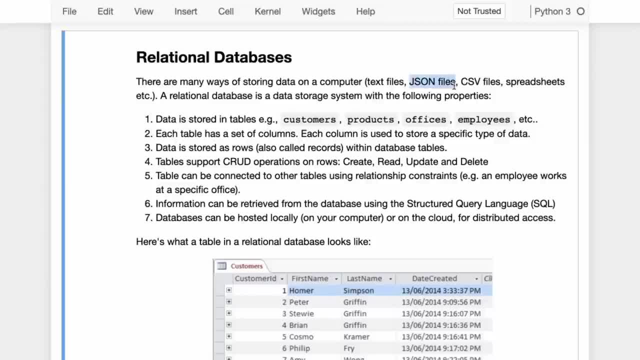 We could put, maybe have a CSV file for customers, one for products, one for employees. We could use spreadsheets, things like Excel, which a lot of businesses use, but spreadsheets become a bit limited in functionality as you deal with really large data sets. 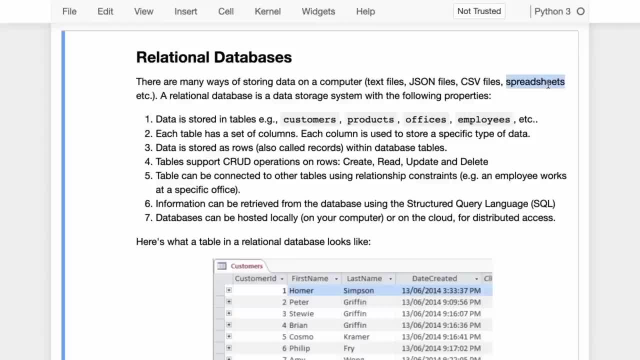 And as you want to do some advanced forms of querying, and also as you want to integrate this with these systems, with other systems. For example, you want to create forms for customers to sign up, You want to create order forms, You want to create a bunch of different things connecting forms with spreadsheets and writing. 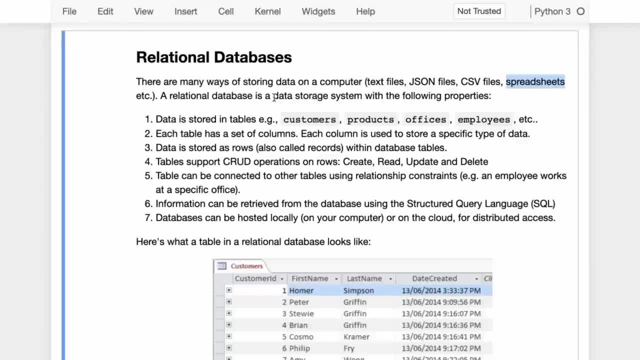 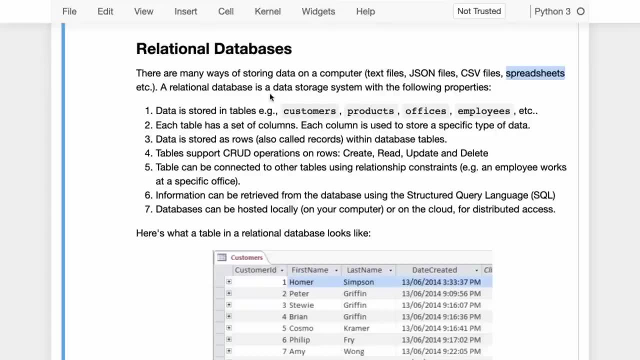 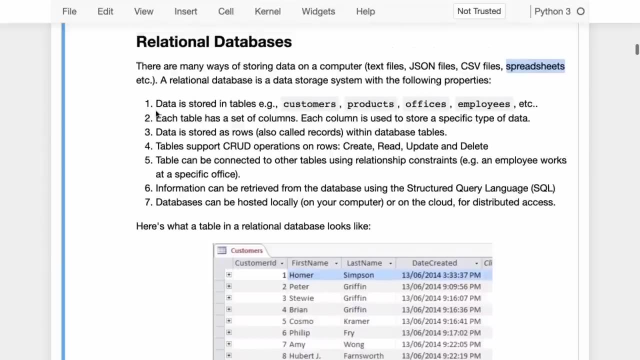 custom business logic can be a bit tricky, So this is where a relational database comes into picture. A relational database is a data storage system, typically, which has the following properties. So the first thing about a relational database is that data is stored in tables. 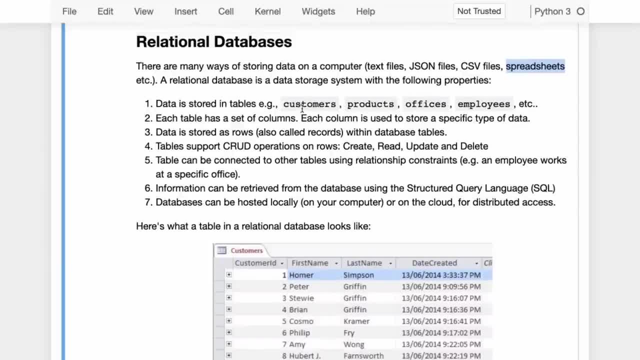 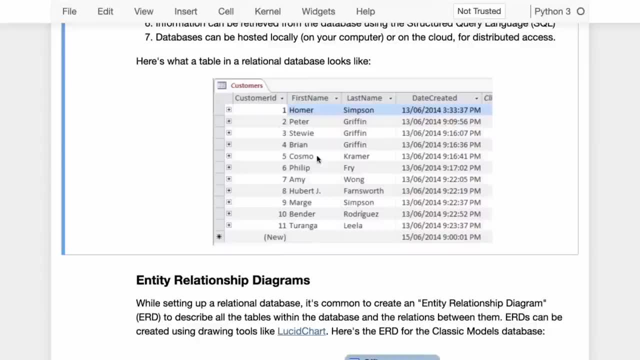 So each kind of entity that we're concerned with, you have a table for it. For example, you have a table for customers and this is a snapshot of some data stored in a relational database. So you have a table for customers and each customer has a customer ID. 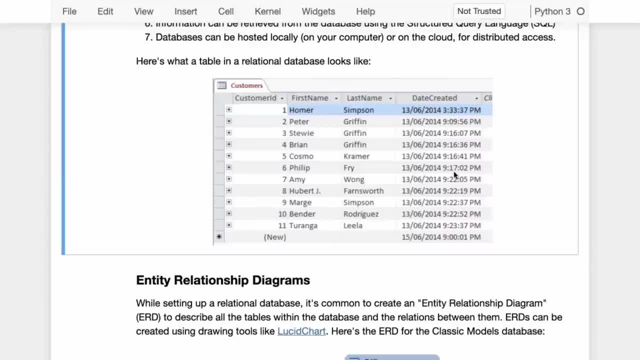 They have a first name, They have a last name, They have a date created, which means the date at which, or the exact time at which, that customer was added to your database, And then you have a bunch of information, maybe where they live, et cetera, et cetera. 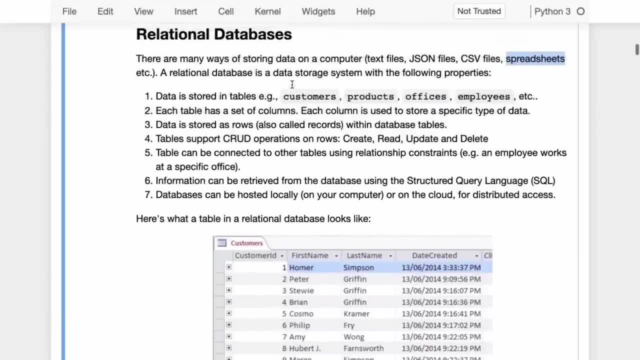 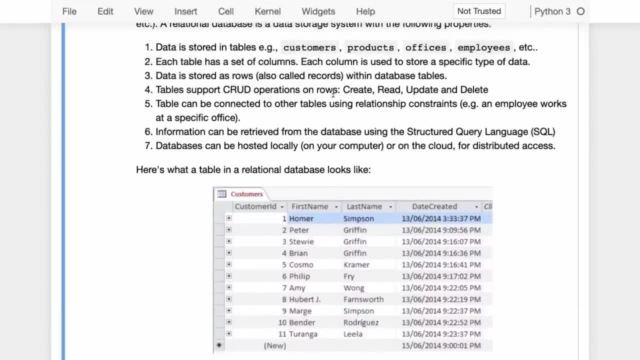 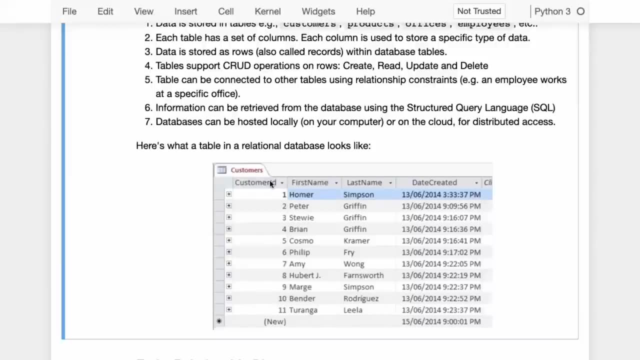 right. So that's one important piece- that data is stored in tables. Second, each table has a set of columns. As you can see here, each table has a set of columns and each column is used to store a specific type of data. For example, customer ID is going to be a number and it's, in fact, going to be a unique. 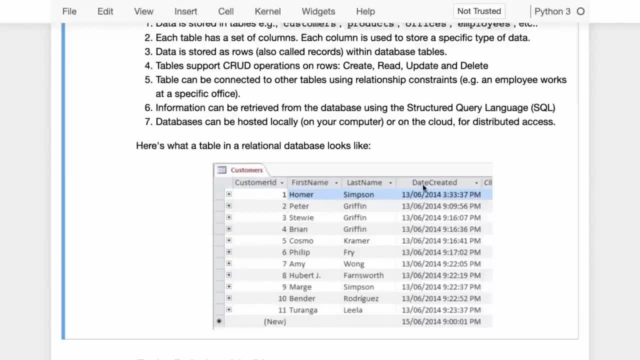 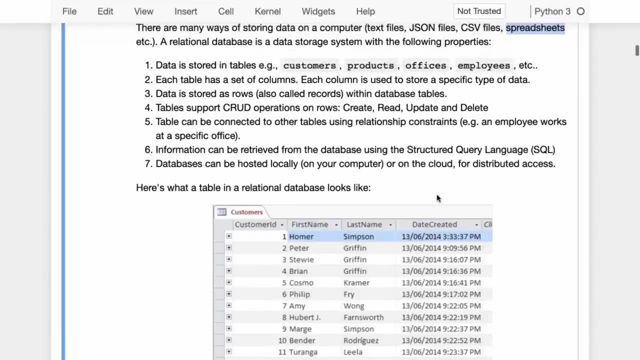 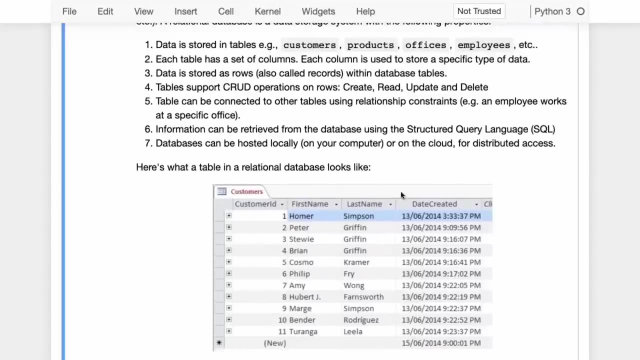 identifier for the customer: First name and last name is their first and last name, And then date created is going to store the date or the time- exact time when they joined, and so on. next data Data in the tables is stored as rows, So each row of this data after this header row represents a customer. 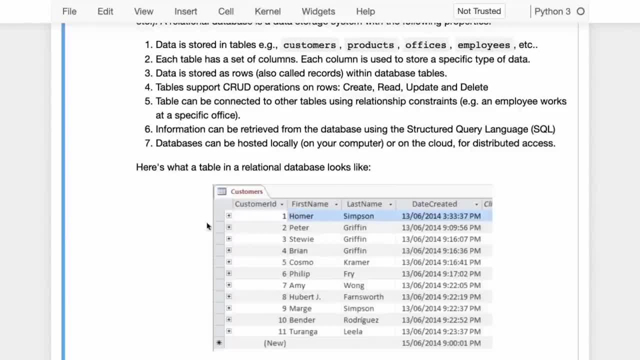 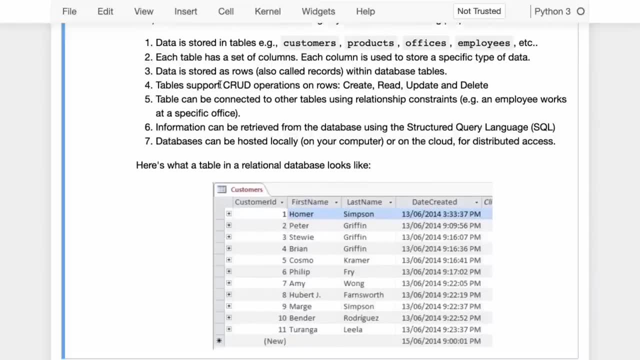 And sometimes these rows are also called records, So data stored using rows within database tables. next table support: crowd operations on rows, which means create, read, update and delete, So you can add new rules into the table. That's the create operation. 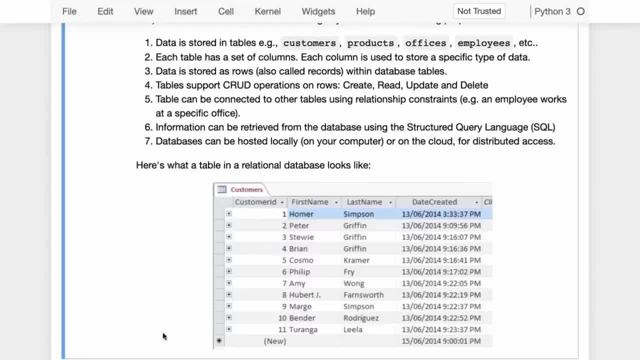 You can delete rows from the table. You can delete rows from the table. Uh, that is the delete operation. You can get data out of the table. Let's say you want to figure out which customers you have in the United States, Then you can query that. 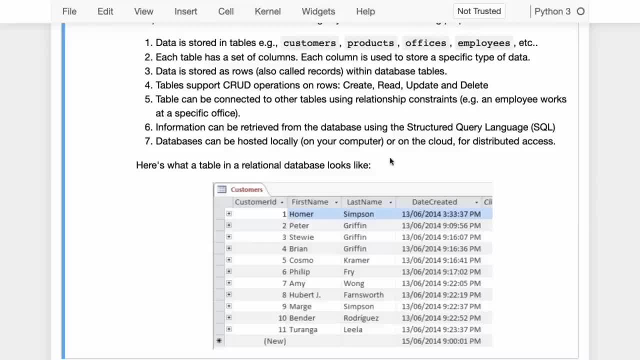 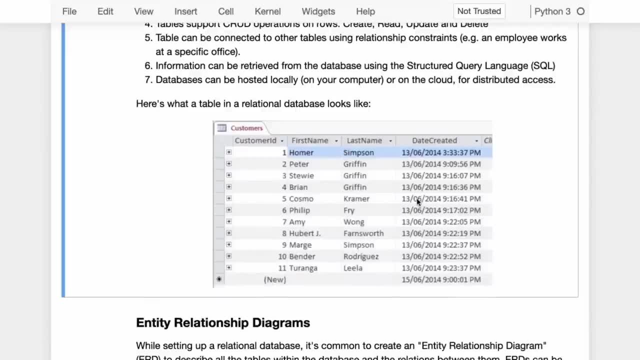 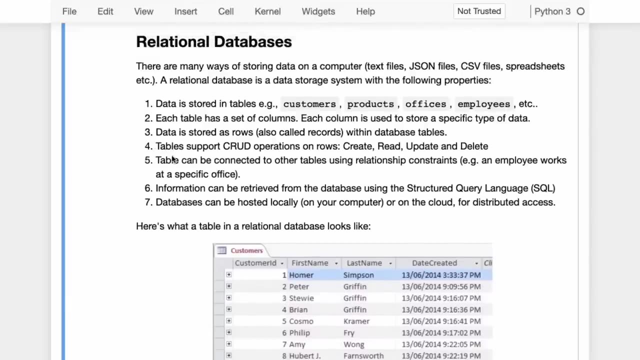 You can just type out some code and you will get back that information. and you can update information, because if a customer changes their address or their phone number or the email, you should be able to change that- Then one important piece- So a lot of databases support this- but one important piece is relations between 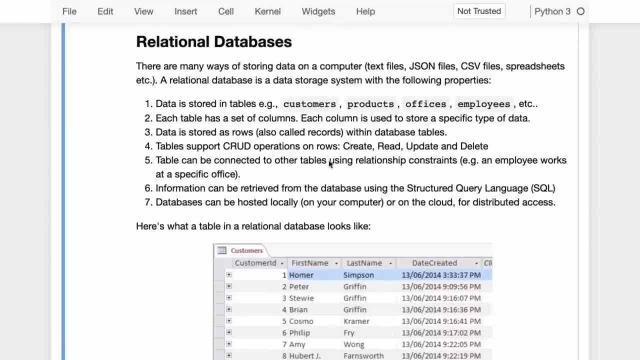 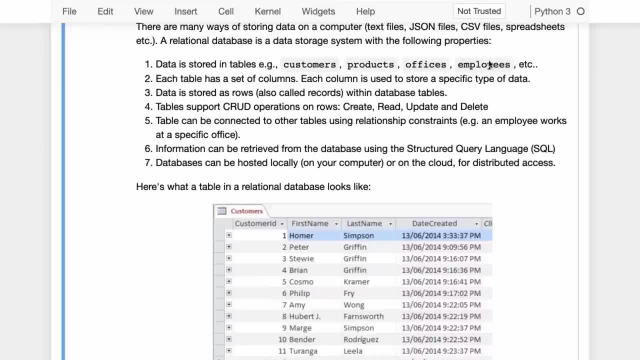 tables, So tables can be connected to other tables using relationship constraints. For example, you have offices and you have employees. We can say in the employees table that an employee works at a particular office. So we can make a relationship between an employee record and an office record. and 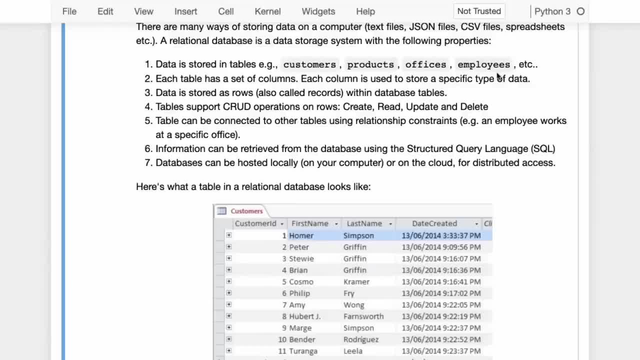 there can be one-to-one relationships, There can be one to many, many to one relationships, And we'll talk about these in more detail when we talk about joints, but at the moment, just the fact that You can link records across tables is an important piece to understand. 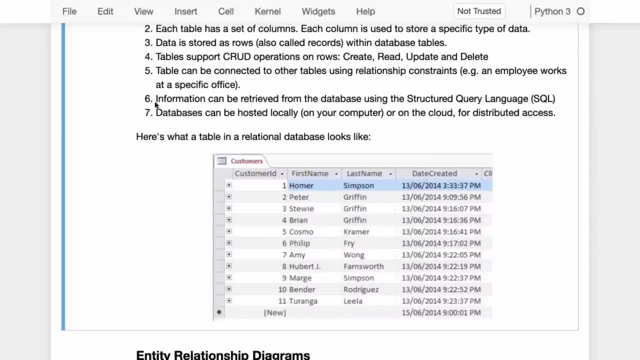 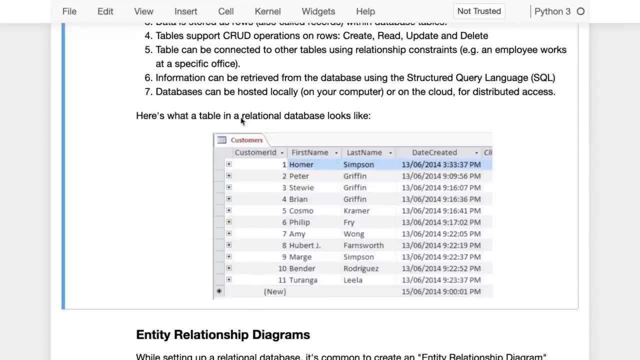 Then relational databases typically allow you to retrieve data from the database using the structured query language or SQL, which is what we will learn today, And these databases can either be hosted locally on your computer or, more commonly, these are hosted somewhere on the cloud for distributed access, for example, for classic models, it's 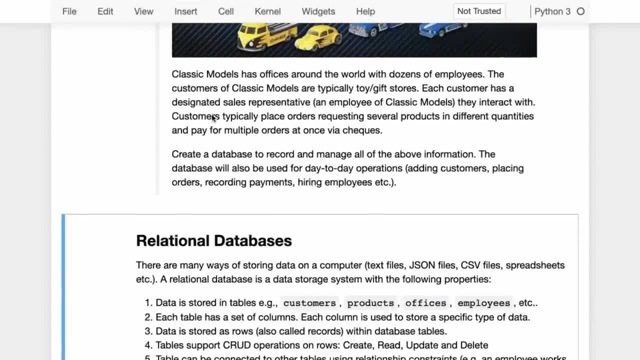 possible that They have set up a database on the cloud and all the employees from all the different offices use this database through some browser based application. Maybe they have forms, maybe they have some kind of access based system where different employees have different permissions and they use this database, but everybody's ultimately making changes or getting 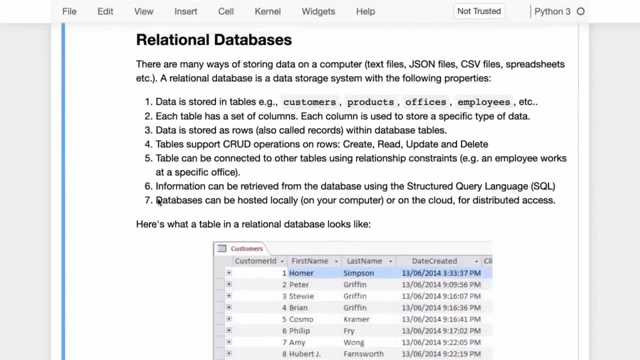 information out of the same database. Right, And this is how most modern applications work. for example, on Joe, We have a relational database sitting somewhere on the cloud and all of your account information is in the relational database And when you open your profile, we get data out of that relational database and we show it to you. 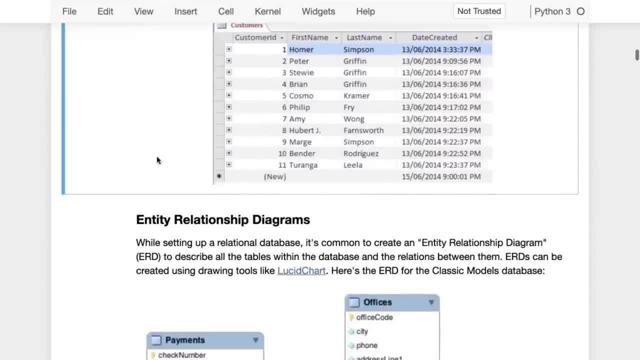 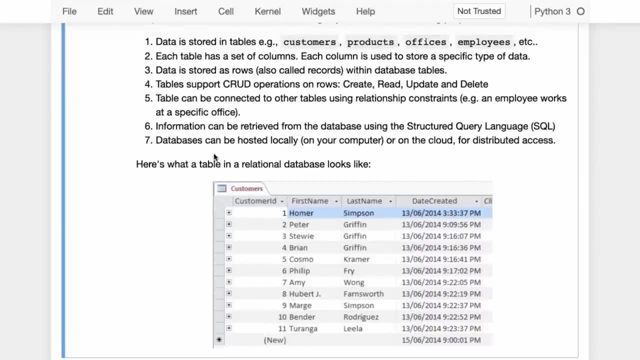 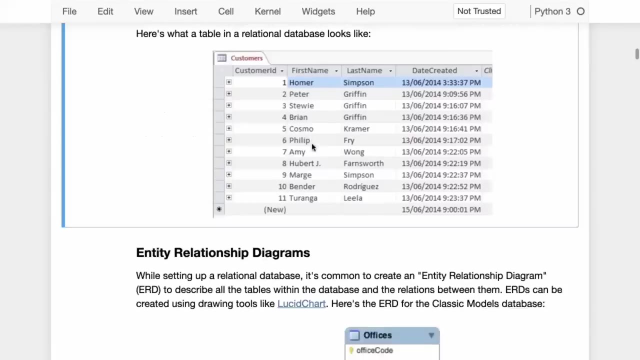 Okay, So that's relational databases. The important pieces are that data stored in tables, a set of columns- each column has a specific type, and then tables can be connected using relationships and the data is queried using SQL or the Structured query language. 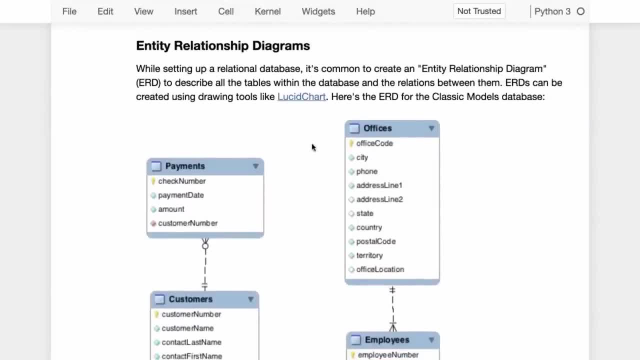 Now, when you are setting up a relational database- which you most likely won't have to do, because in most cases, whatever corporation you work with or whatever client you work with in a project, they will already have a database. But when you're setting up a database, it is common to first create an entity relationship diagram, or it's called an ERD. 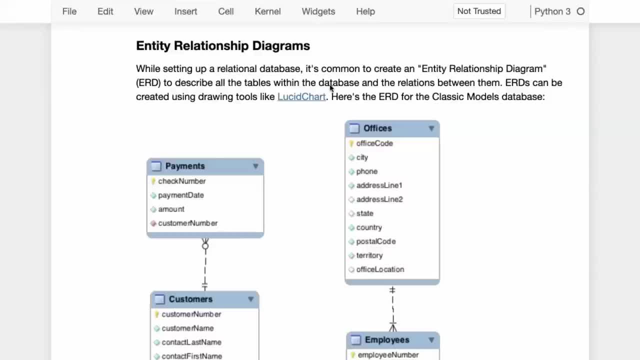 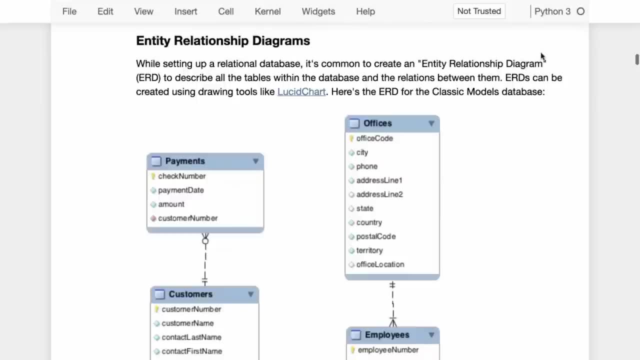 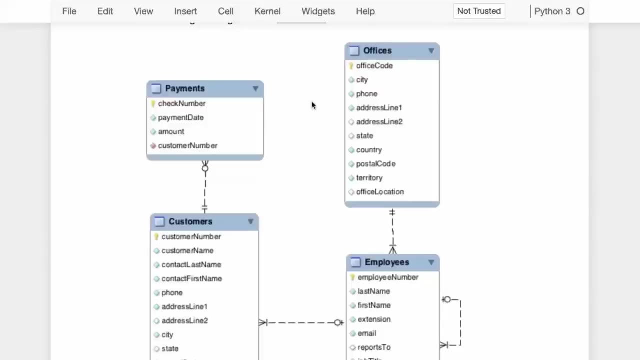 to describe all the tables within a data, within the database, And the relations between them. So ERD. this is what an ERD looks like- an entity relationship diagram- and they can be created using drawing tools like Lucidchart. So typically, this is something. an image like this is what you might be given when you join a company. they may give you an. 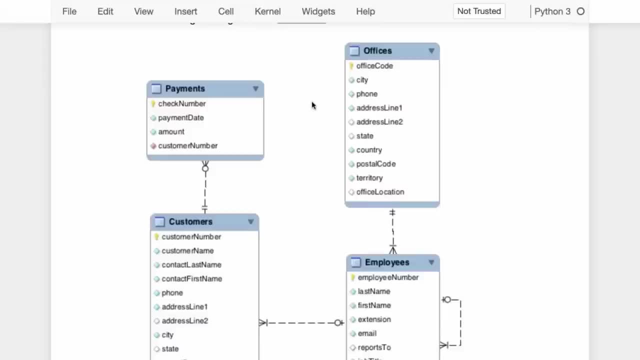 image like this and they will tell you that this is what our data model looks like or this is what our database looks like, And sometimes you may have multiple ERDs because different teams are different, Or orgs or different departments when this in the same company may have their own separate database. 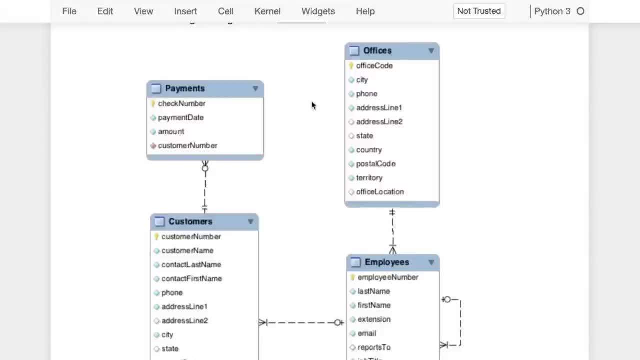 And sometimes you may have data duplicated across different databases and so on. But let's just take a look at this ERD and understand what it represents. So the first thing you will notice is we have these boxes. We have this one box called payments. 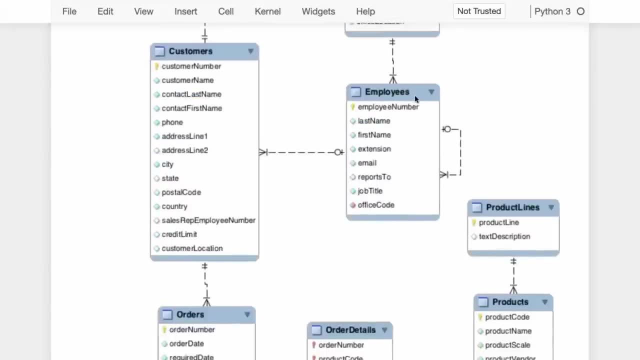 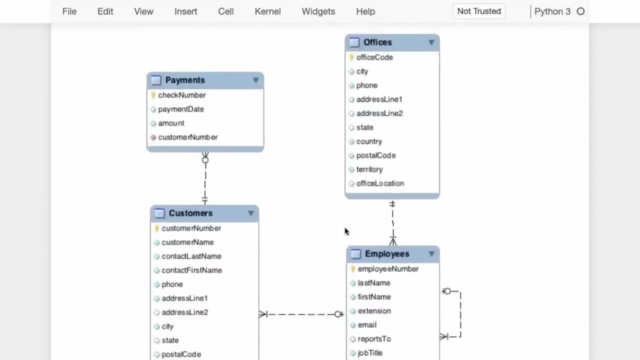 We have this called offices. We have employees, Customers, Product lines, products, orders and audit. So each box in an entity relationship diagram shows you a table. Okay, So, for example, offices is a table and then inside each box this is the list of columns in the table. 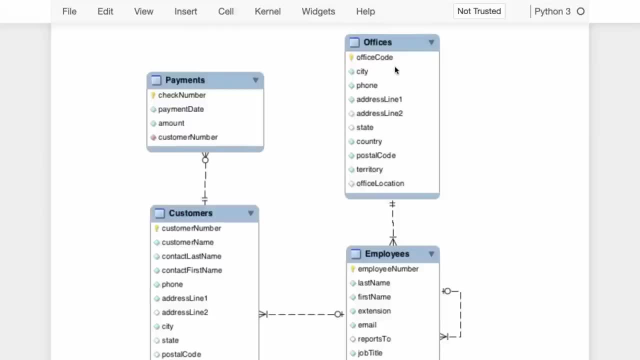 Now, the ERD does not contain any actual data. It is sort of a blueprint for the database on what tables it contains and what are the fields within each table and how the tables are connected. So the Office is stable, for example, will contain an office code and you will see that this is. you can see a key icon here. 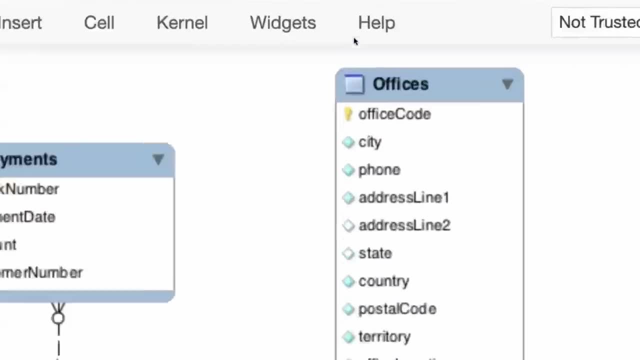 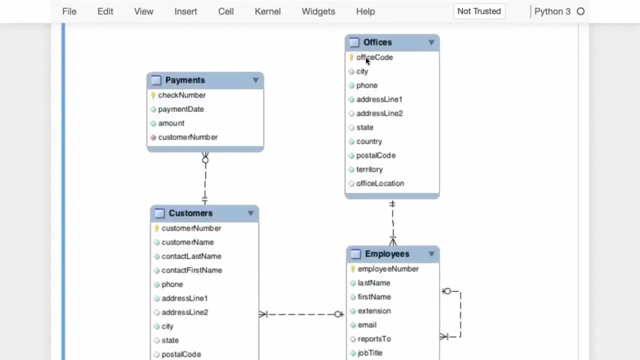 If I zoom in a little bit, so this is a key icon. So that is simply to indicate that the office code is a unique identifier for the office And this is also called the primary key. So the office code is a unique identifier or the ID. just as on Jovian, you have a unique ID which is your username. 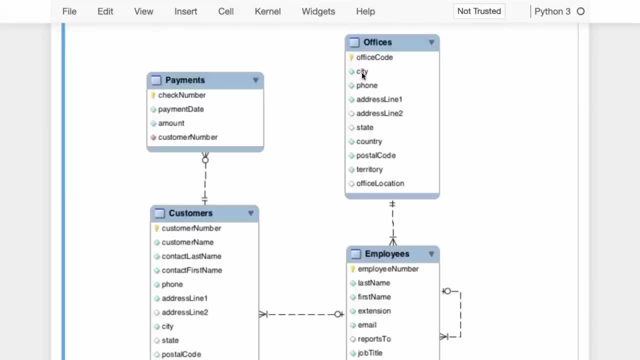 So, similarly, office code is a unique ID, And then the office is based in a certain city, It has a certain phone number, It has a certain address, address line, one address line to a state, country, postal code, territory, and maybe even a location or geo location for plotting on a map. 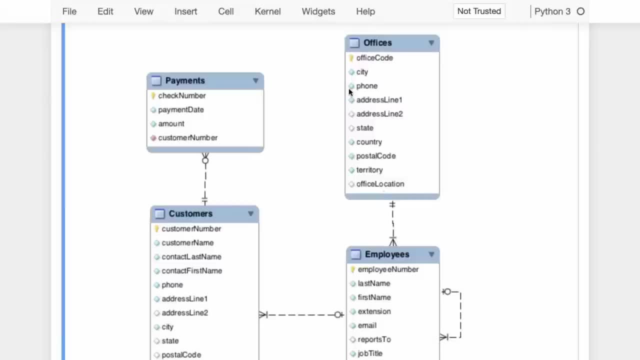 Okay, And different ways in which ERDs are created may or may not contain this additional information. For example, here, what this blue square represents is that this is a required detail if it is filled in, And if it is not filled in, then that means that this is optional. 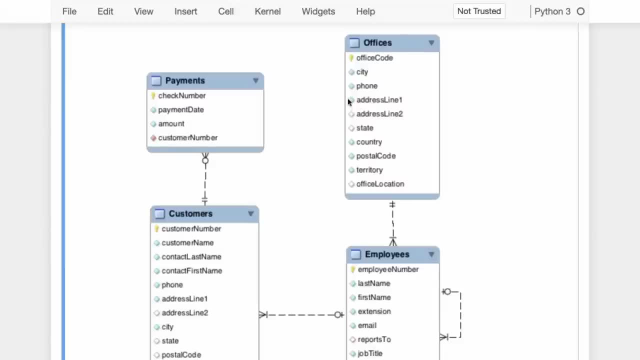 So you can have address line to. may not be present for some offices because it's enough to summarize the address in one line. but, yeah, you may not always have these details And this ERD does not contain information about the types of data. 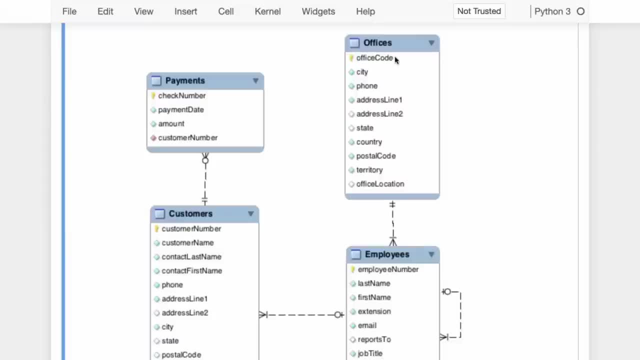 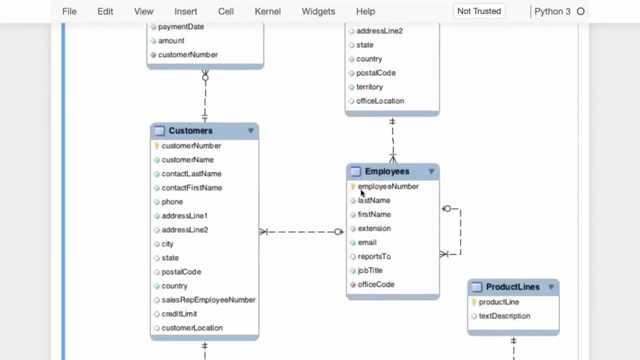 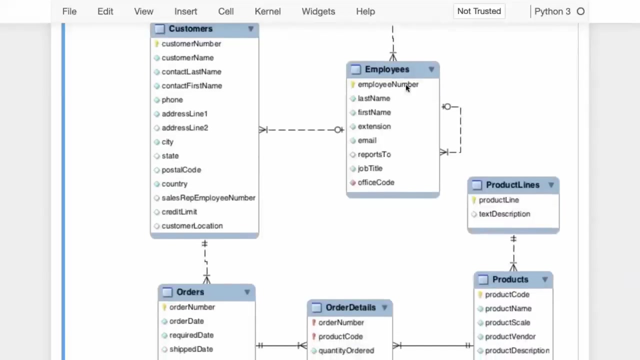 You can probably guess: office code would probably be either a string or a number. a city would probably be a string, phone would be a string. All of these would mostly be strings. Then you have employees. So for employees we have an employee number. 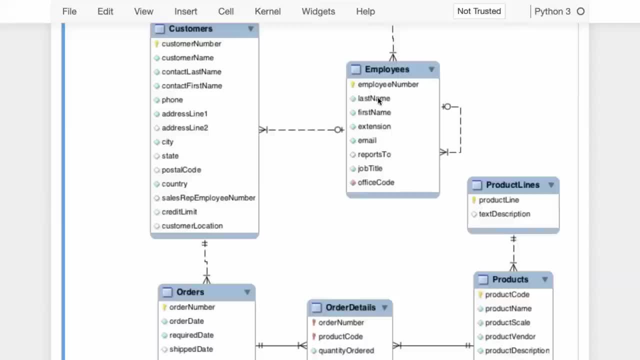 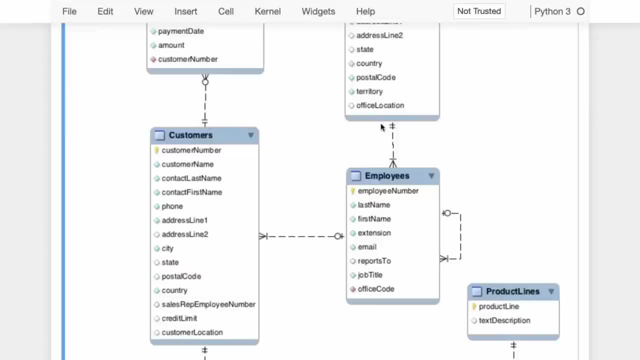 So that's the primary key And I think that is going to be a number. Then there is a last name, first name extension. So this is probably employees work at an office, So at the office, what is the extension to reach this person via phone? 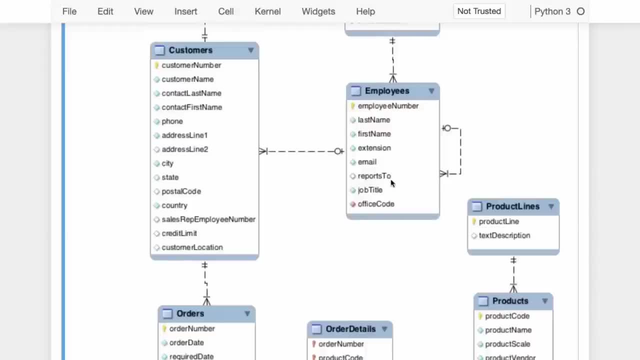 You have an email for the employee And interestingly there is this reports to field. So most employees in most companies report to other employees of the company. So this report Reports to is some sort of a link from employees to the same table of employees. 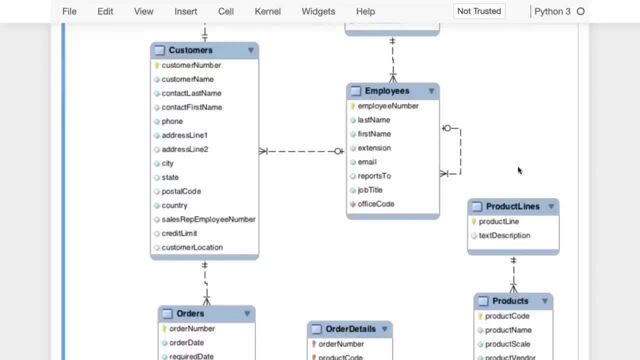 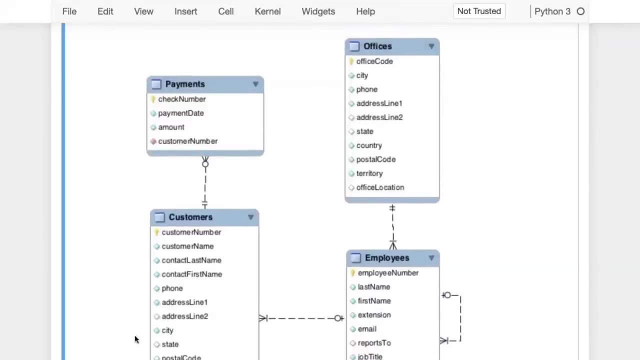 So reports to would probably contain an employee number of another employee in the company. Then you have job title and then you have something called office code. So office code again is going to be the office code of the office where the employee works. So you can already start to see these relationships. employees work at an office. 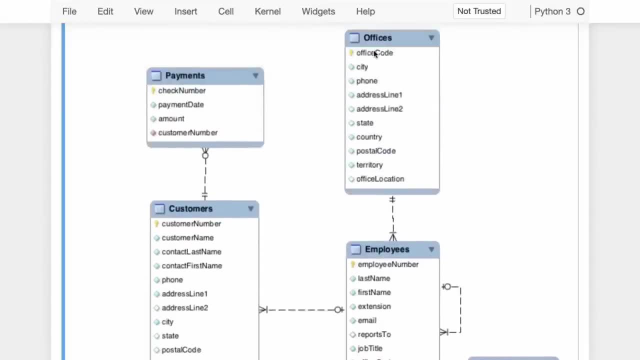 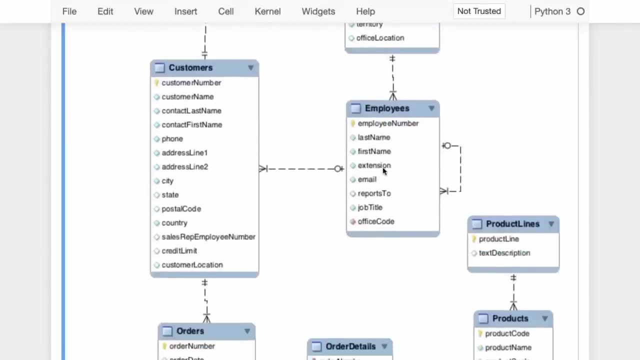 So there is an office code and employee and that office code should match with the office code of a particular office And then you can do interesting things like find all the employees who work at a particular office or maybe, given an employee, find the full phone number, which is the phone number of the office combined with the extension for this employee. 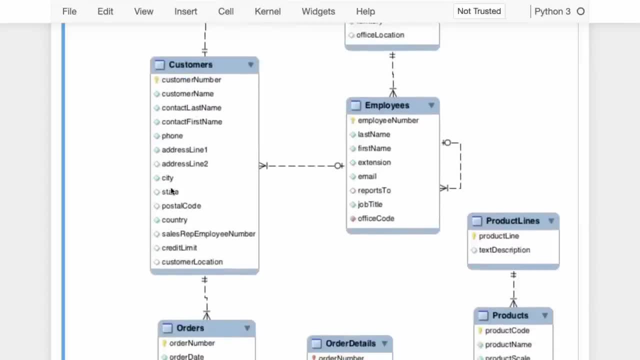 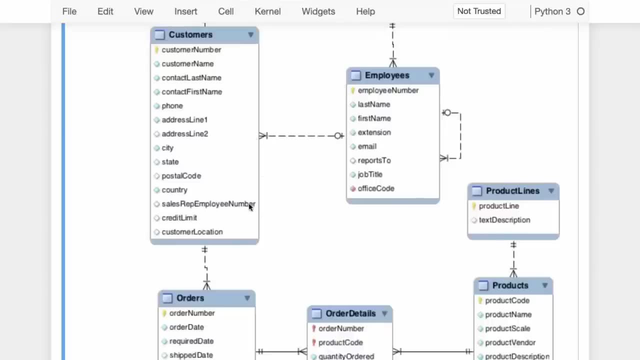 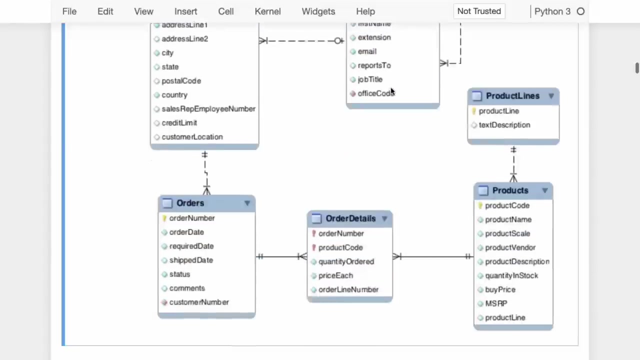 And similarly you will now see other relationships. You have customers, So customers have all this information. and then in customers you have the sales rep employee number. So this is going to be A reference- The customers table- to the employee table. the employee number should match up with an existing employee. 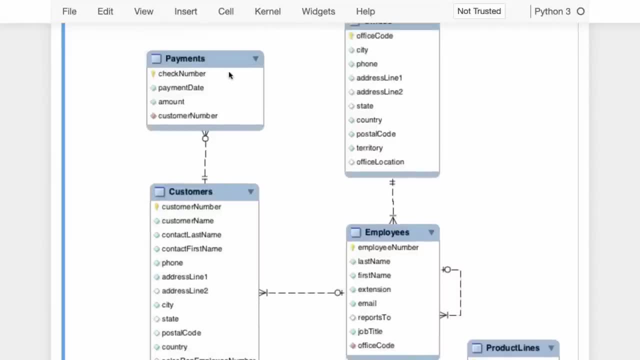 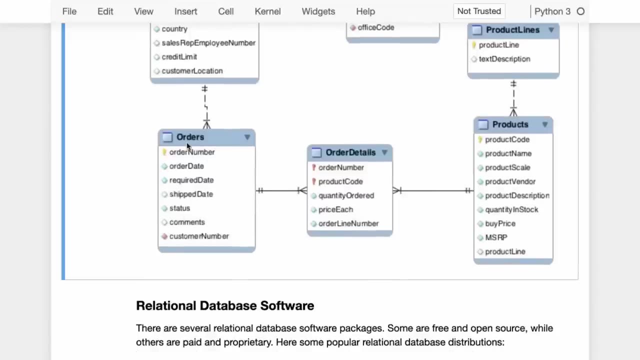 Then you have payments done by customers. So customers pay by check. So you can see, here there's a customer number which is a reference field. Then customers place orders. So there is a table where we are recording orders, where we have an order number, order date, some information about the order, some comments and there is a customer number indicating which customer has placed the order. 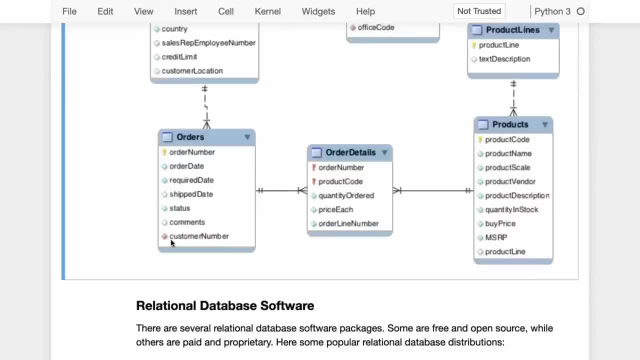 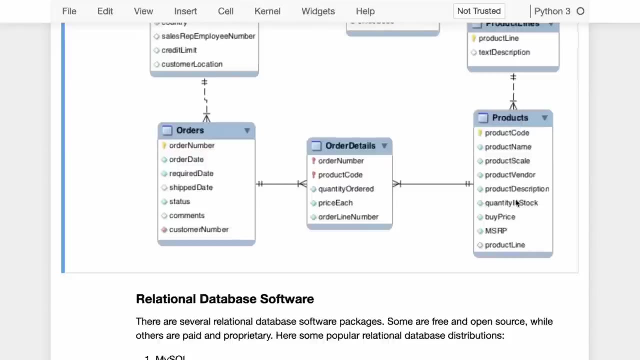 But of course, an order can A lot of information So you can place. you can have many products that you would have or that you can include in an order. So we have a table for products like product code, product name- product code is the unique ID, product name, product vendor, et cetera- and product code. 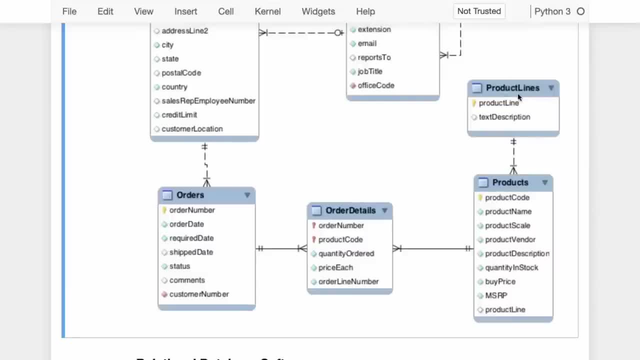 There is also a product line, which itself is another table. So you may have four or five product lines and in each product line, let's say, the product lines are cars, motorcycles, Ships, et cetera. Remember, this company creates small scale models of vehicles. 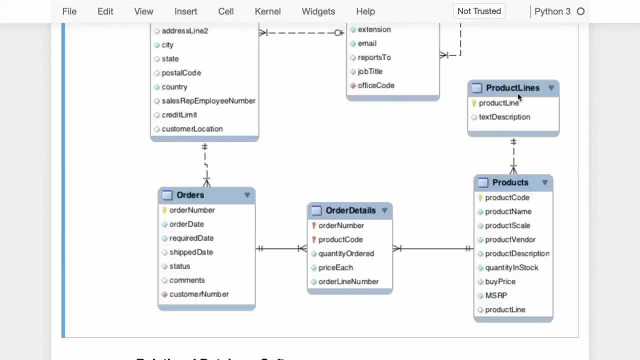 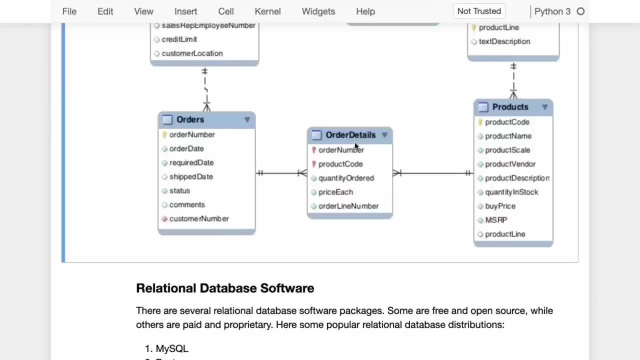 So product lines could be the different kinds of vehicles and the products could be then individual vehicles or individual actual products that they create, And then there is this order details, So an order can potentially have many products that were ordered. So in order details, 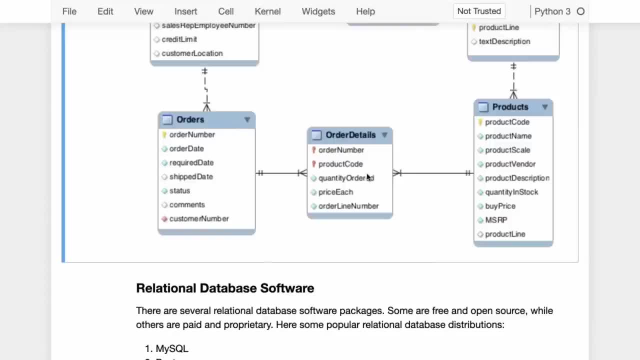 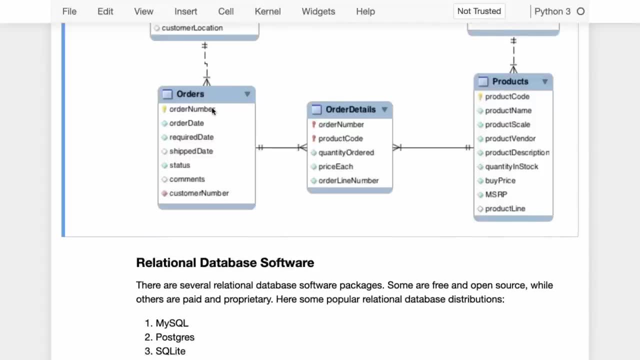 So for One order you may have several records in order details and you may have the order number, You may have the product code and then you may have the quantity ordered. So let's say, in order number one the customer, customer number 10 creates order number one. 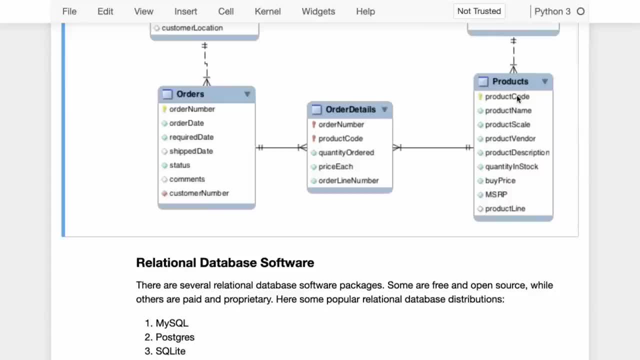 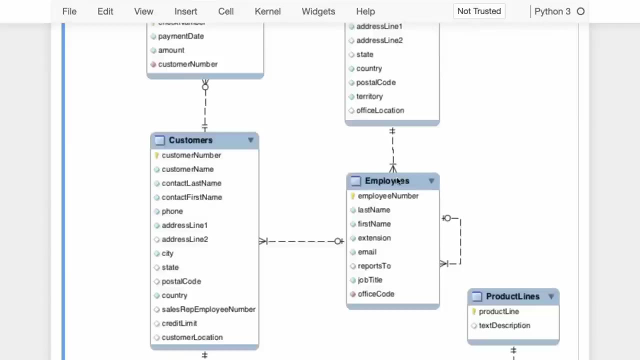 And in order number one they request product number five, product number six, product number seven, and each with a different quantity. So order details is used to track all that information. Okay, So this is how all of this fits together. You have tables with columns and then you have relationships between tables and understanding, an entity relationship. 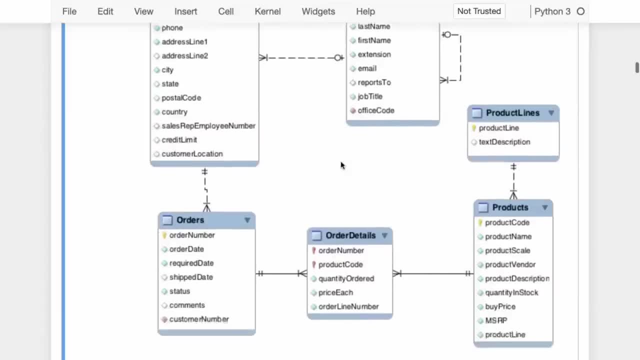 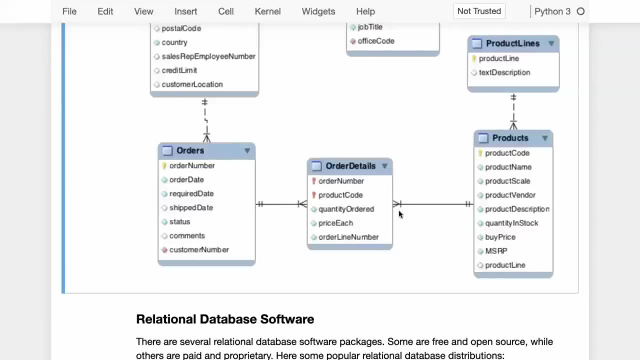 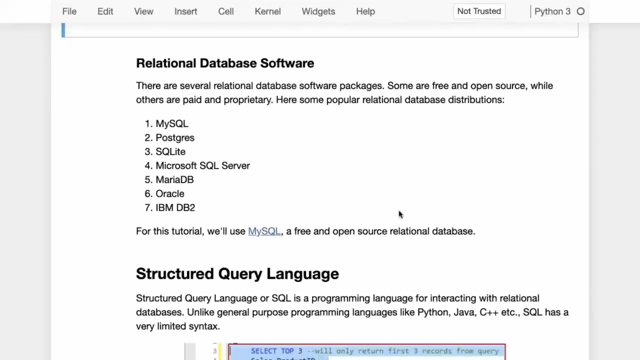 Diagram is the first step towards understanding what a database contains, And all these symbols have certain meaning, which we will talk about the next time when we talk about joins in one to many and many to one relationships. Okay, Now there are several relationship. 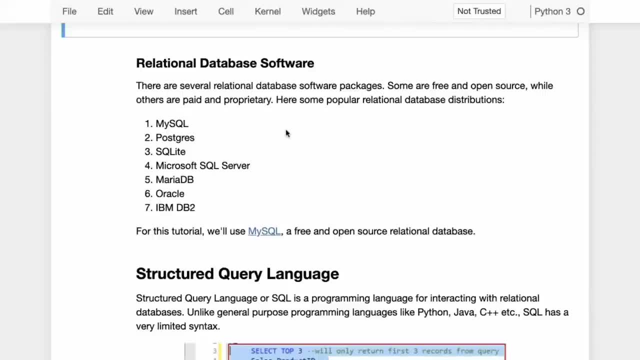 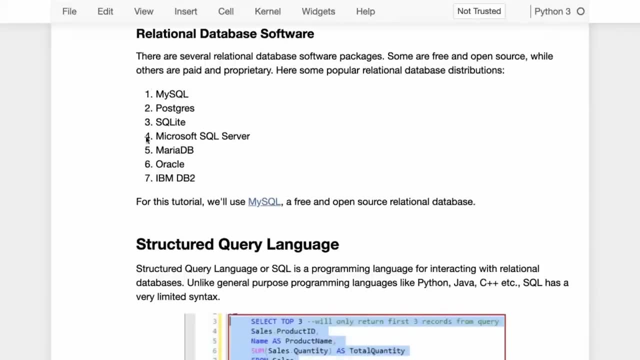 There are several relational database Software packages, And some of them are free and some of them are open source, while others are paid and proprietary, And the most common ones are these: My sequel is an open source and free option. They also have a paid option, but the free option does the job for most people. 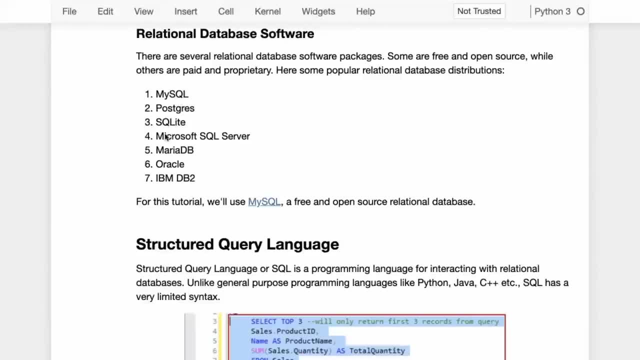 Then you have Postgres, you have SQL light, you have Microsoft SQL server, Maria DB, Oracle, IBM DB too, So some of these are proprietary. for this tutorial, We will use my SQL, a free and open source relational database software. 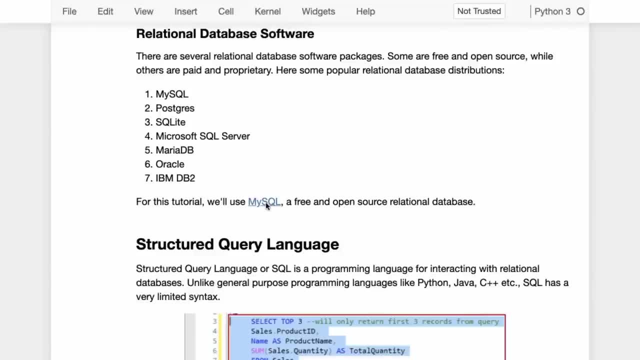 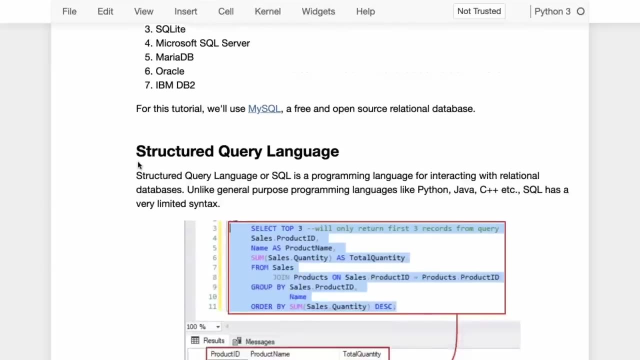 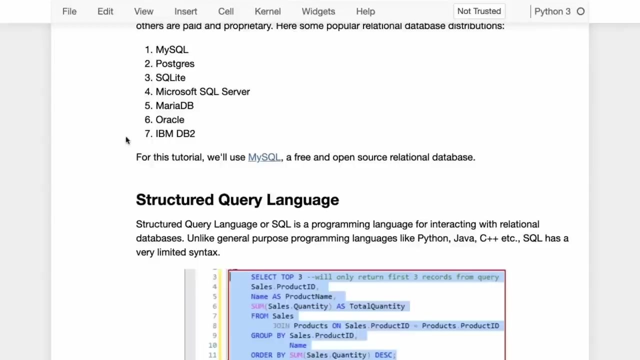 Now, the concepts that we learned today will be applicable across any of these, but the syntax, the actual code that you need to write, may differ. So just keep that in mind and just try to understand the key concepts, And we'll talk about how you can look up the differences in code, maybe by comparing, let's say, with the Postgres database, and primarily, it's simply a matter of looking it up. 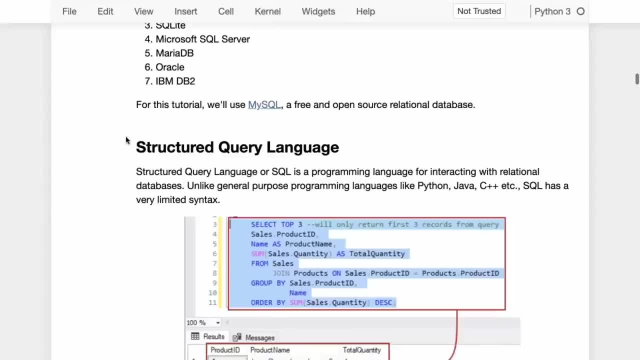 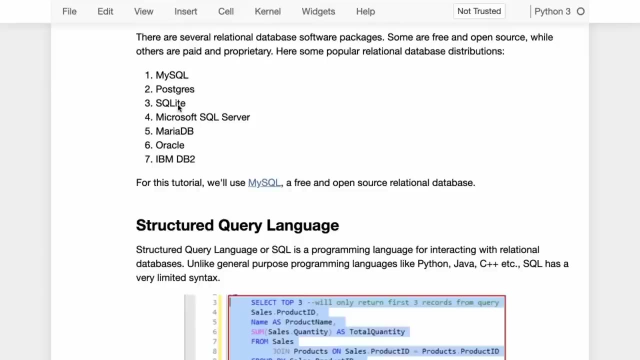 On the documentation or finding a stack overflow answer. over time, once you join a company, most companies will only use one type of database. over time You will become comfortable in the flavor or in the kind of in the software package that your company uses and the variations in SQL in the SQL language that software package requires. but your skills should be transferable across different SQL variants. 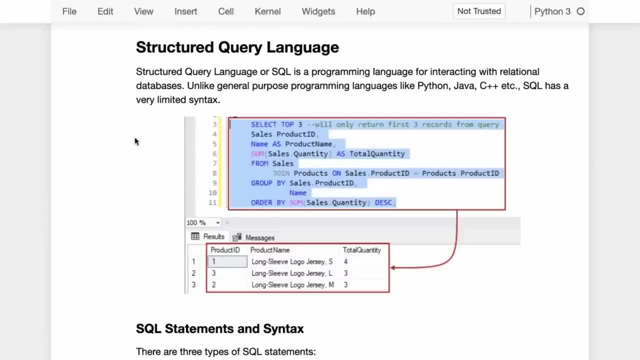 Okay, So we've been saying SQL, a lot more SQL. What is it So? SQL stands for structured query language and it is a programming language for interacting with relational databases. Now we've set up this database somewhere and now we need to put data into it and then we need to get data out of it. 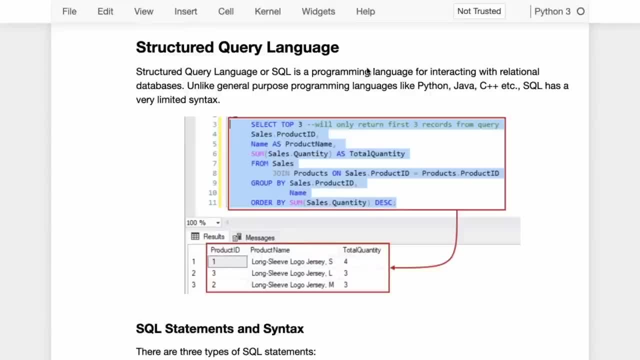 Maybe we need to change some data within it. for doing all of those things, You use the SQL programming language and, unlike general purpose programming languages like Python, Java, C, plus This, et cetera, SQL has a very limited syntax and a very specific use case. 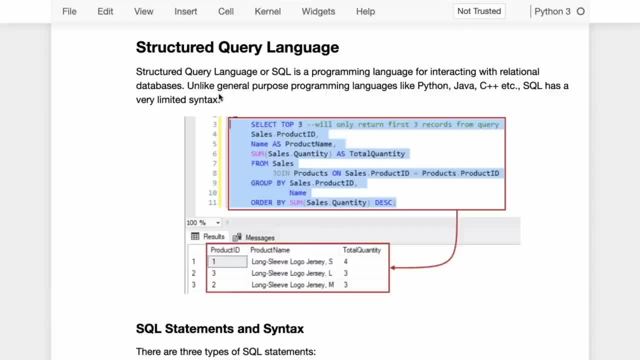 The specific use case is to interact with a relational database It's. you cannot use SQL for data visualization, For example. you cannot use SQL for building software, building web applications. You cannot use SQL for creating scripts. You cannot use SQL for machine learning. 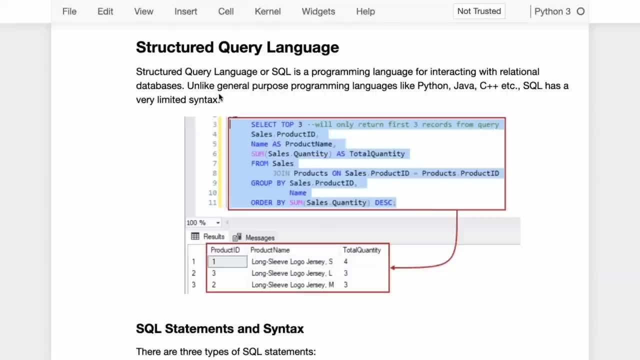 It's. that is not the purpose of SQL. The purpose of SQL is to Okay, Okay, Put data into tables, into relational database tables, and get data out of relational database tables and make changes. So it's all about working with our database, without a database. 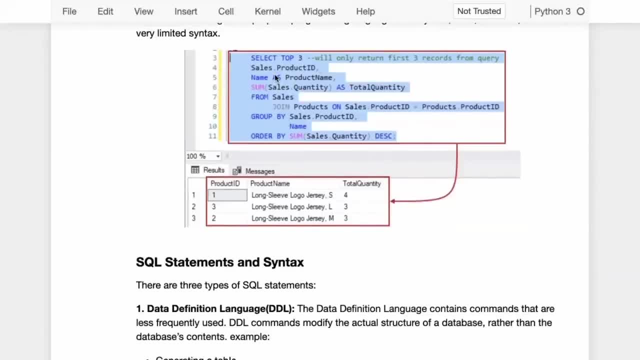 There is no SQL, And this is what it syntax looks like. So this is all one single SQL statement. It's split across multiple lines, but you will see at the end there is a semi-colon indicating the end. So here what we're saying, and SQL is a very readable language. 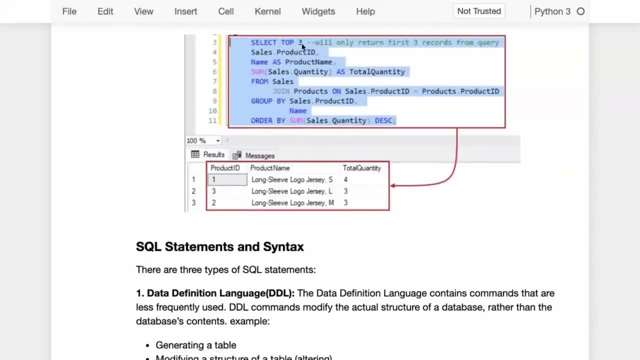 So here what we're saying is Select top three. So we want to select the top three products, So we want to select product ID from the sales table and you want to select the product name and you want to select the total quantity of products sold from the table sales. 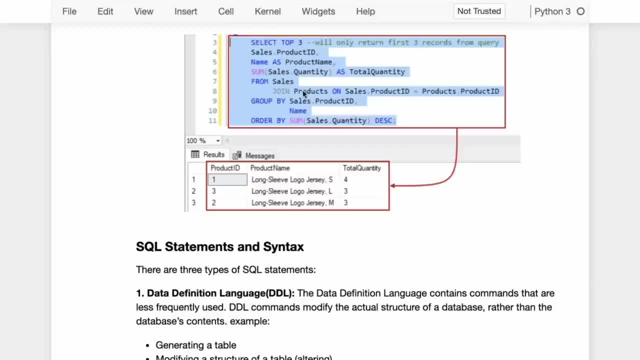 And then you want to do a join. So again there is some joining, merging involved, and then you're doing some kind of a grouping and then you're doing some kind of an order But, And then you're doing some kind of a sum and then you are sorting it in descending order. 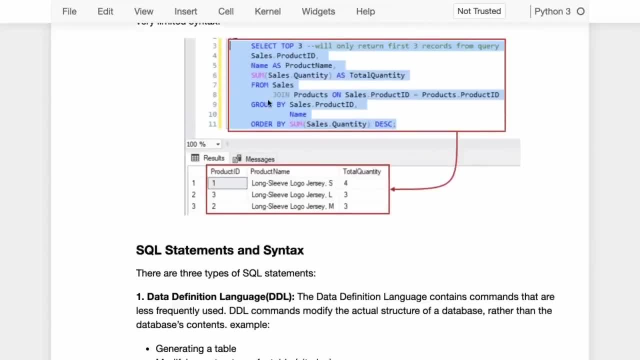 So you have all of these things that you're putting together. There are many pieces that are coming together here, and we will learn some of these pieces this week and some of these pieces next week, But by the end of these two weeks, you will be able to understand exactly what this statement does and you will be able to write statements like it. 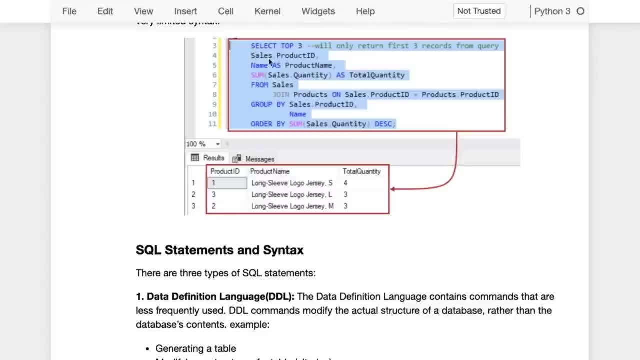 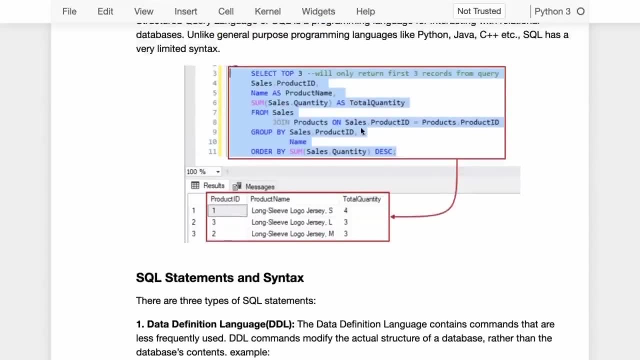 And it's not too difficult. It's just that you have to understand what each of these parts represents. Okay, And that's what we will go Step-by-step. So you type in a SQL query and you send it to the database, and then the database gives you a result. 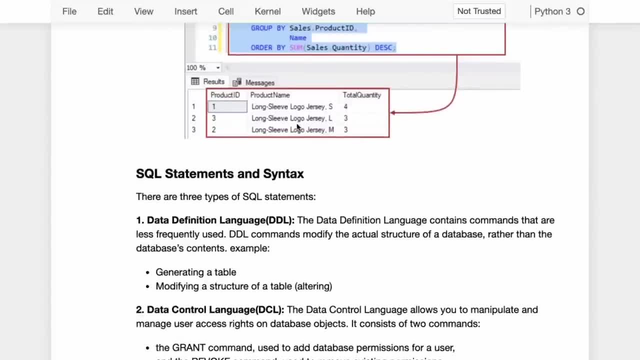 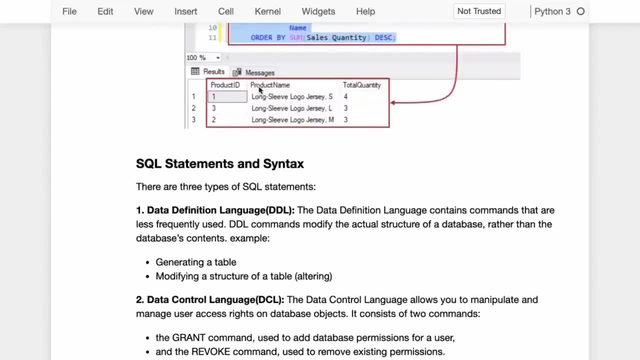 So typically it is some sort of a subset of the table, Like here: we are selecting a certain set of rules so that so the database has given just three rows of data and it has given just three columns of data. The actual table, or tables that this information has been drawn from, can contain several thousands or millions of rows and can contain several columns as well. 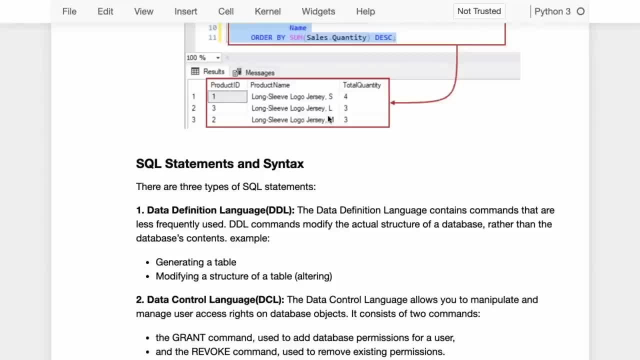 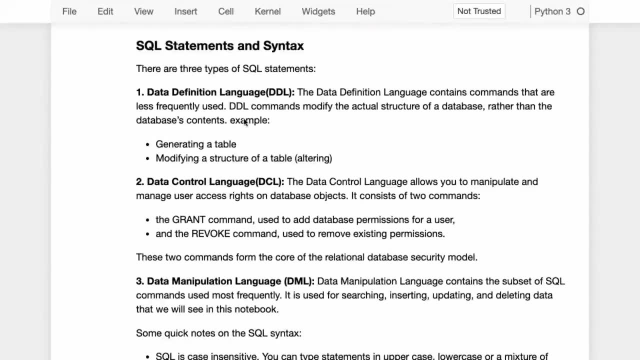 So you don't always want to see all the data. Sometimes you just want to see the data that you are concerned with, And sometimes you want also want to summarize data by taking the sum, et cetera. Okay, Now a quick note on SQL statements. 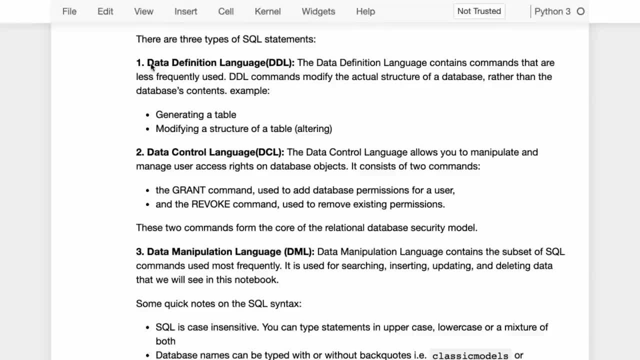 There are three types of statements in SQL. One is called the data definition language. So there are three parts. to setting up a database first, or using a database first is to set it up, which means taking the entity relationship diagram and converting it. Okay. 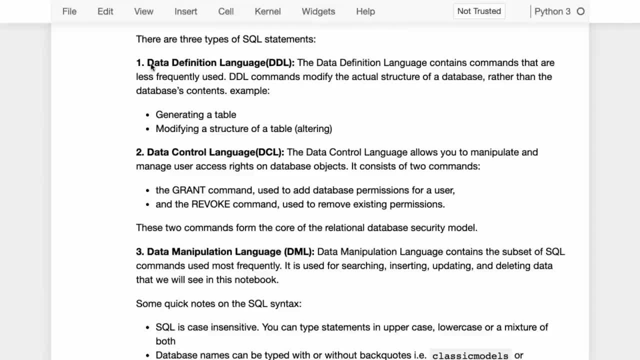 Into an actual database with actual tables, in your local copy of the software or somewhere in the cloud. Okay, So here we are concerned with generating a table, generating a database or modifying the structure of a table, making connections between tables. that is called the data definition language, or that is one of the parts of SQL. 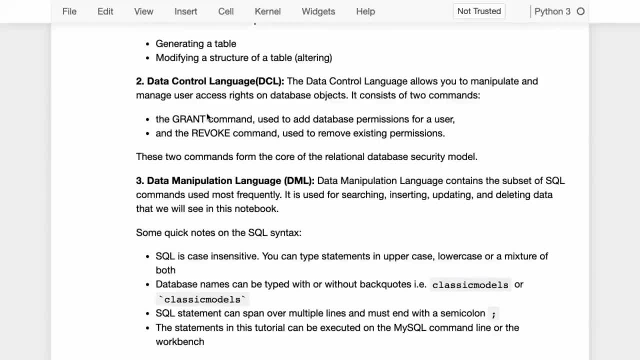 Then you have the data control language. The control language is primarily about managing user access rights. So for any database system you have a way to assign permissions to users, So you can create users and then you can give users permissions and some users may have read permission. 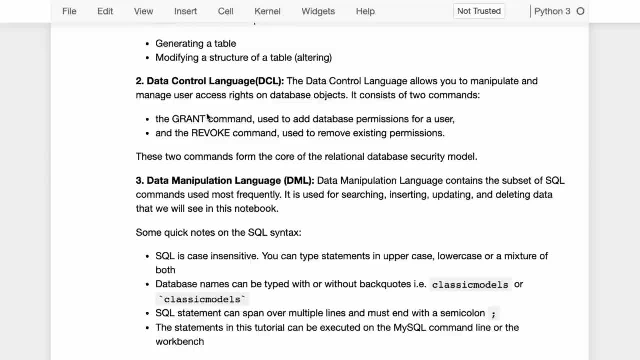 Some users may have right permissions. Sometimes you can also control information per table, so you can control who can write to, let's say, the employees table. So only the administrator should be able to create new employees, but maybe all employees should be allowed to create new customers, right. 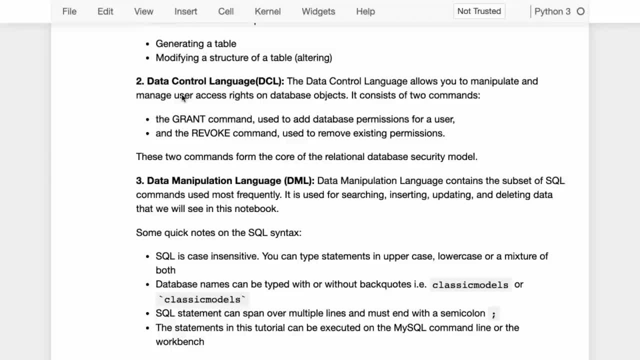 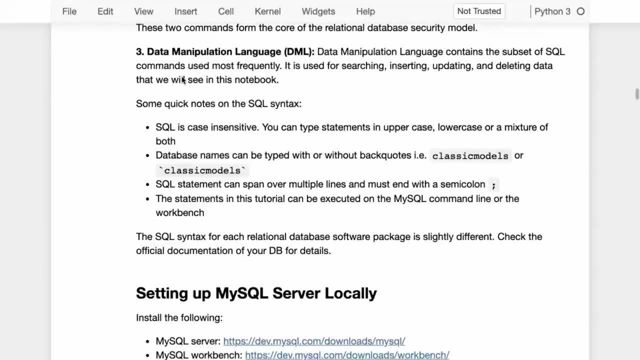 So you have all these rules, And that is also something that you Can do with SQL- not something that we will cover extensively, because this is not something that you will have to deal with. Maybe the database administrator will already set this up for you- but the most important thing that we will deal with is the data manipulation language, which talks about, which is the most frequently used subset of SQL, and it is used for searching data. 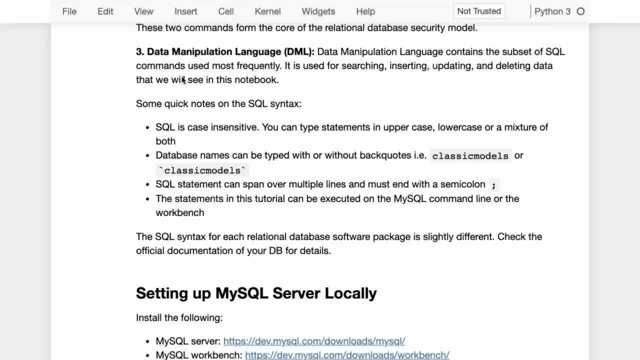 So if you have a database, getting some data out, inserting data into a database, Updating a database, updating some information that's already there and deleting data, right, So the crowd operations create, read, update and delete. Uh, those are the operations covered in the data manipulation language. 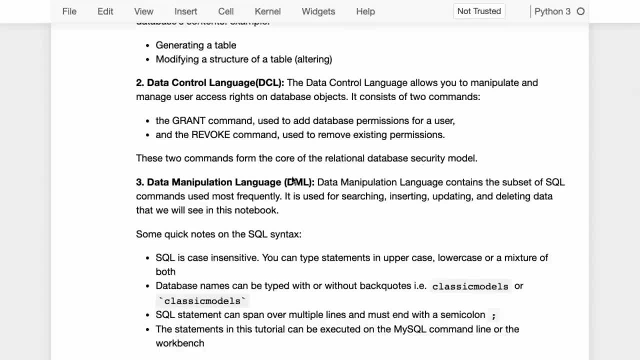 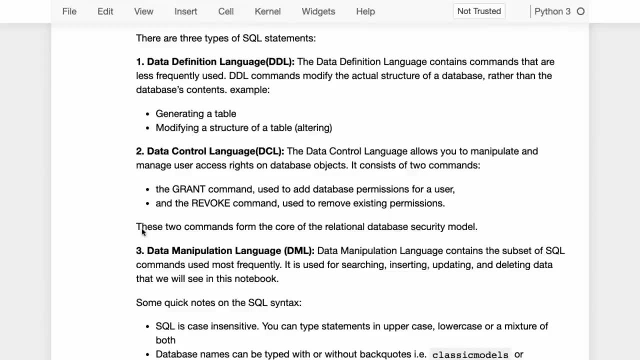 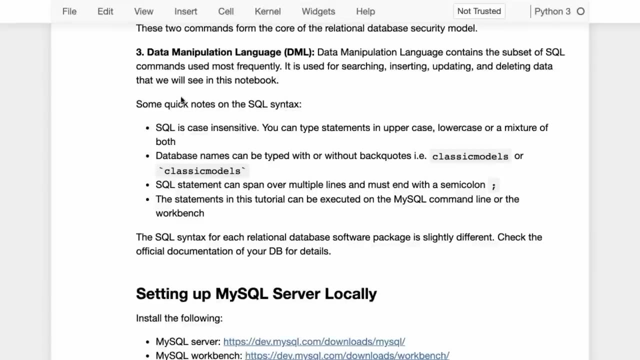 Now you don't need to really worry about these terms: DDL, DCL, DML. You never have to deal with them, but it's just that you have three. there are three ways in which we use SQL statements: to create a databases and set up the structure to manage permissions and, most importantly, to actually 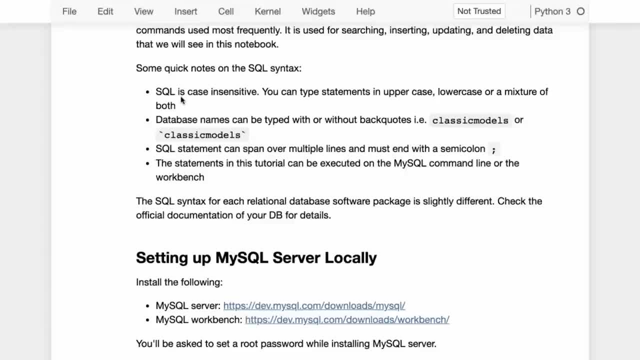 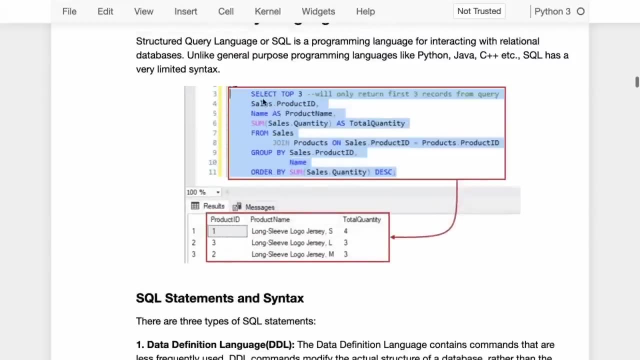 Do crowd operations on the data. And before we start writing some SQL code, a quick note on the syntax. So SQL syntax is case insensitive, which means that you can type statements in uppercase, lowercase or a mixture of both, Like here: we have select top three sales or product ID. 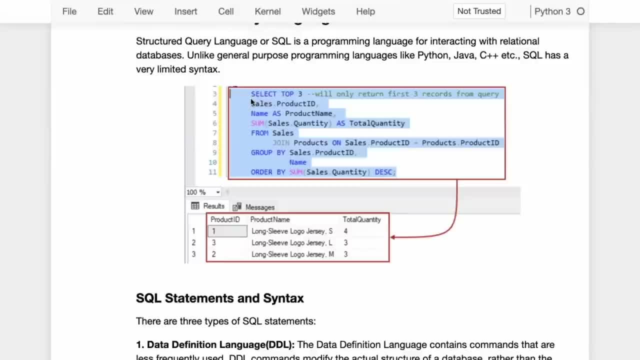 You can write select in lowercase. You can maybe write S as a- S in lowercase and E in uppercase, L in lowercase, It won't matter. Same is true with all the column names. Most of the time in most SQL distributions they are case invariant. 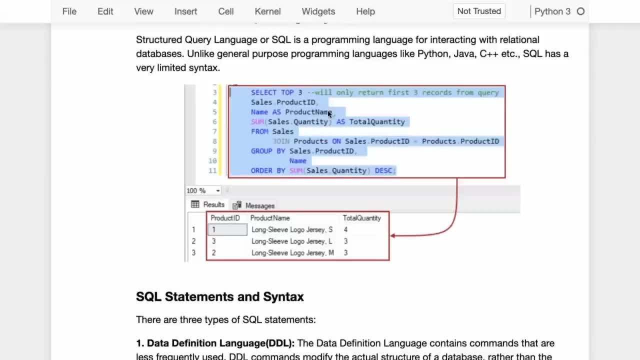 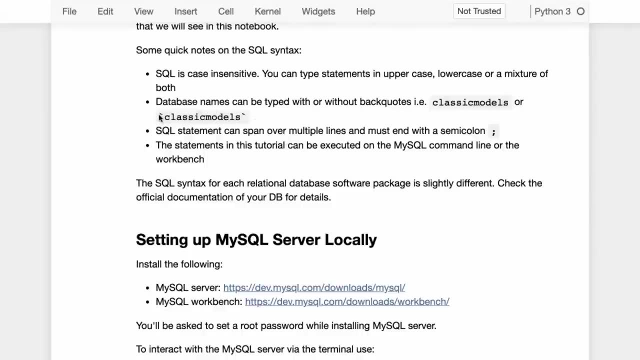 So you can use uppercase, lowercase, whatever seems more convenient to you. Okay, And one thing that you will notice is at certain places we will use these backticks or backcodes- So this is called a backcode- especially for database names and column names and table names. 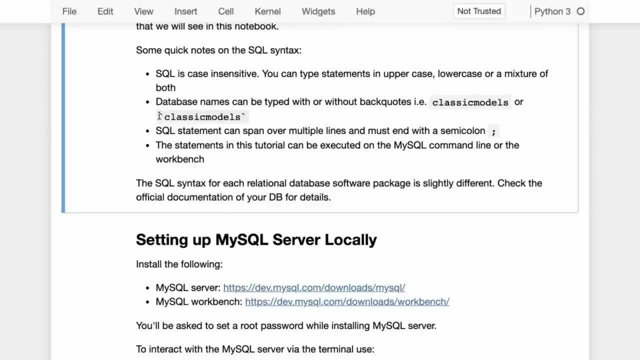 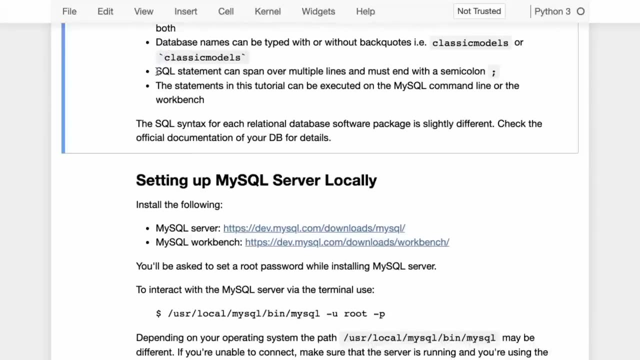 And now these are optional. So wherever you see this character, it is completely Okay, Optional. The reason it's there is primarily just to differentiate between the SQL syntax and keywords and actual table names and such. Can we see this in just a moment? then SQL statements can span over multiple lines. 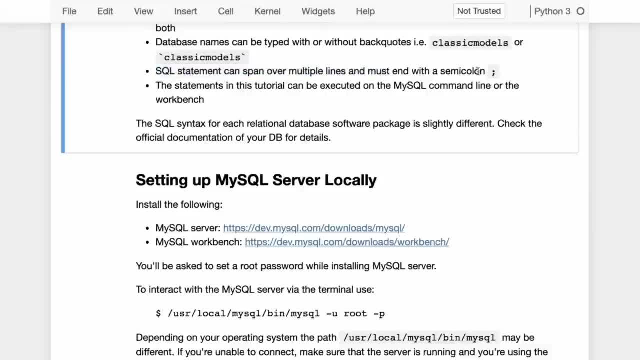 So you can write three, four, five, 10 lines in a C in a SQL statement and you have to end it with a semicolon. That's the important piece. If you don't put in a semicolon, then your statement may not get executed or the system. 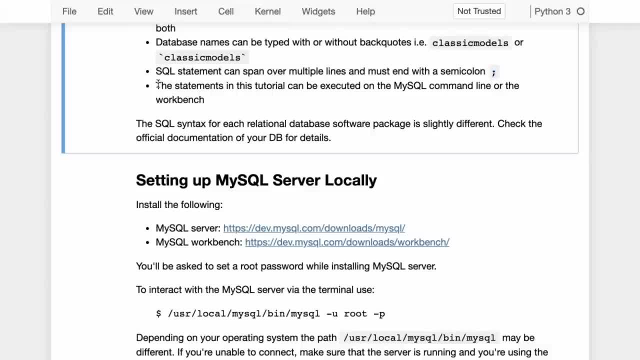 May still keep waiting for some output. And then, finally, all the statements that we are going to execute in today's tutorial can be executed on my SQL. Now, this, my SQL, can be running on your computer, It can be running somewhere on the server, and it can be accessed in two ways, which is the command line or the work bench. 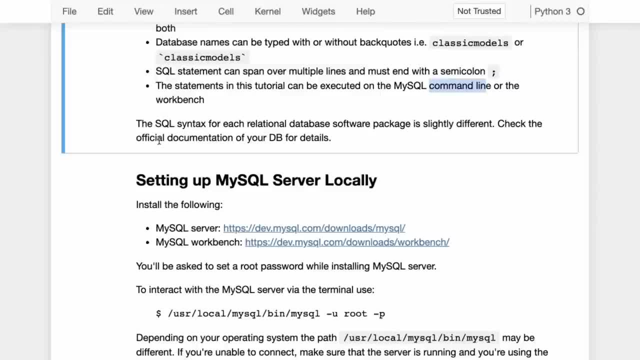 And we look at both in just a moment. Okay Now the SQL syntax, as I mentioned, for every relational database software package is slightly different. So if you're using Postgres or you're using Microsoft SQL server or Oracle, it's going to be slightly different. 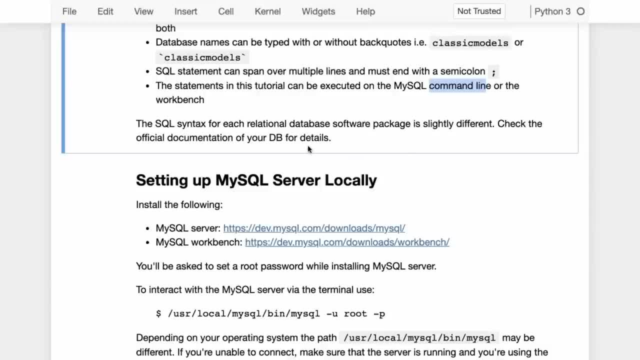 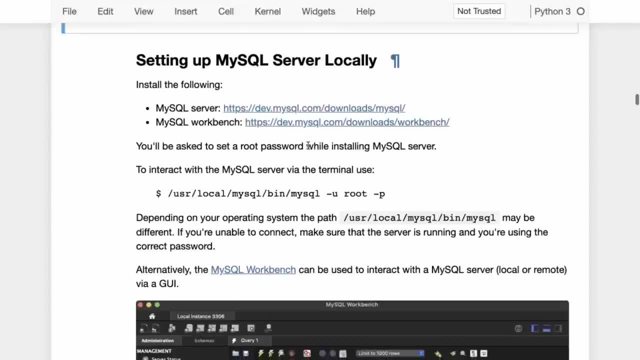 So just check the official documentation of your database for details. What we will learn is the kind of operations that you can do on database tables, And the specific syntax is just a matter of looking it up. All right, So with that, let us set up my SQL server locally. 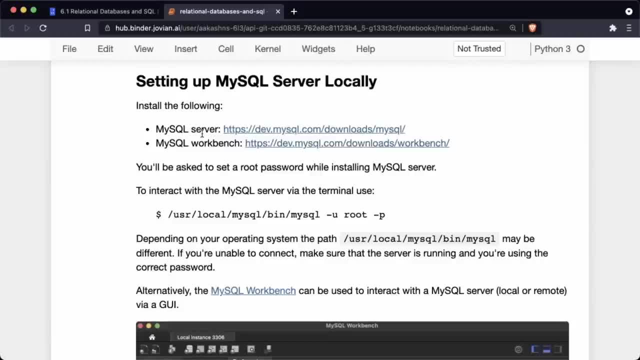 Now. you don't need to do this right now, but whenever you're following along with this notebook, definitely set it up locally on your computer, And the download takes a while. That's why I'm recommending you don't do it right now, but do set it up locally on your computer and experiment with all of this code. 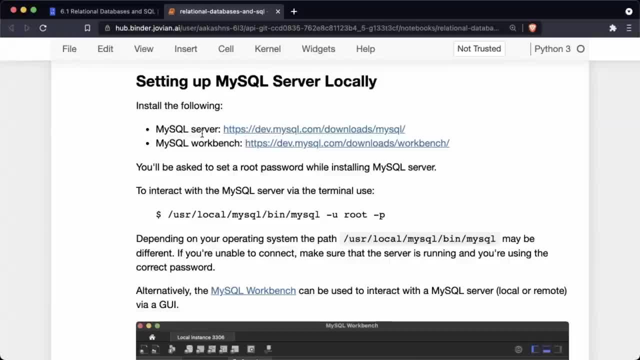 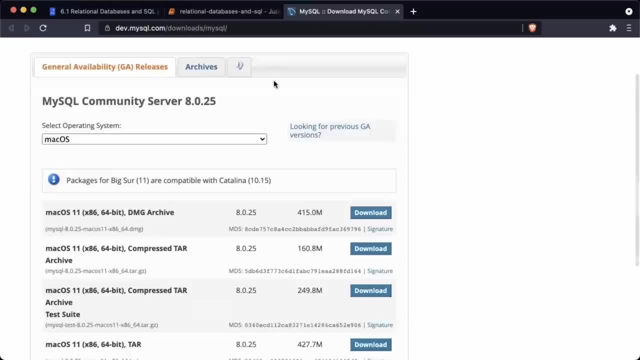 All of the things that we are doing to see the effect that these statements have. Okay, So you can download. you need two things. You need to set up the a my SQL server. So here's the my SQL server. You can go to dev dot my sqlcom, slash, download, slash my SQL and select your operating system. in my case. 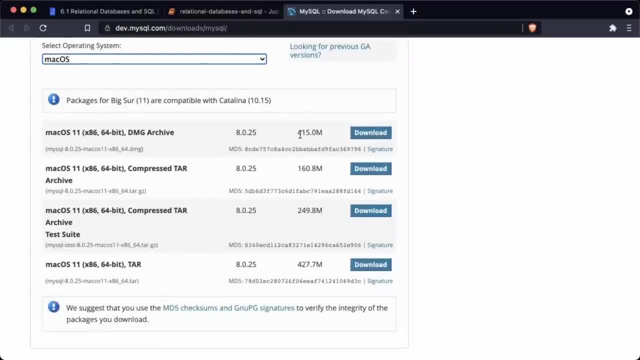 It's MacOS- and then select the kind of archive you want to download. You can see that this is a 415 MB file, So it takes a while to download. Now I've already done the download, so I don't need to do this again, but if you're on Linux, for instance, then you may want to either. 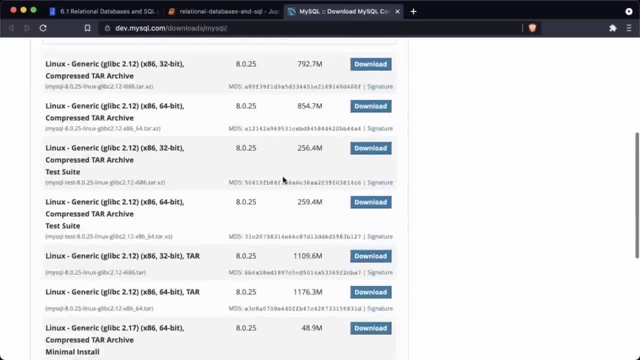 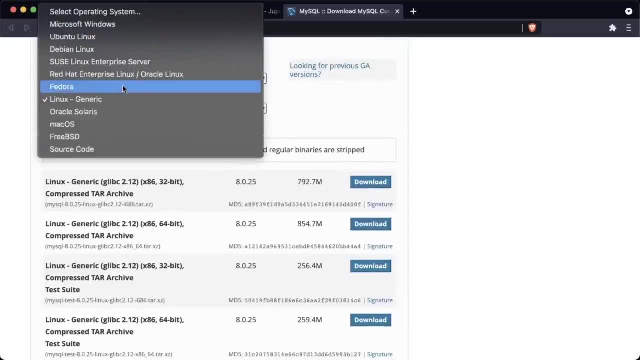 download a tar archive, or yeah, If you do download a tar archive, then you may have to follow some additional instructions as well. If you're on windows, I think you should be able to download. Yeah, you should be able to download. 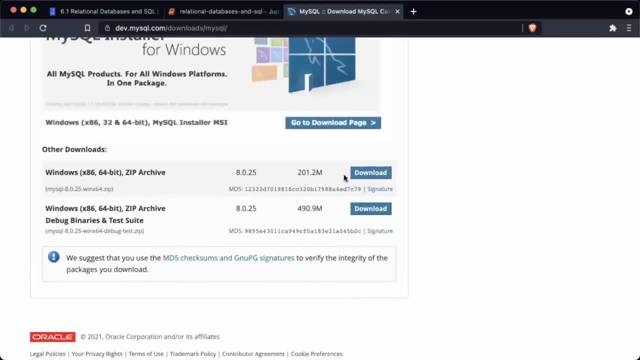 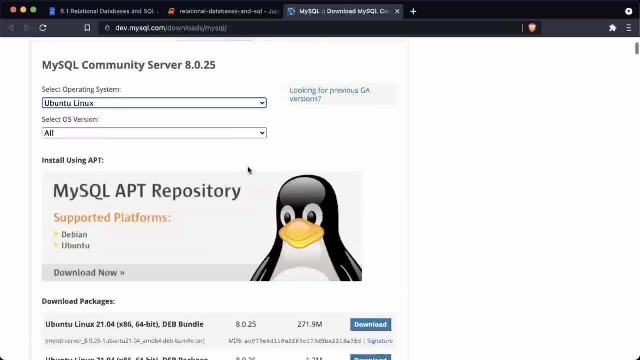 A zip archive that you can directly open up an exe on. I think on lin, on Ubuntu, you should be able to download some kind of installable bundle. So whatever operating system you're using, you should be able to download one version. Now we just need the my SQL server. 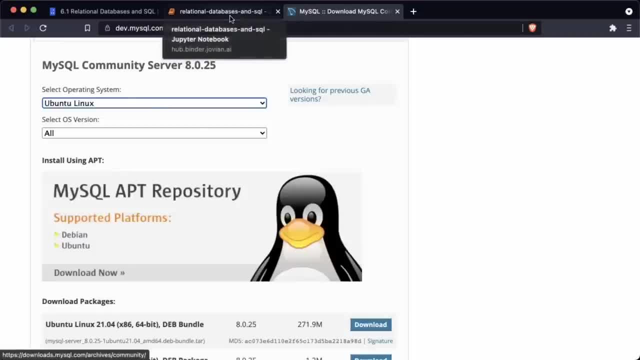 We don't need anything more than that, but and the my SQL server will set up a database for us and allow us to create tables within databases and query databases and so on, And you can run it and we are going to run it locally, but it can just as well be hosted on a server as well. 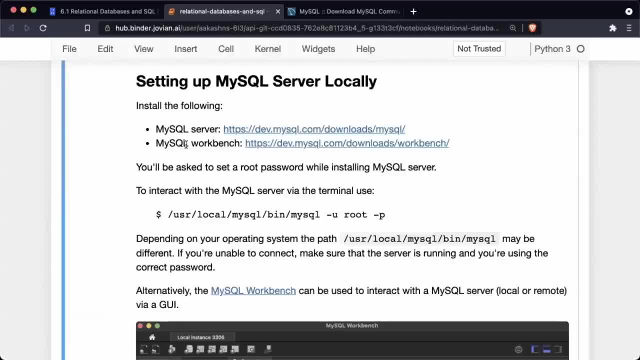 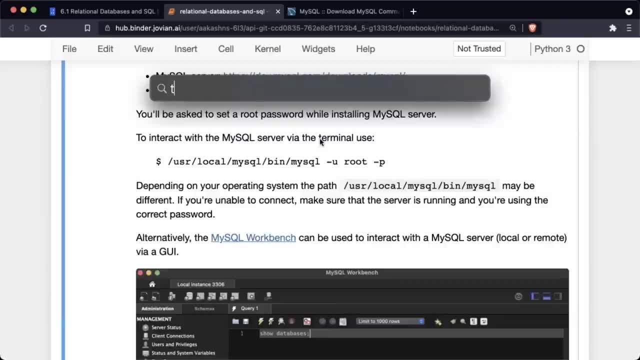 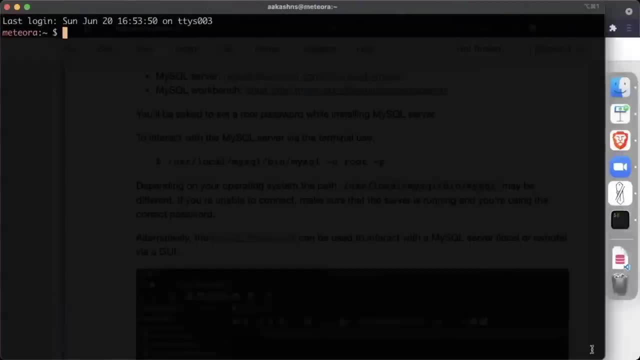 But we are going to run it locally. to interact with the my SQL server, One way is to use the command line interface. So now, in my case, I have installed it on Mac. so I'm just going to open up a terminal and let me zoom in this terminal a little bit. 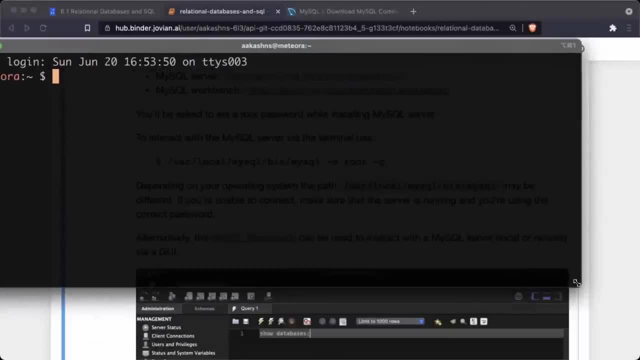 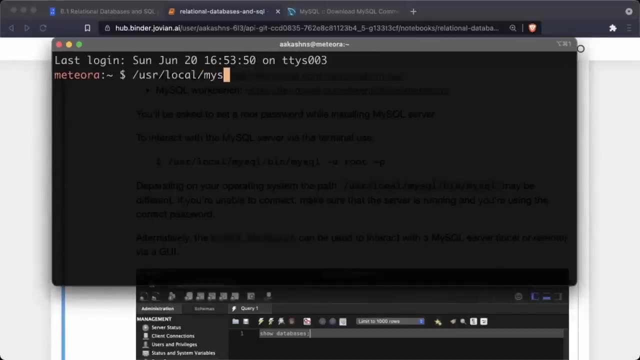 Yeah, So now I have. I opened up a terminal and when I installed my SQL after downloading it created this folder: slash USR, slash local, slash my SQL. So it created this folder and you can see this folder here, If I do LS. and where did I find this? 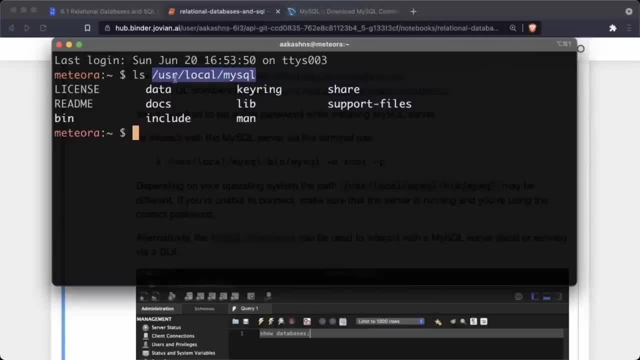 Well, I just looked it up: Where does my SQL get installed on macOS And I got this response that it's in slash USR, slash local slash- my SQL. in your case, in your operating system, This location Maybe different. This may be in C program files or this may be in somewhere else on Ubuntu. 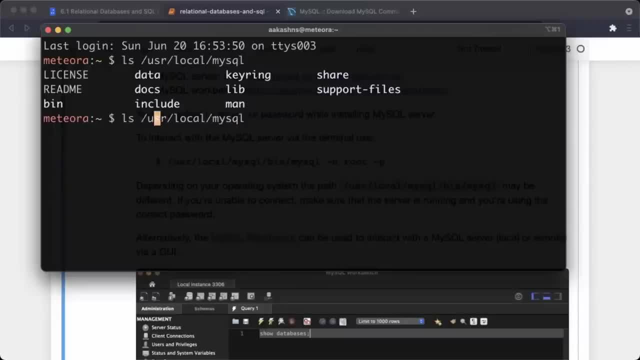 So you would have to look this up. but in this folder- slash, USR, slash, local, slash, my SQL- there is a folder called bin. So I'm just going to type slash bin here, And then there is a folder called. let me just check LS on bin. 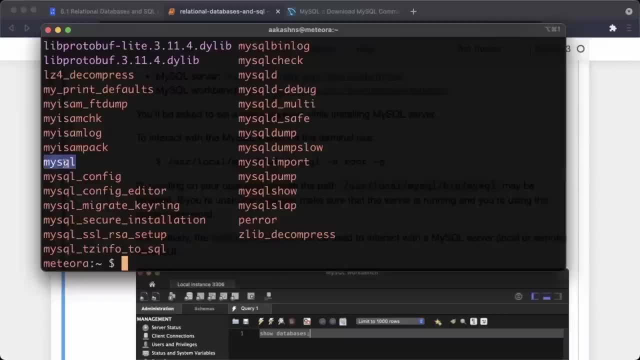 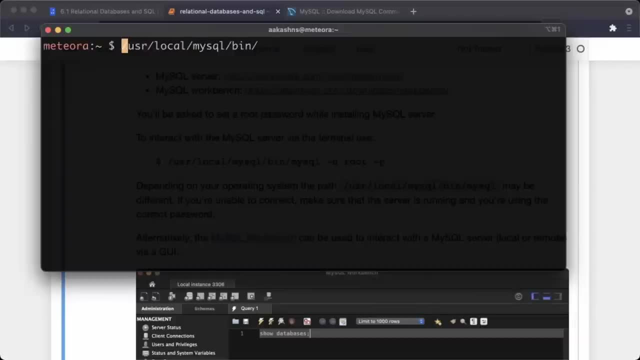 So you have a lot of things inside bin, but the one we should be concerned with is my SQL, the command line interface. So I'm just going to run Slash, user, slash, local, Slash, Slash bin, slash- my SQL. So now this is a command line tool that I'm going to run. 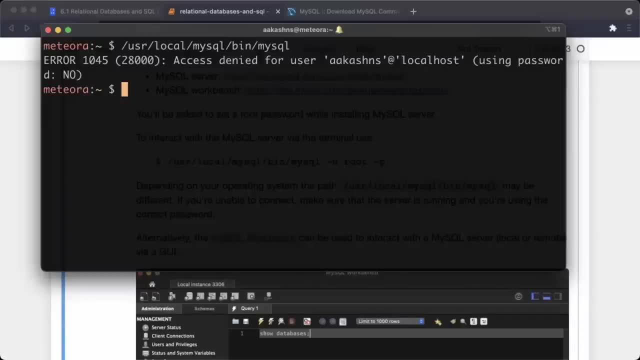 Okay, And to run this, the first thing that you will need to do is you will need to provide a username and, by default, when you install my SQL, it will have the username root, and then you also need to provide a password when you're installing. 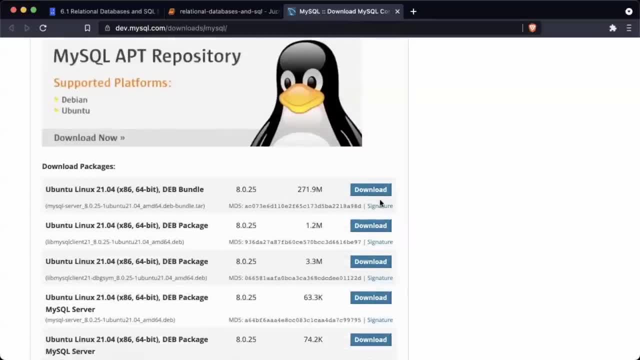 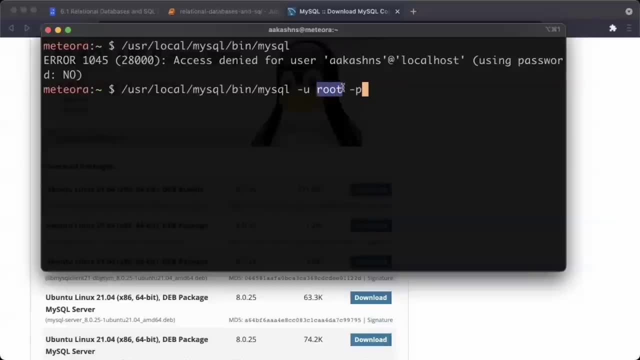 So when you download this file and then you said doing going through the installation steps, it will ask you to set a root username and a root password. In my case, I set my root username to root. That was the default option And I did set a password as well. 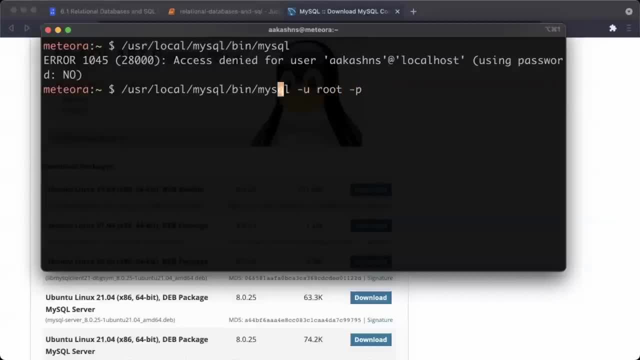 So here is how you specify the username and the password. So you say you give the path to the my SQL binary or the my SQL command line tool and you specify using minus you which user is trying to access it. And root was the default user that they had, that it had set up- and you specify minus P and it will prompt you for a password. 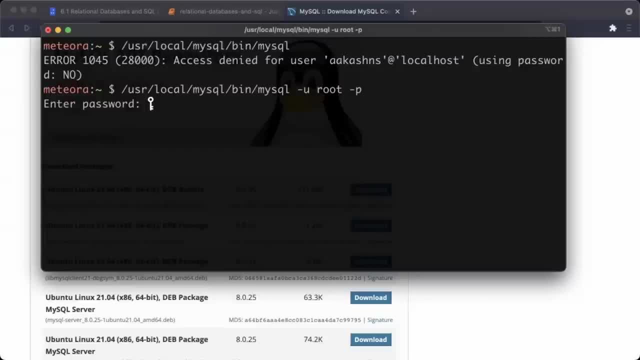 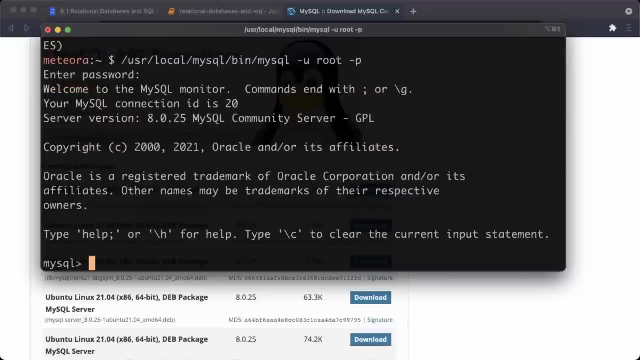 So I'm just going to type in the password here. Yeah, So I've just typed in the password now. And now what has happened is my SQL was already running on my computer after I installed it, But now I have logged in into this database server, which is running on my computer, as the user root. 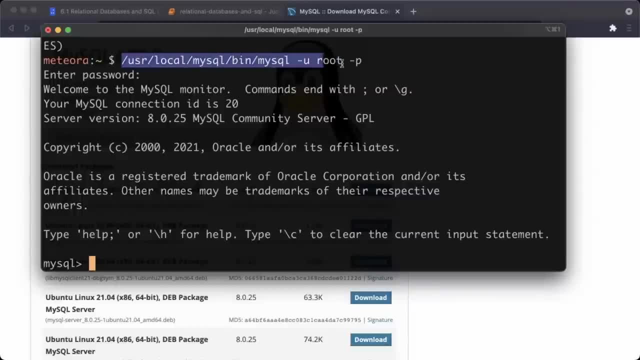 Okay, And if my SQL is not already running on your computer, then you will not be able to log in. So if you get an error here that my SQL is not running, then you would have to go and check in my case. Uh, what happens is on MacOS. 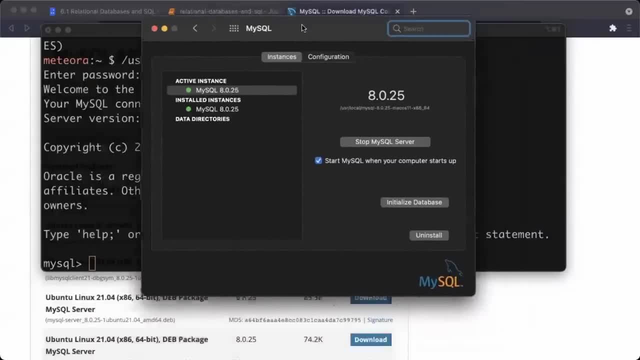 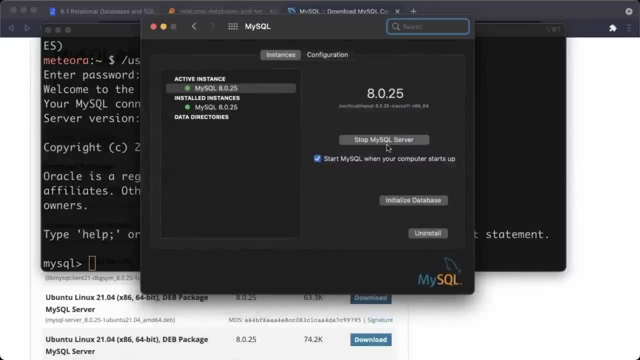 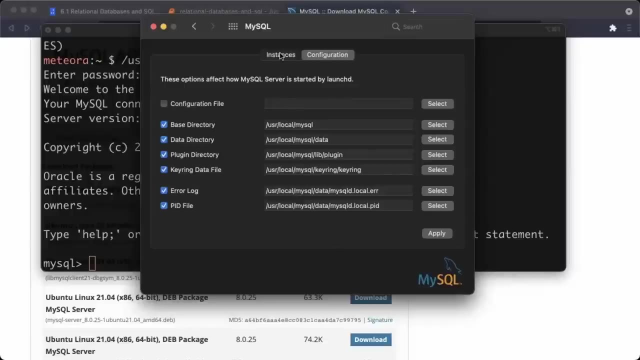 Yeah, So on MacOS it creates a. it creates this my SQL option in settings. So if I go to my system preferences it creates this option, my SQL- and here I can actually stop and Start My server. here I can also just set up some configuration about where my SQL is going to store all of its data. 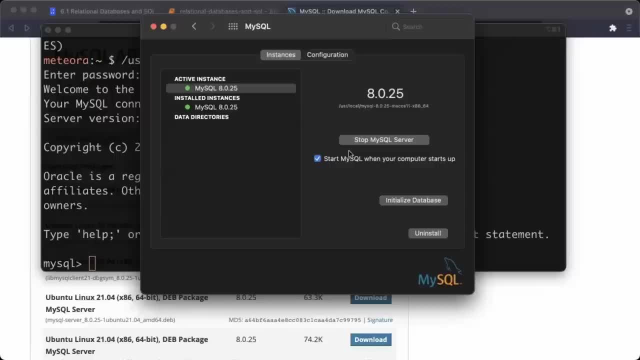 Right. So by default my SQL will start up whenever my computer starts up, So I can set all these configurations right. So the my SQL is is a application that is always running on my computer and it starts up. when the computer starts up it shuts. 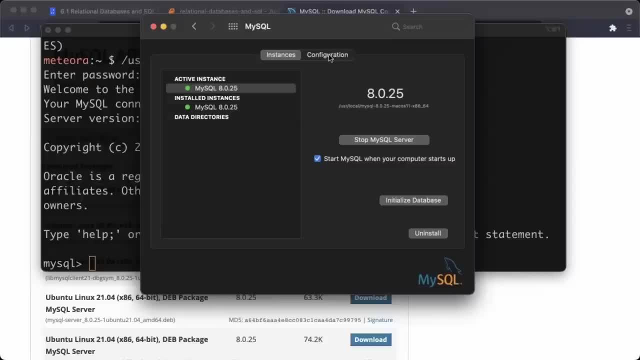 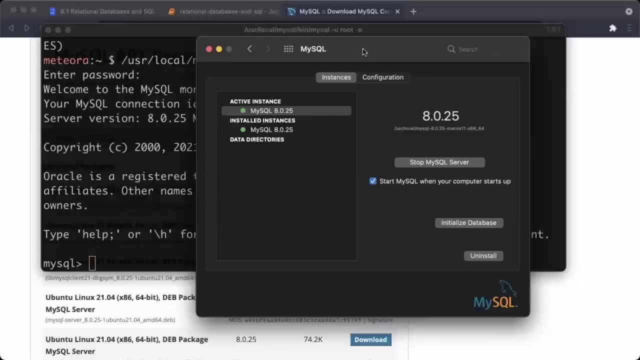 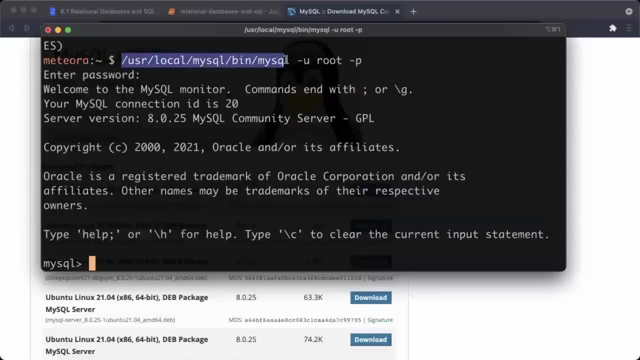 down. the computer shuts down, you will have to set it up separately on Linux or on windows, And when you do install it, normally It's all of this should be taken care of automatically. Okay, So make sure that my SQL server is running and find the path to this. my SQL binary, which is on Ubuntu. 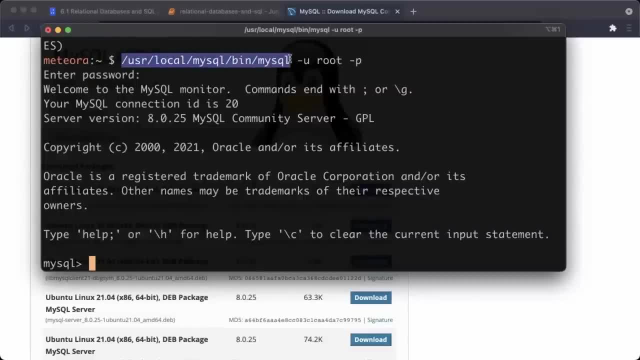 Also I think it's user local, my SQL bin, my SQL. on windows It might be slightly different- and then log in into my SQL. So log in into the server as the root user And once you've logged in into the root user, you will see a welcome message and you will see the version of the. 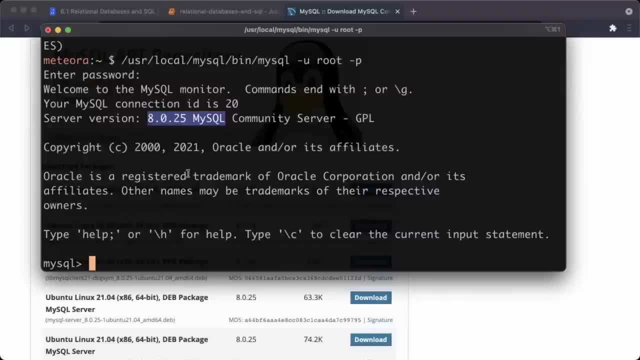 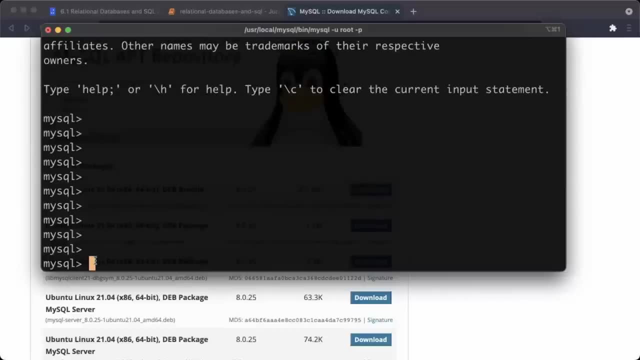 My SQL server that's running on my computer And now I can start interacting with it on this prompt. So, as you see, here it says my SQL and then I can start typing SQL commands here. Okay, So that's one way to interact with this database. 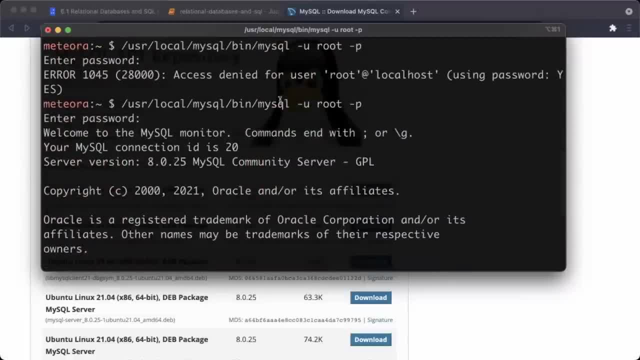 And I am currently running on my local machine, but if there was a my SQL server that was running somewhere on the cloud and I had the URL to that server, So I could also put in the URL. There's a way to specify the URL when running this tool and you can use this tool to connect to any my SQL database anywhere in the world, as long as it is publicly accessible and you know the username and password for it. 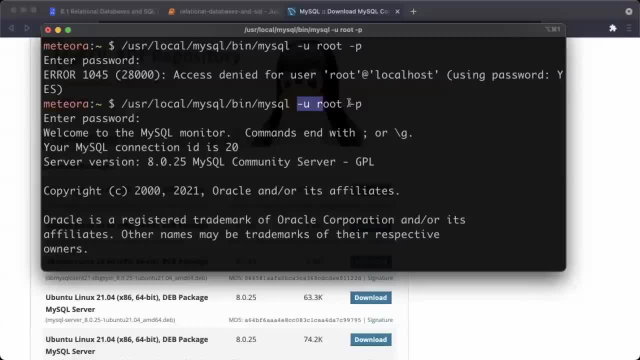 Okay, So if you have the URL to a to my SQL server, you can log in into that my SQL server as well. Like, for example, I from my computer can log in into the Jovian production my SQL server and maybe make changes to my username and things. 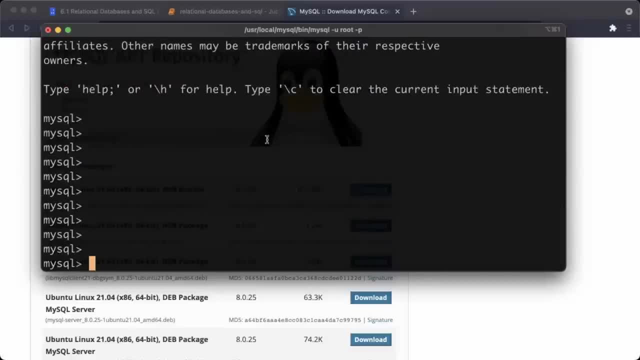 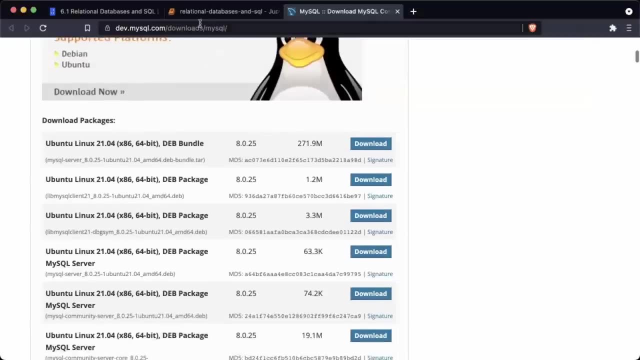 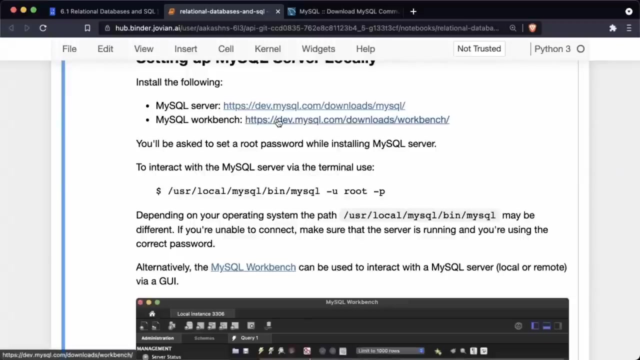 Like that. Okay, All right, So that is one way to access my SQL. That is one way we will look at today, but another way to access my SQL is using the my SQL work bench. So there is another installation link that we've included here. 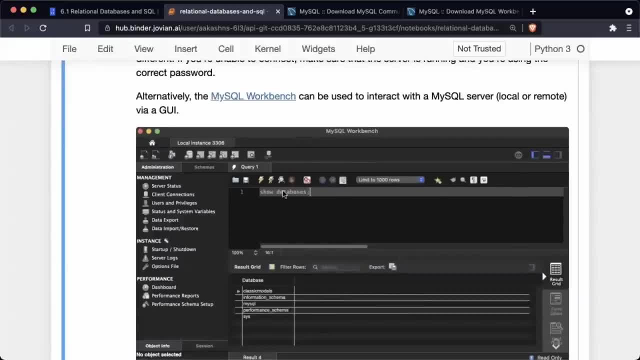 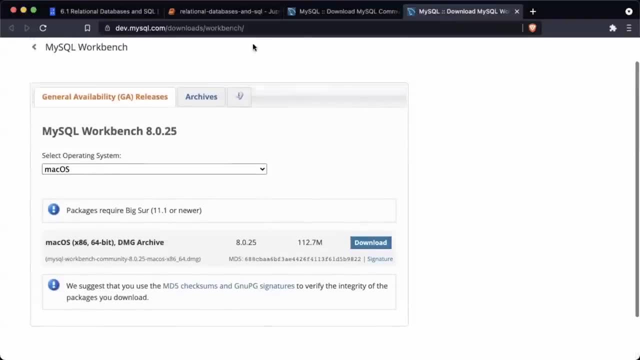 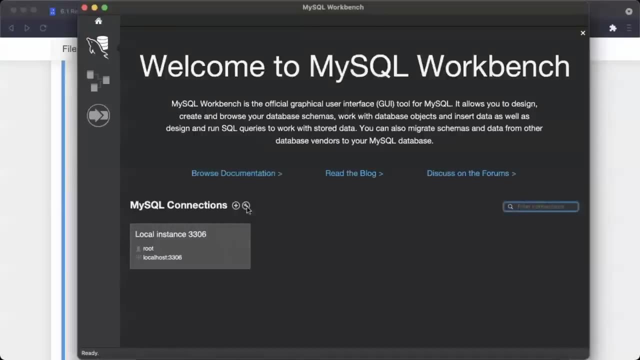 This is to download the work bench, which is basically this graphical user interface. So you can download the work bench. This is a again a hundred MB download And The work bench also. let me open it up. The work bench also connects to a my SQL server. 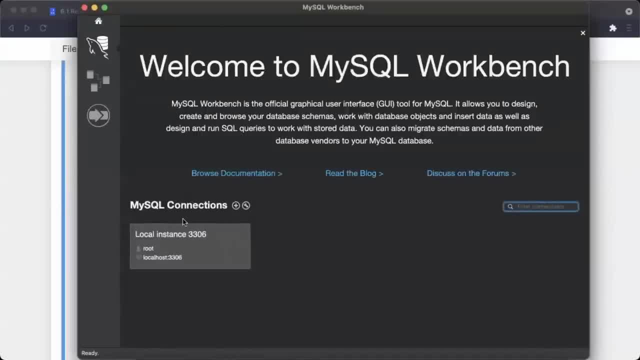 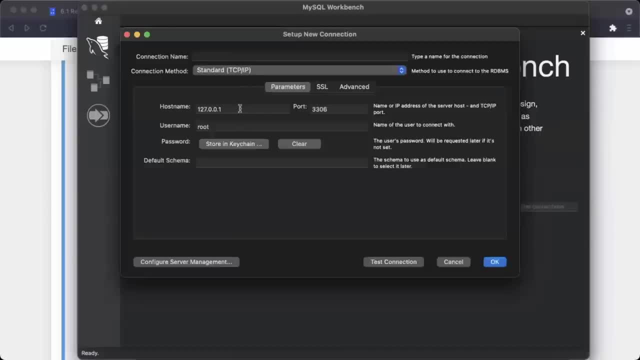 So when you log in for the first time, you will see that it automatically detects that you have a my SQL server running locally. But if you want, you can also connect to something that is running somewhere on the cloud. So again, if you have the IP address or if you have the host name, if you have what port it is running at, if you have the, 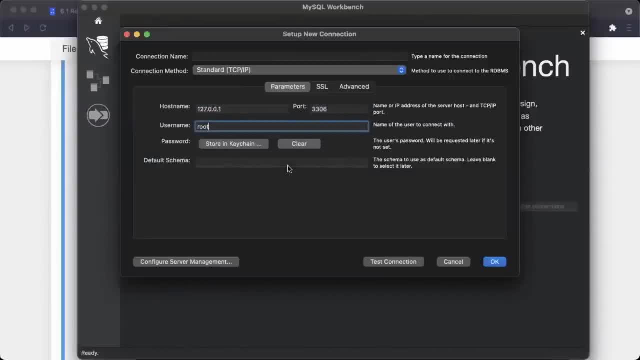 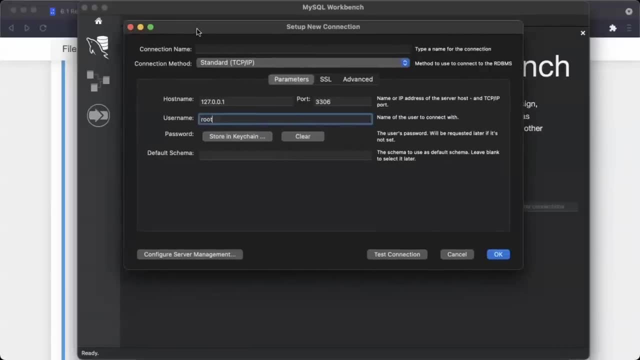 username and password for a database server running on the cloud, then you can get those details, You can connect to that database. So typically in a company setting, what will happen is the team that you're working with or the person that you're reporting you that you're. 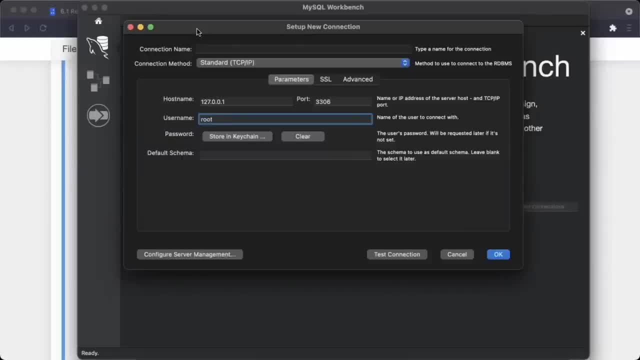 reporting to will tell you that here is where our database lives. So you should set this IP for our database. You should set this port. You should use this username. We have created a username for you. You should set this password and then you should. then you can click connect, or you can even test the connection first and then you can click connect. 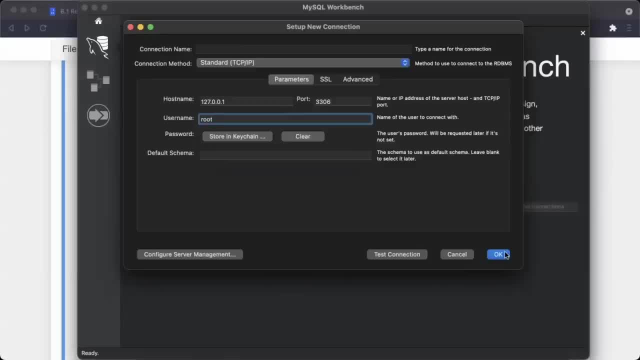 And Then you will automatically get connected to the company database and then you can work on the company database or your team's database and get data out of it or write data into it, do queries on it. In our case, today, we are going to just use the local installation that we have of my SQL. 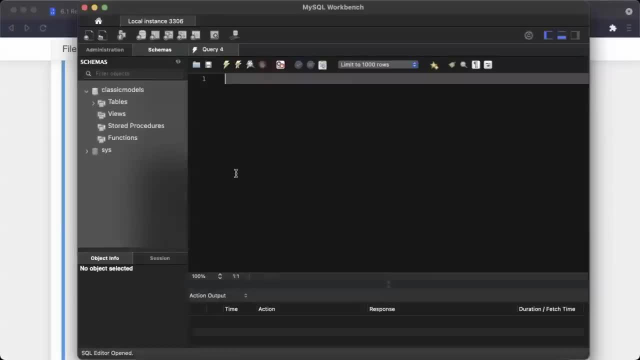 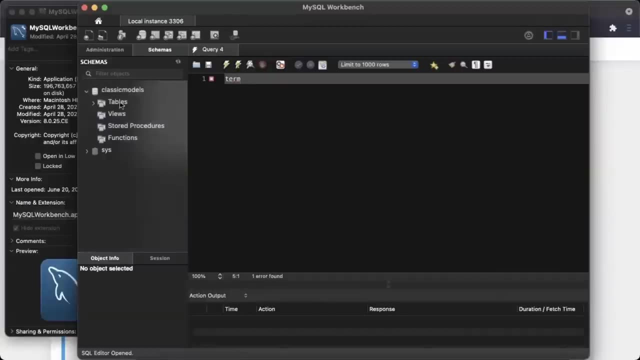 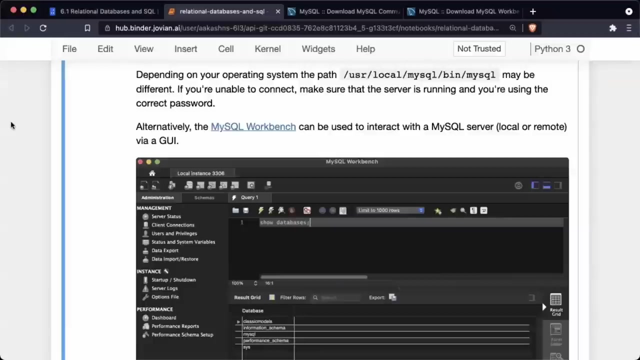 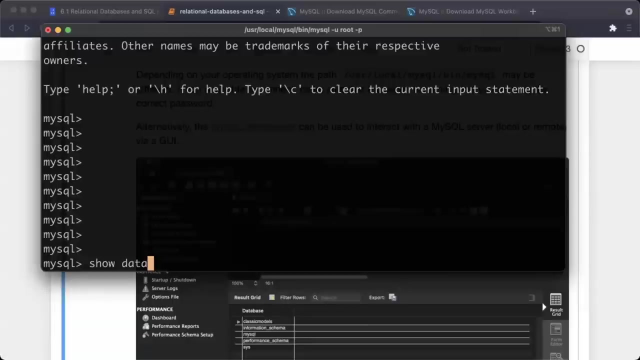 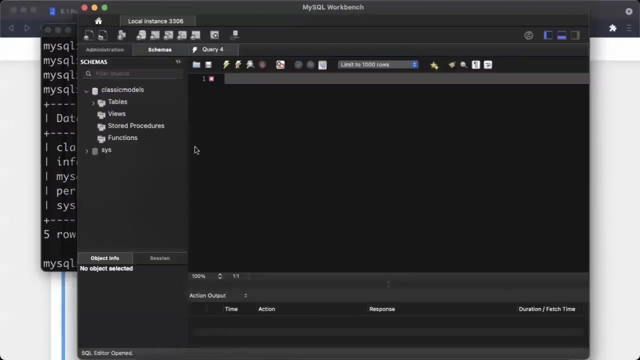 So I'm just going to connect my SQL workbench to the local installation, All right. So this is what it looks like and the kind of queries that you type here, for example, I can type a query. So, for example, I can type a query here on the my SQL command line tool, show databases, and I can type the same query here in the my SQL workbench, show databases, and then I can run it. 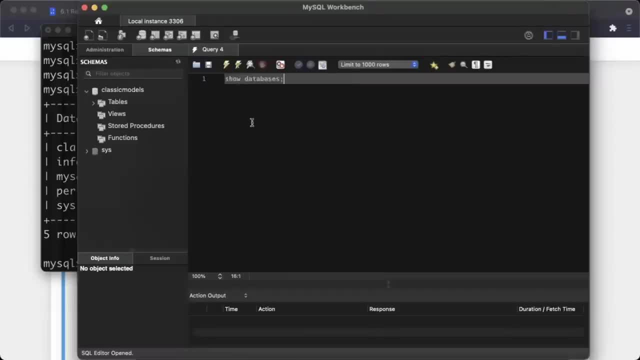 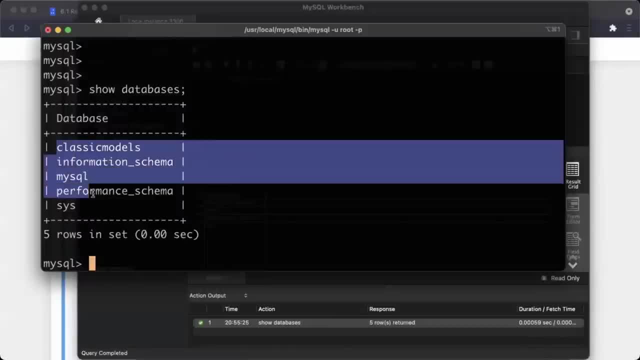 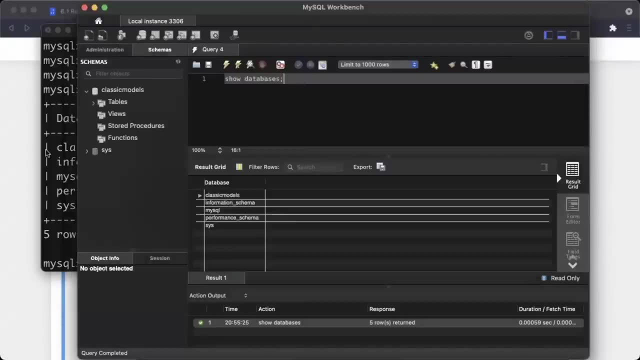 And it shows the same information. So here it says: shows the information, classic models, information schema, my SQL performance schema, et cetera, And here it shows the same information as a table. Okay, So it's just a little nicer here. 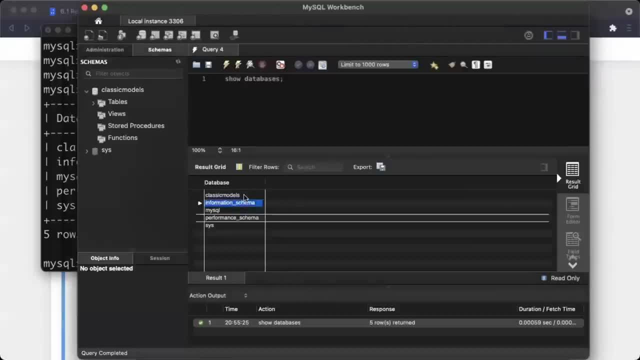 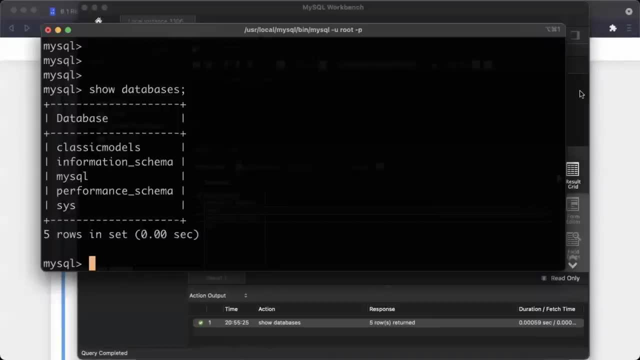 Everything is shown as text here. You can interact with it a little bit. You can click on things and such. So those they are just two different ways of interacting with the same underlying database that's running locally Right now, And both of these can also connect to things on the cloud. 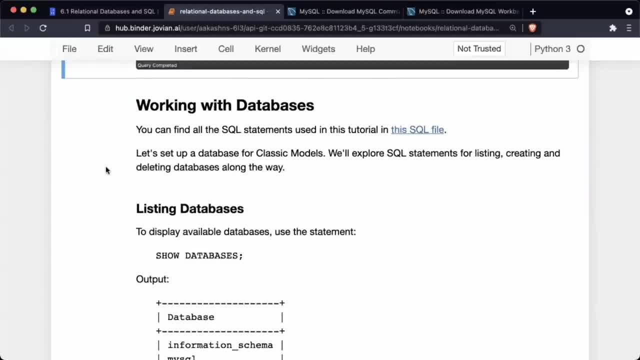 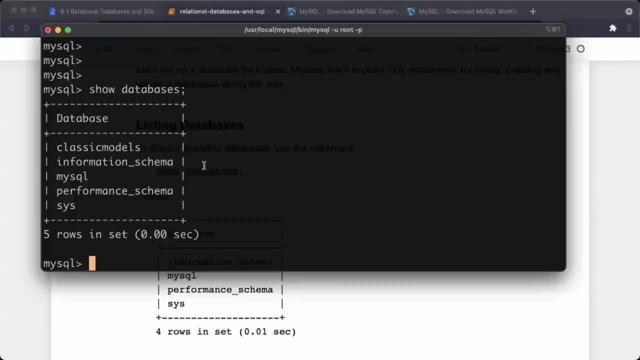 Okay. So with that out of the way, we can finally start working with databases. So let us set up a database for classic models. In my case, I have already set up a database. Let me just remove that database for now. Okay, 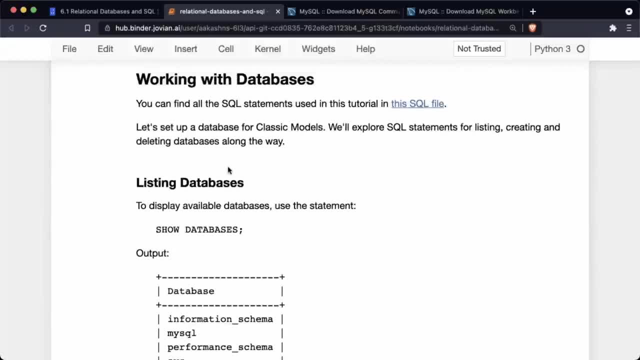 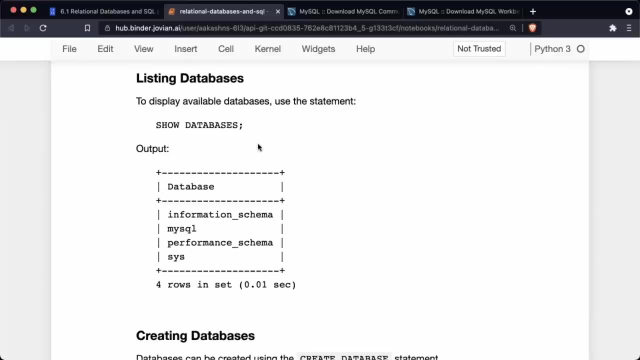 All right. So Once you are connected, either through the command line or using the my SQL workbench, to a SQL server, So the server could again could be running locally or on the cloud- you can start writing SQL statements. So the first thing that you want to do as soon as you're connected to a database server is to just list the databases. 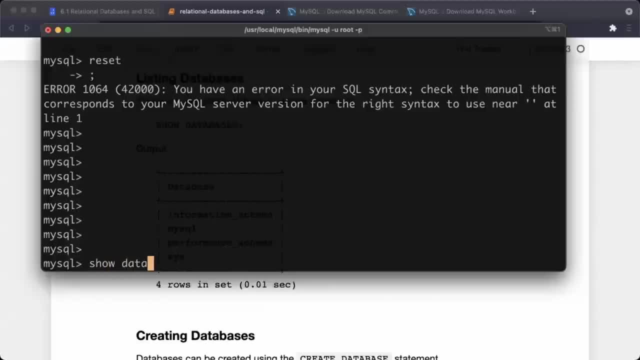 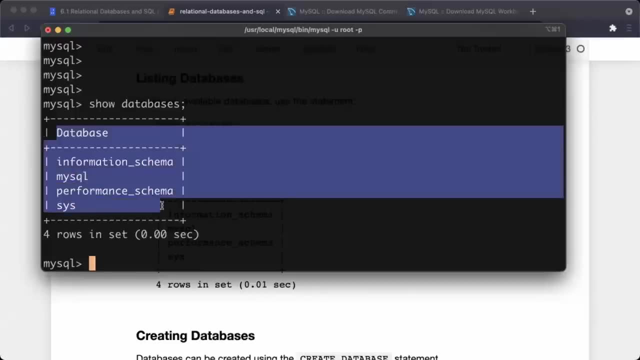 that are present on the server. So I can just type show databases and put a semi-colon and that is going to show me the list Of databases that are present on the server. So by default right now I've just set up this- my SQL server- on my computer. 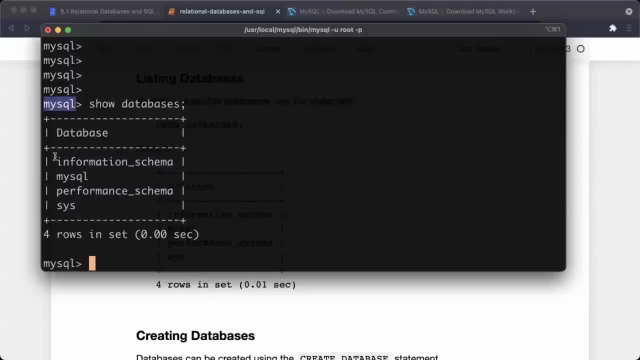 So these are all some of the default databases that my SQL already has, So we definitely don't want to disturb any of these, which is information schema, my SQL performance schema and SIS. Okay, But once you create more databases, you will start to see those databases showing up here. 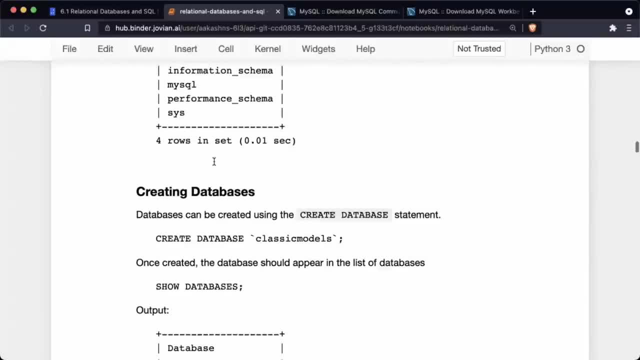 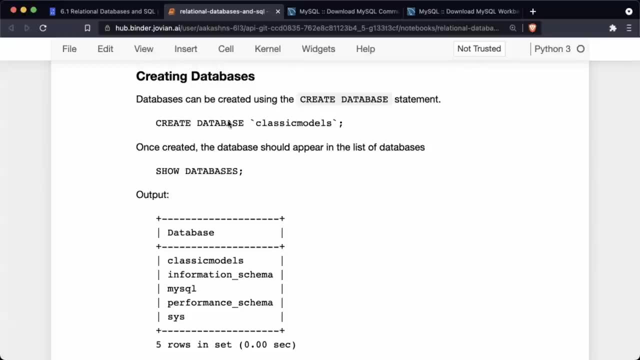 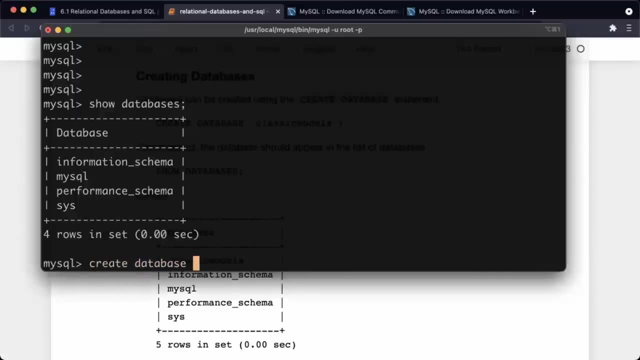 So that's the first thing: show database is going to show you a list of databases. Then the next thing you can do is Create. you can create databases. so here is how you create a database, your type, create database and then you type the database name. 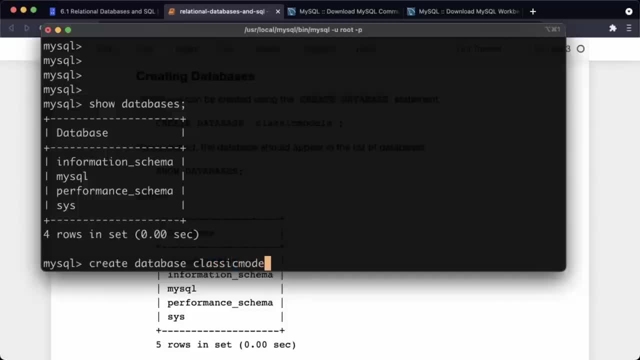 So I'm going to create a database- classic models- and let me just run the statements. I've typed create, I've typed database and I've typed the name of the database- classic models- and now the database is created and I can check show databases. 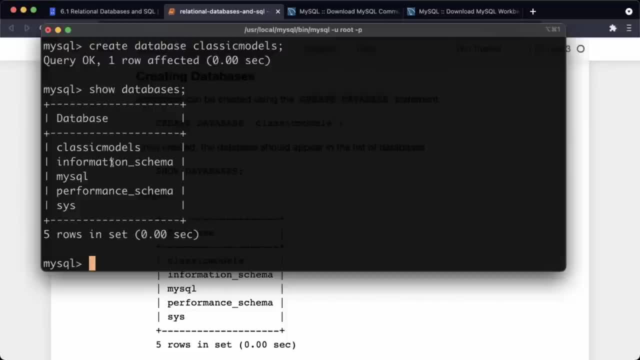 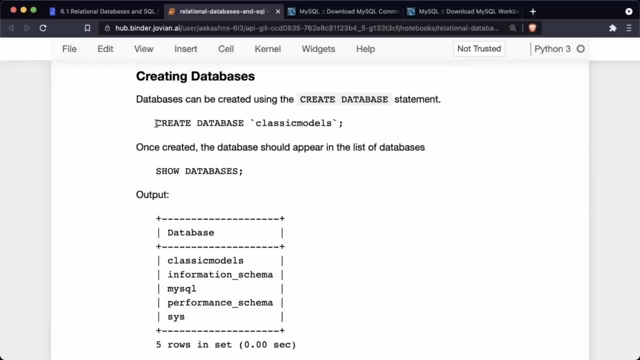 Once again- and now you see you have classic models here as a new database that has been created. Now in this notebook, what you will see is the statements are typed in uppercase- create databases uppercase. And one other thing you will notice is that all database names, column names, table names- all of these are lowercase. 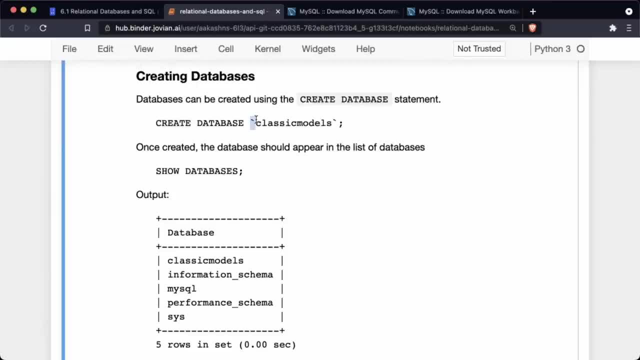 And they are indicated with these back ticks. This is called a back tick. This is just for Visual separation, So that you know that this Is a, this is a SQL keyword and this is the name of a column or a database or a table. 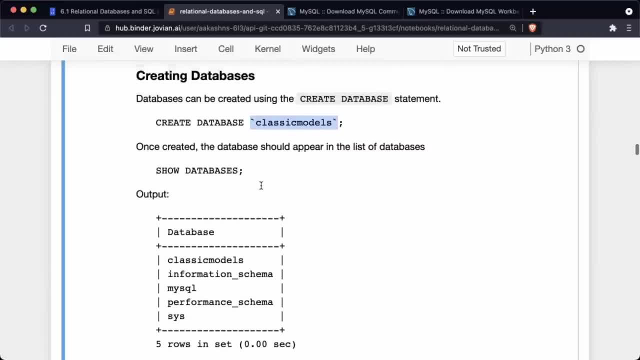 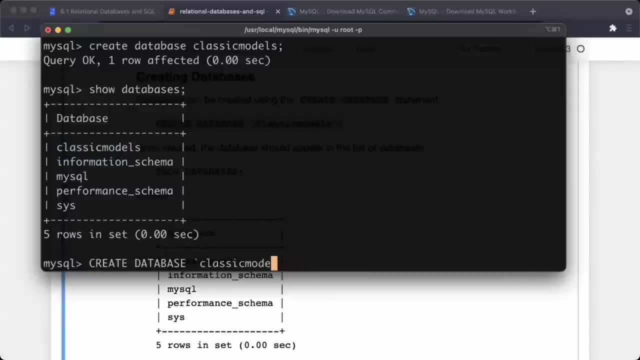 So this is just for that visual separation, so that when you're going through this notebook it's clear to you and you can also run it like this: You can take this code and you can run it exactly the same way as it is typed here, or you can type it without any of the back ticks and just in lowercase. 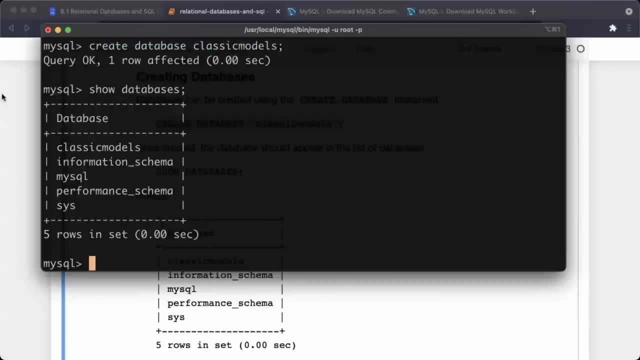 And this is also perfectly fine, except that it's a bit difficult to read. Okay, So now that we've created the database, we can now show the data. We can create a database as well, grade, and if we try to create it again, my SQL will give us an error. 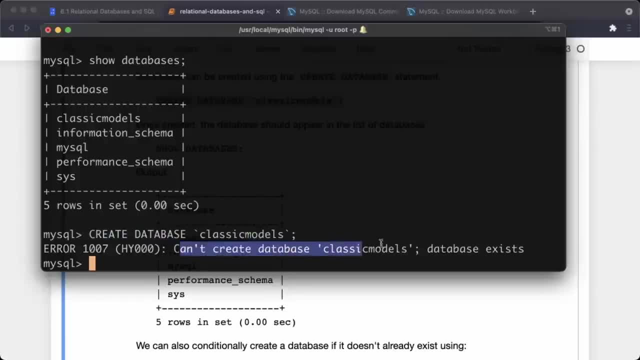 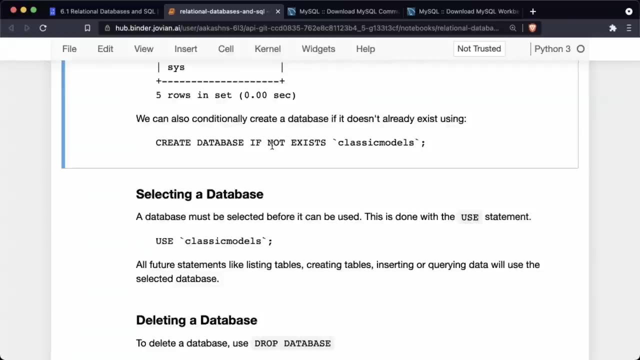 So you can see here we run create database, classic models, and it says it can't create a database because the database already exists. So we can also specify a condition to create the database only if it doesn't already exist. So if we say, create database if not exists classic models, 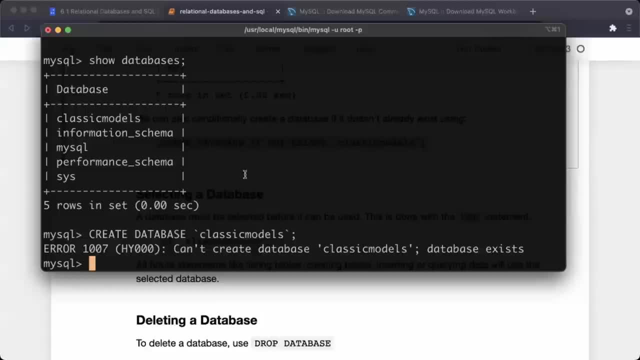 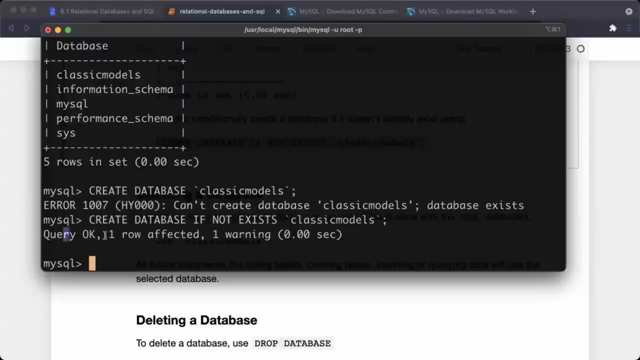 So this is when we don't know if the, if the, if there's already a database with that name on our server, so then we can create that database If it does not exist. if it does exist, then nothing happens. So if we type this: create database, if not exists, you can say: you can see that it says query. 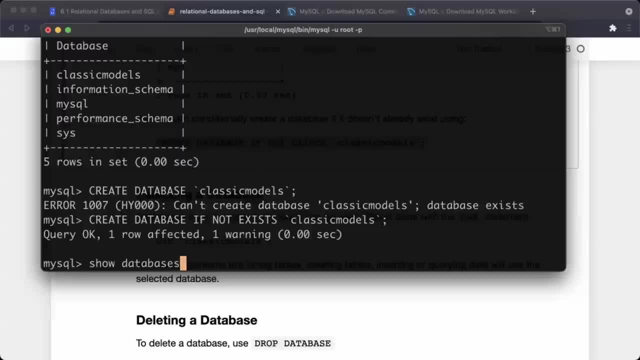 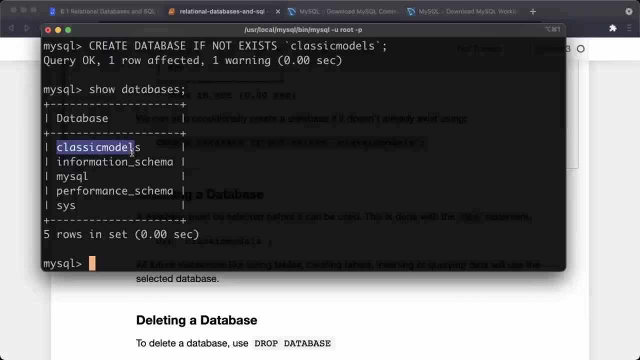 Okay, One row effected, but there was no real change. Like if we say just show databases, you can see that we have classic models information schema. my SQL performance schema insists, So no change here. On the other hand, if we had type create database if not exists classic models too? 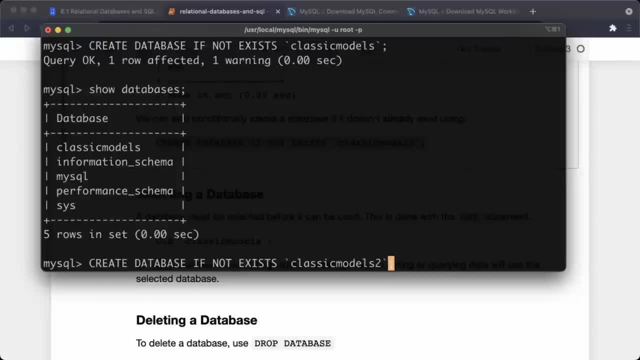 And, by the way, I'm using the up arrow key to cycle back to older commands. So up and down is how you cycle between older and newer commands. So if I type, create database, if not exists, classic models too, you will see now that we have classic models and classic models too which got created. 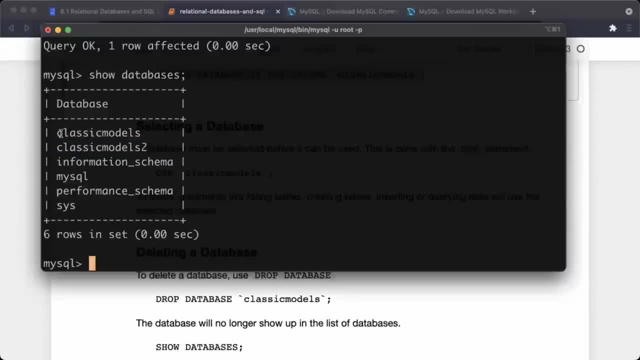 Okay, So now we have Several databases on our server And typically for every project that you're working on, you would create a database, or sometimes every team would have a database on the database server. So there are many different reasons for why you may want to have different databases, but for classic models- the company- we're just going to create this one database. 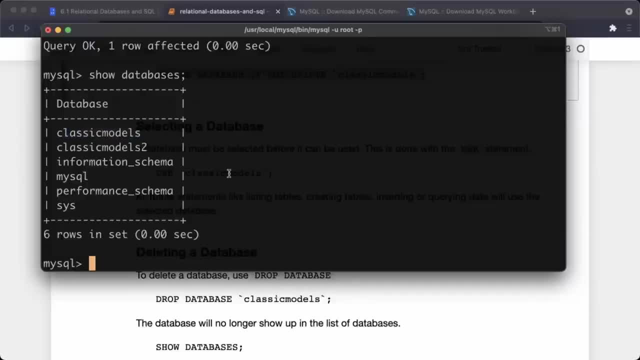 Okay, And when you are connected on a server and you want to work with a certain database, let's say you want to get data out of the database, You want to add tables- remove tables. add rows- remove rows. You have to tell which database you want to use. 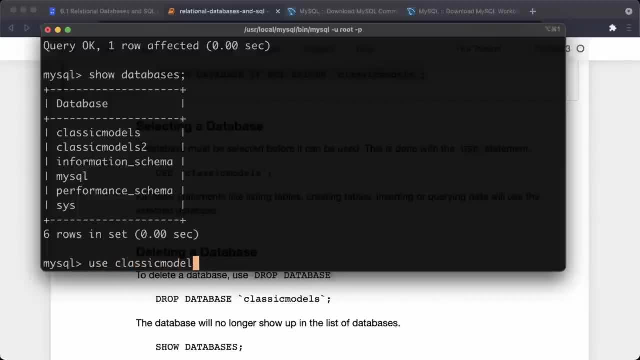 So we can say: use classic models. And once you say that, then my SQL is going to change. the database to use is going to point to classic models as the default database to which all operations will be applied. So let's say now if we do something like a create table operation, which we'll see now, and then we type the name of a table and the columns that it has, then that table will get created inside the 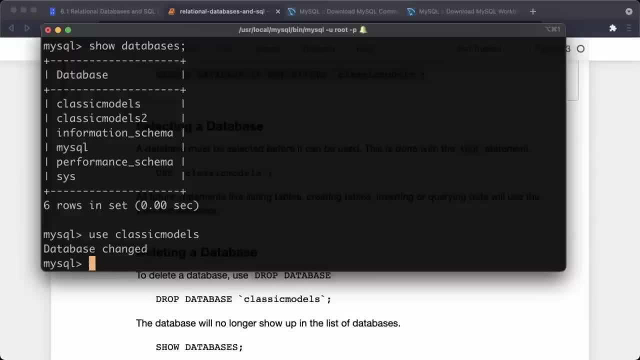 Classic models database. Okay, So whenever you get started, always make sure that you are running the use a statement to select the database that you want to operate on. Typically, my SQL remembers this, So you won't have to do it over and over. but whenever you log in, it's always a good idea to just run use classic models. 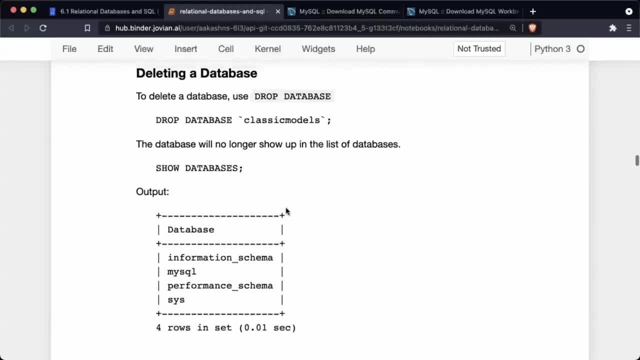 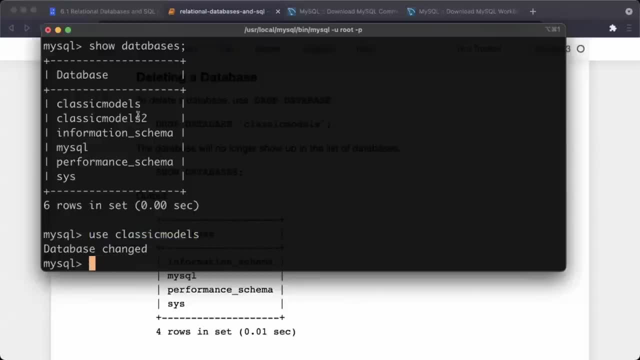 All right. So that's how you use a database. And one last thing I want to cover is how to delete a database. to delete a database, You just type drop. So we have Currently classic models, classic models, two information, schema, et cetera. 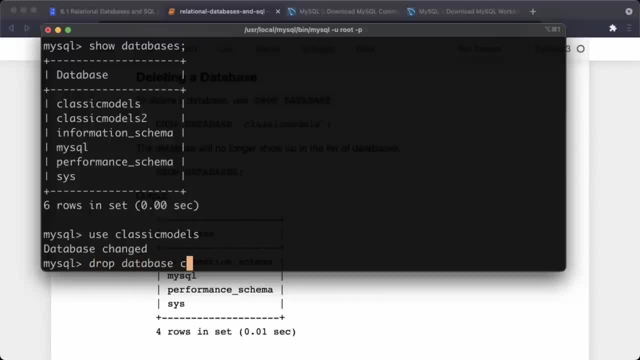 So I'm just going to do drop database, classic models two and a semi-colon. And now if we check show databases, you can see now we no longer have classic models to that database was deleted. I can also go ahead and drop classic models and then you will see that now we no longer have classic models either. 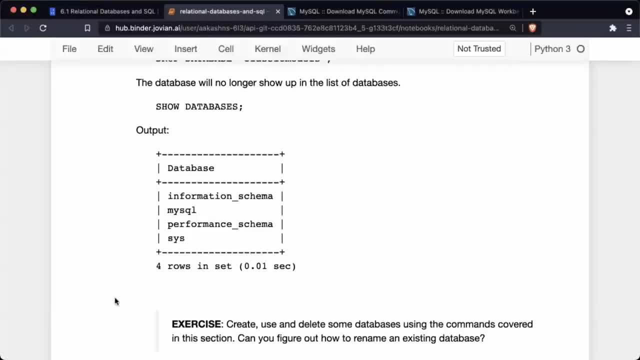 Okay, Now be careful about drop, because as soon as you run the drop statement, the data will be deleted permanently. There is no trash and there is no warning, There is no confirmation And typically your company will not give you access to drop databases for good reason. but regardless, you should be very, very careful about running the drop database command. 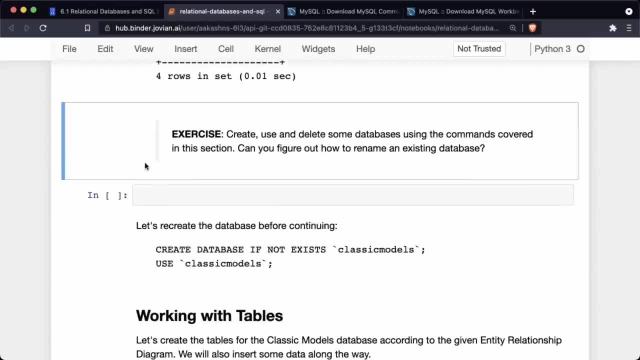 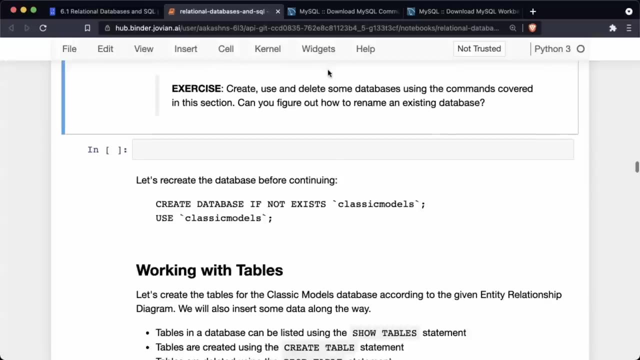 Okay, Uh, so as an exercise, you can now just try creating, deleting using some databases using the commands that we've covered, And also try and figure out how to rename a database. So now you can try and look it up on the my SQL documentation or just by searching online how to rename a database. 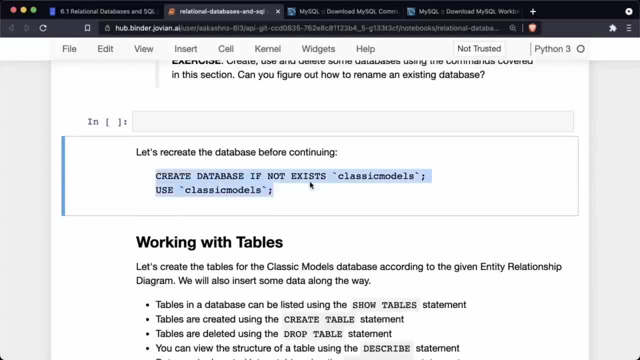 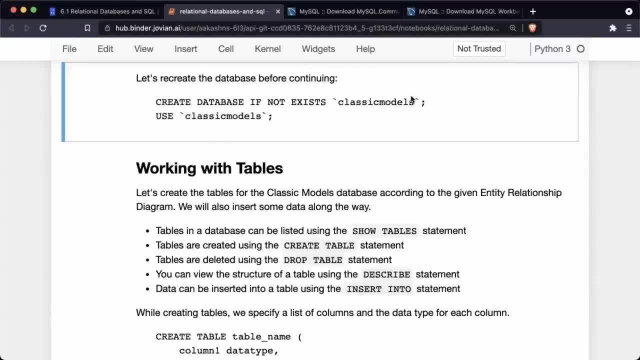 Okay, Next, just before we move forward, let's just recreate the database classic models, because we are now going to create some tables with it. So I'm just going to run, create database If not exist classic models, and use classic models. 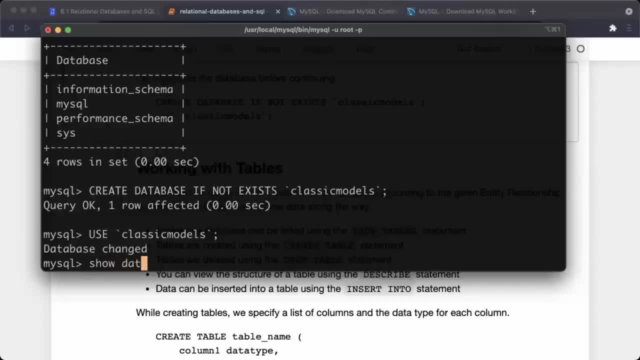 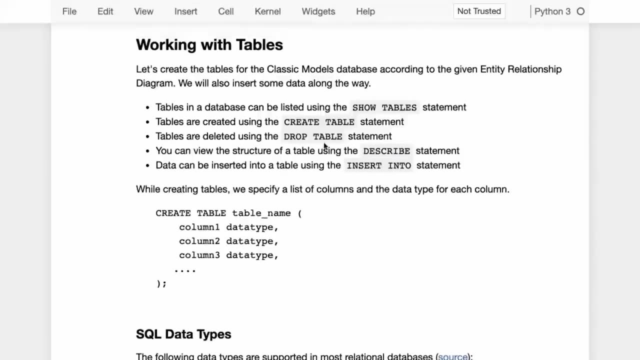 All right, So now our database is created And we can start using it. Okay, Let's now talk about how we can work with tables. Now we remember the entity relationship diagram that we created for the classic models company. We can now start adding some tables based on the ERD. 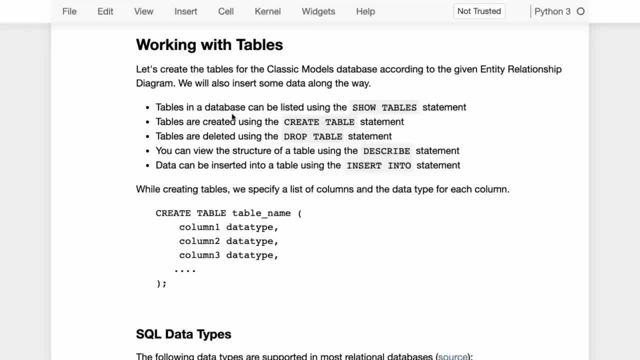 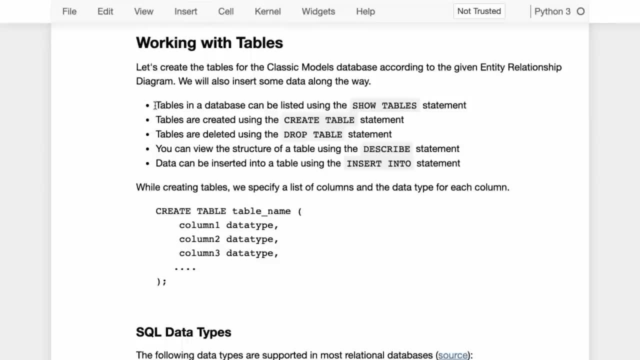 And there are a few statements. There are a few, four or five statements that we need to understand to work with tables. The first one is to list the tables in a database. Now, once you select a database using the use command, you can list the tables in a database using the show table statement. 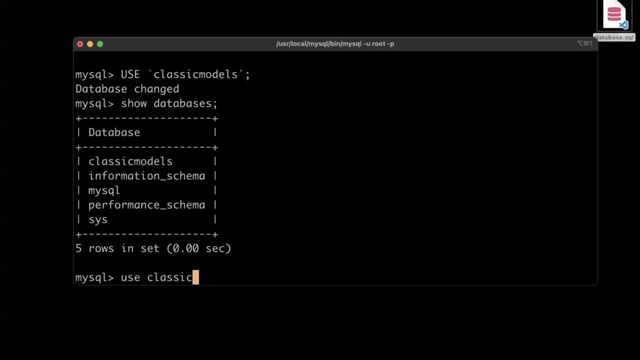 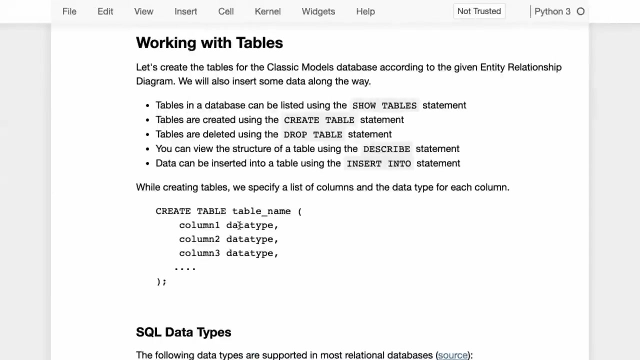 So if we go here and we say use classic models and then we say show tables, you can see that currently it says empty set because we've just created the classic models database, So it does not have any tables. but we know that it is empty. 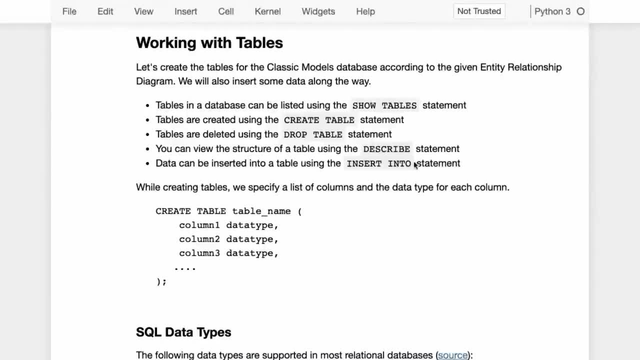 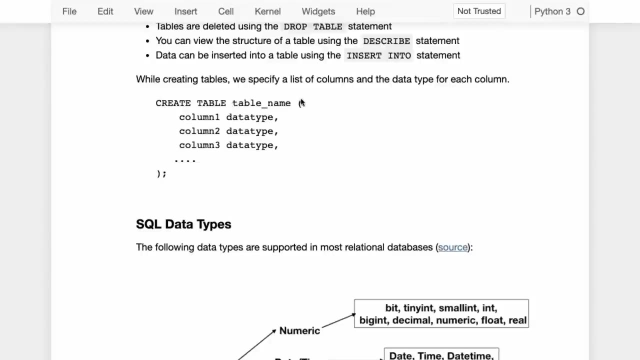 So we know that much, So let's click on that. Then, to create a table, we can use the create table statement, And here's what the create table statement looks like: You type create table and then you type the name of the table and then you have this. 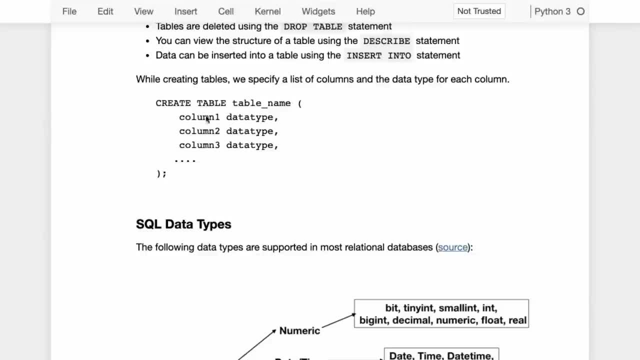 You open these brackets or these parenthesis, and then you type the name of a column and then you type the data type of the column And then below it, You also have some constraints About the tables. Okay, other information that you want to specify about the table. 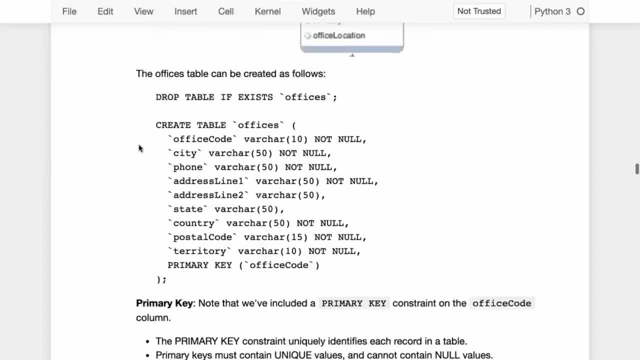 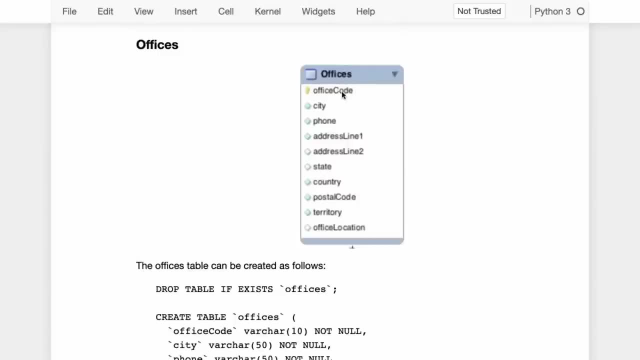 So I just want to show you an example of what a create table statement looks like. So here is the ERD diagram for the offices table. Now for the offices table, we have this office code, which is the unique identifier for each office, or this is also called the primary key in SQL. 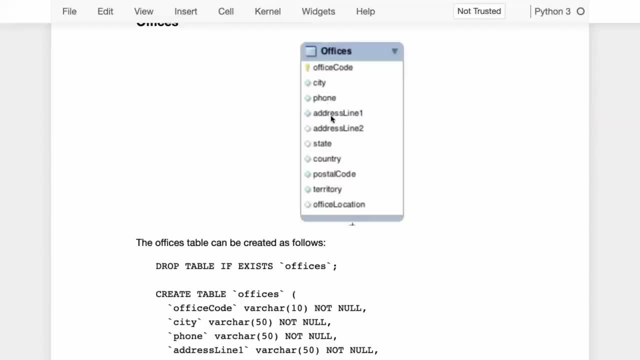 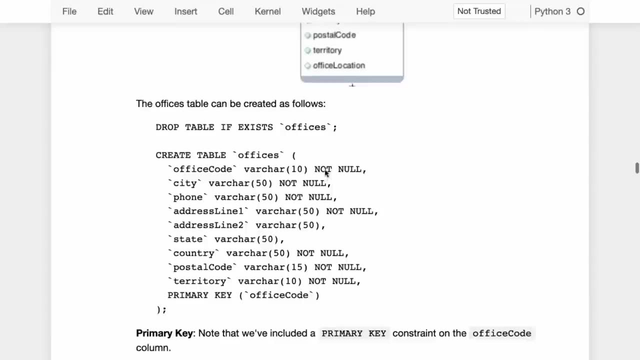 Then we have all this information: city phone number, address line one- This is all required. And then we have address line to state This is optional information. Then we have country, postal code, territory- This is required. And then we have office location, which is optional. 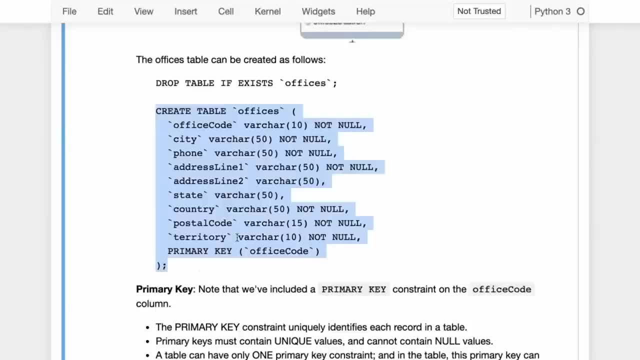 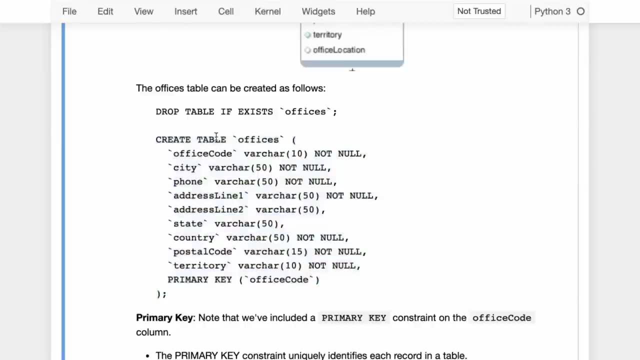 So this is what the create table statement for office, for offices, looks like. So we say: create table offices. And again, you can skip these backticks. These are just for convenience. Sometimes column names can have spaces, So to handle things like spaces we have backticks. but here you can just use you. 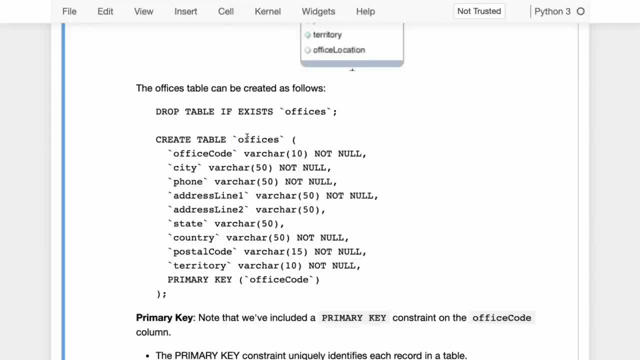 can just use it To visually identify what is a SQL statement and what is a name of a database or a column or a table. So we say create table and then we type create table with the name offices And then we open up this bracket and we say office code. 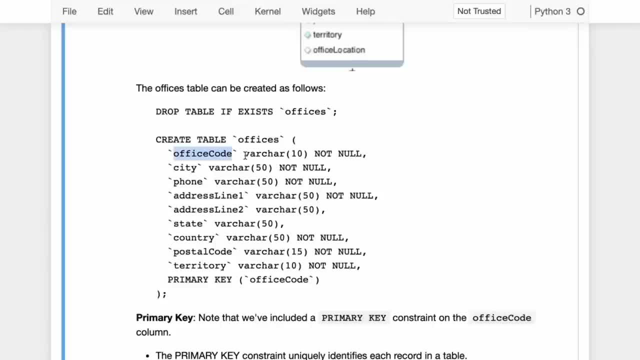 So that is the name. name of the first column and office code is going to be aware care. So this is the data type and we'll talk about the data types. So it is going to be a character list or an variable number of characters. 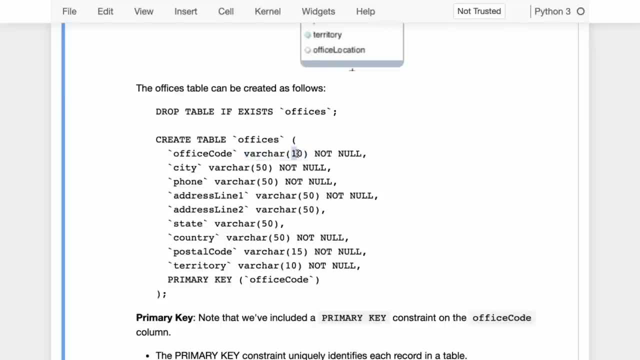 That's What it means where care of up to size 10.. So office code can be one: one character, two character, three character, up to 10 characters. Then we are specifying here a constraint, that it is not null, which means that it cannot be empty. 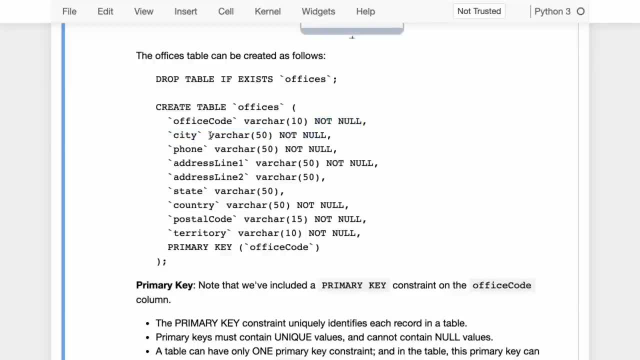 Then we have city again, which is a vat care 50. So it can be a string where care simply corresponds to a string. Essentially it can be a string up to 50 characters long again, not null. Then it will have a phone number again. 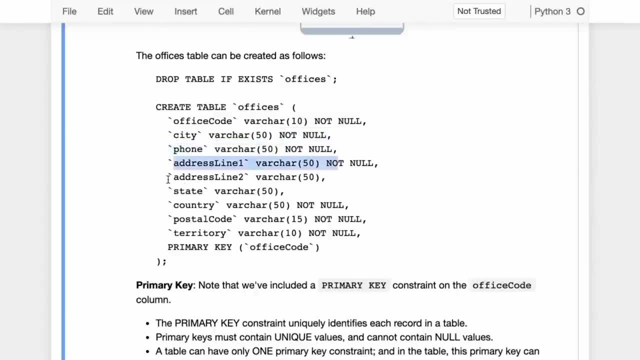 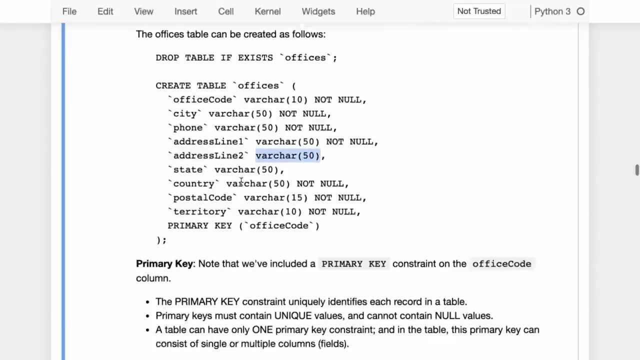 It will be a string, Not null. It will have an address line. It will have a second address line and this time it will. this can be null, So we don't necessarily need to have a second address line. It can have a state again. this information can be null. 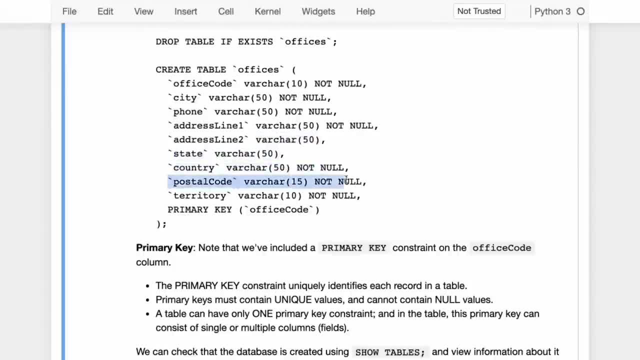 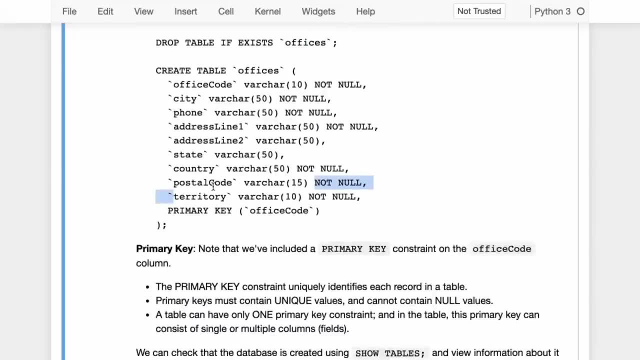 It can have a country. This should be. should we not know a postal code at territory? Okay, So territory would typically be, I think it would probably be country, or maybe the territory which the office operates in. Okay, So we'll see an example of this. 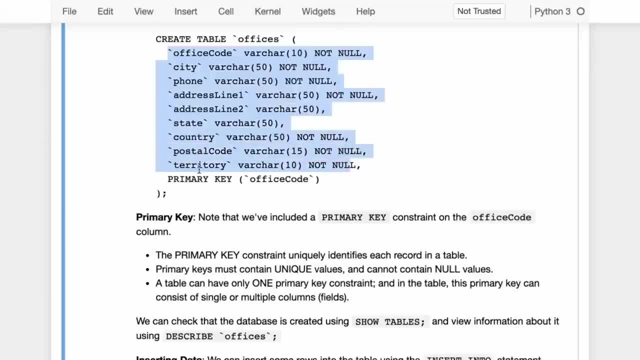 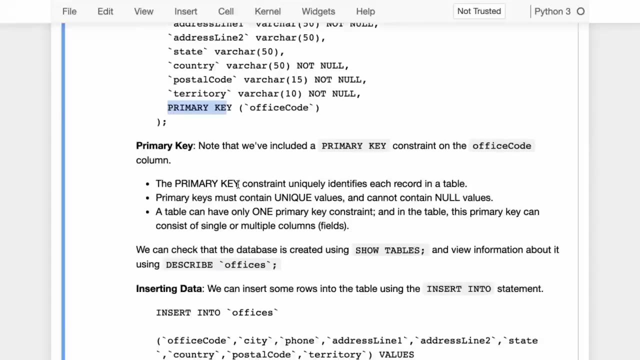 And finally, at the end of specifying all the columns, we are also specifying this constraint, or this additional piece of information that we want office code to be the primary key for this column. So what this does is the primary key constraint uniquely identifies each record in the table. 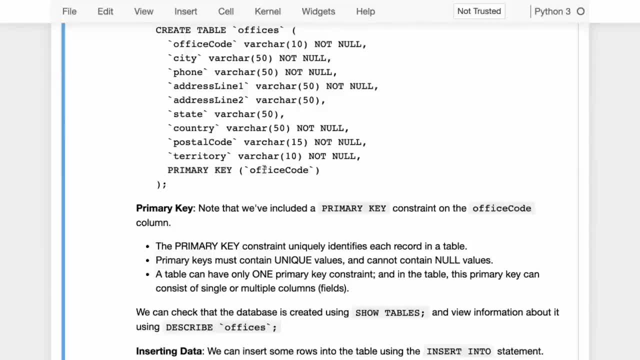 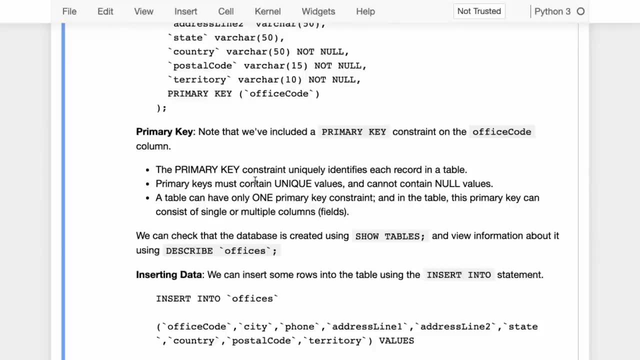 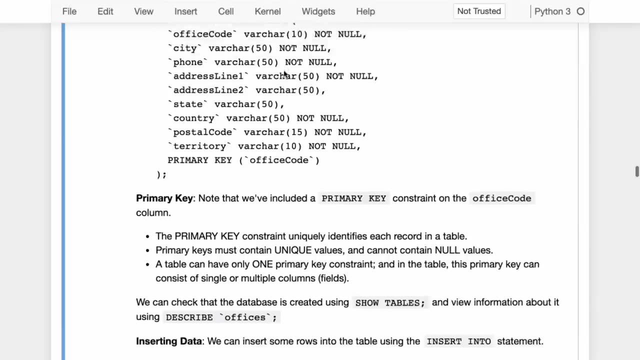 So the office code value in the office code column will uniquely identify each office, And what that means is that You can only Have one row with a specific office code. You cannot have two offices or two rows of data with the same office code, and it also cannot be null. 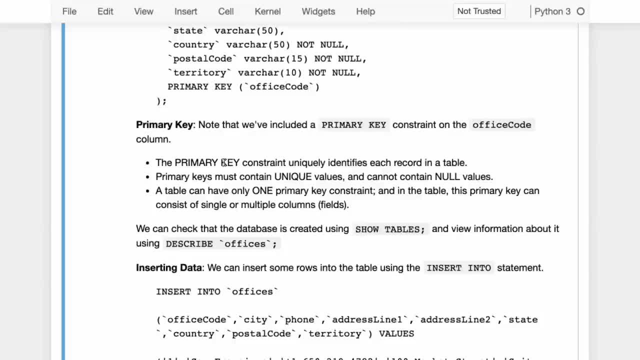 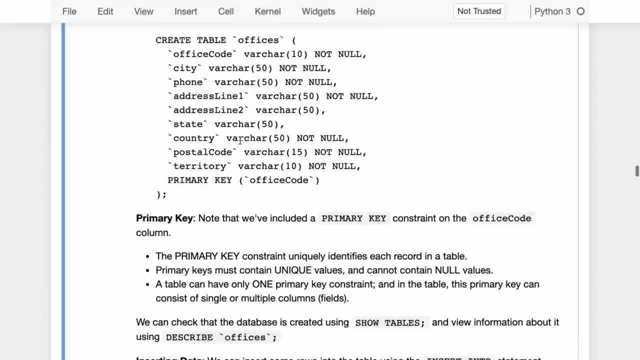 And that's why we have specified not null here already. Okay, And a table can have only one primary key constraint, So you you can select multiple columns. You can say that the primary key is office code comma city, although in this case it will not make sense. 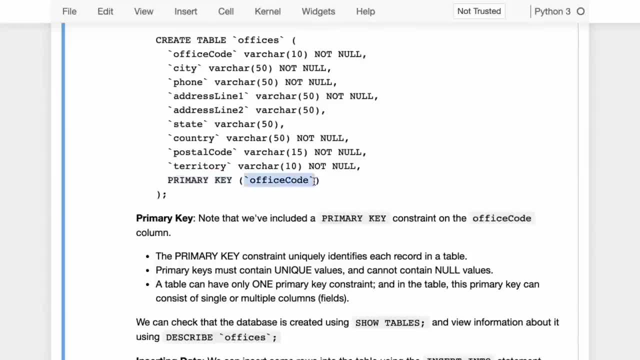 Sometimes it does. Uh, so you can select multiple columns as the Primary key. So primary key can consist of multiple columns, but you should only have the statement written once. So if you want to select office code, comma, cities or both of those together as a primary key, then you you should write: 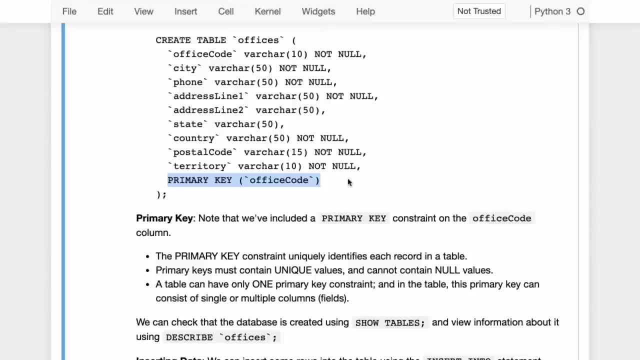 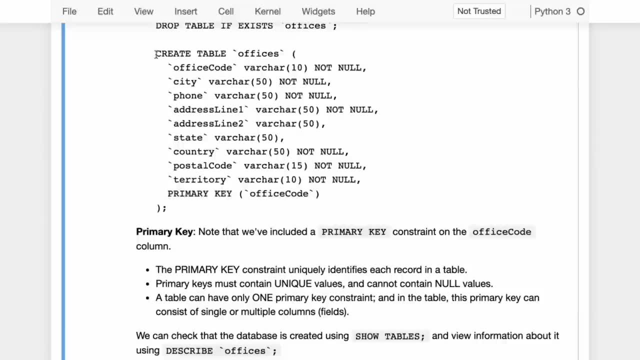 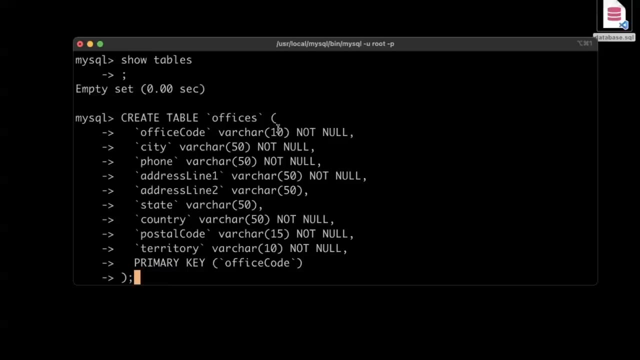 primary key office code, comma city and not primary key office code, and another line: primary key city. Okay, that's a more special case, That doesn't really happen. So for now let's just take this code and let us run it here in: 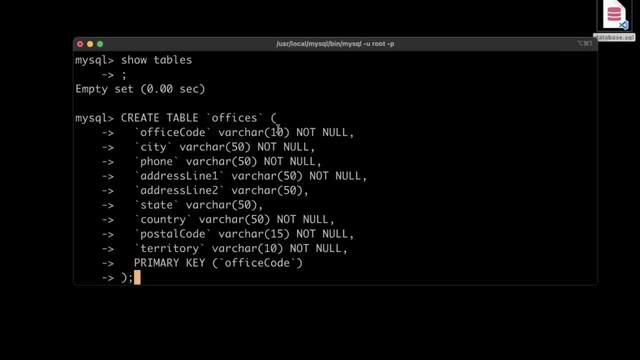 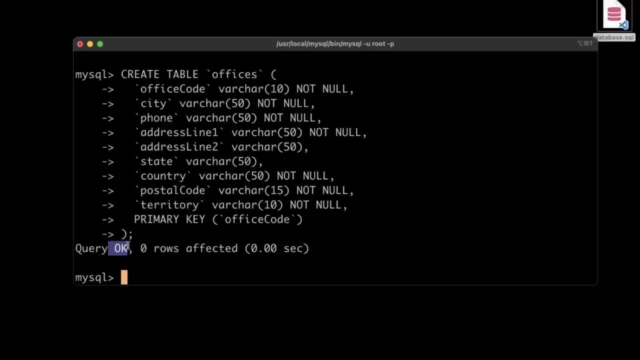 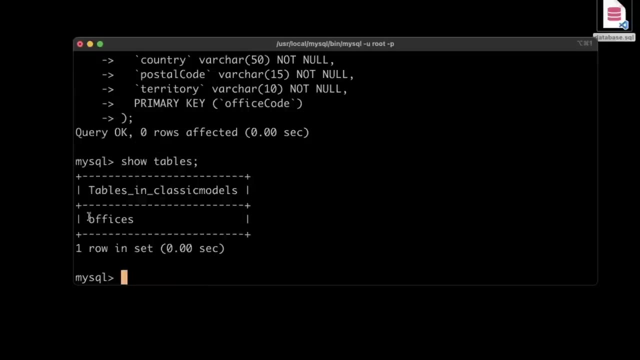 Our MySQL command line Okay And we run it And as soon as we run it it says: query Okay, Zero rows affected. So whenever you see okay, that means that it has had the intended effect. So now, if we run show tables again, you will see now that there is one table in classic models. 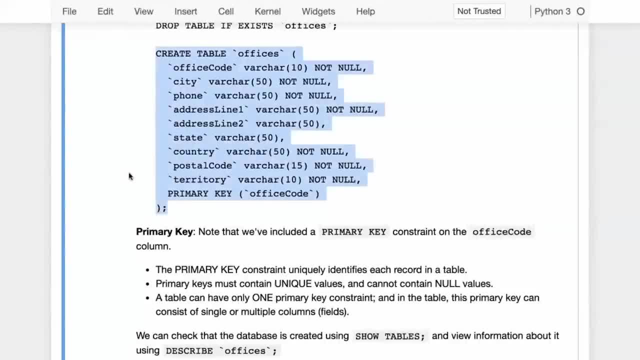 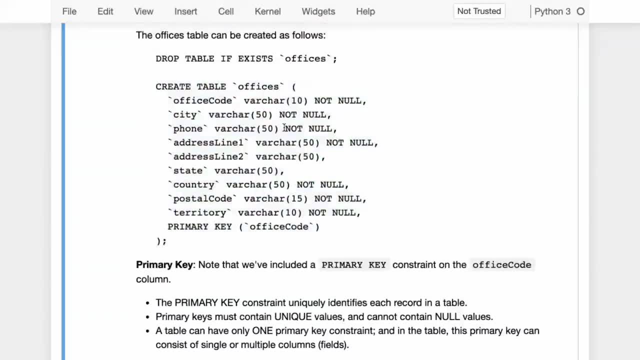 The table is called offices. Okay, Now talking about the data types. you see where care you've most of These are where care, but there are several supported data types in SQL, So here are some of them. You can have numeric data. 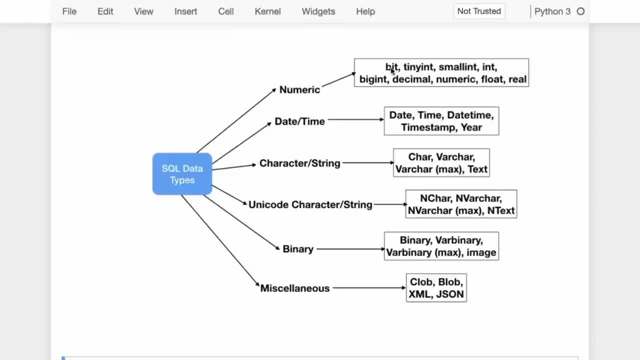 So you can specify that a column is a bit bit, means it's going to be a zero or a one or a tiny integer. I think that is going to be one bite, which means it can take values from zero to 64, a small integer. 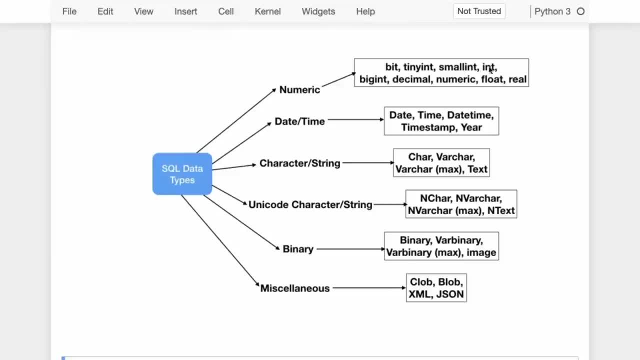 I think that would be four bites. a normal integer, I think that would be. a small integer, would be two bites. a normal Okay, It would be four bites. A big integer would be eight bites, et cetera. So the differences between all of this is simply in the range of values that they can hold. 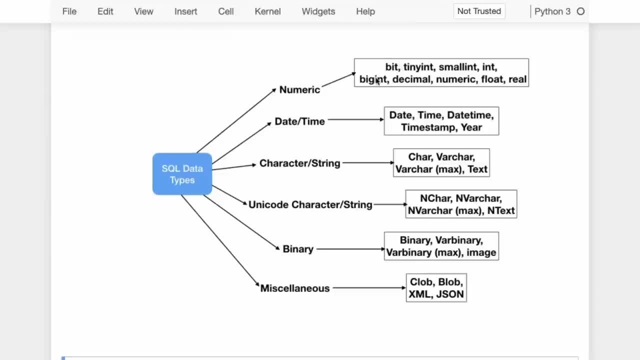 Bit can only hold zero to one big and can probably hold from minus 2 billion to 2 billion. So depending on what range you think that your numbers can take, you can choose the right data type And if you're unsure, just go with int or begin just to be safe. a lot of companies have. 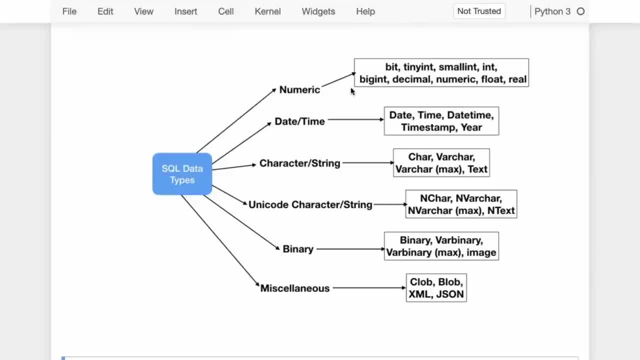 had To change from int to begin once. they hit maybe a billion users, So not many such companies, but that is. that was a real problem. They probably didn't expect to hit a billion users and they had to change from int to begin for user IDs- numeric user IDs. 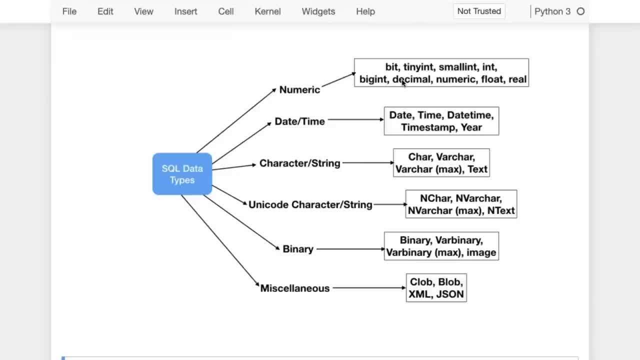 Then you have the decimal data type. So if you're sure about how many digits of decimal you want, then you can use the decimal data type as well, Or you can also use a numeric data type. I think this allows you to put in any kind of data. 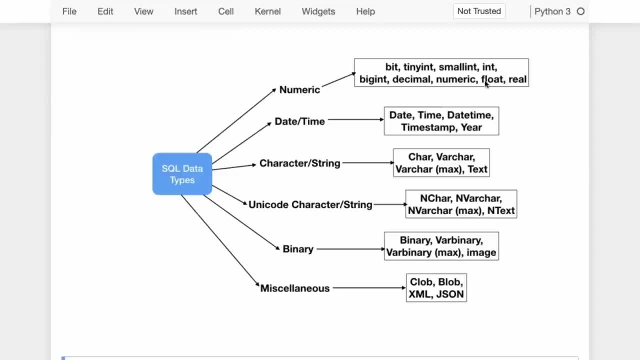 Something that you would have to look up. You can use the float data type to work with floating point numbers. here You can specify how many digits of precision you want, and then you have the real data type as well. So, again, not all of these data types are supported by all SQL software, because every all companies have implemented their own version and they have their own optimizations. 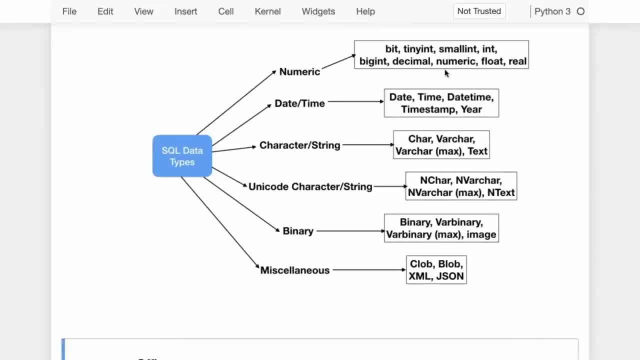 So you would have to look up whichever package you're using, like for my SQL. you would have to look up which of these numeric types my SQL supports. and then there, So these are date related types. So you typically have a date time and then a date time or a timestamp data type for working with dates. 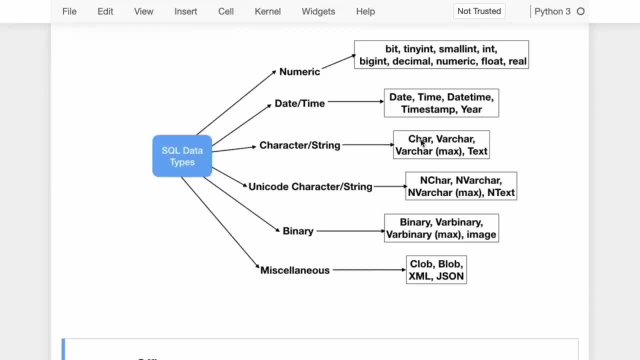 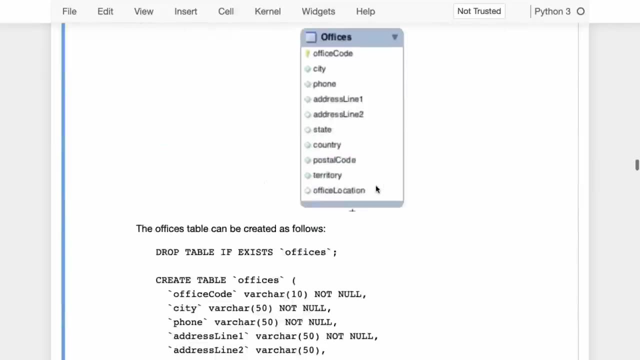 Then you have the character types, So you can have a character which is a single character, or you can also specify, when creating a cat data type, how many, what is going to be the exact length? So if you have, if you are sure that you will always have five characters in a column, you use cat or cat five. 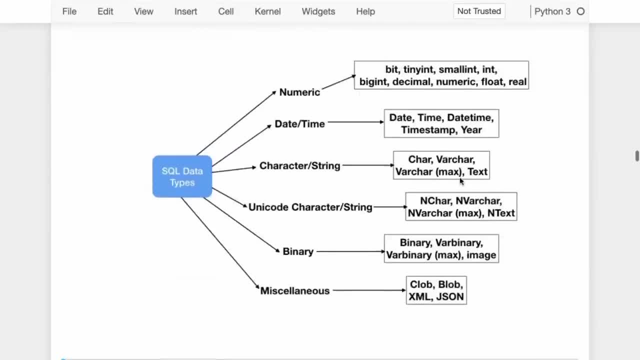 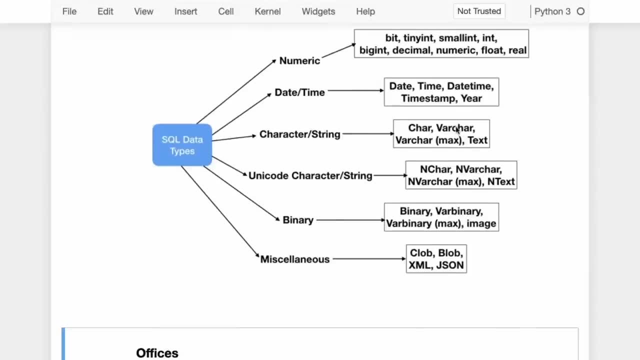 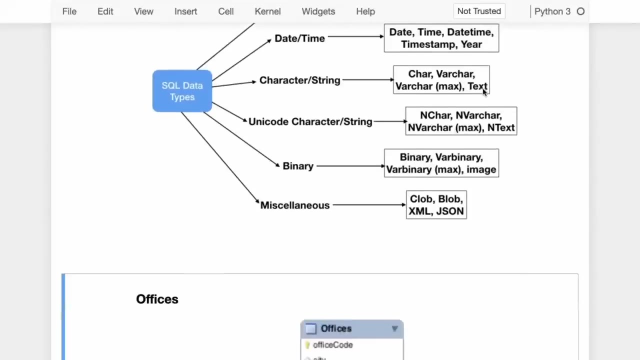 So, just as we have written where cat 50. Cat, cat five, and then you always have to put in five characters, or you can put in where cat, and where cat means that you can put up to 50 characters. So if you type where cat 50, that means you can put up to 50 characters and then you have the text data type, which is typically used for very large strings. 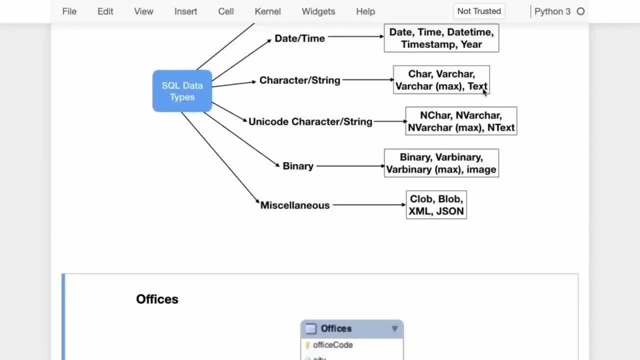 So if you want unbounded, if you don't want to limit on the number of characters, then you can use the text data type. Now, what Is the benefit of not using text? maybe using where cat. it is efficiency When you can specify the number of characters your data can take based on that. 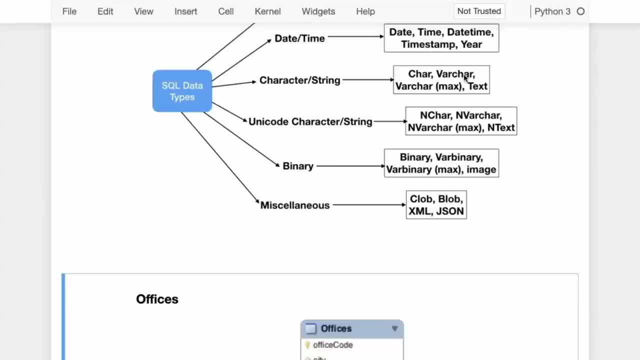 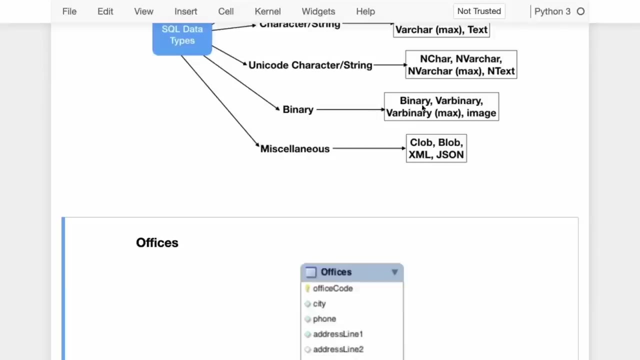 The database server can perform some optimizations to make queries faster. but if you want to use the text data type, then you are giving up on some performance. Then you have these Unicode characters, which is just a special case of characters. You can also store some binary data. 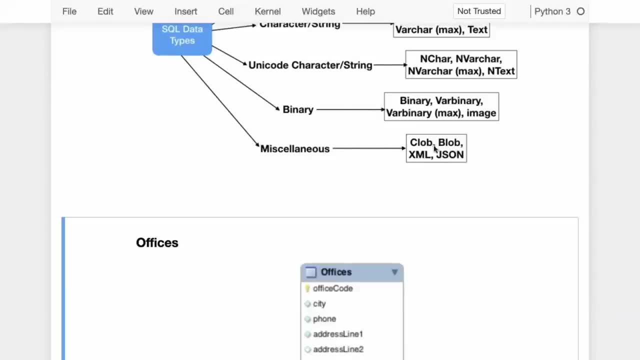 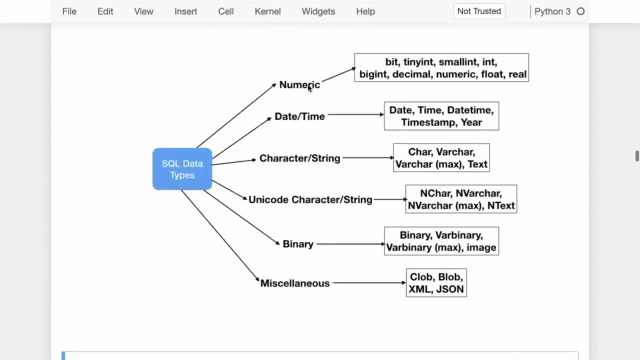 And then you can also store Something called a blob, which is like a large binary object. So you can store XML, Jason, and these are more specialized types that are not supported by all SQL servers, but numeric, date and characters or strings are the most common data types. 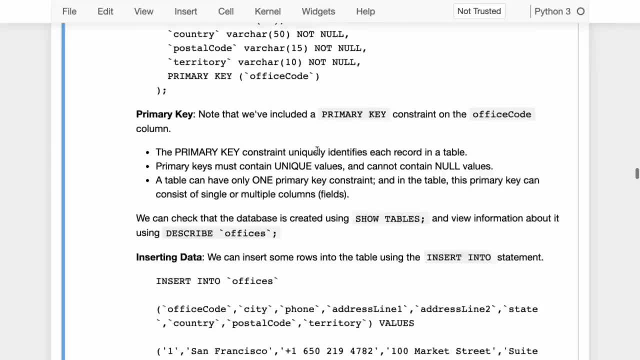 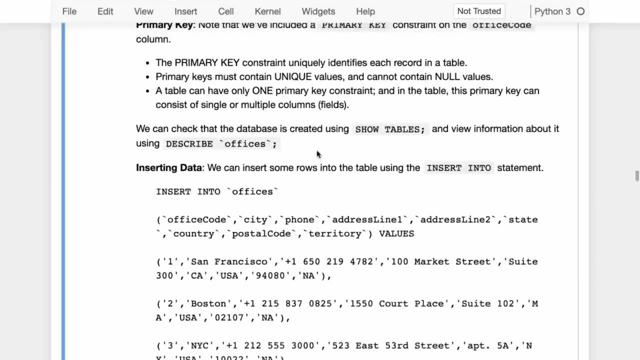 Okay, So that was data types. And next, once a table is created, you can also check. once a table is created, You can also check the table that the table is created using show tables. here We've typed show tables And 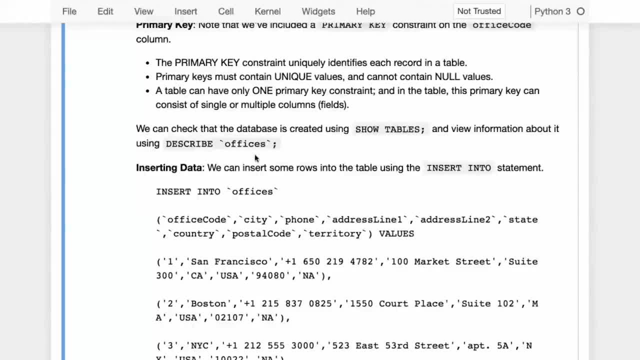 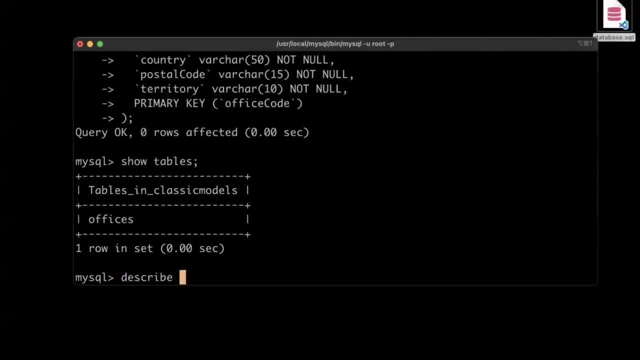 We Were able to see the table And if you want to get information about what columns the table contains, you can use the describe command. So let's type describe and let's type the name of the table. The name of the table is offices. 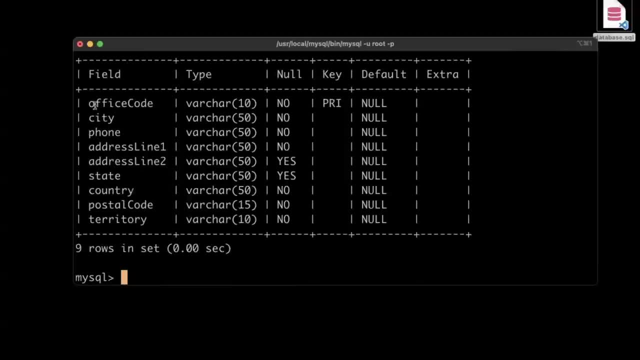 And when you type describe offices, you can see here. these are all the fields: office code, city, phone address line, state, country, postal code, territory. All of these are where care. some of these are nullable, which means some of these can be null and some of these 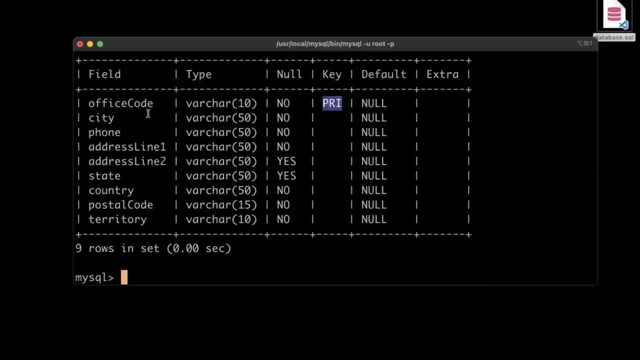 Cannot should not be null and office code is a primary key. Okay, So still, this is still information about the table. This is not information in the table. There's just information about all the columns of the table, and you can also specify default values for some of these columns. 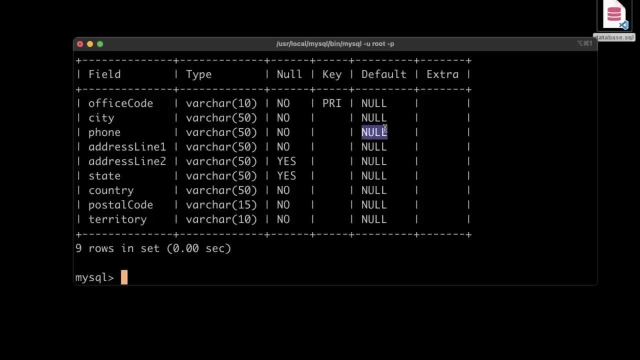 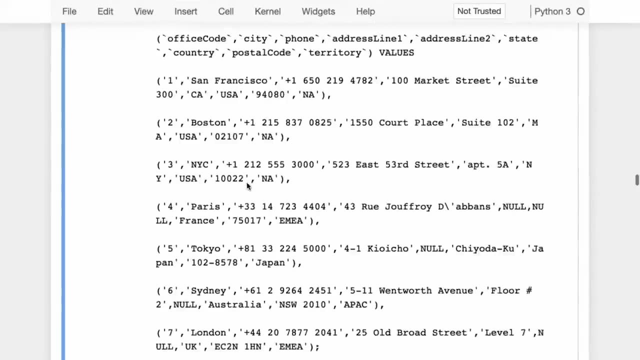 Let's say you want to specify a default value of phone number to the phone number of the headquarters, so that there is always a number listed on your website. So you could have specified that the way to specify a default is to say, let's say, phone number. 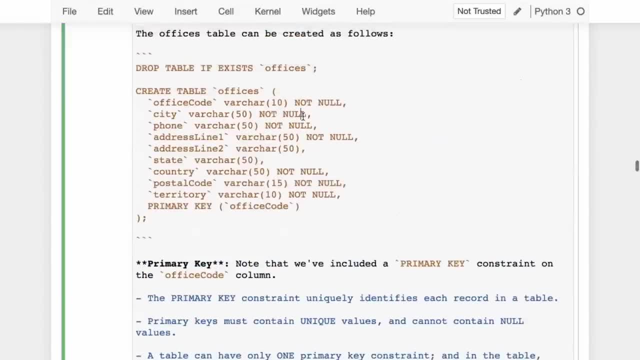 Not null, And you could instead say here: phone number default, and then you can give the phone number that you want to have as the default phone number. Okay, It'd be plus one. There's a default phone number, So that will be the default phone number that will be put in for any role in the data. 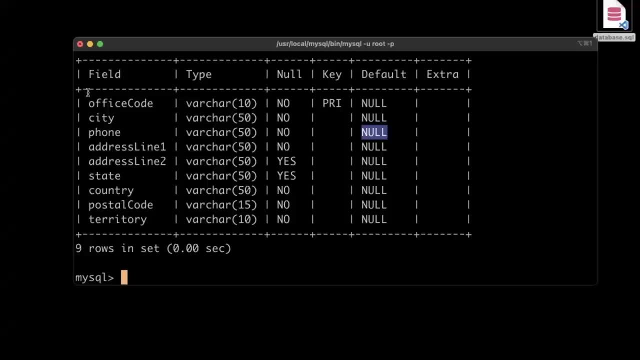 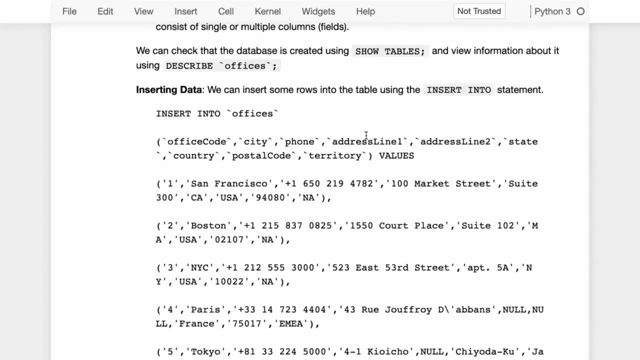 Okay, So now we've created a table. We have seen what its fields look like. We have seen that that table got created. Let's put some actual data into the table. So to insert data into the table, we use the insert into statement. 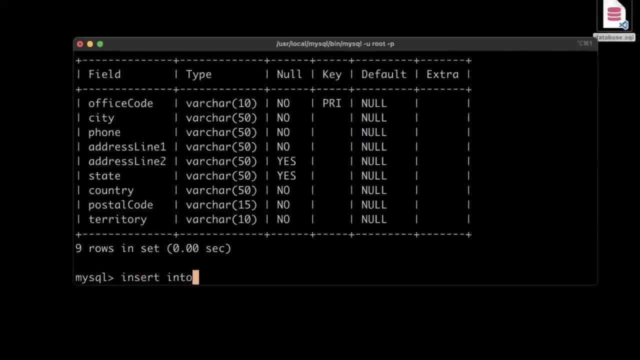 So here's how the insert into statement works. You type insert into and then you type the name of the table. So the name of the table is offices, and then you type the columns, the names of the columns that you want to specify. 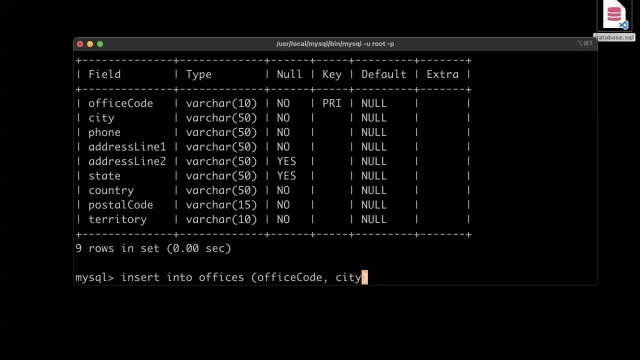 So I want to provide the office code, I want to provide the city, I want to provide the phone, I want to provide the address line one and maybe I won't provide address line Two Because I don't have that information. 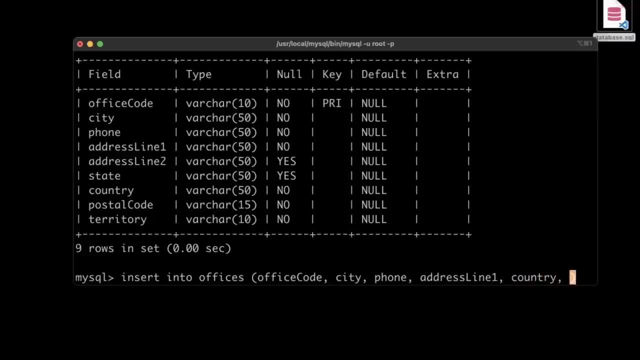 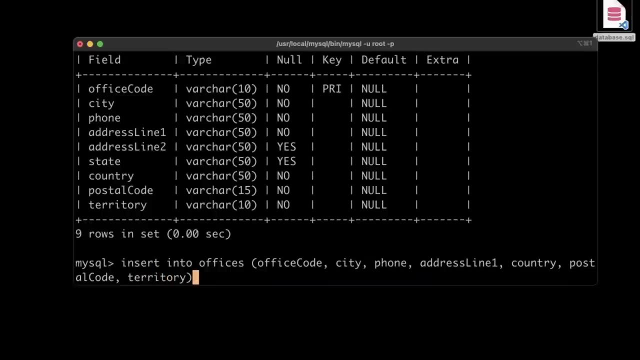 I am not going to provide state, I'm going to provide country, I'm going to provide postal code and I'm going to provide territory. Okay, So we say insert into offices and then we give the list of the column names that we're going to supply. 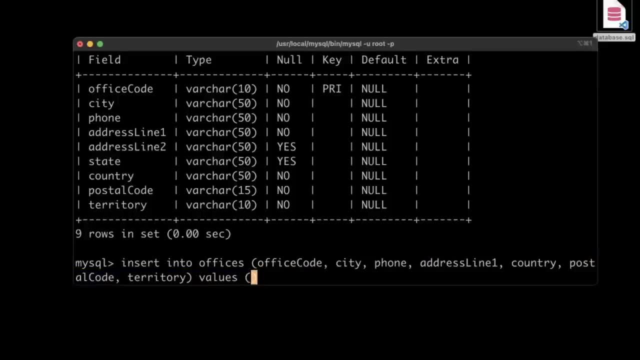 And then we say values and then we provide the values for these column names. So, okay, now I'm going to insert: create this new office with the office code a, a, a, and it is going to Be in Bengaluru and the phone number is going to be plus nine one that, and then the address line is just going to be: 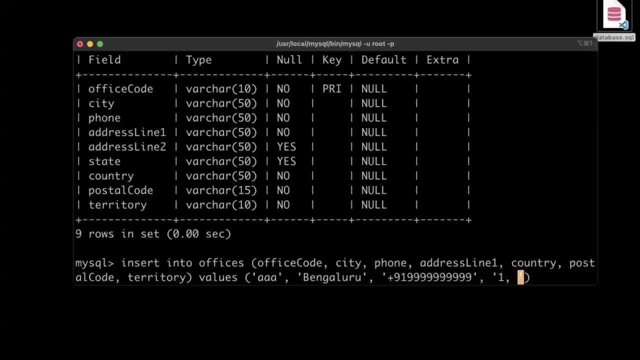 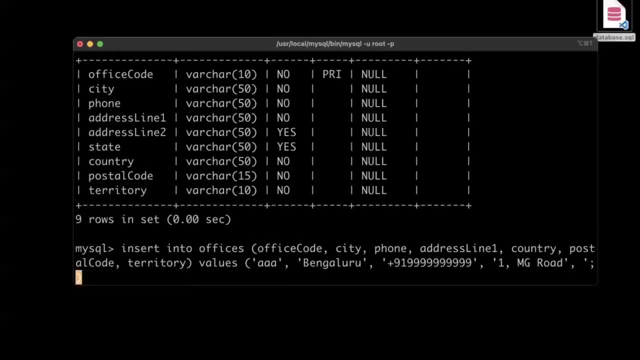 Well, let's just put it as one MG road. and then we have a postal code. Let's just put that as five, six, 5,, 6,, 0, 0, 1.. Oh, we also had to specify the country. 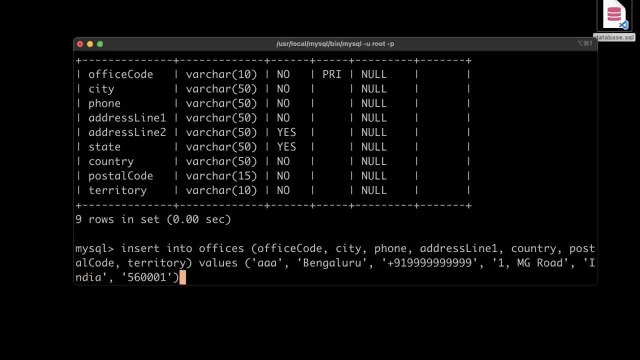 So the country is India, And then, finally, let us put in our territory here. So I guess that this will probably serve the territory of Asia, right? So let's then put the semi-colon here. So what have we done? Insert into name of the table list of the columns that we want to supply information. 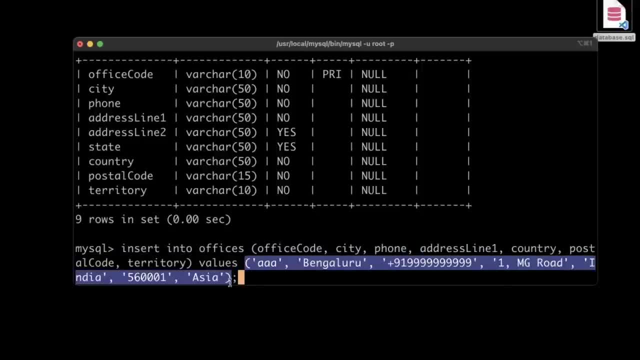 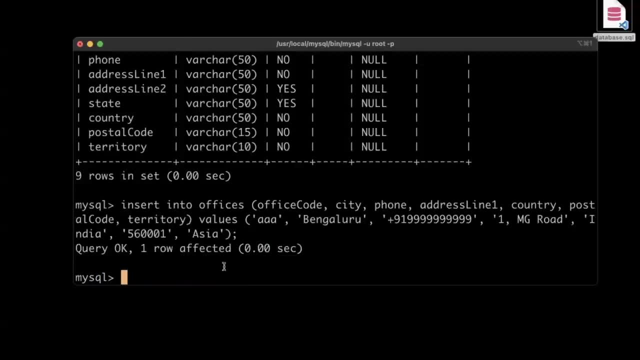 for. put in then type values, then give a list of the actual values for each of these columns, And then we can hit enter and you can see query. Okay, One row affected. And now this is going to insert the data into the table. 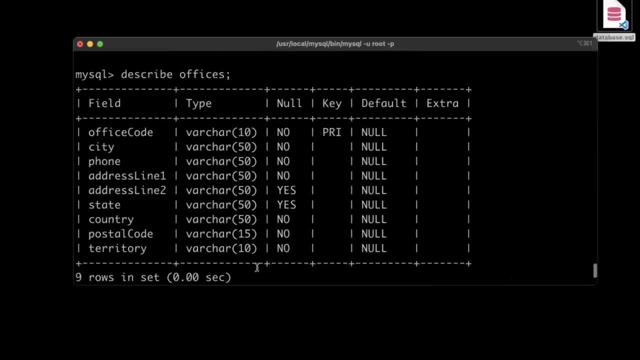 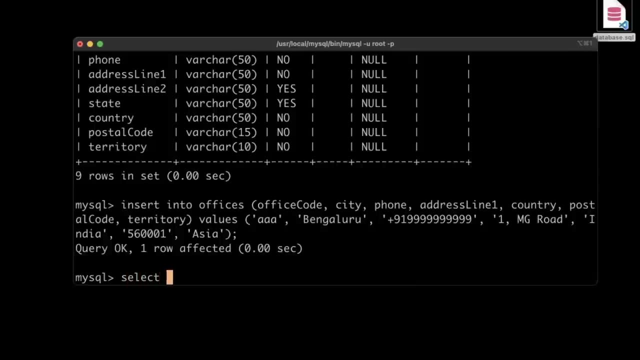 How do you get data out of a table? Well, the way you get data out of a table is by typing select. you can type select and then, after typing select, you type which columns you want. So let's say, I just want to get the office code and I want, I want to get the city from the name of the table. 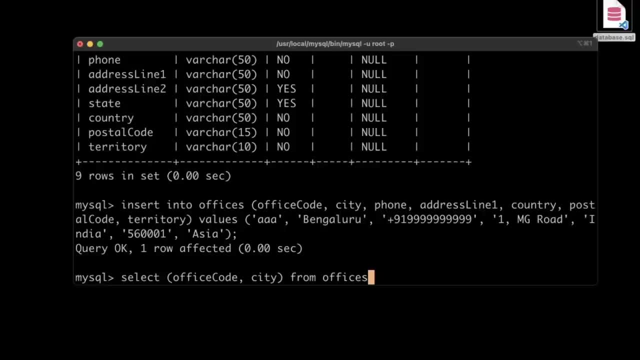 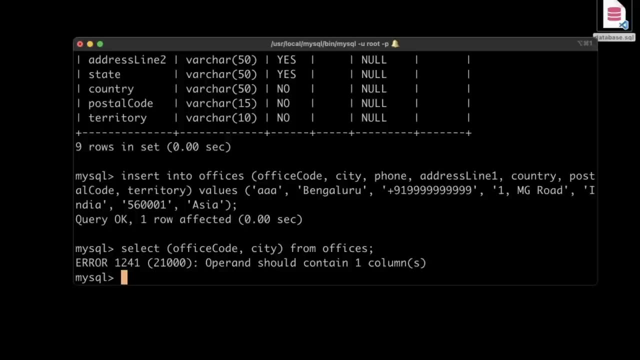 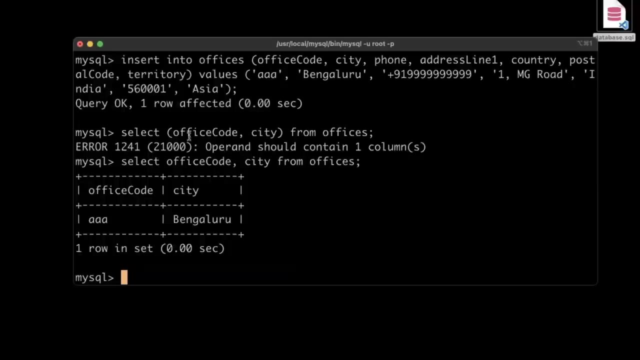 The table name is offices, And then I put in a semi-colon: Yeah, so you know no brackets here. So you type select and then you type the name of the columns that you want to select And then you say from offices. 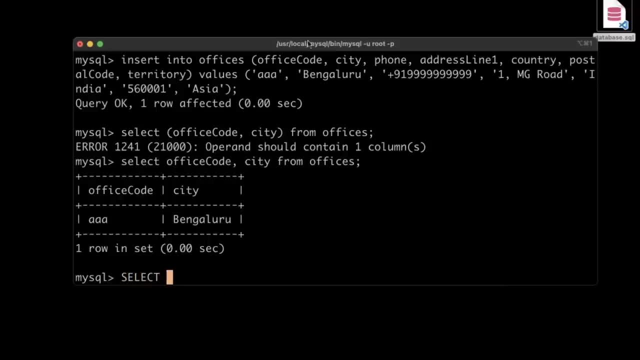 Okay, And you can see that it starts to get a little bit confusing now, because everything is written in lower case, And that's why we often write the column names in lower case and we write the SQL commands in upper case. Okay, And sometimes we also put back ticks just to make it super clear, and especially if we 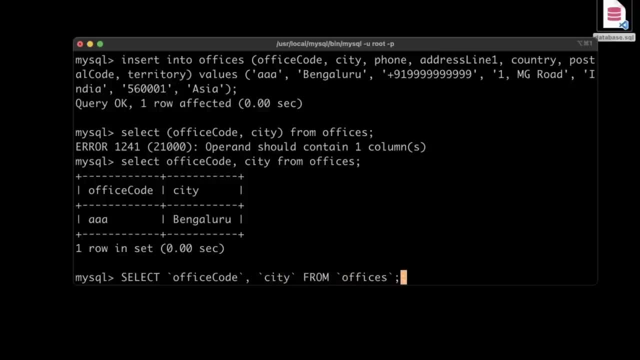 Have names in, if we have spaces and column names. Okay, So select office code, comma city from offices. So now it is giving us the office code and it is giving us the city for all the rows of data in the database, in the table offices. 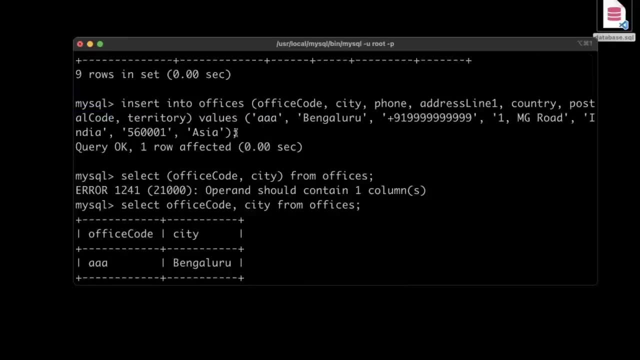 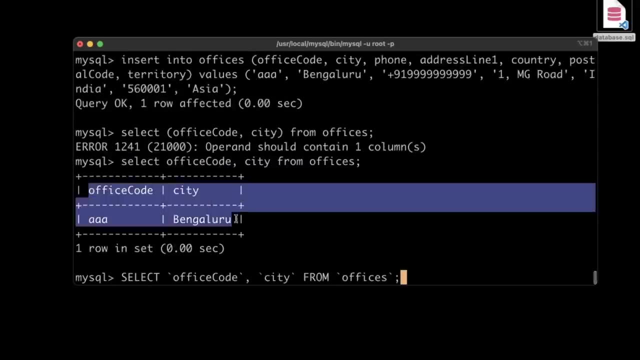 So we have inserted one row. We inserted a row with all this information and then we viewed it using select. Now, if you had inserted multiple rows, we would be looking at the data for multiple rows of data. How do you insert? 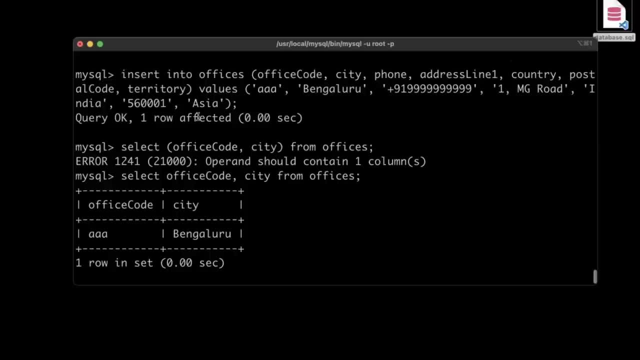 Multiple rows. inserting multiple rows is the same as inserting one row. You just say: insert into offices and then names of columns and then type values, And then you give one set of values, Then you give a comma and you give the second set of values, and so on. 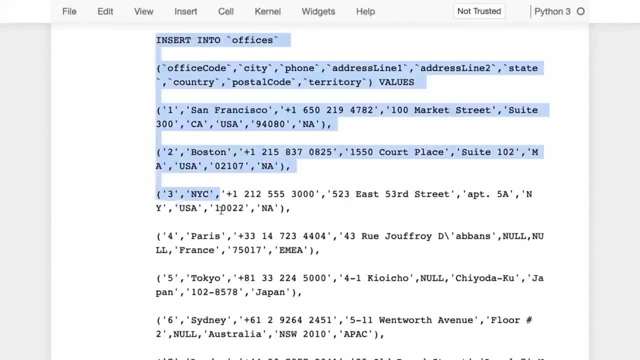 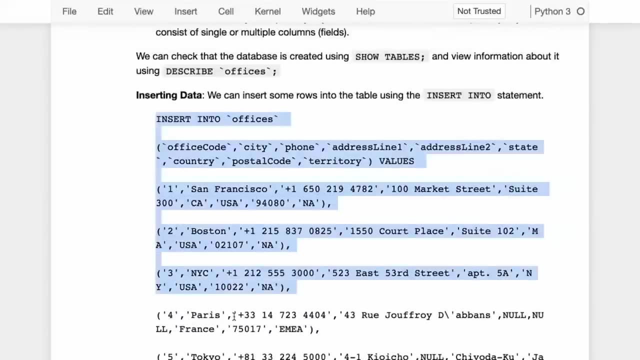 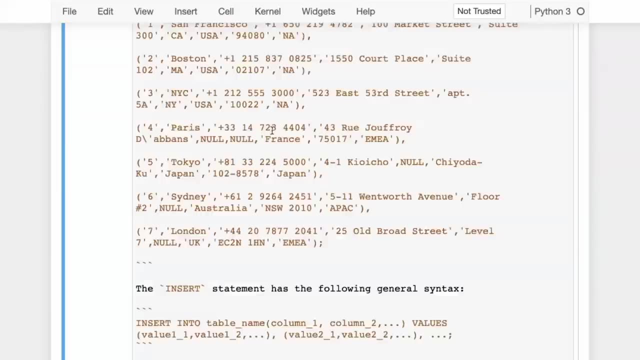 So let's insert multiple rows. I'm going to copy, insert into offices and then I have a bunch of rows of data here, So I'm going to copy all those rows of data. Okay, It's going to be a bit difficult to copy this. 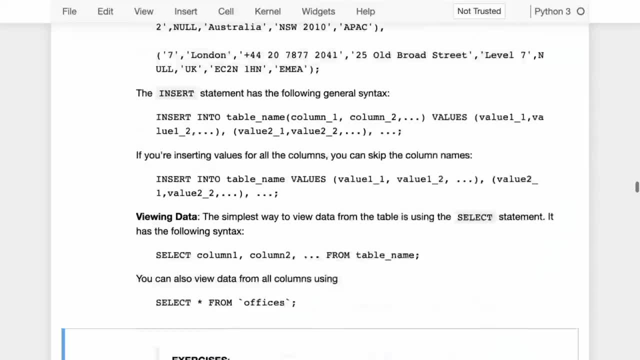 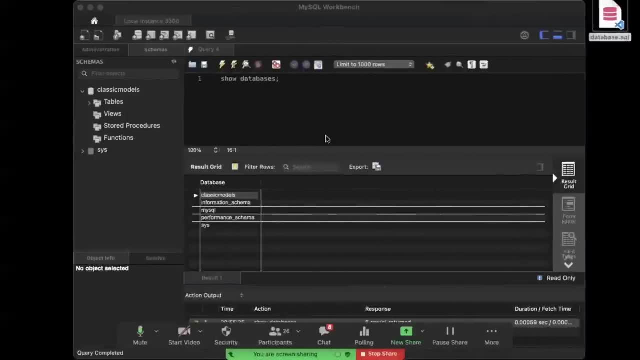 All right, Let's just copy it this way. And now this is a lot of code there, So I am going to, instead of using the my sequel command line, which I can do, I can just paste the command based on the command line here. 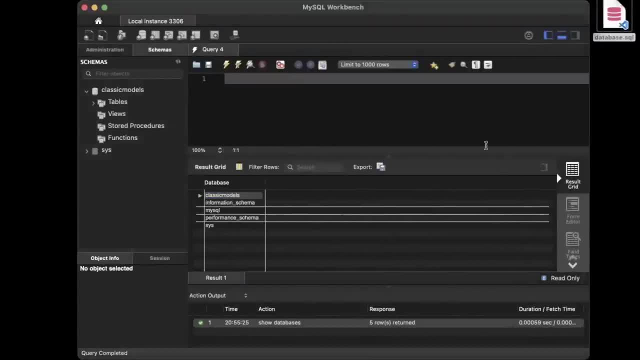 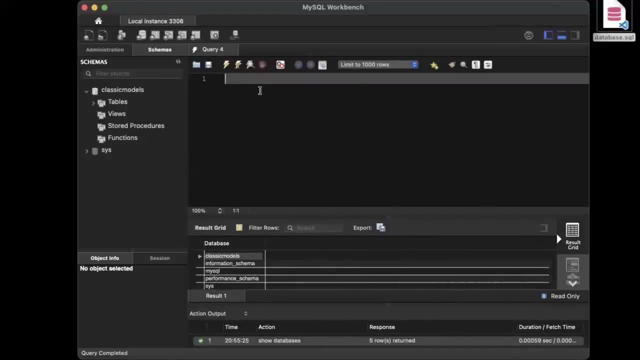 I'm just going to show it to you on the work bench. Okay, So I'm just going to type it here into the work bench. You can always just click new query. and also: yeah, you can just always click this new query here. 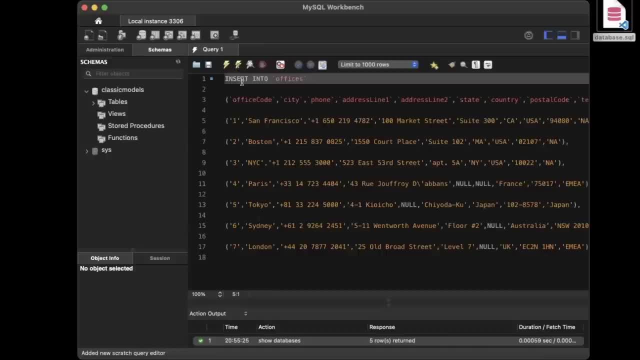 And then just type it. So here now we have insert into offices, We have all these columns that we want to insert And then the values we have on. we have one, one set of values, two set of values, three, four, five, six, all the way up to seven. 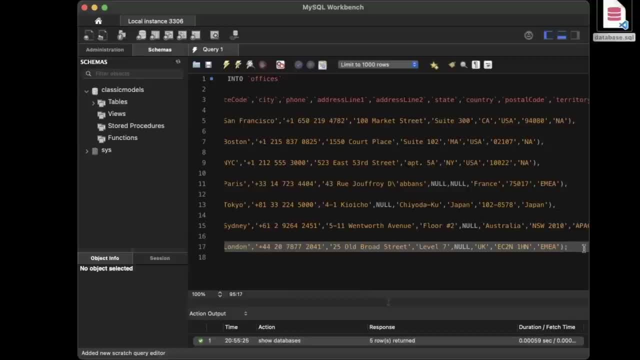 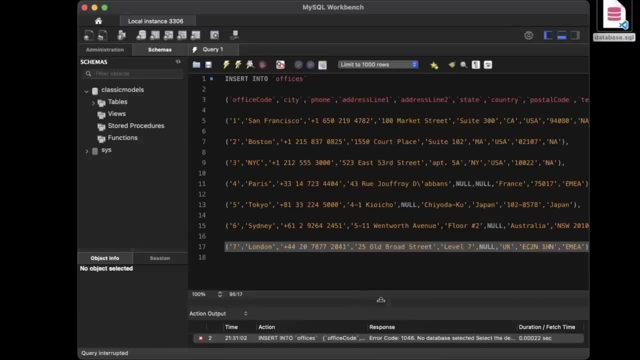 So we are inserting seven values And at the end you will notice a semi-colon here at the end of the last statement, And we can run this command and now we get a success result here. Oh, we need to select a database. 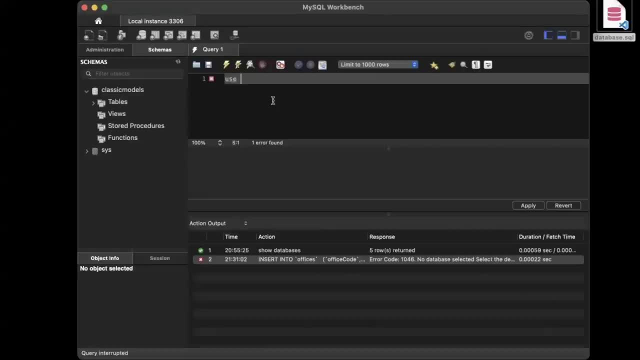 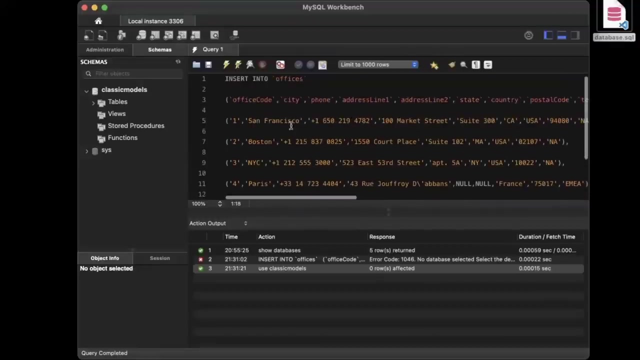 First. So let me cut this and let me say: use classic models and let me run that. So that has been selected, The database is selected. Then let us paste it back. Okay, Now we have inserted into offices and now we run insert into offices and you can see that it executed successfully. 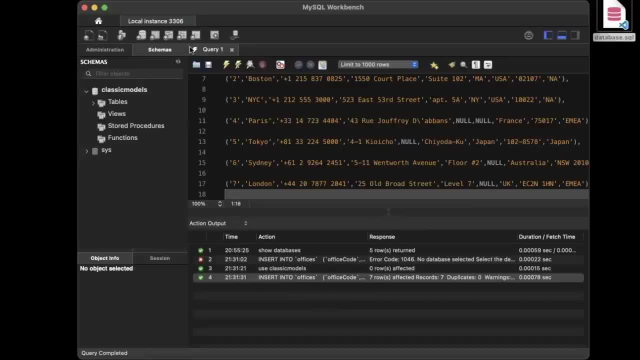 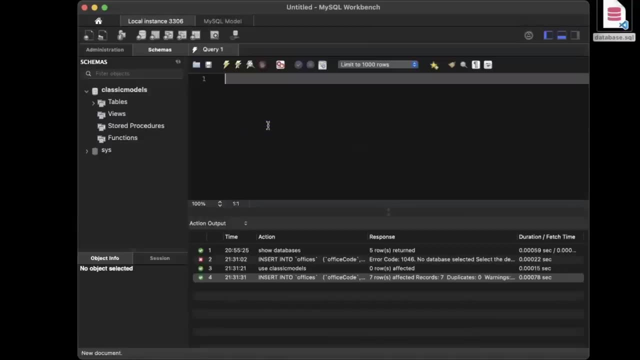 So now we have inserted into offices and I can create a new query here. I can, Yeah, so I can now remove this and I can type select, and if I want all the columns I just type star. So select star from offices and then I run it. 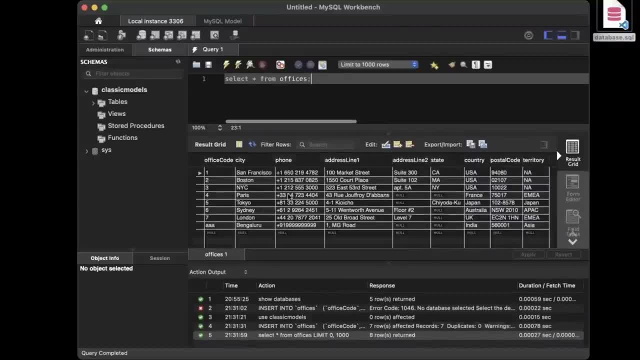 And that is going to now show this data in this tabular format. Okay, So now you can see that we have all these offices: San Francisco, Boston, NYC, Paris, Tokyo, Sydney, London, Bengaluru- And this is same information that we had shown, that we had inputted here. 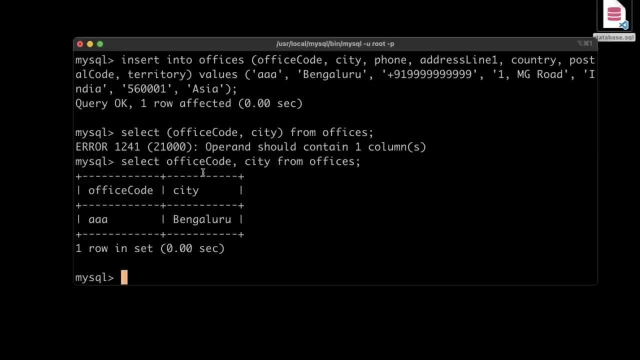 That is also available. So through the command line and through the workbench we are connecting to the same database and we can run these commands in either place. And I can type it here as well: Select star from offices. So now when I say star, it is going to select all the columns. 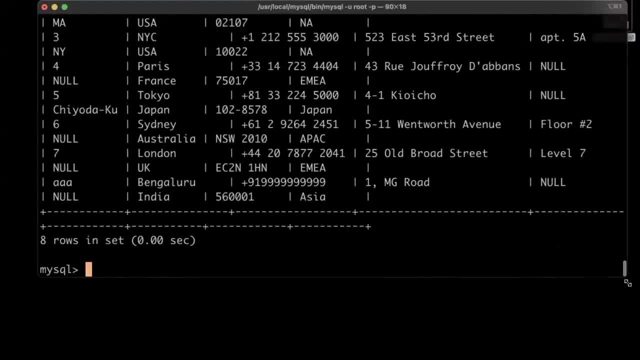 And here's what that looks like. It's a bit messed up the output, because it's trying to display it all on one line, Right, Okay, So If I zoom out a little bit, you should be able to see the output. 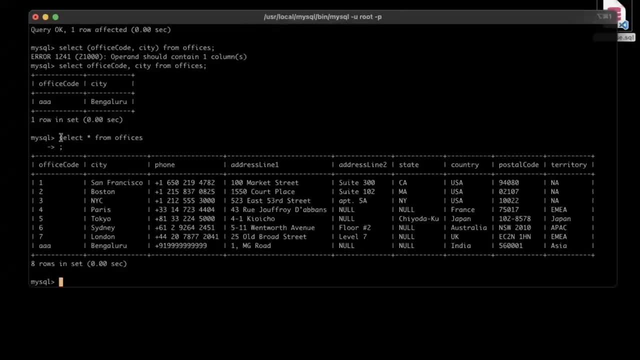 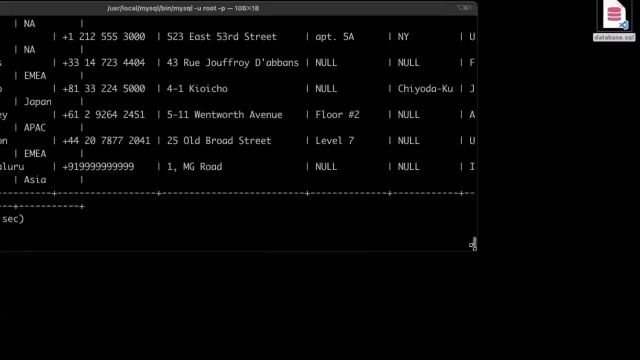 Yeah, So you can see the output. Now, when I do select star from offices, it is giving me the same table that I am able to see here on the workbench. Okay, So that is insert and select. just a quick reminder on how these work. 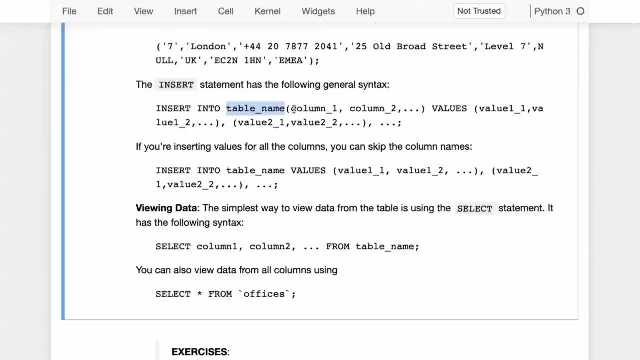 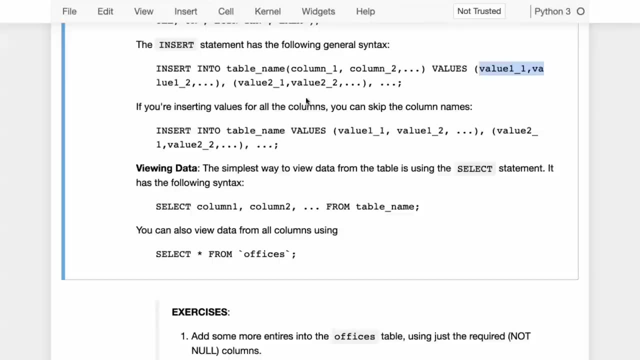 So you can say: insert into And then provide the table name, provide the names of the columns You want to insert, provide the values and then provide lists of values to insert, So list of rows, and if you're providing data for all the columns, then you can skip this part, which is the column names. 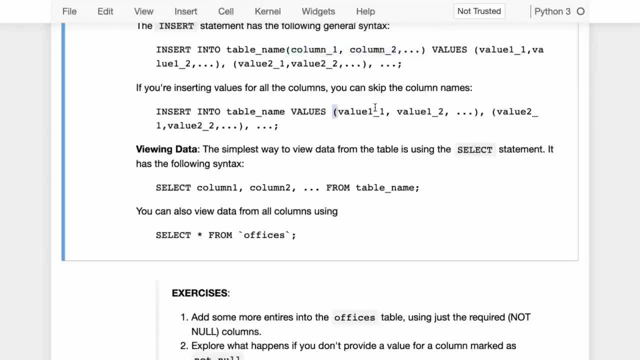 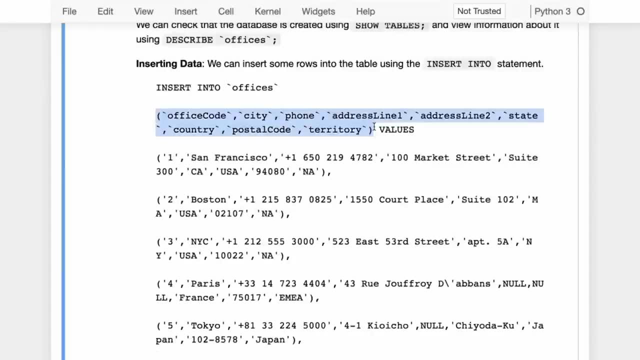 So you can just say: insert into table name values, and then you can give lists of values, and that will work fine too. For example, here, when we are inserting offices, we are using all the columns here, So I can actually just completely skip this last thing. 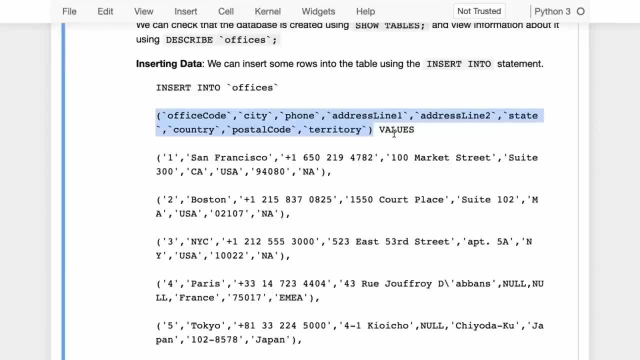 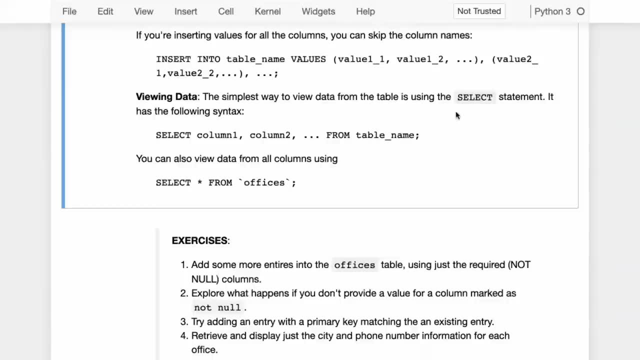 I can skip this names of columns, I can just say insert into offices values and give it the list of values. Then to view the data, the simplest way to view data is using the select statement So it has the syntax select column one comma, column two comma, so on from table name. 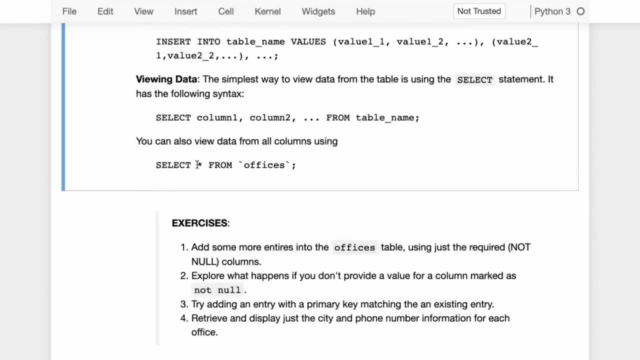 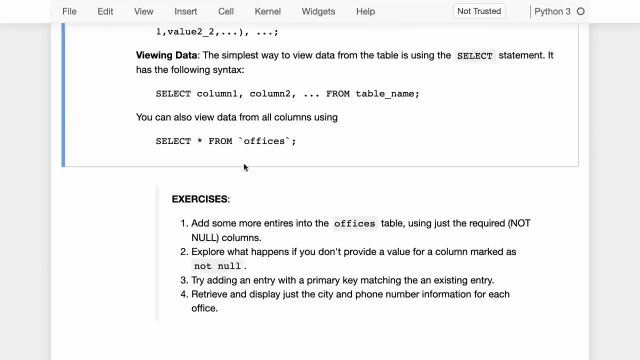 And you can also view the data from all the columns using simply saying select star from table name. Okay, So that's how we put data and get data. So now we've covered C and R- create and read, and we'll look at update and delete as well. 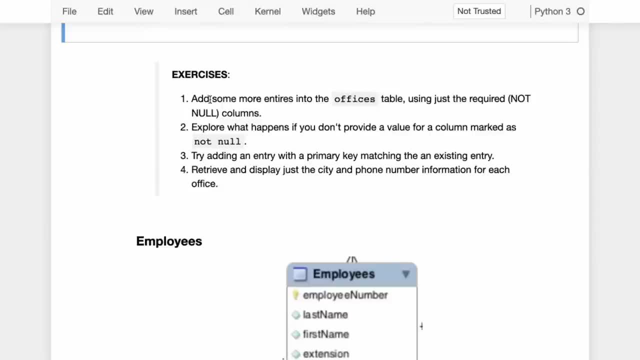 And here are some exercises for you. Try adding some more entries into the offices table using just the required column. So an example that we typed out on the MySQL command line. try typing it out yourself. Try doing it from the command line, try doing it from the work bench and see what happens. 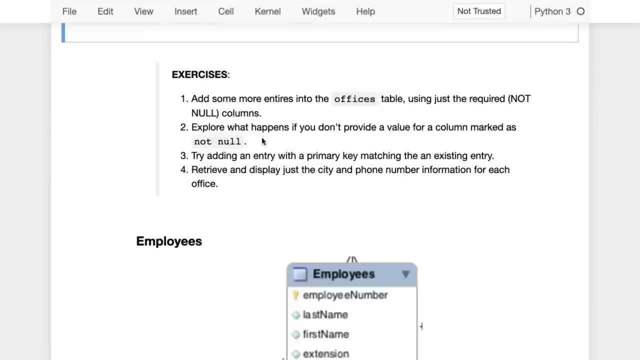 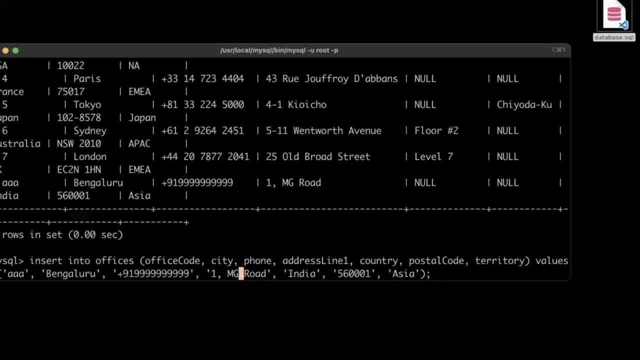 See what happens if you don't provide a value for a column marked as not null. Okay, Maybe here, if I go back to one of these and if I try and change this, Let's say I changed the office code to AAB and I provide- I don't provide a value for territory. 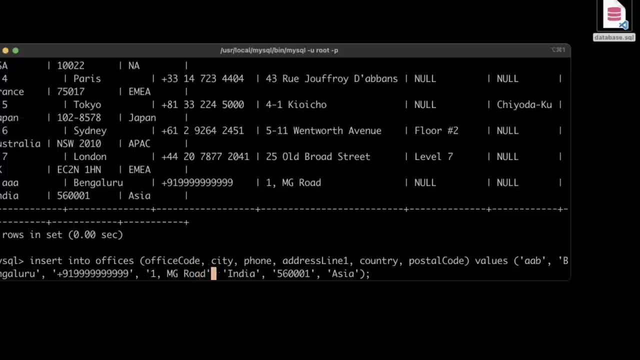 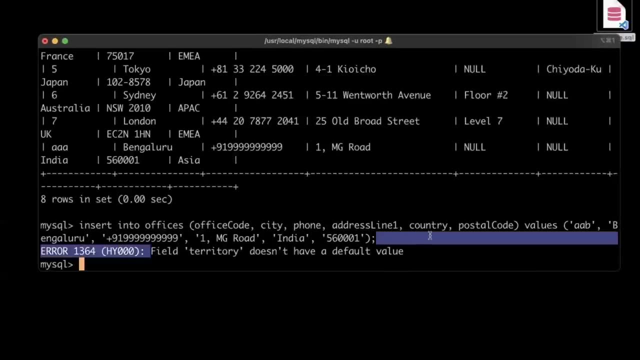 which is supposed to be non-null. Let's see what it's going to give us. So it's going to give us an error, but you want to do, you want to make these mistakes and you want to understand what kind of errors you get. like here it says: field territory doesn't have a default value. 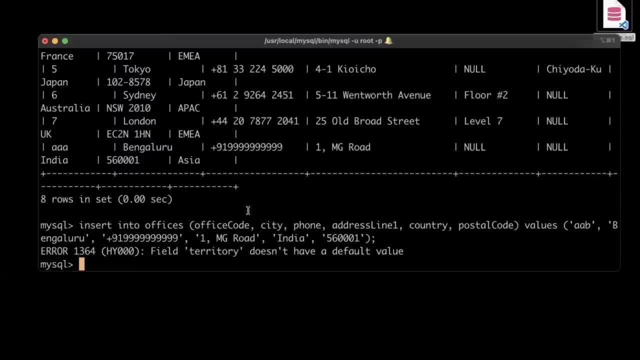 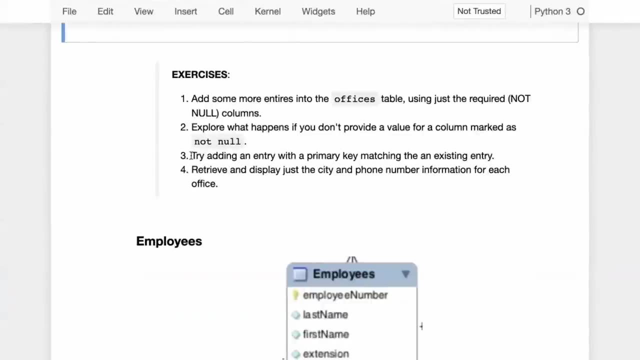 So look through it and try to break things and try to become familiar with errors so that when you encounter them, you will be able to debug them more easily. Try Adding an entry with a primary key matching an existing entry. So maybe let's try that. 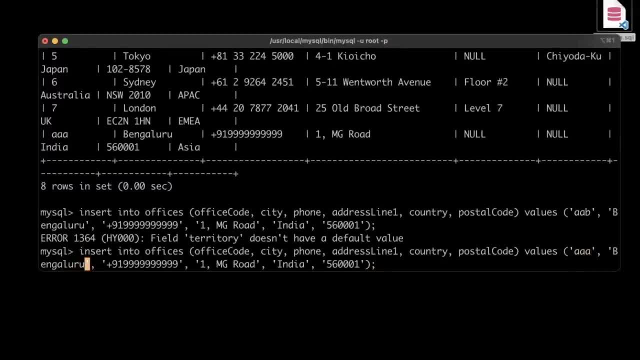 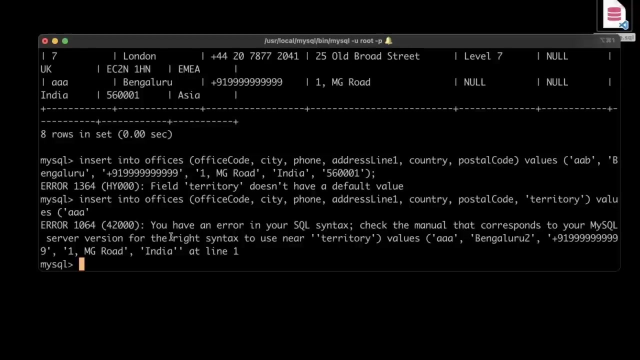 Let's try putting in AAA again and let's just make it Bangalore too, And let's just put in territory Asia here and let's add back territory here. So you will now see that. Okay, I probably have. Yeah, there's probably a syntax error here. 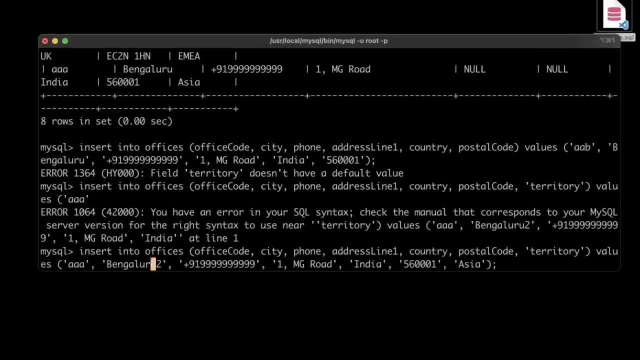 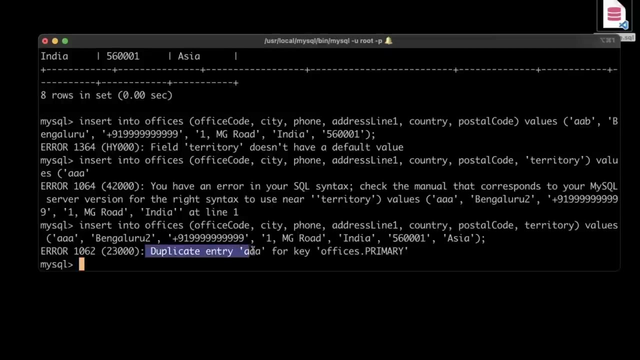 Okay, I made a syntax error here somewhere, but if I just try to insert the same data again, like a Bangalore too, you will see that now it says that there's a duplicate entry, AA for the key offices, dot, primary- and that data is not inserted. 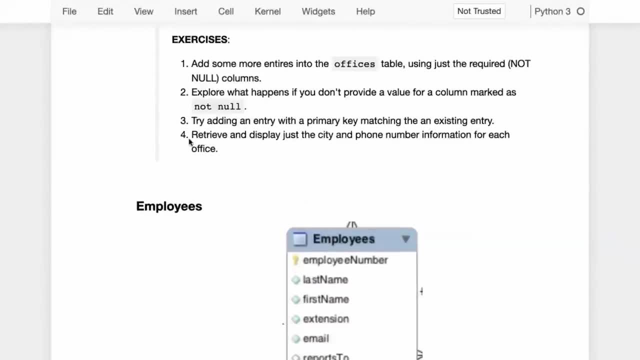 Okay, So test these out. The more you try, the more, the better you will understand how some of these things work. Okay, So let's try it. Okay, And try and retrieve and display just the city and phone number information for each office that has been created. 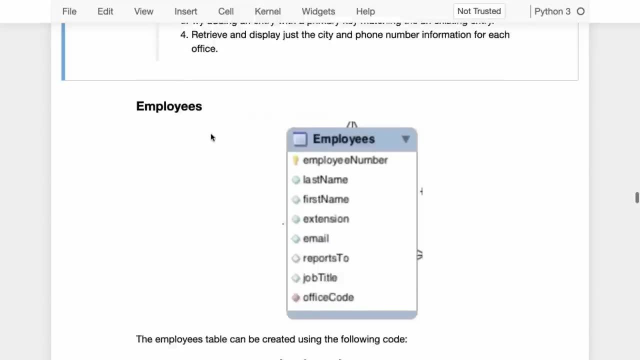 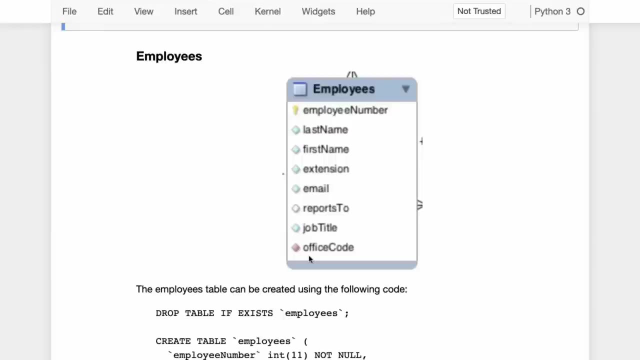 So just do a select statement and try that out too. And that's the first table that we've created. We've put some data into the table, We have looked at the structure of the table and we've retrieved some data from the table as well. 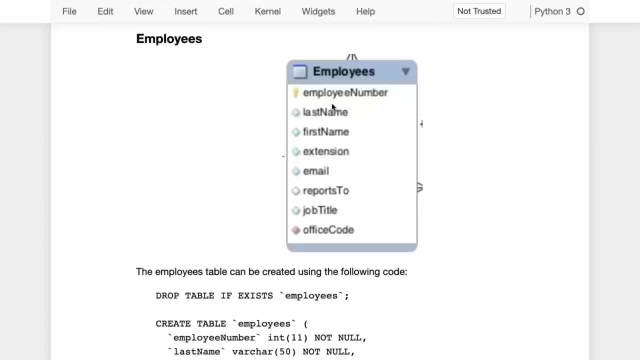 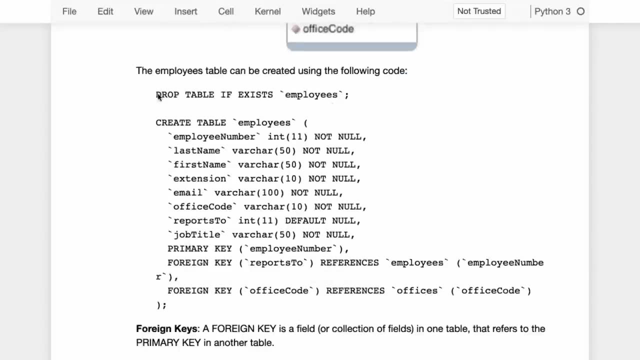 Next is the employees table. So we've created one table and now we are creating a second table and we will connect this table to the first table. Uh, and a quick note: if you want to First delete a table, then you can use drop table. 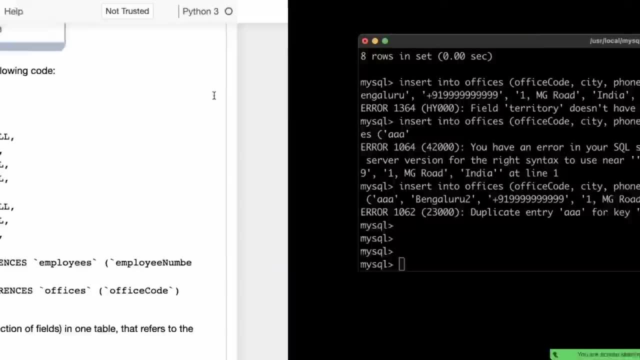 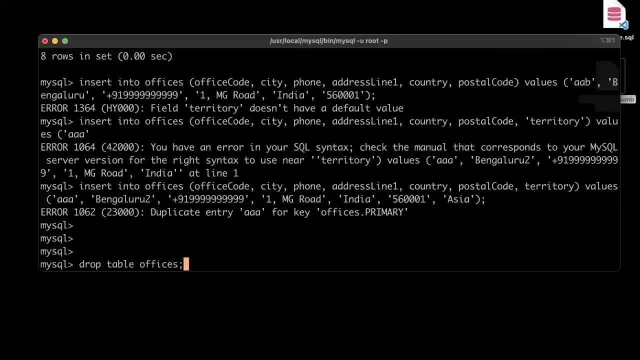 So if you type drop table, that will delete the table with all its data. Like if I type drop table and then I type offices here, that's going to delete the offices table. I don't want to do that right now because I've put some data into it. 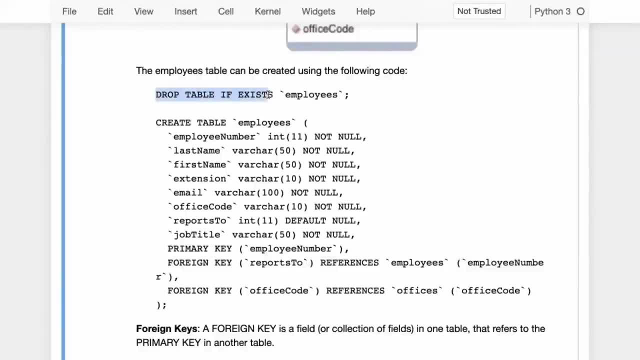 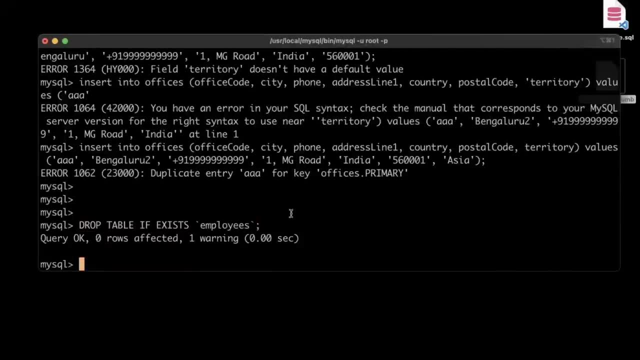 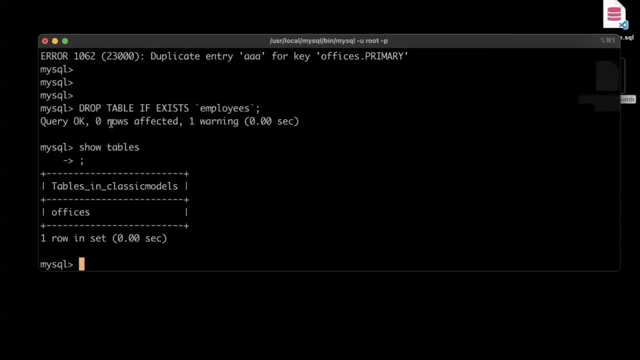 And you can also have something like this: that if the table exists, you can drop it. So if we type drop table if exists employees, this is not going to make any change because if I do show tables, Okay, There was no employee stable before and there's no employee stable now, but whenever you're creating a table, you can always- it's a good idea- to first maybe drop the previous table. 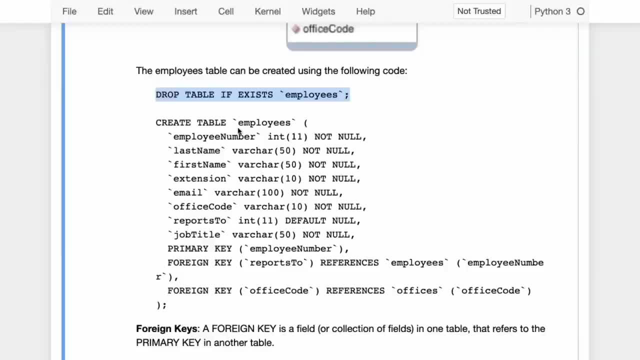 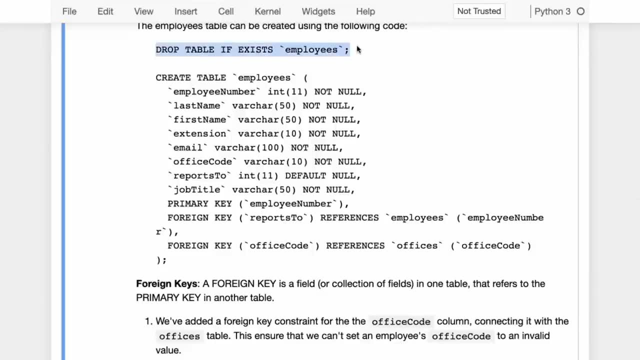 If you're sure that you don't need the old data, if you want to fresh table to be created, so you can just drop the previous table, if you, if you want, Right? So that's why we have the statement here for you as well. 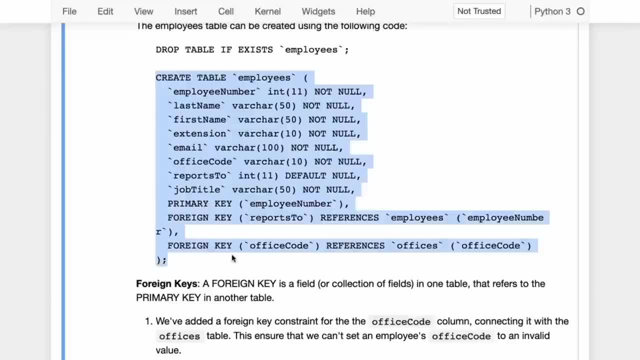 So, okay, let's talk about creating the table employees. So let's copy this code and here we have an employee number. So that's an Integer- our first encounter with integer- and here we're saying 11.. So I think what we are specifying here is- I think it might be 11 bites or 11 digits. 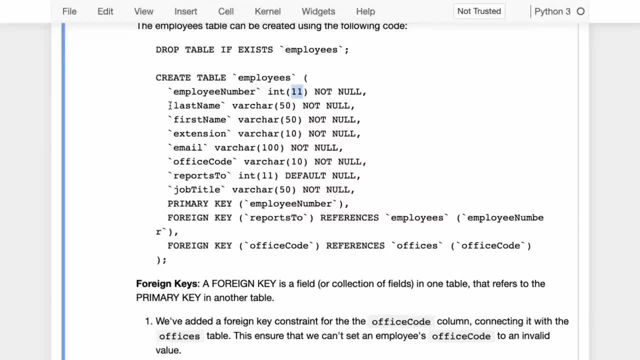 I'm not sure. I think it's going to be 11 bites. I'd have to look it up. Then we have the last name, which is a vat care or a string. A first name is a string extension. This is their phone number extension. 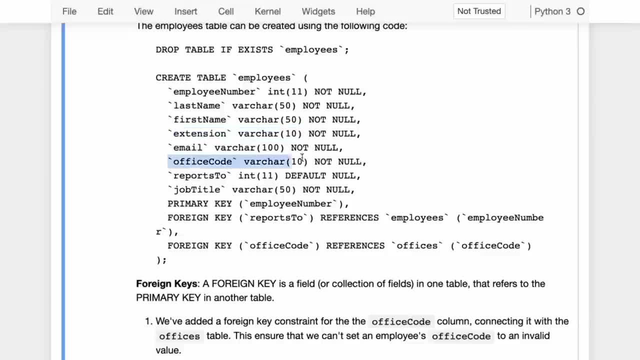 So they will be at a certain office, and that's why we have office code here. And then we have an email, which is again a vat care Of a hundred, and then we have a reports too. So two interesting things here. 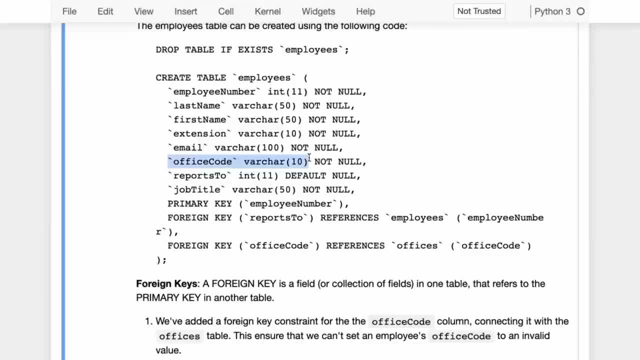 One is office code. So we have now our office code column, and this should ideally contain a value of a valid office code. How are we going to ensure that we will see in second reports too, and this can be null. So office code should not be null. 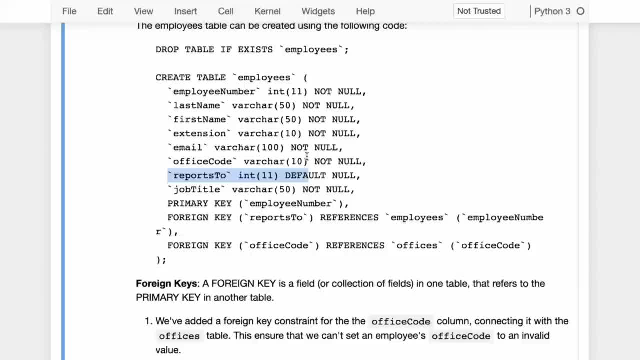 Every employee belongs to an office, but reports too can be null, because obviously there will be somebody in the company who does not report to anybody, But otherwise reports too, and maybe some people may not have been assigned a manager or a reporting person. So reports too can be null. but reports too should be somebody's employee number. 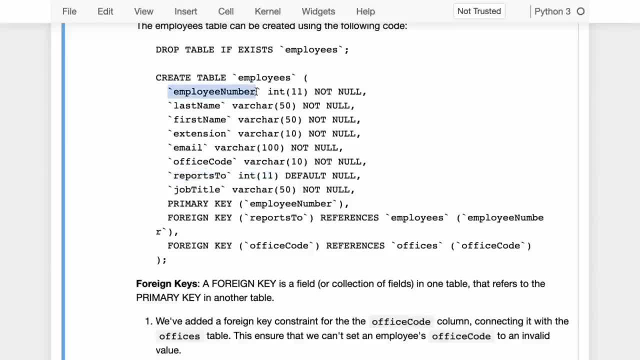 Let's say, um, you have Siddhant and Barrage, and if Barrage reports to Siddhant, then reports too. in the entry for Barrage should be the employee code or the employee number of Siddhant and Barrage. 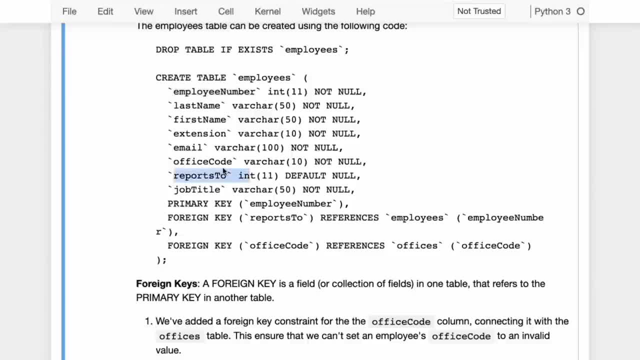 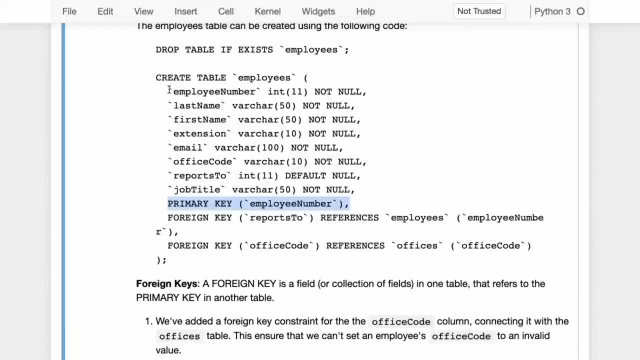 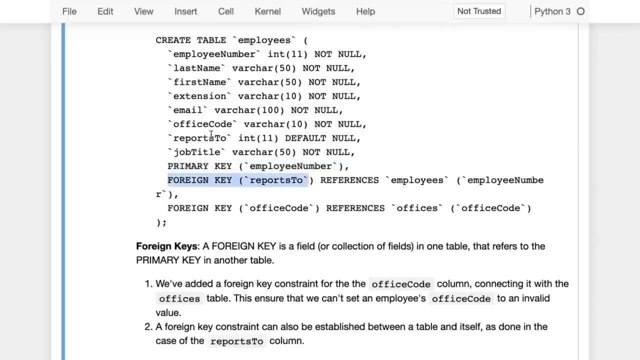 That makes sense. We want to uniquely identify each employee with a primary key, and this was going to be not null, So that's fine too. And then we have these two, two statements, foreign key. So here we are saying that reports to the column reports too. 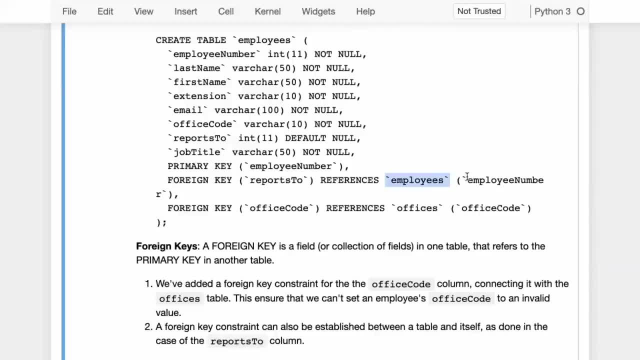 References the table employees and in the table employees it references employee number. Okay, That's one. And then we have another foreign key office code. So here we are saying that the tape, the column office code in this table, references the column office code from the offices table. 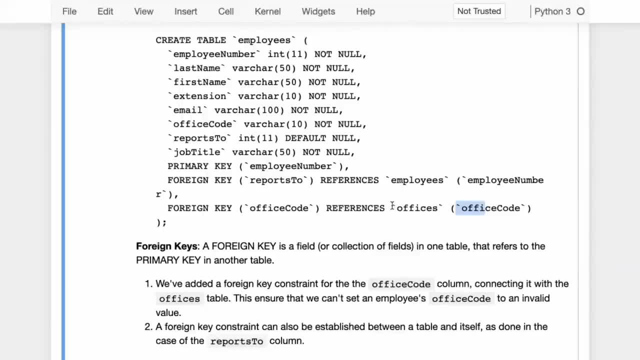 Okay, So there are two references here. One is a, one is a reference to another table. One is the reference to this table itself, but probably to a different record. So what we are saying through this or through a foreign key, in general, 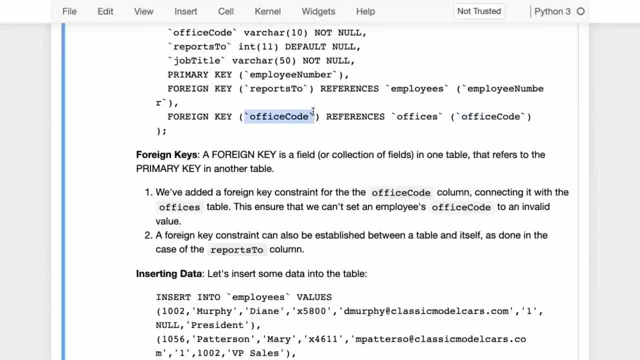 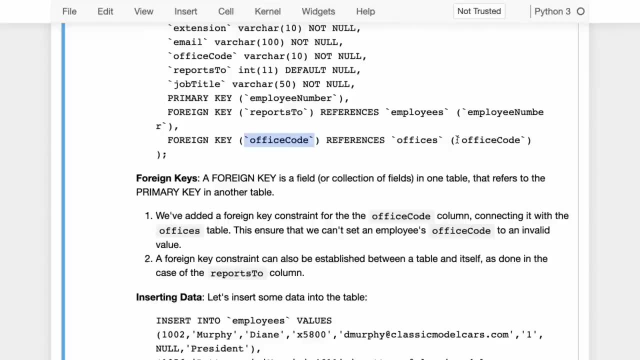 is that we want to ensure that the office code column contains a value which matches a value in the office code column from the offices database or from the offices table right. So for every employee there should be an office code and that office code should contain a valid 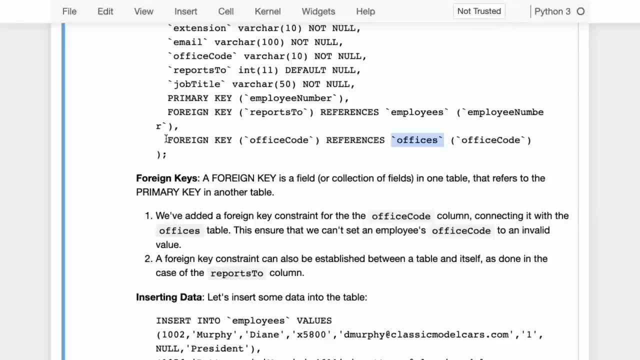 value from the offices table, And that is what the foreign key constraint ensures, And we will test it out in just a bit. And then, similarly, we have a foreign key within the same table. We want to say that the reports too, for any employee should be a valid employee number from the 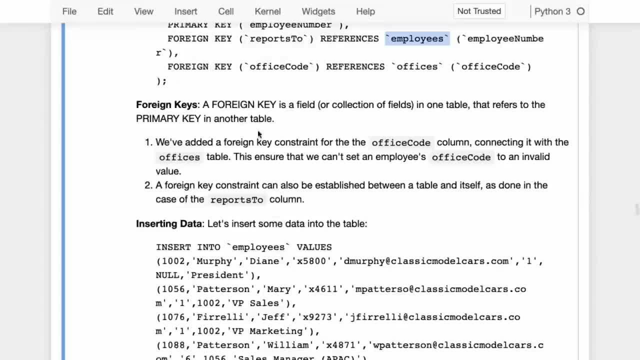 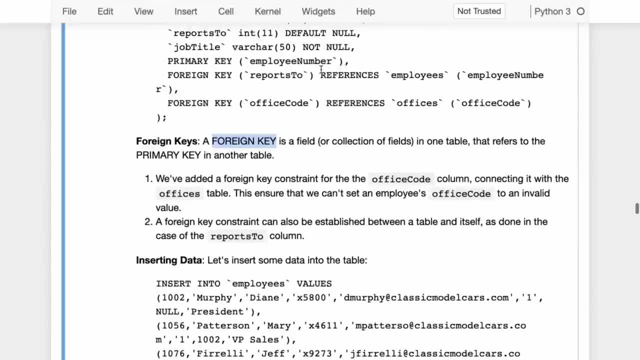 employee's table and it can be the employee number of a different employee. So that is all enforced. using a foreign, A foreign key is simply you're saying that this number or this column has a special property, that it refers to a value from another table. 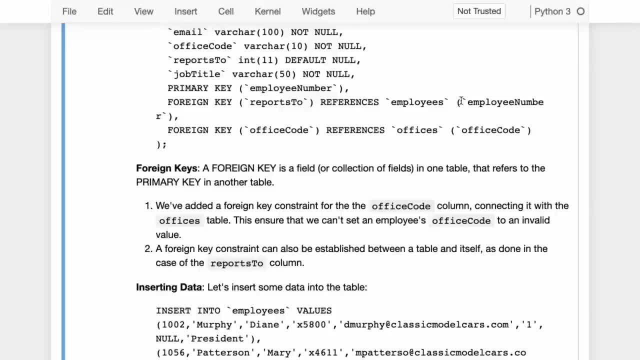 And there is one important constraint with foreign key: The value that you reference to must be the primary key in that table. So, for example, here we are referencing office code of offices. So office code must be the primary key In the offices table. 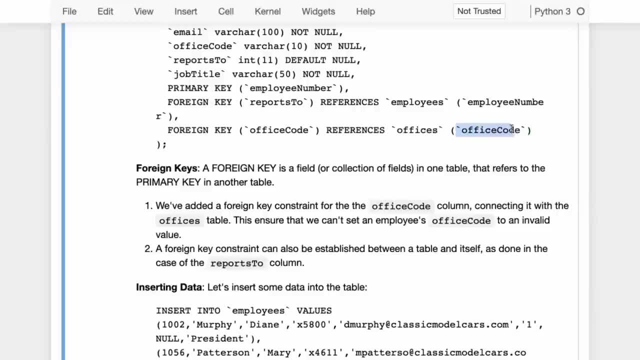 Now again, this is not a criteria that all SQL software or the or all relational databases have. Sometimes they do, Sometimes they don't, but in general, just to be safe, you should always assume that you should only reference primary keys. 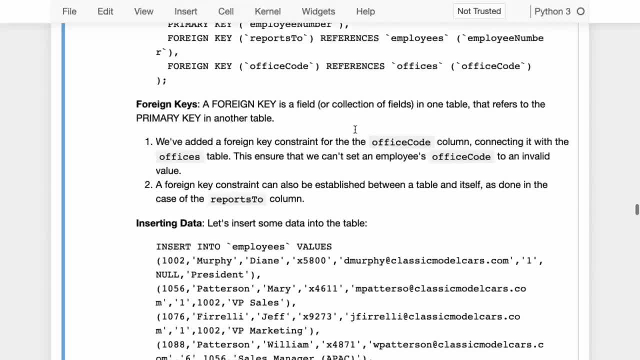 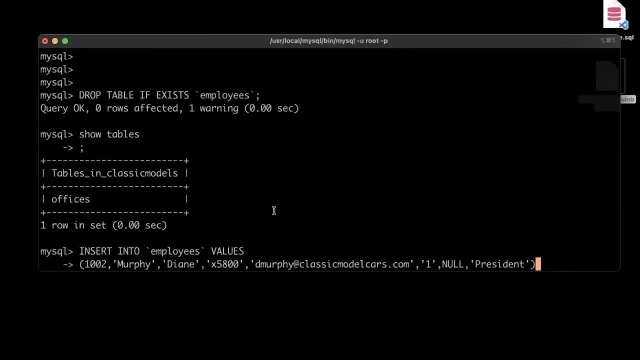 Okay. So let's try it out, Let us insert a value into employees. So let's just- let me just grab this- insert into employees the values one, zero, zero, two. So that's the employee code: Murphy Diane X 5,800.. 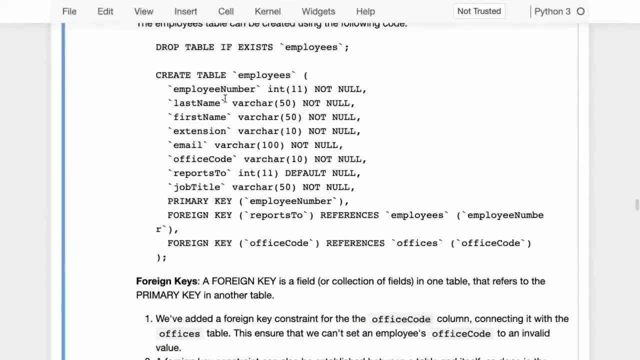 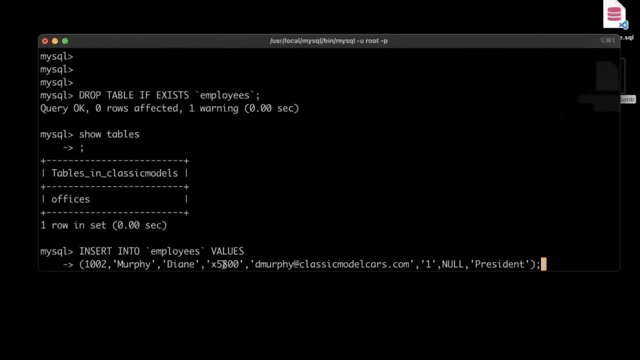 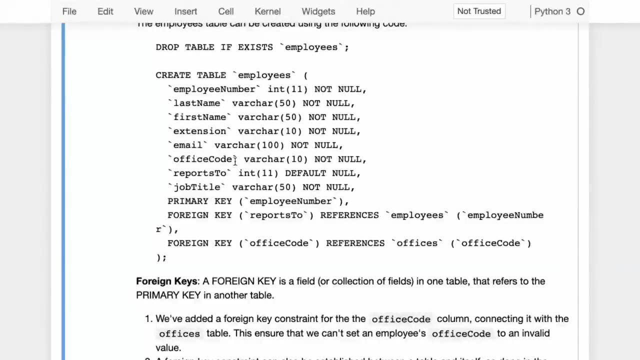 And so this is what is this: employee number, last name, first name, So Diane Murphy, one zero zero two, and their extension is 5,800 and their email is D Murphy at classic model carscom, then their office code is one: 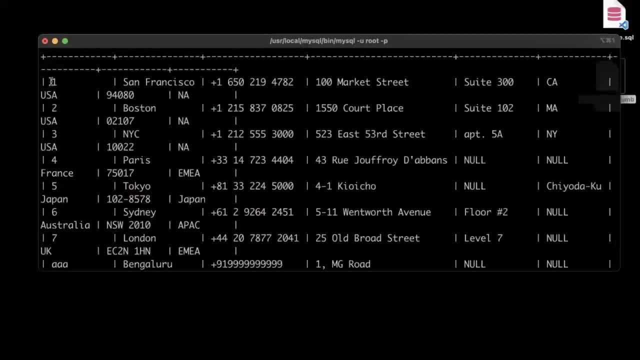 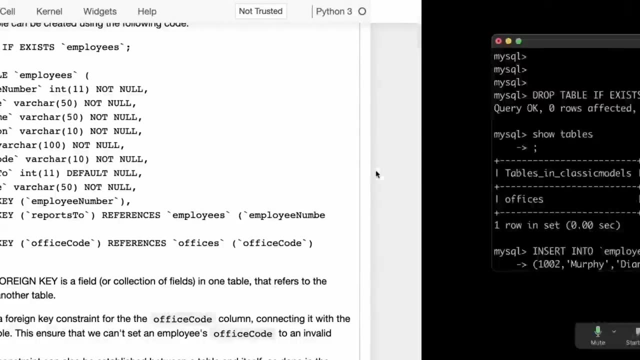 And do we have an office code one? We do have an office code One. one is San Francisco, So that means they belong to the San Francisco office, Then reports to none, So they do not report to anybody. And in fact Diane Murphy is the president. 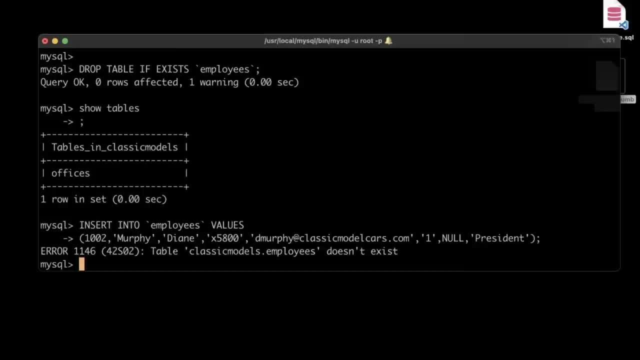 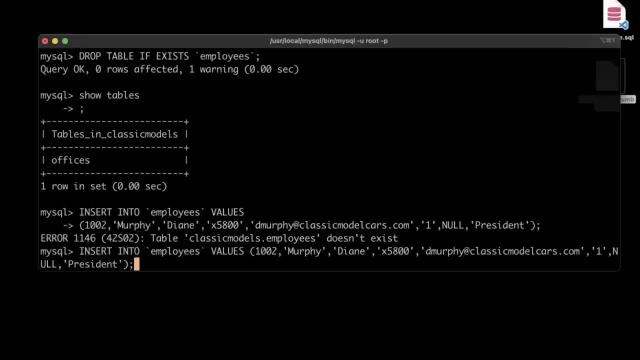 So they're the boss, So let's run it. Oh, it says employees doesn't exist. Oh, that's because I dropped the employees column. I never created it in the first place. All right, So let's first create the employees column. 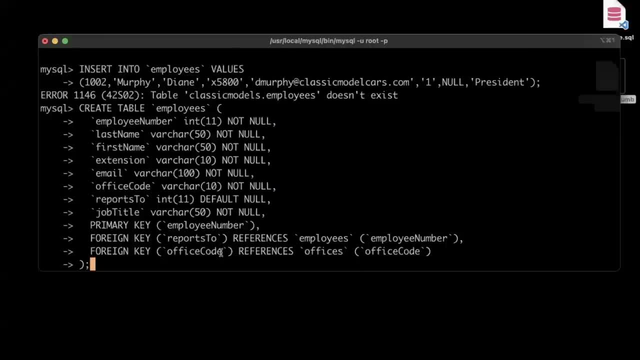 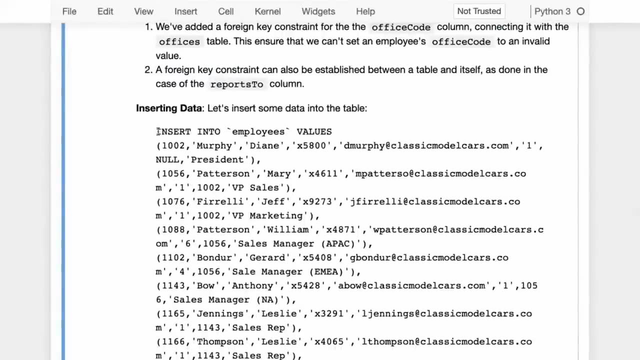 Okay, So let's create table employees. Let's take this and let us run it here. So now the employees column is created and then let us insert some data into the employees column. I am just going to insert this one person right now: Diane Murphy. 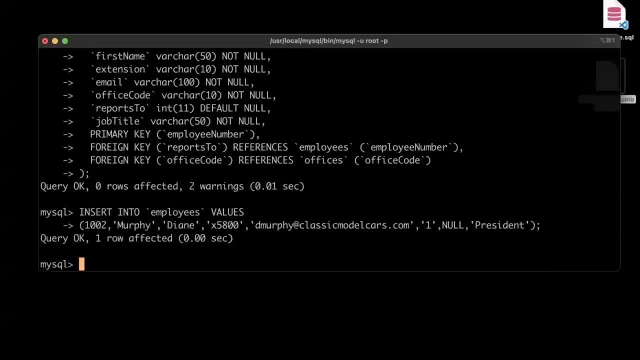 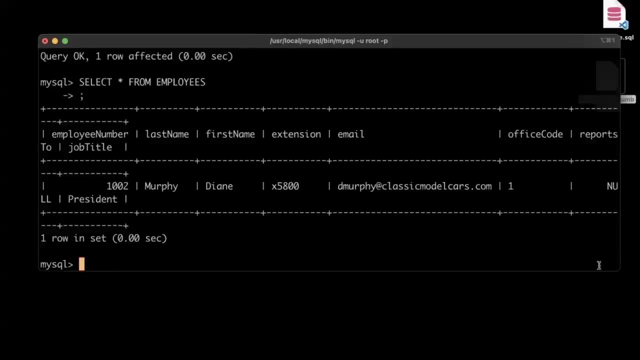 and that's it. And let me just put a semi-colon here and insert the person. It's not if I do select star, Okay, Okay From employees. you should be able to see. sorry about the formatting, but you should be able. 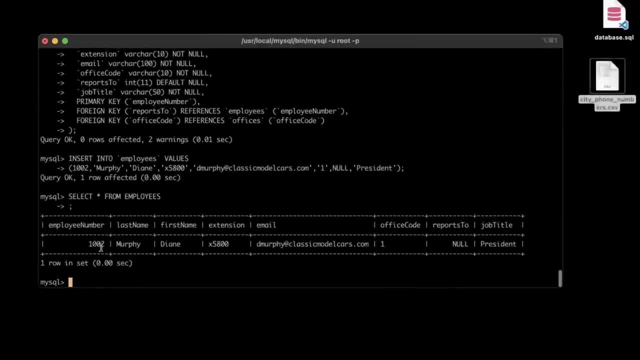 to see this information about this person. Diane Murphy, with the employee number 1 0 0 2, has the office code one and reports to nobody. Let's add another employee, Maybe. let us say there: yeah, let us set their office code. 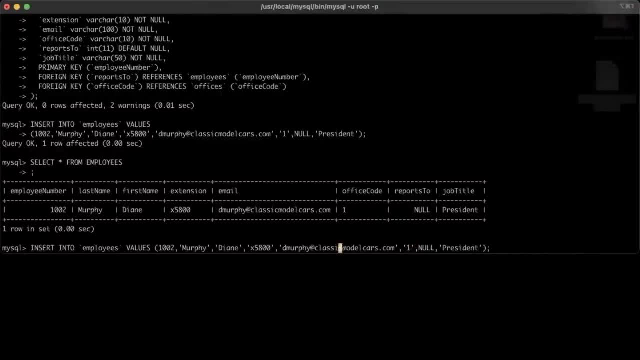 So let's set their employee code to 1 0 0 2 or 1 0 0 3, and let's call it Daniel and let's give an invalid office code here. Maybe let's give a hundred and let's see what happens. 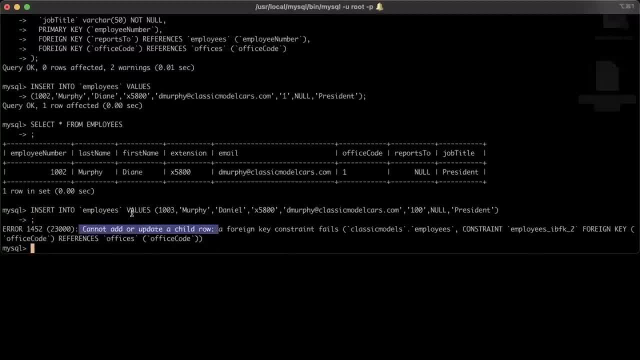 So here you will see that it cannot add the child row. So this is called a child to the employees, now called a child of office, because it has a child of office. This is a foreign key constraint and the foreign key constraint fails. You can see that the key, the foreign key constraint that this should be a valid office ID. 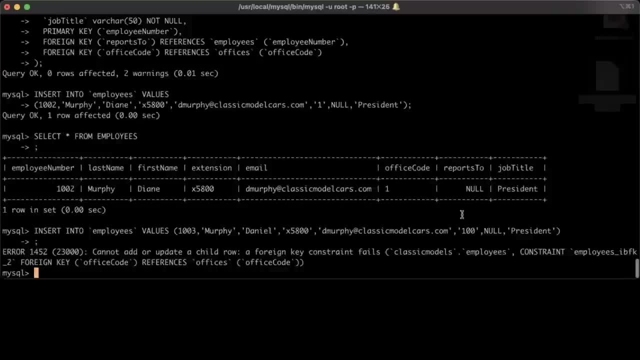 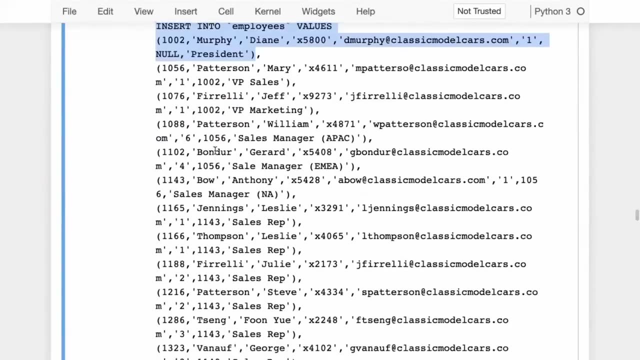 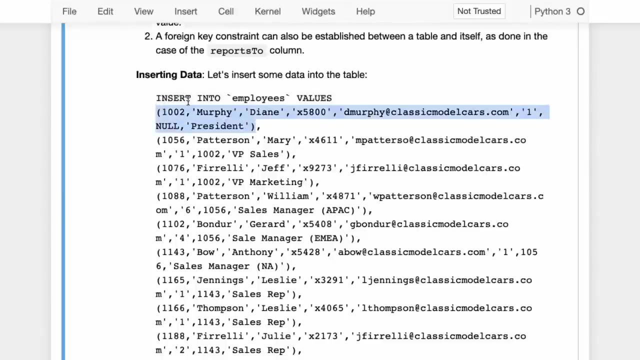 fails And that's why you cannot add that row again. That's how the whole thing works, All right. So maybe let's add all these employees and then we will move forward. but to add all these employees, there are going to be some issues, because I've already created an employee with. 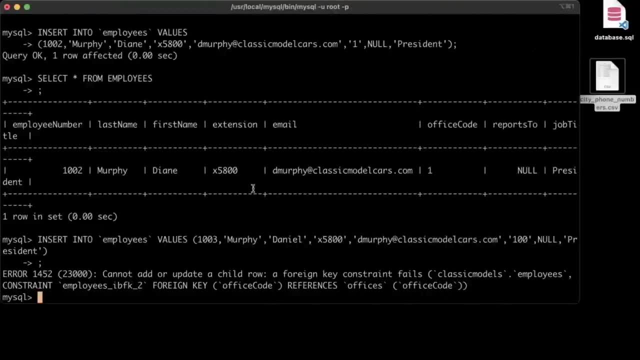 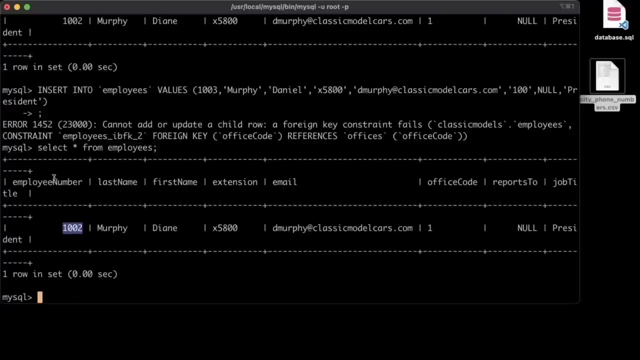 the primary key 1 0 0 2.. So before That, I'm just going to delete the employee that I've just created. You see, right now I have this one employee, Diane Murphy, So I want to delete the employee with employee number 1 0 2.. 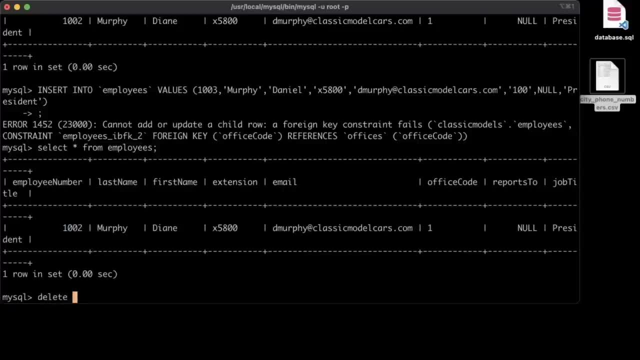 So I can say this, I can say delete. Well, actually, let's come back to delete later. for now I'm just going to drop the table entire entirely. So drop table Employees, Okay. So now the table employees is gone. 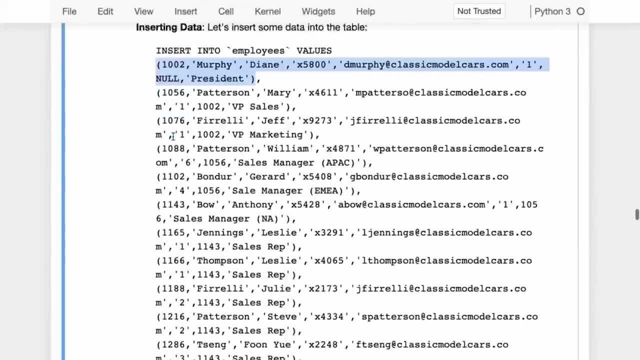 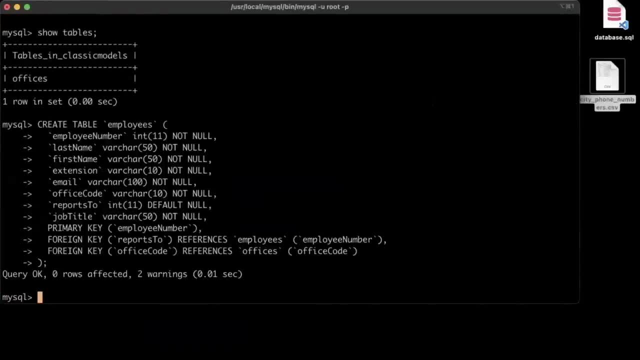 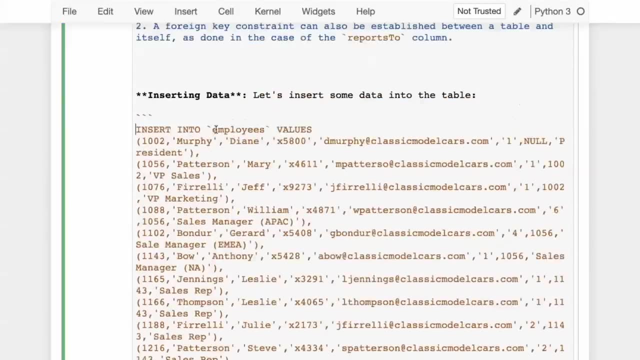 If I do show tables once again- and now I can create the table Once again- I will go create table employees and then let us insert all this data. So we have a bunch of employees here. I'm just going to capture, cap, copy all of this and paste this command. 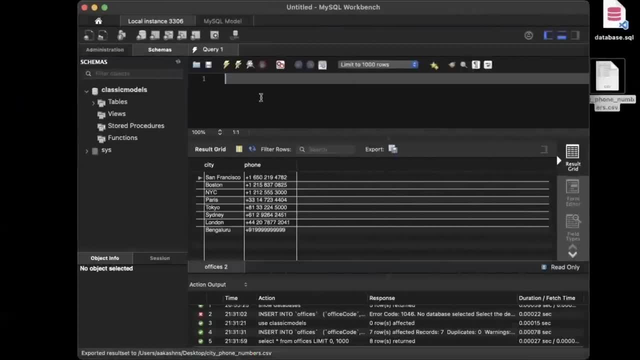 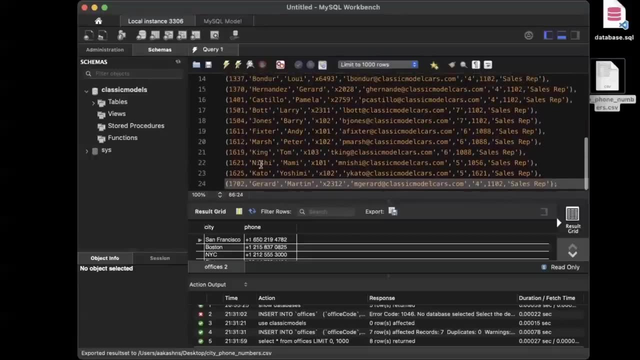 If you want to do the insertion here, So maybe let's just do the insertion here. So we're just going to insert all of these employees. How many are these? We are going to insert about 23 employees using the my sequel workbench. 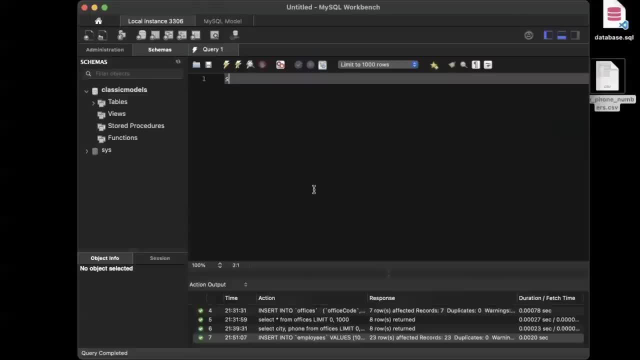 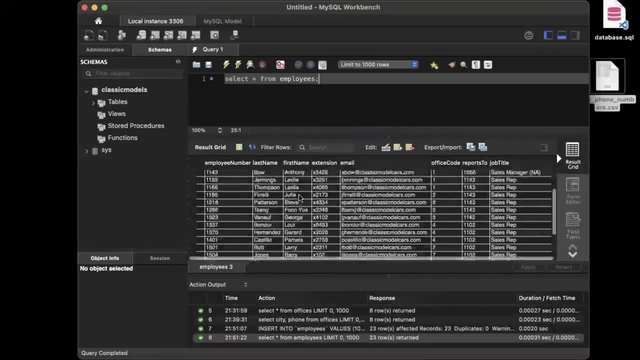 And now they should be created. So now, if we check sure, select star from employees. you should now be able to see: Okay, Okay, Okay, Okay, All the employees that we've created. Okay, Now here are some exercises for you. 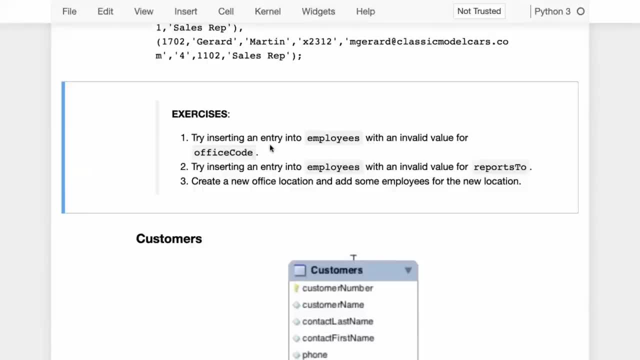 Try inserting an entry into employees with an invalid office code. You saw what happened, but try it Maybe from the workbench. try inserting an entry into employees with an invalid value for reports too. Okay, That is something that we haven't tried. 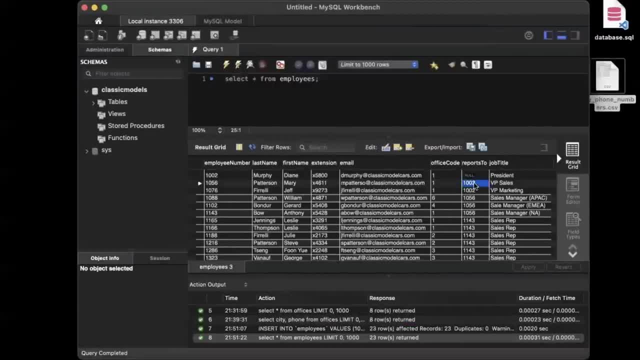 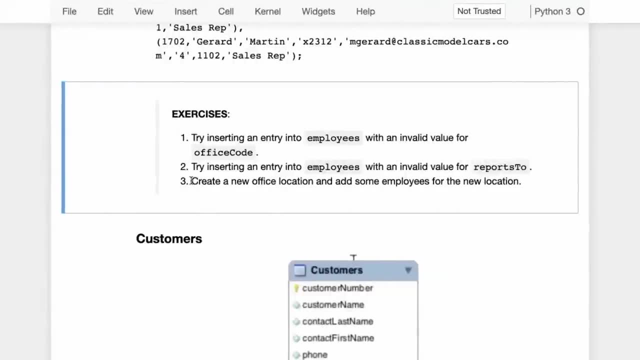 So reports to can either be null or it must be an existing employees ID or employees Number. And try this. try creating a new office location first and then try adding some employees to the new location. So when you open a new office first you will have to add a new office object or a new office record. 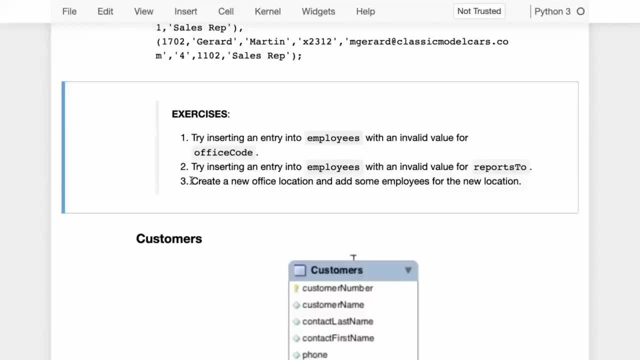 And then you will have to add an employee, add a bunch of employees for those office records, And maybe you will have one office manager and that office manager will probably report to the president, And then you will have a bunch of employees at their office and they will report to that office manager. 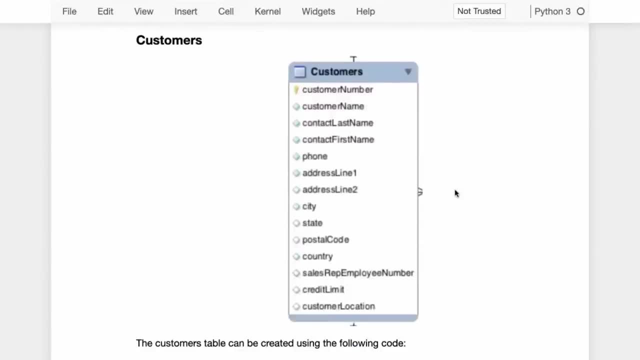 Okay, Do try out that exercise. Okay, Moving ahead, Now we have the customer's table. So now, by this point you're probably getting the idea. There is a primary key, There are a bunch of required columns, There are some optional columns and then there are there is some. there is this foreign key. 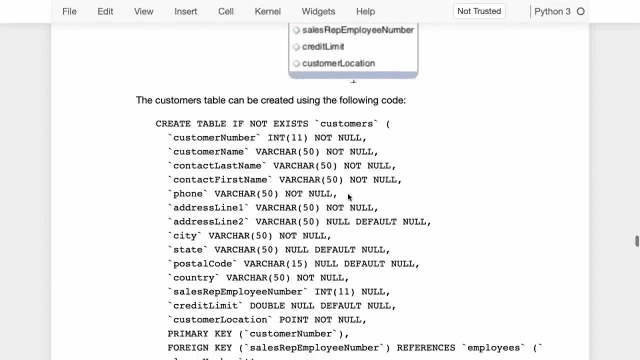 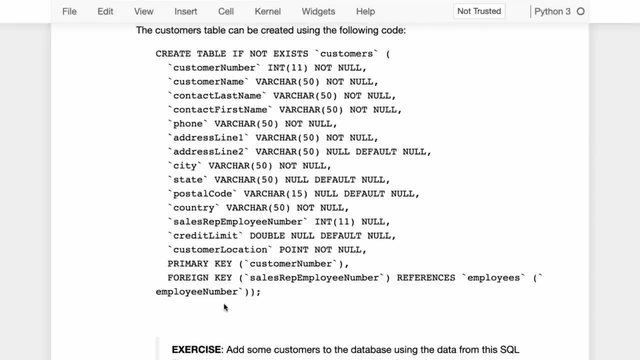 So every customer has a sales rep, optional sales rep. So you can take this foreign key sales rep employee number and that should reference in the employees table some employee number And you can see here that sales rep isn't it Integer but it can be null. 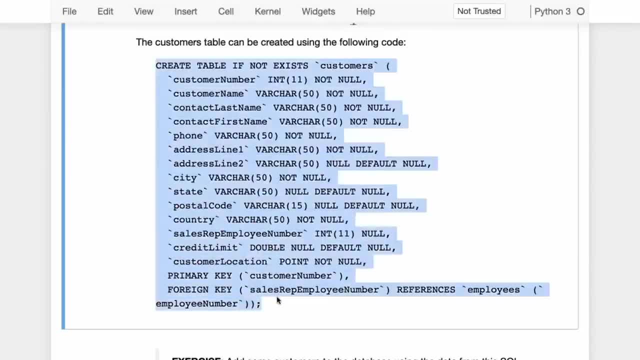 So I can just copy paste this. I can take this: create table if not exist. So this is another way to go about it: create a table only if it not, it does not exist. All of these are slightly different If you try to create a table without this. 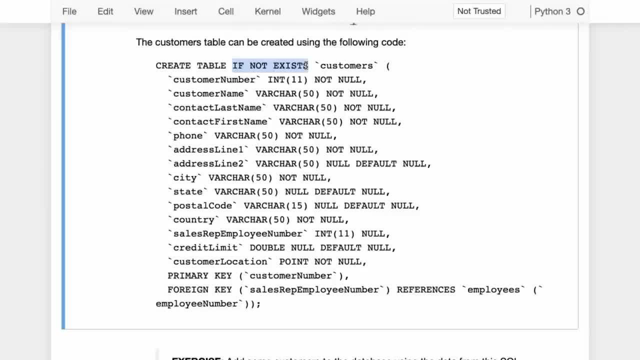 So if you just say create table customers if there's already a table customers, it's going to fail. If you drop the table first, then it's going to delete all the data. If you say create table if not exist, then if the table exists it won't do anything. 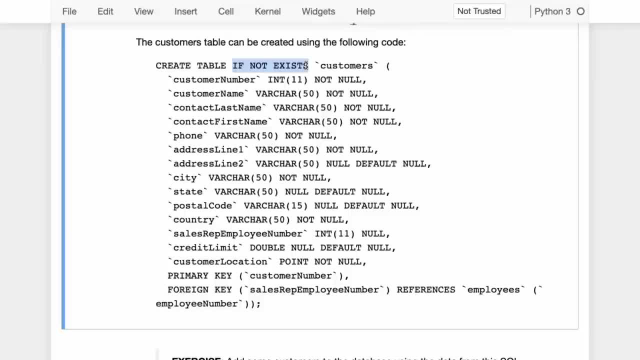 If the table does not exist, It is going to then create the table. So think about what is the right thing you want to do And, based on that, use these. drop and not exist and does exist, and play around with them and see what they do. 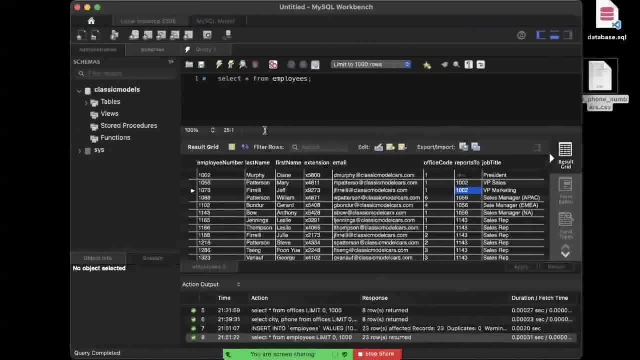 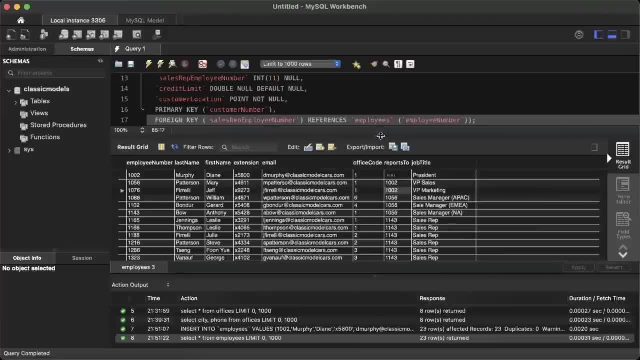 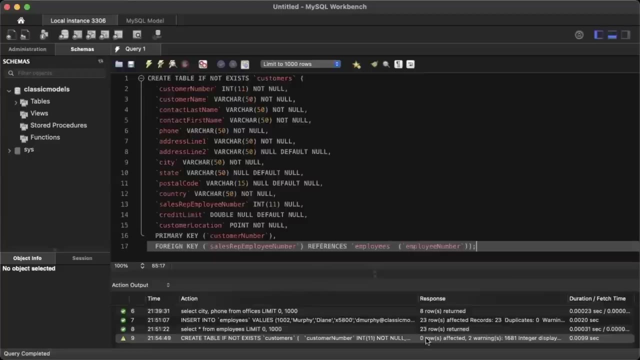 Okay, But I'm taking, I'm going to take this create table, put it into my work bench and just executed And this should create another table. Yeah, This should Create another, another table, customers, And on the left, if you just check the schemas tab, you should be able to see all the tables that are present. 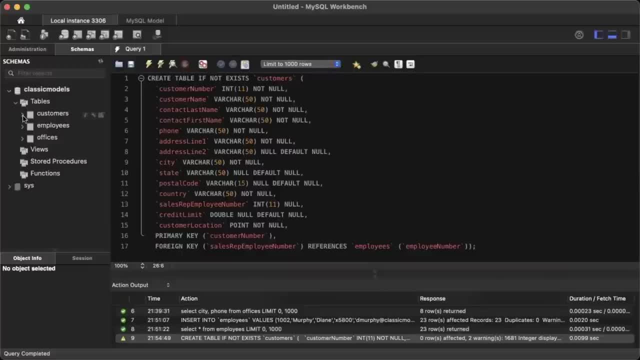 So now you see here you may have to refresh it a couple of times, but you have this customer's table, You have employees and you have offices, And when you click on a table, you will also be able to see the information about that table, like on customers. 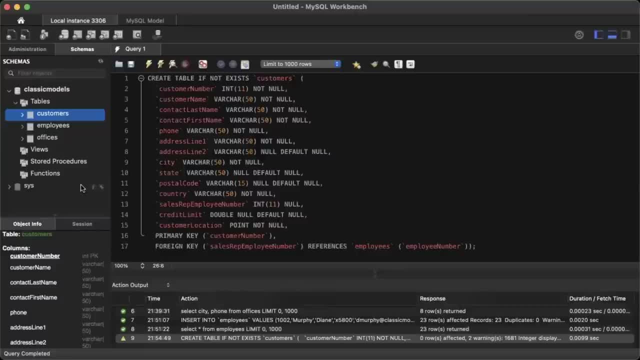 You have customer number, customer name, last name, first name. So this is how my SQL work bench makes it a little easier for you. You don't have to type a lot of commands Like describe and such. you can just browse the tables that are there. 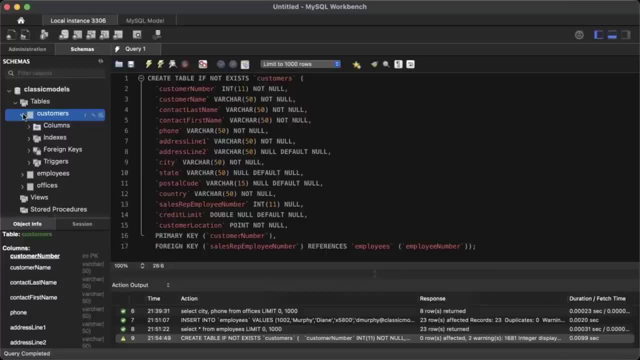 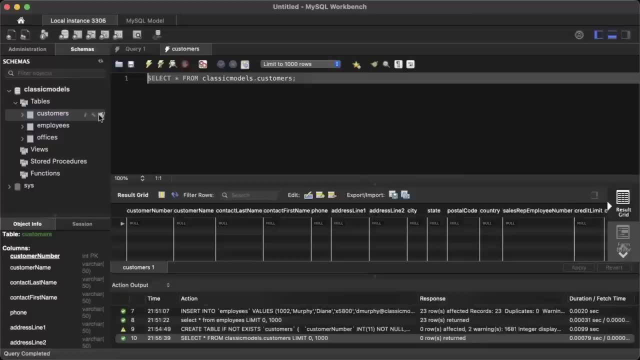 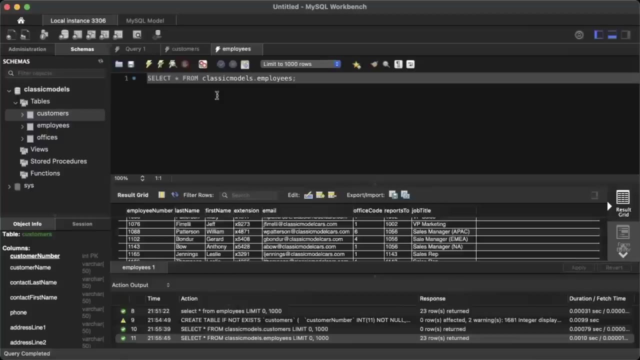 You can also browse the information about the tables. You can, in fact, even check values within the table. I believe if you would just click this button, it is going to automatically run this select star for you. So if I just click this button here, it's going to show all the employees by running a select star from classic, from employees. 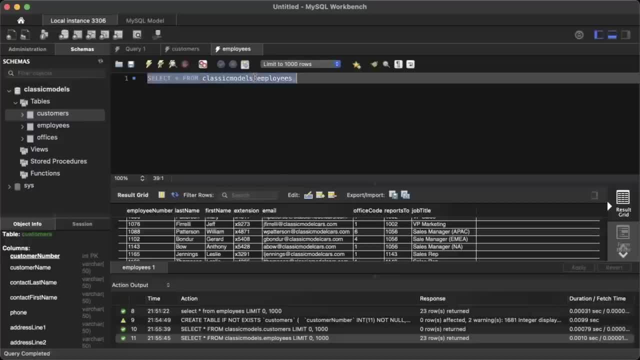 Right, And this is one other way to write, something you will see often. You can also type database name, dot column name or, sorry, dot table name and then put a query. So if you're not already set a default database using the use command, like use classic models, you can just put select star. 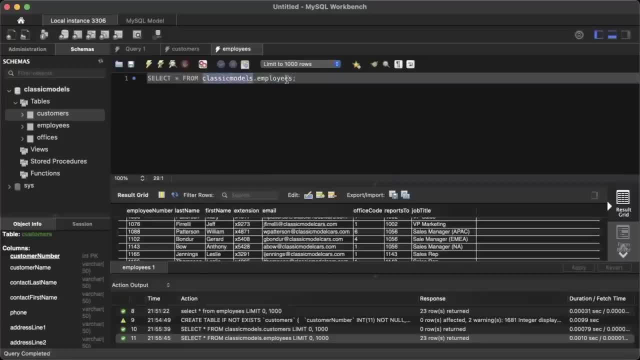 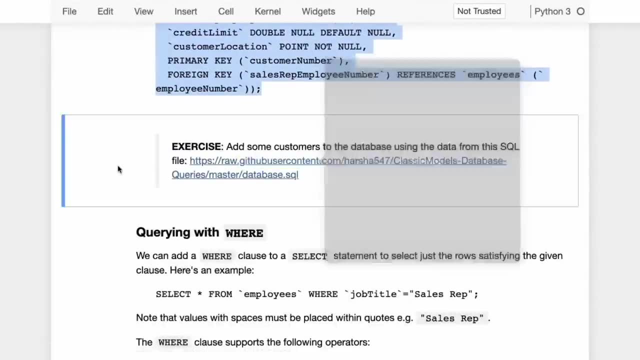 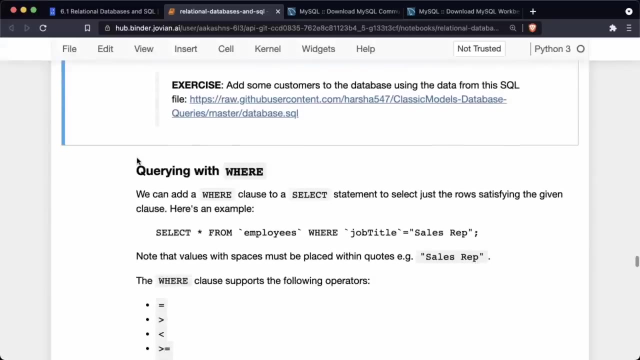 from classic models: dot employees. So this is database. dot table name. Okay, So here's an exercise: add some customers to the database using data from a SQL files. Somebody asked what to do. Oh, okay, Can you get data at data programmatically? 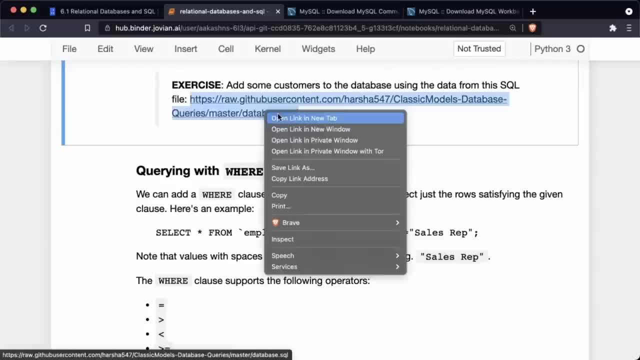 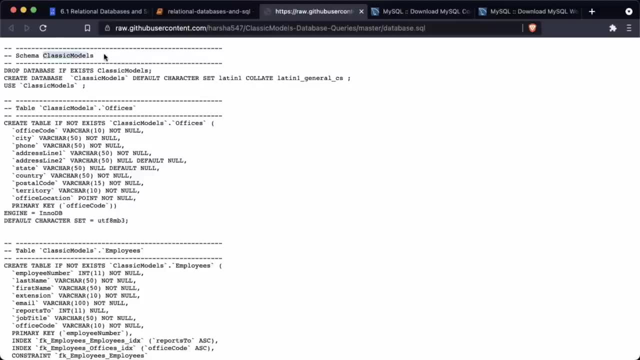 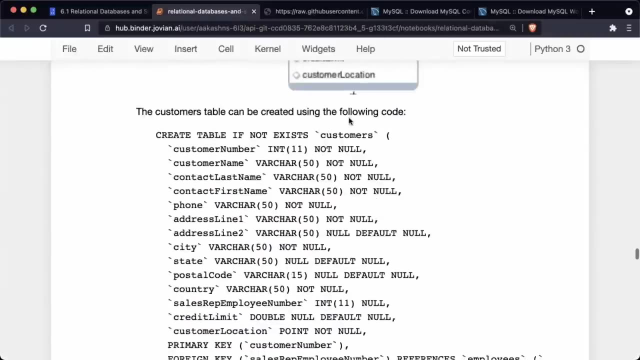 Can you add data which is already there somewhere else. So let me open up the SQL file, and this equal file contains code for everything that we are doing today, of this classic models SQL file, And in the SQL file you will find some rows for inserting data into the customer table. 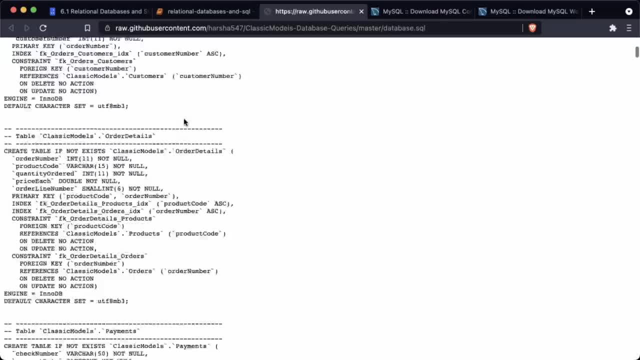 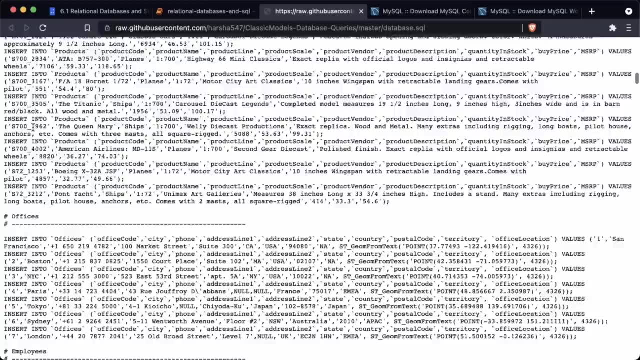 So let's find it, Let's see. So here we have a bunch of create table statements, Then you have these insert statements for customer, For products, And then you have an insert statement for offices, employees, and okay, here is where we have an insert statement for customers. 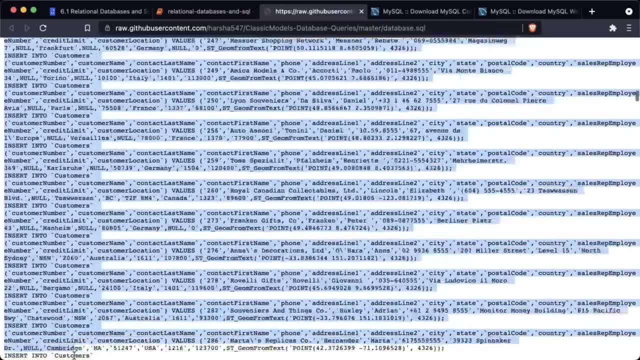 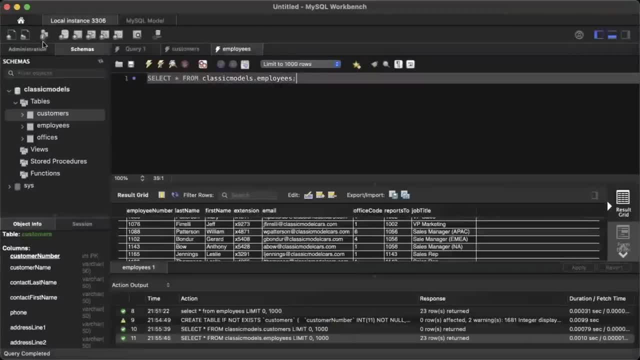 So I'm just going to grab this. This seems like a whole bunch of insert statements here, So these are all the insert statements for customers. I'm just going to go back to the work bench and I am going to do a new query. 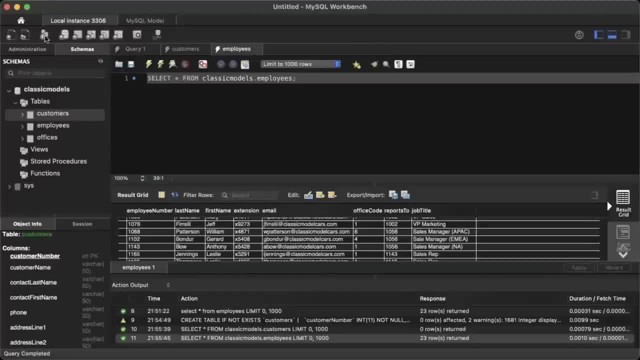 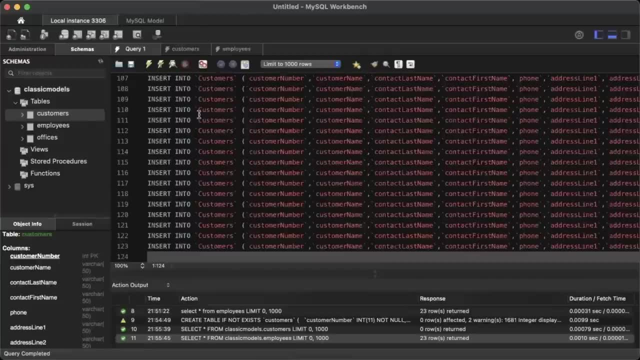 I think. not sure which one it is, I never mind, I'm just going to edit it here. I'm just going to go to query one, paste this, All right. So it seems like there's a lot of insert statements. 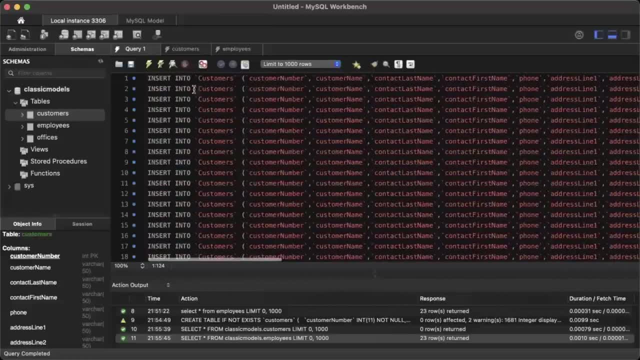 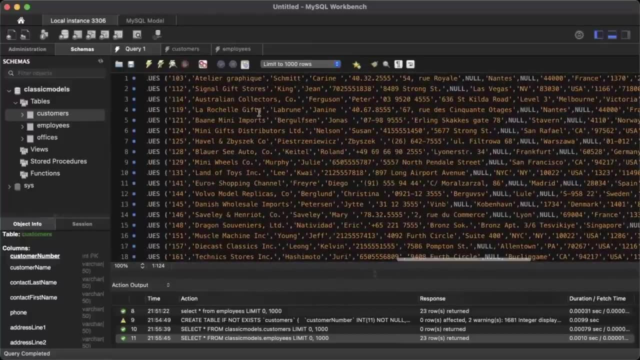 I'm not sure why they wrote it like this. They could have written it all in a single insert statement too, but in any case, we have 125 customers. You can see here you can see the details of these customers They are so these are typically customers, are stores. 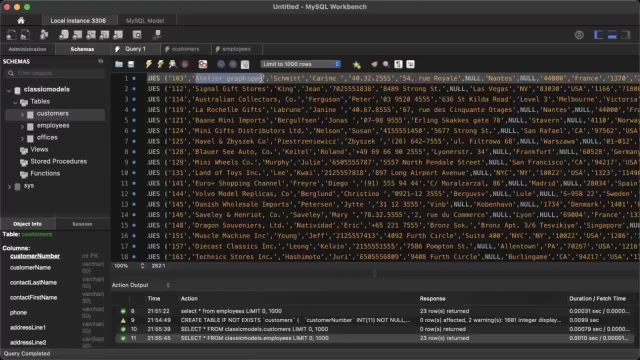 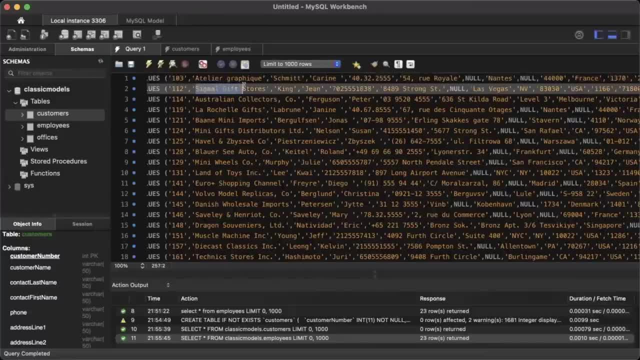 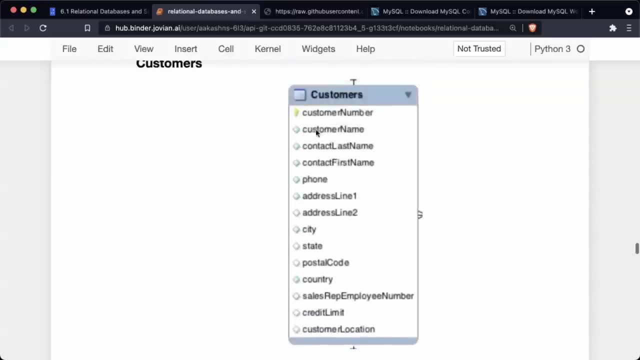 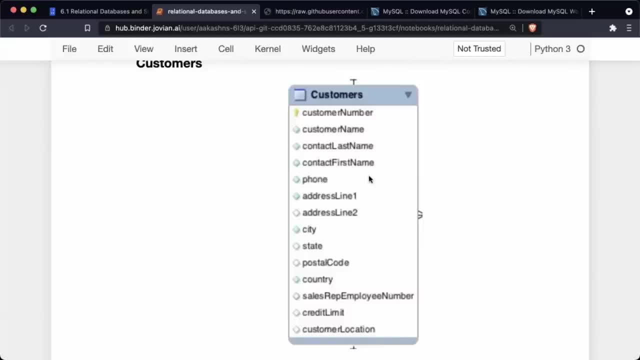 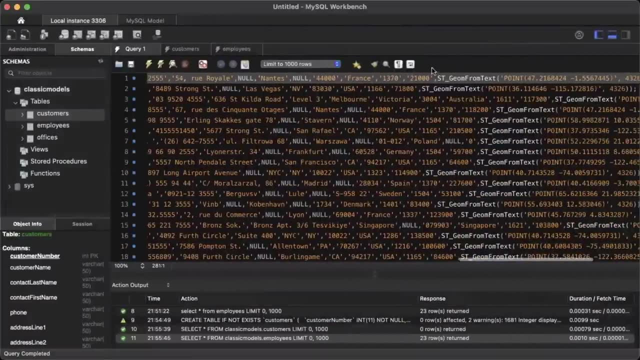 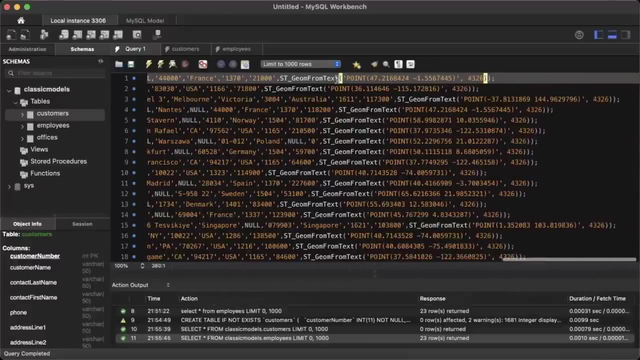 Customer name is a store name. Contact- last name, First name, is the information about who to contact their phone number, et cetera. So all that information is captured here. You will also see an employee ID, So this one is probably the employee ID and then you have: okay, so here there's also some kind of a look. 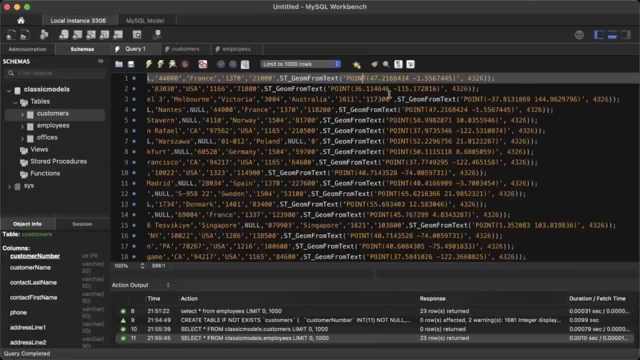 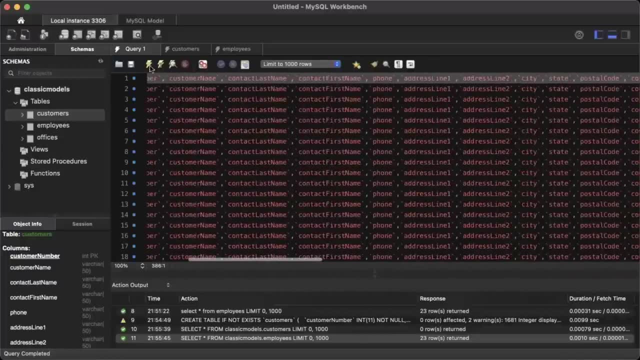 You see location or data, you see S T G, O, G, E, O, M from text, et cetera, So you can also put location data into my sequel. That's pretty interesting. So let's run this. Let's see if this gives it correct result. 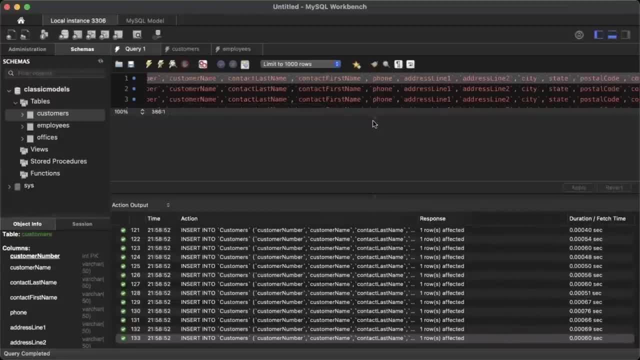 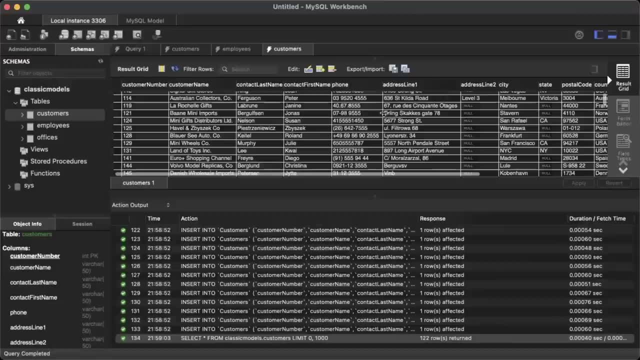 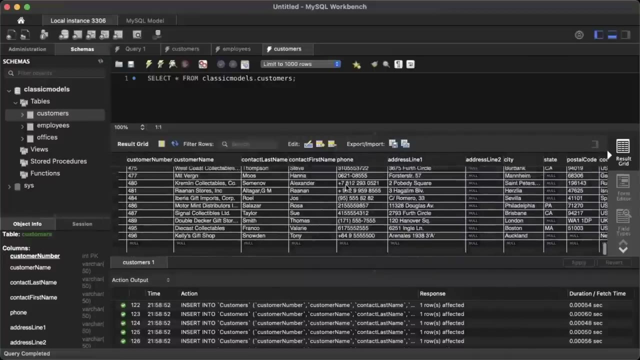 Yeah, It seems like it was able to insert data into the customer's table. All right, So now we've inserted data for about one 20 customers and we should be able to see that here in the response. Yeah, So you can see we have data for over a hundred customers and that's great. 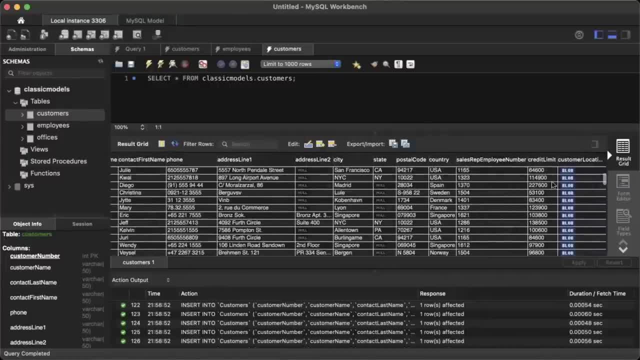 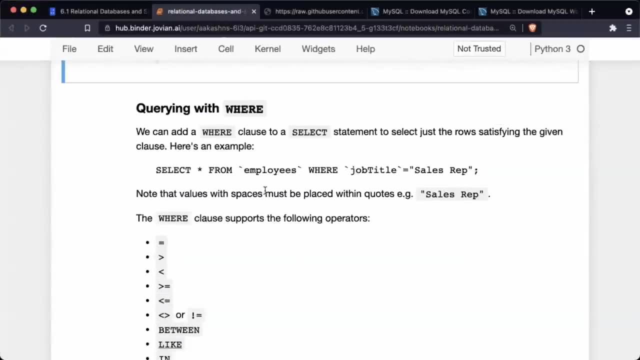 And some of them have a sales rep, Some of them don't have a sales rep. Customers also have a credit limit in such Okay. So now when you start getting to this point where you have a lot of rows in your database, then it may not make. 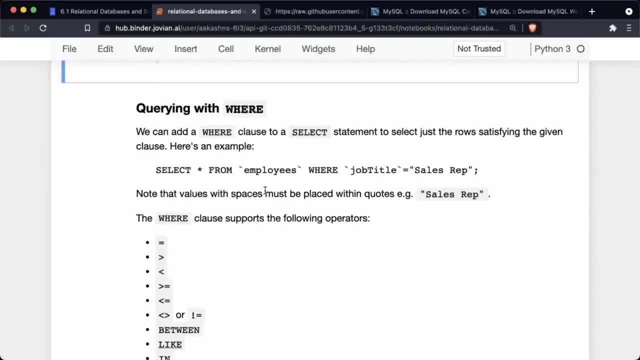 sense to look at all the data at once. That is where you may want to select some data, You may want to query some data, You may want to filter out data based on a particular condition, and that is where the where clause in the select statement becomes useful. 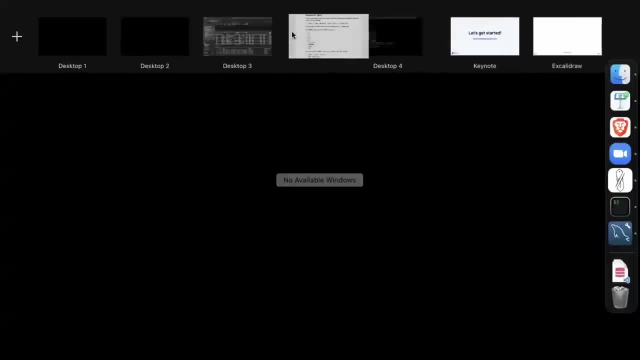 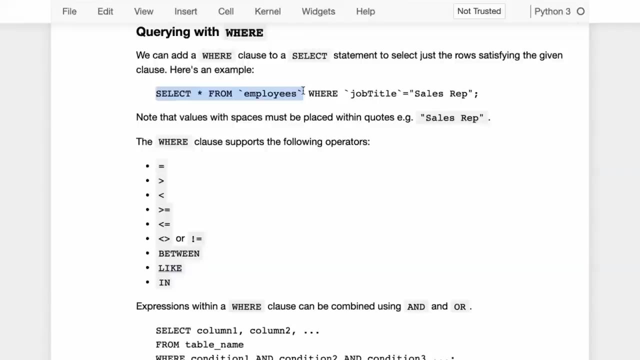 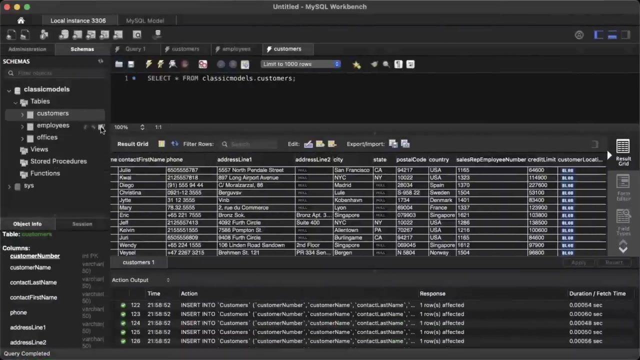 So you have this where clause, so you have this clause called where that you can include after your select. So when you say select star or select some columns from the employees table, you can say where job title equals sales rep. Now if you go back and check the employees table here you can see that employees table there is a job title here. 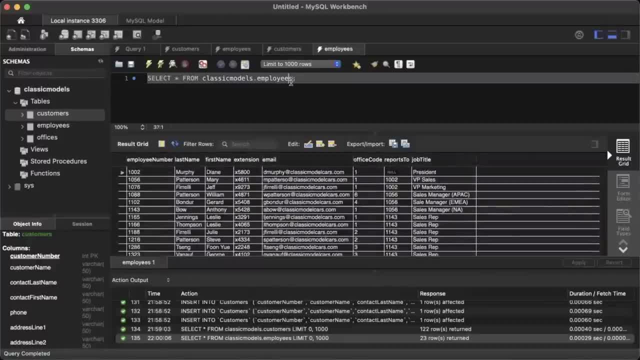 And let's say, if you only want to get a list of the sales reps, So we say select star from employees where job title equals And then whenever you want to put an actual value for comparison, you use double quotes. Very important sales rep. 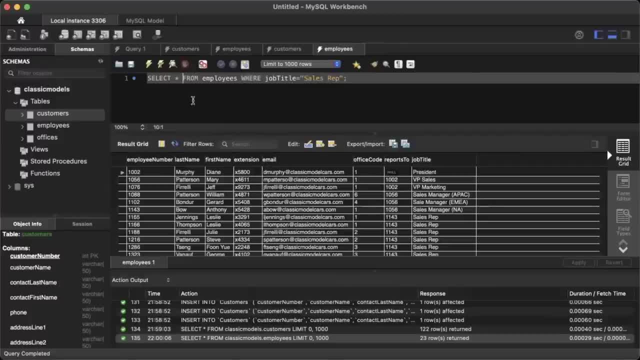 Okay, So select star from employees where job title equals sales rep, And maybe I can also select specific columns. So let's say I want, I just want to select the last name And I want to select the extension, or actually, let me just select the office code. 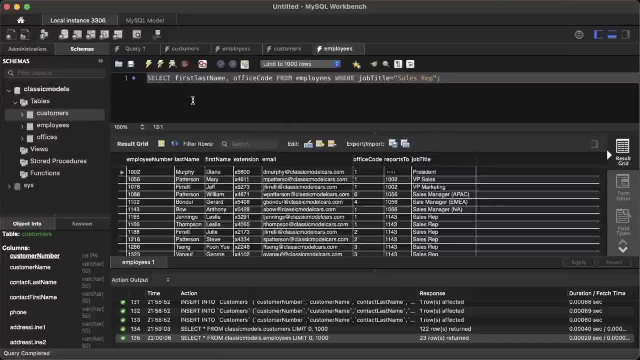 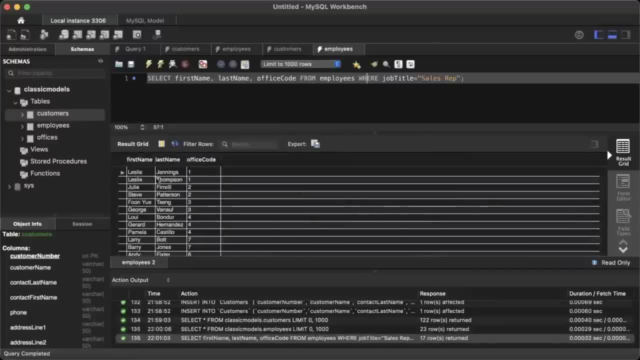 Okay, So last name, first name, last name and office code from employees where job title is sales rep, And now it starts to become more useful. So now we know that at office code one we have Leslie Jennings who is a sales rep. at office code two: 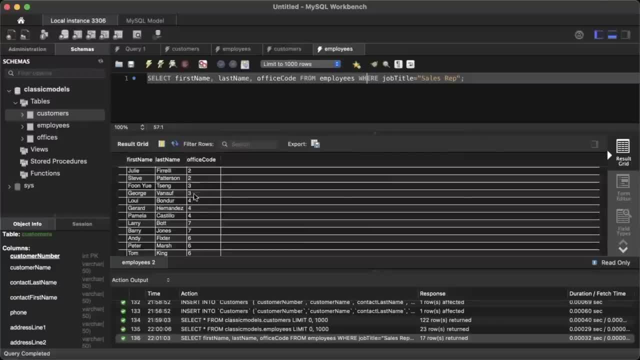 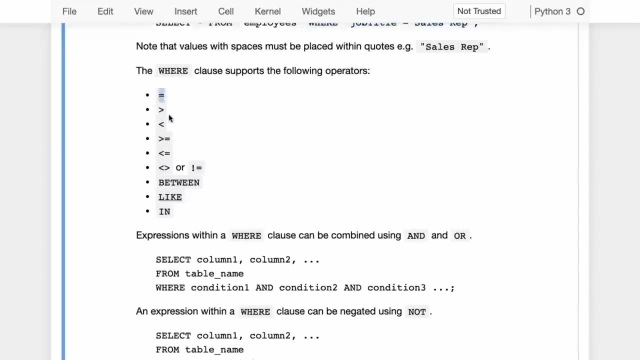 We have Julie Farrell, who's a sales rep. Okay, Okay, Okay. At office code three, we have George one, who was a sales rep, and so on. The where clause supports a bunch of operations where clause supposed to equal to, which is what we have used here. 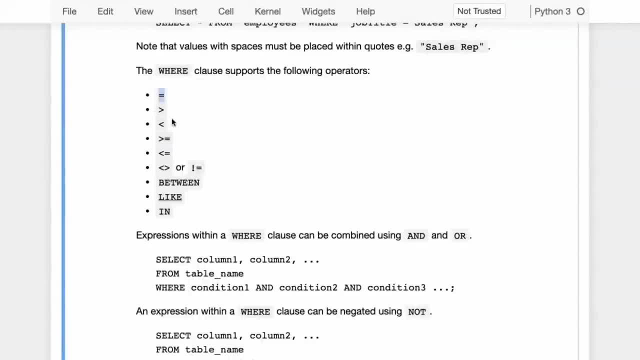 It supports less than and greater than so both of these work with numbers and with strings and with dates, So pretty much all data types with numbers. they expect as expect. they work as expected. Three is greater than two and three is less than five, with strings. 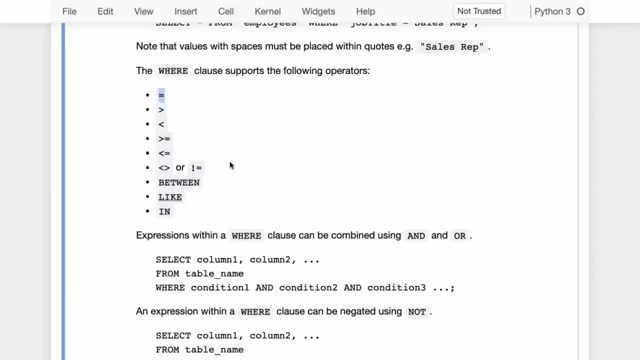 They compare The alphabetical order. So a is less than B, and any string that starts with A is less than any string that starts with B and any. so let's say AA is less than AB. And so you can have this lexicographic or alphabetical order: from A to Z is lower to higher. 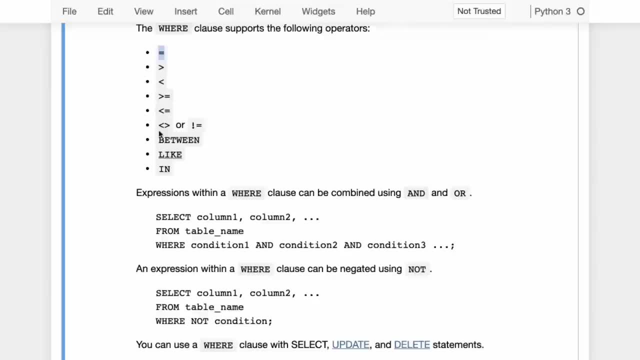 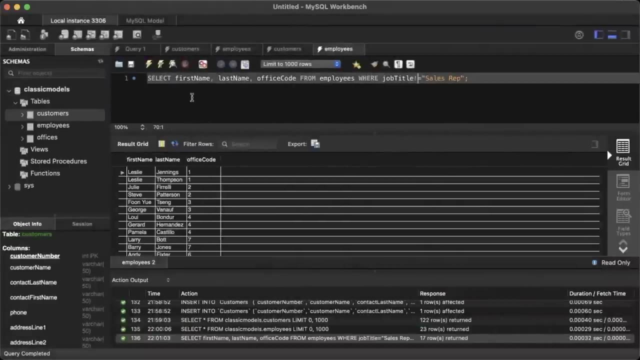 You can also have less than equal to or greater than equal to, and you can have not equal to. now, some variations use this less than greater than. some relational database software use this not equal To. so let's see what my sequel uses. How about we first try not equal to, okay? 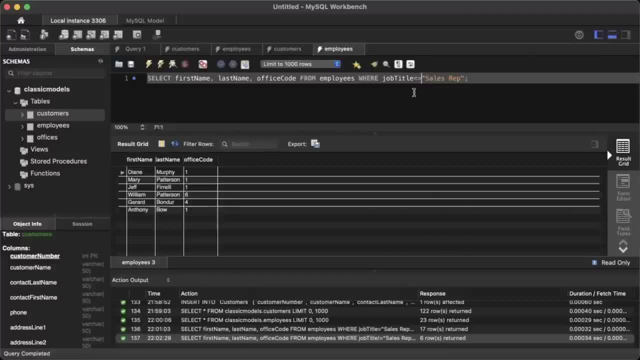 My sequel seems to support this, but you could also have in some places this kind of a statement, So it seems like my sequel supports both. right, If I do start here, we can verify if that is the actually the case. Yeah, 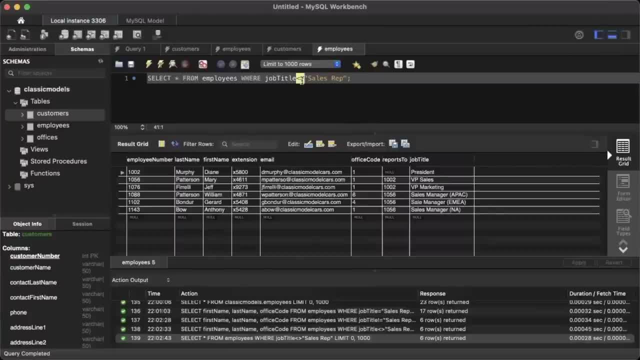 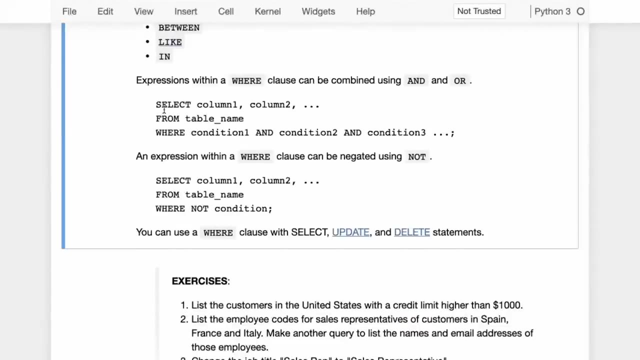 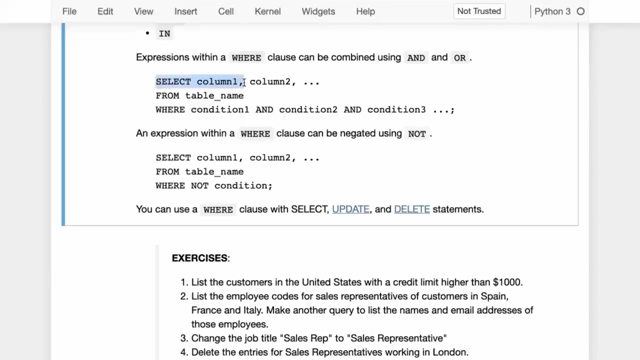 So we are now getting the list of people who are not sales reps by using less than, greater than or. we can also do or not Equal To here, All right, So here's what that looks like. You can also combine expressions in the where clause using and and or so, let's say. you can say things like: select column one, column two, a comma from table name where, condition one and condition two and condition three. 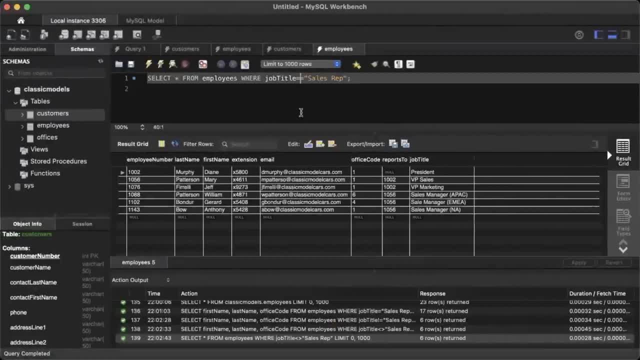 So, for example, if we want to select the sales rep in San Francisco, so what San Francisco, let's First open up offices. and in offices, let's check San Francisco, that's office code one. So if you want to get the sales reps in San Francisco, so we say, select star from employees where job title equals sales rep and or we can put in the additional condition: office code equals one. 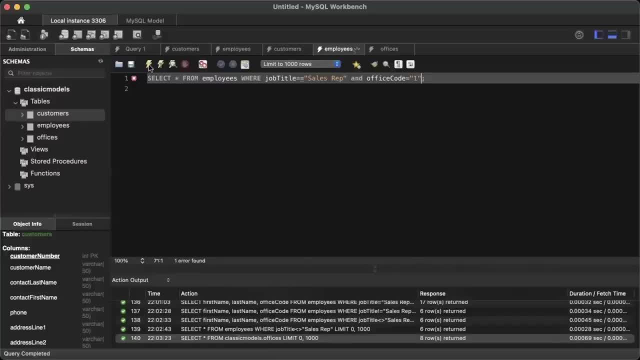 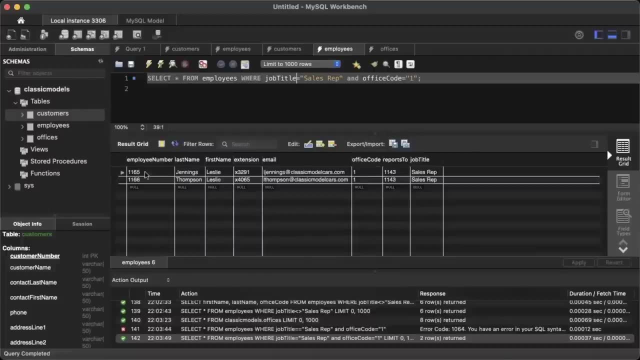 And again, we should put this in courts, ideally. Okay, Just a single equal to Yup. So now you see, here We have the data for Leslie Jennings and Leslie Thompson, their extension and their email, And both of them are in office code one which is San Francisco. 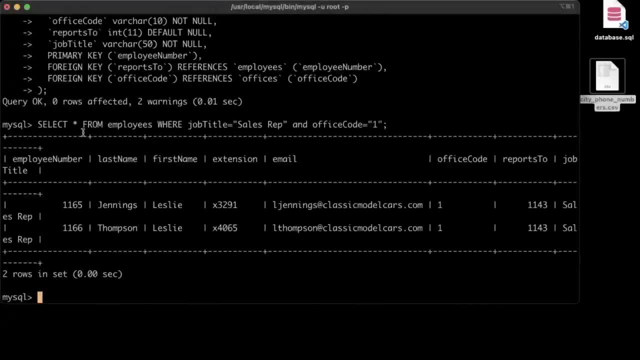 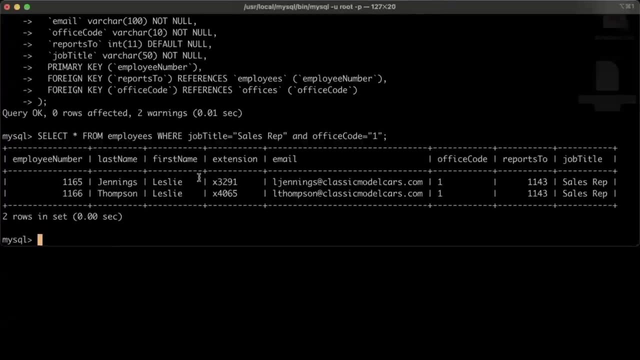 So that's how you filter data out Like I can. I'm just showing, showing you here. it's going to be a little bit bigger here. So that's how you filter data out from a database table. You use the where clause. in where clause you can have one of these conditions. 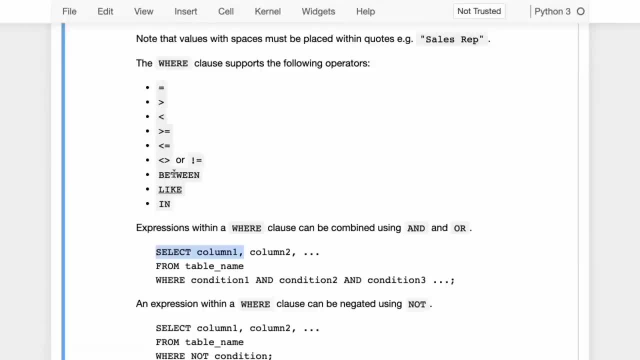 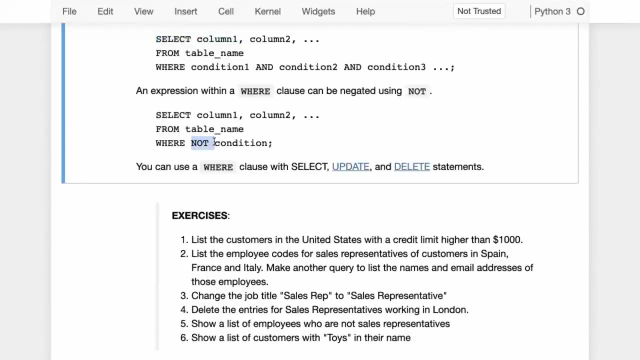 You can also have. you can also do something like this: You can use in Between and like, and then you also have this option to negate things. So you can also negate a condition by saying where, not condition. That's another thing to just keep in mind. 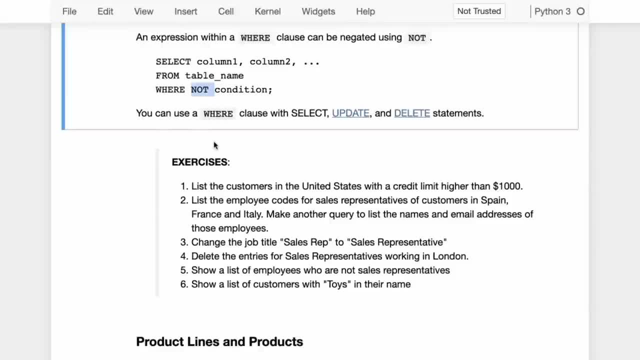 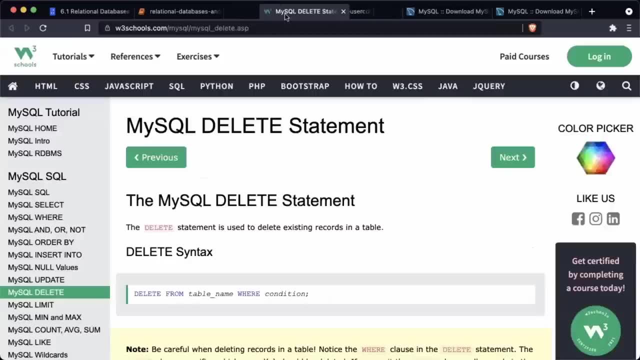 And aware clause can be used with select, but it can also be used with update and delete statements. So we were talking about delete earlier, So maybe let's check out the delete statement once And now. from this point on, mostly you would just have to look up how certain statements work. 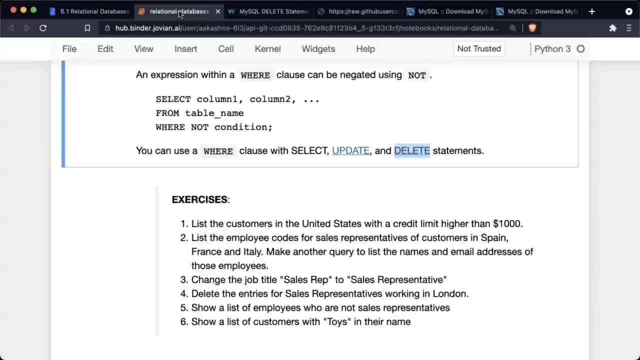 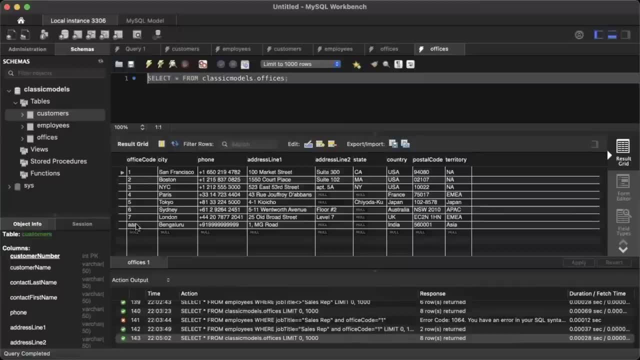 So here we say: delete from table name. Where condition? now, remember, we had this one office that I had inserted, initially called Bengaluru, and this had the office code AAA. Now, if you want, if I want, to delete this office, then here's one thing I can do. 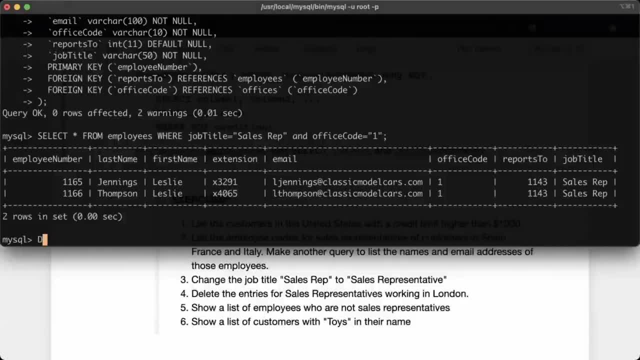 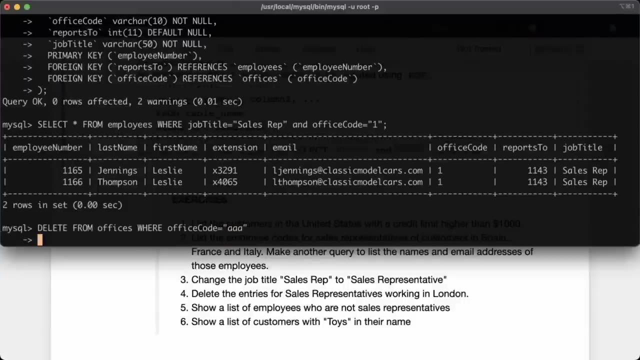 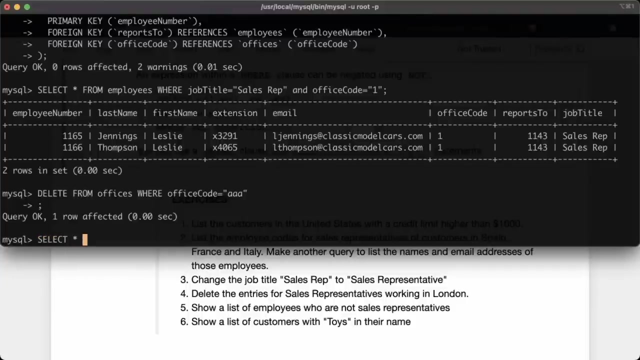 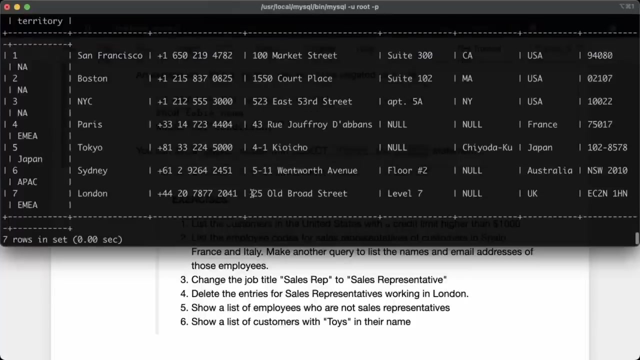 Let me go back here. I say: delete from offices where office code equals AAA. And that should have deleted the Bengaluru office. Let's see. So now you can see that we no longer have the Bengaluru office anymore, because we've just deleted it. 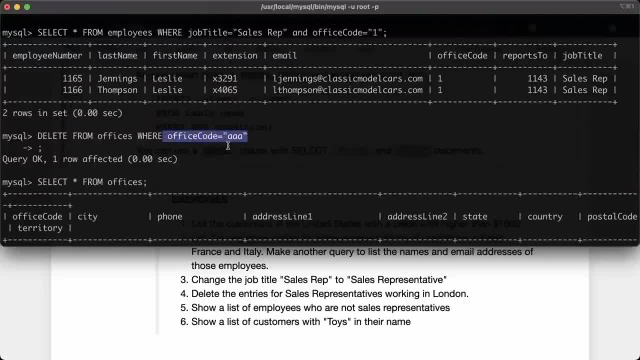 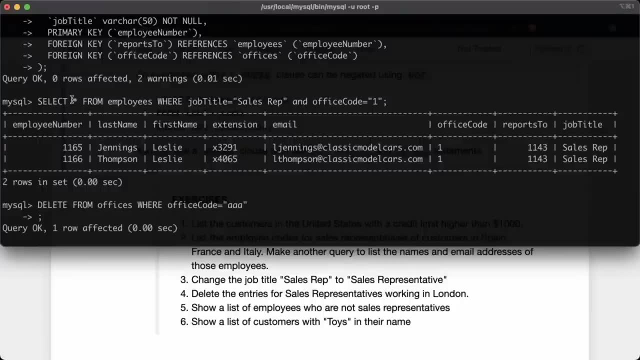 Now here I've deleted exactly one column, but I can delete multiple columns as well. Let's see if I wanted to delete. If I want to fire the sales reps in San Francisco, Okay, So then I would do delete from employees where job title equals sales rep and office code equals one right. 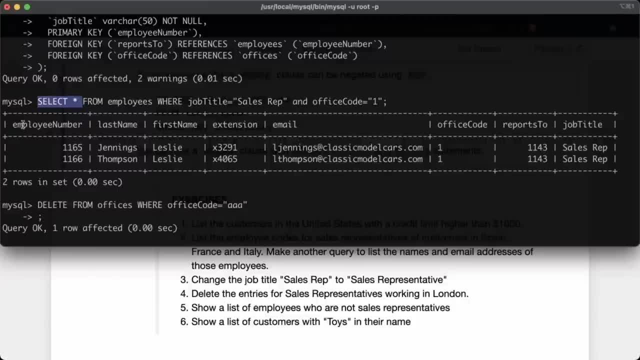 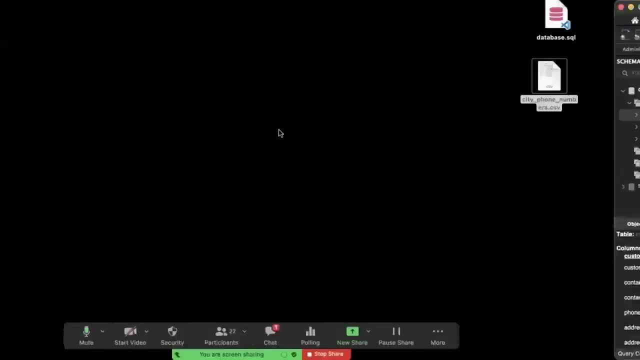 Instead of select star, I would just type delete, And then, instead of just showing this information, it would simply remove these rows of data from the database. So that's that. And let's also check: update: similar just like delete. We have update. 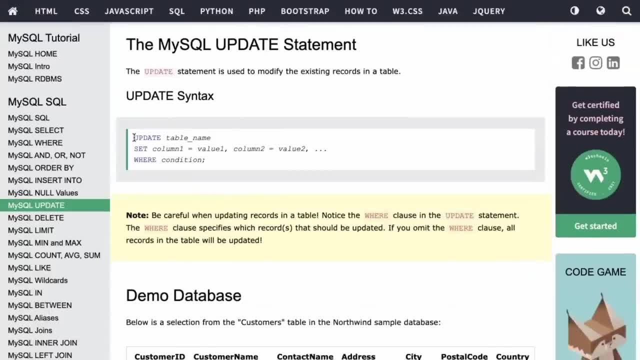 So let's check update to now. here's how update works. You say update table name and then you said the value of column: column one to value One. column two to value two. column three to value three where a condition holds true. 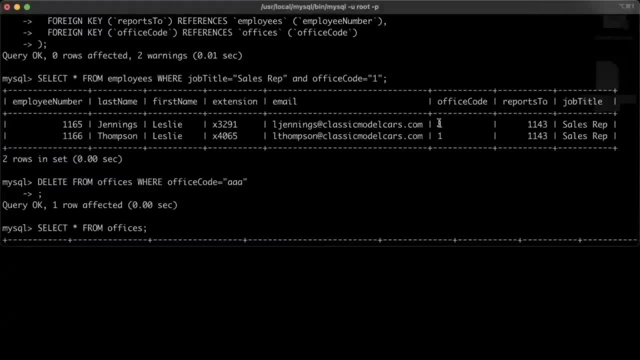 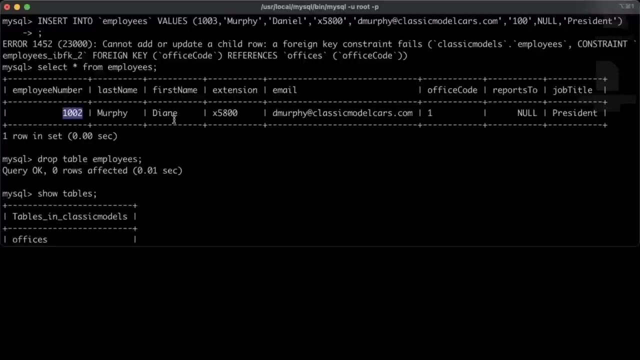 So let's try update. Maybe let us change the reporting person for Jenny, Leslie Jennings and Leslie Thompson. So who are we going to set them to report to? maybe let's set them to report directly to the president. Maybe Diane Murphy directly wants to talk to the sales people in San Francisco. 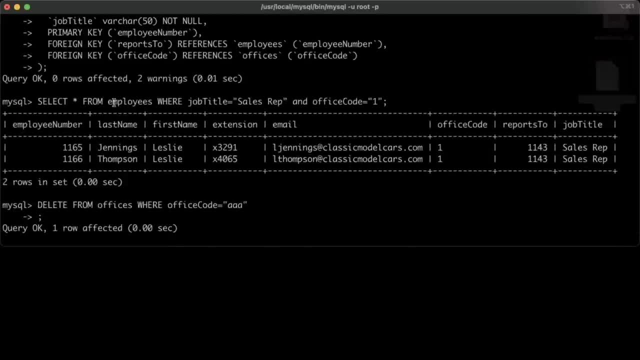 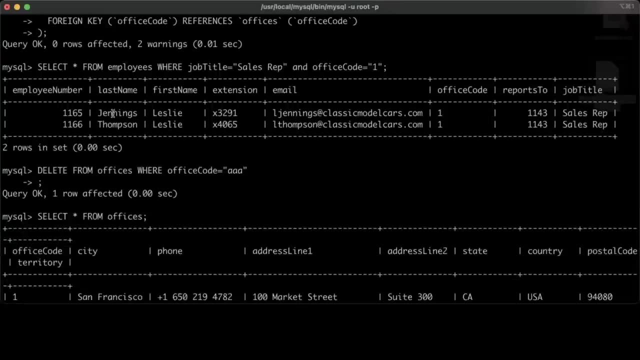 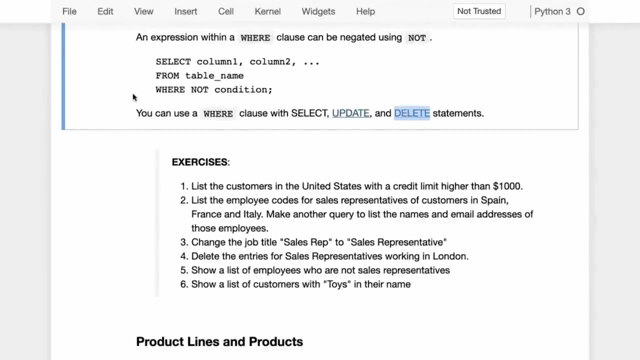 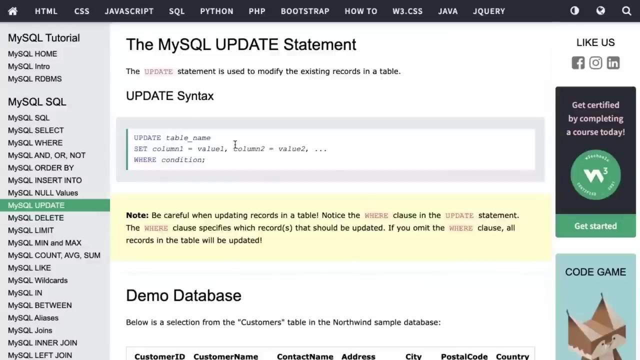 So we want to get these employees where job title sales rep and the office code is one And we want to update their values. So let's see, we say update. What does that code look like? Update set. column one equals value one. column two equals value two. 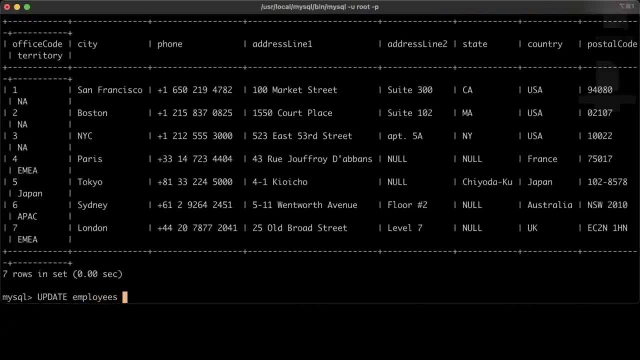 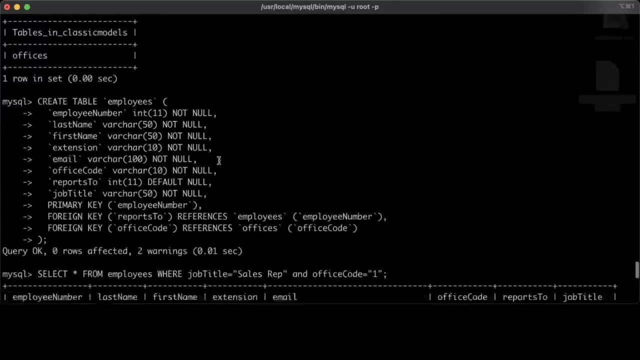 Okay, So we want to set update employees And we want to set their reports to two, one zero zero two. And again we should put in quotes here: update employees set reports two to one zero zero two. And then we want to have the where and in the where clauses where we want to add the selection, where we are only 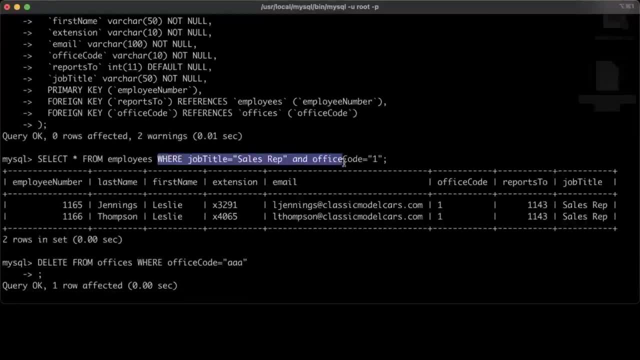 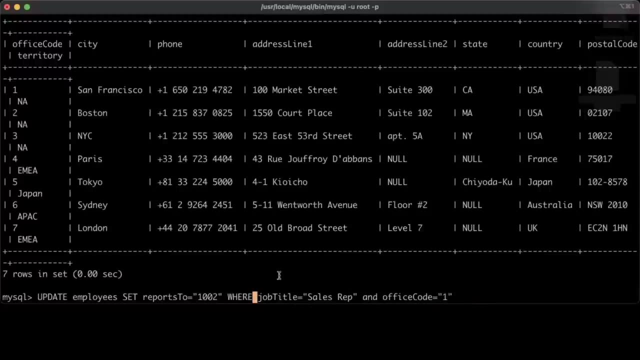 selecting the sales reps from San Francisco. So where job title equals sales rep and office code equals one. Okay, All right. So the good thing about SQL is that it's very readable. So update the employees table and set reports two to one. zero zero two, where job title is sales rep and office code is one. 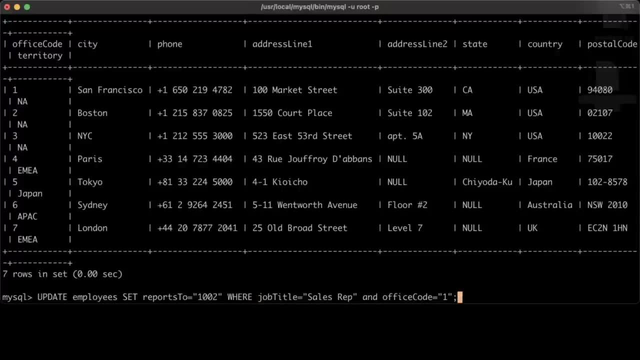 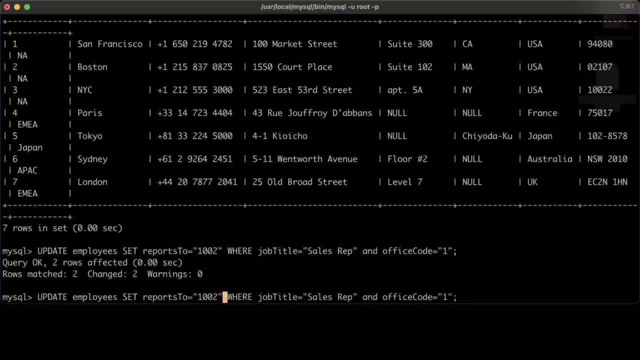 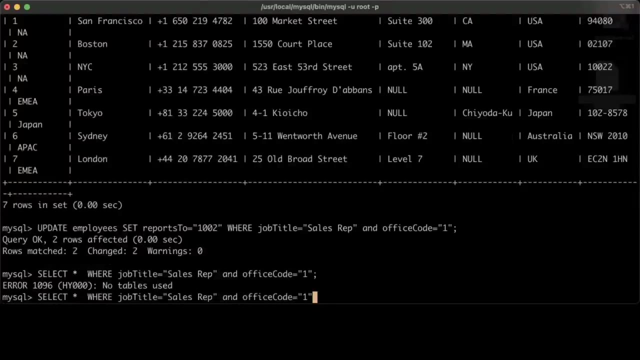 So only for people in the San Francisco office who are sales reps, you want to update their employee. We want to update their reports too, and let's just do a select star and let's make sure that that was updated. So select star from employees. 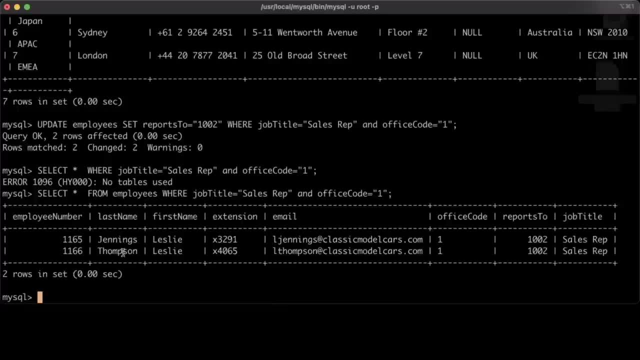 Yeah, So now you can see, with Leslie Jennings and Leslie Thompson, they now report to one zero zero two. Okay, If we remove this, we can also see that no other rows were affected. You can see that there are very few other people who actually report to one zero zero two. 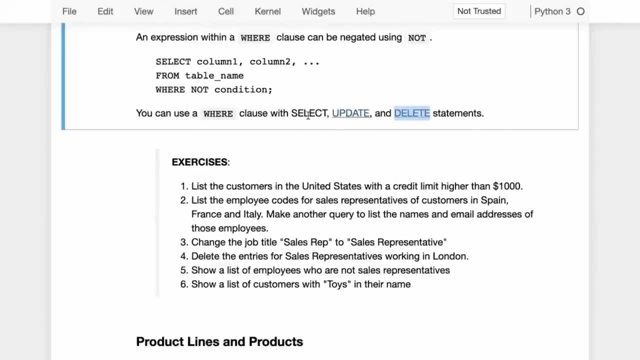 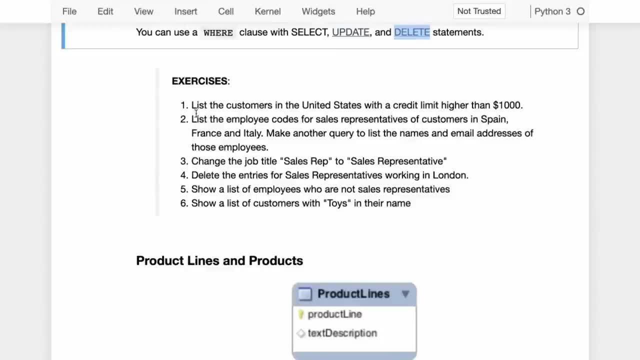 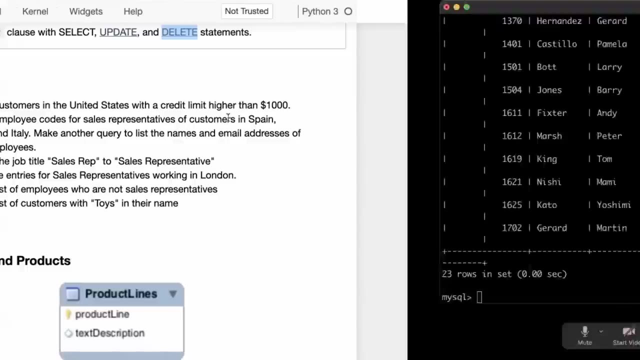 All right, So that is the select clause, The where clause, though Update command and the delete command. So here are some exercises for you. Try and list customers in the United States with a credit limit higher than a thousand dollars. So you'd probably start out something like this: 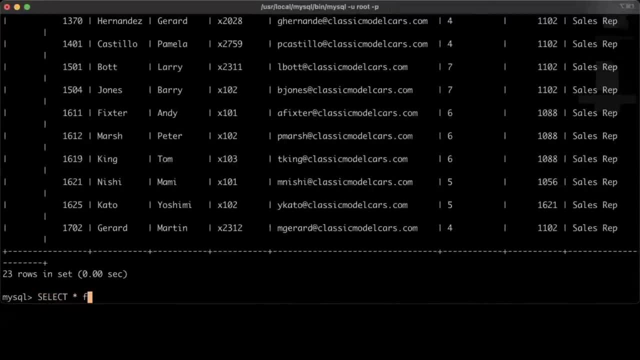 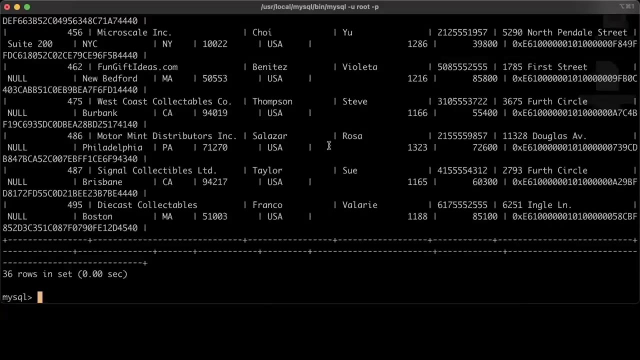 You would say select star from customers where country Equals. I think it's USA and you can check this out. So these are all the customers in in the USA- Quite a few of them. but we want customers with a credit limit higher than a thousand dollars. 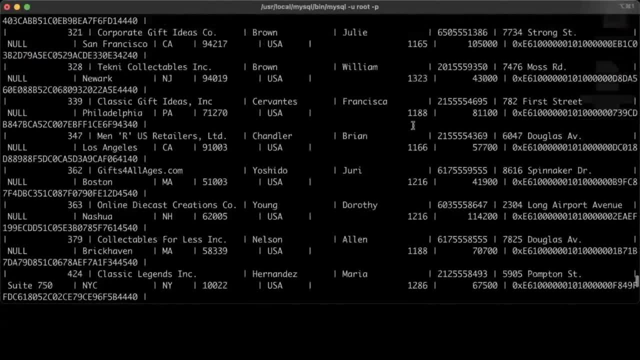 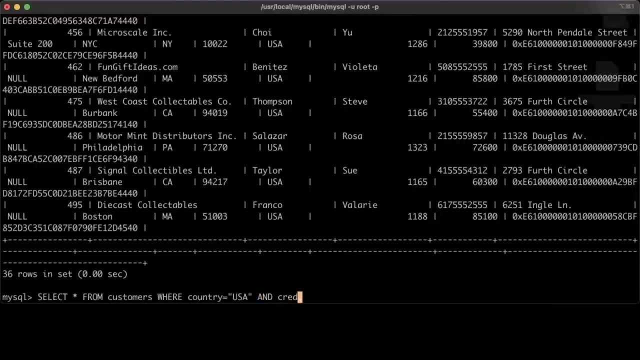 Maybe we probably want even an even higher credit limit. but let's see, let's try a credit limit higher than thousand dollars. So here you would say: country equals USA, and then you would say: and credit limit greater than a thousand. Okay, 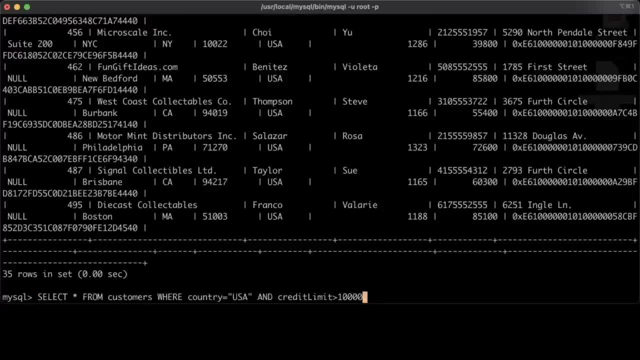 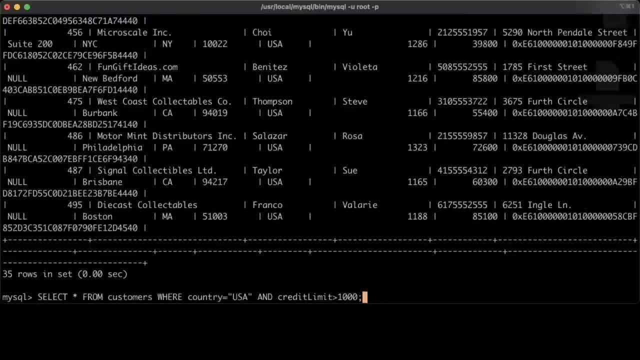 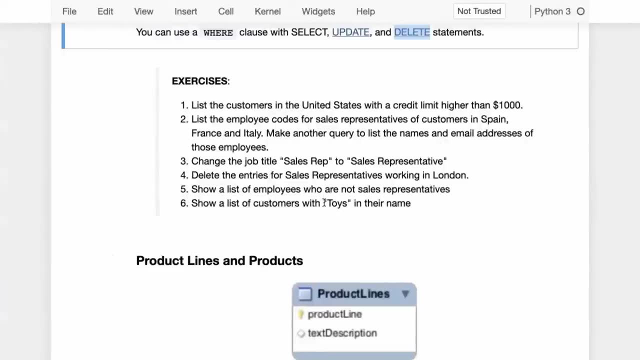 Yeah, So there are nine rows with more than a hundred thousand, but with a thousand there are 35 rows. So you can see that changing the credit limit is going to change the number of results. All right, Then here's one more list. 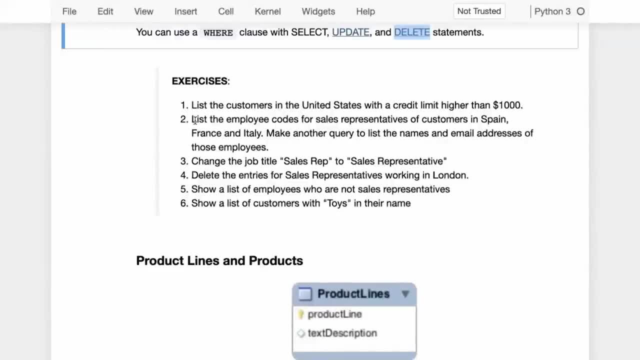 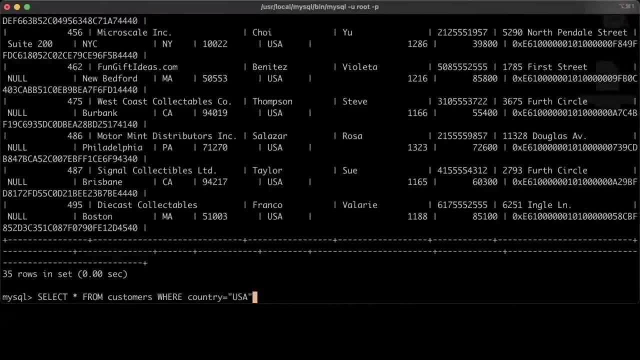 The employee courts for the sales representatives of customers in Spain, France and Italy. Okay, How would you do that? Well then, uh, you would say: select sales first, let's describe customers. So let's say describe customers, So we have the sales rep employee number. 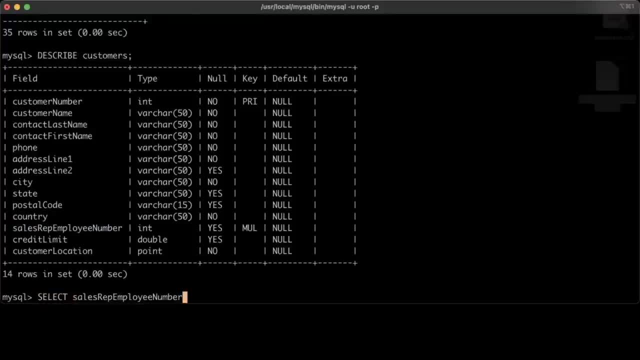 So now we would say: select sales rep employee number from customers and then we can put in a where, and now we want the Location of the customer or the country, and we can put in an in, and then I think we can give it a, give it a list of values. 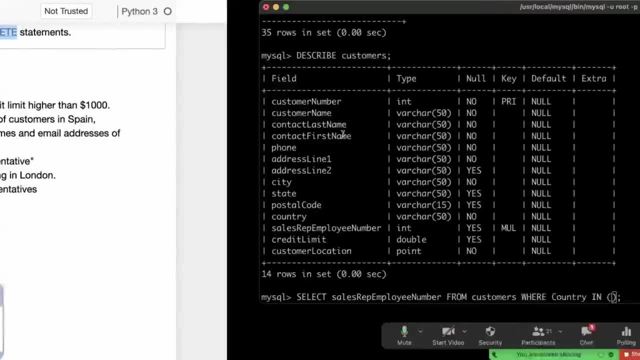 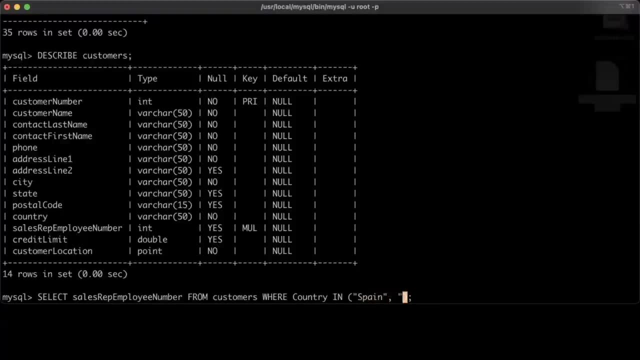 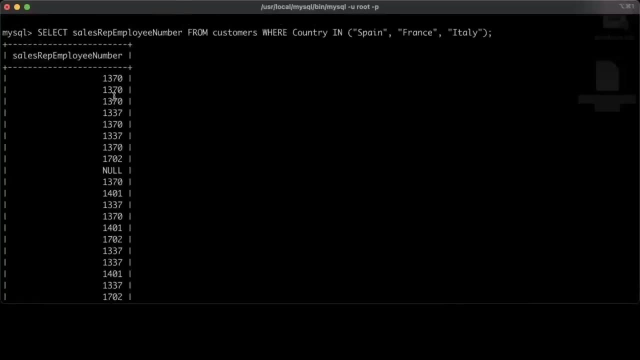 So we are concerned with? we are concerned with Spain, France and Italy, So we can now put in Spain- I think we have to use double quotes here- So Spain, France, Italy. Okay, So here is the list of all the sales reps who work with customers in Spain, France and Italy. 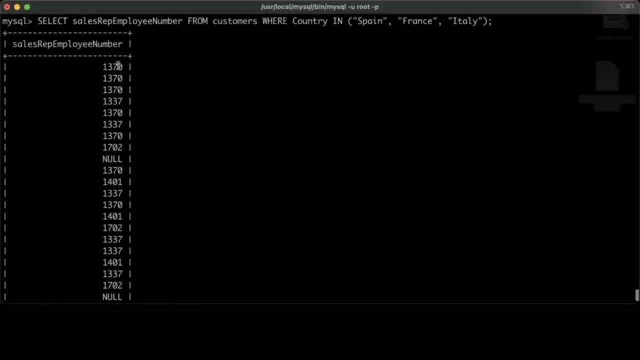 Okay, Now I can probably just put a, put, put together a list of these. So there's 1, 3, 7 0, 1, 3, 1, 3, 3, 7, uh, 1 7, 0, 2, 1, 4, 0, 1 and 1, 4.. 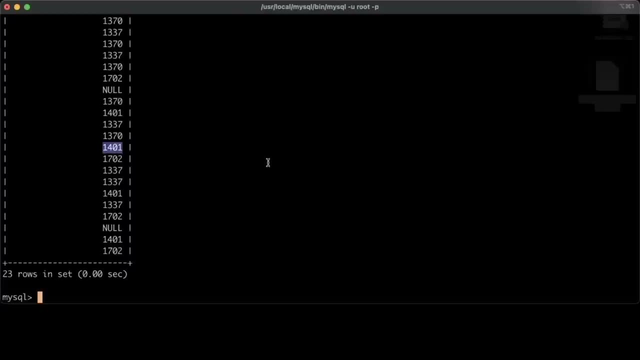 Yeah, that seems to be all. So there are only about four or five such sales reps. And then the question is: make another query to list the names and email addresses of those employees. So now we can do select, Let's say first name. 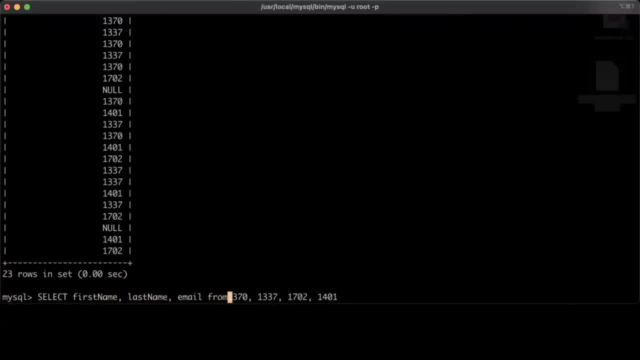 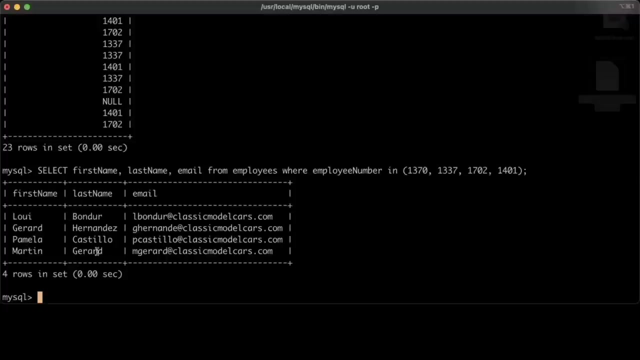 Last name email from employees where employee number in, and then give it this list. Okay, So now we have Louie Bondo, Gerard Hernandez, Pamela Castillo and Martin Gerard. So these are all the people who are selling to customers in Italy, Spain. 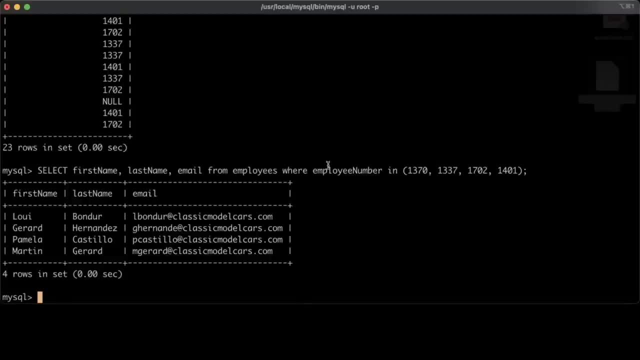 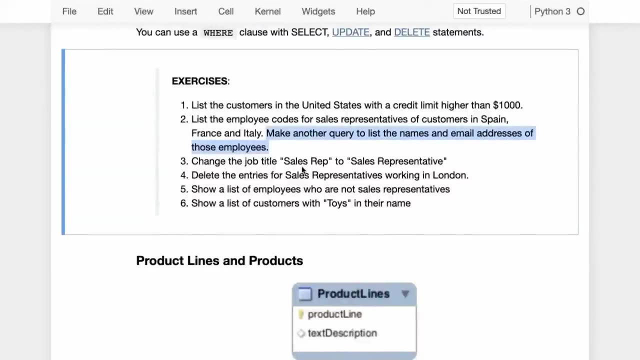 So this is the kind of Q and a that you can do using SQL queries. Here's one more: change the job title sales rep to sales representative. I let you work on this, or you can use update to do this. delete entries for the sales representatives working in London. 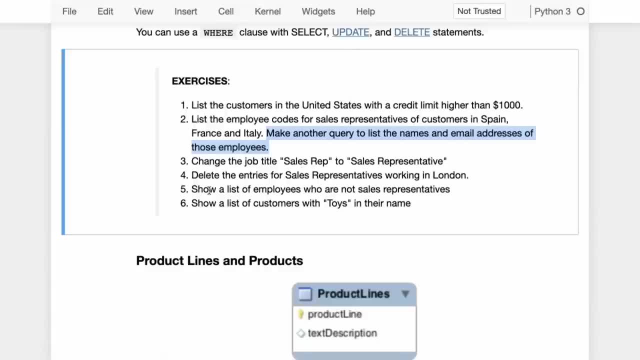 So first you find out the sales rep, first you find out the code for the London office. How do you do that? Well, you can use a select statement to get the data for London. Then you use that code, that office code, to get the data for London, and then you use that code to get the data for the London office. 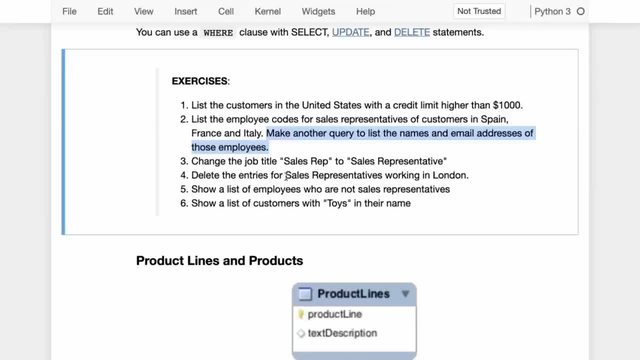 So this is the kind of Q and a that you can do using SQL queries, That office code, to delete the entries for those sales representatives. So you'll have a where clause with delete. Then you have show a list of employees who are not sales representatives. 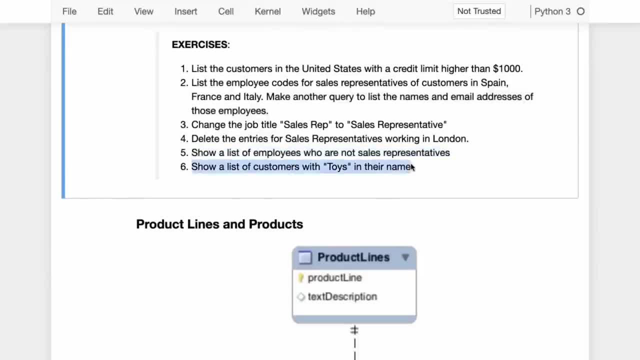 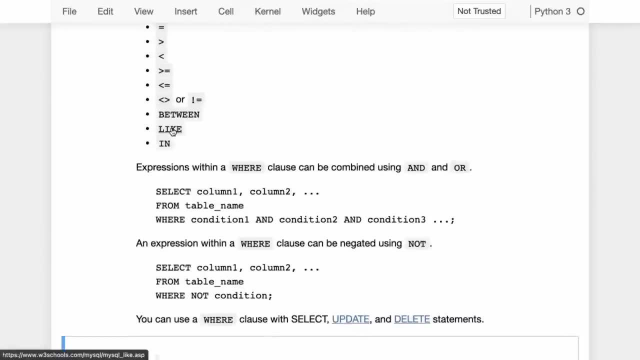 I think we've already done that. And here's one interesting one: show a list of customers with toys in their name. So this is where you would have to use the like statement. So if I just click through here, you can see this is how the like statement works. 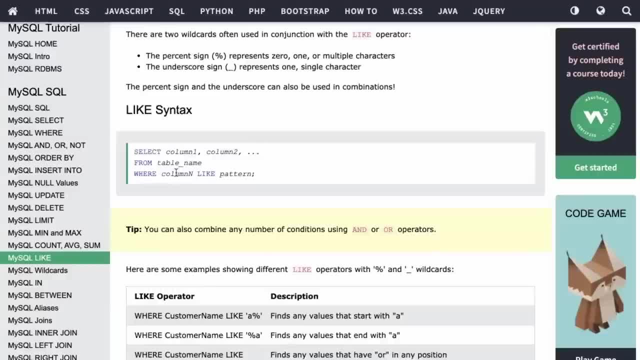 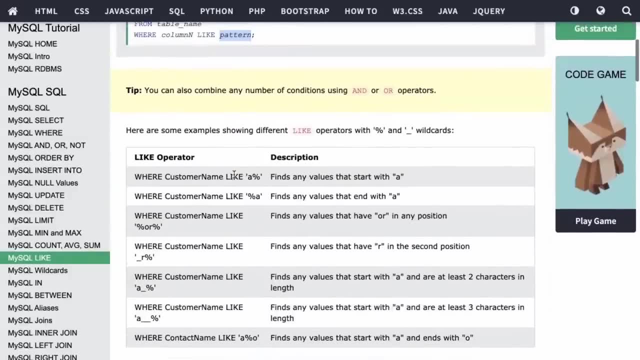 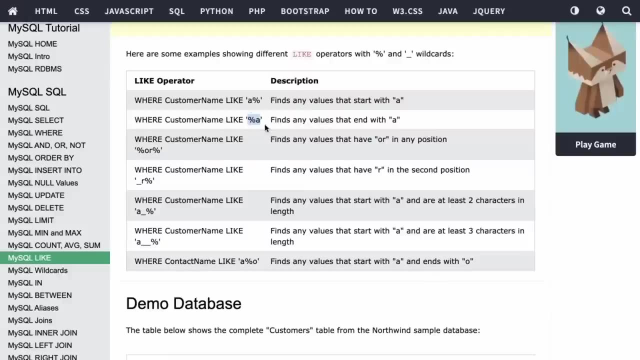 So you can say: select columns from table Where a certain column is like a certain pattern and the pattern can be a string or the pattern can be something like this: You can have a percentage or percentage. So whenever you have a percentage, that means zero or more characters. 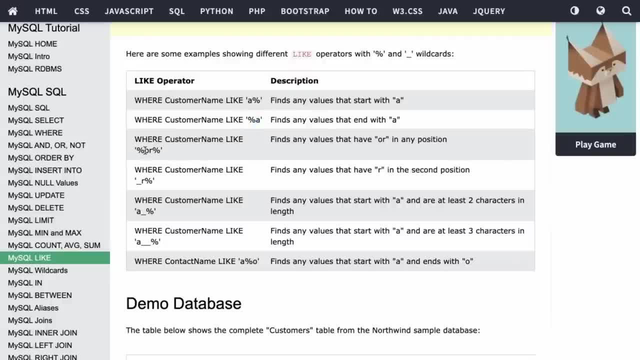 So if you want to just check for a somewhere in between, like if you just want to check for or somewhere in between, then you have percentage or percentage. So percentage represents zero or more characters, and then underscore represents exactly one character. Okay, 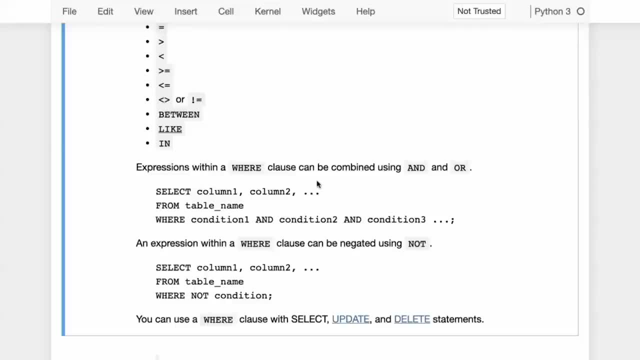 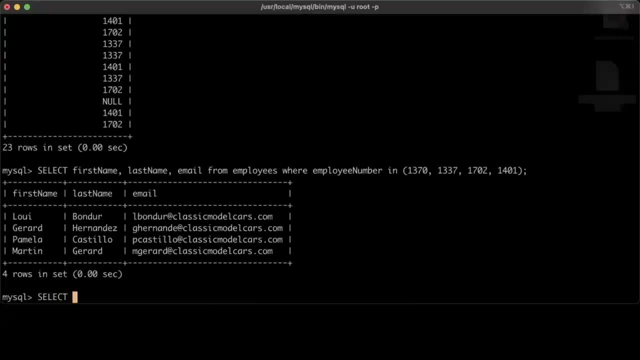 So check out this reference on how exactly it works. What I'm going to do is I'm going to just try and solve this answer. Show a list of customers with toys in their name. So let me see select star from. or maybe just select the customer name and the country from. 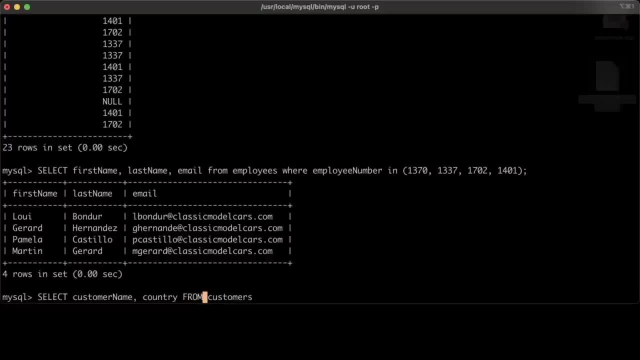 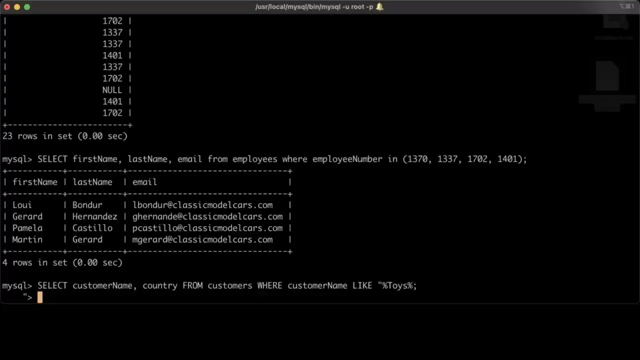 Okay, Customers, where customer name like: and here is where we can put in percentage, And then we want toys and percentage and let's run that. Oops, I think I had to close it, So let me just undo that percentage toys. 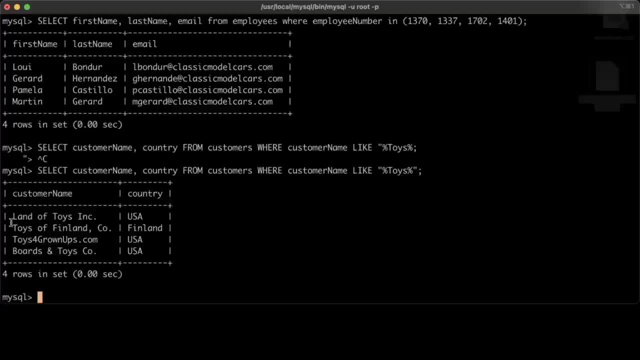 Percentage and let's run that Okay. So it seems like you have land of toys incorporated in the USA. You have toys of Finland in Finland and you have toys for grownups in USA and boards and toys in USA. So it's a very basic selection. 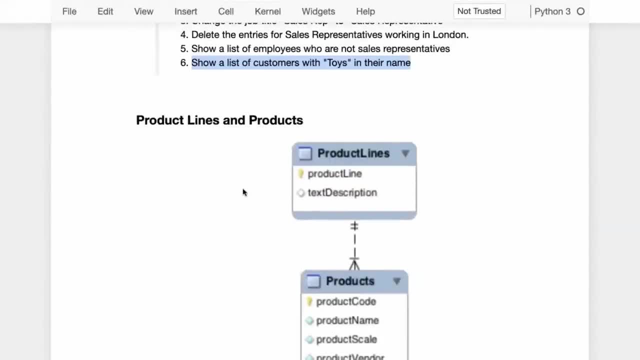 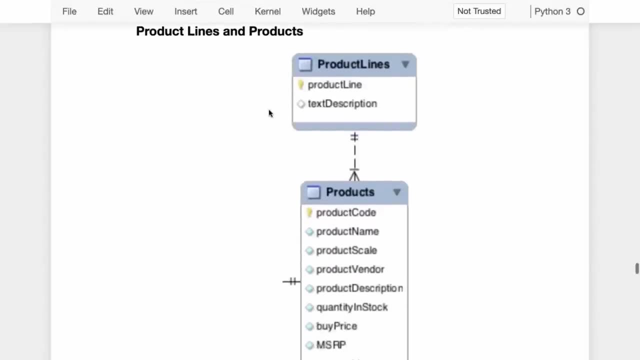 You can't do a lot of advanced rejects kind of selection, but a very basic selection can be done. A very basic search can be done using like okay, Then you have product lines and products. So you have a bunch of product lines like motorcycles or flights. 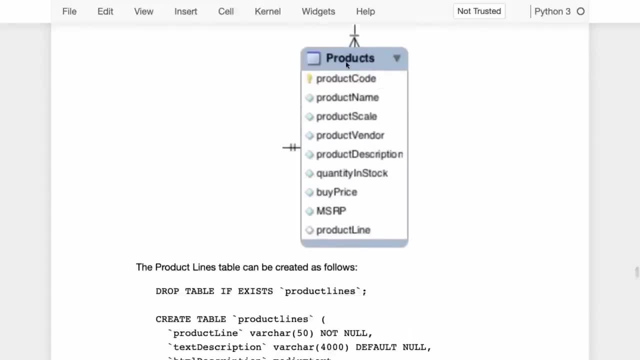 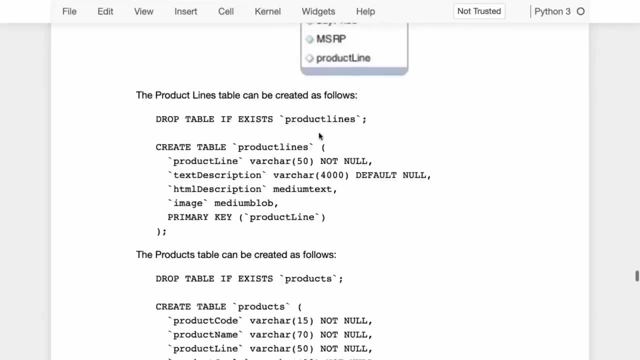 Oh, planes, cars, et cetera. And then you also have products, So you may have different models of motorcycles, different makes, for which you offer small scale models. So here is what they look like. Product line is a very simple table. 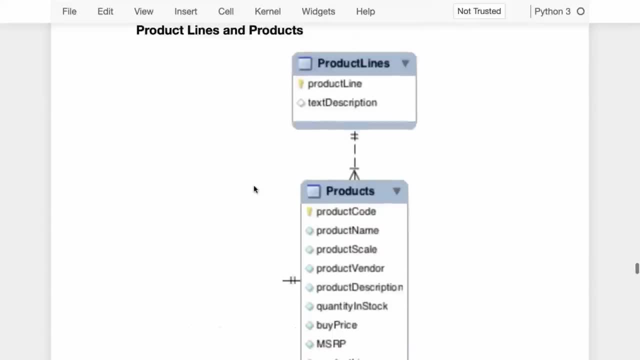 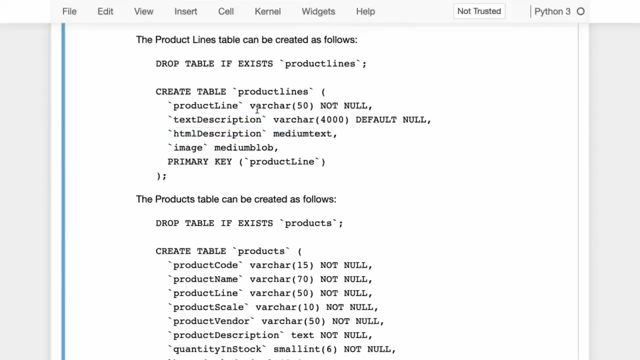 It contains a product line. It contains some description, So it seems like it contains a text description here. for some reason, There's also an HTML description. Maybe this is going to be used on the website and there's also an image. Yeah, 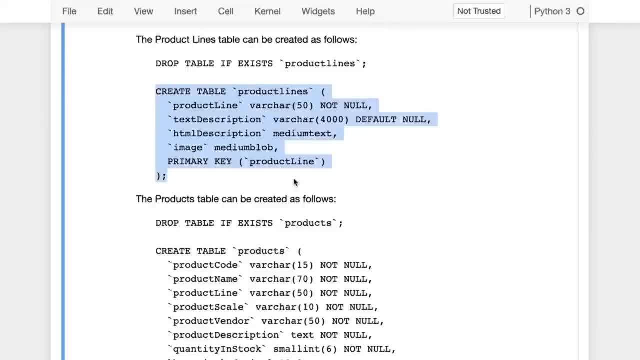 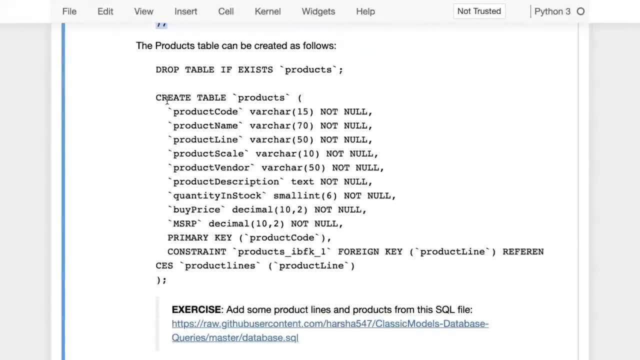 So let's just take create that Product lines table Once again, I'm just going to paste it here and that will create the product line stable. And similarly, we have a product stable as well, which has a product code, product name. 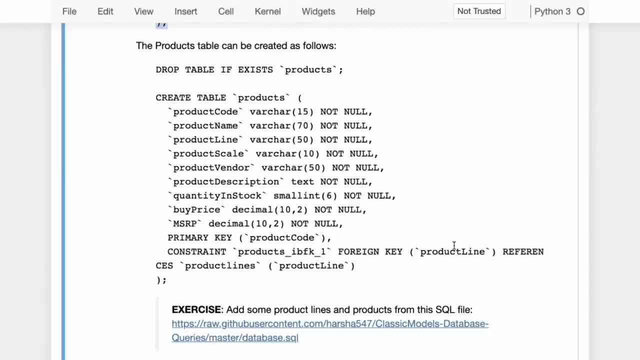 Product code is the primary key. It has a product line, which is a foreign key, and it has a product vendor description. It has a quantity in stock, So that's a small integer. Then it has a buy price, So which is the price at which we are buying. 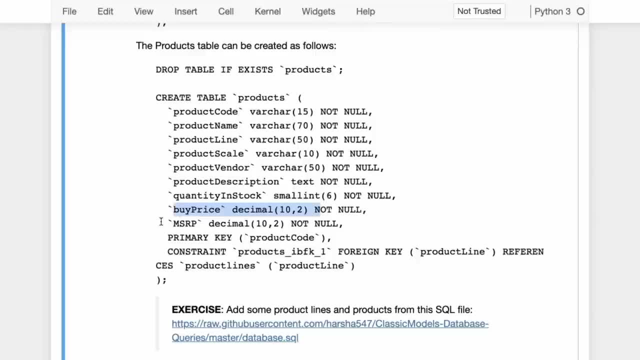 Let's say the Raw materials for the product or sort of the manufacturing price. Then we have the retail price, So this is the price at which we are selling the product, So that can be used to just determine the profit on the product. 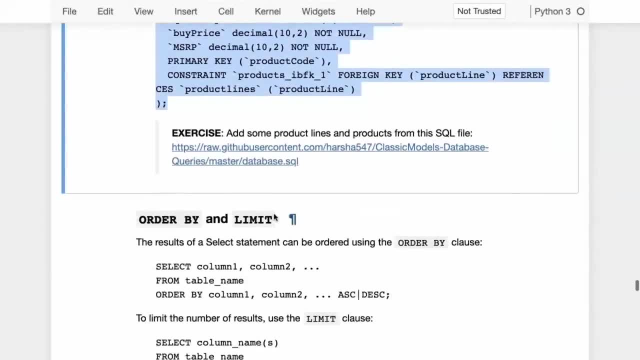 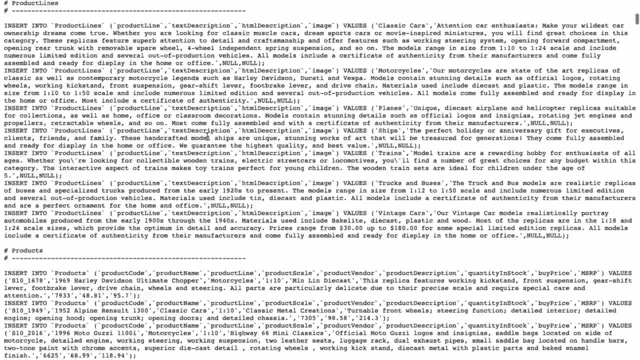 So here's our product, right? And then, once again, you can use this link to download some products. So here we have the SQL file, and then from the SQL file let's see, let's find some product lines and some products. 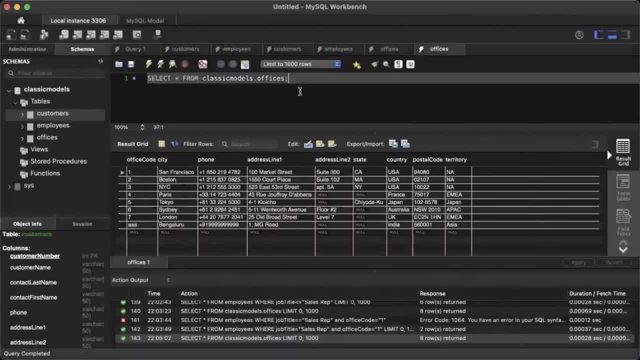 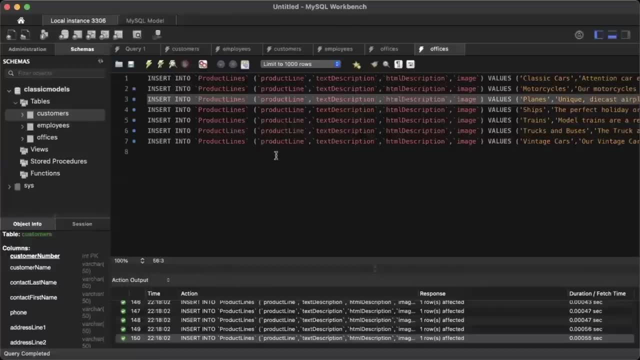 So let me get all these product lines. I'm going to come back Here and I'm going to just put all these product lines in and I'm going to just run this. So we have put in all the product lines: classic cars, motorcycles, planes, ships. 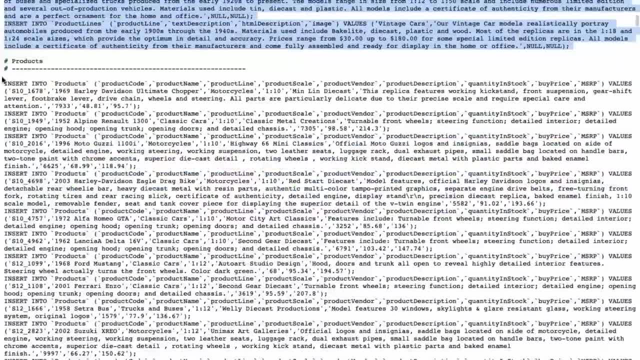 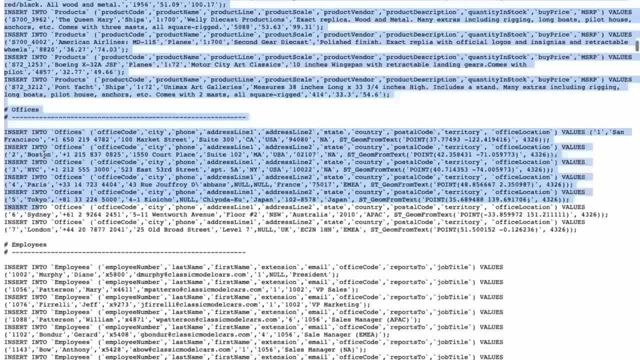 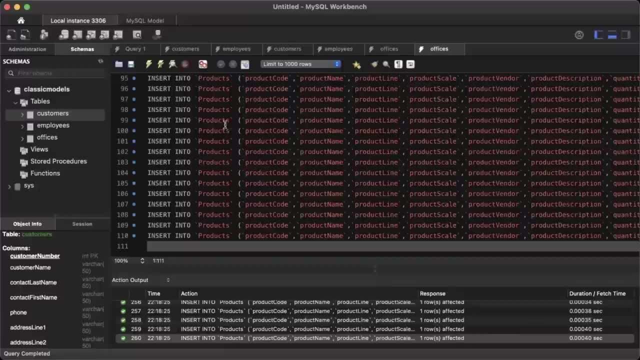 trains, truck, vintage cars, and let's also put in a bunch of products. Let's get all of these products from this page. Okay, Quite a few products and let's put it in there. There you go. So now we should have a bunch of products and a bunch of product lines as well. 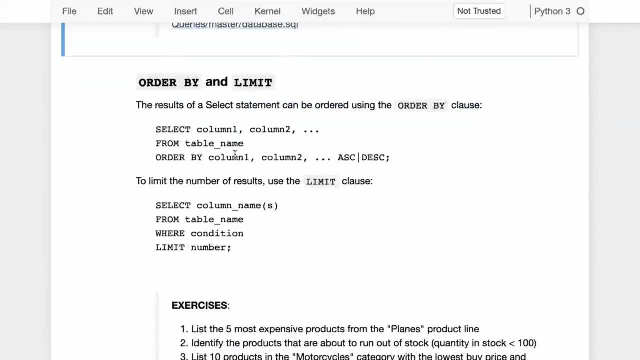 Okay, Now, once you have such huge tables and such huge, such a large number of products and product lines and such, you may want to do some sort of ordering and you may want to also limit the number of results. You may not want to look at thousands of results all the time, or even hundreds. 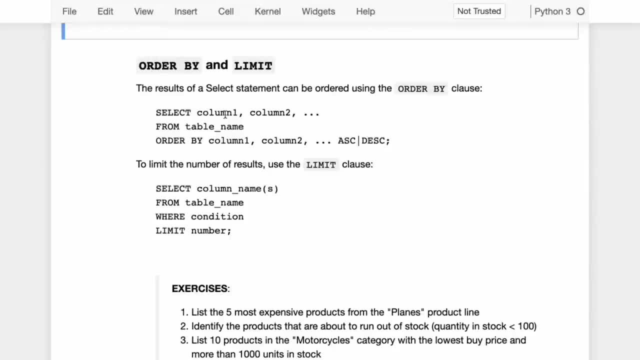 You may just want to look at the top five or top 10.. So if you want to order data, then you just include order by at the end of a select statement And you just Mention which columns you want to order by. So column one, column two, 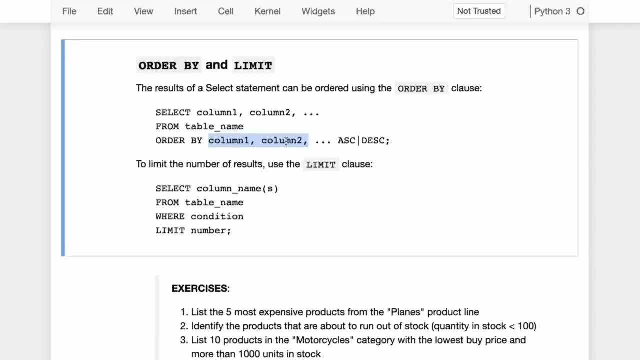 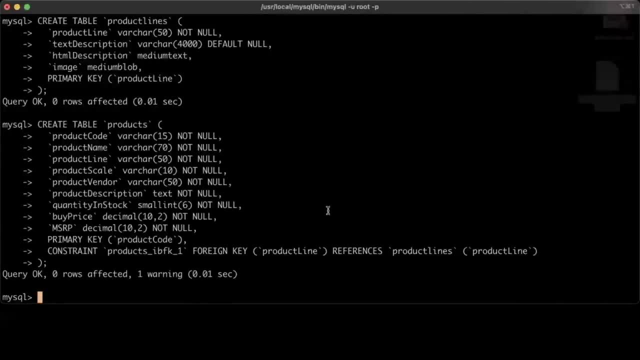 So first it will try to order by column one. If the values in column one are equal, then it will try to order by column two and so on, And then you have the ascending and descending. For example, if you want to list customers by country, you would say select, let's say customer name, comma, country from customers. 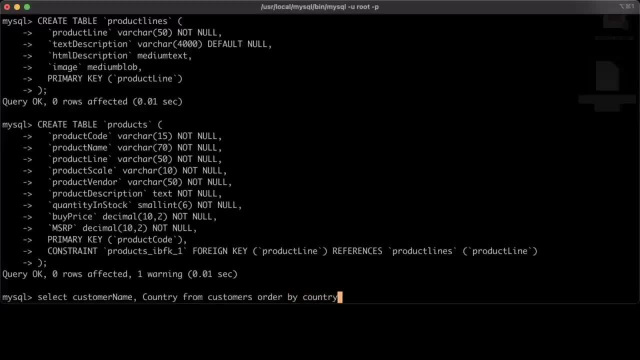 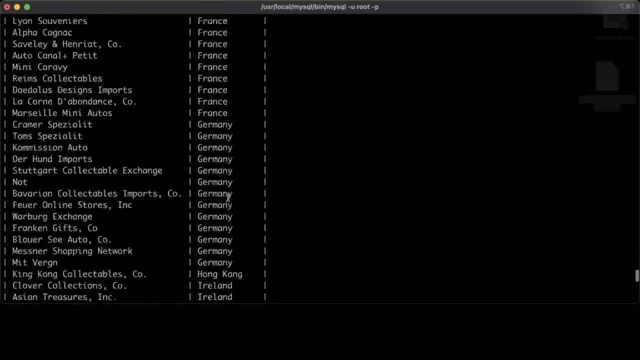 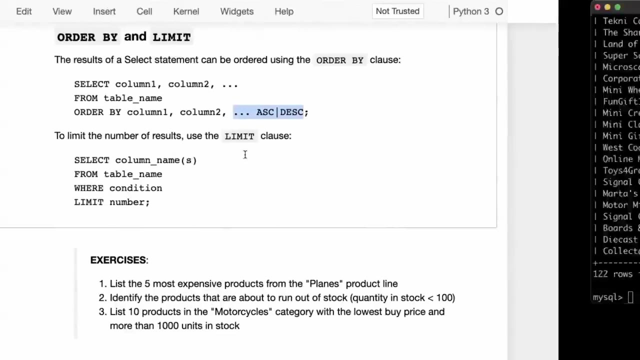 Order by Country. and now you can see that you have customers ordered by country: Australia, Austria, Belgium, Canada, et cetera. you can also then use a limit clause If you just want to then see maybe just one page of data, something that you can display at once. 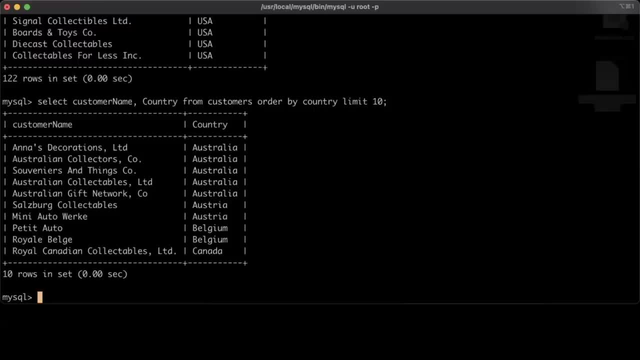 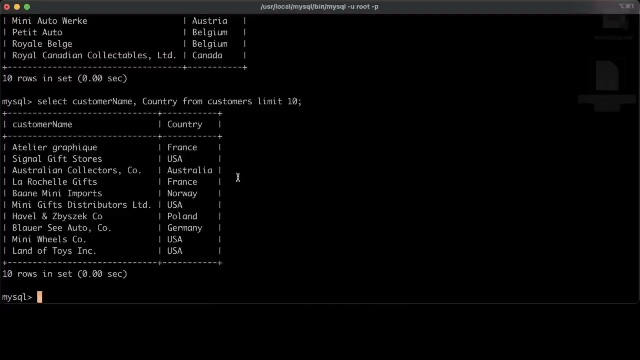 So you can also type your limit then, and now you just see 10, and of course you don't have to use order by with limit. You can use a limit without order by as well. So if I just do, limit 10,. so this is now the natural order or the order in which the data was inserted. 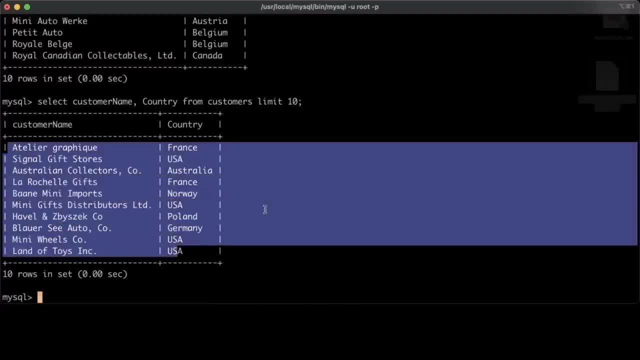 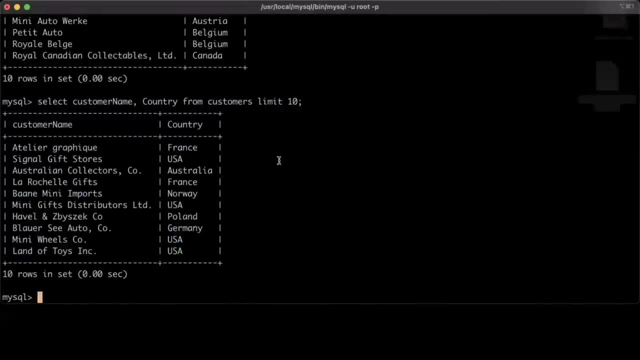 That is the most. that is the default order that is used. So this is how you combine order by limit And you then you can also combine it by where clause. maybe you can also only check for customers which have a credit limit greater than a thousand dollars. 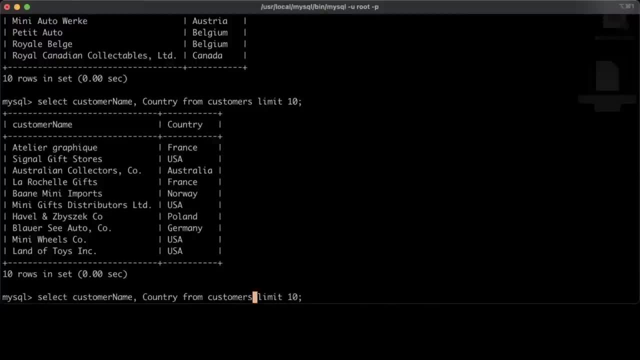 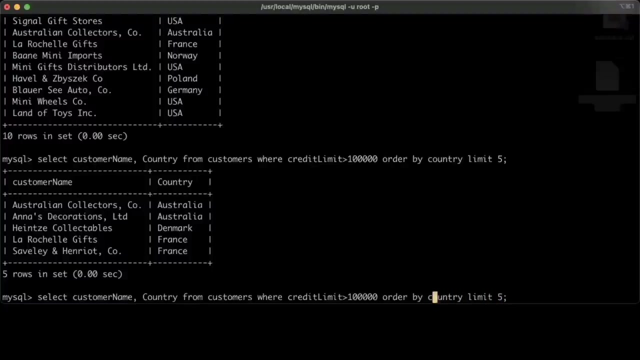 So let's say, select customer name, country from customers where credit limit Greater than a hundred thousand and, ordered by country, limit five right. So maybe also get the credit limit here. So that's how you combine all of these. here We are combining select. 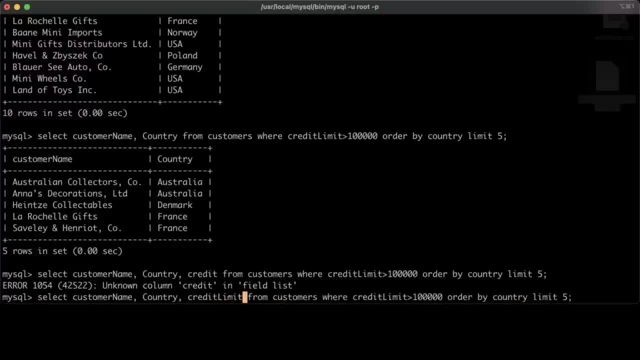 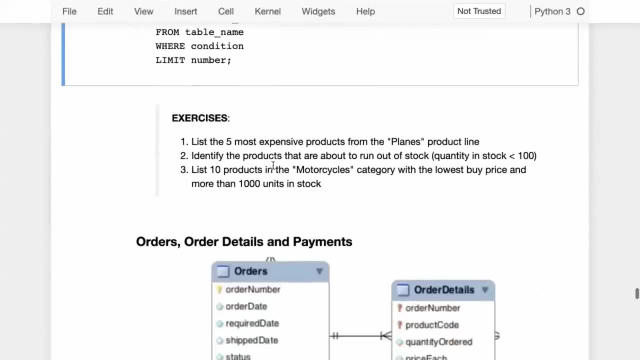 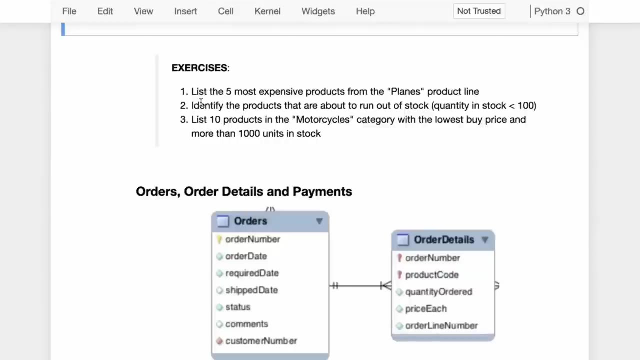 We are combining where we are combining, ordered by and limit, And this is What that looks like. Okay, So here are some exercises for you: identify the five most expensive products from the planes product line. identify the products that are about to run out of stock. 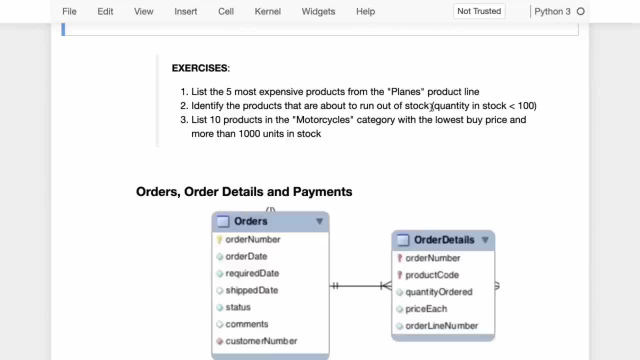 So products which have a quantity in stock less than a hundred, and list 10 products in the motorcycles category with the lowest by price and with more than a thousand units in stock. Okay, So there are a lot of things you'll probably have to. 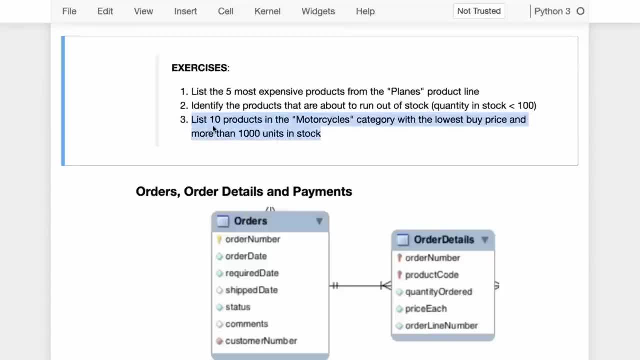 Put, Put together everything that we have covered so far, ordered by and not order by. but you will have to put together a limit, You'll have to put together an order by as well, because the lowest by price, and you have to put together a couple of conditions, which is the category, product line. 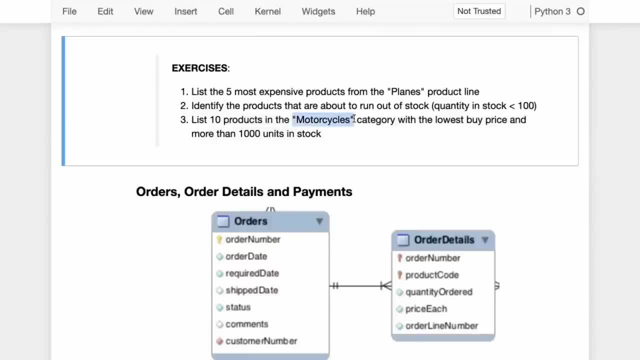 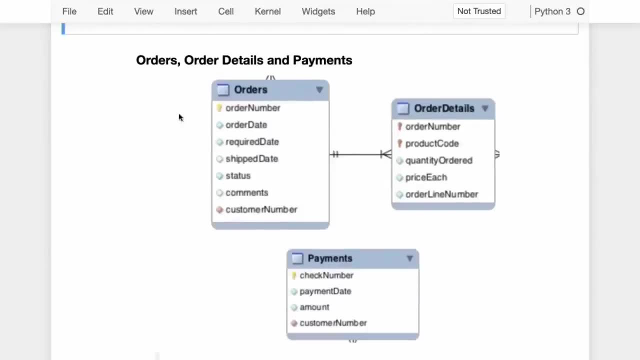 And for the product line. you will have to figure out what the product line code for motorcycles is, And you will also have to add a check on the units in stock. Okay, Then you have these orders, order details and payments, The tables. 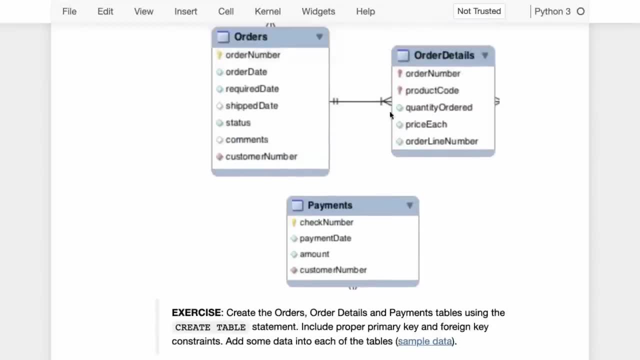 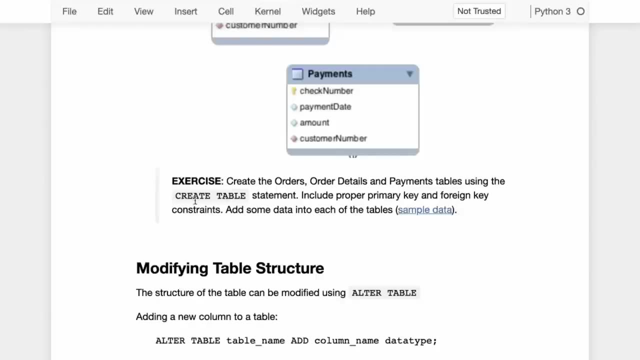 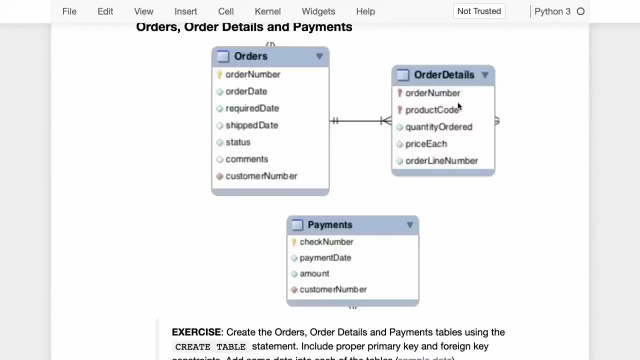 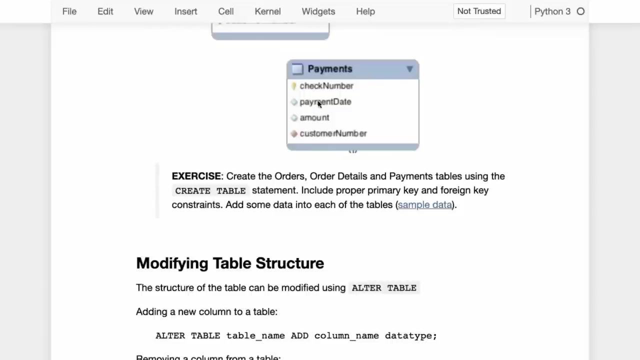 So I let you build these as an exercise. You have the code, you have all the information here so you can create the order, order details and payments tables using the create table statement and include proper primary key and foreign key constraints. For example, order has a customer number or the details has a order number and a product code, and then payments also has a customer number and the check number is a primary key. 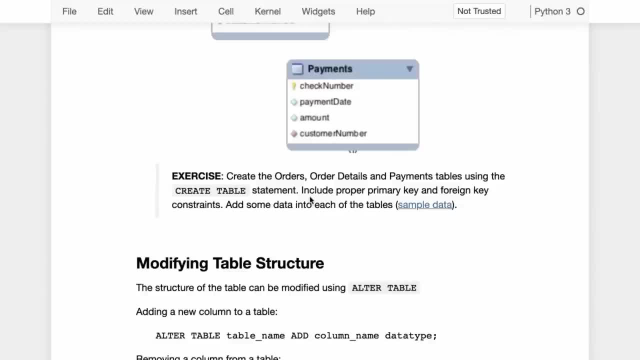 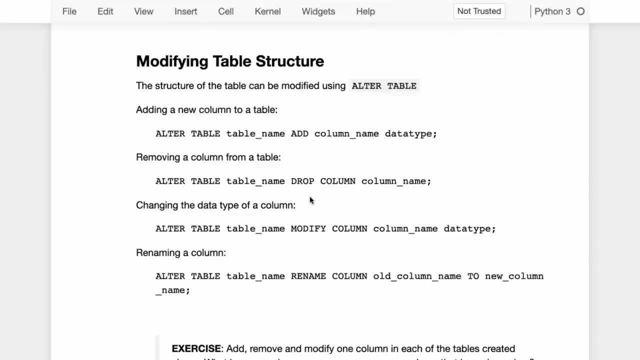 And then you can use the same sample data that we've been Using so far to populate this too, Okay, Next, I just want to briefly touch on how you can modify the structure of a table- Not something that we will do right now, but if you want to add a new column to a table, here's how you do it. 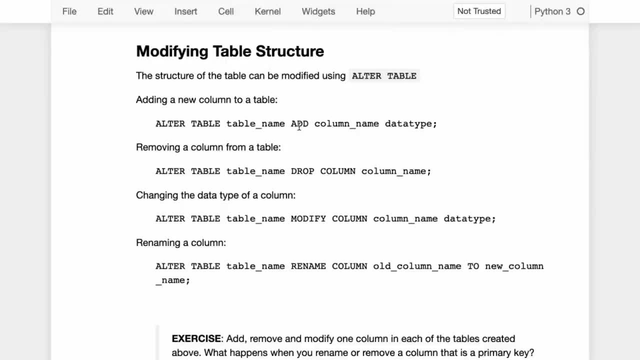 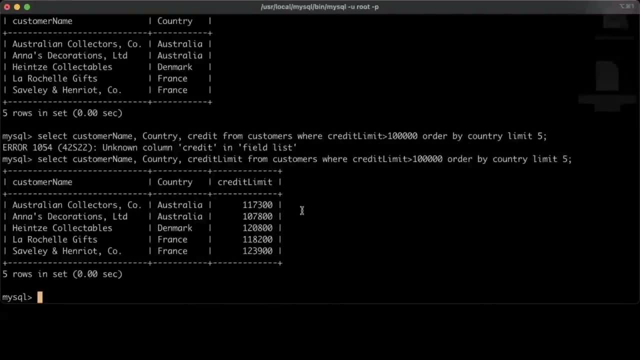 You say: alter table, table name and then uh, add, and then the column name and the data type And that's going to add the column. Maybe let's do it very quickly for employees. So alter table, let's. 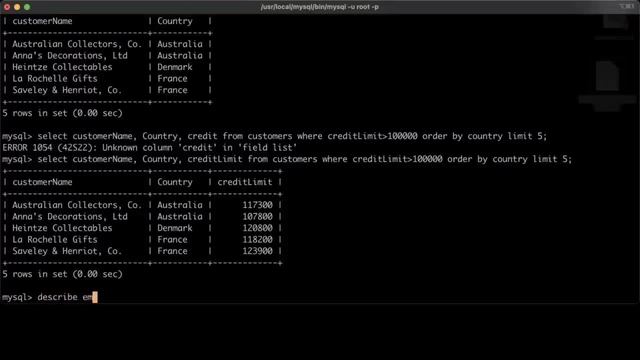 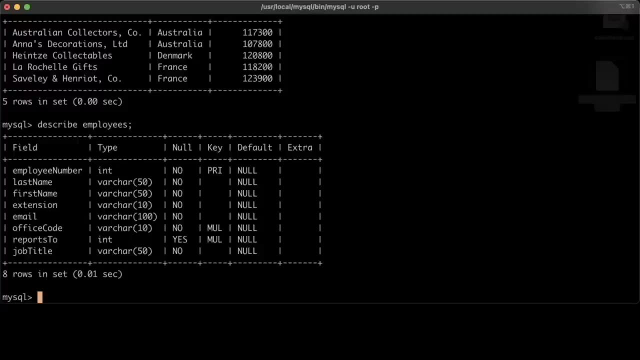 See employees, the let's, let's check the employees table first employees to describe employees, And now let us maybe add the date that they were hired on. So we will add, we will say: altered table employees. What's that Add? yeah, 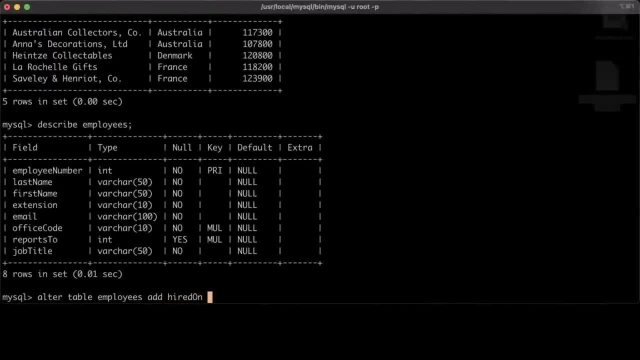 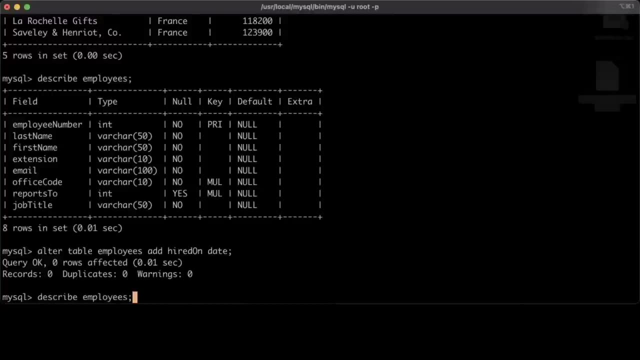 Add and then the column name hired on and we want it to be a date. Okay, See, It seems like that was added. So now if we check describe employees, you should see that there is uh hired on column. 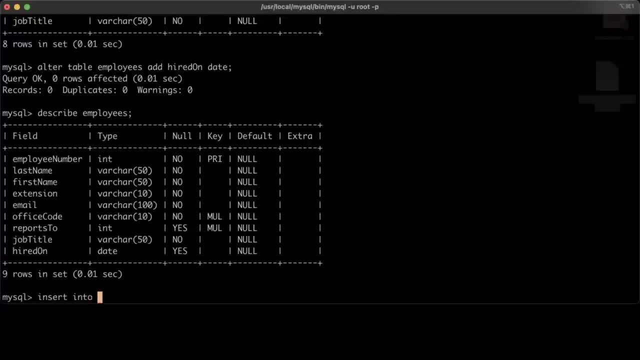 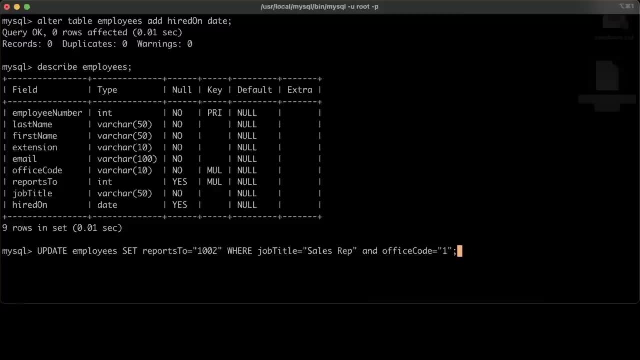 And if I want to insert an employee, insert into employees, yeah, if I insert an employee now I can probably. then I can probably then add some information, let's say set employee reports to, et cetera, et cetera. 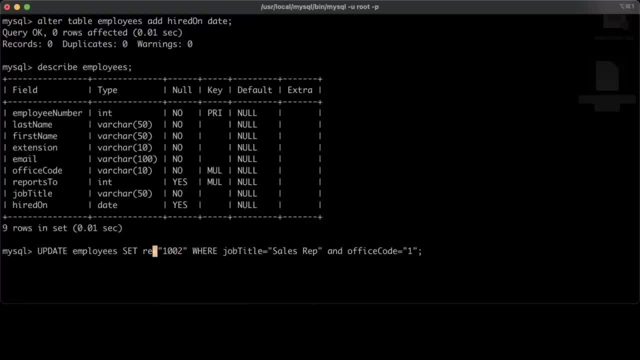 So we can probably uh set the hired information Right. So hired on to 1 0 0, 2, and let me change this to an actual date. So 20, 20 is a 12 0, 1.. 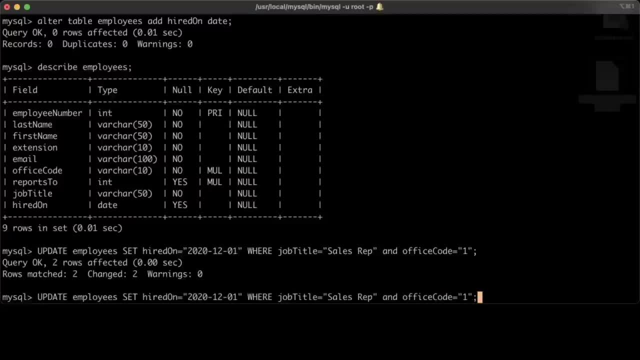 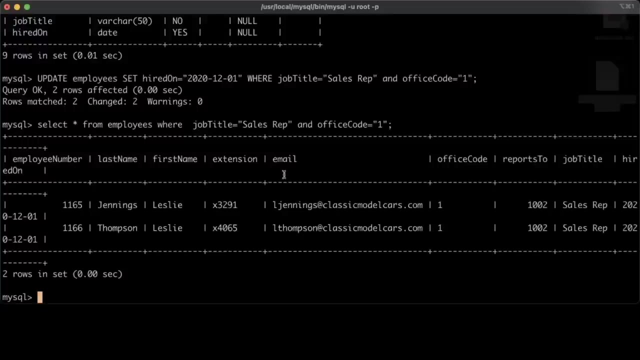 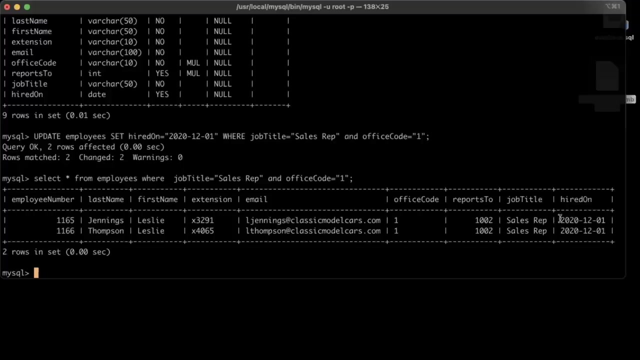 Okay. So now if we check employees again, let me just get these employees So select star, select star from employees Where job title is such and data such. so you can see, now with these employees we have a hired on column and in the hired on column the value is 20, 20, 12 0, 1.. 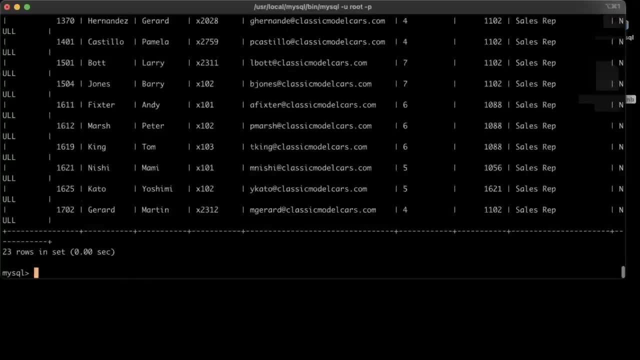 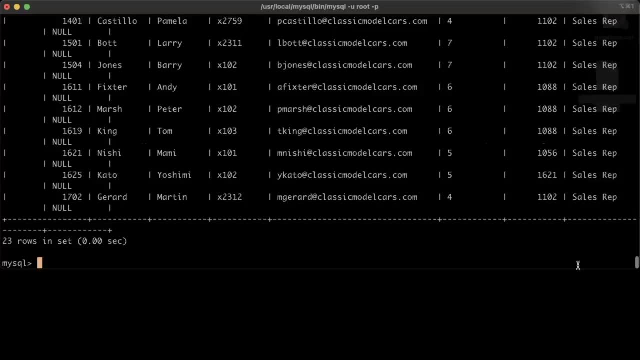 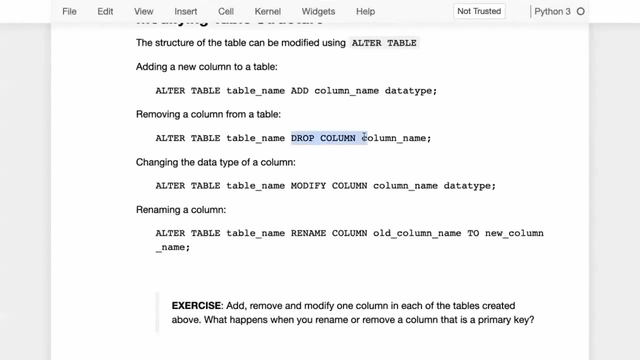 And for the other employees, you will see that the hired on column does not have that value. So that's how you add data. nothing too special, nothing too complicated. It's just one more thing to know. You add a, And similarly you can drop columns using the drop column command. 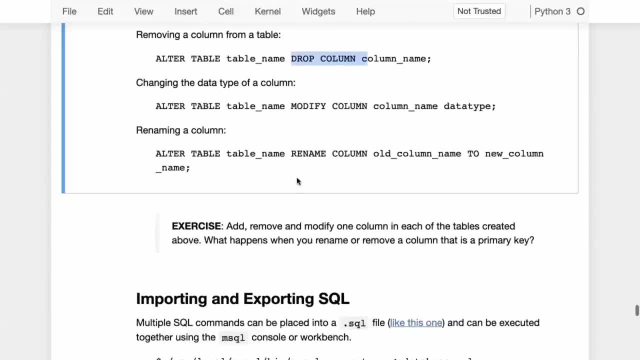 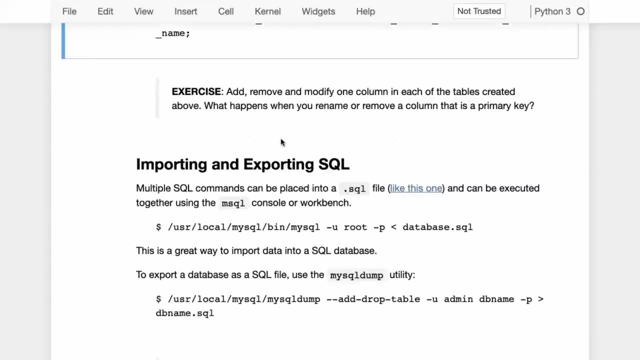 You can modify column using the modify column command. You can rename column using the rename column command And here you say rename old name, old column name to new column name after alter table. So as an exercise, try adding, removing and modifying one column in each of the tables created and what happens? check what happens when you remove or rename a column. that is a primary key. 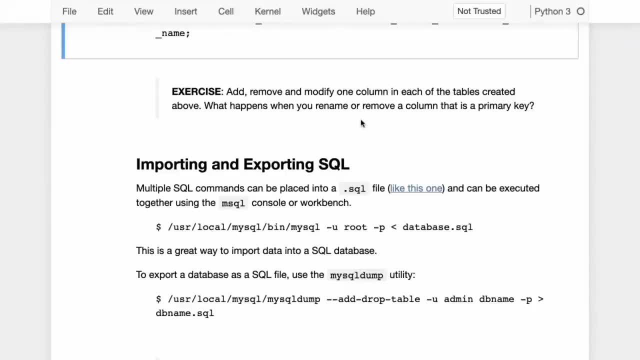 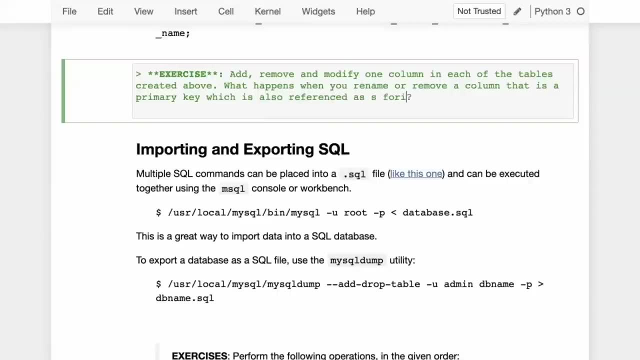 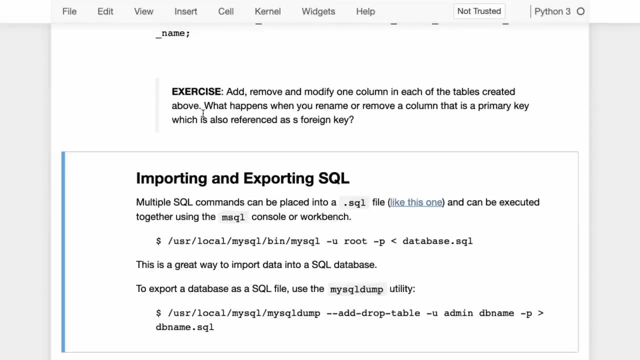 Because that is a primary key which is also used as a foreign key. Yeah, So do try that out. So if you change the employee code, for example the employee number, now that is used in a bunch of different tables, like the customer table. 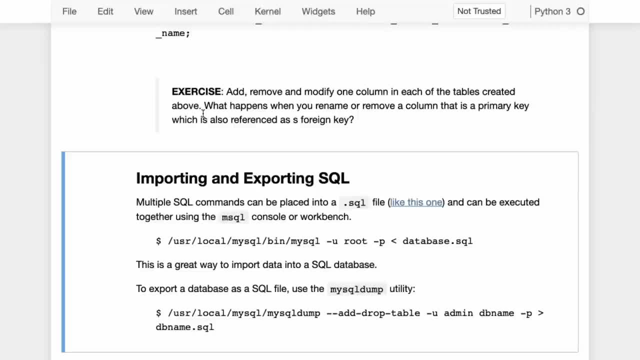 So what happens when you change the employee number column? Try it out. That's the best part about interactive. Okay, So if you change the employee number, that's the best part about interactive. So if you change the employee number, that's the best part about interactive. 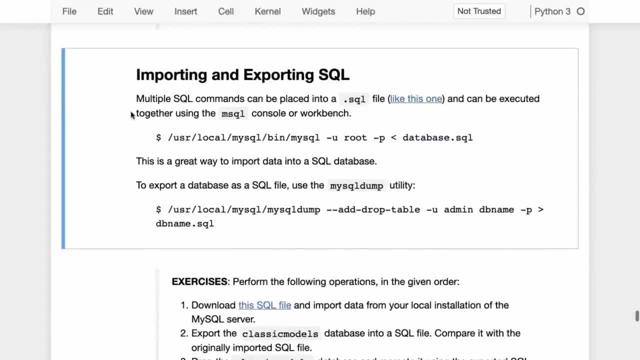 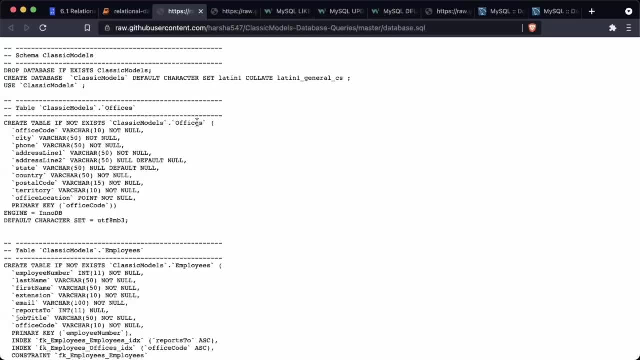 And you can try out things and you can break things and figure out what happens. Now you can also place a bunch of SQL commands into a dot SQL file, like this one that we've been looking at so far, and then you can execute all of these commands together. 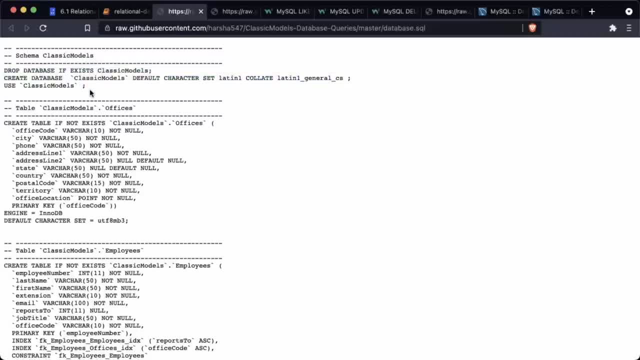 You can see that here we are dropping the database. We are then creating a database. We are then using that database. Then we are creating a table offices. We are creating a table employees. Yeah, Yeah, Yeah, Yeah, Yeah Yeah. 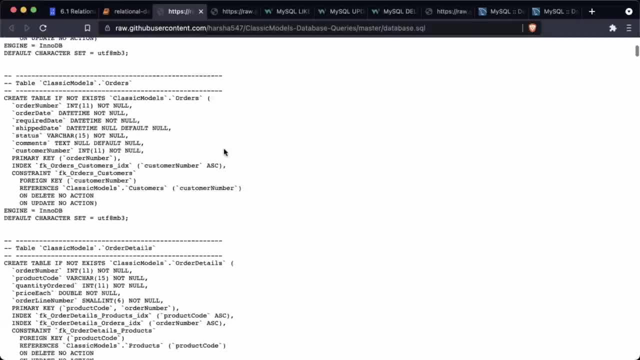 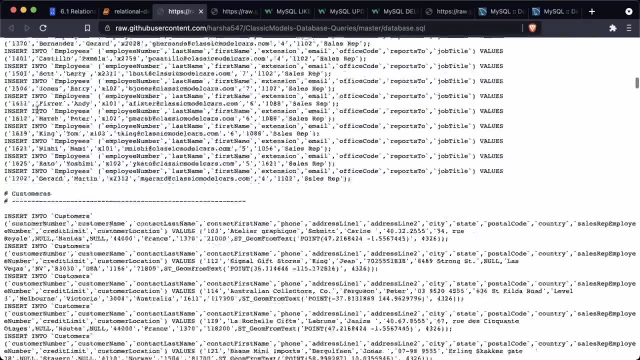 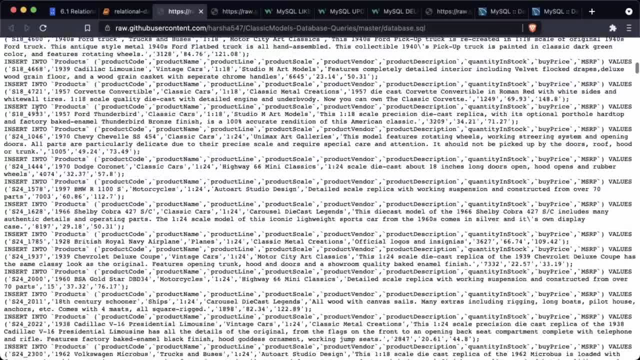 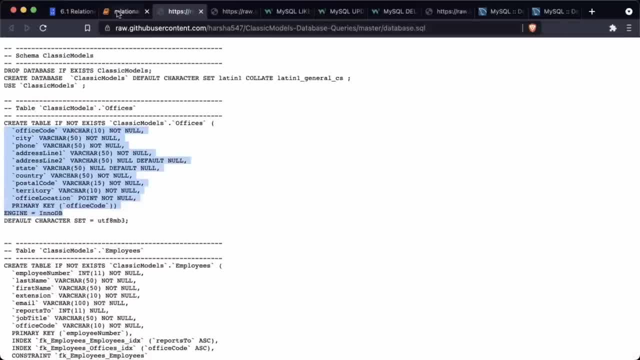 So this SQL files is basically what's called a database dump, that somebody had this database and then they exported it and we'll see how to export it as well. But now you can take this data and import it into, or just run all these SQL commands and automatically import the data into your SQL Server, into your SQL database. 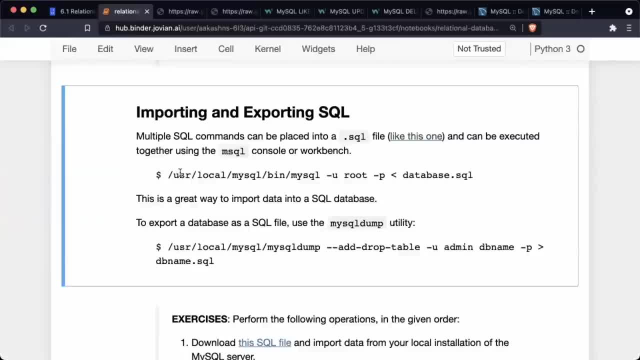 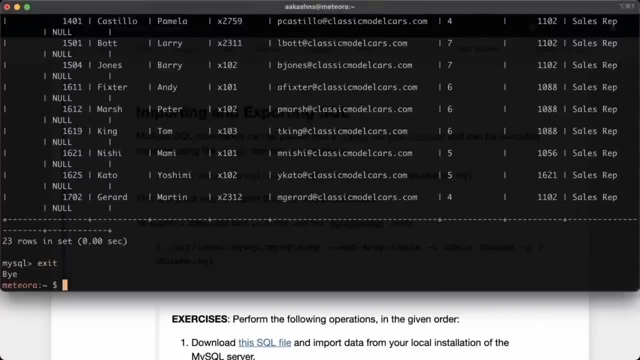 And here is how you do it. So you, there are two ways to do it. One is through the command line. Now, through the command line, let's say: go back here, I exit, I exit the actual command line and let me come to my desktop, which is where I have this file: database dot SQL. 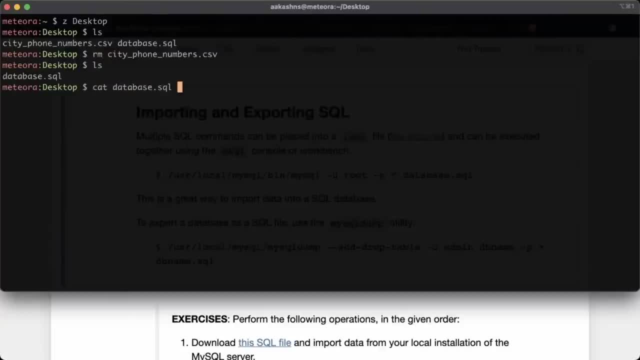 So I have this file here- database dot SQL- and I can check this file. It contains exactly what I was looking at. I have just downloaded this file here, So I find my MySQL binary, which is in slash user, slash local, slash MySQL, slash bin, slash MySQL. 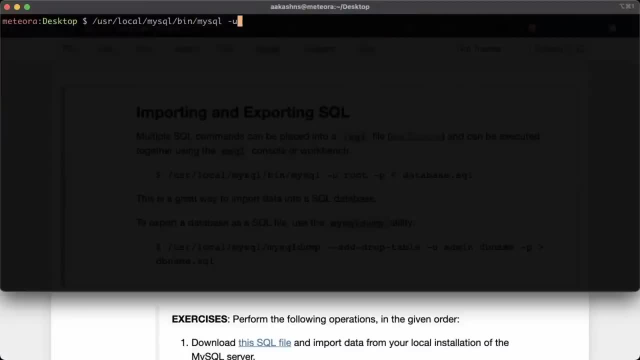 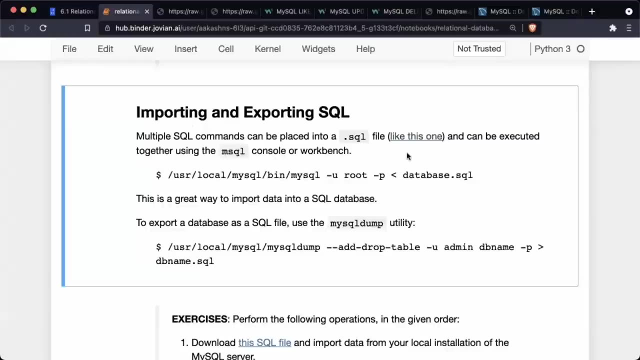 So this is the MySQL command line tool. And then I say minus, you root, So I want to log in as a root user. And then I also say minus P because I want to use a password. And then this is the magic part, where you use this less than symbol. 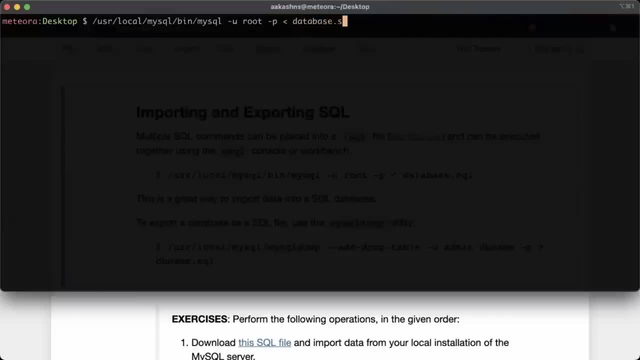 And I'll tell you how to think about this. So you have this less than symbol database dot SQL. So what you're indicating Here is: take the data and database dot SQL and passes that, pass it as inputs to this command. So now we're no longer opening up the console, but we're taking all of these commands. 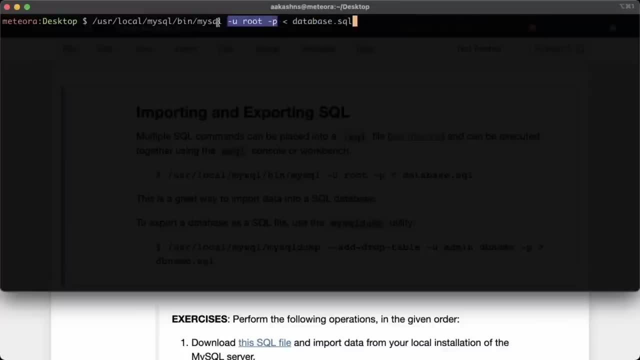 inside the SQL file and passing it as inputs to MySQL, which we are logging into as the root user. So when I run this, let me just just to make things very simple, what I'll do is I'll first just open MySQL Slash. 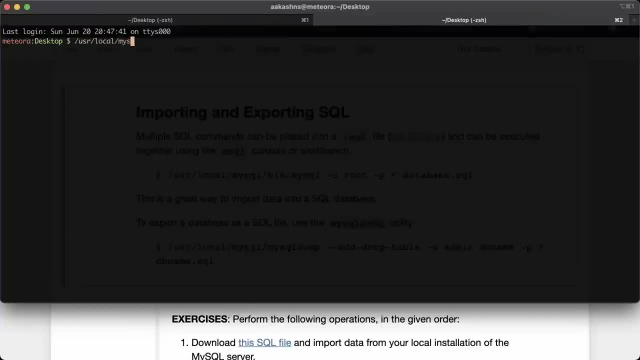 Slash user: slash local. slash MySQL. Slash bin slash MySQL. So I'm just going to open this first. Minus U, root, minus P. I'm just going to open this first and I'm going to drop Data base: classic models. Okay, And let me just do show databases. 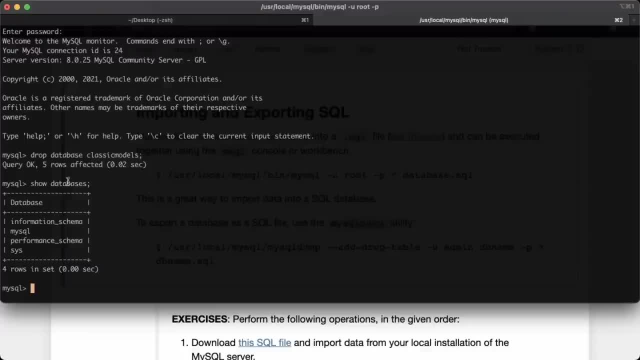 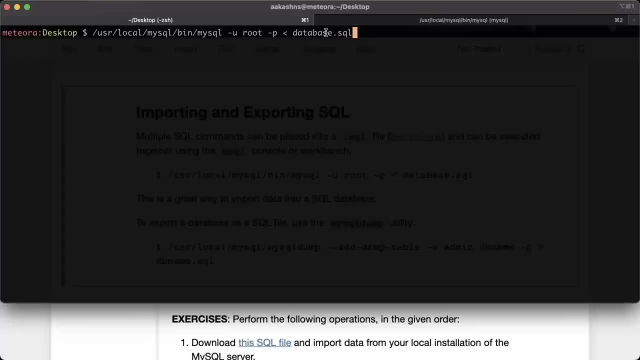 Okay, Let me just do show databases And you can see that we don't have classic models here. So now we have, we run this code: my SQL, minus your root, minus P database dot SQL, And this should take all those lines of code and it should. 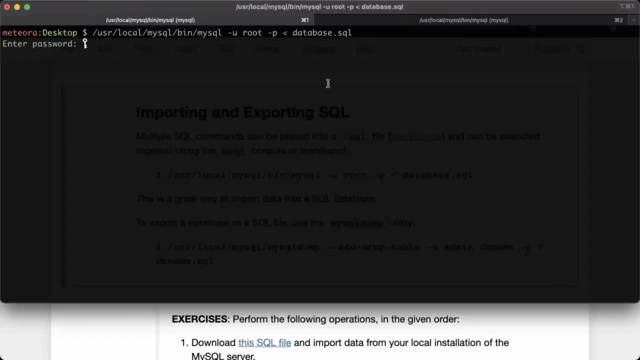 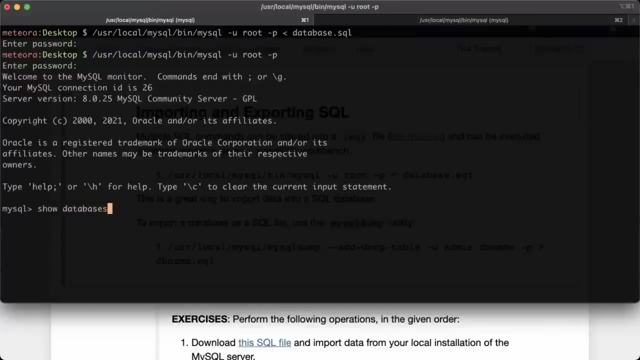 execute them against this server. Yeah, it'll take a minute or two, but it's done. And now, if we come back here into this, or if we just open up my SQL now and just log in and do show databases, you can see that we now have classic models and it is not showing up. 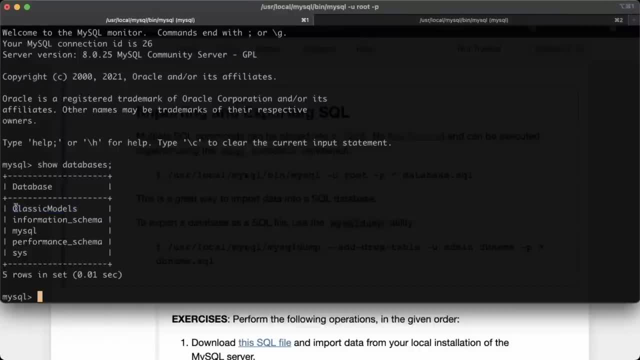 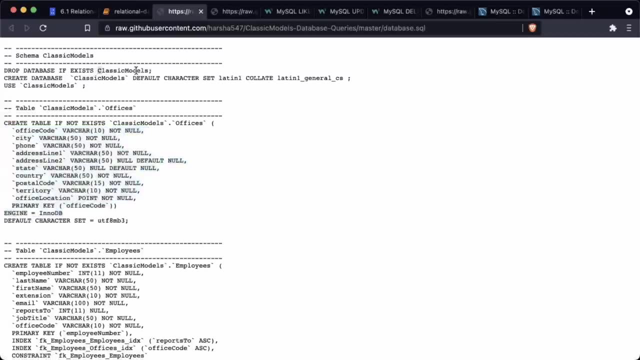 showing up in a uppercase, because in this script file, the database, when it was created, it was created with this uppercase in uppercase M, but as such you can still just say: use classic models without uppercase. We can just say classic models and it should work just fine. 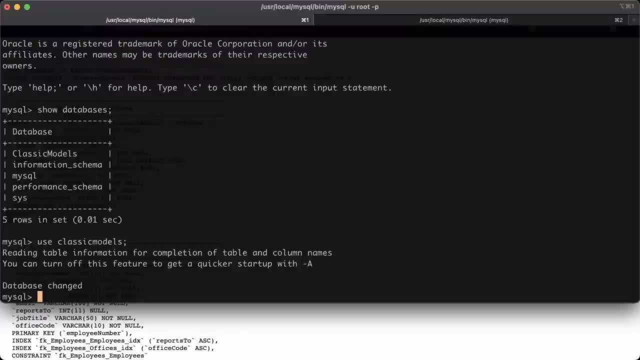 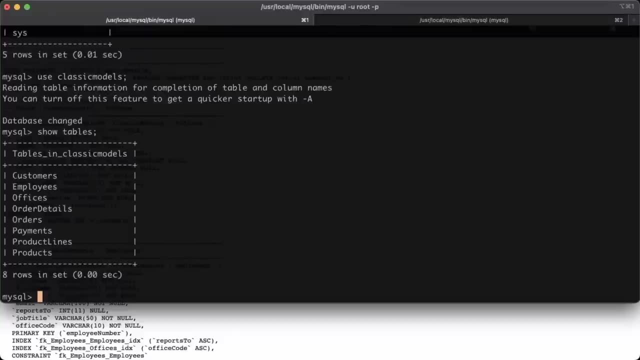 So now we have classic models, and we can see that we have classic models, and we can see that we have classic models. and now you can do show tables and you have all these tables- customers, employees, offices, et cetera- And now we can do select star from offices. 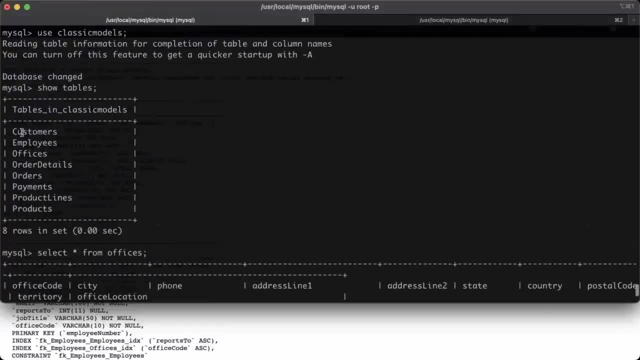 And you can see that these are all the offices that we have, And so, even though it shows up as uppercase here, because that's how it was created, but you can still access it as lowercase, uppercase or this title, Okay, So whatever, right. 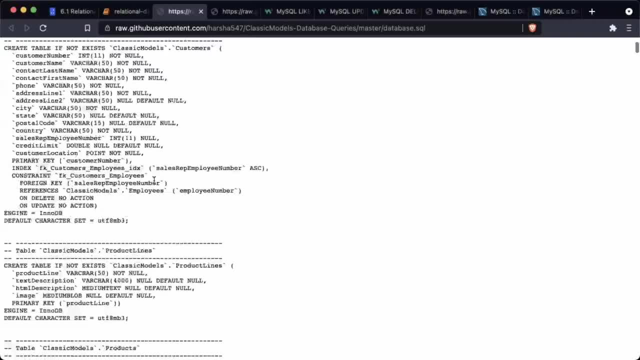 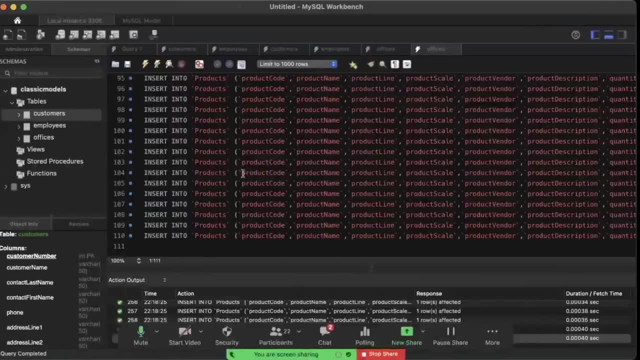 So we have taken all that information and then we have taken all these lines of SQL code and we have executed them on the database. So that's how you execute data. One other way to do it is you can also do it this way from seeing my SQL workbench. 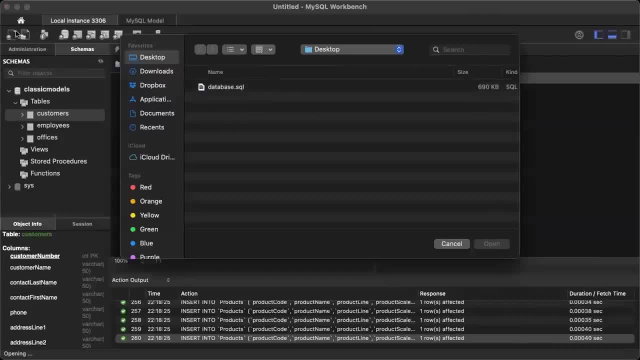 You can click on this or you can see open SQL page, open SQL button. So you have this open SQL file button here, the second button: click on it and go to desktop and open it up. Now, depending on which database you're using, the UI will be a little. 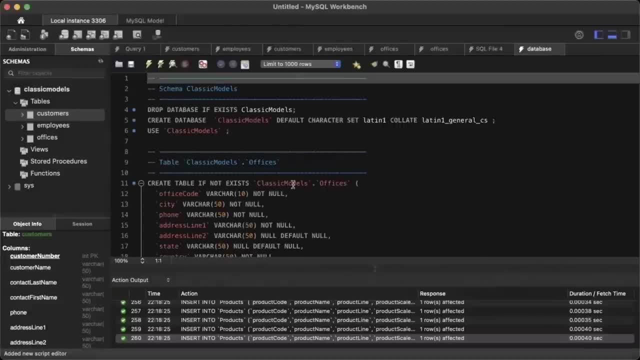 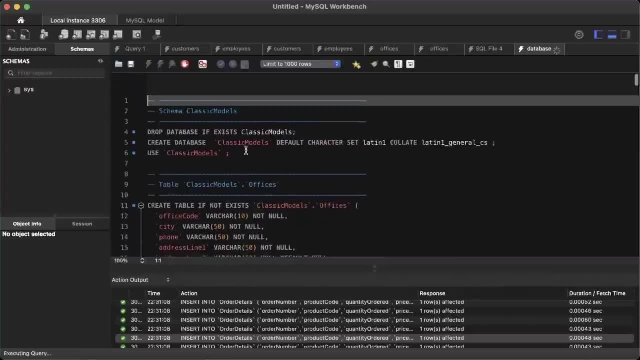 A little different, but the concept here is that you can do this. You can take a bunch of SQL code and then you can execute all at once, and it should do the exact same thing. So here it drops the database, So it's going to empty the database and then it's going to add all this information. 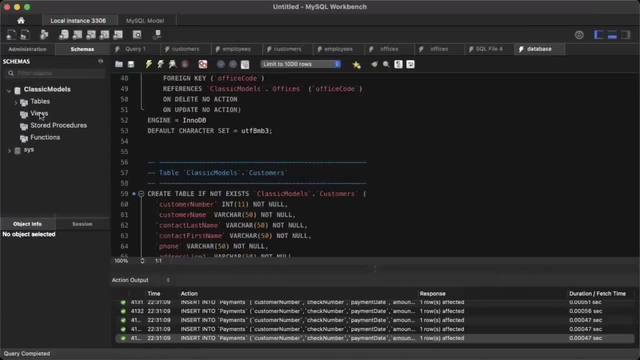 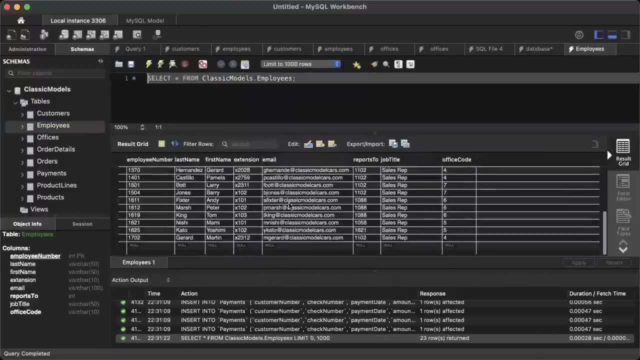 And now, if you just refresh here, you should find classic models and inside it you should find these tables and then you can maybe click on employees and you can see all the employees. So you have all the employees, just fine. One other thing. 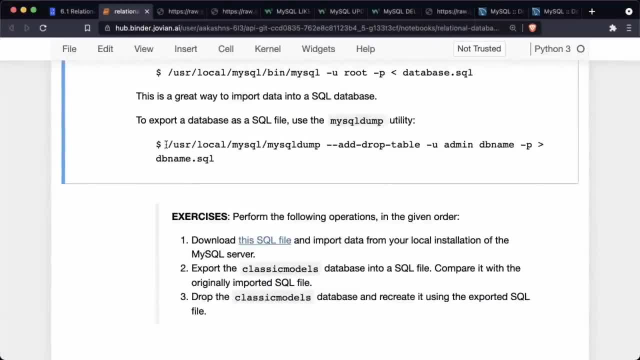 You can do is you can export data out. So there are a couple of ways to do this. One is to use the MySQL dump utility, So the same place where you have the MySQL utility, which is at. let me just exit here. 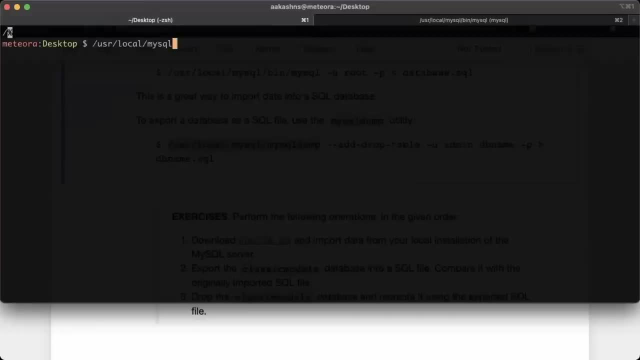 So we have at user local MySQL bin. Again, this will be different on windows or probably different on Linux as well, but you can find it quite easily, Just Look it up. So use a local MySQL bin, MySQL- right. So this is how you open the command line. 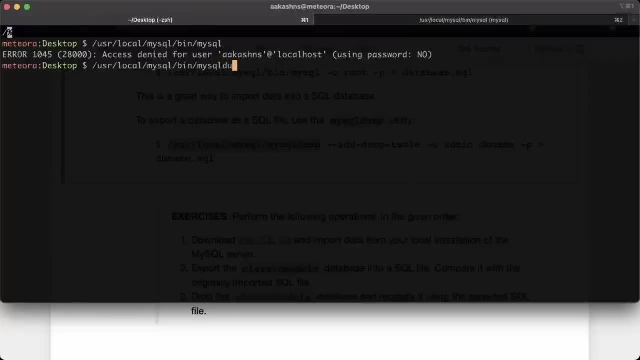 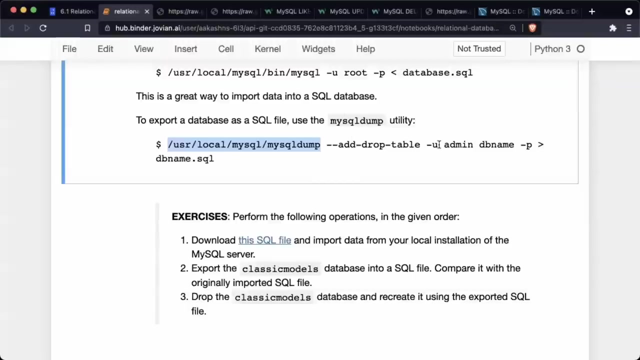 This is what we have been looking at so far. but you have a MySQL dump utility, so you can call MySQL dump and I want to use the root user and I want to use a password, and what? how does it work? So we have to provide it the name of the database. 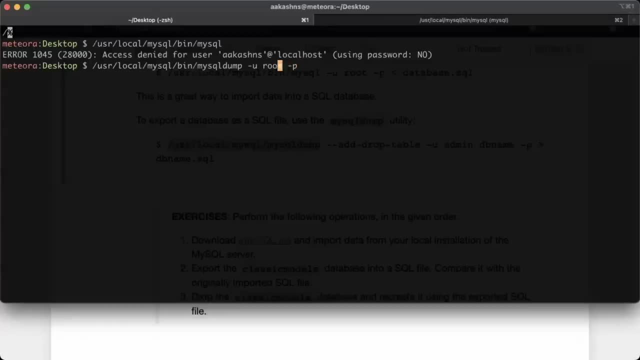 So we provide the name of the database after minus Yeah, Or even at the beginning: So MySQL dump. the database that we want to dump is called classic models And then there are certain options that you can specify that. Do you want to have these drop table lines? 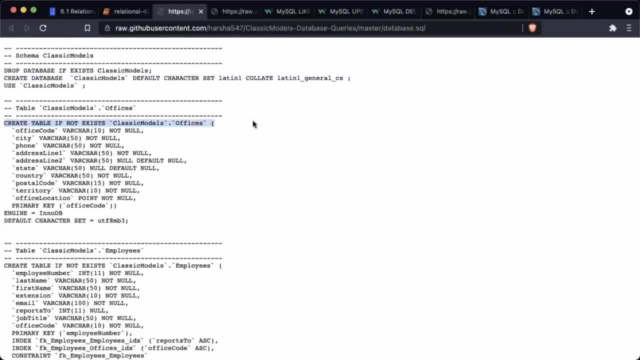 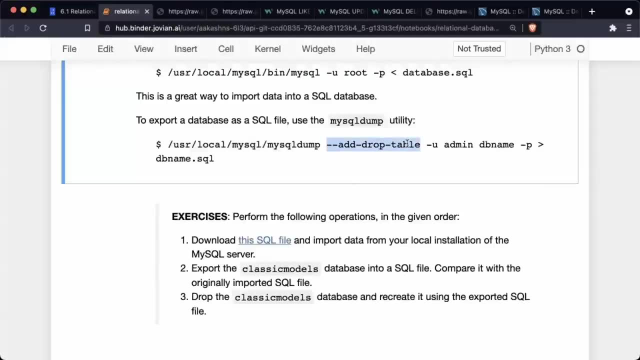 So if you see here, before every table creation there's no doc, there's no drop table statement, but we can add that drop table statement as well by specifying this option And again, you would just have to look up the documentation online to figure out how exactly this. 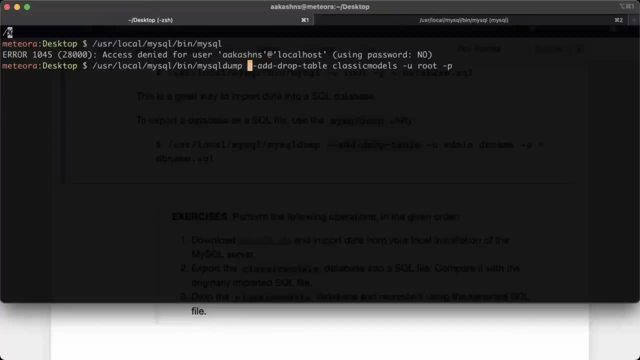 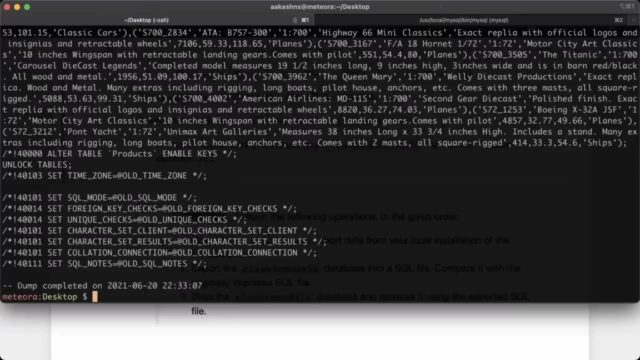 All these options Work. but yeah, MySQL dump draw at drop table classic models minus you root, minus B. Okay, And that has created this sequel file. Oh, but we forgot to write it to file. We want to actually write it to a file. 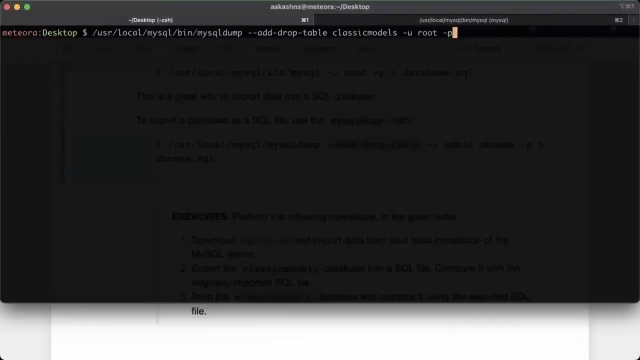 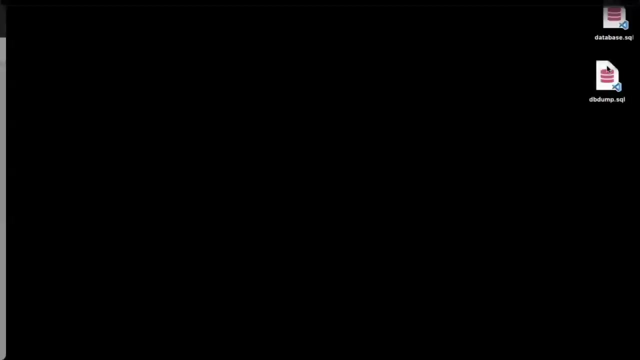 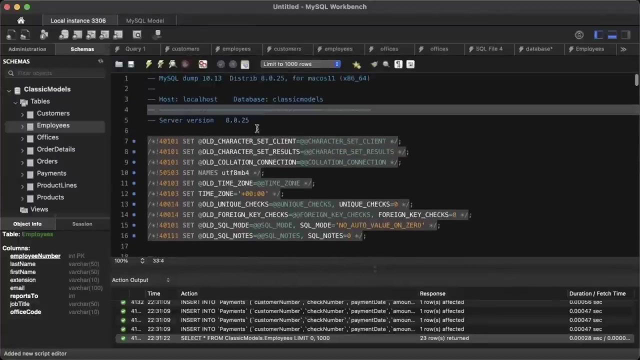 So right now, it is just printed it out. So what we're going to do is, instead of printing out all this information, we want to write it into, let's say, DB dump dot SQL. Okay, Okay, And just like that. this should be now. there should be now this file, DB dump dot SQL, which should have all the information that we're looking for. 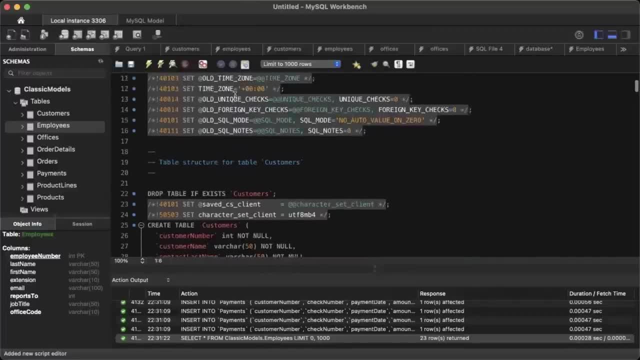 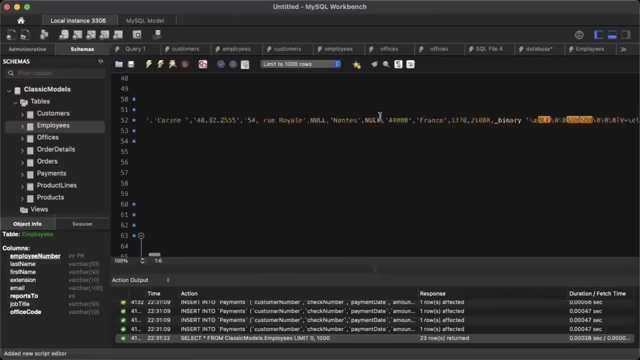 So it has. it has this drop table- If exists customer, then create table and then below it it has the data for customers. So Okay, Insert into customers and you have all this customer data and then you have data for employees. 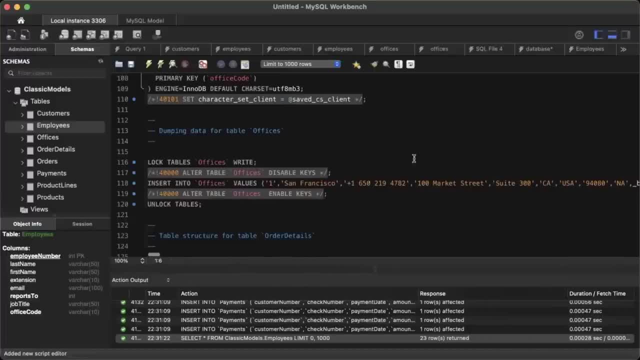 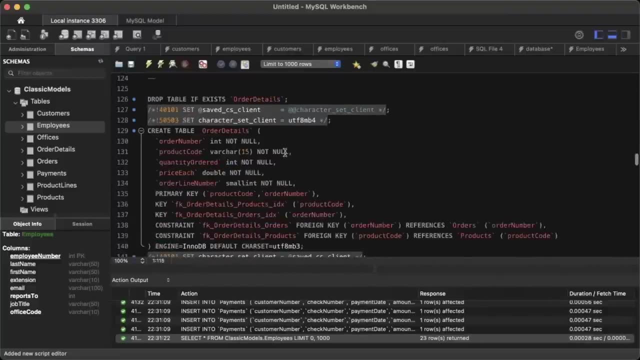 Then you have data for offices and so on. Okay, Now there seems to be some encoding error here. for some reason, this is treated as binary. I think it's probably the office location that is causing an issue, but as such, everything seems to be just fine. 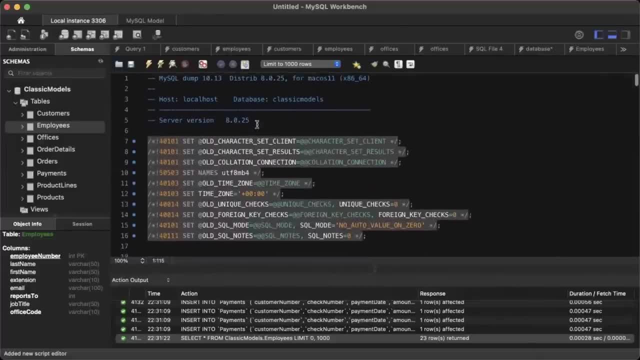 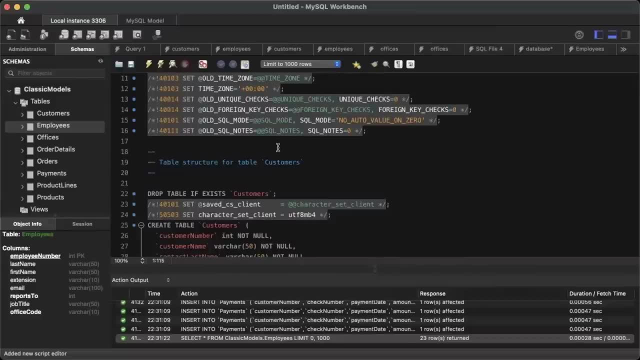 And then you can take this and then you can use that to reload the data. Now here it does not have the commands to actually create the database. I'm sure There is some option that you can specify in SQL dump to create the database. 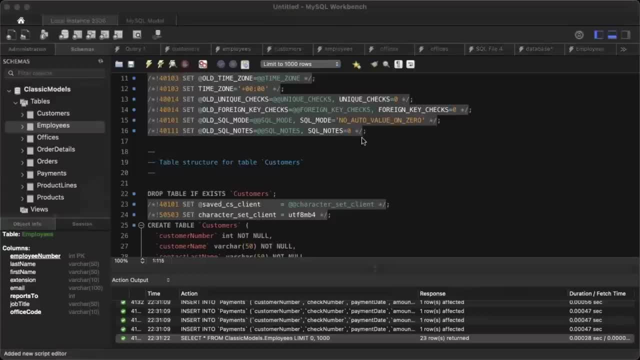 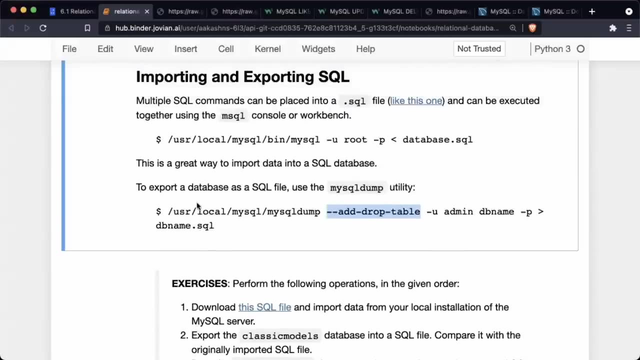 If it does not exist and drop an existing database as well. So I'll let you figure that out. but yeah, but this is what we are interested in And this is something you can do if you connect to a remote database. right now we are connecting to a local database, but if you 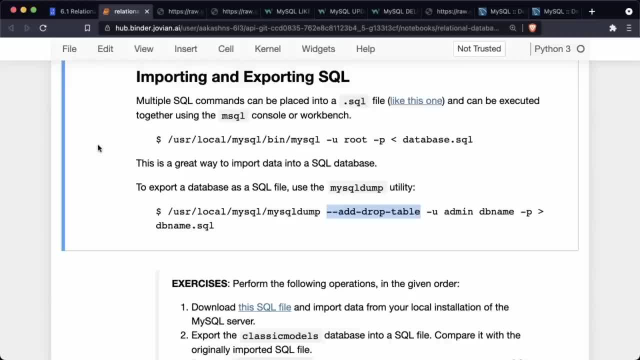 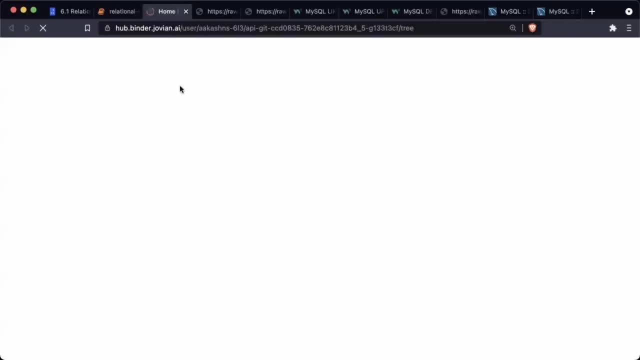 connect to a remote database on some server, you can export all its data into a SQL file, And then there are converters in pandas. What you can do is you can actually load up SQL files. Okay, Maybe let's try that. Maybe let's do file open here and let us upload. 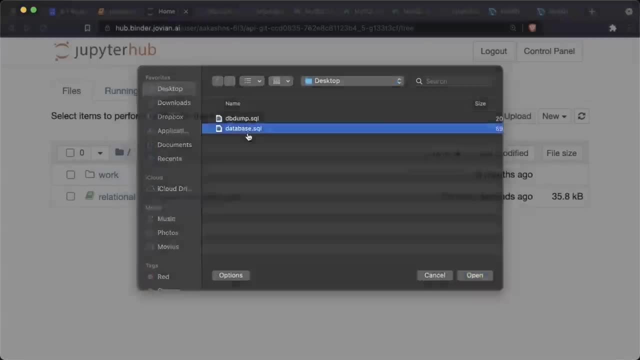 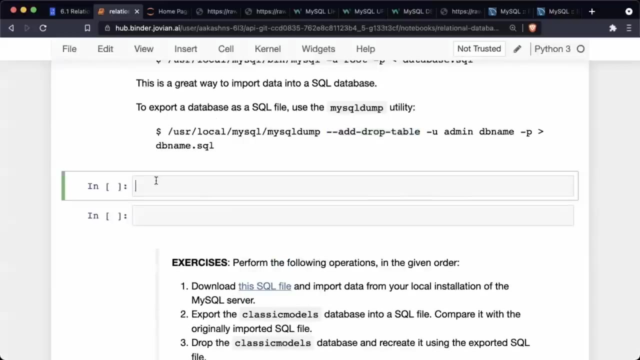 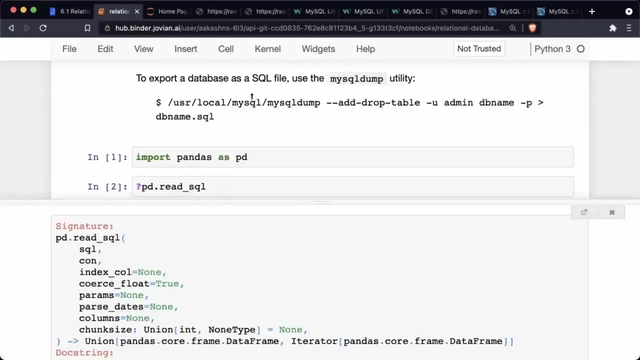 I'm not too sure, but I think this might work. So let us upload database dot SQL. Yeah, And you should be able to do something like this: import pandas as PD and that PD dot read SQL. Let's see. Oh, I think this needs to be a SQL command and a connection. 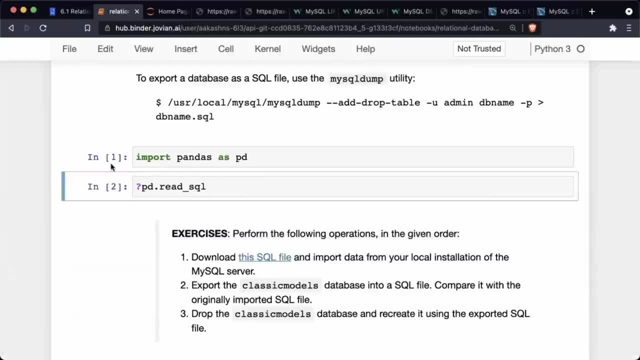 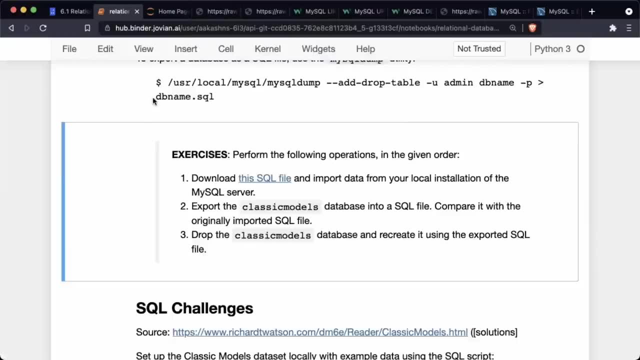 So it's not going to work. with a SQL file. You need to actually connect to a database. So we look at it the next time. but yeah, but there are ways to read that SQL file. There are ways to convert SQL files into a bunch of CSV files. 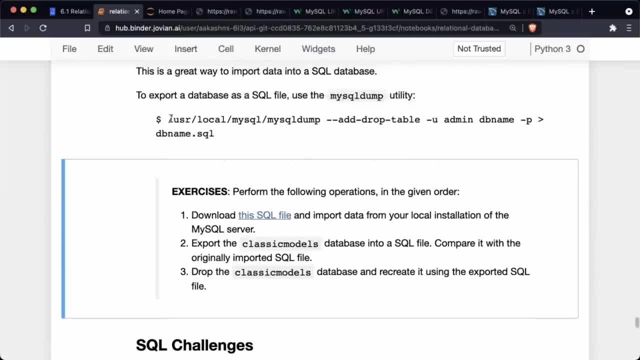 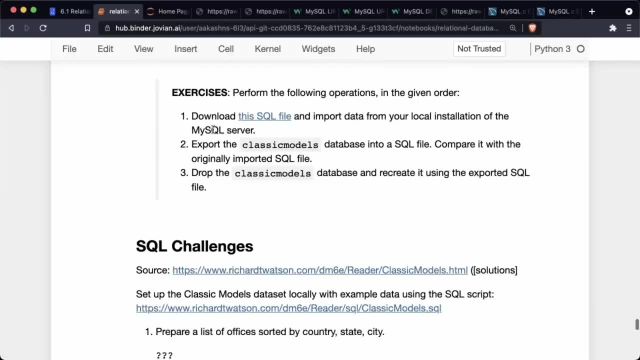 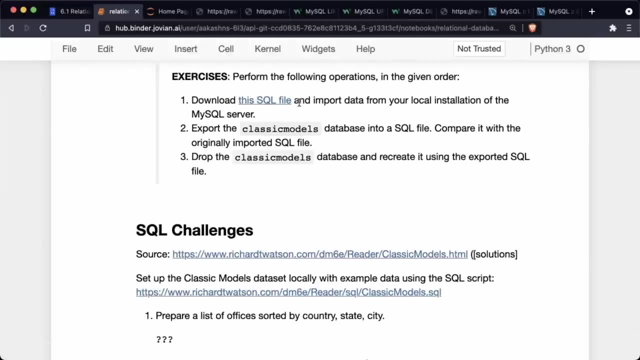 I know that there are ways to convert that into a bunch of different formats. So exporting it is useful because you can then load back that data into a new database server, or you can also convert it Into different formats. So try this out on your own: download the SQL file, import the data from your local installation of my SQL server and then 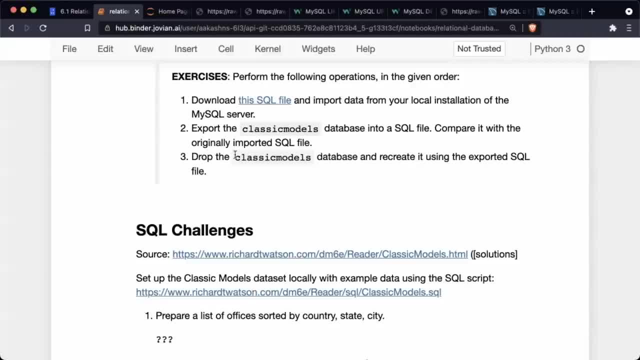 export the classic models database into a SQL file, then drop the classic models database and then recreated using your exported file. So make sure that your exported file can actually recreate the data. That's an important thing you should be able to do, Okay. 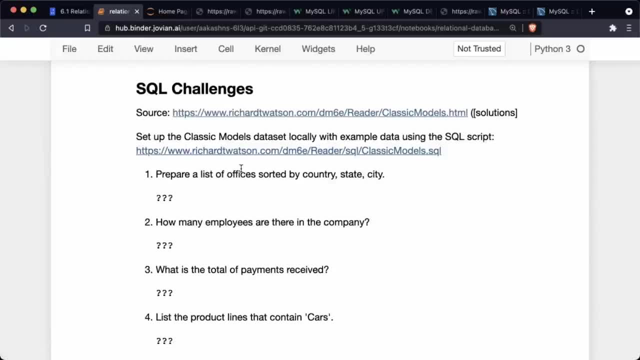 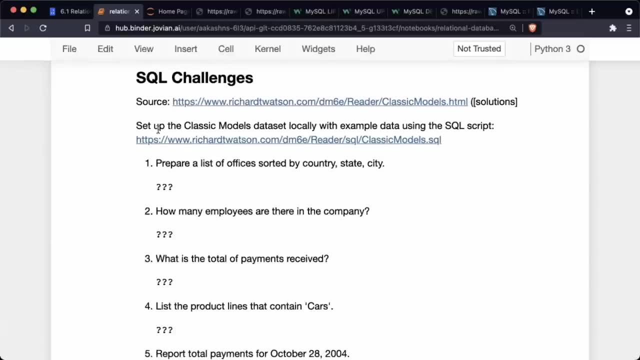 So with that we reach the End of today's lesson. there's not much more that we're going to cover today. There is a lot more that we need to cover in SQL, but we'll talk about the next time. but here are some challenges for you to try out. 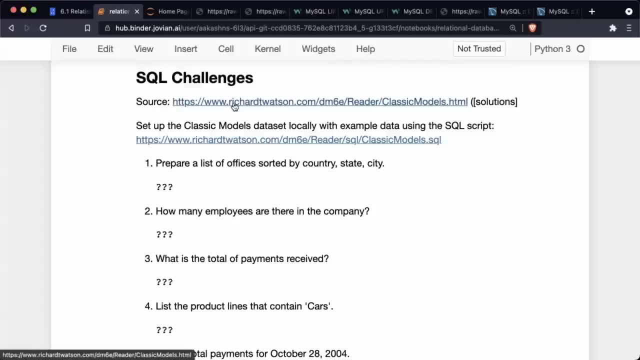 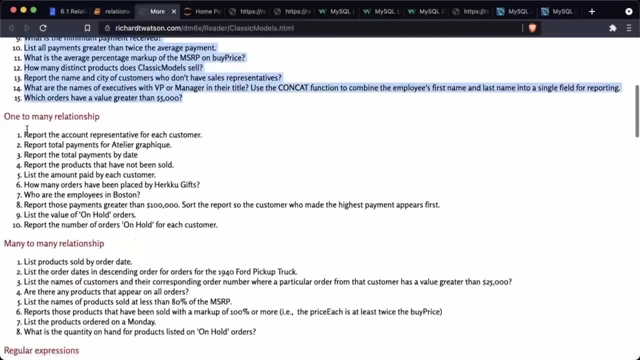 So this classic models data set is taken from this website, richardwatsoncom. This is- I think this is a professor and they teach a database management course. So you can, and there are a bunch of exercises here. So today what we've covered are mostly the single entity exercises, but you also have 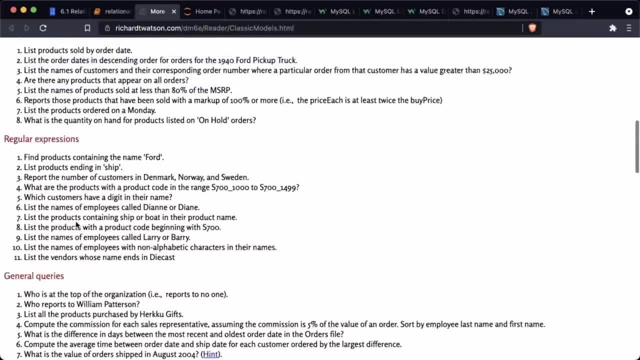 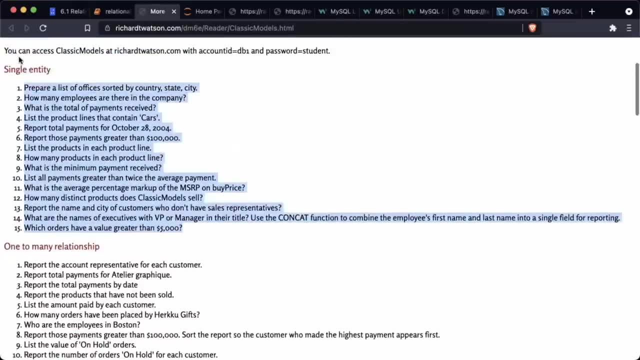 These other exercises which require some joints and some other things which we have not covered yet. So you may just want to try out this. prepare a list of offices sorted by country, state and city. This should be straightforward. How many employees are there in the company? 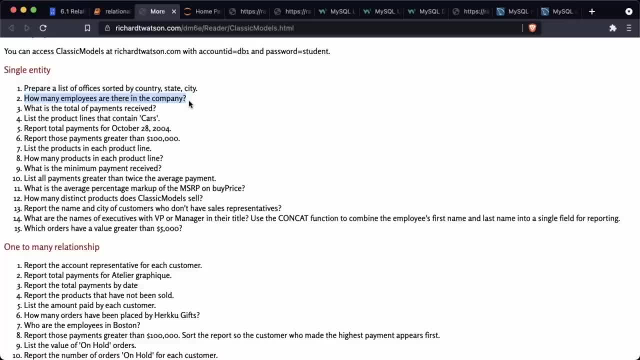 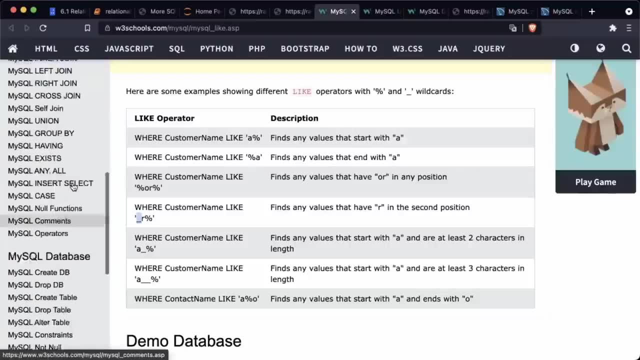 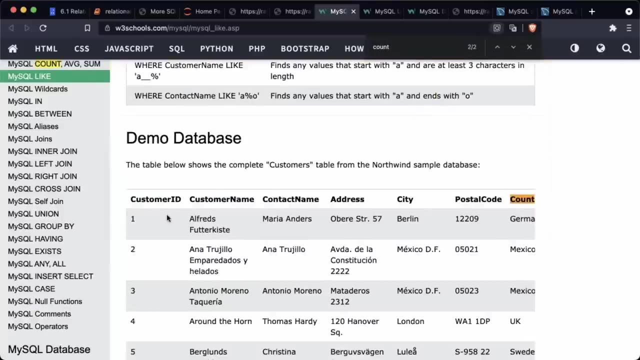 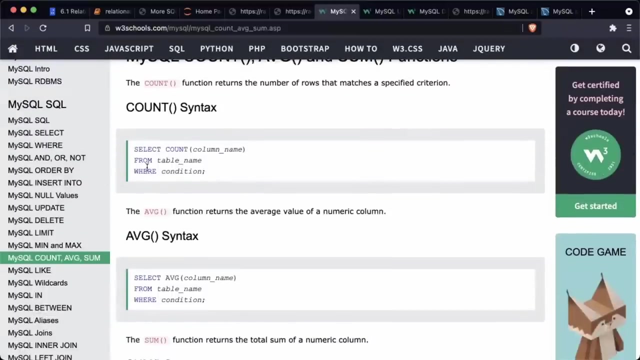 Okay, This will require some sort of aggregation or you can just look at the list of employees. but yeah, but one thing you should check out is you can check out things like count Where's count, count average and some, so you can do something like this: select count column name from table where condition and you can use that to answer this question. 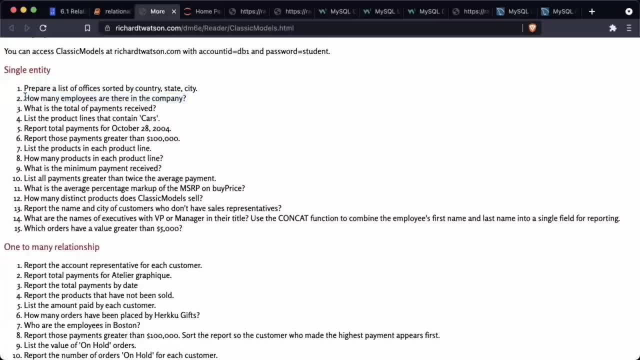 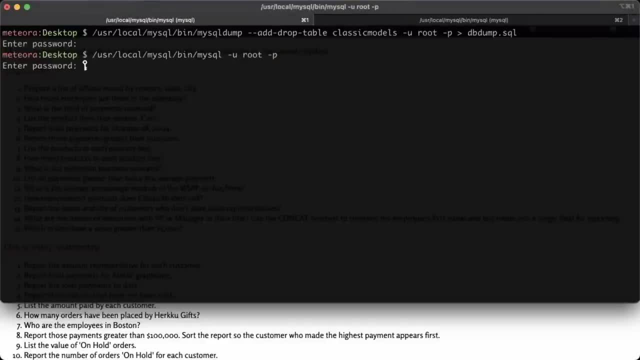 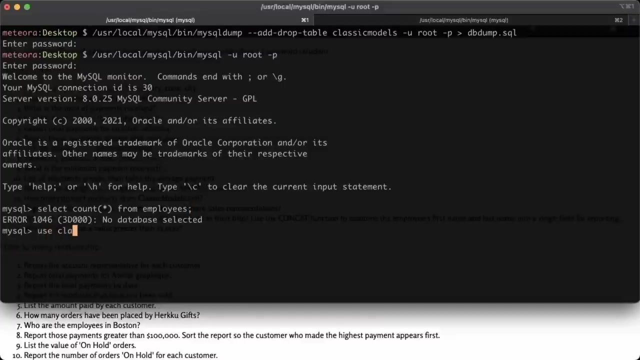 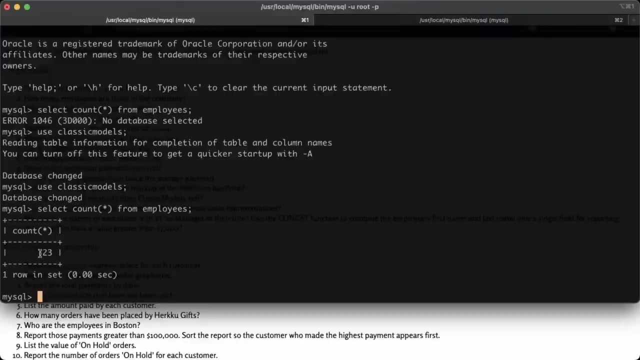 How many employees are there in the company. So here is how I would do it. I would say: select, count Star from employees and just use classic models. Okay, Select, select, count star from employees, And it tells you that there are 23 employees. 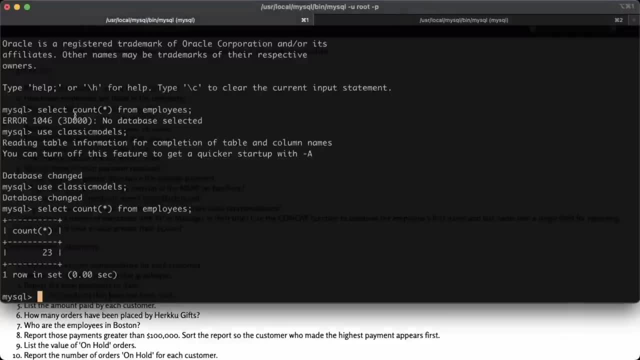 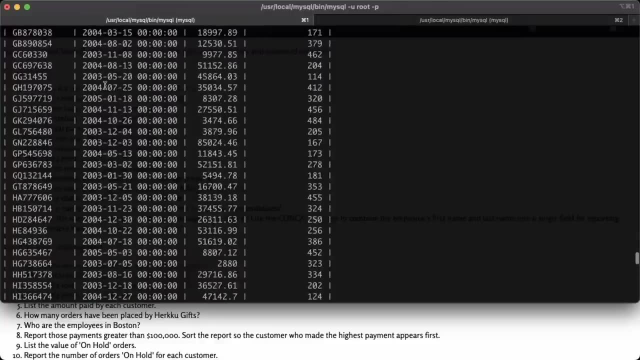 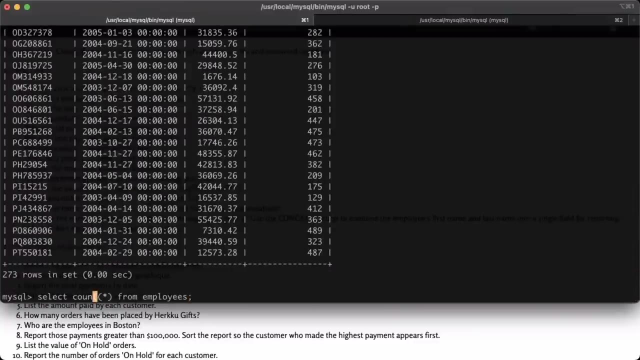 Then here's a question: What is the total of all the payments received? So let's see select star from payments And you have all these Payments And now among these payments there is this amount column. So if you just want to get the total amount, we say select amount and then we can do a sum. 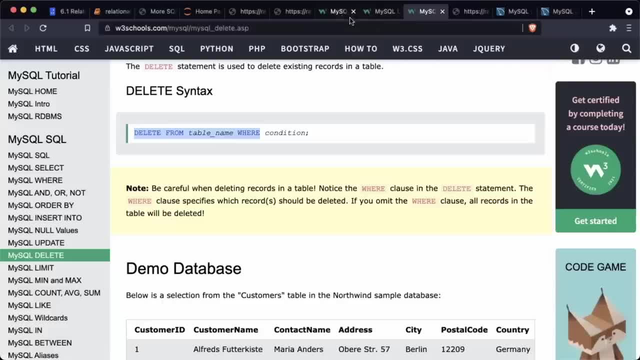 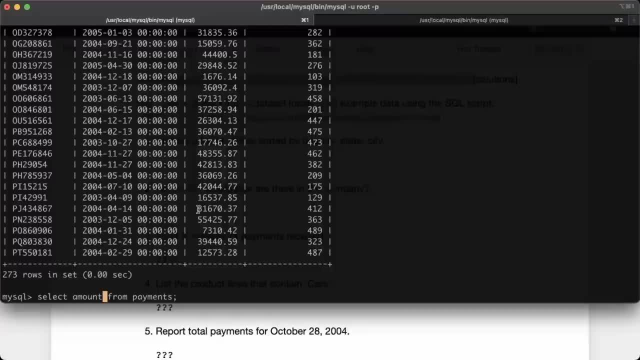 How do we do a sum? Well, I think it should be there here somewhere, So we can just do a sum on the column. So we do select sum of amount from payments. So this is the total payment that we have received, So we can do a sum of amount. 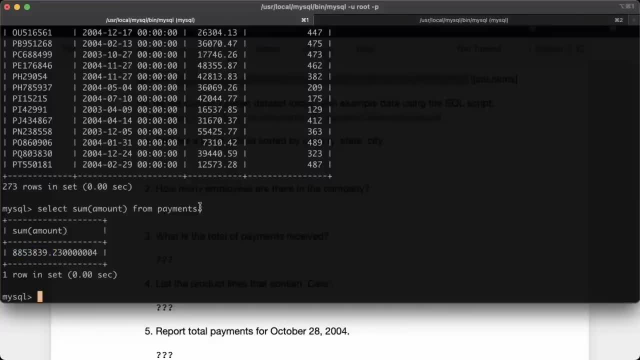 Okay, So we can do a sum. So this is the total payment that we have received. Now you can do things like: what is the total payment we have received from customers based in the USA or from a particular location, and you can do like a group by as well. 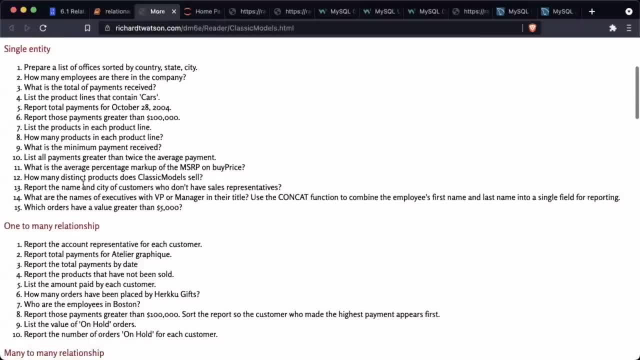 And we'll cover group by and all the next time. then you have questions like list of product lines that contain cars and report total payments for October 28, 2004.. So here's a where clause: report Those payments, A $100,000 list of products in each product line. 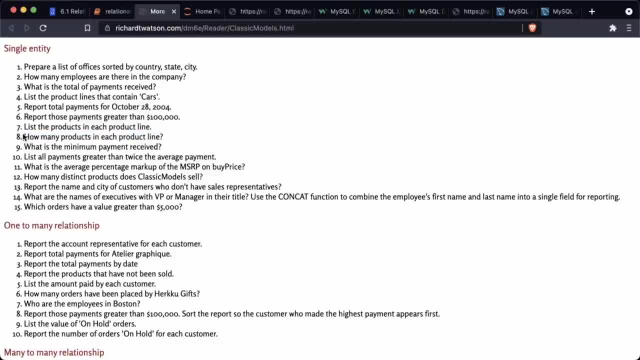 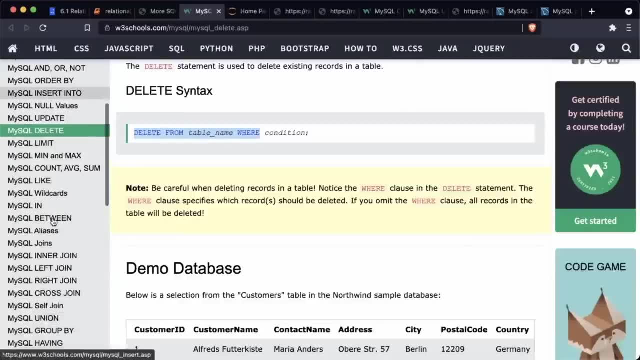 How many products in each product line. Okay, So this might be worth figuring out. You may have to, uh, use this as a reference. W three schools is a good reference here You can check out and see which one of these might be useful for you. 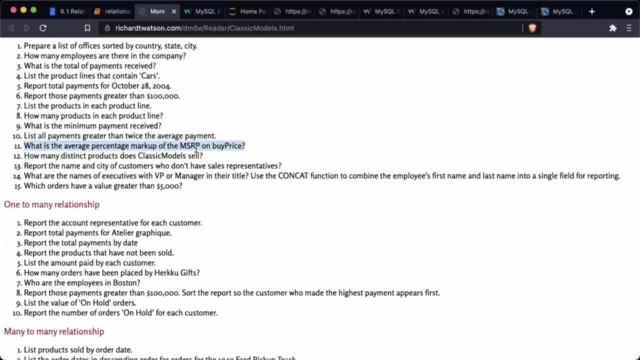 Then what is the average percentage markup on MSRP, on the buy price? So now you are comparing, you're doing arithmetic between two columns, Again something that We'll try and cover the next time. How many distinct products does classic model sell? report name and. 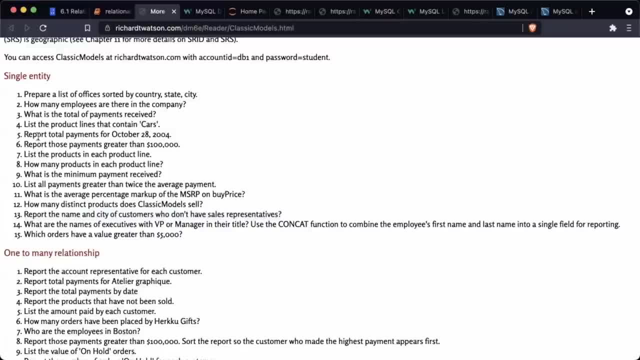 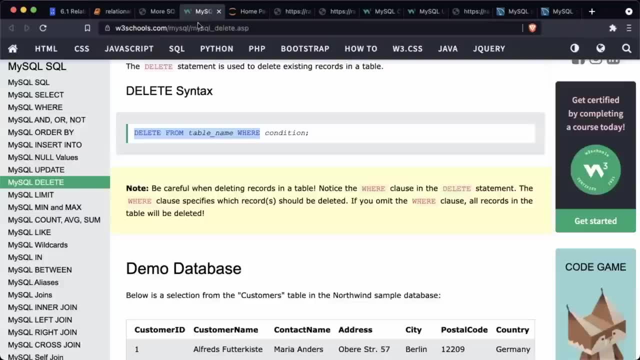 city of customers, et cetera, et cetera. So whole bunch of questions and whichever you're not able to figure out right now using what we have covered today. just try and look through this documentation. So this is everything that MySQL supports is listed here. 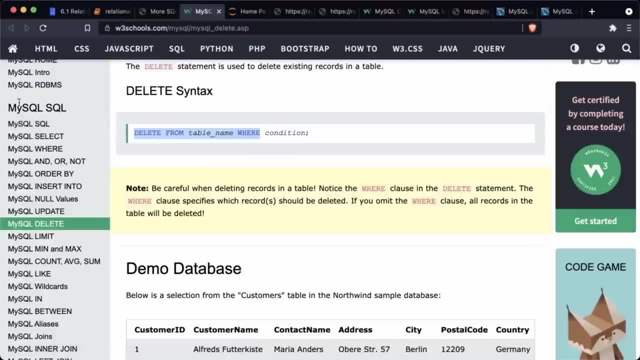 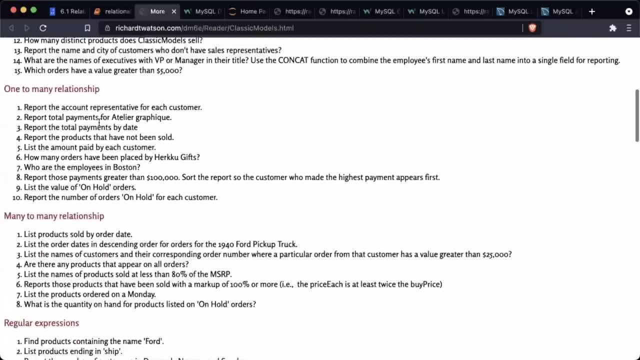 Most likely you will. everything that you need will be covered in this MySQL SQL section. If you just go through most of these, you should be able to answer these questions And then, wherever we have more than one to many relationships, or any relationships between multiple tables, we will look at the next time. 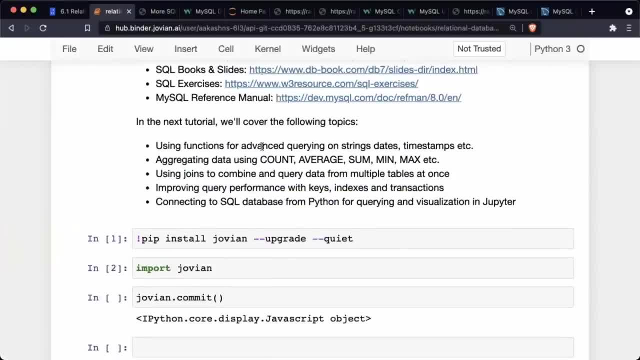 So the next time we will look at using functions for advanced querying on strings, dates, timestamps. We will look at aggregating data using count average, some main max. We will look at using joins to combine and query data from multiple tables at once. 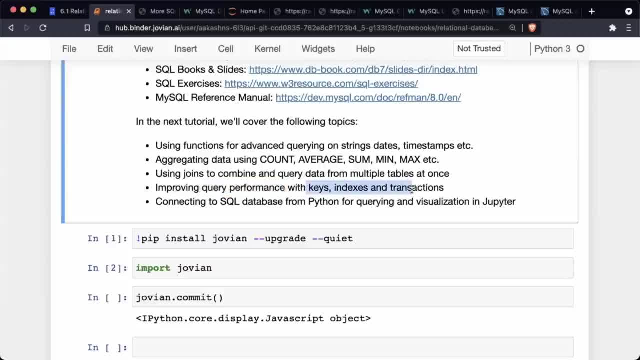 We will also see how to improve query performance with keys, indexes and transactions. And finally, we will look at how you can connect to a SQL database from Python for querying and visualization in Jupiter. So we'll look at how to do it using pandas. 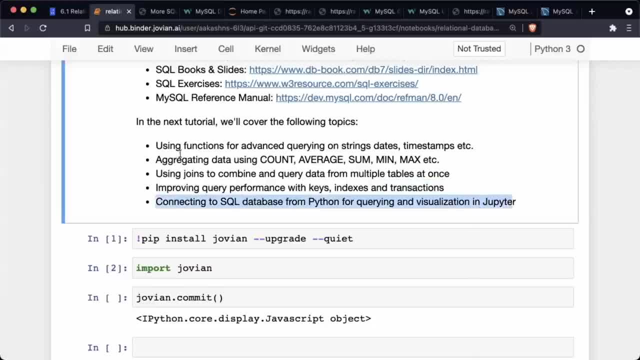 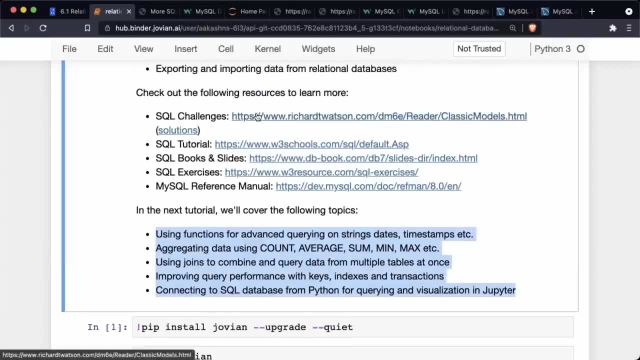 And we'll also briefly try and look at ORMs. So there's a bunch of things to cover here, But the more important thing in SQL is practice. So you want to definitely try out these challenges and there are solutions for these challenges as well. 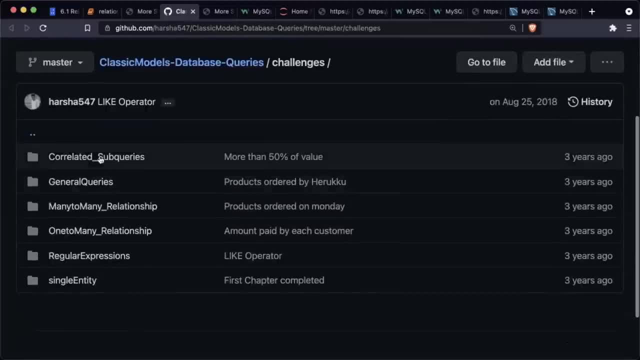 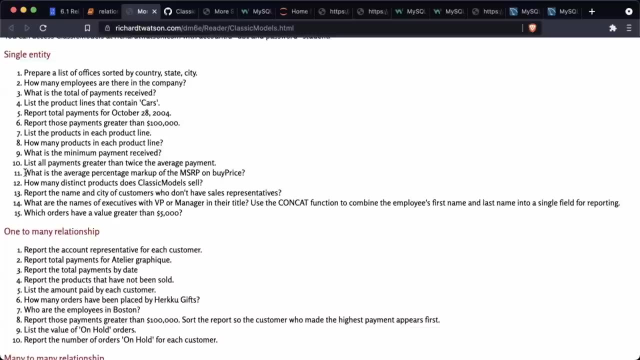 You can click the Solutions link and use that to check the solutions. For example, there was this query about what is the average percentage markup of the MSRP on by price. This is question number 11.. So let's see question number 11.. 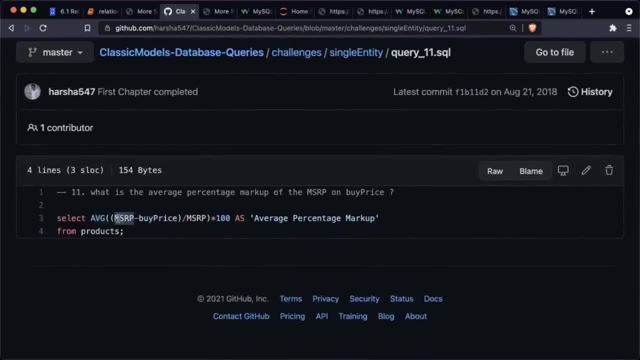 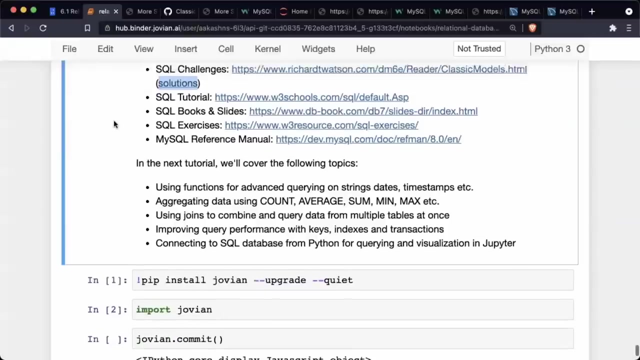 Okay, So it seems like we are doing some sort of a calculation here, So average of MSRP minus by price divided by MSRP multiplied by a hundred, As the average percentage markup from products. Okay, So we'll also talk about as the next time. now a few resources for you. 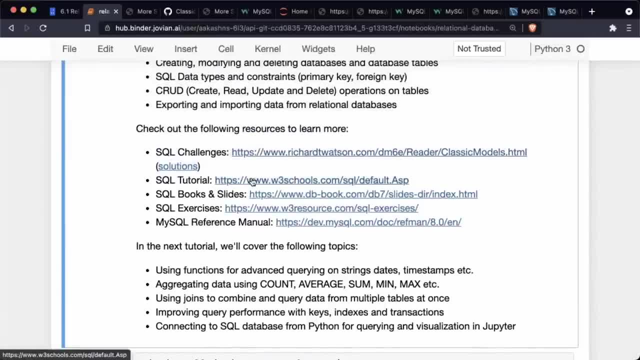 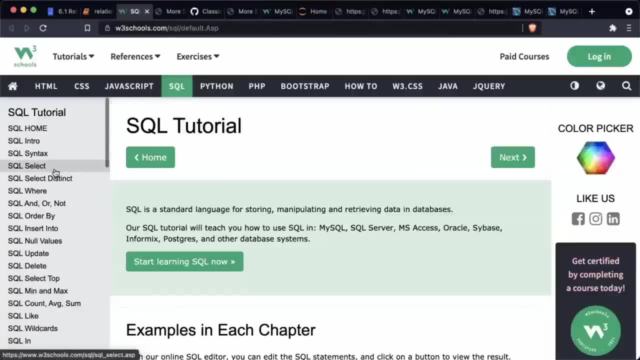 One is the SQL challenges, for sure. Then the other one is the w three schools reference. It's a great guide to just quickly look through all the different SQL, all the different SQL commands and all the different SQL statements and keywords That are present. 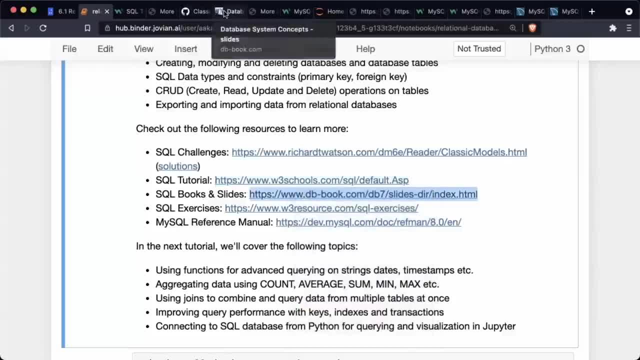 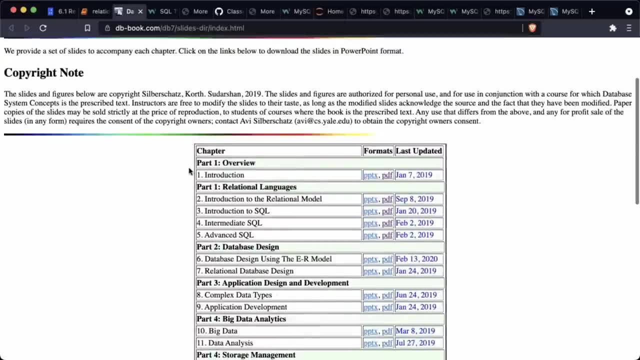 Then there is this book called db bookcom. So this is db hyphen bookcom. It's called database systems concepts. you can get this book if you wish. it's a great book, but you should also check out these slides. So they have made the slides available for free online. 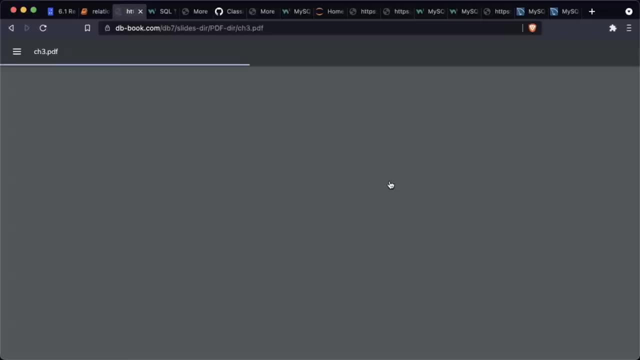 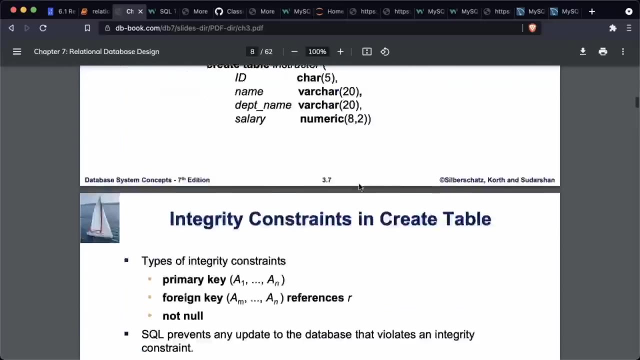 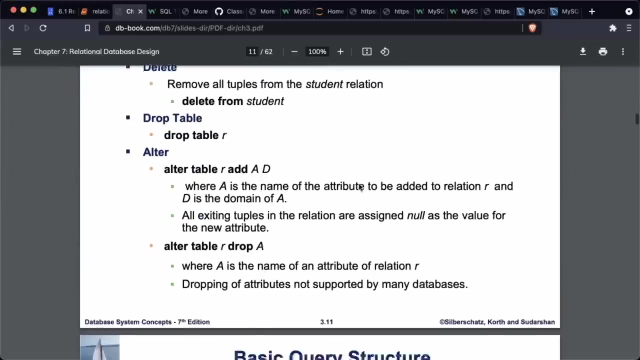 And these slides are a great comprehensive introduction to SQL and relational databases and pretty much everything to do with relational databases. So you can use These slides just whenever, let's say, you're preparing for interviews or if you want to get a deeper theoretical understanding of how the whole thing. 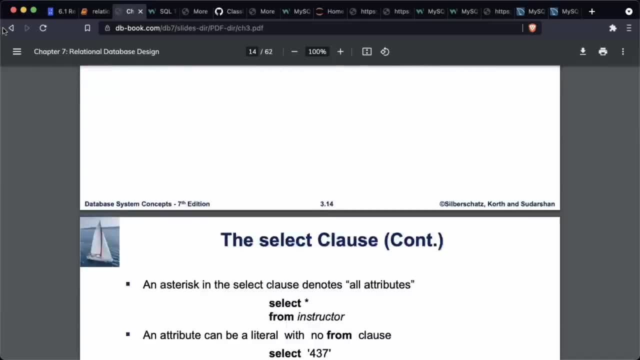 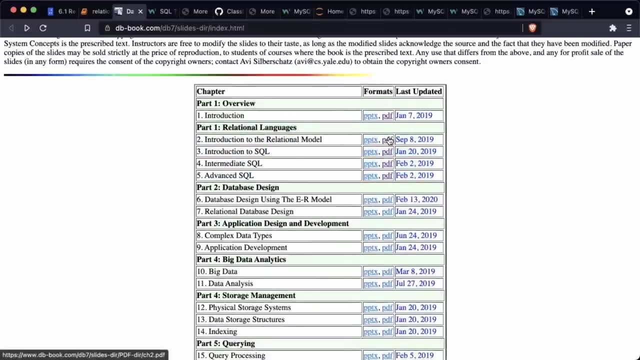 works. do check out these slides. I think you'll find them useful. Now you just need to look at part one, relational languages, where we talk about relational models, introduction to SQL intermediate, SQL advanced. SQL advanced is already beyond what you will need to know. 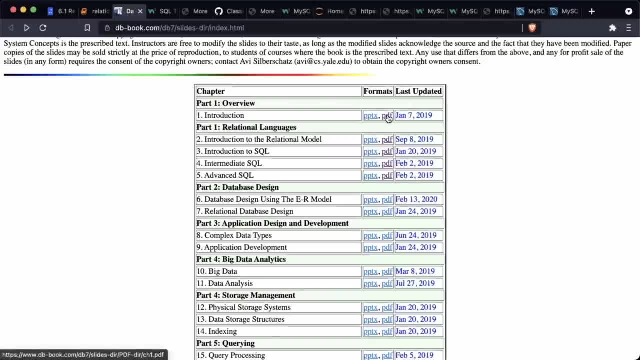 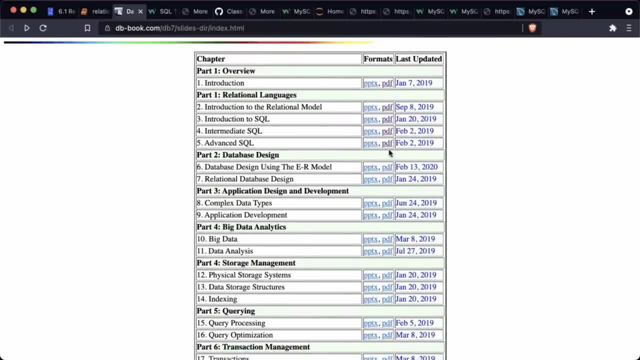 But if you cover these four or five slide decks and maybe also the introduction, uh, then you will pretty much master SQL. At least you'll know everything there is to know. Then you'll just need to practice. Then you also have these slides on database design, which is about the 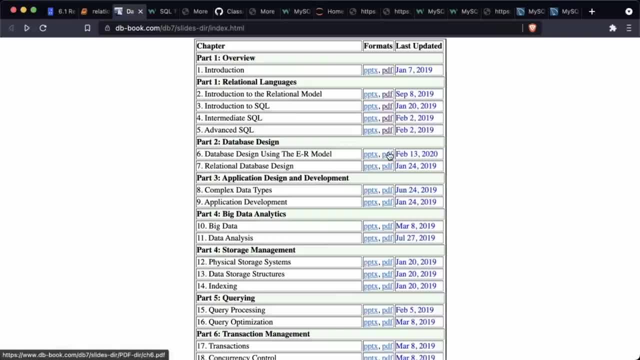 end uh. entity relationship diagrams and models. You don't need to know this as a data science practitioner. Generally, somebody else is going to do the database design, but if you want to interpret entity relationship diagrams correctly, then you should check this out. 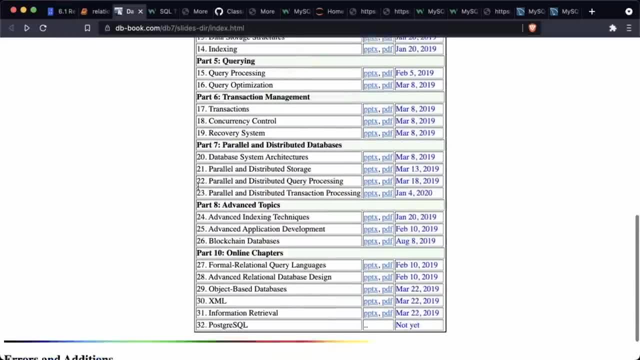 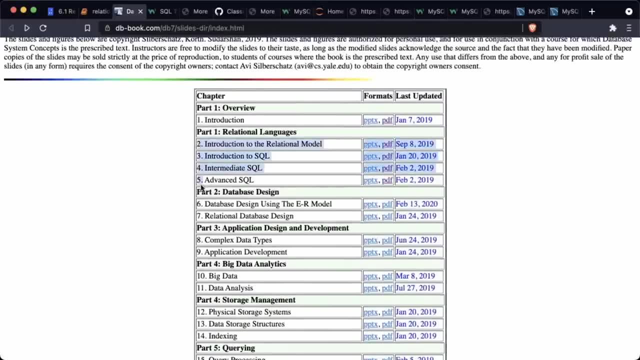 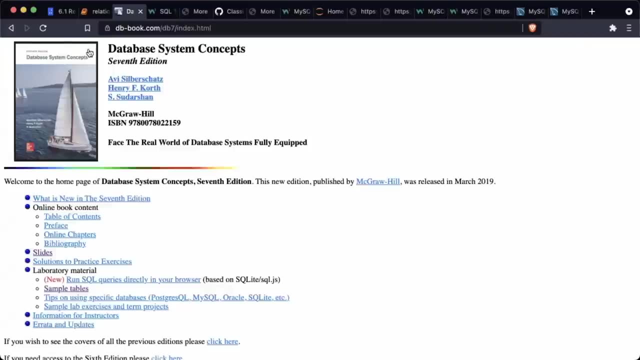 This might be useful for you. The rest of it is not really that Important, not something that is relevant here. It goes into the internals of databases. but definitely check out chapters two to five of dbbookcom. So you want to go to db-bookcom, go to the seventh edition and click on slides. 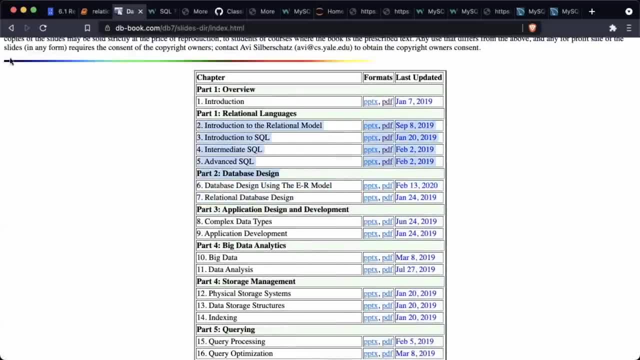 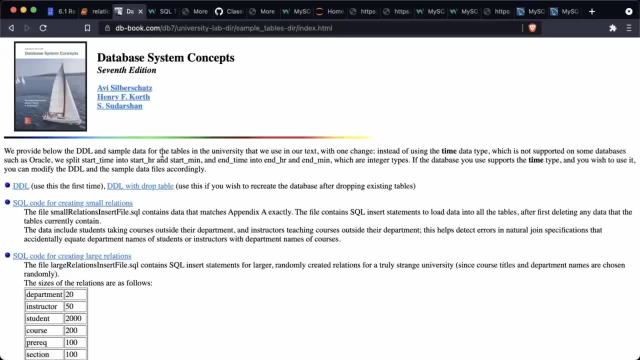 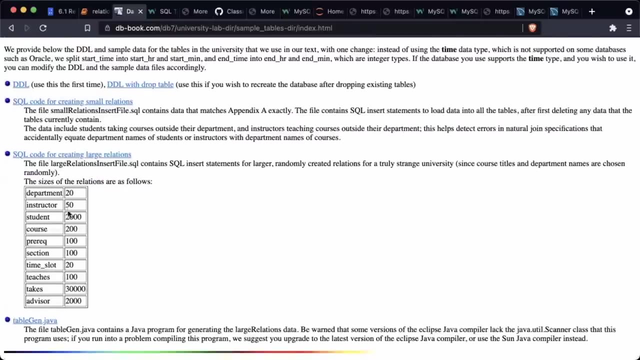 And here you have all these slides that you can access here. They also have some sample tables. just like we had this SQL file for CREA, Creating the classic models data set, Similarly you have sample tables for creating this university data set. 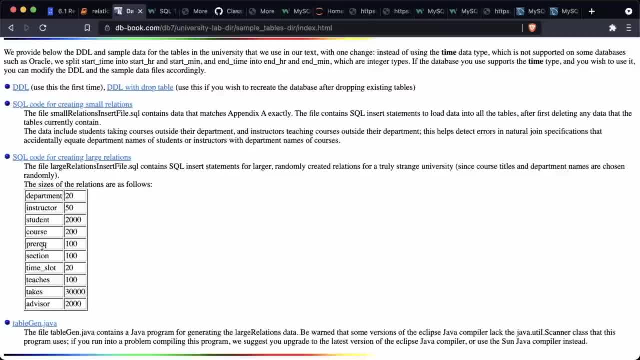 So where you have departments and instructors and students and courses and prerequisites, and students take courses and instructors teach courses, And then each course is taught in a section with a certain time slot, And then instructors are also advisors for students. So it's an interesting data set. 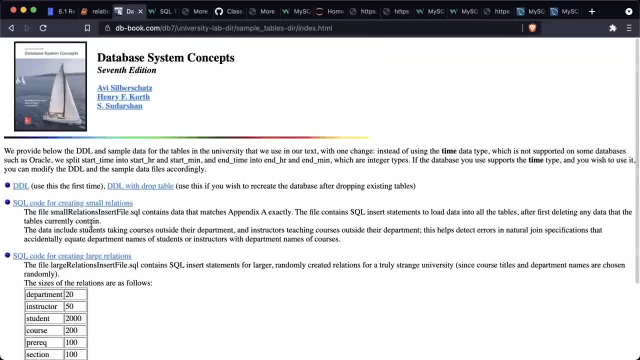 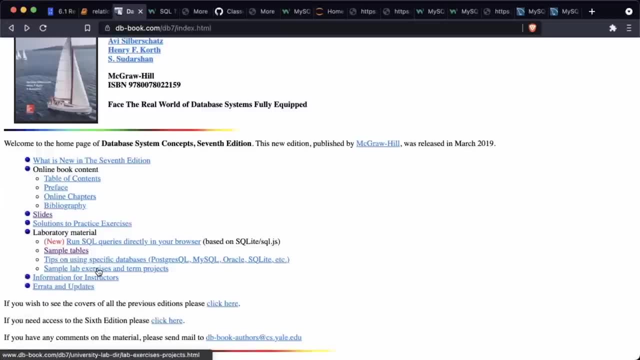 It has about 2000 rows of data And then there are a bunch of questions that You can try and answer on this data set as well. I think they're mentioned somewhere here in the exercises. So you see there are some exercises here on accessing the database, basic SQL. 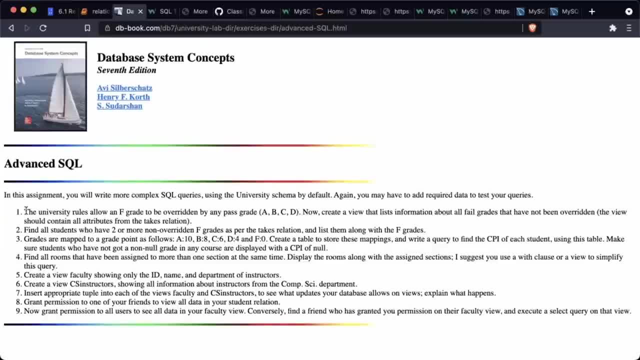 intermediate SQL, advanced SQL, Yeah, So here, so there's a SQL- is all about exercising, all about trying out these exercises. So, dude, maybe we'll try and put all of this together into a single notebook and we will also see. we'll also find. 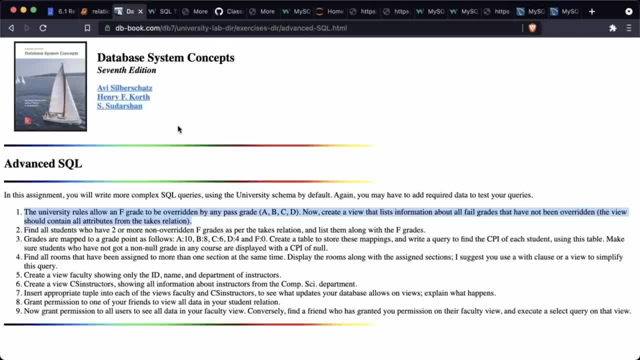 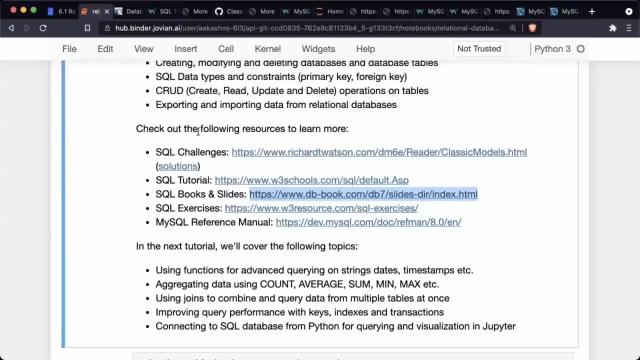 a way To do it so that you can type all the code in Jupiter and get the results immediately. In fact, Jupiter just like Python. there is a way to type SQL directly into Jupiter and interact directly with the database. So we'll try and set that up for the assignment. but in the meantime do check out dbbookcom. 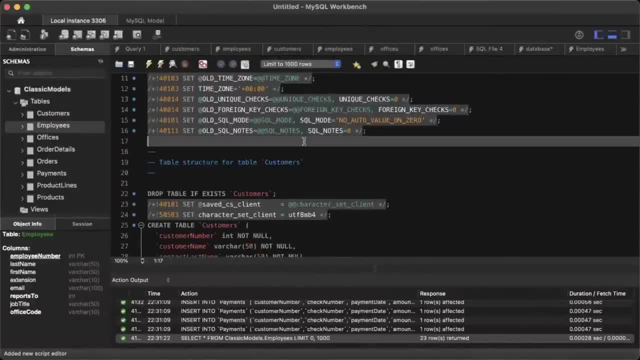 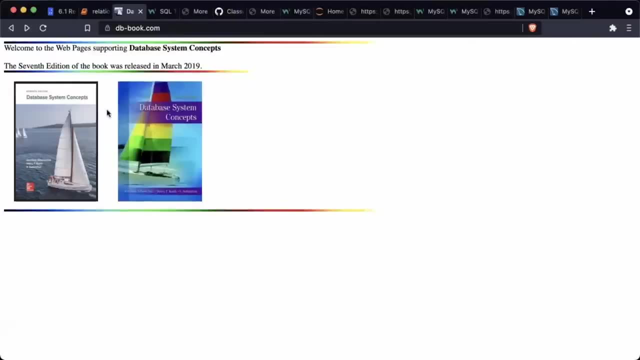 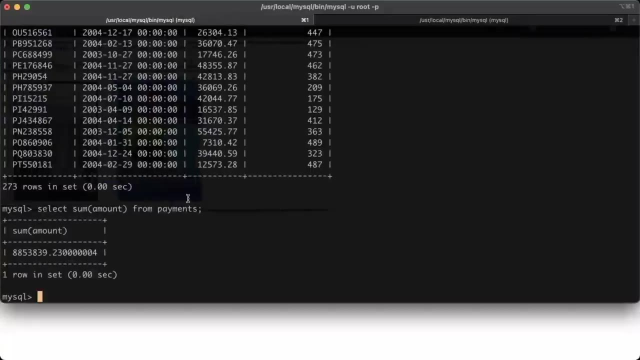 You also want to get familiar with the work bench or whatever tool your company is going to use. So don't lean too much on Jupiter for this particular course especially, and SQL in particular. become used to this Work bench, become used to working with the command line and typing commands there, because that is how you will be. 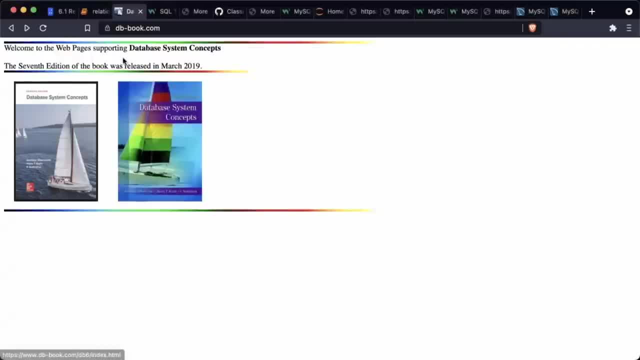 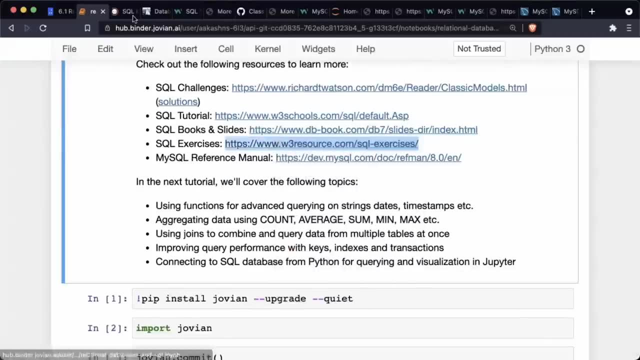 working with SQL databases in the real world. Okay, And we will touch on how to access them using Python. to more SQL exercises on w3resourcecom You have more exercises, hundreds of exercises really, And that's all. SQL is about exercises and more. 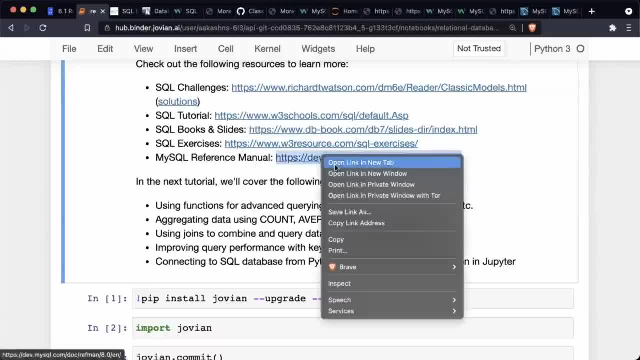 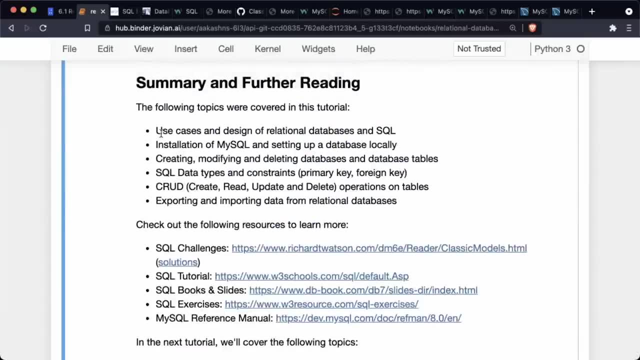 And if you really want to read through my SQL reference manual, then you can check that as well, although you would all Most never need to do that. And that's it. So we've just covered the use cases and the design of relational databases and SQL. 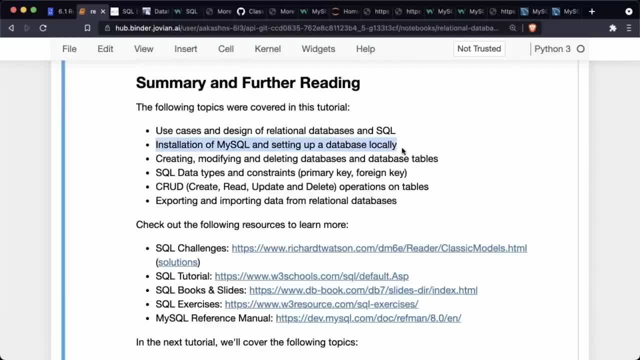 We've looked into the installation of my SQL and how to set up a database locally. We looked at creating, modifying and deleting databases and database tables. We looked at SQL data types and constraints like primary key and foreign key. We looked at the create, read, update and delete operations on database tables and we looked at exporting and importing data. 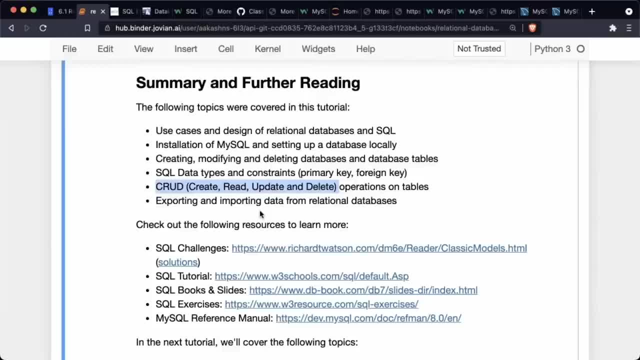 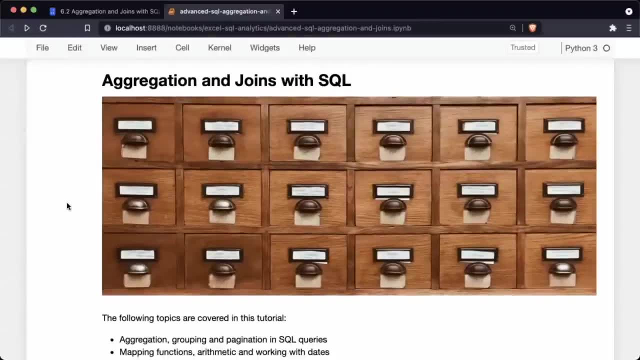 Okay, From relational databases, The topic for today's aggregation and joins with SQL. Last time we looked at some basic SQL commands, or we saw how to create databases, We saw how to create tables, We saw how to put data into tables, how to get data out of tables, all the crowd operations, which is create, read, update and delete. 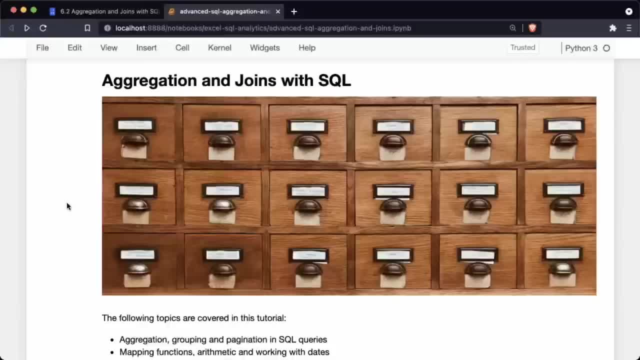 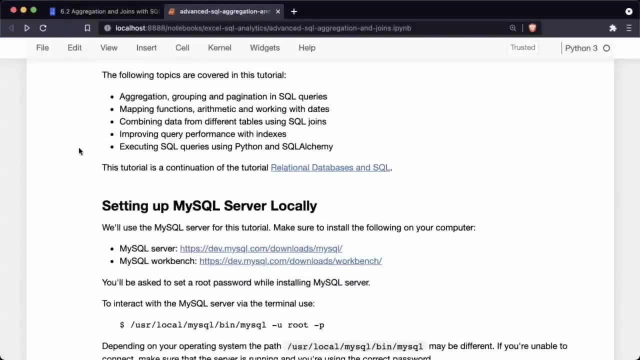 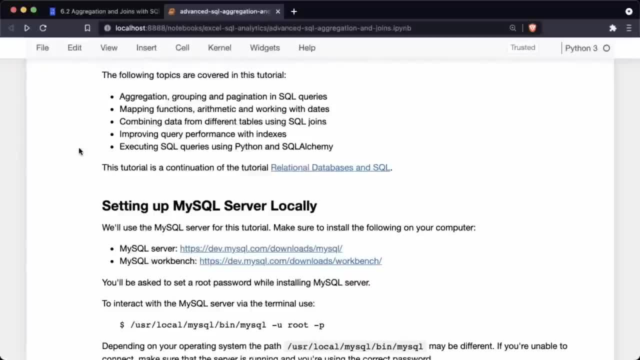 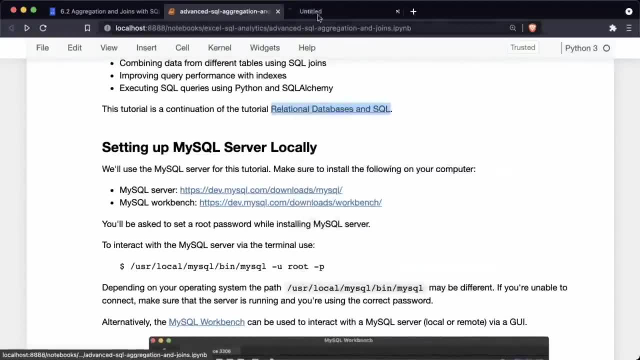 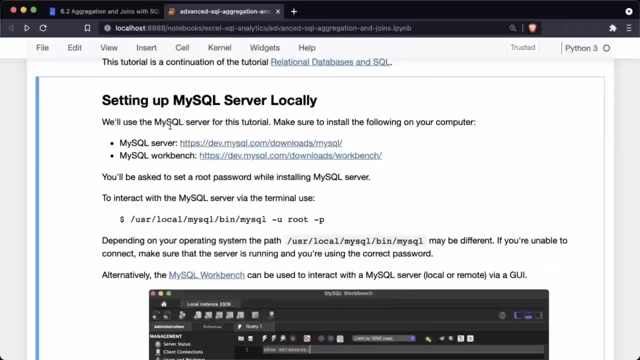 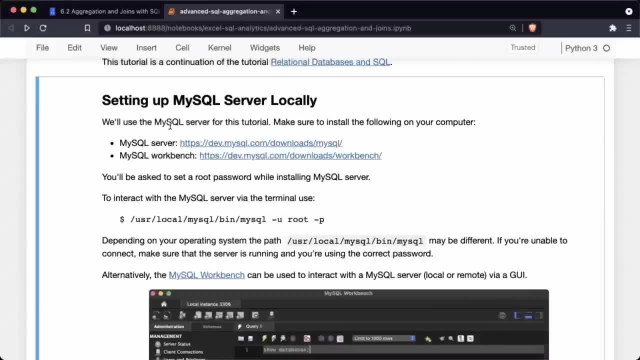 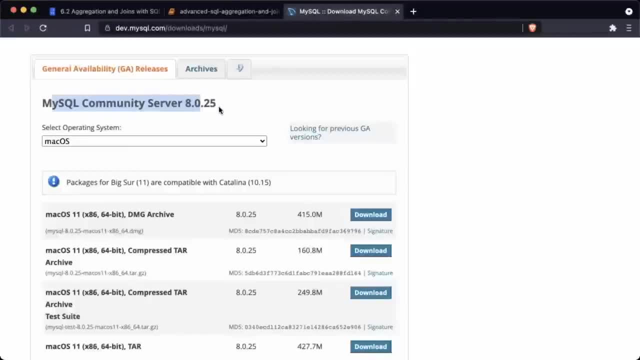 a program which runs in the background and listens for instructions. So the my SQL server is something that you can download from dev dot my sqlcom. this is just a package that you download to your computer and then you install it on your computer. 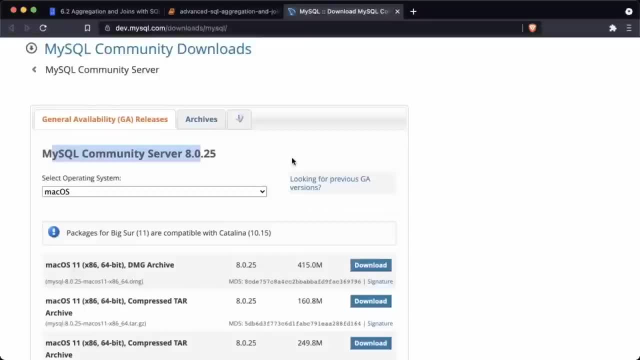 And once you install it on your computer, You can start up a database server on your computer so that software is running now in the background and you can then issue instructions or send instructions to the database server in the form of SQL queries, like creating databases, creating tables, putting data in, taking data out, et cetera. 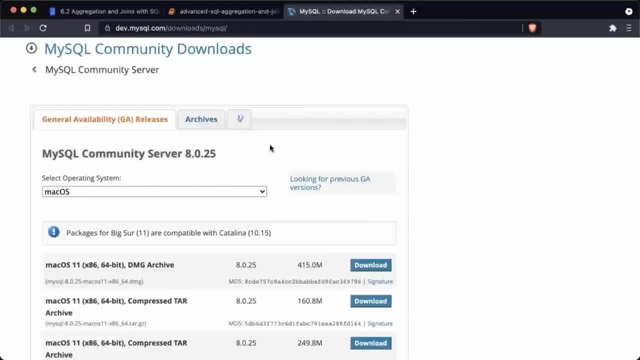 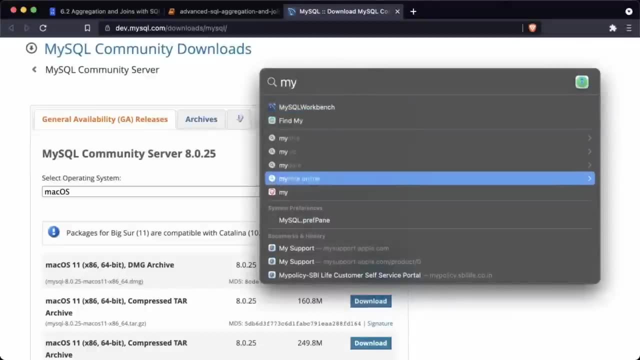 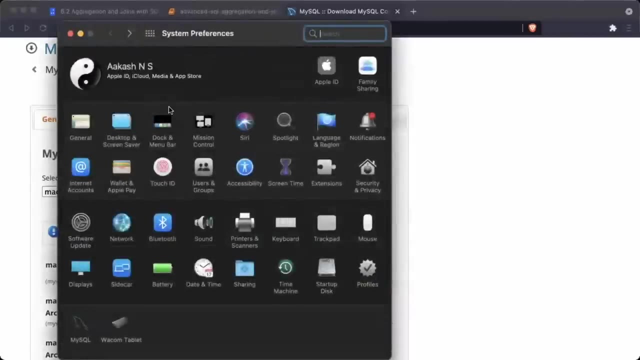 Now, depending on your operating system, the way to start and stop this server is going to be different. in my case, What my SQL does is When I installed my SQL community server. it adds a system preferences pain. So inside my system preferences this is the max system preferences. 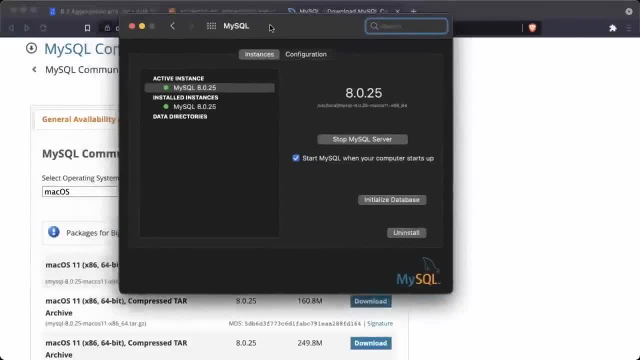 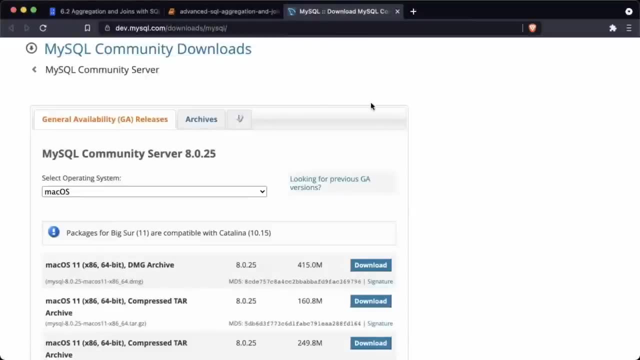 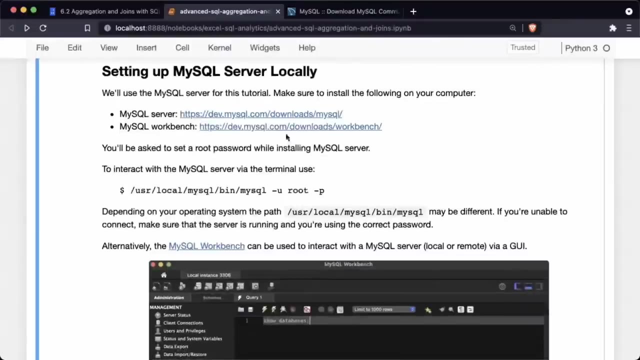 There is a my SQL page that gets added, but in your case this could be different. So make sure that you have downloaded my SQL server, the software, and then it is running on your computer And then anytime you have a server running, you need a way to connect to that database server. 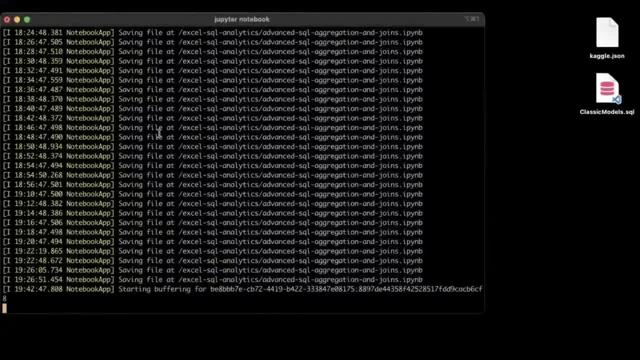 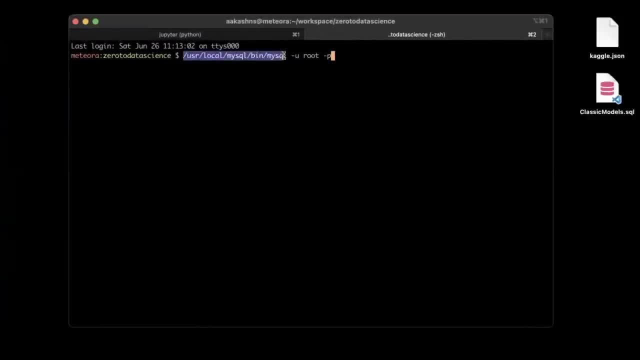 So there are multiple ways to connect to a database server. One of them is to use the my SQL command line, which is typically installed at some kind of a location like this: slash, user, slash, local, slash, my SQL. This is, on Mac again, the my SQL command line tool based on your operating. 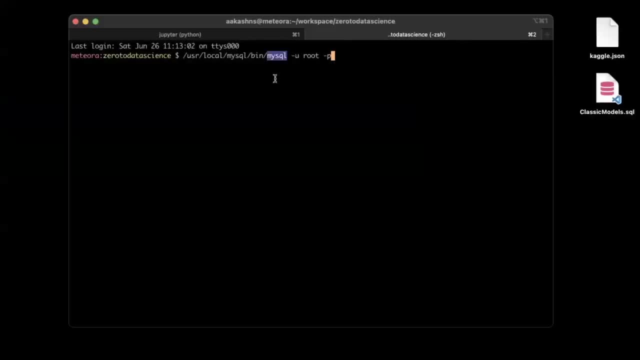 system will be at a different location. So check out the documentation or search online on where you can find the my SQL command line tool once the community server is installed. So one way you can connect to the server and issue commercial server is by running the my SQL command line and here you specify that you want to log in as the user root. 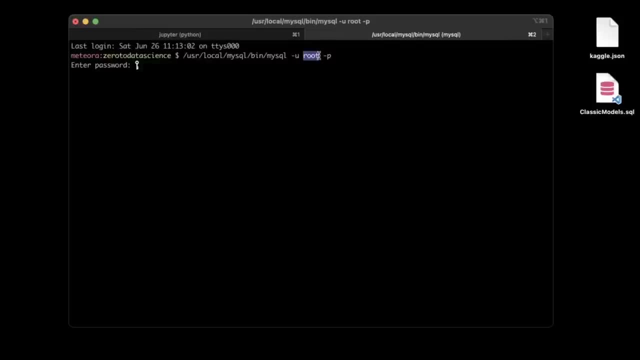 So when you install the server, you're asked to set up a password for the database server and a username. So the default username is root and you have to set a password. So in my case I have set up a certain password and now I am connected to the server. 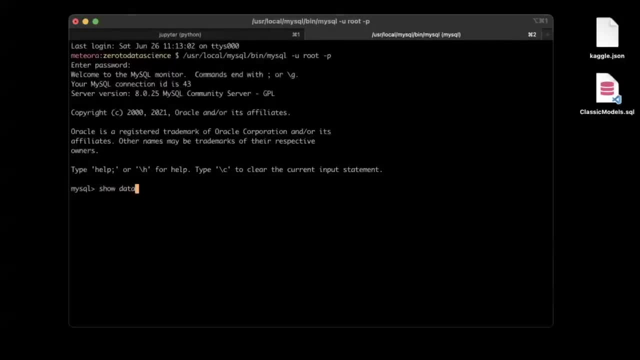 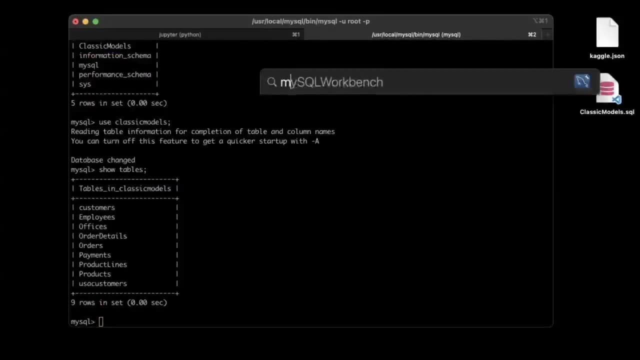 And now I can issue commands to the server. For example, I can say: show databases, And that's going to show me the databases I have. but what we're going to do is use this software called the my SQL work bench. So this is the second piece of software you'll have to install. 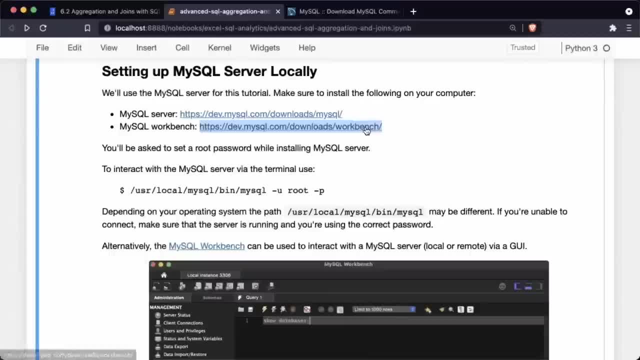 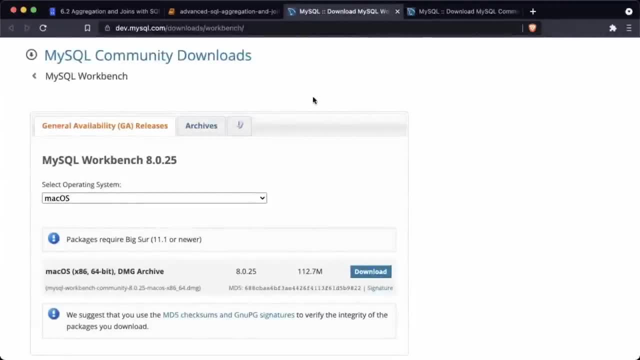 And I have given you a link here: dev dot my sqlcom slash download, slash work bench. So go to this page and download the my SQL work bench for your computer, for your laptop, for your operating system, and then open it up. 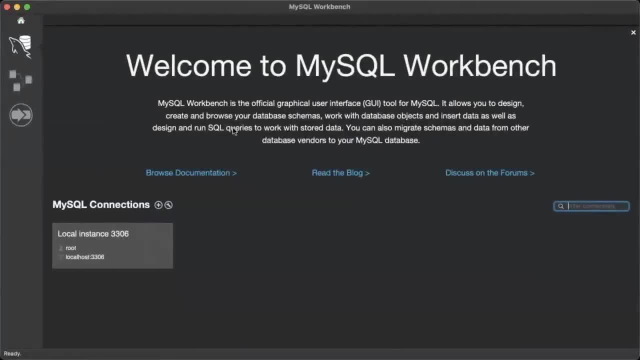 So now we have a server that's running On a computer And then we have this work bench, which can connect to a server and gives you a graphical user interface to connect to that server. So one way you can connect to your servers: click plus, and here you can then provide. 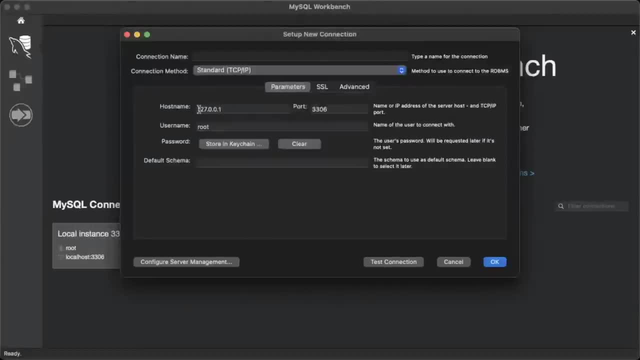 This is a connection name that you can set, but you have to provide some parameters. by default This is set to connect to a local machine, a local database server on your computer. But again, if you have a database server that is somewhere on the cloud, you can. 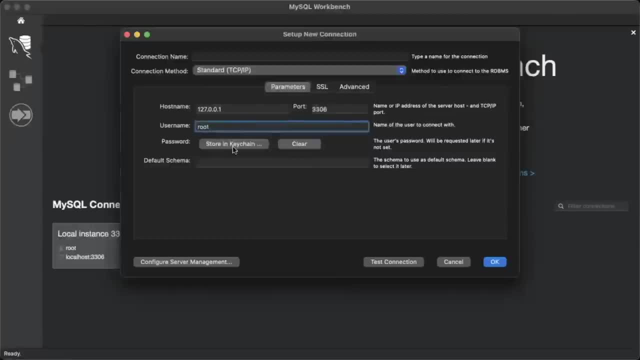 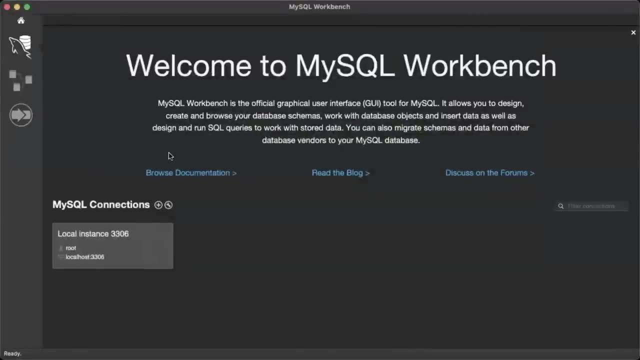 simply ask for the host name, port, username, password and then you can connect to that server as well. So my SQL workbench does not just collect, connect to your local database, It can connect to any database on the cloud If you have the credentials, and when you join a company they will give you the credentials to the server. 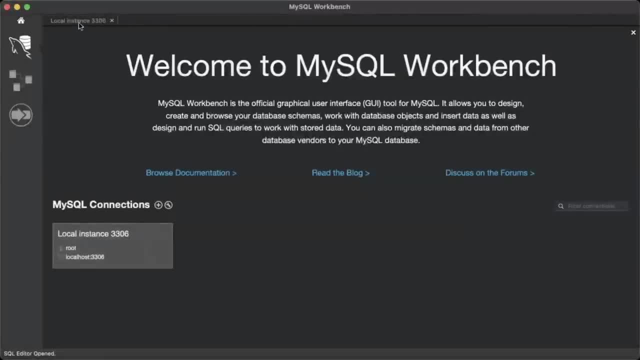 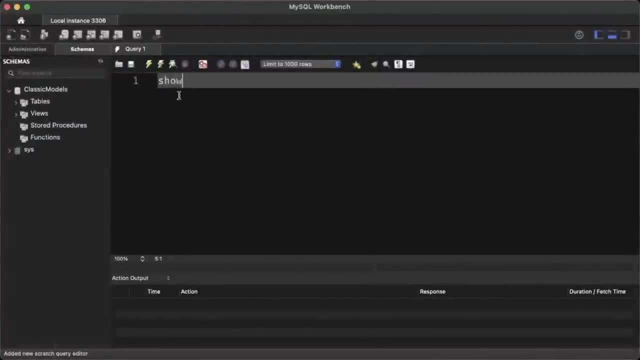 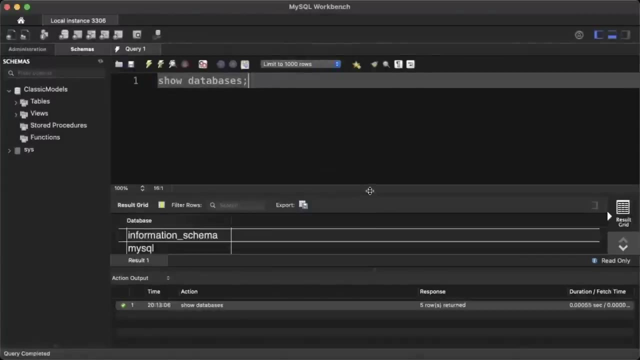 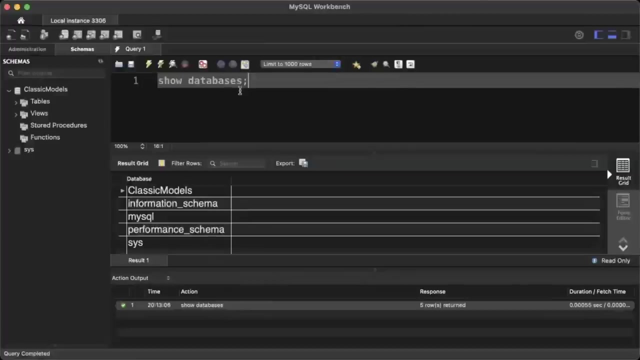 In my case, I already had the local instance set up here, So I just clicked on it and now I'm connected to my local instance. For example, if I just type Show databases, that's going to show me the databases that I have here, which is classic models, information schema, my SQL and performance schema, and then I can run use database and all my select queries. 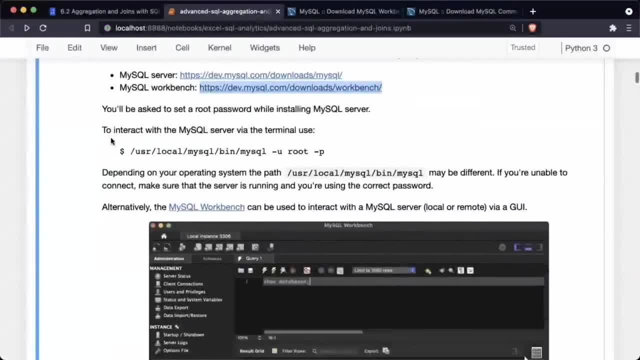 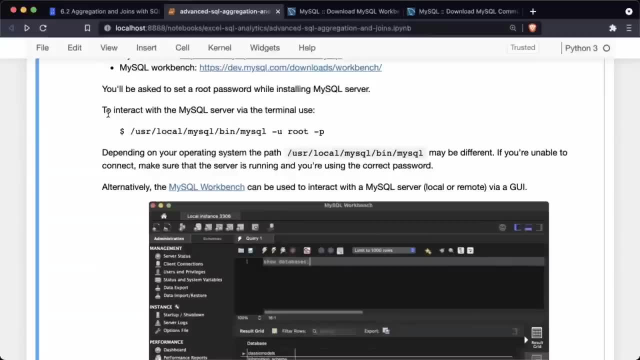 Okay, So that's the setup you need to do, That's the software you need to have installed and let us know if you face issues. Um, and I hope the server and the workbench- uh, separation is clear to you. So here's the my SQL workbench. 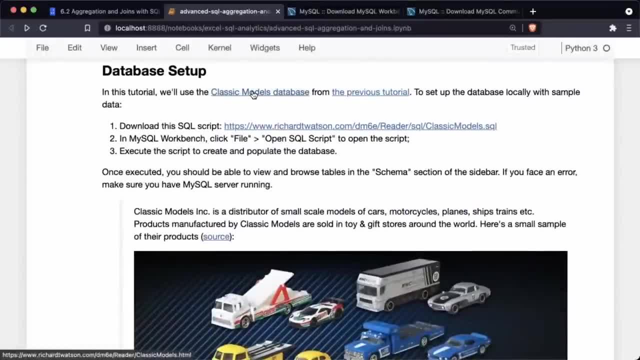 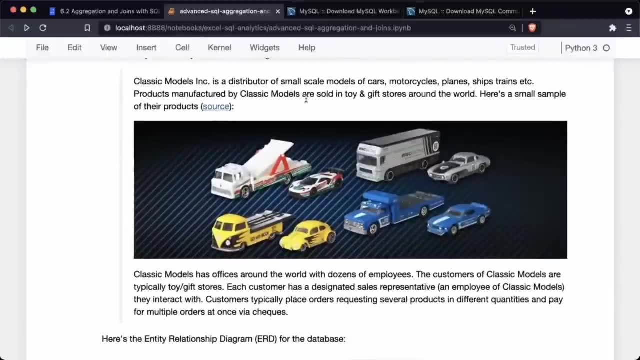 We have that running and in this tutorial we will use the classic models database from the previous tutorial. So classic models is a hypothetical company. It's a distributor of small scale models of cars, motorcycles, planes, ships, trains, et cetera. 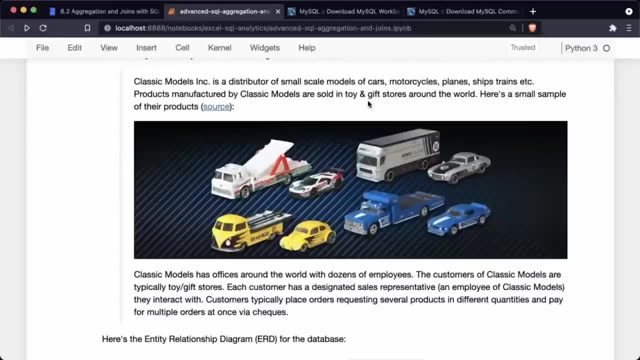 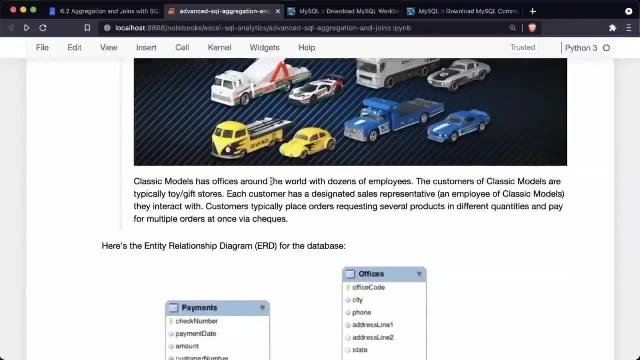 And the products that are manufactured by classic models are sold in toy and gift stores around the world. So here are some of the products they sell, and classic models has offices around the world with dozens of employees, And the customers of classic models are typically toy or gift stores. 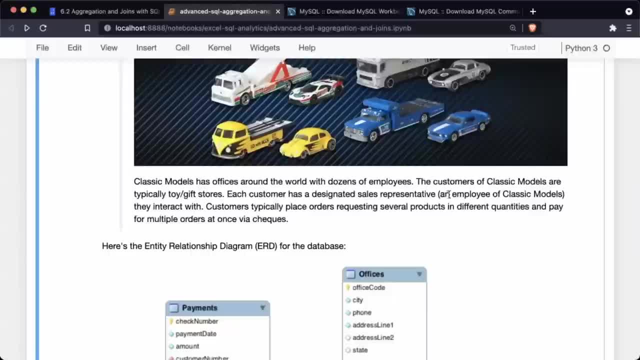 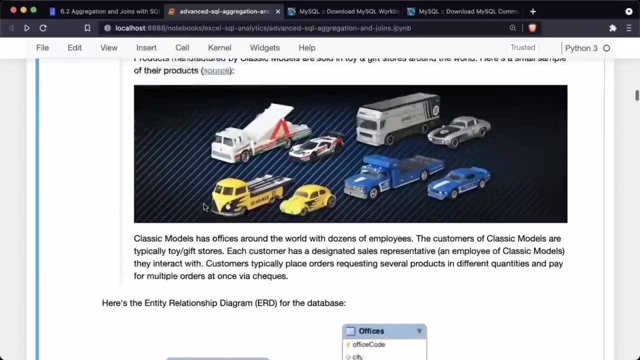 So each customer has a designated sales representative who is an employee of classic models that they interact with. Now, customers typically place orders requesting several products in different quantities, and then they pay for multiple orders at once via checks. All right, So that's the setup here. 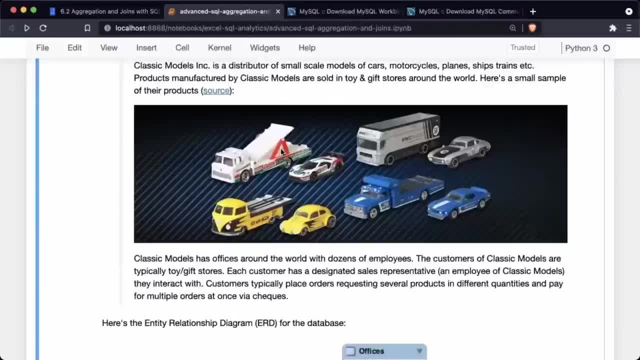 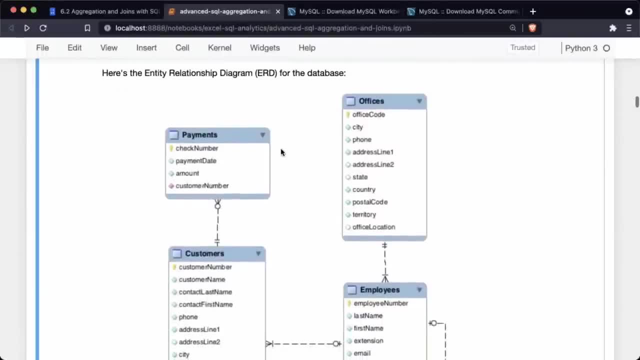 We have this company, this hypothetical company, which does all of these activities, and we want to track all their activities in Relational And to do that, an entity relationship diagram has been given to us and this simply tells us what the different entities are, what the different tables in the database are and what the different columns within those tables are. 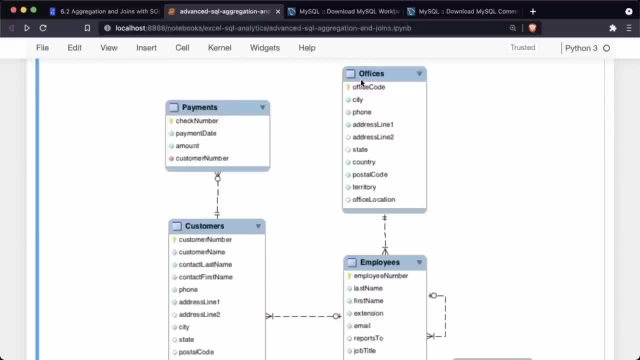 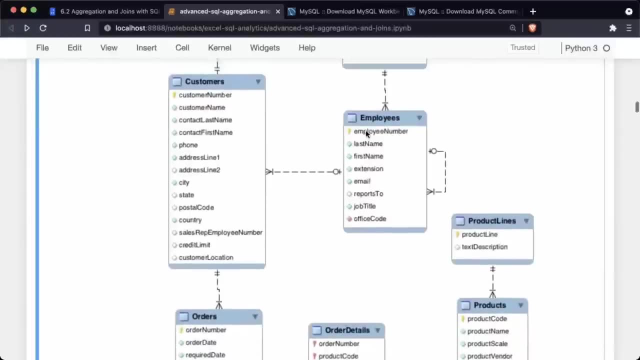 So we have an offices table here. It contains information about different offices. The primary key is office code, which is the unique identifier. Then we have the employees table, So we have an employee number, last name, first name, extension, email, et cetera. 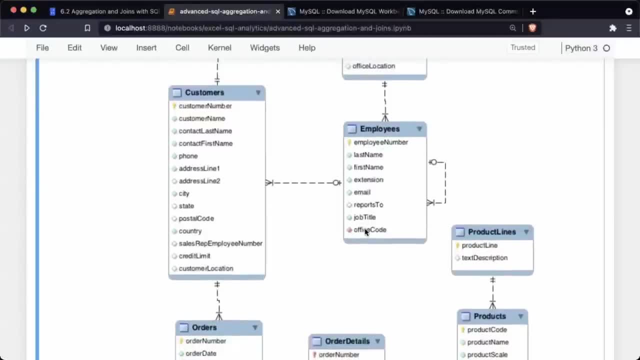 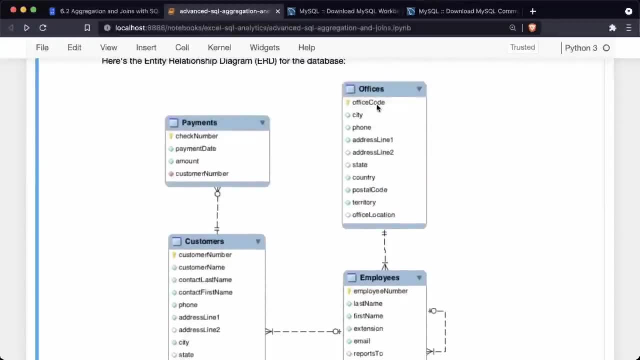 And there are a couple of relationships here. Okay, There is an office code in employees. So for every employee there is an office code which is the office code of a certain office. So this is called a foreign key, because an employee cannot have an office code, which is invalid. 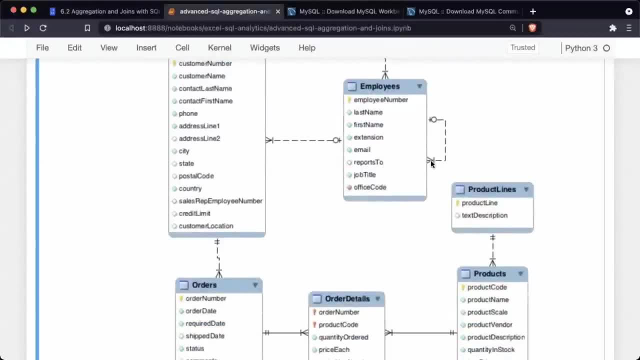 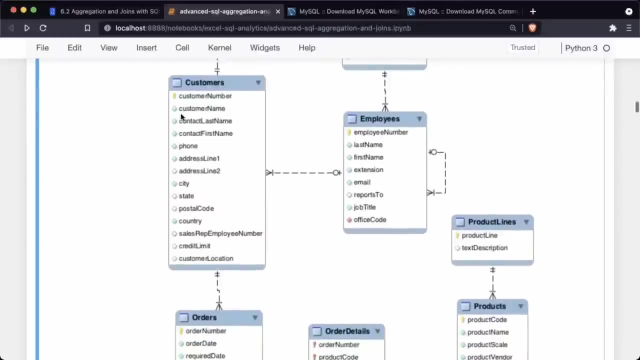 And then you also have reports to. so reports to tells you which employee and employee reports to. So this is a foreign key from the employee table to itself, right? So Reports to must be a valid employee number of another employee. Then you have customers and you have a bunch of information about customers. 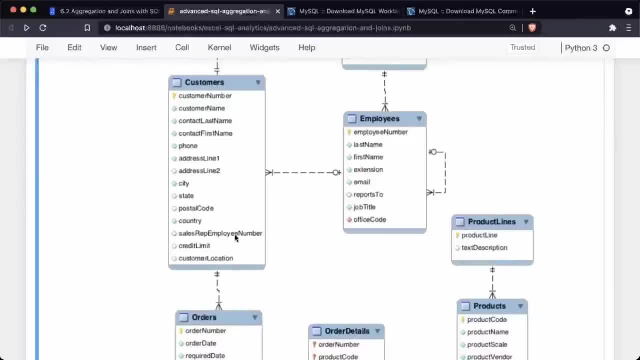 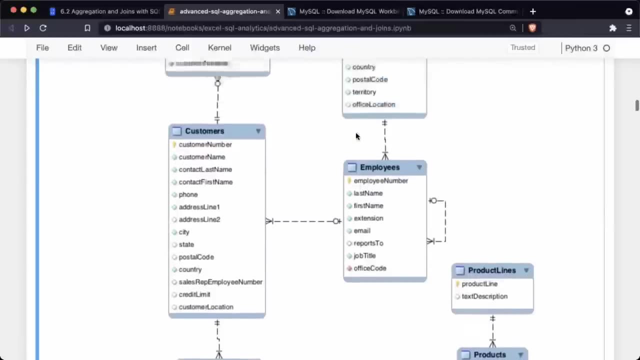 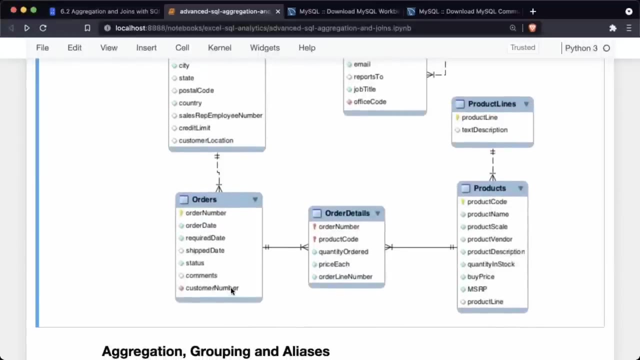 Customer number is the primary key and every customer has a sales rep employee number, which is the employee number of a certain employee Who's a sales rep, And then for customers, customers can place orders, So every order is placed by a customer. 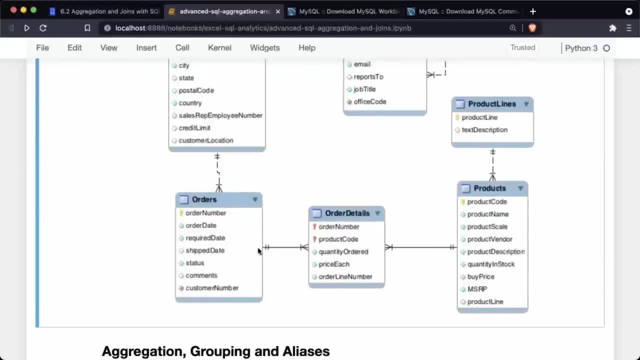 That's why you have a customer number, foreign key here. But apart from that, Orders can have a lot of items, So there is an order details table for each item, each line item in the order. Let's say you've ordered five products. 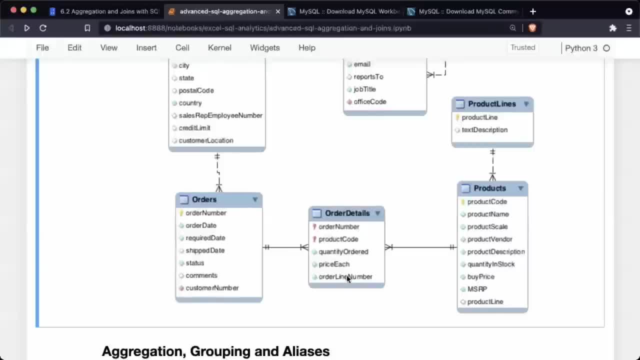 You have five line items and you can have the quantity, et cetera, of each one, And then you have products as well. So there's a table of products and there's a table of product lines, because you need to track information about the product somewhere as well. 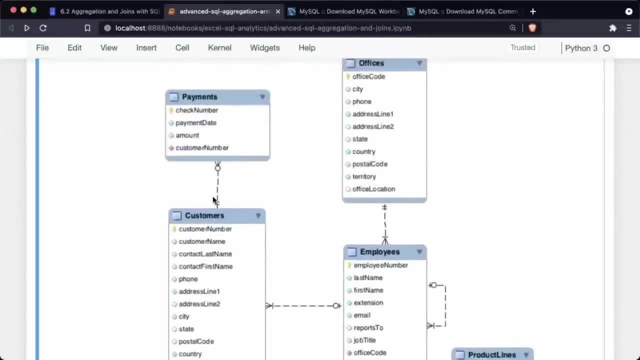 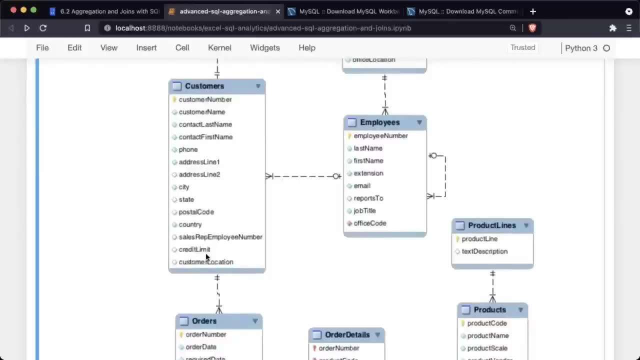 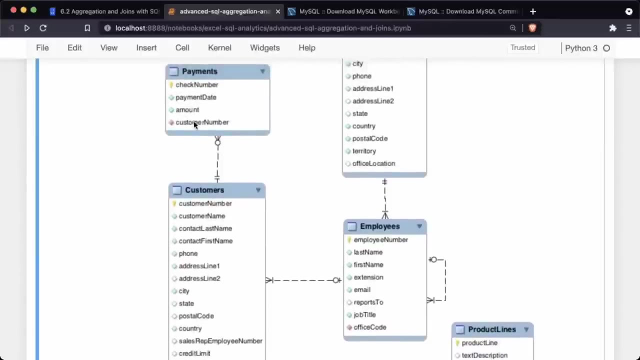 Finally, you have payments. customer main customers make payments at separate times, So this is a slightly different flow, where you don't pay per order, but customers have a credit limit, which means they can make place orders up to a certain amount and then they can clear all their pending payments at once using a check. 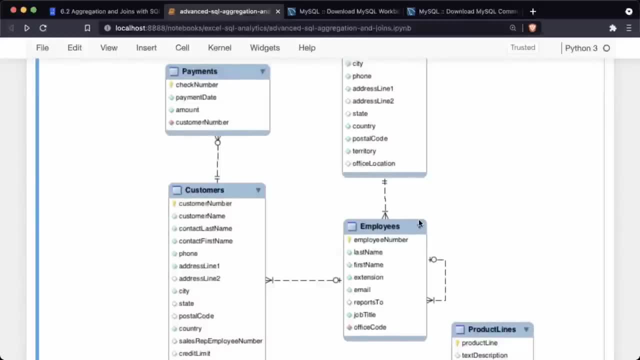 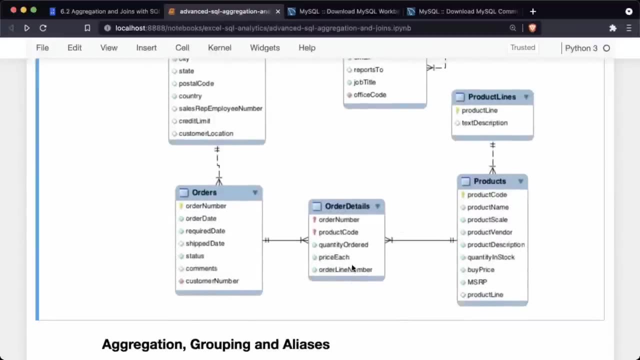 So that's the setup they have here And depending on how your company operates, this system may be different. It's possible that if you take payments upfront, then maybe the order details is connected to payments or the order is connected to a payment rather than a customer. 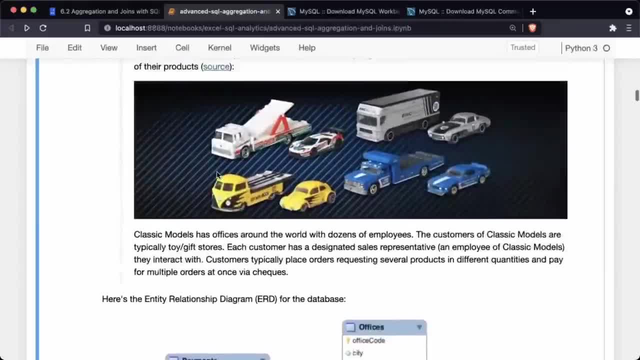 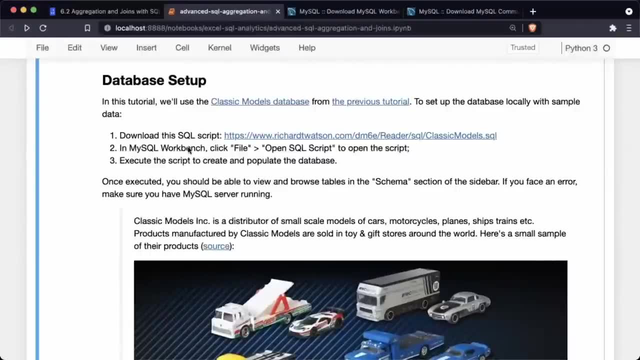 Okay, So that's the entity relationship diagram here And that's the sort of the overview of the database that we're working with Now we will use. we will set up this database locally with some sample data using a script, So let me just set that up and then we will take some questions. 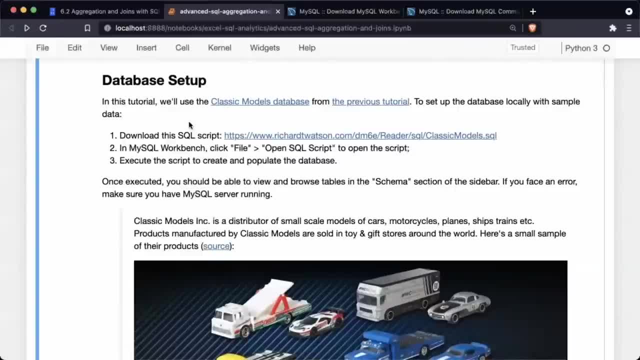 And, by the way, if you have any questions, please post them in the zoom chat. So to set up this database, we first need to download the SQL script. So I'm just going to open this in a new tab And that's going to try and download it. 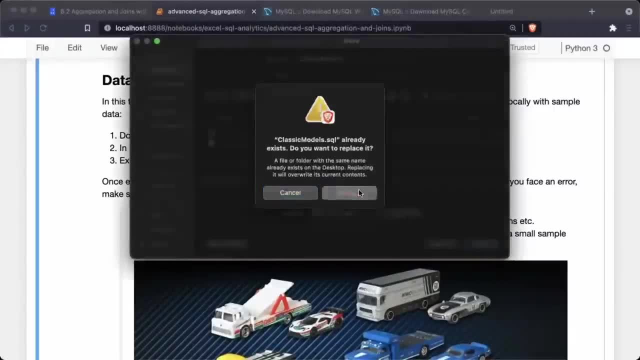 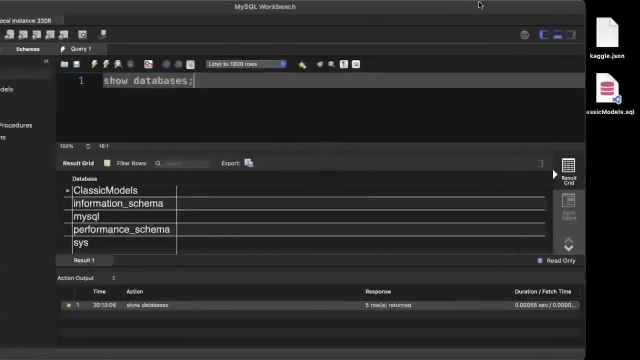 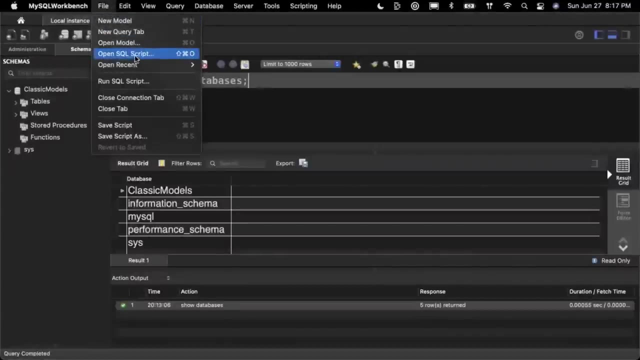 And I'm just going to download it on my desktop here And you can see that now the SQL script is downloaded on the on my desktop And then, once you have downloaded it, you can go to file, open SQL script in your my SQL workbench. 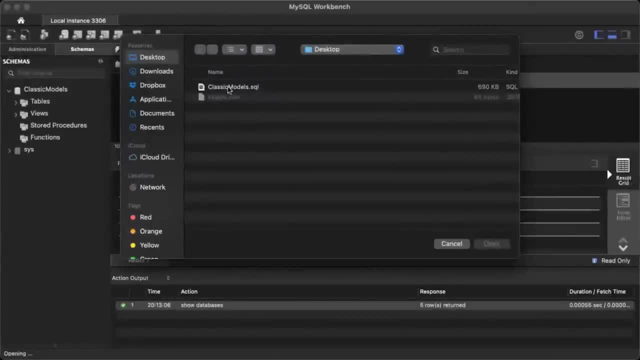 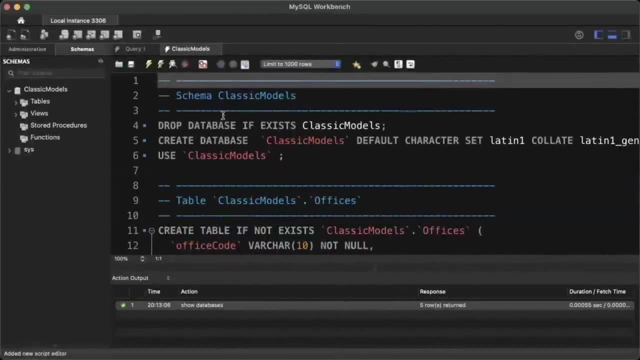 So open up my SQL workbench, connect to the local database and click on this open SQL script, And then here you can see the Contents of the SQL script. So this contains all the information to set up the database that we just saw. the ERD for the entity relationship. 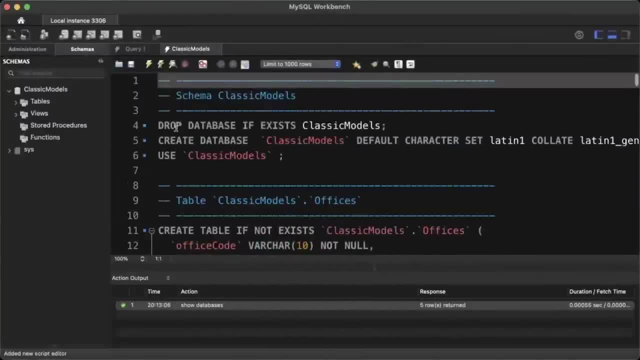 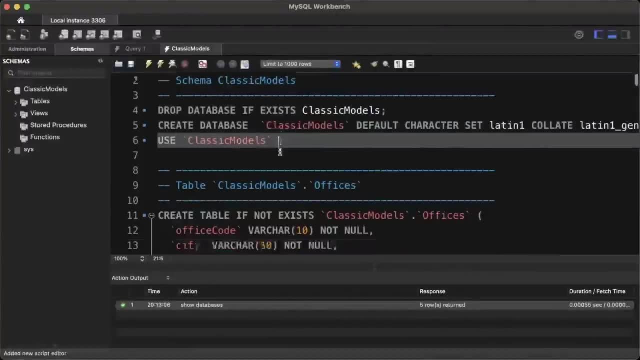 diagram for, and it also contains a lot of sample data. For example, it's going to drop the database classic models, If it exists. it's going to then create a new date, a database, and it's going to use that database. 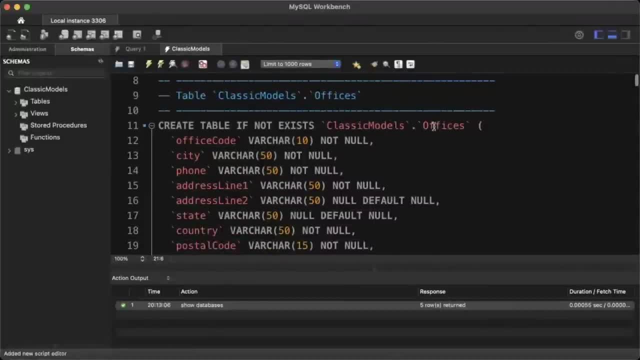 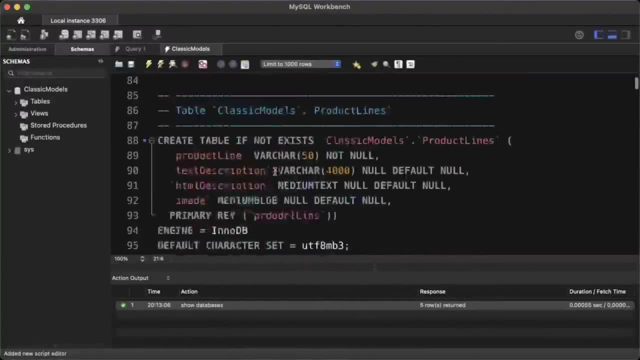 Then it's going to create tables one by one. For example, here it's creating the offices table with all this information, and then it is going to create employees, a customer. It's et cetera, et cetera. 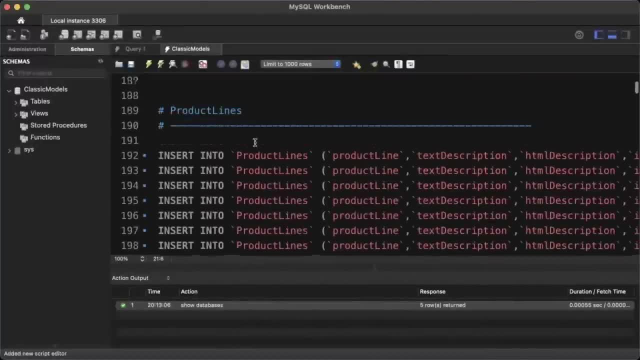 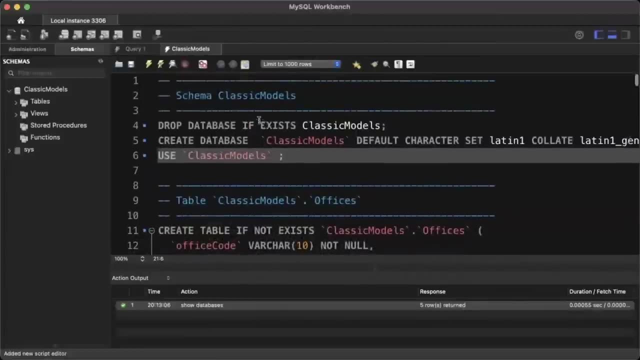 Once tables are created, it is going to insert data into these tables, like product lines, products, customers, employees, et cetera. Okay, So it's going to set up a database with a lot of information for us. Now, once you have this SQL script loaded up, you will see this run: SQL. 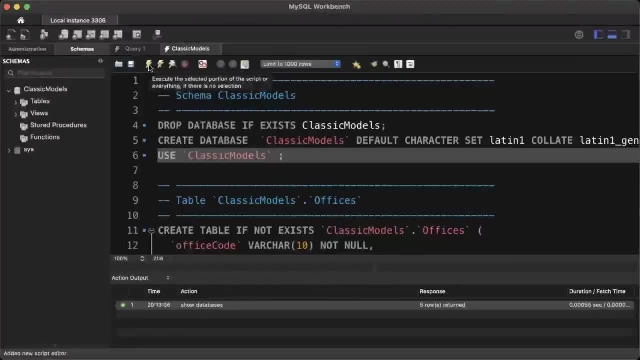 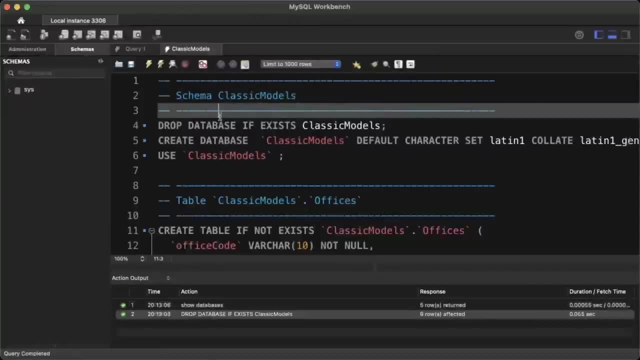 So execute button, which is like a lightening button here, So you can just run a, press that, or you can just press command enter or control enter on windows. So I'm just going to run command enter And now my previous classic models database has been removed and this new database has been set up. 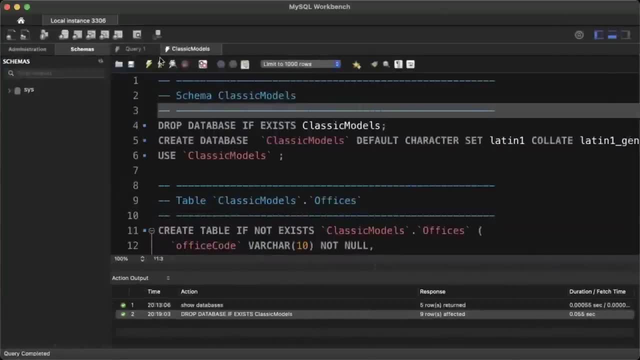 So if I go to the left sidebar, if your sidebar is not open, you can click here and open up the left sidebar and just go to the schemas tab in the left sidebar. I should be able to find a schema. Let me just connect again here. 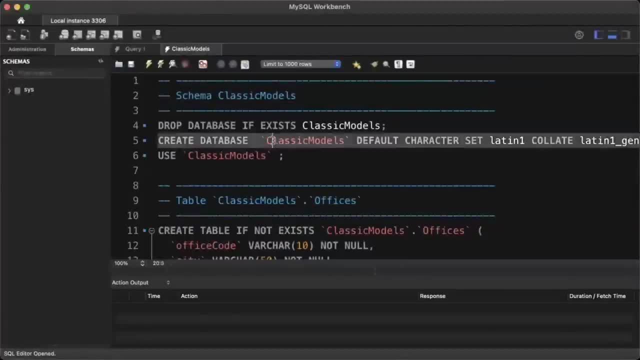 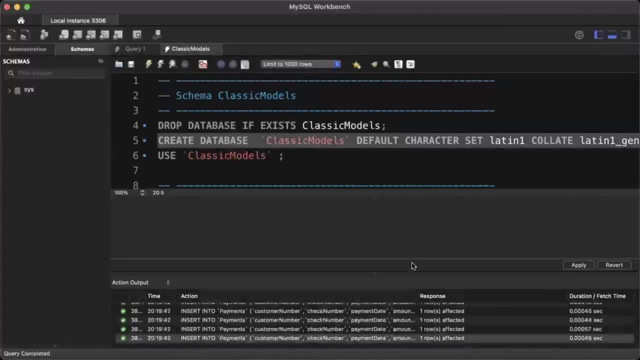 Okay, Let me just run that once again. Yup, All right. So now if I check the schemas here, so I should be able to find in the schemas, Once I reload the schemas, the classic models database. Now in the classic models database I can browse all the tables here. 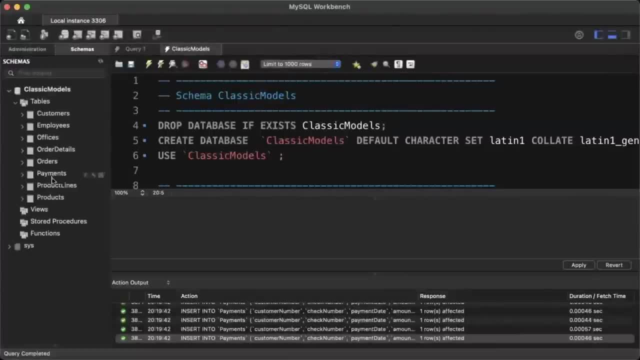 You can see that we have tables, customers, employees, offices, order details, payments, product lines, et cetera. And if you double click on a table or if you just click on this table, click on this button which shows: 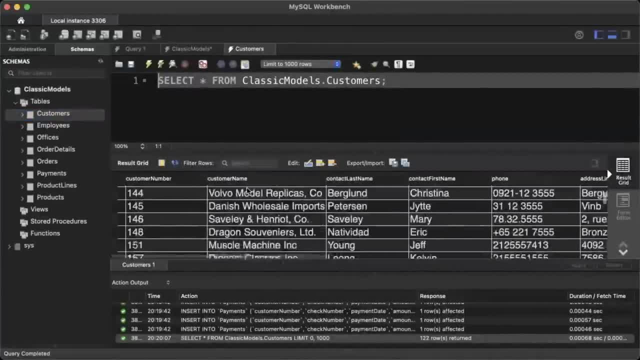 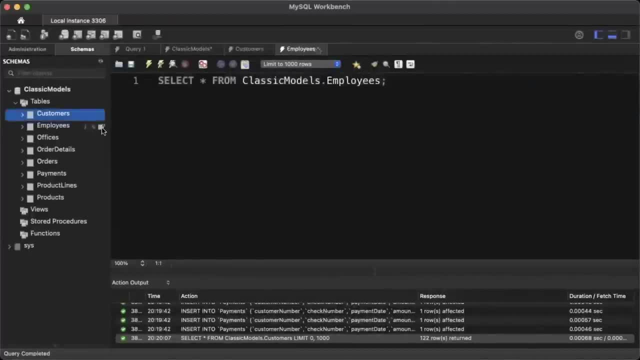 information from the table. then it is: you can view some information from each table, All right. So my SQL workbench gives you an easy way to browse the schema, see different tables and actually look at information from different tables very easily. 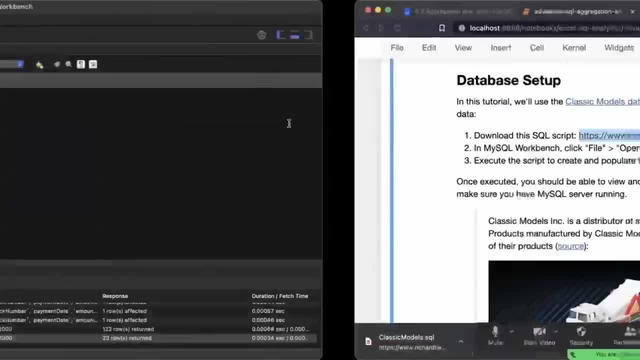 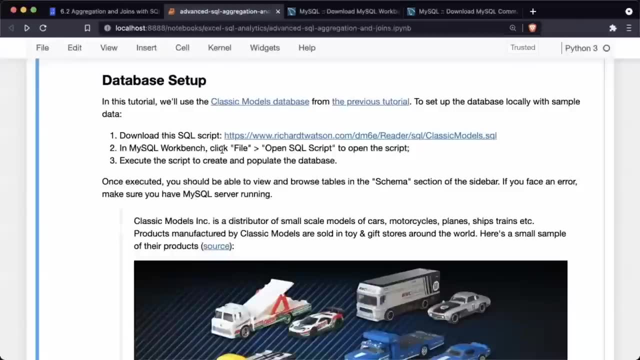 Okay, So now we have just to recap. we have downloaded the SQL script from this Yeah, And then we have loaded it into my SQL workbench using file open SQL script. Then we have executed the script to create and populate the database. 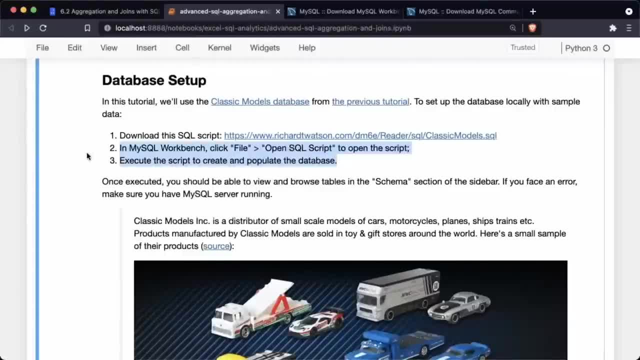 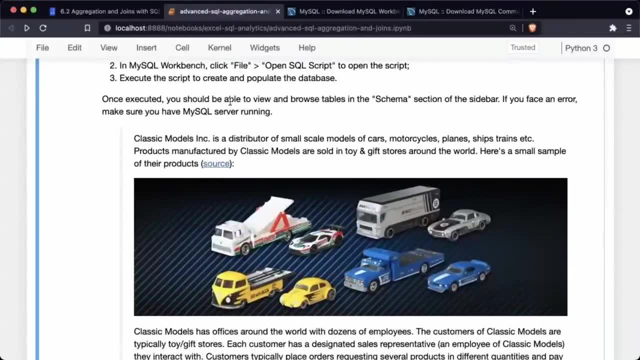 This part can also be done using the MySQL command line tool. It's simply a matter of passing the script to the command line tool, and you can look up how to do that. But once executed, you should be able to view and browse all the tables in the schema section of the sidebar. 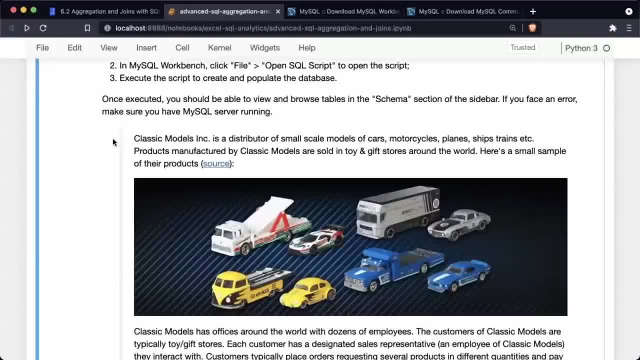 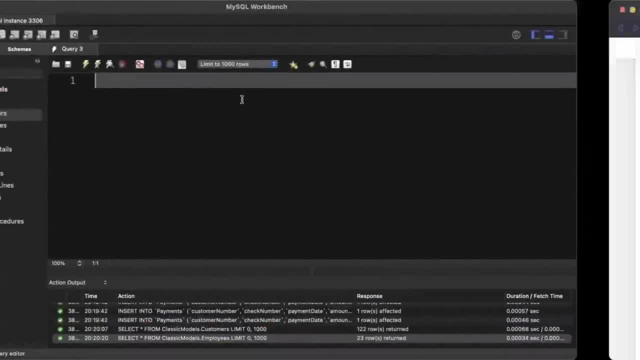 And if you face an error, the most Likely issue is that your MySQL server is not running. So just because you have workbench open does not mean the server is running. So make sure that the server is running and then you will be able to communicate with the database server. 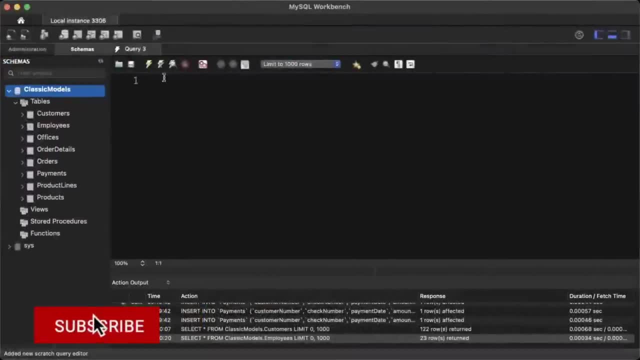 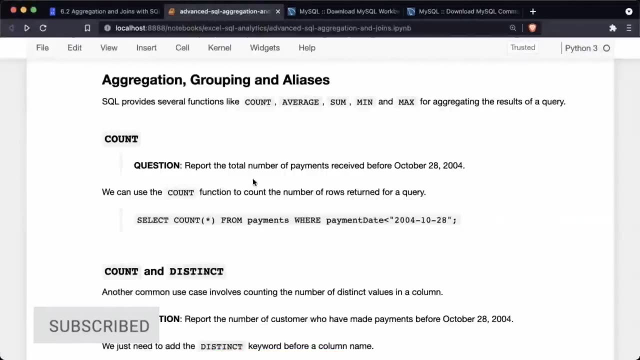 All right, So with that, we have our database set up. now you're ready to go and we have our MySQL workbench connected, So let's get started. The first topic we look at is aggregation, grouping and aliases, So let's get started. 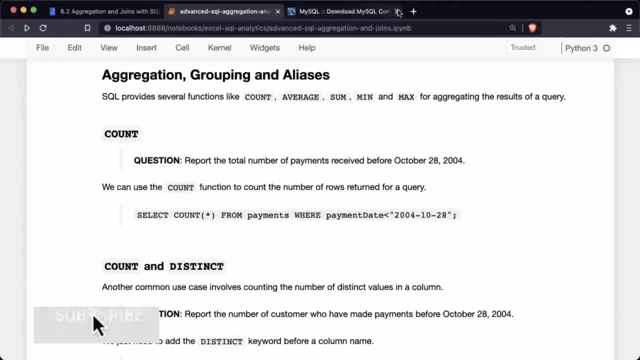 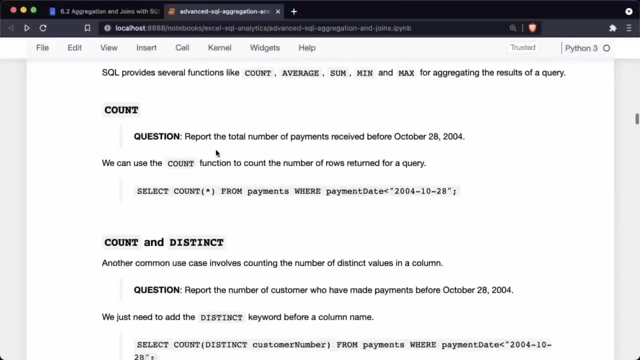 Aliases. SQL provides several functions like count, average, some min and max for aggregating the results of a query. What do you mean by aggregating? Well, it's combining the results that you get, typically into a single number, or maybe one or one or more numbers. 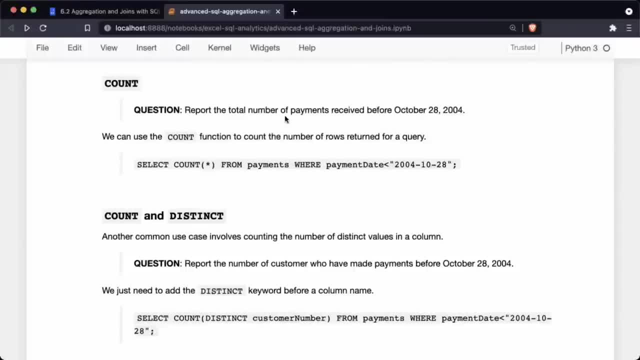 So here's an example report: the total number of payments received before October 28th 2004.. Okay, So this is the kind of question that will be posed to you or the other, The kind of information that you will have to figure out. 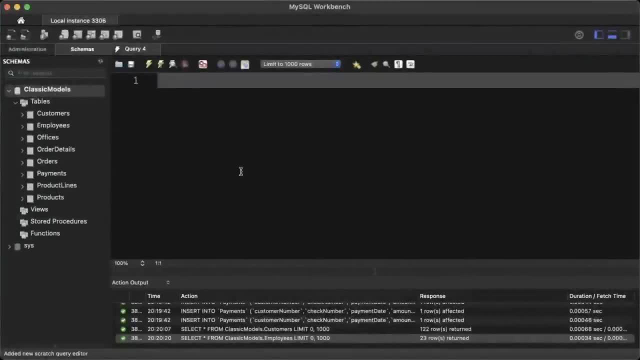 Now we know from the ER diagram and we know from. let's maybe just copy the question and put it here. Yeah, So this is the way to create a comment in a SQL file or a SQL query: You just put in hyphen, hyphen, space, and that's going to be a comment that is going to be ignored by them. 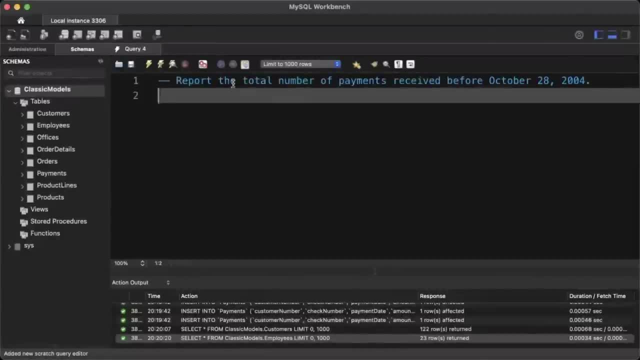 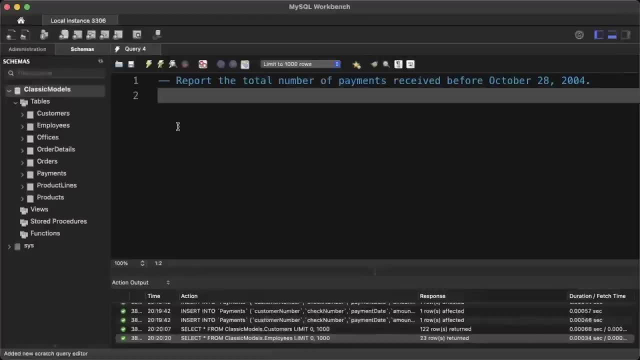 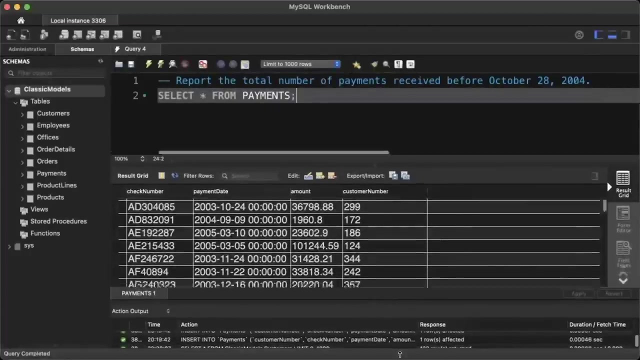 So we have a table called payments, So let me just do a select star from payments, All right, And once I run that I will get back a list of results. Okay, And once I run that I will get back a list of results. 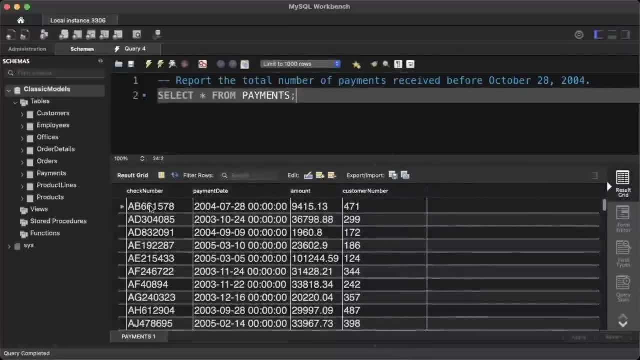 Yeah, Here's the list of results. So these are all the payments in the database. You have a check number, you have a payment date, you have an amount and you have a customer number- the customer who made the payment. All right, 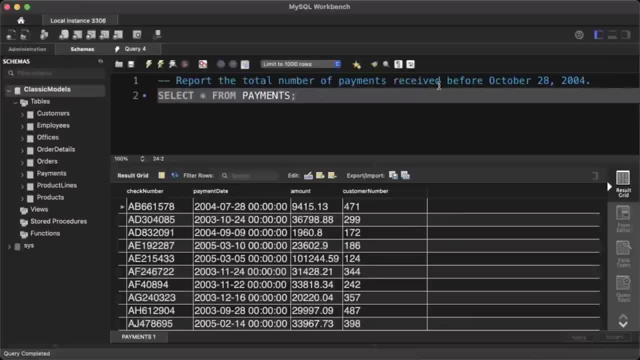 But we're not interested in all the payments. we're interested in payments received before October 28th 2004.. So there is a payment date here And it seems like this payment date is in this year, month date format And, in fact, if you want to know the data, 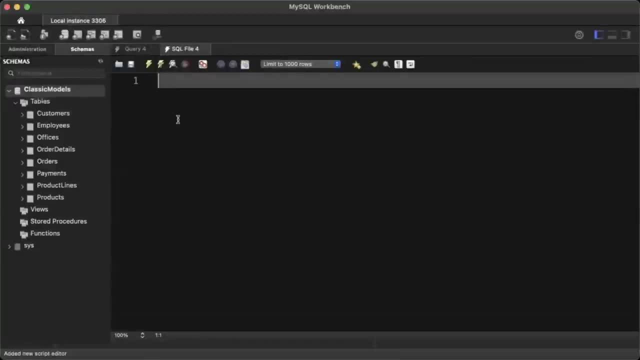 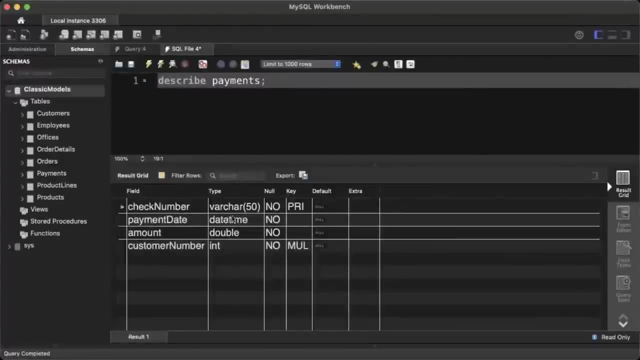 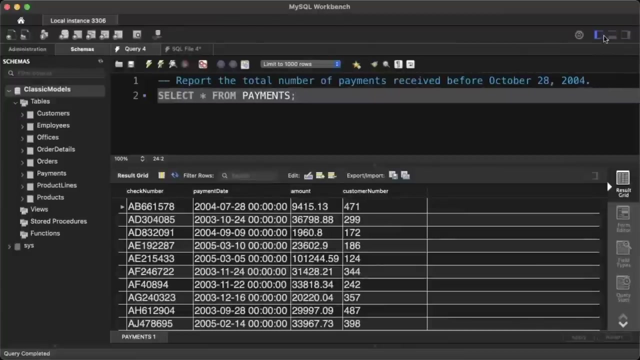 type of this payment date. you can just spin up a new query here and just type describe payments And you can see that the payment date is a date time. Okay, Now a date time is an ordered field. Obviously, dates have a intrinsic order. 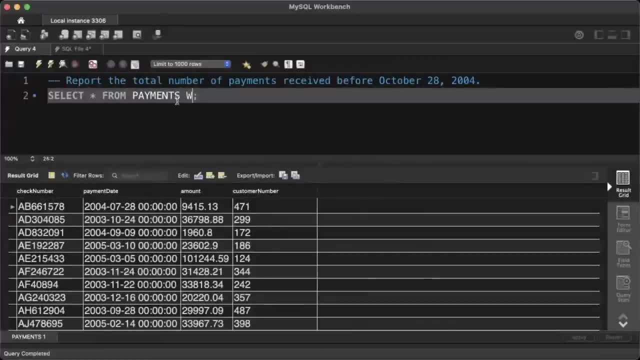 So here's what you can do: You can say: select star from payments where payment date is less than, because we want payments before October 28, 2004,. and then you provide the date that you want to check here, So that's 2004, and then you have October. 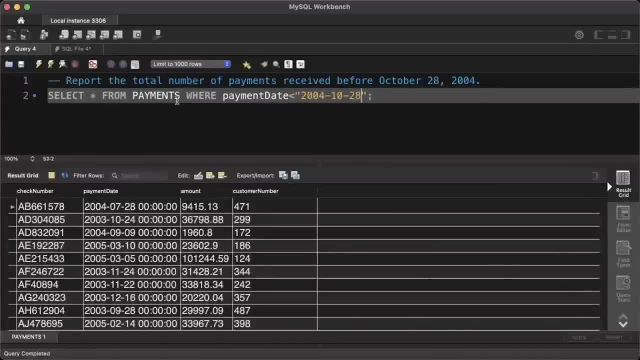 That is the 10th month And then you have 28,. so there should be enough. You don't need to put in the time here. So I'm just going to run that And if you see, now we only have payments that have occurred before October 24, before. 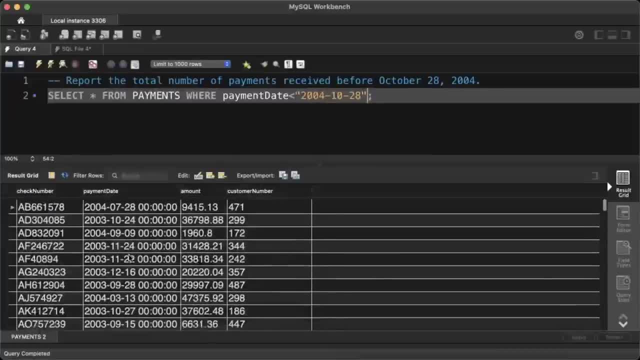 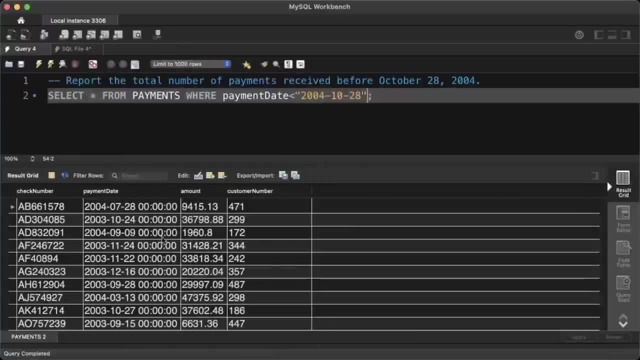 October 28, 2004.. And I recommend Just going through this list manually if you want to verify this. but that's, that's how you get that. All right, But we don't want every single payment, We want the total number of payments. 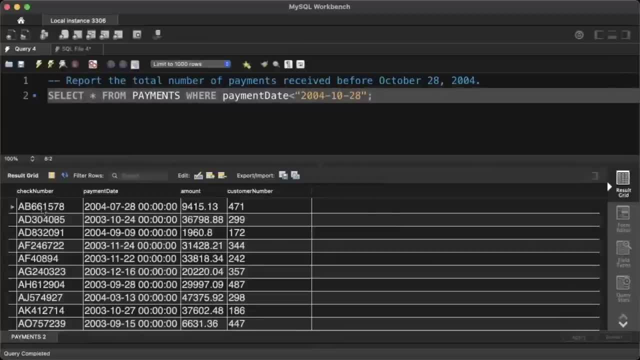 Now, if you want a total number of payments, it's very simple to. we simply want to count the number of rows that were returned by this query, And the way to do that is just type count. So count is a function in SQL and you can see it highlighted in green. 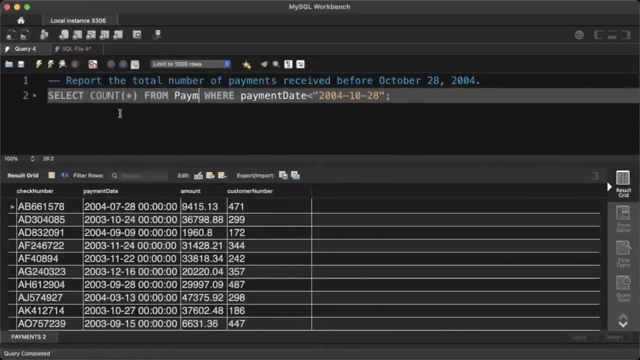 And uh, typically this is what we do. We put all the SQL Commands in. So typically this is what we do. We put all the SQL keywords on the SQL functions in a capital letters or uppercase and we put the column names in lowercase or whatever is the actual column name, whether it uses 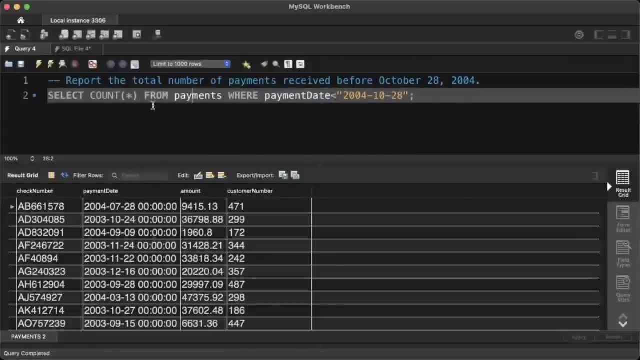 lowercase, uppercase or combination of both, And this is just to visually separate actual keywords with column names. but remember that SQL is completely case insensitive, So you could type all of these in lowercase and you could type all of these in uppercase, and it would work just fine. 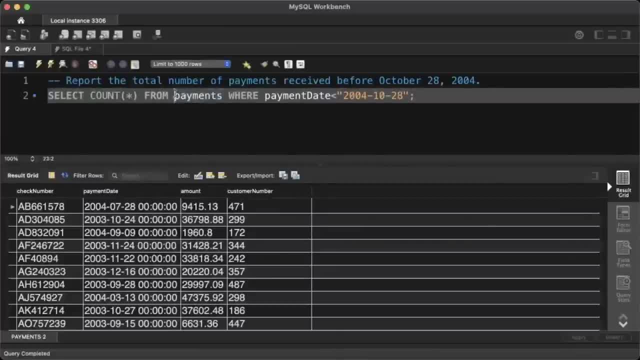 Okay, And this is just for visual separation in any case. in any case, we have the count function, So you just put instead of select count star, or use uh instead of select star. you just type select count star and run that. 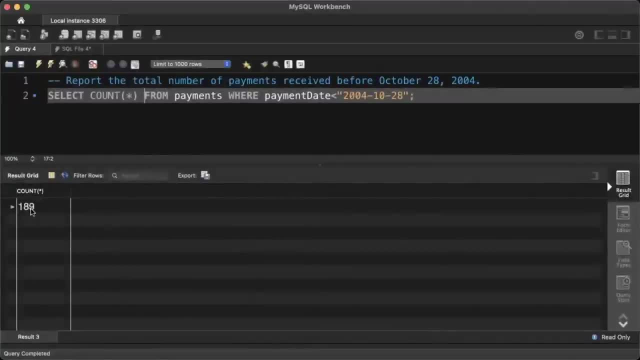 And now you will see here that there are 189 payments that have been made before October 28, 2004.. And if you did not have this, where clause this filter? Okay, Then you can see that there are total of 273 payments. 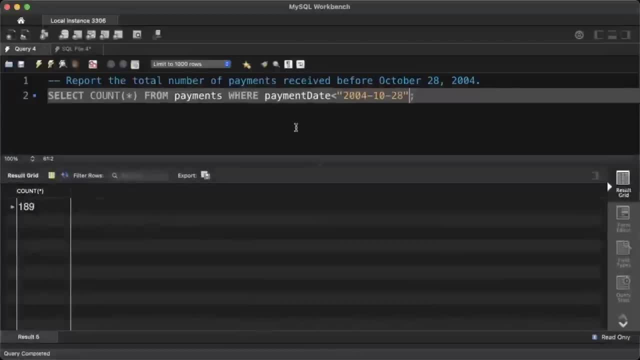 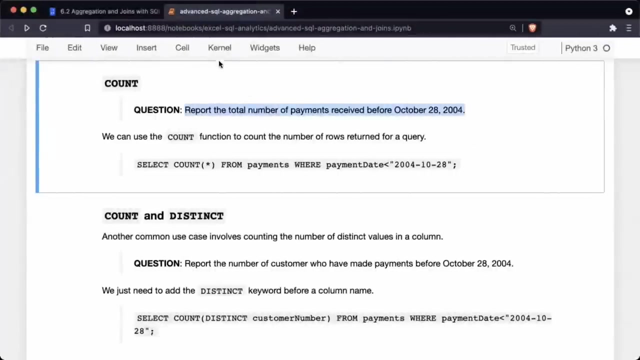 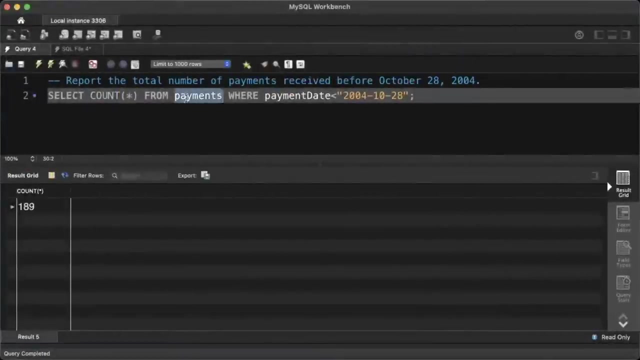 So, out of 273 payments, 189 payments were made before October 28, 2004.. So that's how you count the number of rows returned from a query. Just put in a count. Okay, And there, and there's a quick question here about payments where this payments table come from. 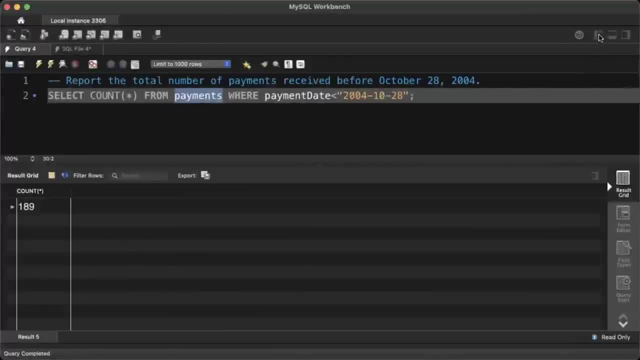 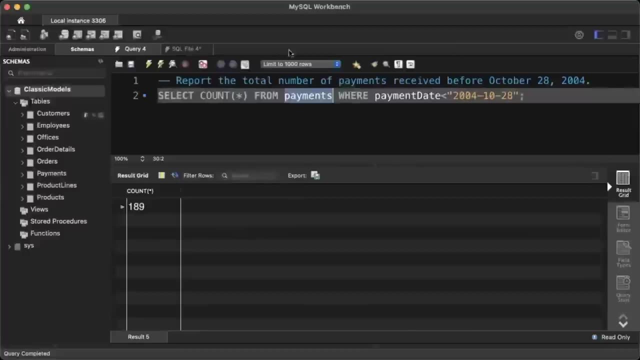 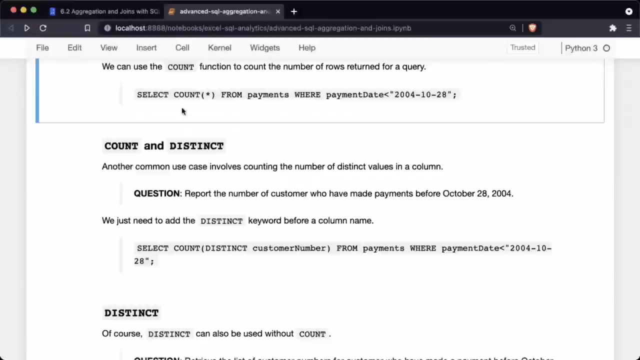 So this is the Table that we've just populated. when we downloaded the SQL file, classic models, dot SQL, and then we executed it, That gave us the stable and that gave us all the data inside the stable. Okay, So that's count. just put count around the selection criteria and that will count the tip. that will count the rows for you. 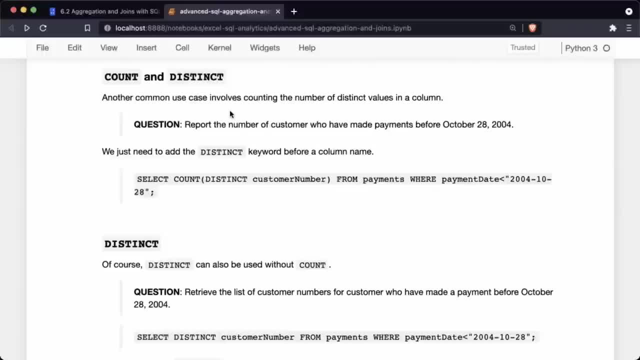 Next, another common use case involves counting the number of distinct values in a column. So here's a question report: the number of customers who have made payments before October 28, 2004.. So now we are no longer interested in the number of, now we've no longer interested in the number of payments that were made. 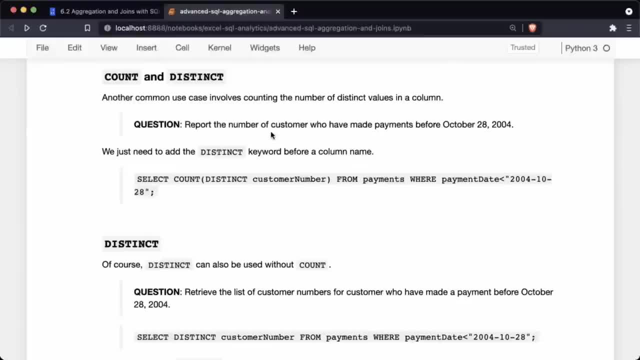 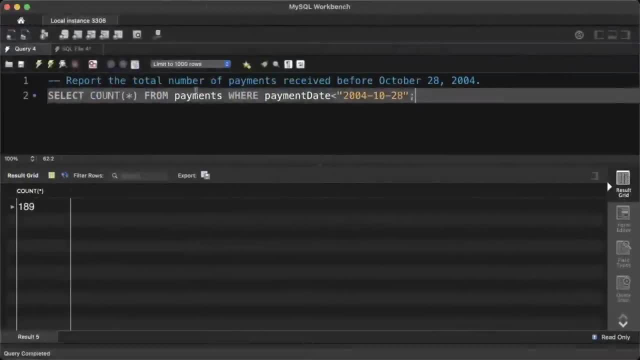 We are interested in the number of unique customers who have made payments, and one customer can make multiple payments, So number of customers who have made payments before October 28, 2004.. So, once again, maybe let's open up a news. Oh, let's just continue typing. 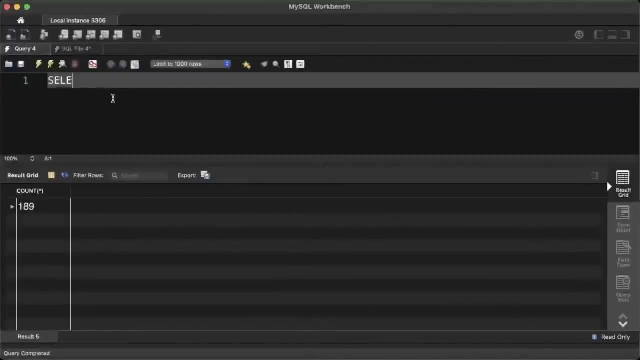 Here. So here's my select query: select star from payments And I can write payments, or I can write payments or I can write payments, and it will all be the same thing. Okay, This is the name of the table, So anything you see after from is a table name. 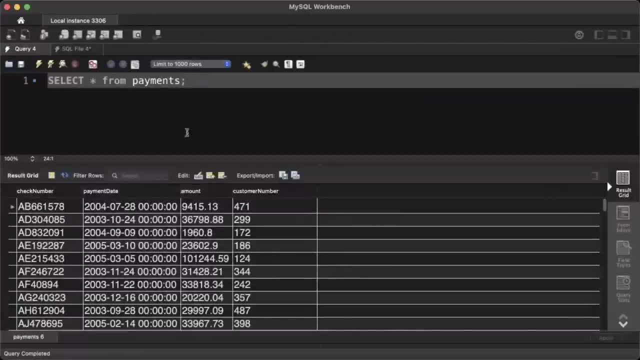 So select star from payments. that gives us a list of all the payments And once again we want to select them. I'm just going to mix cases here, Uh, but Don't worry about it. So let's just say, select star from payments where payment date is less than 2004,. 10. 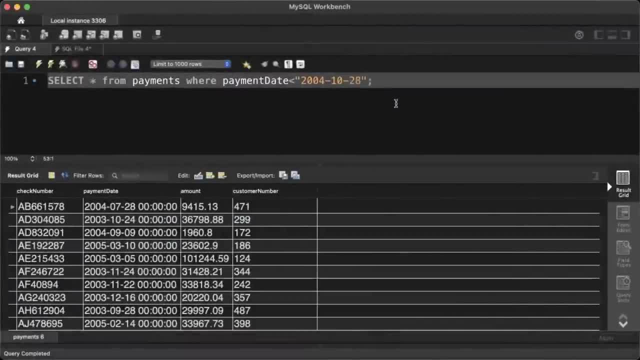 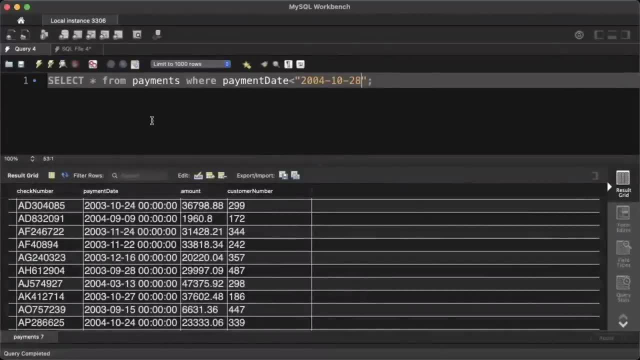 What's that? October 28,, so 2004, 10, 28.. So that gives us all the payments that have occurred before 2004, 10, 28.. Now we are interested in the customer number. I'll be interested in the unique customers who have made payments before the state. 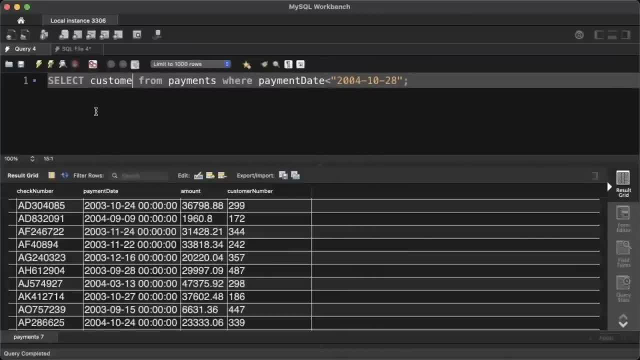 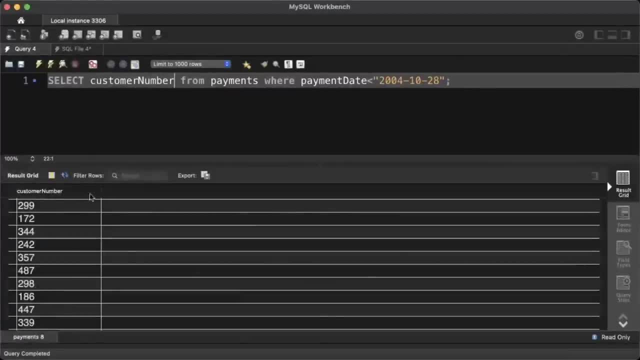 So here's the first thing I'll do. Maybe I'll just select the customer number first. Okay, So if I just select customer number now, I have ignored all the other columns. I have just selected the customer number column. So now I have 20,, 2, 99,, 1, 72,, 2, 42,, et cetera. 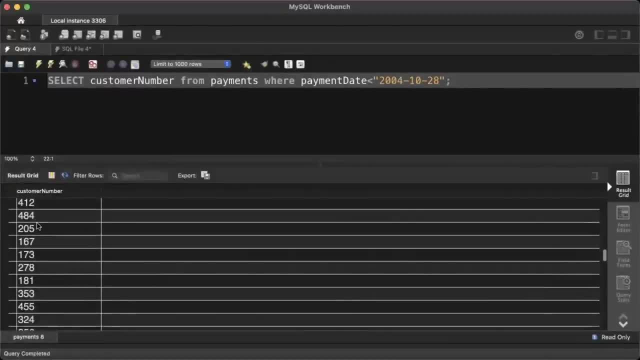 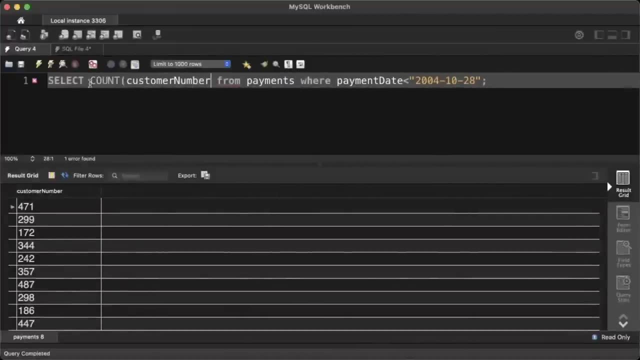 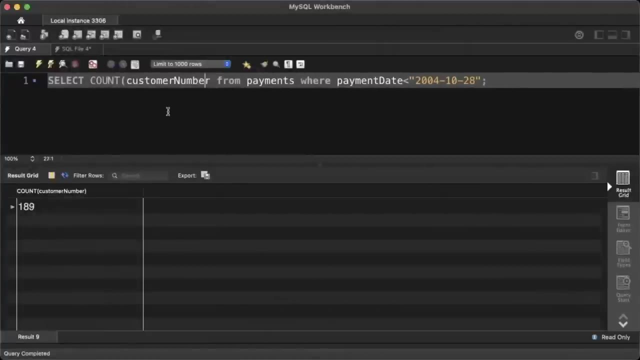 But of course there are probably going to be repetitions here, and you can go through this list and verify that there are some repetitions. Okay, So if I did select count customer number, this is giving me one, 89.. Okay, Which is actually the total number of rows returned, but we want simply the number of unique customers who have made payments. 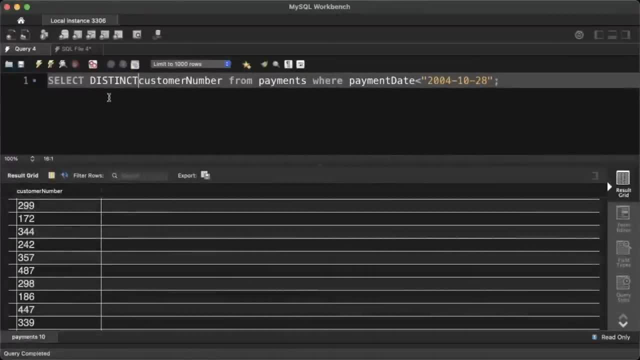 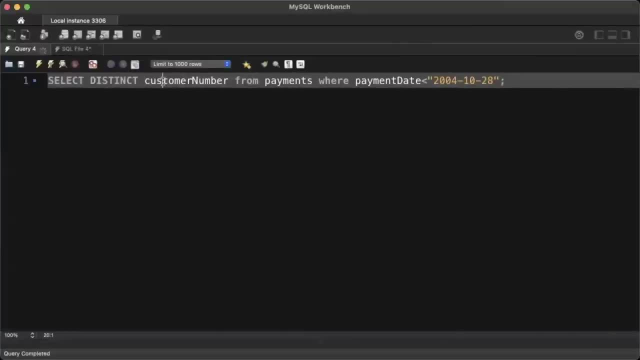 So what you do is you type distinct. Okay, Now, when you type distinct, repetitions from this list will go away. So if I type distinct here now, you can verify that this list is a bit smaller. This list is not that big anymore. 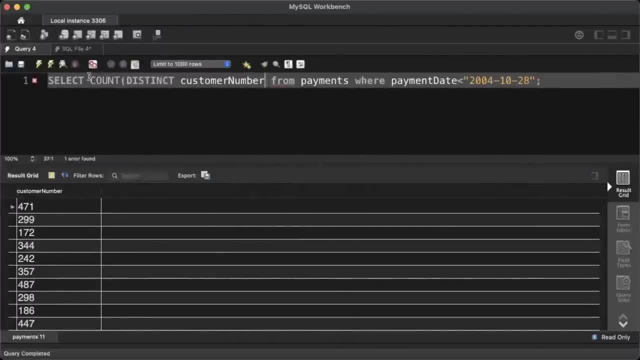 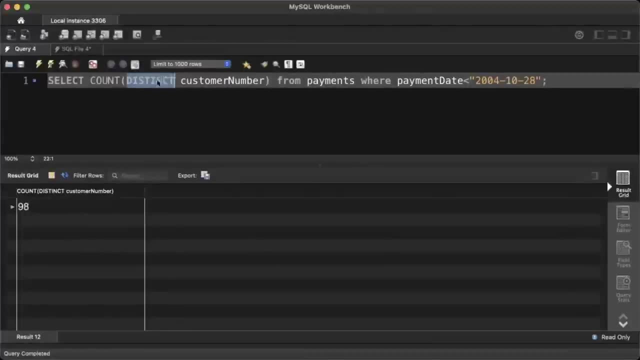 And in fact if I type count now, You will see that the count is only 98.. So what distinct does? when you type distinct before a column name, it is going to just select distinct values of that column. And if you type multiple column names after distinct, it is going to just select all the distinct combinations. 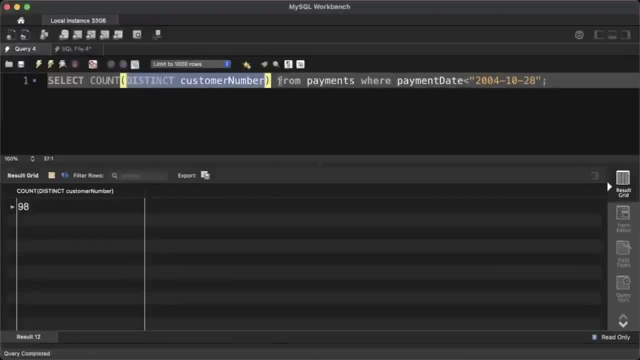 But in this case we first get the list of all the distinct customer number, which is a customer ID, and then we count the number of rows. Okay, So count is a function, but distinct is still a keyword, which is part of the SQL syntax. 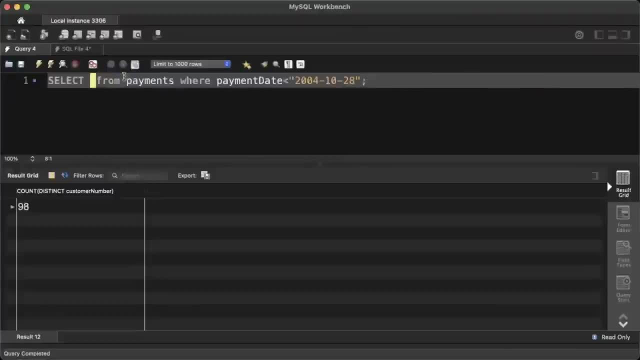 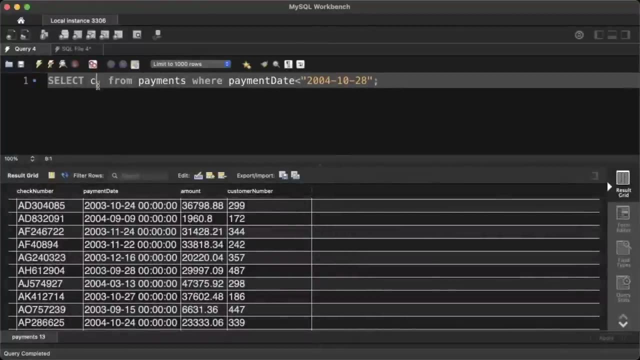 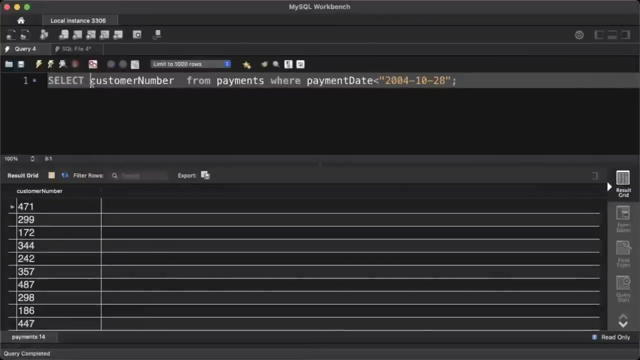 Okay. So once again, I'm just quickly going to repeat that we have select star from payments where payment date is less than October 28, 2004.. Now, instead of selecting all the columns, I just select customer number, and that gives me the customer number for each payment. but I'm only. 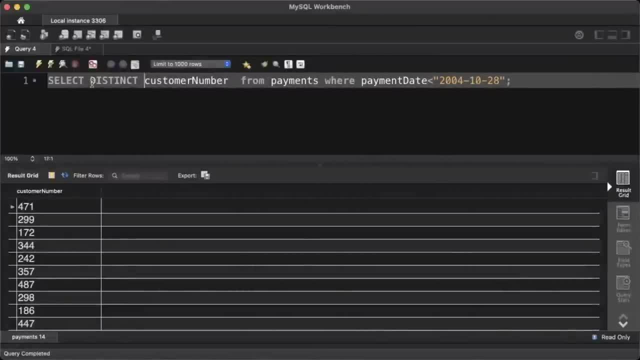 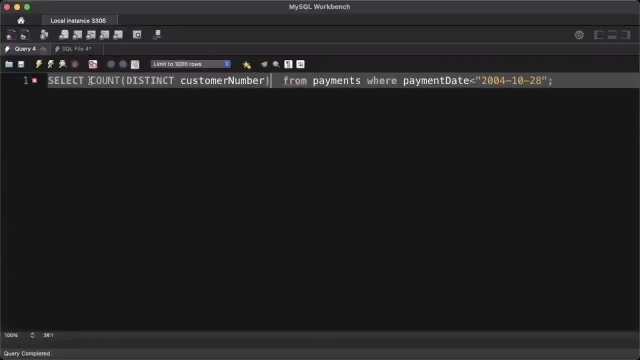 interested in the distinct customer numbers I don't want to show. I don't want customer numbers to show up again and again, So I type distinct and then I want to count them. So here is the count function which is going to count the customer numbers for me. 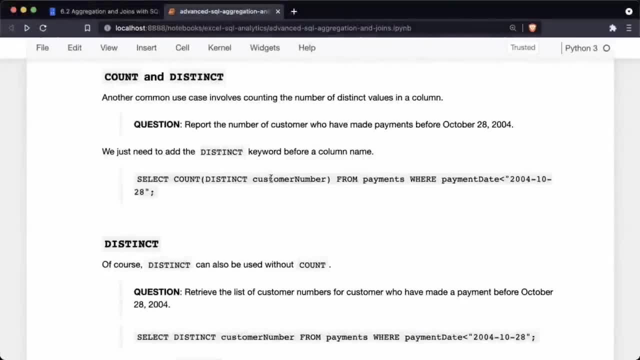 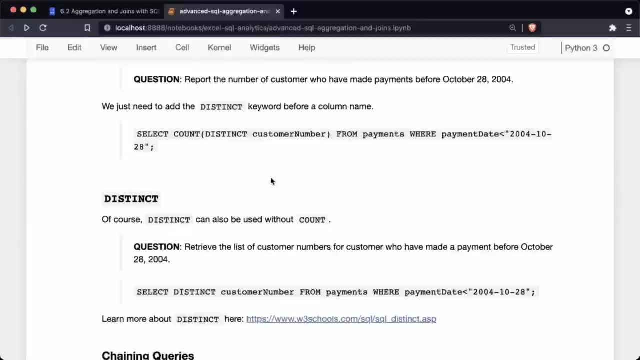 And there are 98 of them. Okay, So that's how you solve any SQL query or solve any SQL question. You could just go step by step. You start by looking at the table and then you simply keep adding in criteria, one by one. 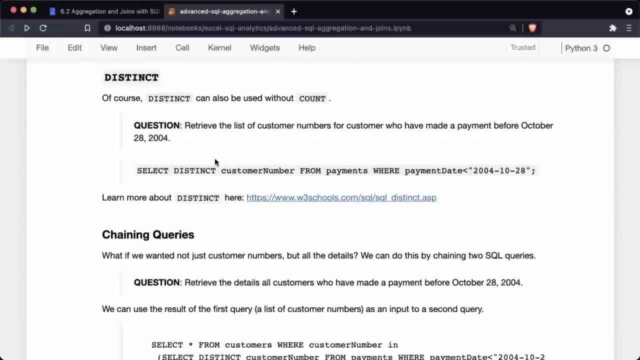 Of course, as I said, distinct can be used. can also be used without count. So if you just wanted the list of customer numbers for Customers who have made a payment before the 28th of October 2004,, then you just type select distinct customer. 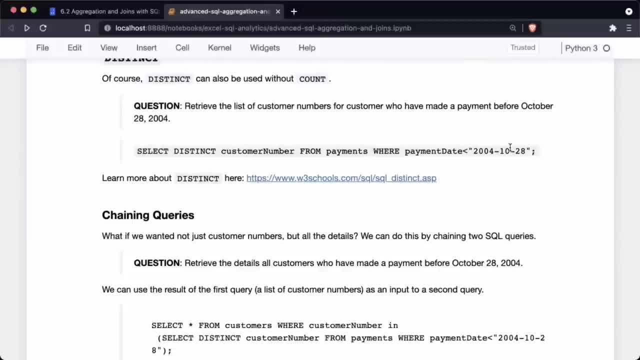 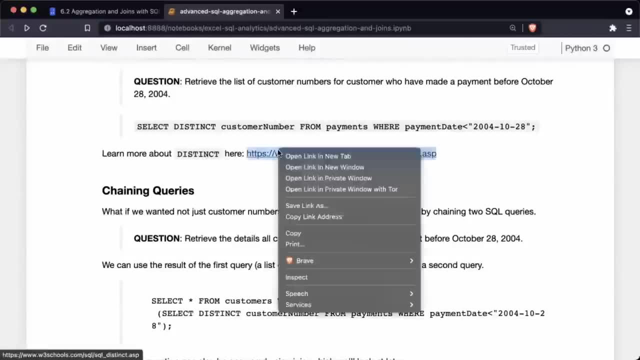 number from payments where payment date is less than 28th of October 2004.. Okay, And you can use distinct with multiple columns as well. So if you want to try out, learn more and try out what distinct does, just check out some documentation here on W3 schools. 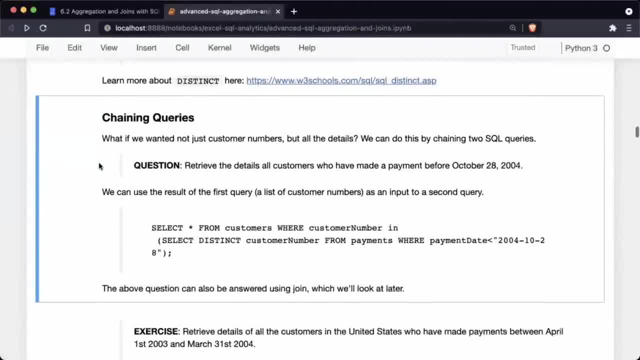 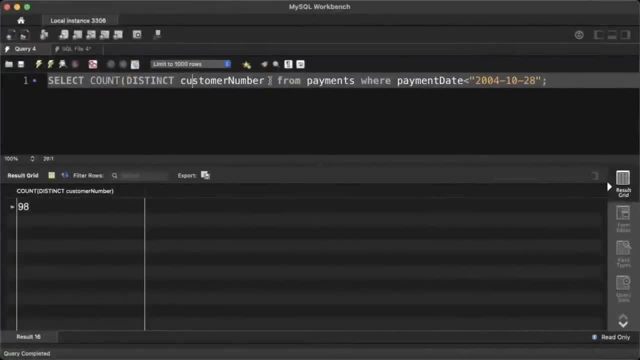 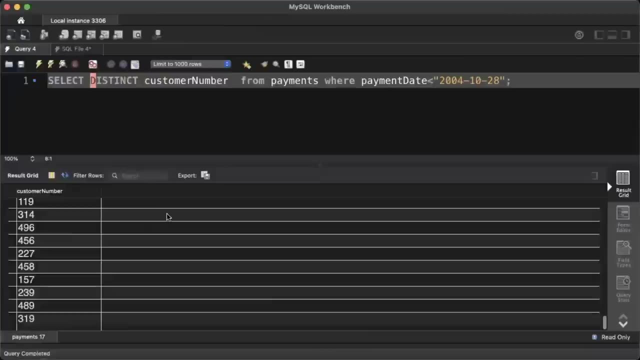 And you can also practice this online. Okay Now, If I look back at this query, just the distinct customer numbers- this is just giving me a list of customer numbers, right, And this is not very informative, because ideally what we want is details of those customers. 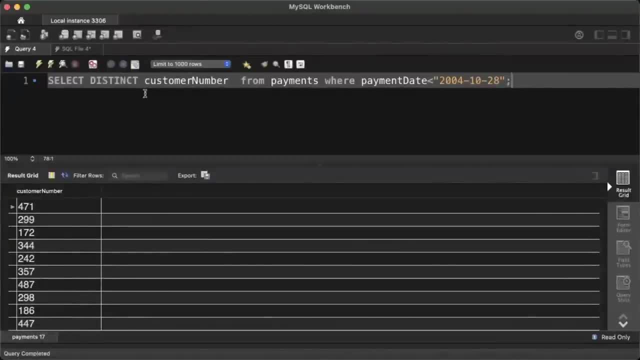 I want to know which people, which stores, have made payments before the 28th of October 2004.. So how do you do that? Well, here is one way to do that. We know that this is a list And you can write a query which uses the result of this query. 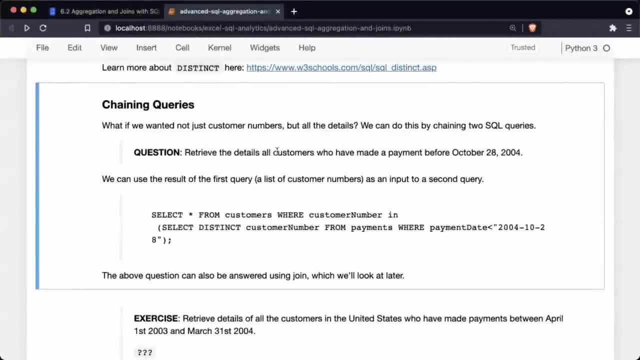 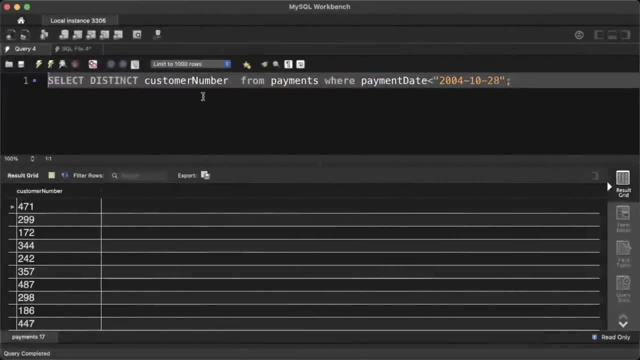 Okay, And here's what we want to answer. We want to retrieve the details for all the customers who have made a payment before October 20, 2004.. Okay, So how do we do that? Let me just put this query aside for a second and let me start typing. and let's just comment it out here and let me start typing. 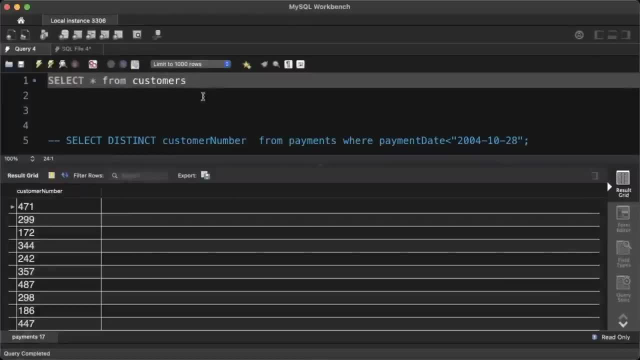 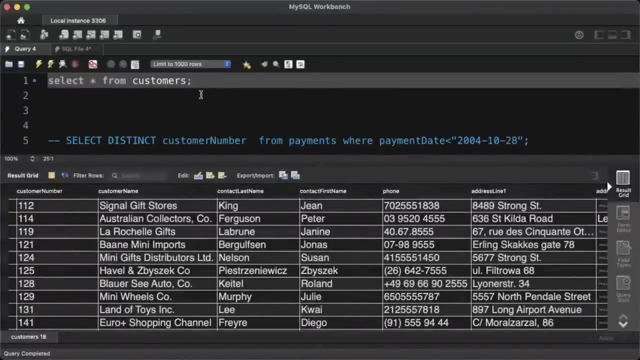 select star from customers. Okay, So I guess I'm just going to use lower case here, but select star from customers. So now I have details of all the customers, but I'm not interested in all the customers. I am interested in simply the customers where the customer number is in this list that I had earlier. 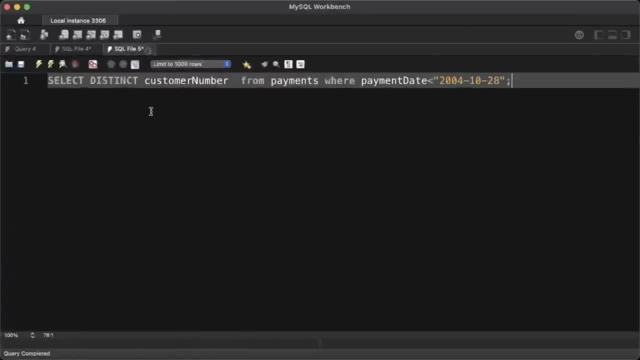 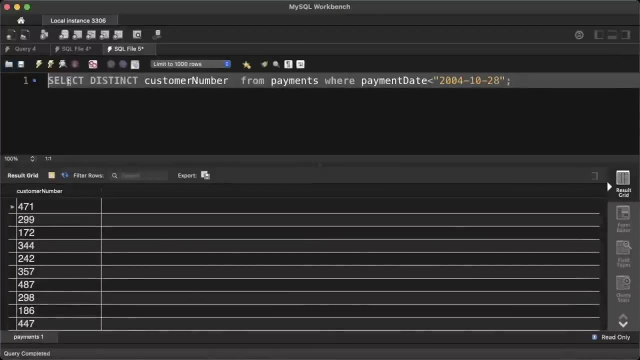 And I'm just going to run this again here in a as a new query. So I just want to get the details of customers who are in this list- 98 or so customers. So what I can do is I can take this query without the semi-colon and I can come back here. 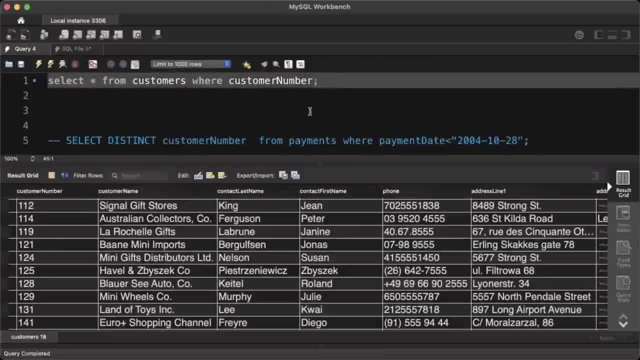 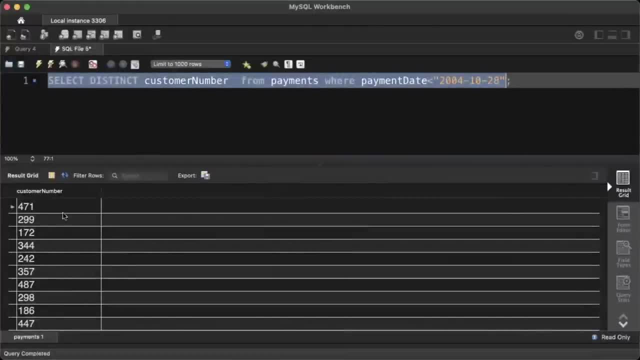 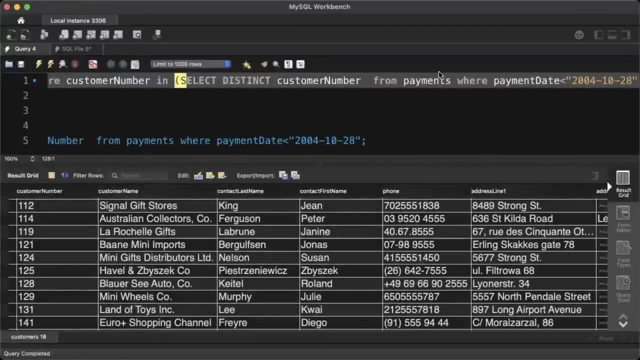 I can come back here: select star from customers where customer number in and then you'll have to give a list. So instead of giving this actual list, I can give a query with generates that list. So I can just put in a bracket here and type: select distinct customer number from payments where payment. 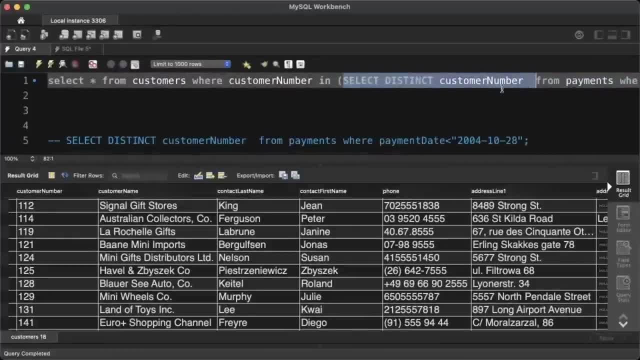 Okay, So we take the result of this query, select distinct customer number from payments where payment date, and then we run a second query which is going to select details from the customer's table where the customer number lies in this list. 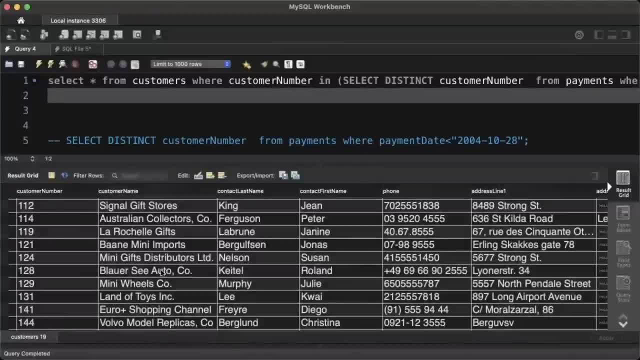 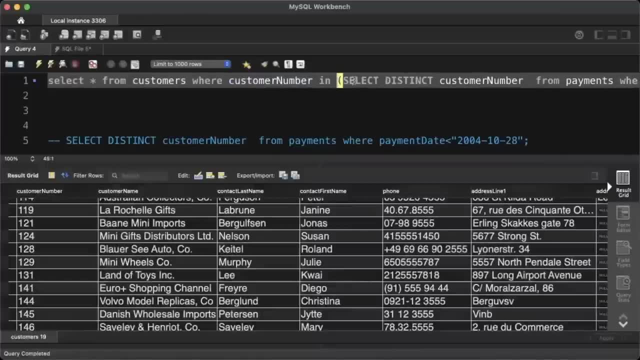 Okay, So if we run that now, so now you will only get details of customers where the customer number is in this list. And what is this list? This list is simply the number. Okay, Distinct customer numbers from the payments column where the payment date is less than 2004,. 10, 28.. 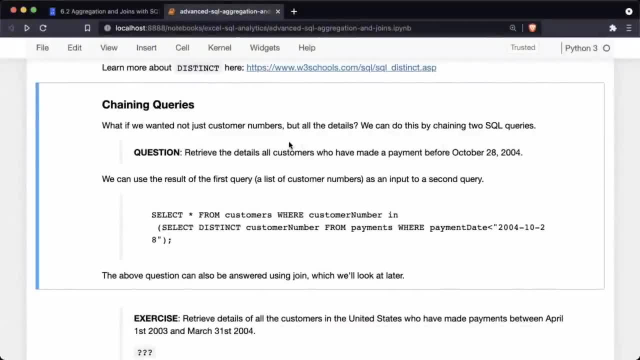 Okay, So that's how you change SQL queries. You can take the result of one SQL query and use it in a where clause, or you can even select from it again, So you can treat, uh uh, treat the result of a query as another table, essentially, and then write SQL queries on top of the results of other SQL queries. 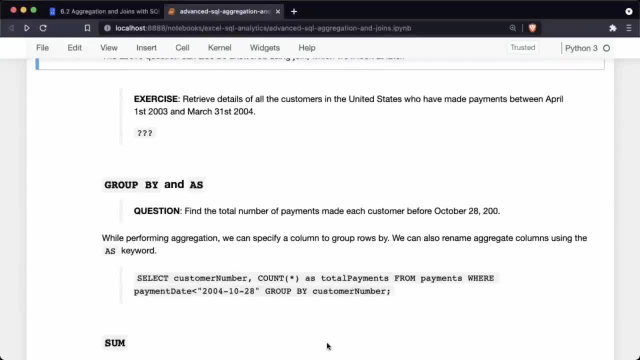 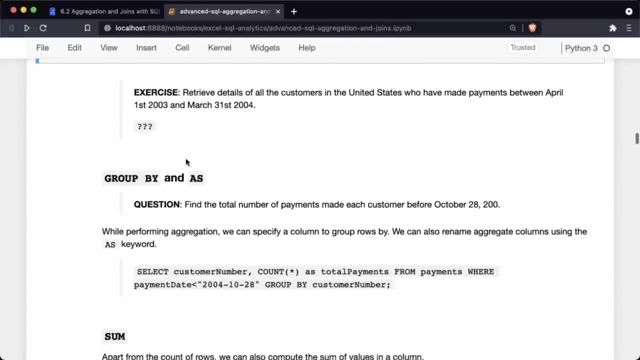 Okay, So that's how you chain queries. Okay, So here's an exercise for you: retrieve the details of all the customers in the United States who have made payments between April 1st 2003,- uh three- and March 31st 2004.. 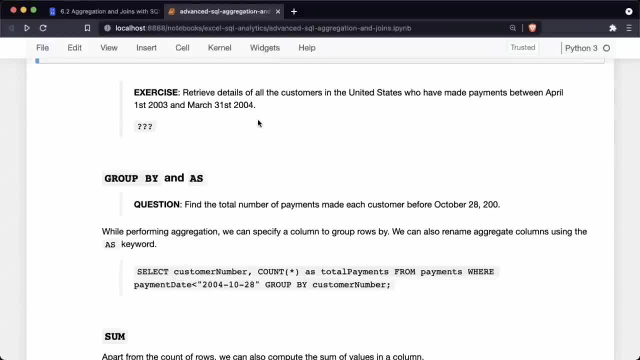 So how would you do this? You would first think about it the way you would do this as first you would just look at all the payments, So you just do select star from payments, And then you would look at payments between April 1st 2003 and March 31st 2004.. 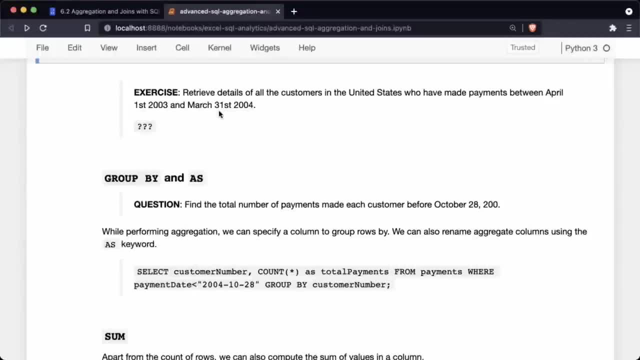 So you would put some kind of a where clause where you would combine two conditions using an and keyword, And once you get the results of four payments just between these two dates, then you simply retrieve the customer ID for those payments And then, once you have that list of customer IDs or the distinct list of customer IDs, you can 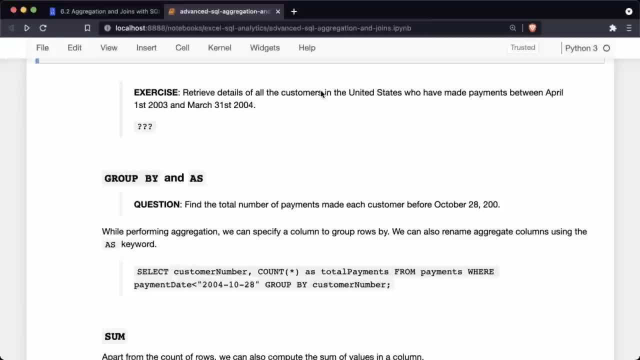 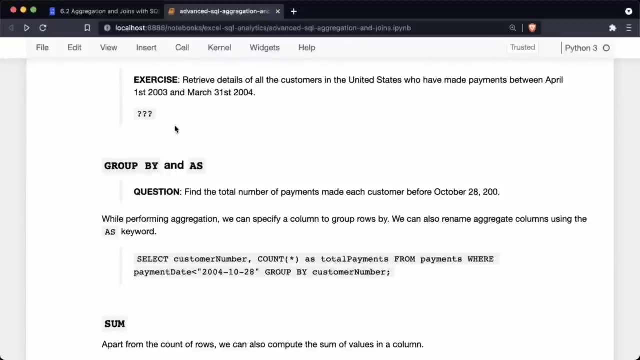 You can use that to get the details of customers and you add another where clause where you will check whether the customer is in United States or not. So it's going to get a little complex here, but I will let you figure this out And if you're unable to do it, uh, do ask on the slack group and we'll help you out. 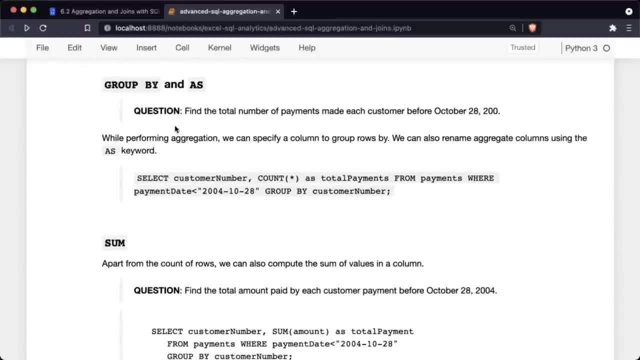 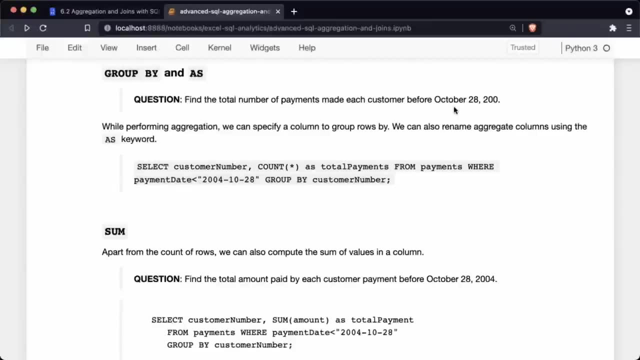 Okay, So let's talk about grouping then. So here's a question: find the total number of payments made by each customer Before October 28th 2004.. All right, let's go back and let's try and solve this. 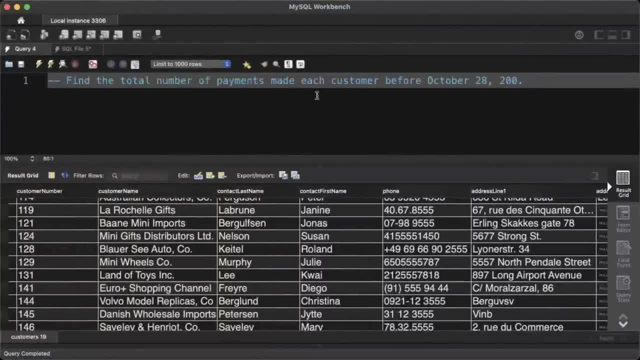 So here's the question: Total number of payments made by each customer before October 28th 2004.. So we say select star from payments again. So we were selecting. We want to show all the columns On the payments table. 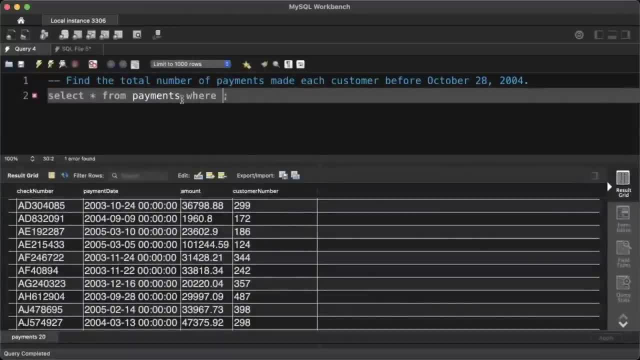 All right, And we just want to look at payments before October 28th 2004.. So, where payment date is less than 2004, 10- 28.. And now we want to count the total number of payments. So we could do this count, but this is the total number of payments across all customers. 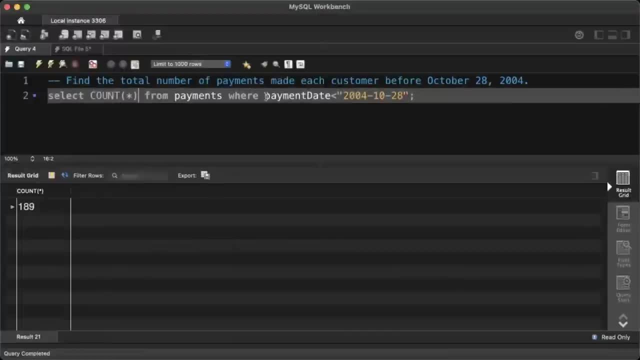 We want to count the number of payments made by each customer. So here's what you can do. You can provide- uh, you can provide- a group by clause. So you can type something like this: You can say: group by- well, I believe it shows up after where. so, yeah, this, this. 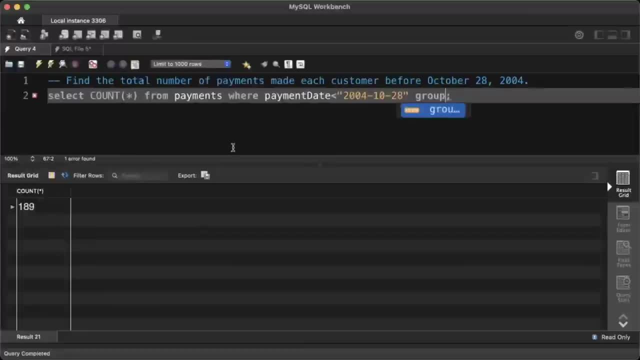 can sometimes be confusing which clause comes up to which, but let's try here. Well, actually let's start with that, and then we'll see if that works. So group by- uh, so you type select count, Start from payments and group it by customer number. 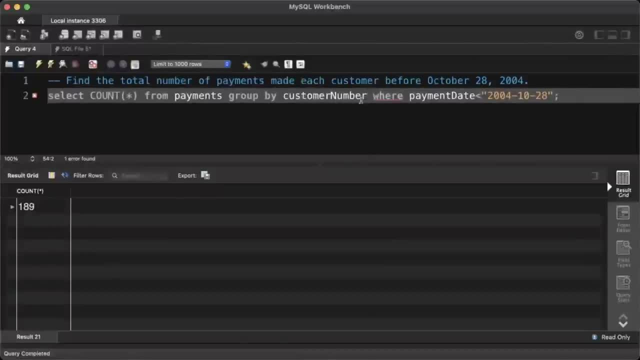 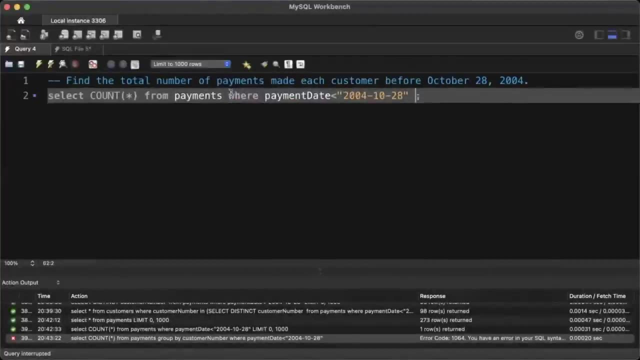 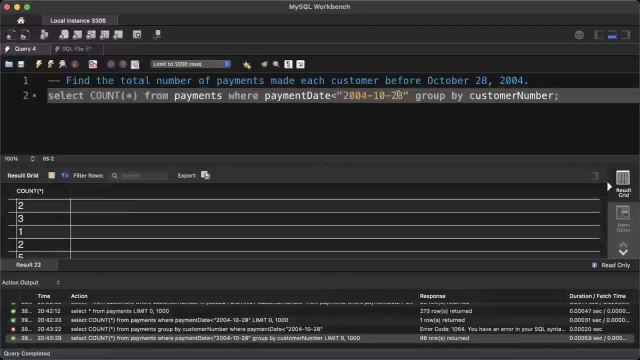 So now you're just looking at count star of payments and grouping by customer numbers. Okay, I think this. this comes after Yup. So you type select count star from payments where payments date is less than two- 20, 2004,, 10, 28,- and you group by the customer number. 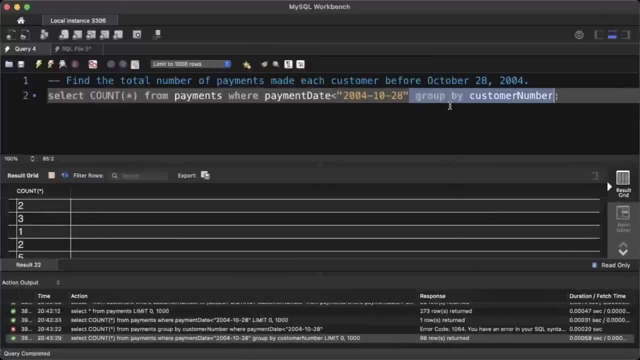 So what happens here? Yeah, SQL first creates all groups of groups of rules for each customer number, and then it computes the sum or it computes the count of the number of rules for each customer number. So here it seems like for a certain customer there are two rules. for a certain customer. 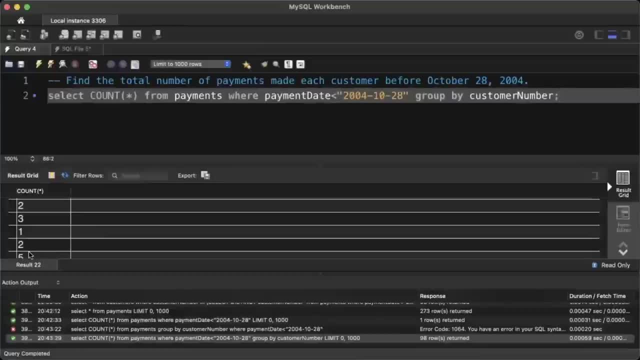 There are three rows, for another customer There is one row, et cetera. Uh, but of course we also want to see the customer number. So what we can do is we can just take this customer number column and select that too. 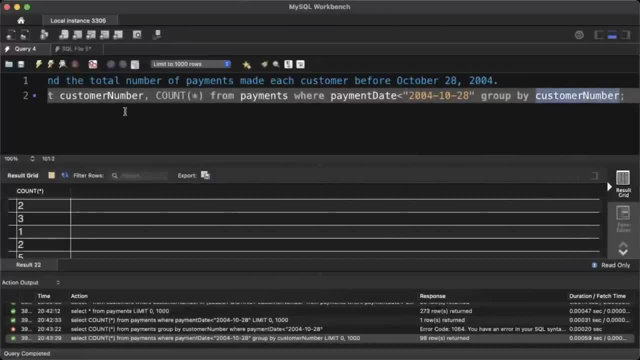 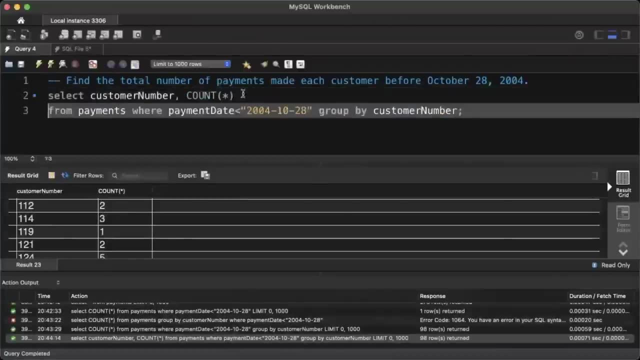 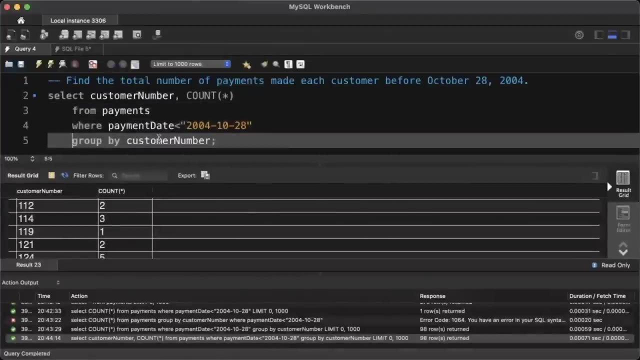 Okay, So anytime you Group by a certain column, you can also show that column in the result. So here's what that looks like: Select count star from payments where payment data is less than a certain value. So like customer customer number, comma count star from payments where payment data is less than a certain value and group this data by customer number first. 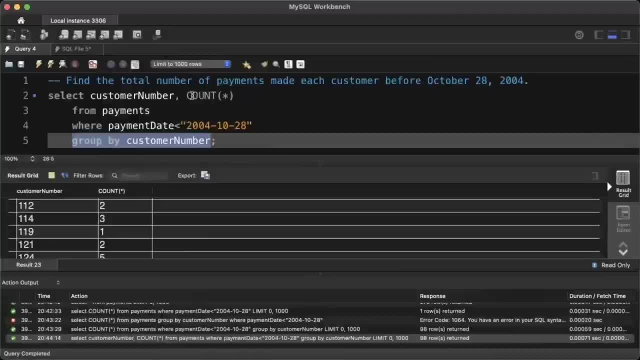 So first SQL creates groups for each customer number, then it performs this count star And then it gives us a customer number and the count star. Okay, Now here's one other thing we can do. This is not very informative, because we're looking at count star here. 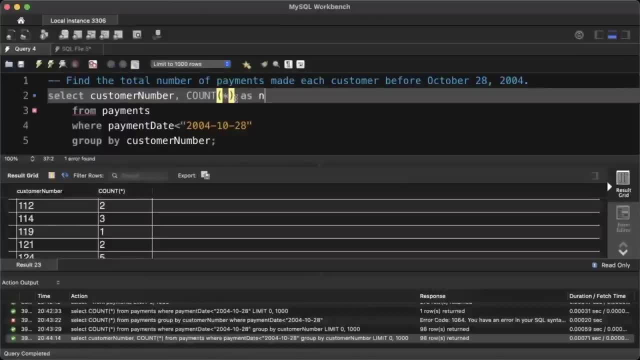 What we can do is we can just say, uh, number of payments. We can rename this count, the output of this count, as number of payments. Okay, This is called aliasing. So now you have this table where it says Customer number and it shows you the number of payments. 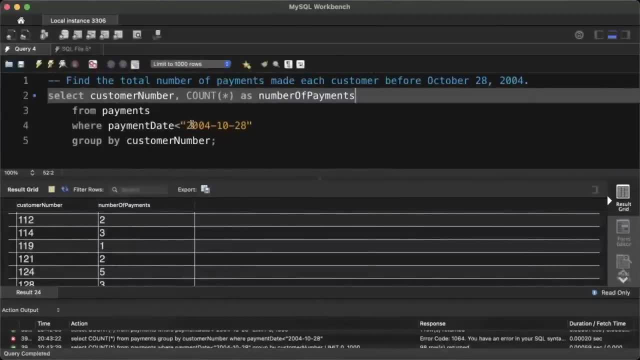 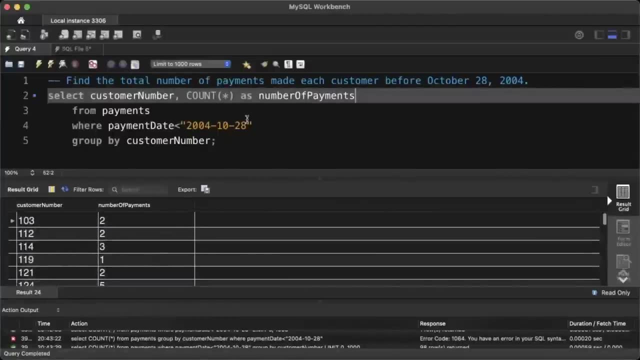 And you can see that the customer number one one- two had two payments before the state. customer number one one- four had three payments And for each customer in the database you get how many payments they've made, Only the customers who have made payments before this particular date. 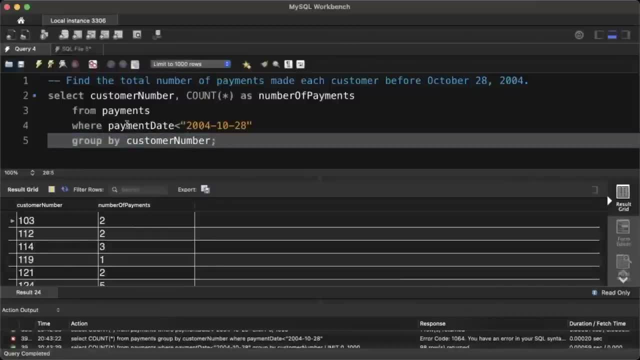 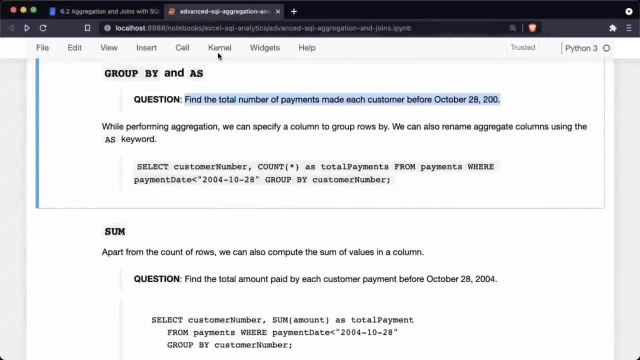 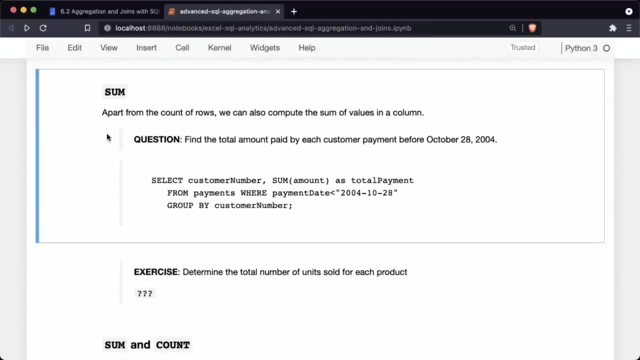 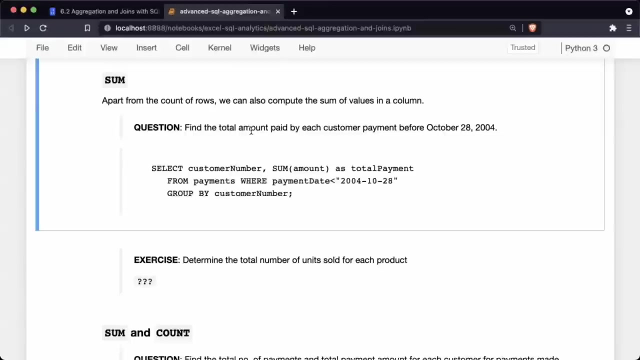 So this is how you use group by grouping is very commonly used with aggregation functions like count. Now, apart from the count, you can also compute the sum of values in a column. So here's one thing you can try and figure out: find the total amount paid by each customer, which is the sum of all their payments before October 28th 2004.. 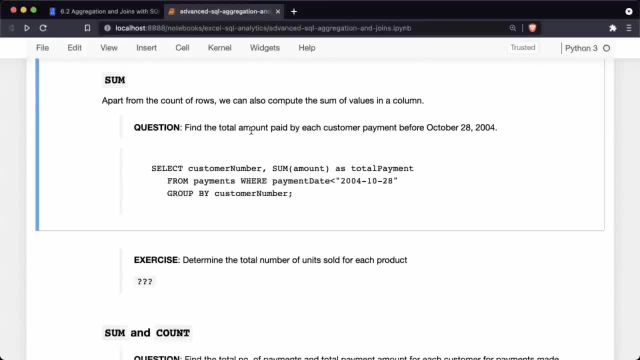 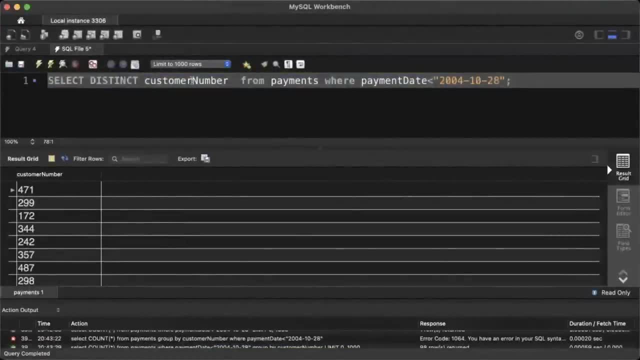 So let's see if we can do that. I'm just going to once again select- uh, I'm just going to select star from payment payments here and just see: Okay, So we can see that the total amount paid by each customer before October 28th 2004.. 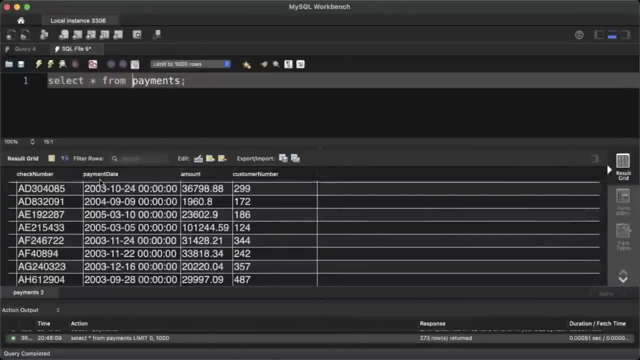 So let's see if we can do that. Okay, What columns we have? So we have a payment date which we have been looking at. We've been looking at this customer number, but there is also this amount. So what we want to do is we want to total up the amount for each customer. 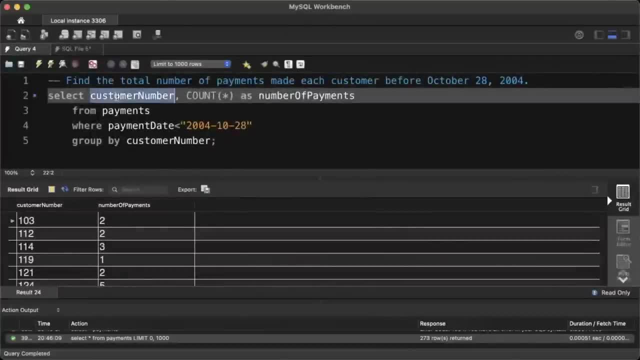 So let me go back here. So now I have select customer number and instead of count star, which is going to count the rules, I am going to call some and I'm going to sum the values in the amount column. So count. you generally put in star because you're discounting the number of rows. 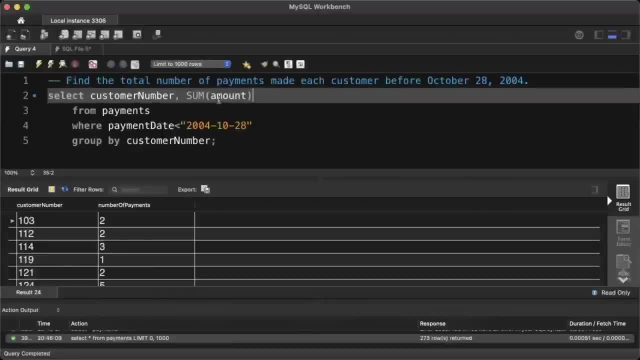 So you don't have to specify a column, but when you want to compute the sum, you specify the column for which you compute the sum. So sum of amount and I'm going to call that as total amount. Okay, So select customer number and some amount which I'm calling total amount from payments where payment date is less than 28 October 2004, and group by the customer number. 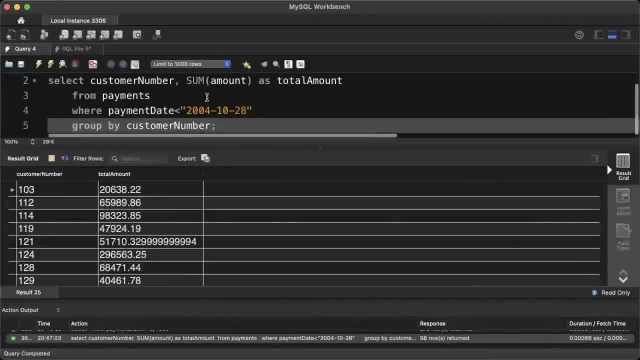 And that now gives you, for each customer, the total amount. Okay, So that's the total amount. Okay, So that's the total amount. Okay, So that's the total amount. Okay. So all we've done is we've replaced count star with some amount. 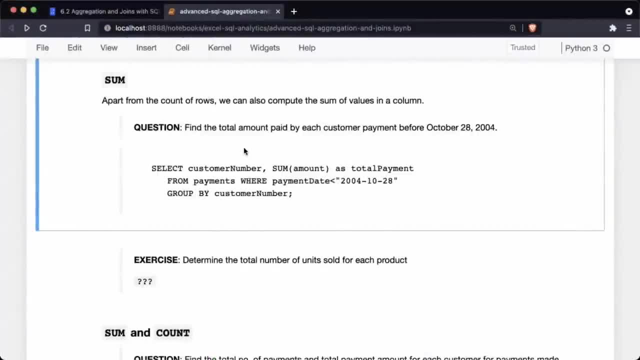 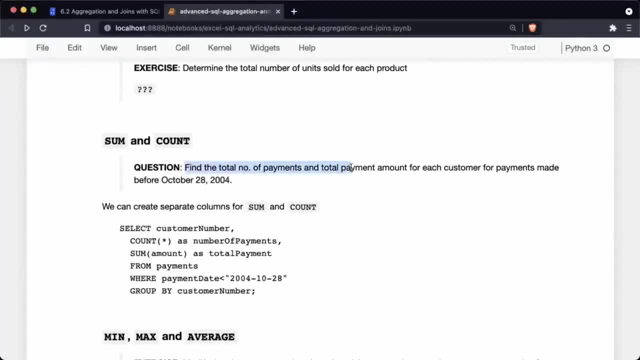 Okay, So these functions are generally work, all work in the same way. some count and you can also use them together. So here's an example: find the total number of payments and the total payment amount for each customer for payments made between uh before October 28, 2004.. 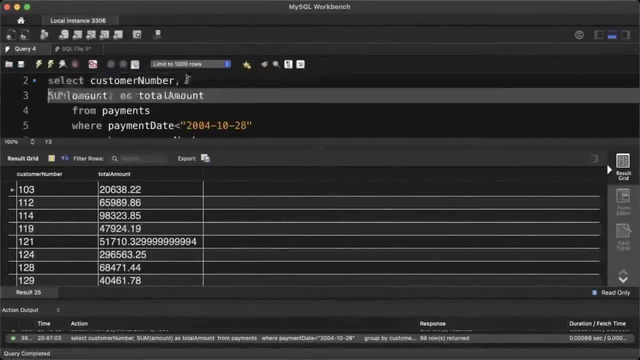 So how would we do that? Well, we have select customer number, uh, and then we We have the total amount already. I'm just going to add another column here. So I'm saying I'm going to say count star as number of payments comma. 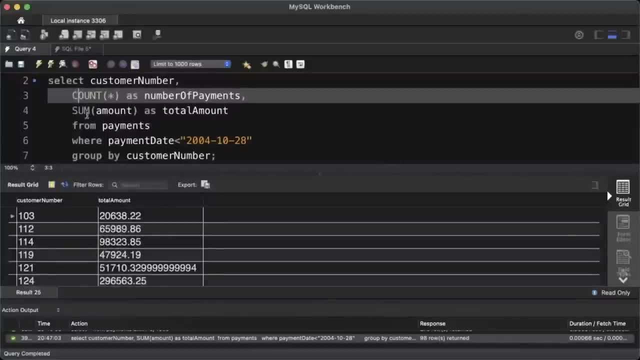 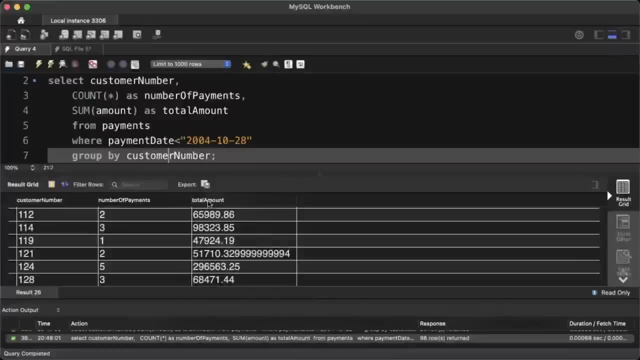 Yeah, So we have select customer number, count star as number of payments, Some amount as total amount from payments where payment data is less than such and such, And then we group by customer name. So now we have for each customer what is the number of payments they've made and what is the total amount that they've made. 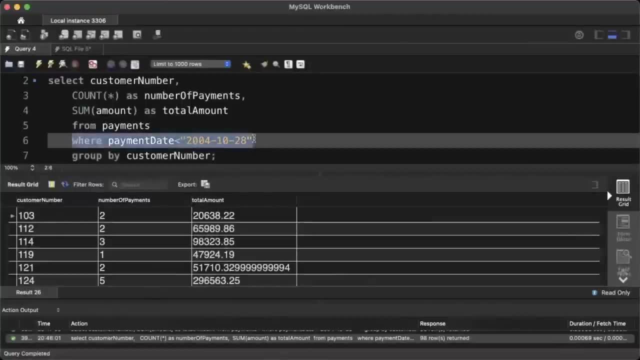 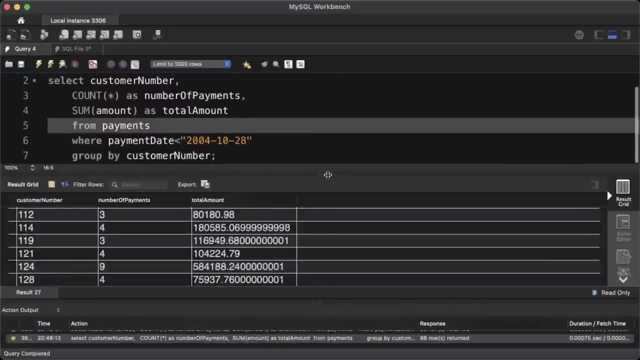 They've paid before this particular date and you can try and remove this where clause and see that the result actually changes. And you see now that the result is different, right? So try and understand each part of the SQL query. the same SQL query is mentioned here. to try and understand each part of the query. 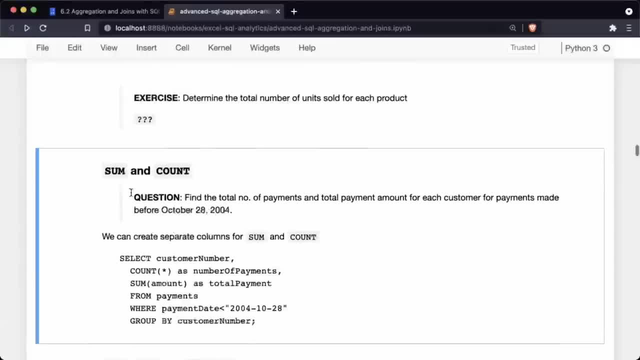 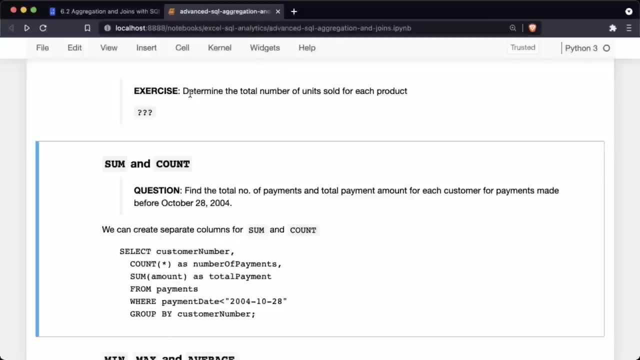 And if you can make sense of it, then you're getting familiar with SQL. And here's an exercise for you: determine the total number of units sold for each product. So there is a product's column And then there is a Okay. 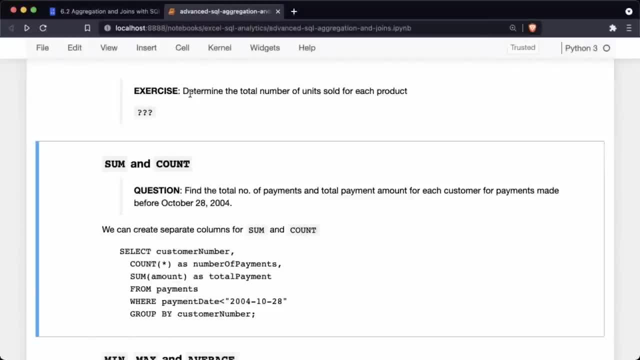 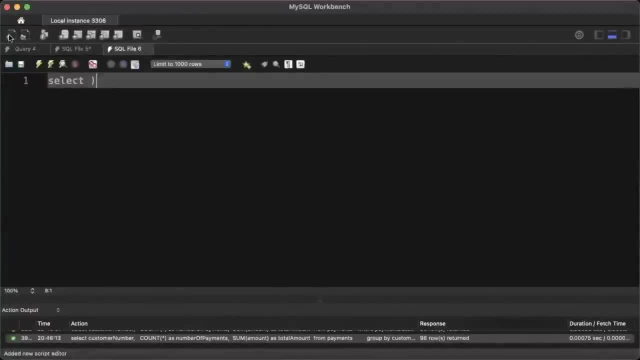 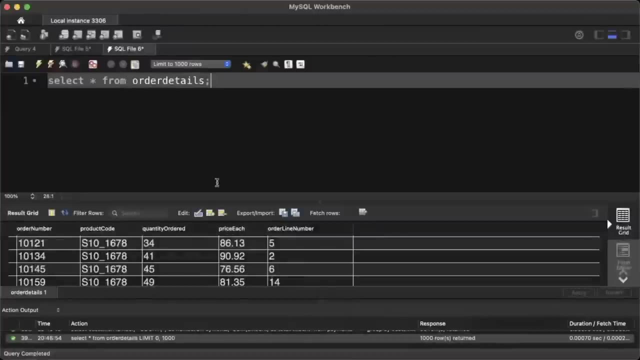 Okay, Okay, Um. so there is an order details column, I think let's take a look at that quickly. select star from order details. So there is an order details table and this contains the details of all the orders that have been placed. 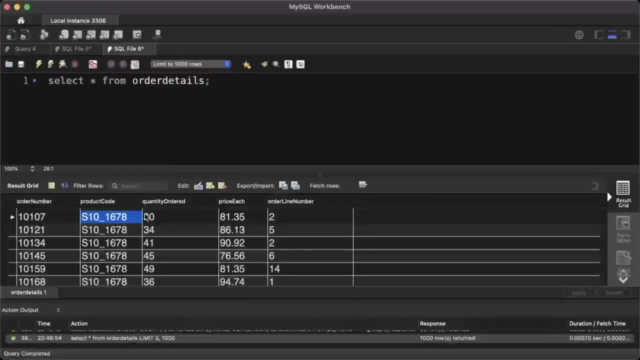 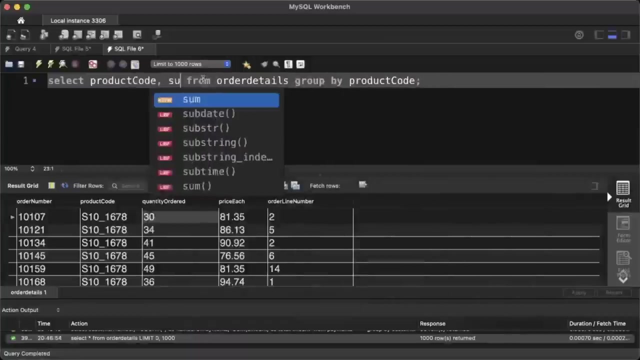 And then here you have the product code and you have the quantity ordered of that product in that particular order, And what we want to do is we want to find the total number of units sold for each product. So if I simply do group by product code and here if I do product code and I do a sum and in the sum I put in the quantity order, 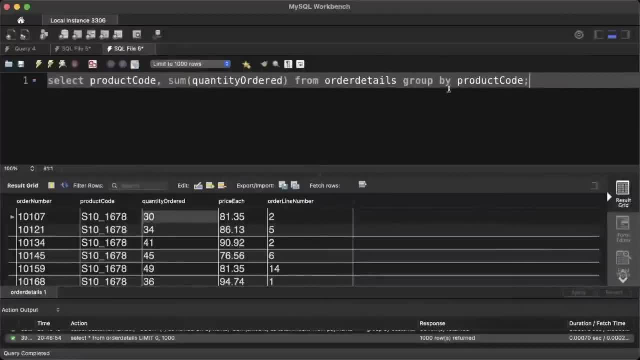 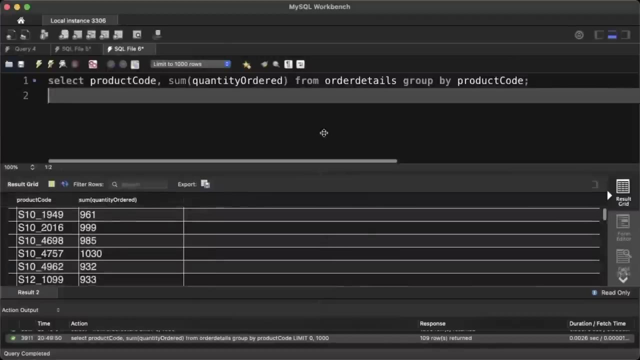 So now what we're saying is we want to Group the rows in order number, in order details, by the product code, And for each product code we want to take a sum of the quantity ordered column. And if we do that and run this query, you should see here that we have the product code. 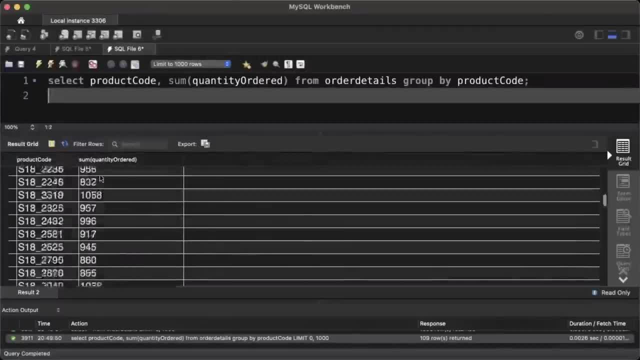 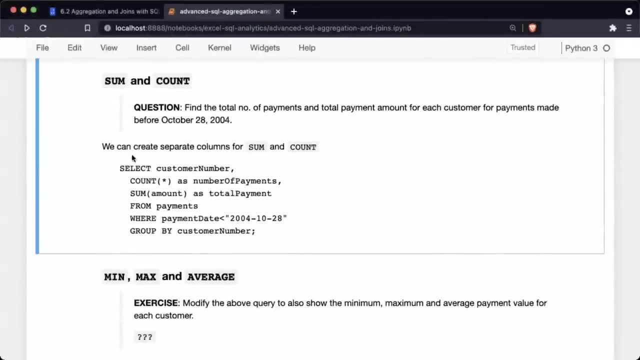 And then for each product code, we have the quantity ordered. Okay, And that's how you answer this question. again becomes easier to understand once you try it yourself. So here's how I would go about solving Uh, working through this notebook. just read the question. 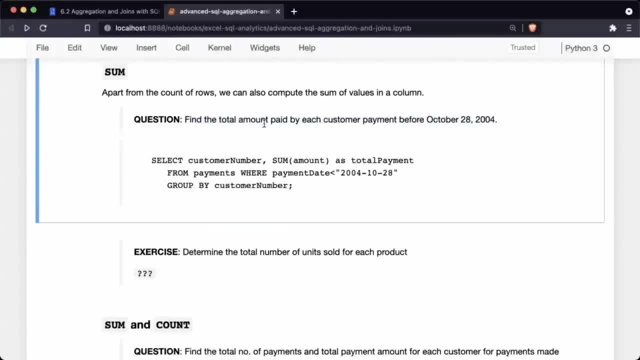 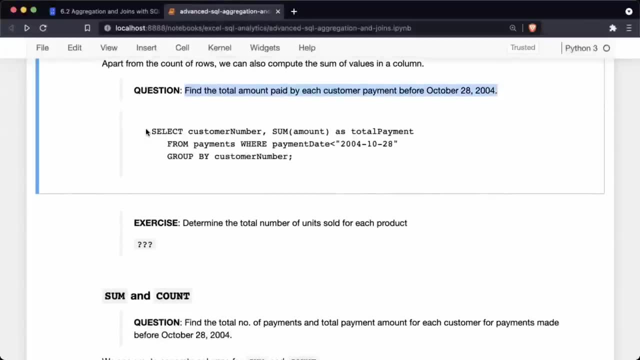 Don't look at the answer. Just immediately go to your SQL workbench and then start typing out and start figuring out how to solve the question. And if you're able to solve the question, great. If you're not, then you can look at the answer. and, uh, again, don't copy paste the answer. 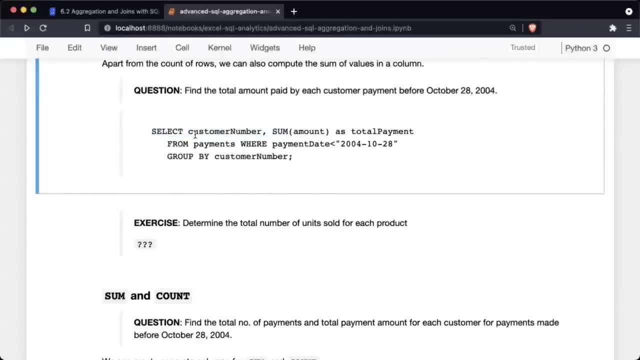 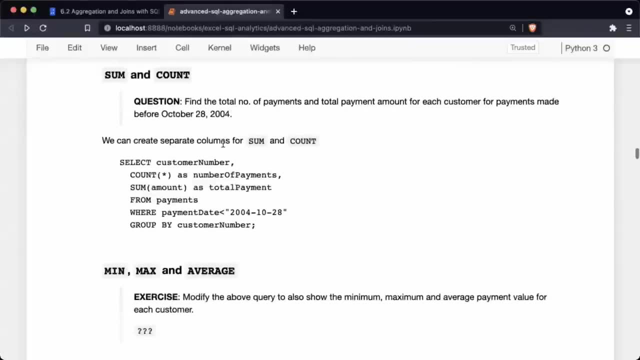 Look at the answer, maybe for a couple of minutes, try and understand what it does and then go back and try to type it out Again. typing out code is a very important part of becoming familiar with SQL or Python or coding in general. 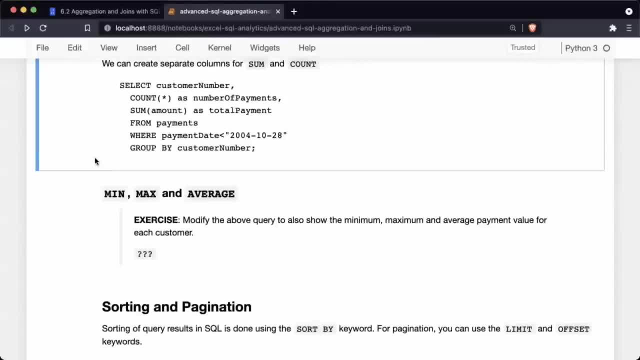 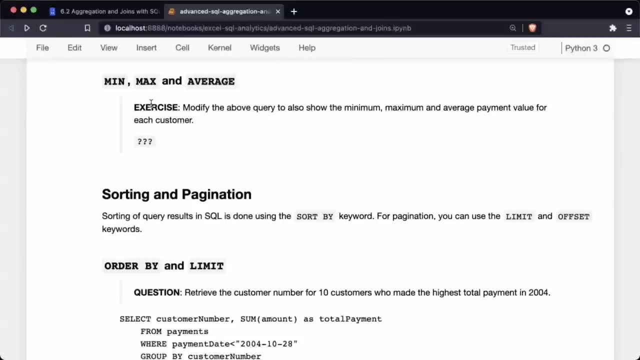 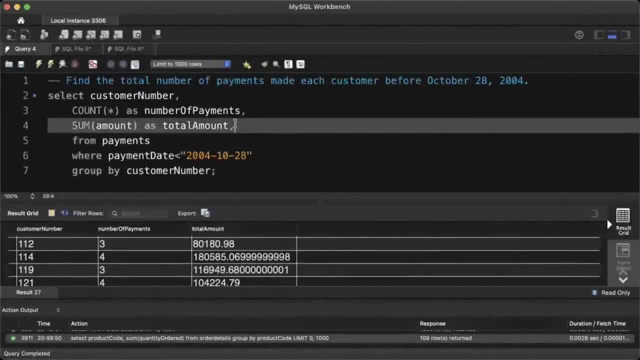 Okay Now, apart from some and count, you can also do the min, max and average. For example, if you want to figure out what was the maximum payment made by each customer before a certain date, you can do that. All you need to do here is in this table you can maybe just add max amount as a- let's just call it- larger than or equal to the maximum amount. 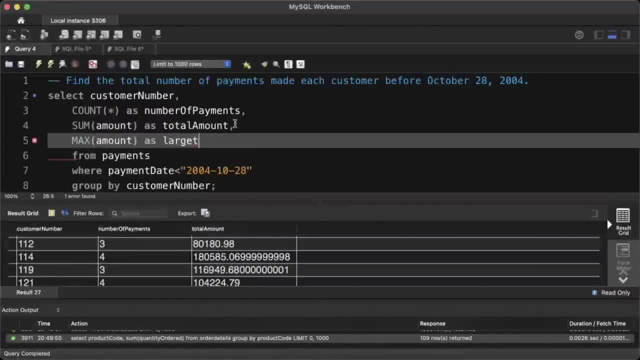 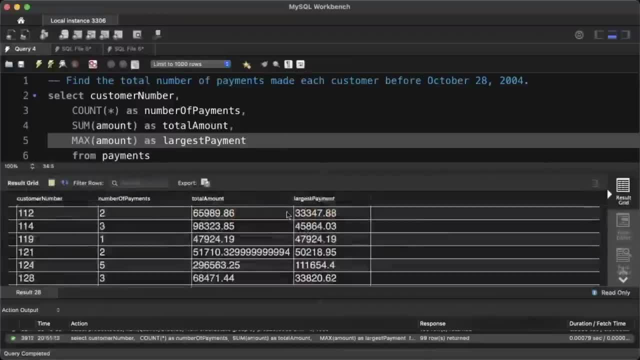 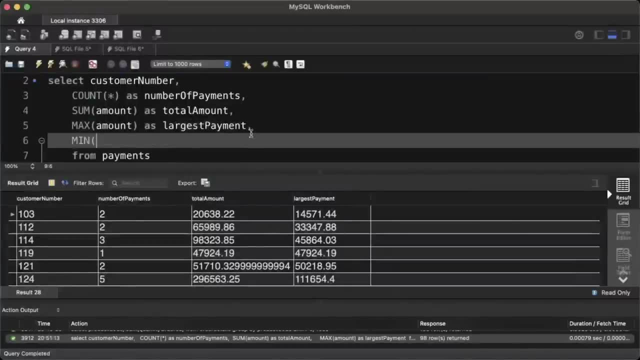 So now you have for each customer what is the largest payment they've made, And you can see: this year the largest payment that they've made is a four. This person has made as a $14,000, but they can also- you can also- add the minimum amount that they've paid. 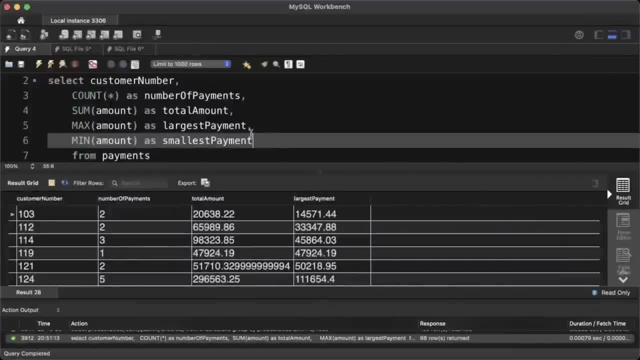 So smallest payment. So the smallest payment they've made is 32,000.. So already we're getting some insights. It turns out that in this case, customer The largest, the largest payment is $14,000 and the smallest is 6,000, but for one one, two, the largest payment is 33,000 and the smallest is 32.. 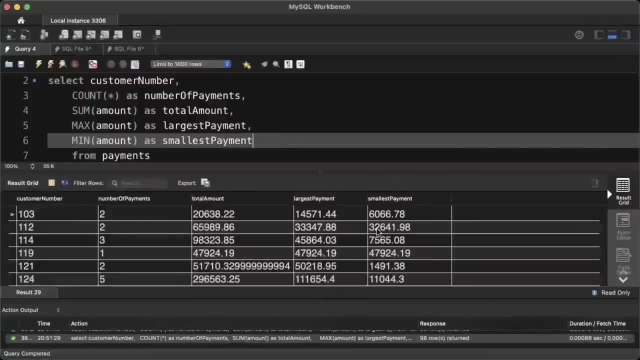 So maybe this customer is just clearing bills as soon as they hit a certain amount, right? You can also then look at the average payment. So what is the average order amount? I think it is average, Okay. So what is the average amount? 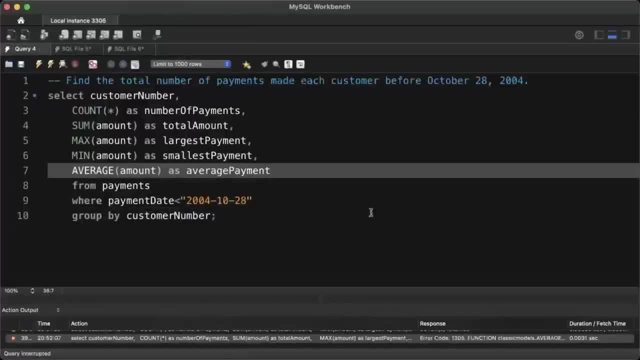 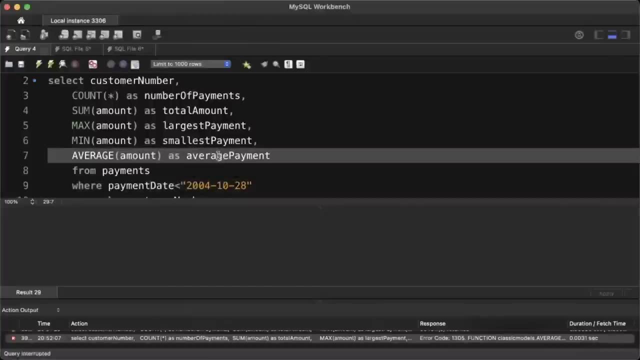 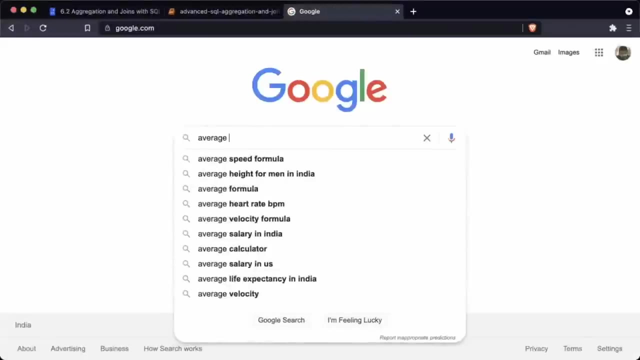 And this is the average payment. So that's the average. So we can see there's an issue here. Okay, I think there's a an issue here. Um, I'm not sure what the average is called, but let's see average, my sequel. 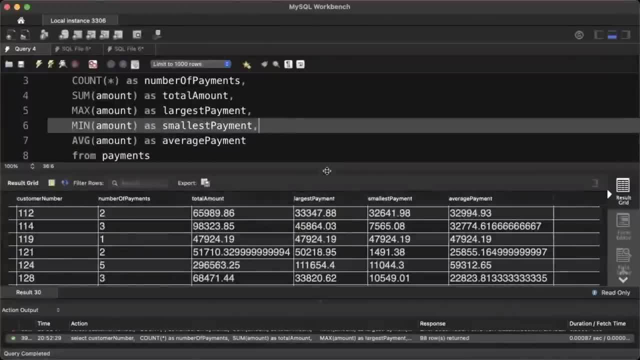 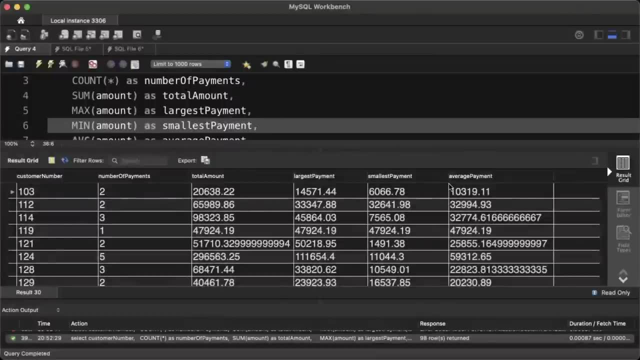 It's called ABG, So let me just change that to ABG. Yup, So ABG is the function name here And you can see that. So you can do basic analysis directly within SQL. You don't even have to export the data. 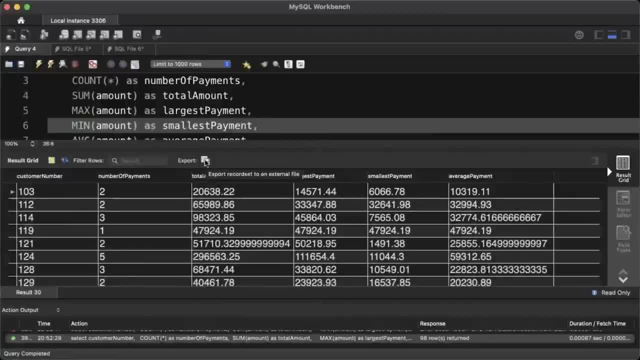 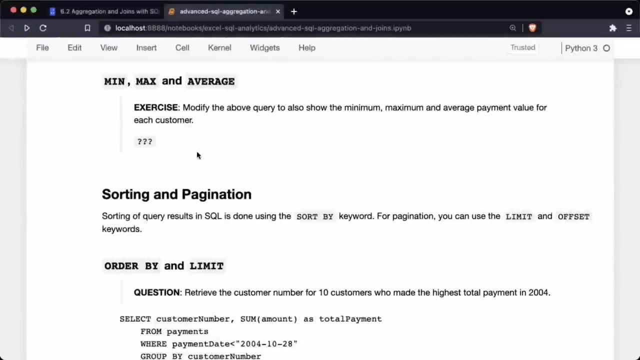 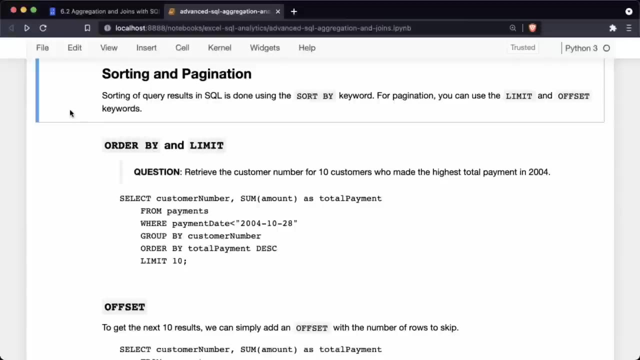 Although, if you want, you could export it to a CSV file. Uh, that's an option from the MySQL workbench, but a lot of analysis can be done directly within SQL. Okay, So let's talk about sorting and pagination Now. so far we've been doing all these queries and through these queries, 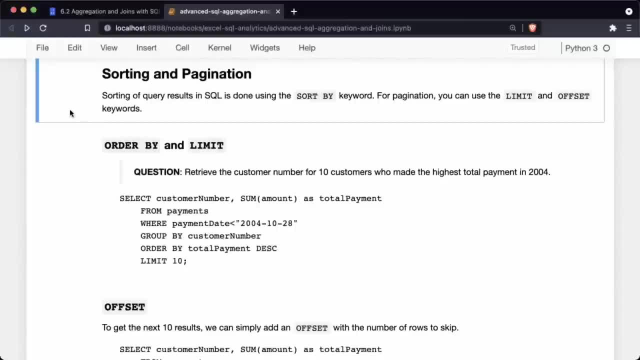 we get a lot of information, but in a lot of cases we are looking. we're interested in finding the top 10 or top five or the maximum value. So here's an example: retrieve the customer numbers for the 10 customers who made. the highest total payments in 2004.. Or actually, let me change that to before October 28, 2004.. Okay, So retrieve the customer number for a customer numbers for 10 customers who made the highest payments total payment before October 28, 2004.. 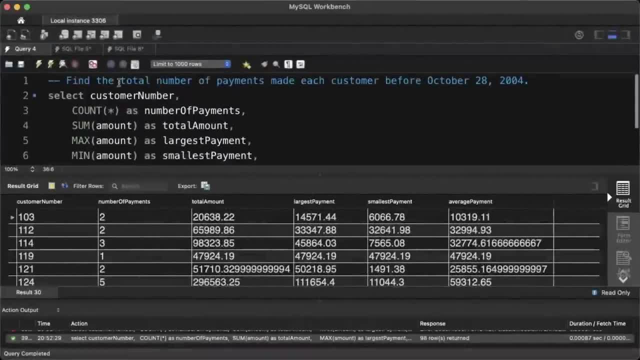 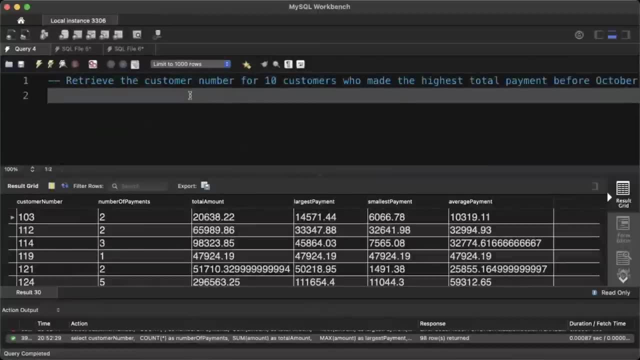 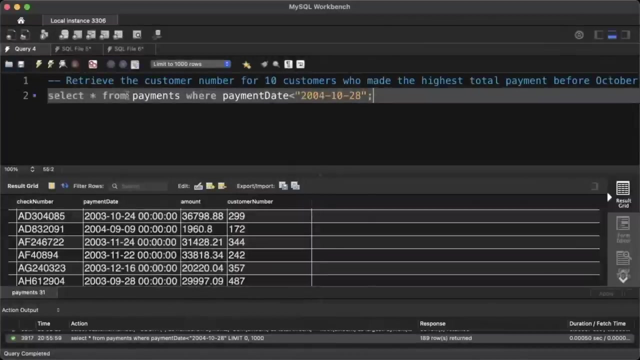 So let's try and answer this step by step. We want to retrieve the customer number so we can say select star from payments, And once again, we are interested in payment date before 2004.. October 28,? great, We have that information. but now we want to retrieve. uh, we were 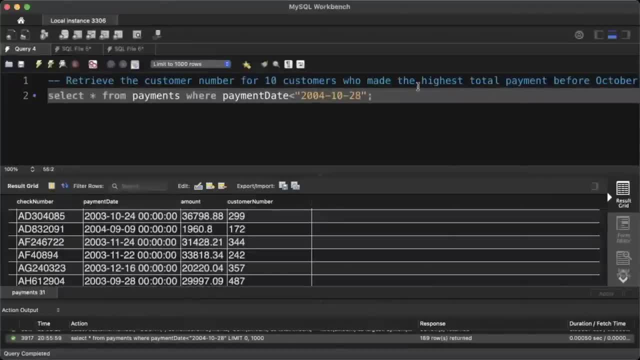 interested in the highest total payment. So before that we're interested in the total payment per customer. So if we do this, if we do a group by customer number, and then we do- uh, we select the customer number for each group and then we do a sum of the amount- column. 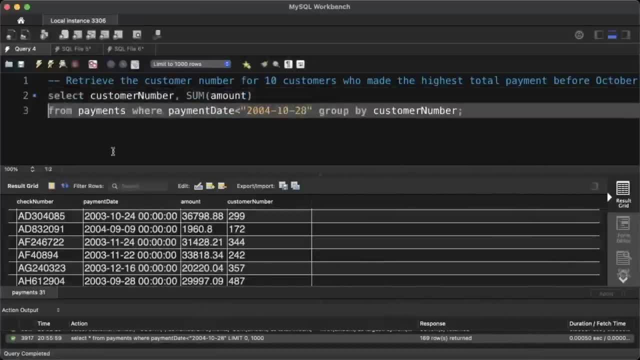 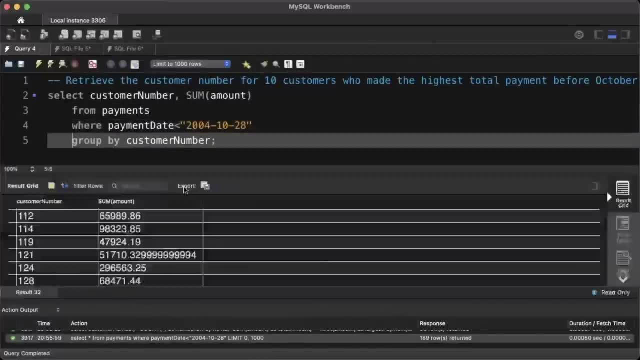 So now what that gives us is the total, the total amount paid by each customer before October 28, 2004.. So we have that, but now we're interested in the people who made the highest total payment. So here's what we can do. 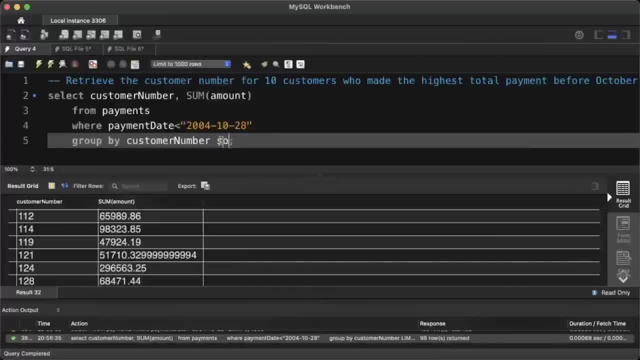 We can type at the end: uh, order by. so we type order by and then we tell the column name that we want to order by. So we want to order by this column, which is the sum, the total amount. So let me just type order by. 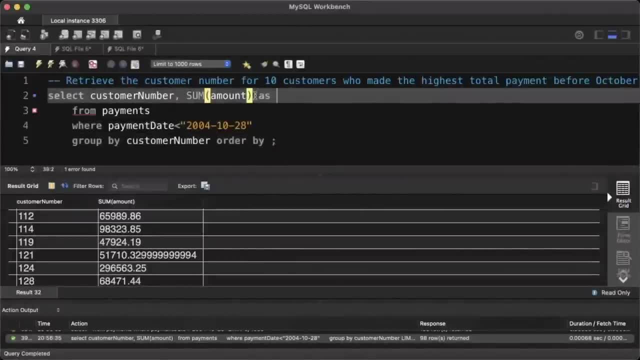 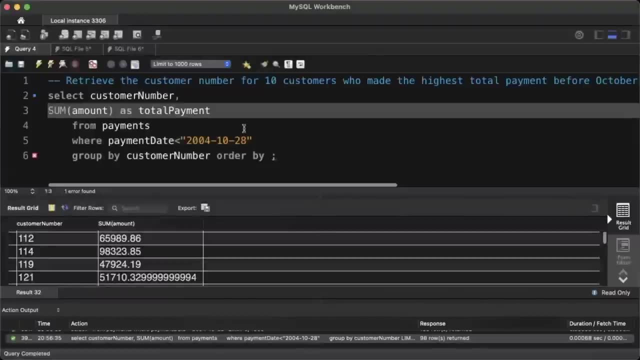 So let me just type order by, Okay. So let me just rename this as total payment. So I'm going to call this column the sum column, I'm going to call it total payment and I want to order it by total payment. 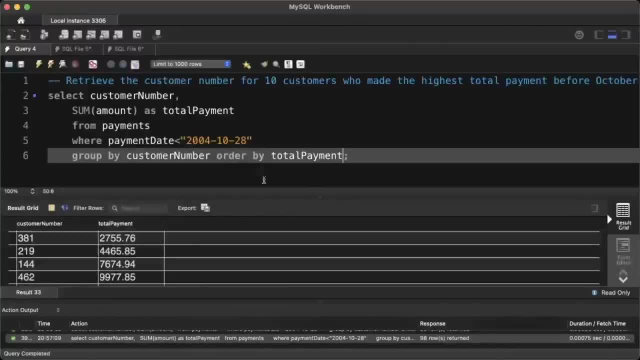 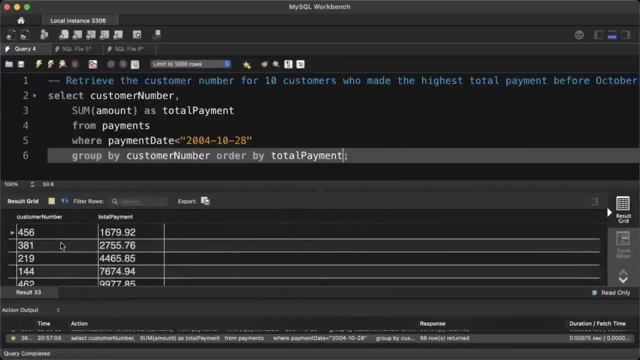 So let's run that and order by generally comes at the very end. So now you have customer number four, 56. They have a total payment of 1, 6, 7, 9. customer number 3, 81, has 2, 7, 5, 5, and so on. 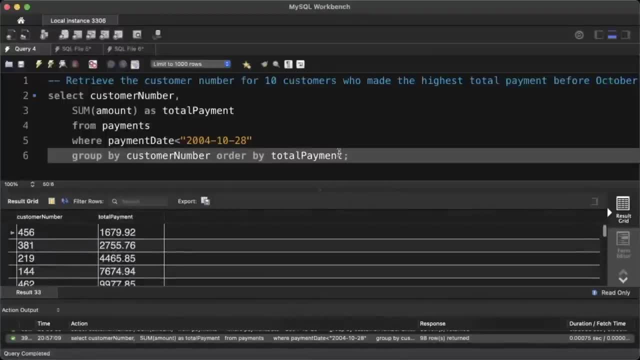 Uh, but of course we are interested not in the lowest. So this is ordered in ascending order, but we are interested in the highest. So to do that, you type D E S C, descending, So A A S C for ascending and D E S C for descending, and let's run that. 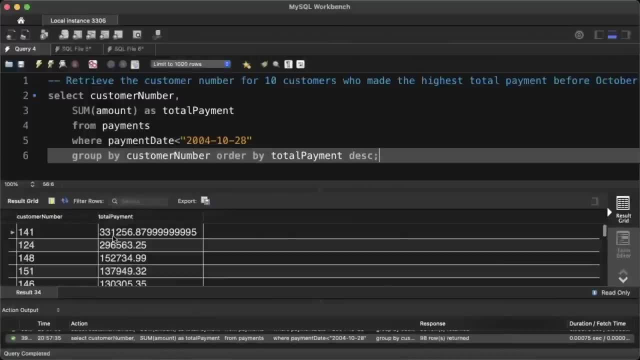 So now you have the maximum value: 31, 33,, 331,000, $256 was spent by customer number 141.. Okay, And we have this information for all the customers, but the Question asks only for the top 10 customers. 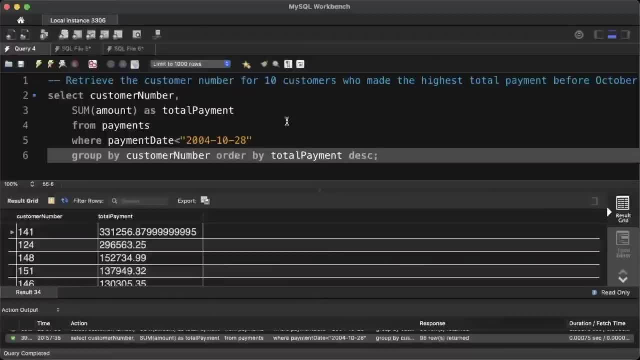 And typically anytime you issue queries like this in a very large database, you probably only want to look at maybe the top 10, the top 50 or the top a hundred. So here's how you can do that: You just call, at the end you type limit and then you tell the number of. 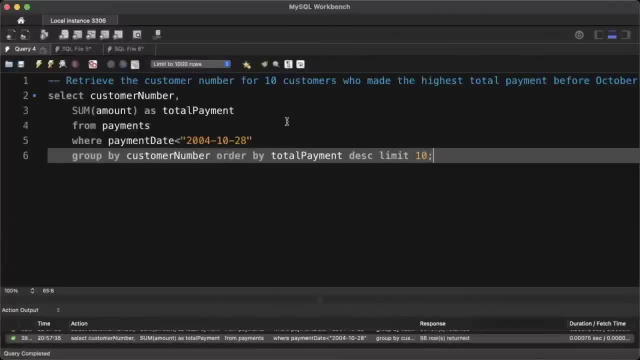 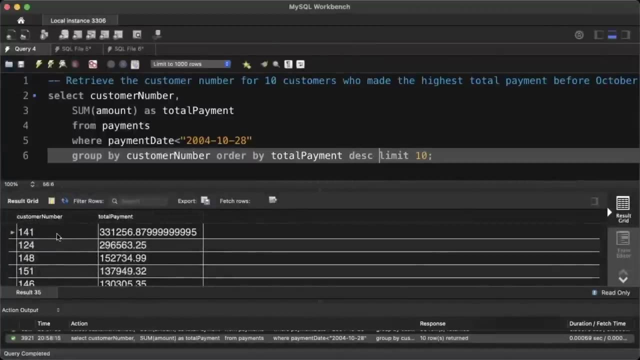 rows that you want to see in the result. Okay, So if I type limit a 10 at the very end, so that's going to just give us 10 results. You can see these are the 10 customers: Uh, one 41, one 24, one 48, one 51,, um, and three 20.. 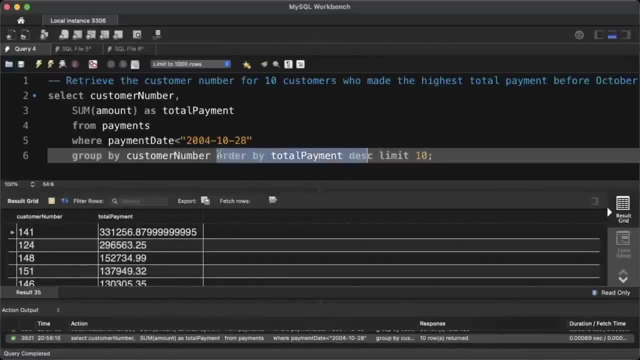 Okay, And, by the way, limit works without order by as well. If you don't need an order, you can do a limit just like this too. So these are both independent, but in general, whenever you're doing an ordering, it's common. 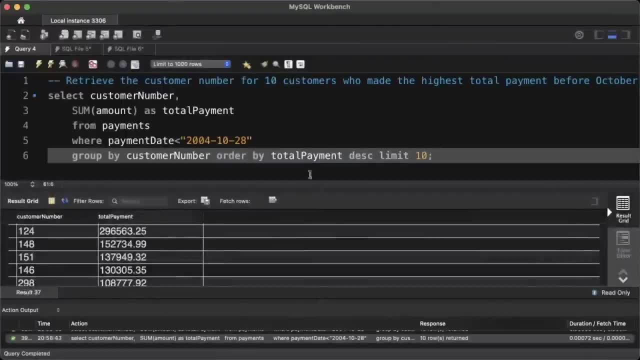 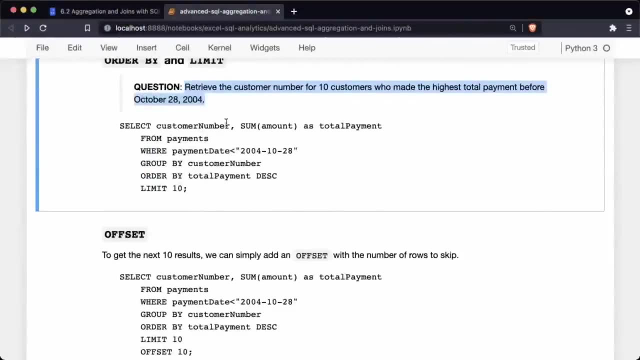 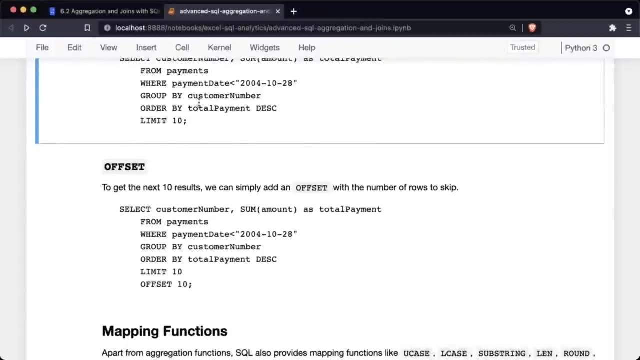 practice to also limit the number of results so as to not put a very heavy load on the database. So that's what we created. So like customer number and some amount as total payment, That's total payment from payments where payment date is less than the value, and we group by customer. 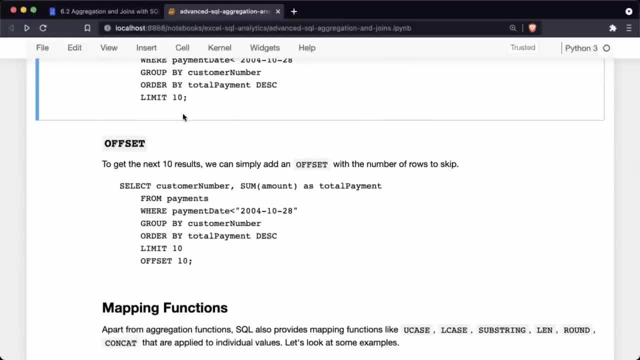 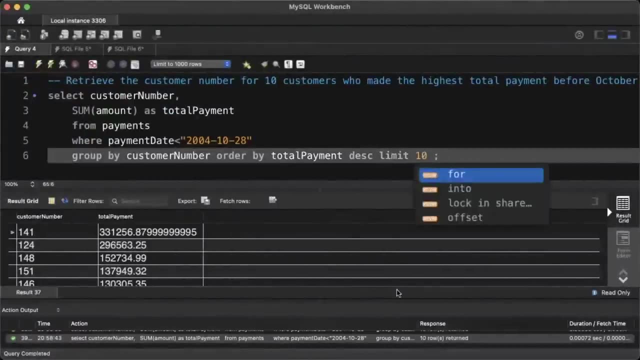 number order by total payment descending, and limit the results to 10.. Now, if you want to see the next 10 results- because we've just limited the results to 10, all we need to do is add an offset. So let's say we want to skip ahead. 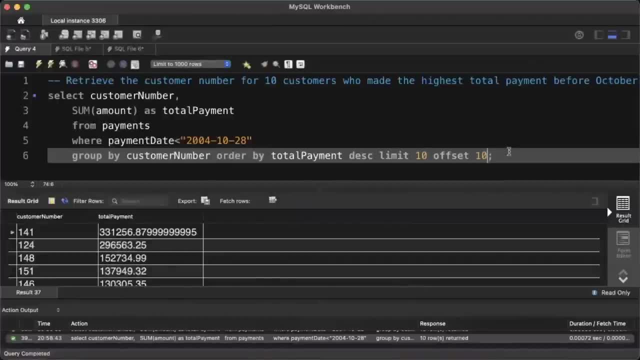 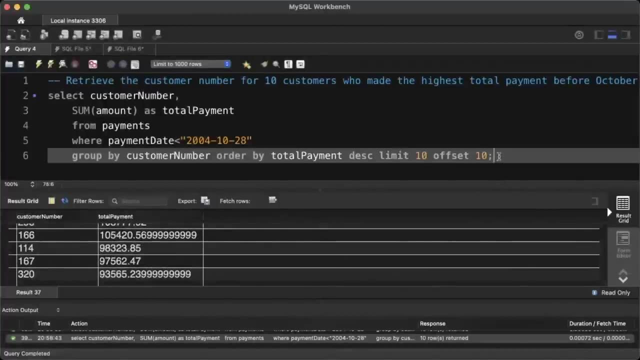 We want to skip the first 10 rows and you want to see the next 10 rows? We type offset 10.. And just notice this number here: three, 20 and nine. three, five, six, five. If I type offset 10, you will see that now we have three, 86,, which is less than the previous value. 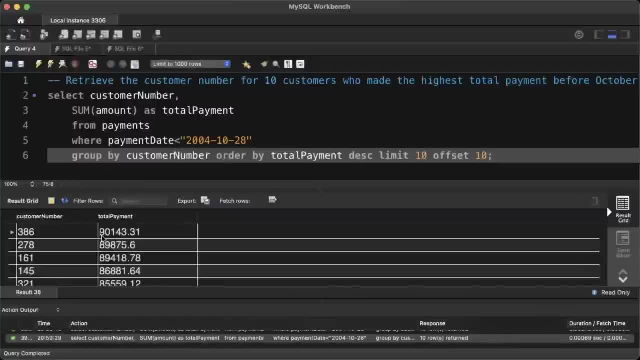 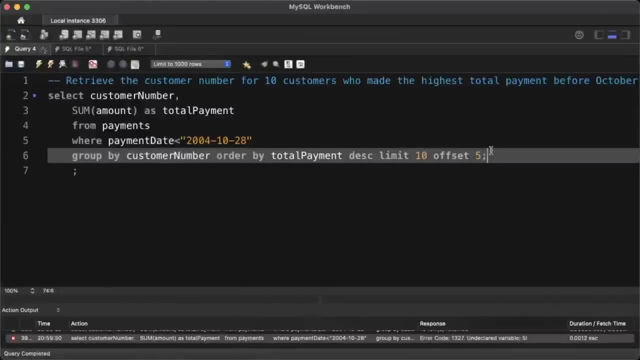 So now I'm no longer looking at the top 10.. I'm looking at the next 10.. So customer number 11 to 20, when they are sorted by the total payment. Uh, and if I, let's say, if I said the offset to five, if I, if I said the opposite, offset to five. 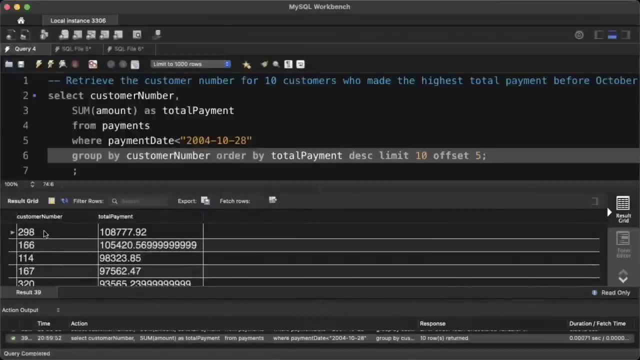 So I'll just skip this query. We'll just skip the first five rows and it'll show me from the sixth row onwards, Right. So limit and offset can be set independently. Limit tells you how many rows you want, Offset tells you how many rows you want to skip. 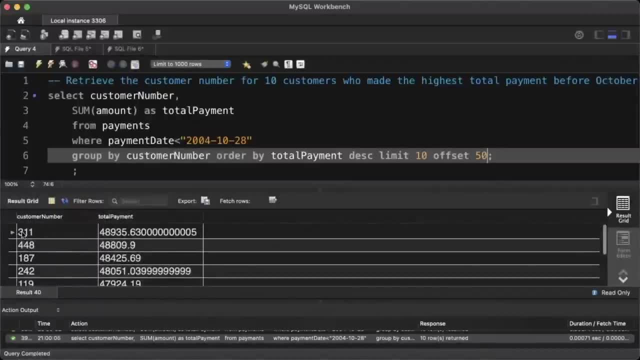 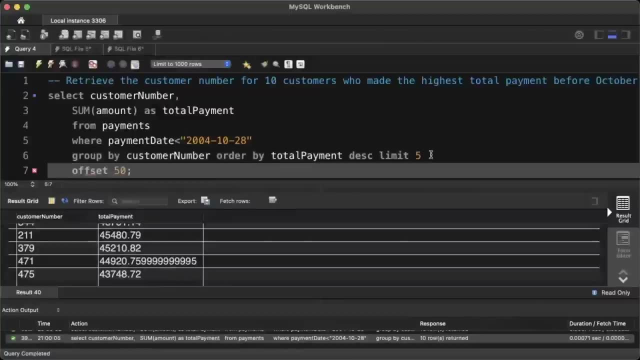 Now here I've skipped the first 50 customers, So I'm looking at customer number 51 to 60. Okay, And I could, maybe even if I wanted, I could look at just five of these. So play around with limit and offset. 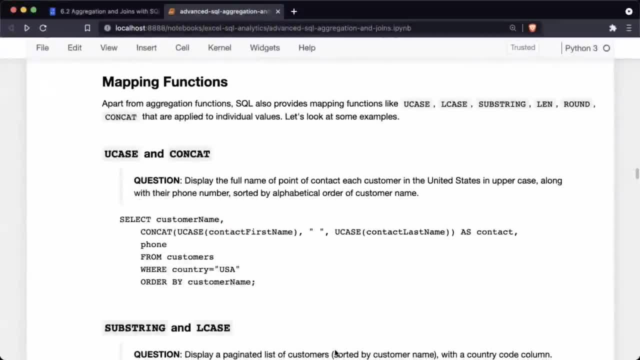 They're used to limit and page, So you can just imagine the queries. SQL also provides mapping functions, and these mapping functions are applied to individual values. So now we no longer combining multiple rows of data, Now we are just applying them to individual values. 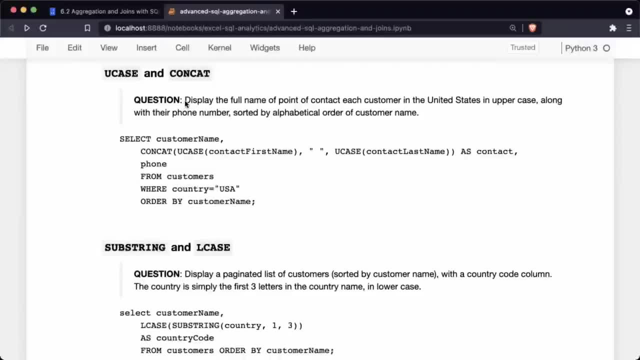 So here is a question: display the full name of the point of contact for each customer in the United States in uppercase, along with their phone number, And we want this information to be sorted by the alphabetical order of customer name. Okay, So there's a lot going on in this question. 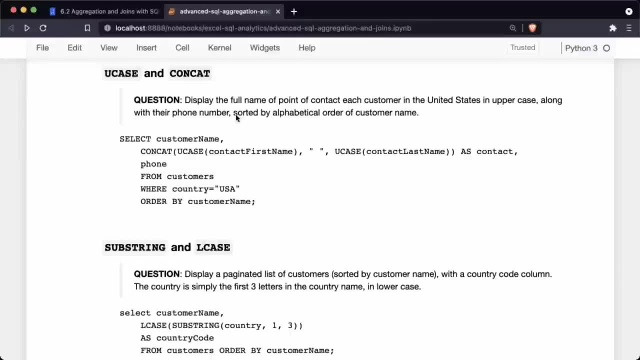 And these are the kinds of questions that you will see in interviews often. and don't feel intimidated, Just go step by step. The first thing here is we want information about customers, So we go here and let's clear all this and we just type select star from customers. 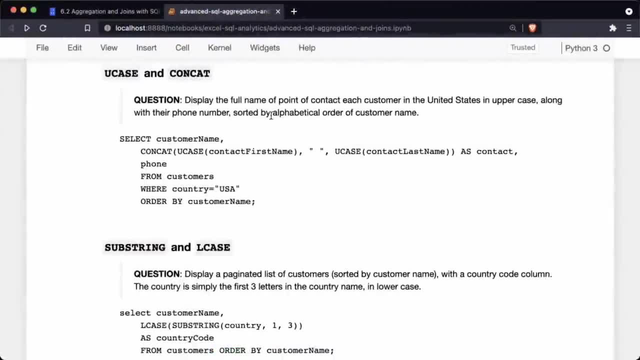 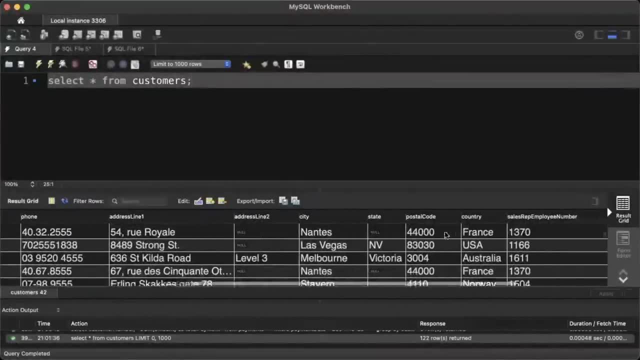 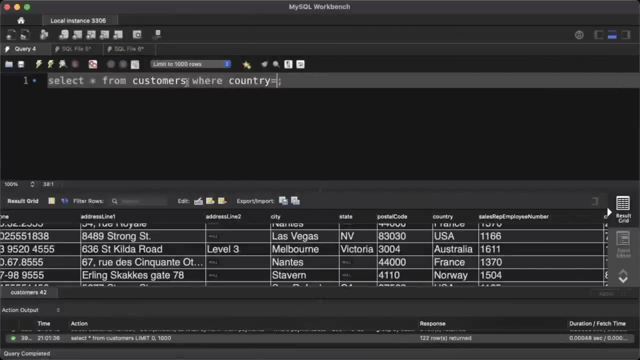 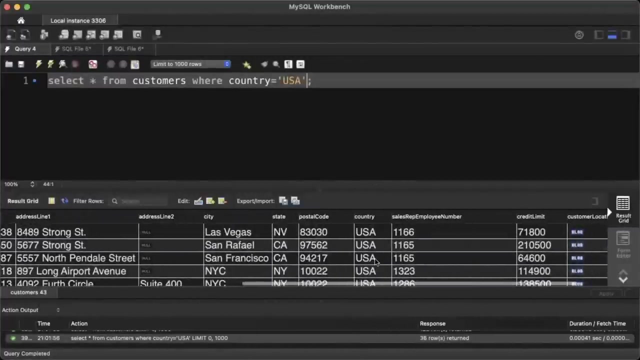 Great, Now we have information about customers. next, We want customers in the United States. So we have what's that? we have this country column and in country we have USA. So if I just type where, country equals USA- So now I'm just looking at customers in the United States and you can check here- then all of the all of them have country USA. 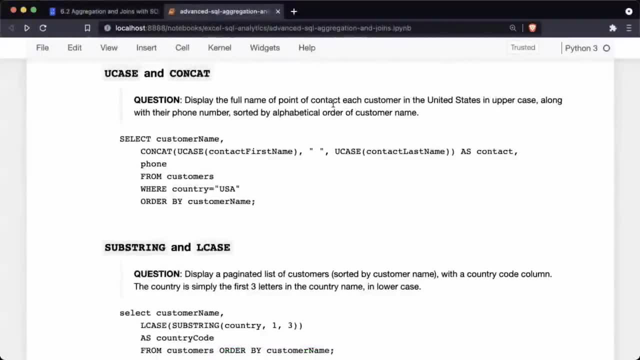 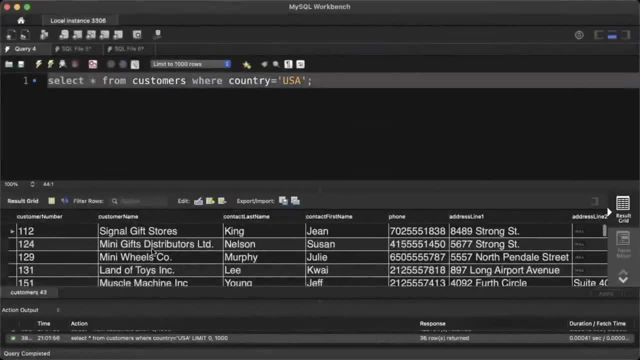 Okay, Great, One more thing done. next, We want to display the Full name of the point of contact for each customer. So if you see, here we have contact first name and we have contact last name, So we could do this. 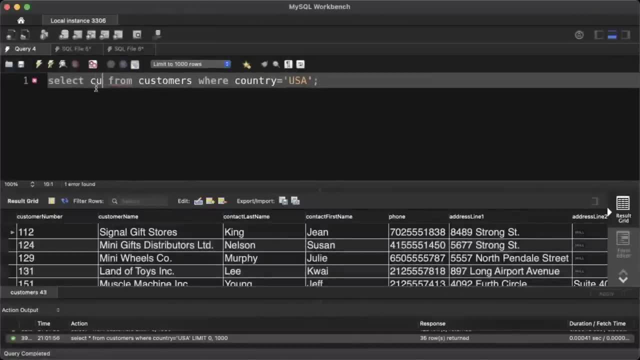 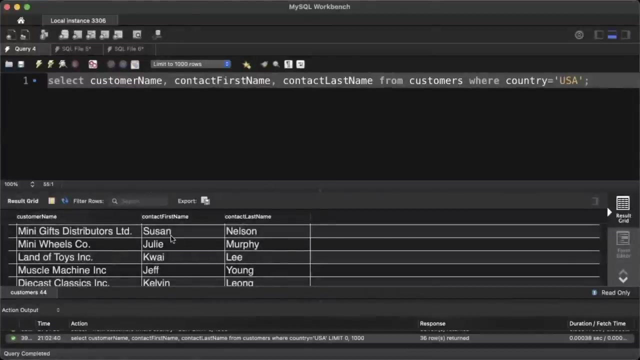 We could just say: let's just print the customer name. I think that is something that we should display, and let us display contact first name and let us display contact last name. Okay, All right. So now we have the customer name, We have the contact first name and contact last name only for those customers where country is set to USA. 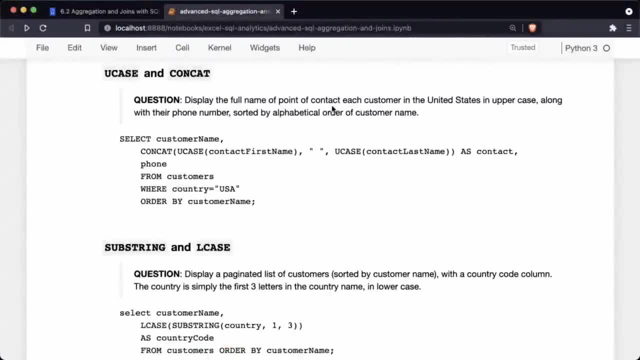 Okay, So display the full name. It's still not the full name. We are showing two separate columns, but we'll figure out that piece. But here it says we want to display these in upper case for some reason, or maybe we want to print them somewhere or copy paste this information somewhere. 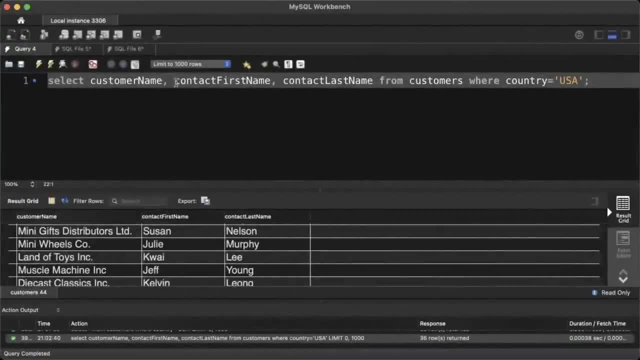 So how do you convert a string into uppercase? Well, there's a function for that. Okay, You just call you case. So you case is going to make it uppercase and L case is going to make it lowercase. So I just call you case on first name and let me maybe do L case for now on contact name. 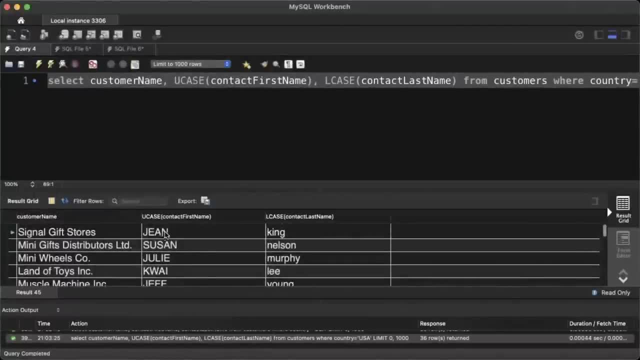 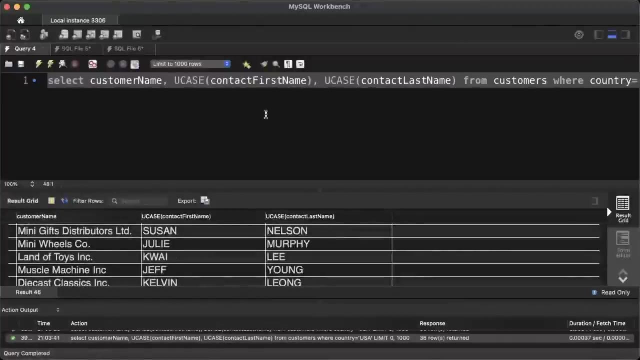 And you can see here, the first name becomes upper, uppercase, all capital letters or uppercase letters, and the last name has become lowercase. Let me turn that into uppercase as well. So now we have both in uppercase and notice that these are not aggregation functions. 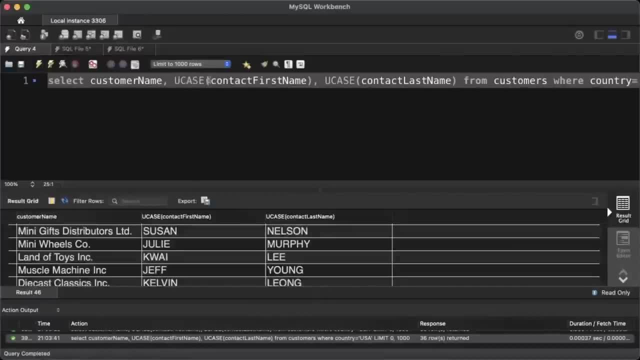 They did not combine all the rows into a single value. They applied this function uppercase to every individual value. So this was applied to Susan, It was applied to this row and this row and this row, and so on. Okay, So that's why these are called mapping values. 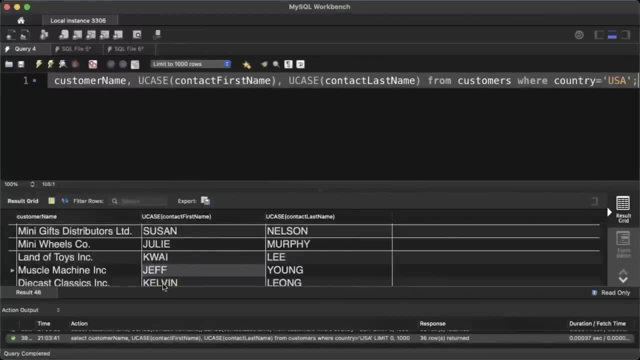 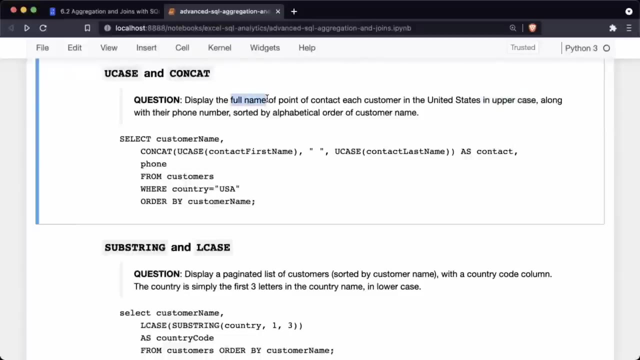 They take a column and the map that column onto a based on a function. So that's why these are called mapping Functions. Now, last bit here is- or maybe a couple more things left- One is display the full name. So you want to take the first name and last name and we want to combine them. 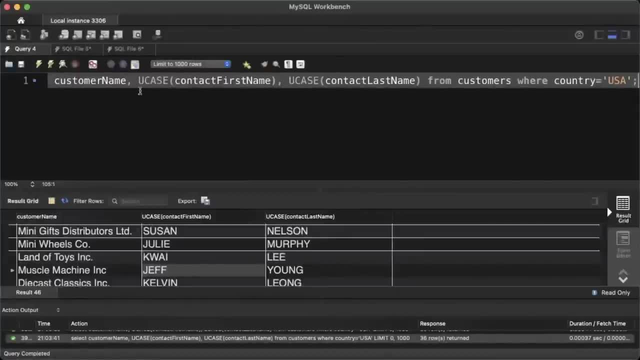 So there are certain functions which can combine columns, and the combination that we want to use here is called concat. Concat is short for concatenation, So I'm just going to call concat here. C O N C A T, And let me drop this for a moment. 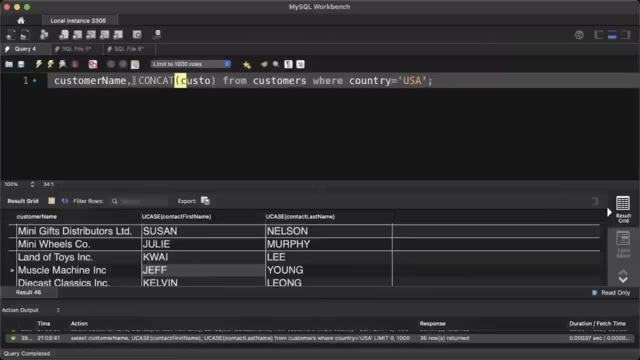 Let me just get rid of these and I'm just going to do customer first name and- oh sorry, this is contact, So contact first name and contact last name. So now we've combined contact first name and contact last name, but there's a problem here. 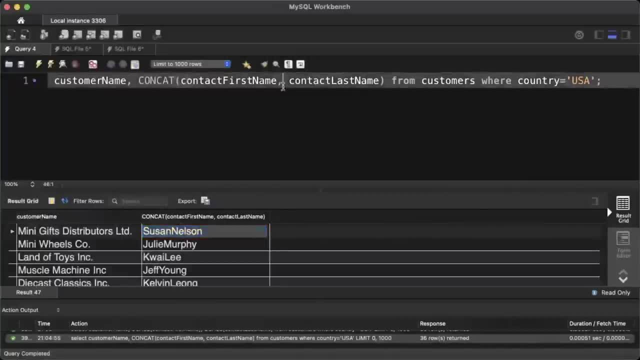 You see, Susan Nelson is. there's no space between them. Well, that's easy to fix. You just add a space here and now you have Susan Nelson And we want to make this uppercase. So now, concat, first name, et cetera, is the uh string that we're dealing with or is a column that we're dealing with? 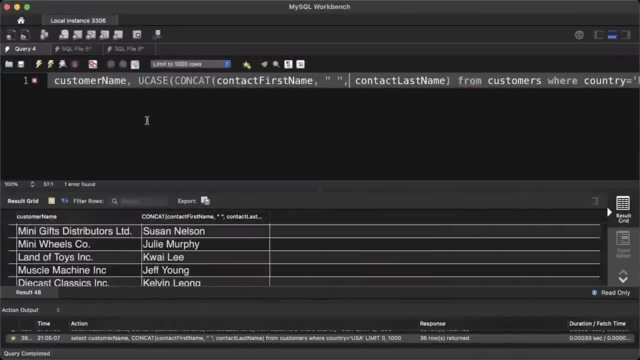 So we just called you case here, and that is going to now make that uppercase. Now you could do it two ways. You could apply it to each column first and then concatenate them, or you could apply it outside. Both will do the same. 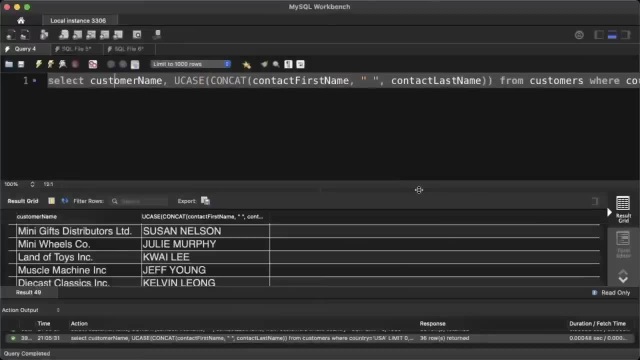 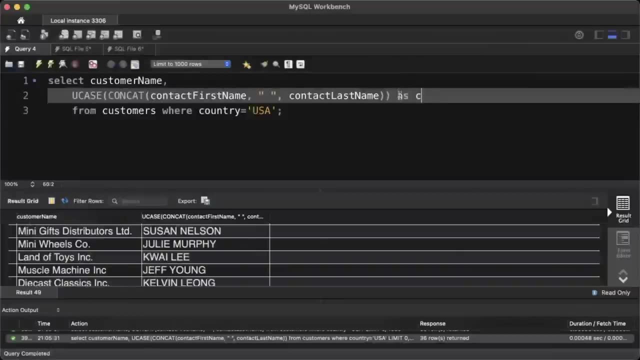 So now we have that. one last piece of cleanup is- let me just get this on. a new line is to simply get: Uh, this is simply rename this column, So I'm just going to call this contact name. Okay, So we concatenate first name and last name with a space between them, convert that to uppercase, call it contact name and list it out. 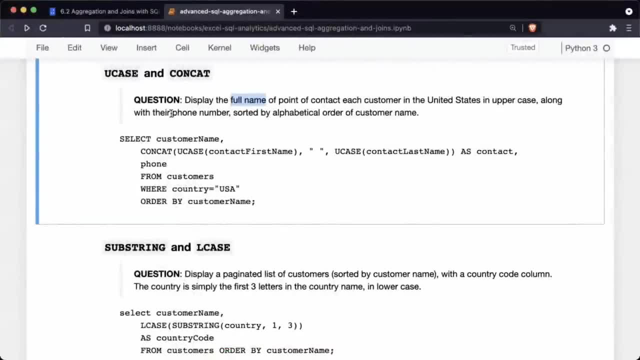 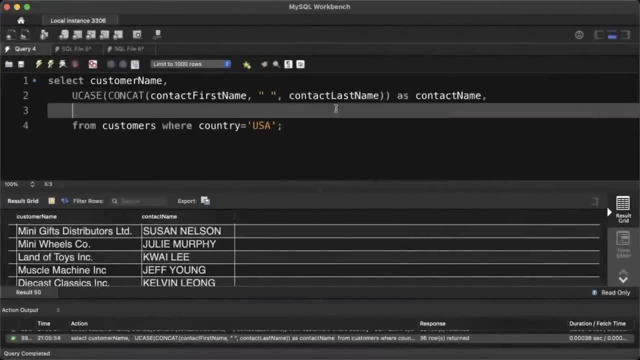 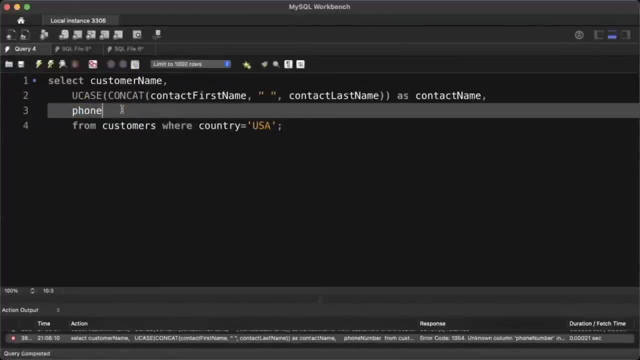 One last thing. we also want to display their phone number and we want to sort by the alphabetical order of the customer name. So let's display phone number here. Let's just put in comma phone number. I think it's just called phone, if I'm not mistaken. 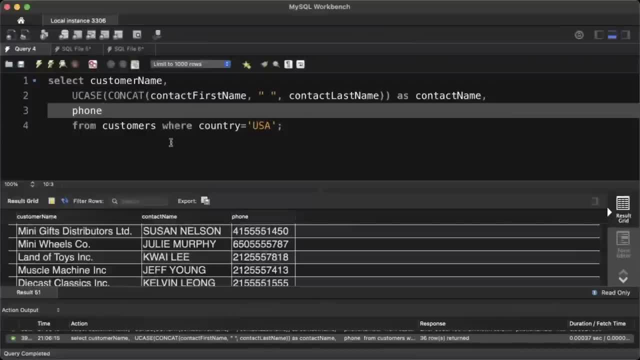 Yeah, So now we have customer name, contact name, phone and we want to order them. So we just put in order by and here we put in what was that number customer? We want to order by customer name in alphabetical order. 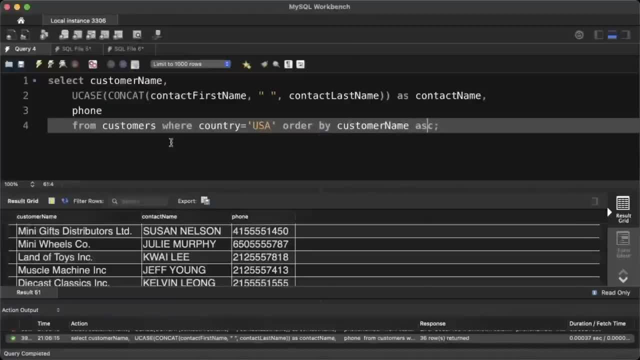 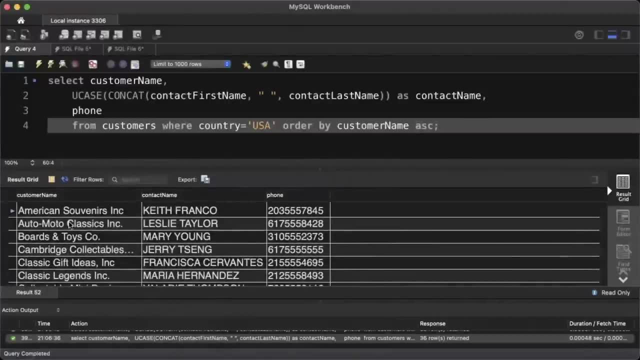 So we can even just put in ASC here, or ascending to mean increasing alphabetical order. So now you see, we have this customer name, Okay. Okay, So we have American souvenirs, auto moto, classics, board and toys, Cambridge collectibles, classic gift ideas. 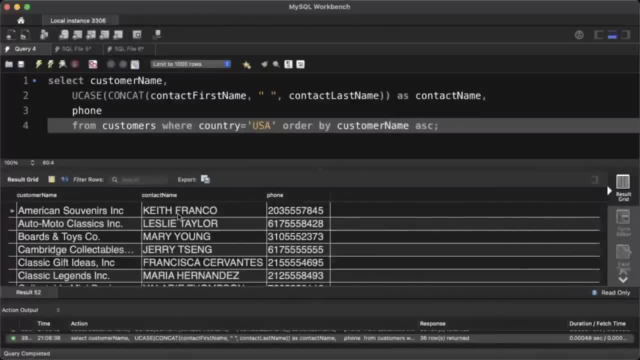 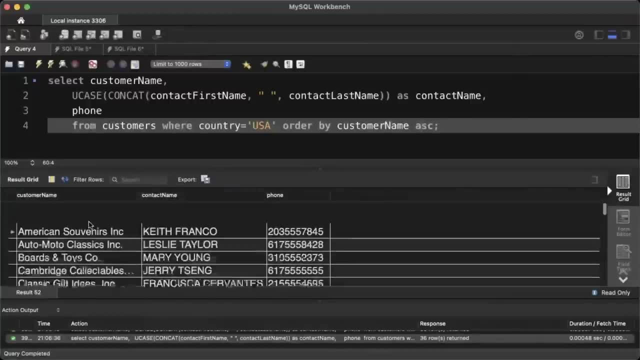 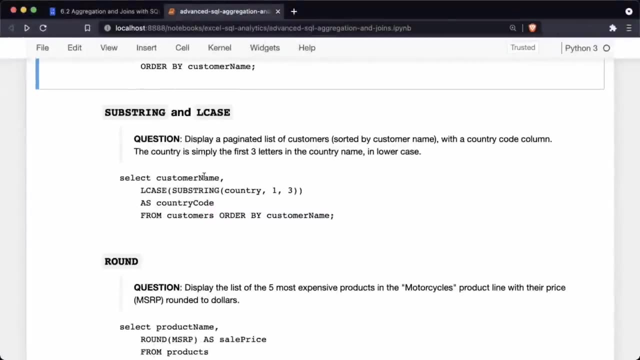 All of these are customers in the? U in the USA. We have the contact name listed in uppercase, We have the phone number of the contact and we have sorted this list in alphabetical order. That's how you answer SQL queries And that's all we're going to do over and over for the rest of the session. 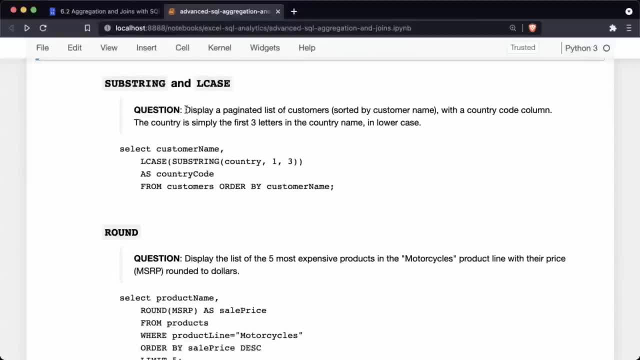 Essentially. Here's another example. This is a paginated list of customers sorted by customer name with a country code column and the country code is simply the first three letters in the country name. They should say country code, So the country code is simply the first three letters in the country name in lowercase. 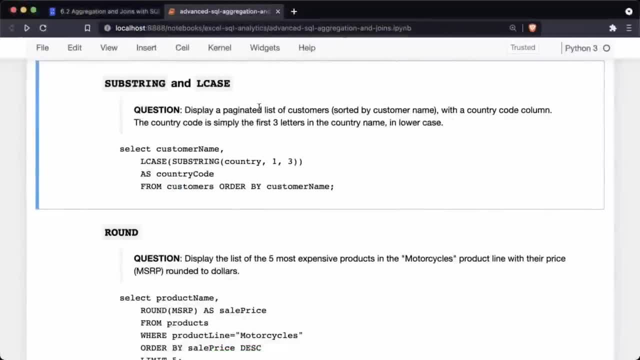 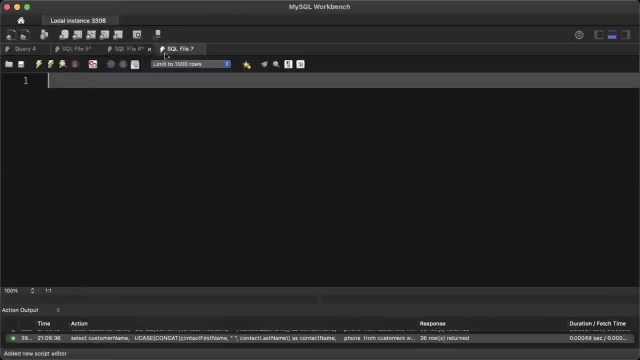 So here's how you can do that. We want to show customer, So just paginated list of customers. So let me just do, let me open a new query here. Let me do Select star from customers and we want to show a paginated list. 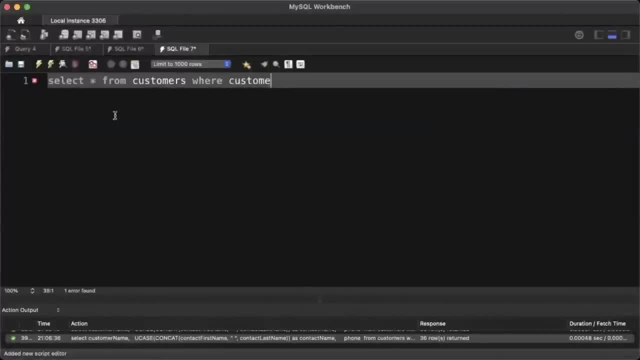 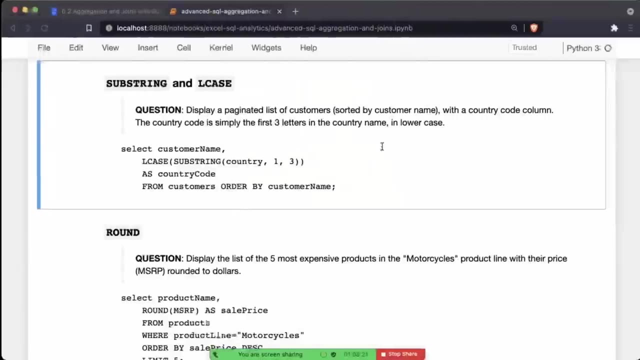 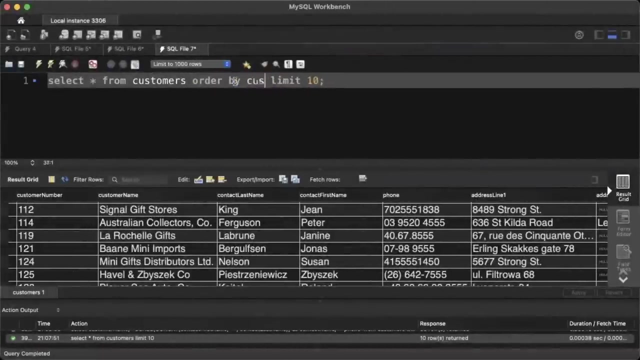 So we want to show where, um sorry, we want to limit to, let's say, 10 customers, So these are 10 customers. Then we want to sort them by customer name. So let's do order by. all right, It is sorted by customer name. 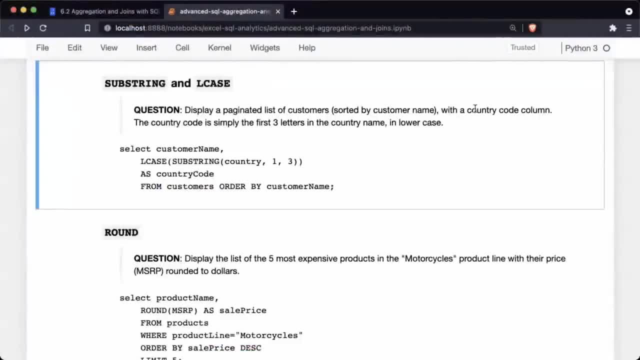 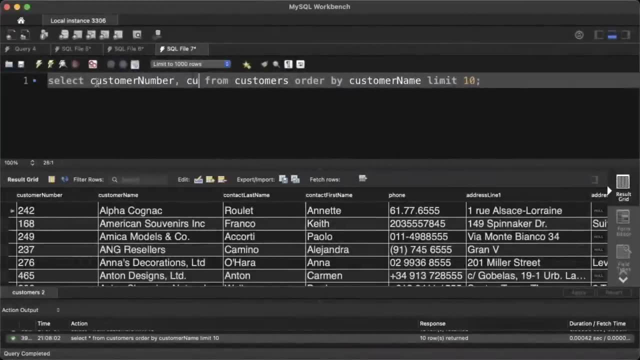 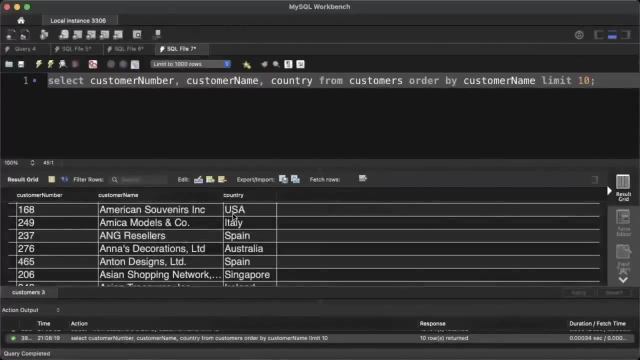 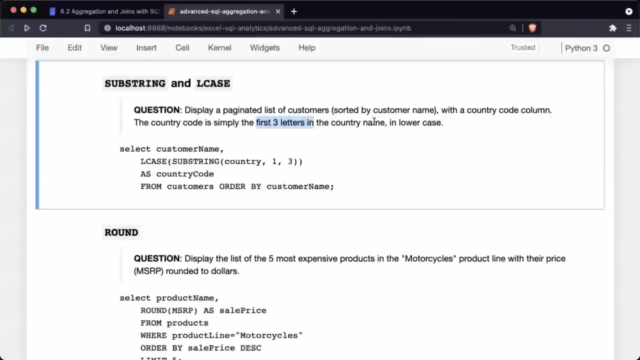 Just fine. And then we want to show country code Column. So maybe let's just show customer number and customer name and country. So now we have customer number, name and country, but we are interested in something called a country code. And what's the country code? the country code is simply the first three letters in the country name in lowercase. 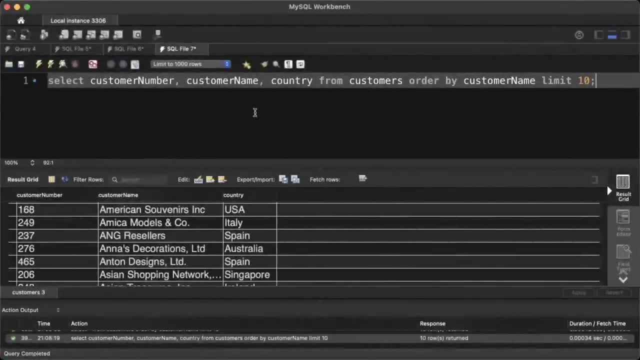 So we want to get the first three letters out of every country name, and that can be done using this sub string function. So instead of country we put in sub string country, and in sub string you specify where you want to start. now in SQL, numbering starts at one, not at zero. 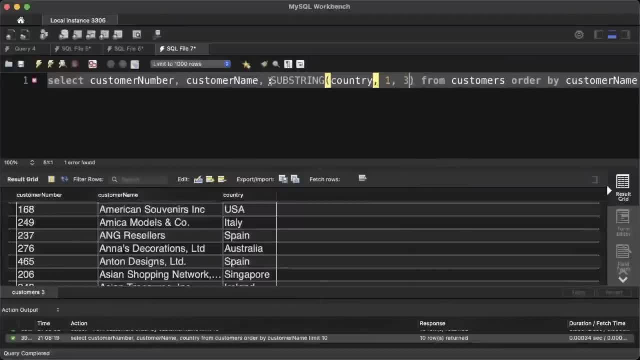 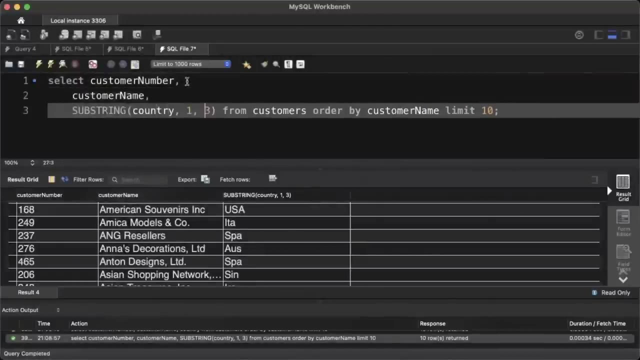 So just be careful about that. And we want to take three values, I think. So we just say one comma three, and yeah, so that gives us just the first three characters of each country name, And let me just clean that up here. 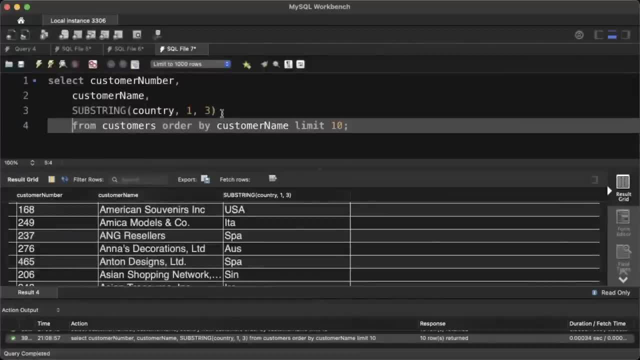 So that gives us the first three characters from each country name but we are interested in. we want to make it lowercase, So we just type L case here and that's going to make it lowercase for us And let's just rename that using as to country code. 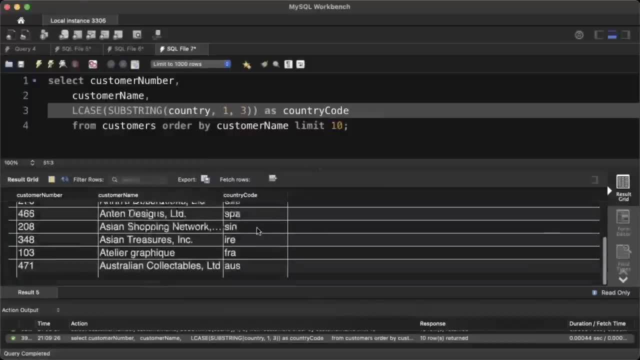 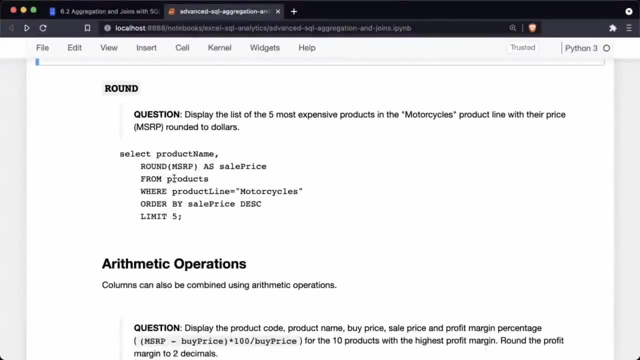 Okay, And there you go. So now, for each customer name, we have a country code. for whatever reason, we need the country code. All right, So that's another function. Here's one last Function: display the list of the five most expensive products in the motorcycles product line, with their price rounded to dollars. 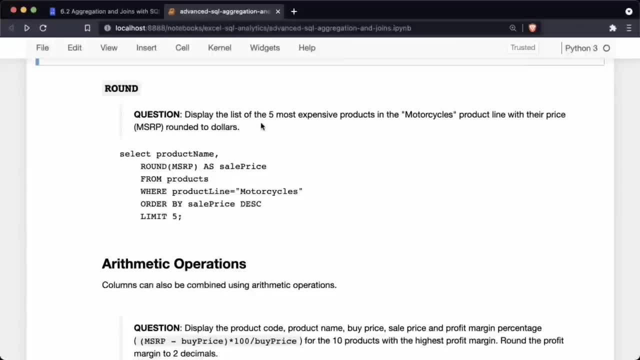 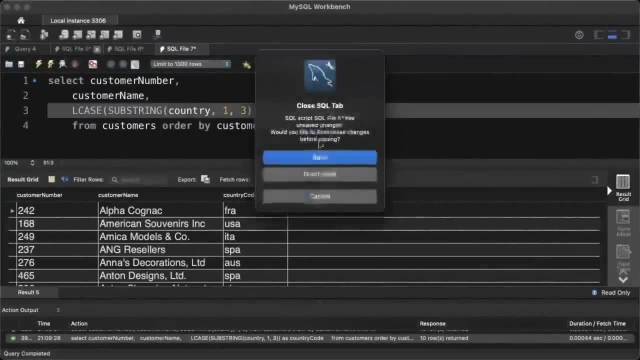 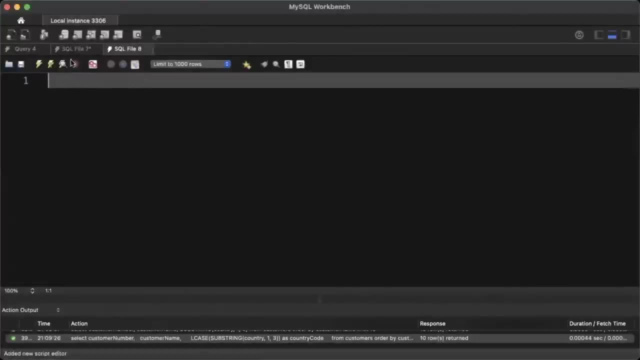 And the price is the MSRP column. Okay, Let's try and answer this to five most expensive products in the motorcycles product line. So let's get rid of some of these, Okay. So let's see select star from products. There's our products, a list of all our products. 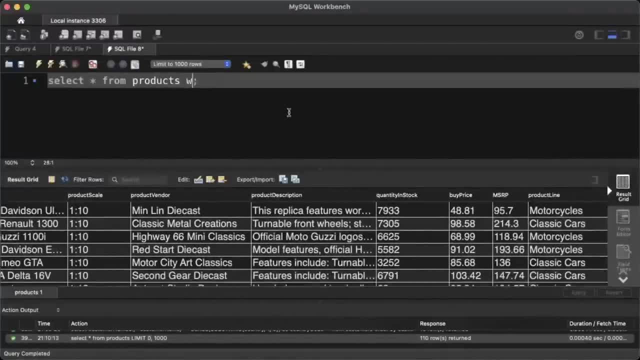 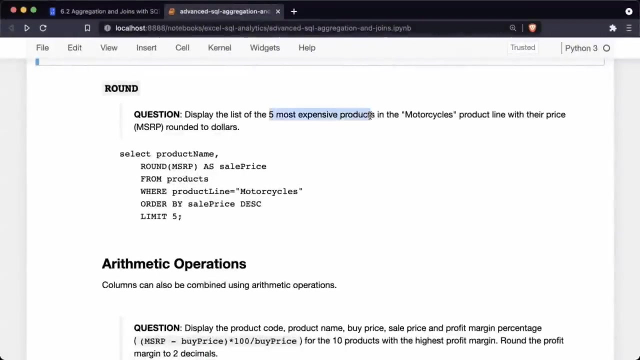 And here one thing you will see is a product line. So we can, we simply want to look at motorcycles. So where product line, the column, product line, has the value motorcycles- Okay, Now we're just looking at motorcycles here And we want to check the five most expensive products. 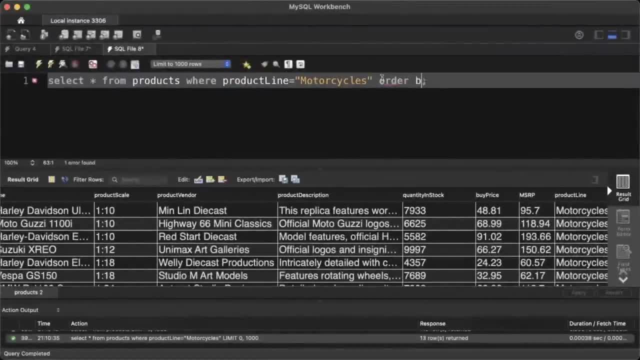 So we let's order them. Let's order by um. MSRP- maximum sale retail price, I guess. Uh, so yeah, we ordered that by MSRP and we can also just type MSRP. It should not be a problem here. 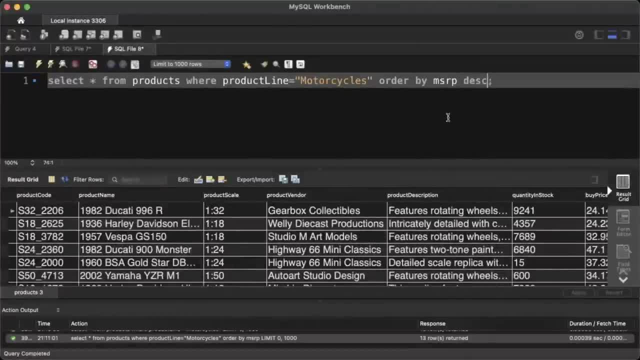 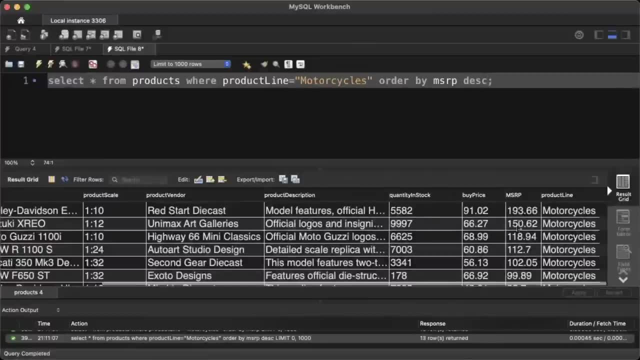 Okay, Now they're ordered by MSRP, but of course we want the most expensive, So we typed the ESC descending. So now you can see that we have only motorcycles and we have ordered them in the decreasing order by MSRP, And we just want to see the top five products. 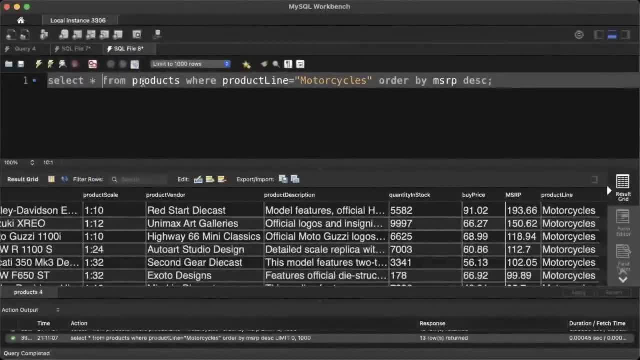 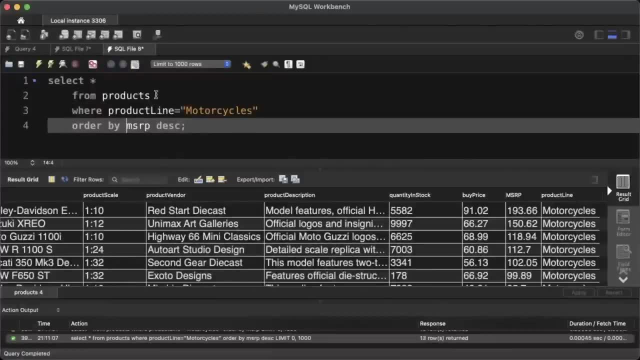 So I'm just going to add a limit here, So let me just move this down. Yeah, So let me just add a limit. order by MSRP descending limit five: So now we have the top five products and maybe we don't need all the columns. 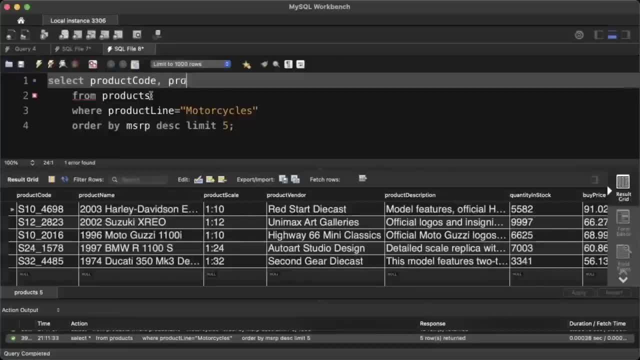 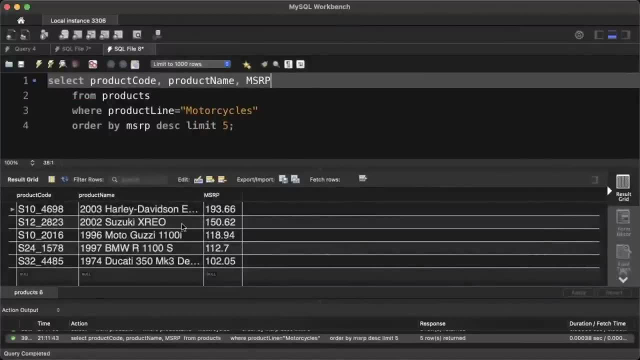 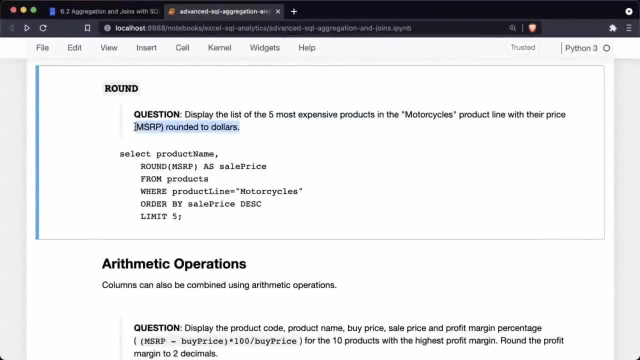 Mostly, we just need, let's say, the product And product name and MSRP. all right, this is the required information. There is one last condition here: We want to round the price to dollars. Maybe we're creating a report where we don't want to show the full price. 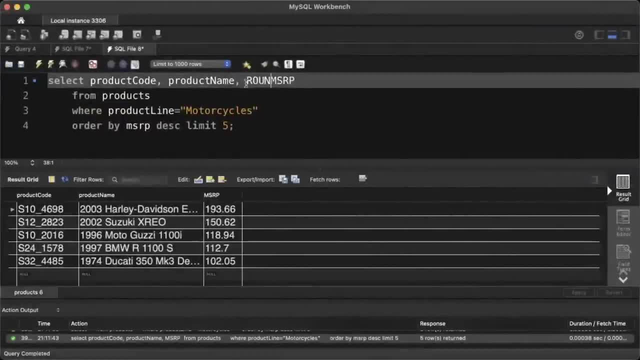 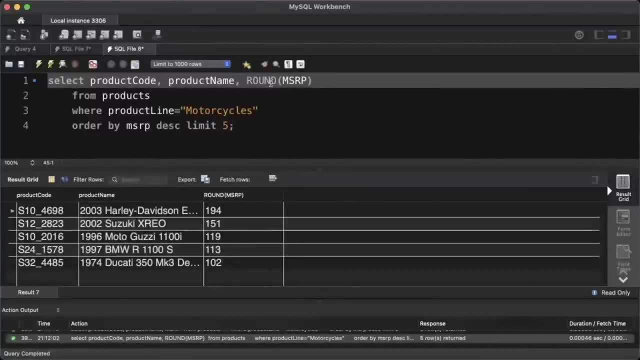 We just want to round it to dollars, And the way you do that is just type round, So round function will do that for you. So now this number is rounded to dollars. You also have a ceiling and a floor, So if you want to round down or round up, you can use those, but round does the job. 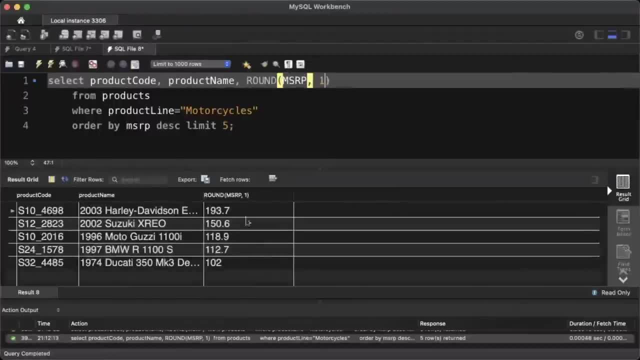 And in round you can also specify the number of decimal points that you're interested in. For example, if you want to see one decimal point, just specify round one. Okay, So that's how you answer this question. five most expensive products in the motorcycle category. 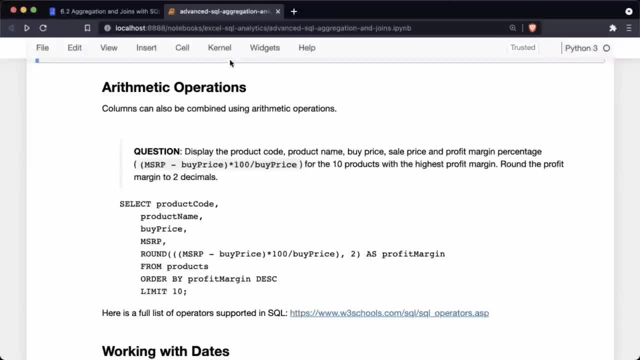 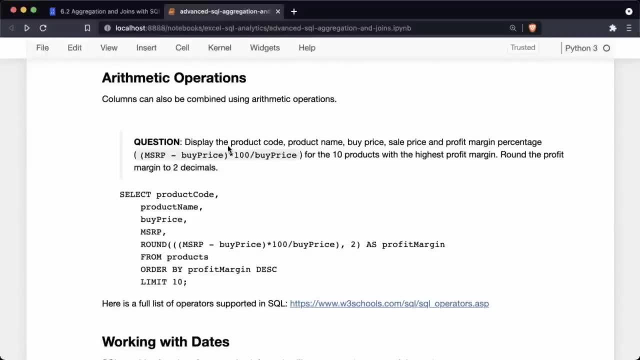 So that was about the mapping functions. You will not. Uh yeah, there are a lot more mapping functions, So you Generally don't need to remember all of them, although it will help again for interviews, for exercises, And as you solve more exercises you will automatically start memorizing them. but there 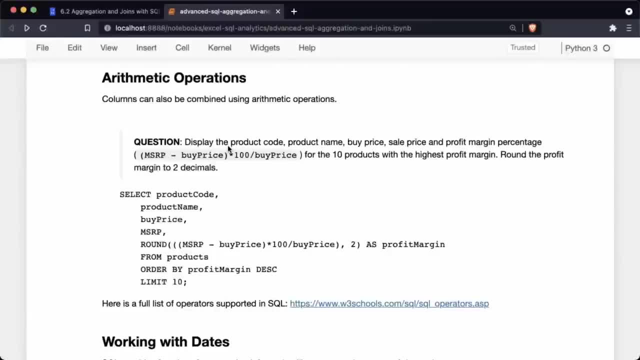 are a bunch of different functions that you can apply to dates and you can apply to numbers and you can apply to strings. all of them And one other kind of function or operation we should look at is arithmetic. You will often have to combine data from multiple columns using arithmetic operations. 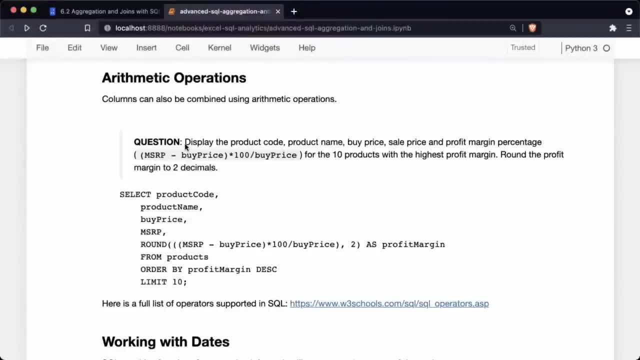 So here's a question: display the product code, product name, buy price, sale price and profit margin percentage. So what's profit margin percentage? Will you buy the product, or maybe you buy the parts for that product at a certain price and then you sell it at a certain price? 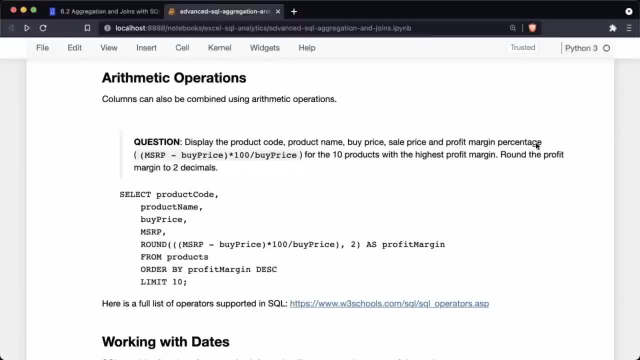 The difference is called the profit and the margin And the percentage is basically the sale price, MSRP minus the buy price, Multiplied by a hundred divided by the buy price. Okay, So that's the profit margin percentage: sale price minus buy price divided by buy price. and convert that to a percentage by: 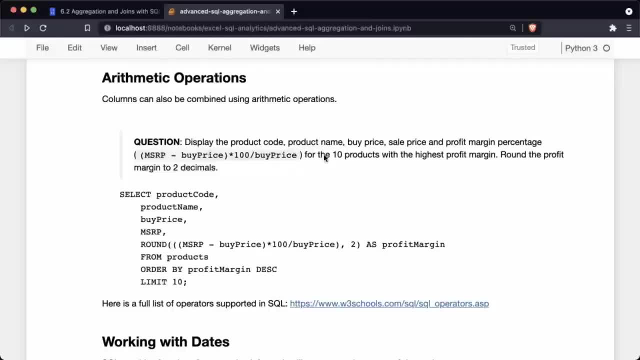 multiplying with a hundred for the 10 products with the highest profit margin. So we want to show the 10 products with the highest profit margin And we also want to run the profit margin to two decimal. So there's a lot going on here. 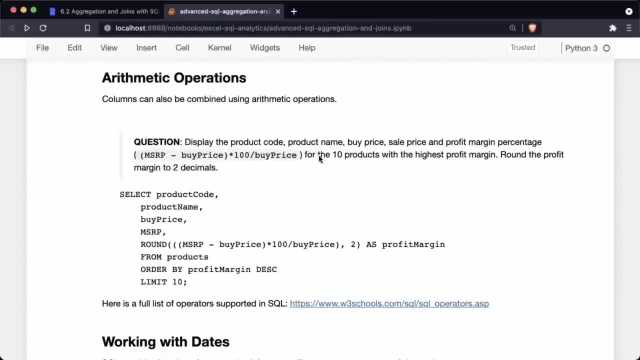 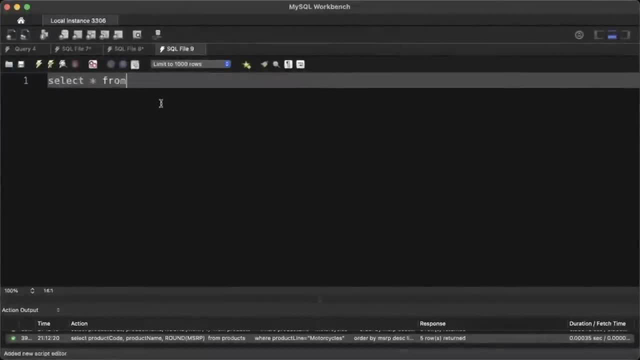 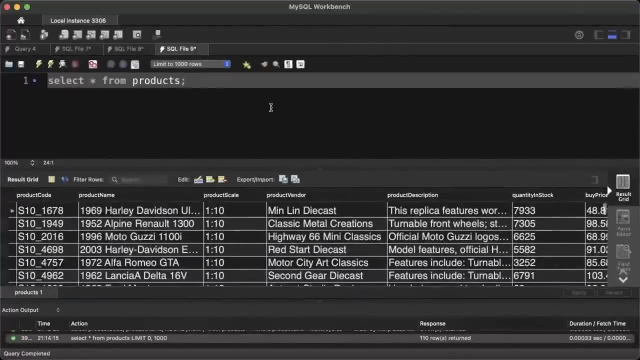 Let's go step by step here. First thing is we want to get some information out of them. Products table right. So let's go select star from products. Yup, So now we select a bunch of products, All right, And what are we interested in? product code, product name, buy price, sell price. 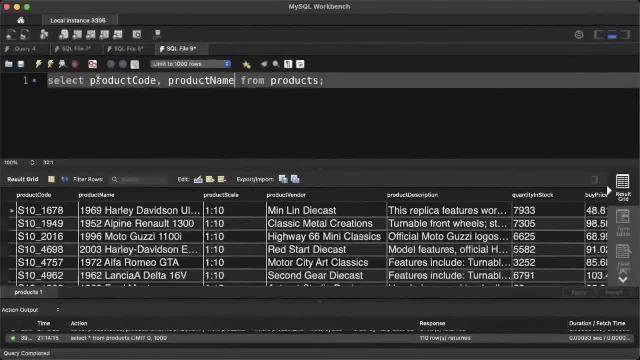 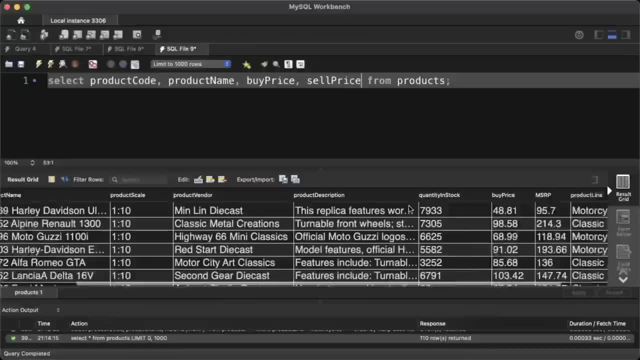 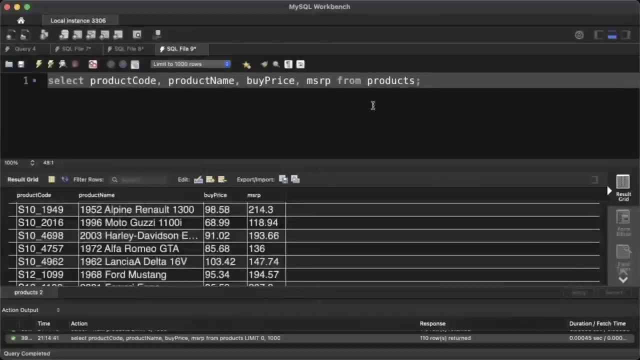 So let's get product code, product name, buy price, sell price. Oh okay, Is there a sell price? I don't think so. There's just an MSRP, Yup, Okay. So now we have the information that we're interested in, but there is this last column that we need, which is: 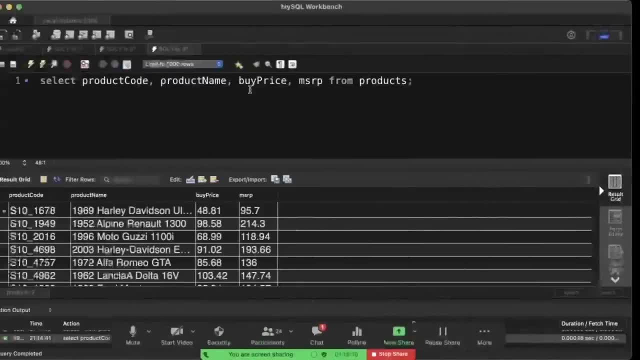 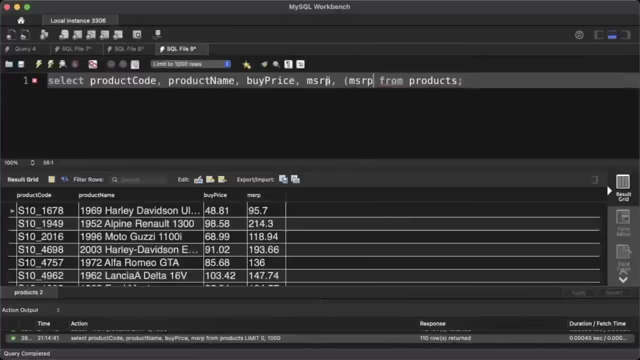 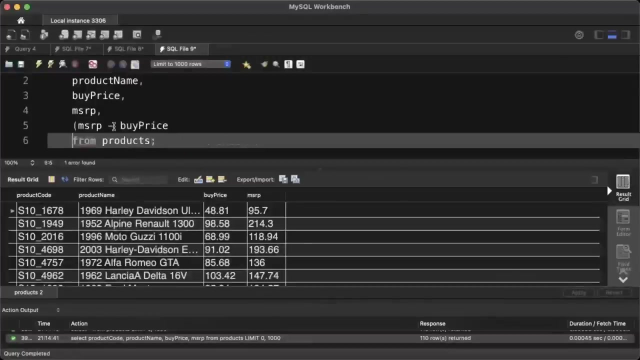 profit margin percentage And fortunately I have the formula here. So here's what I can do. I can simply put in the formula here: comma um M S R P minus by price. Let's get these on different lines, So M S R P minus by price, and let's get that down as well. 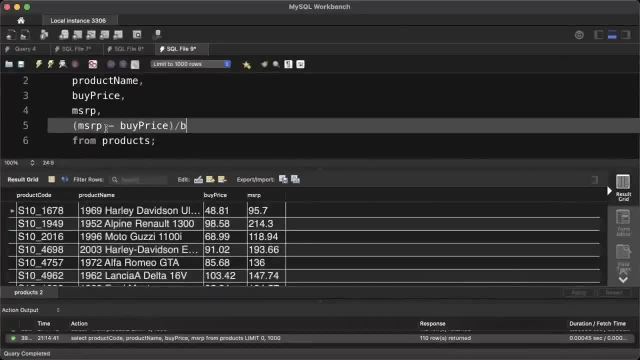 Yeah, So this is the profit. And if you divide that by by price, so these are all column names, right? So you you're saying we want to take values in the MSRP column from them, subtract the values in the by price. 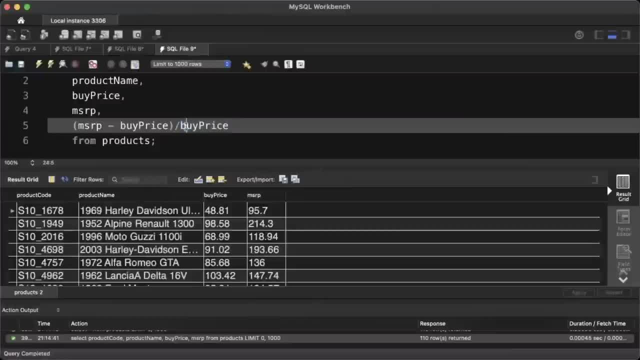 column and then divide by the values in the by price column, And we want to multiply that by a hundred too. So let's just put it: We're going to put in a multiplied by a hundred, and let's put the entire thing within a bracket. 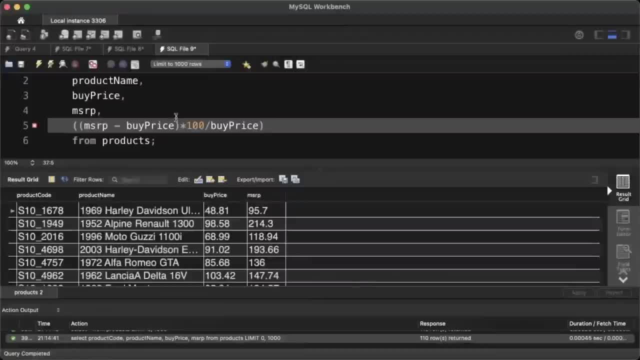 Okay, So now we have MSR. Oh yeah, So now we have MSRP minus by price multiplied by a hundred, divided by by price, And let's just call that profit margin. So let's just rename that, So that's our profit margin. 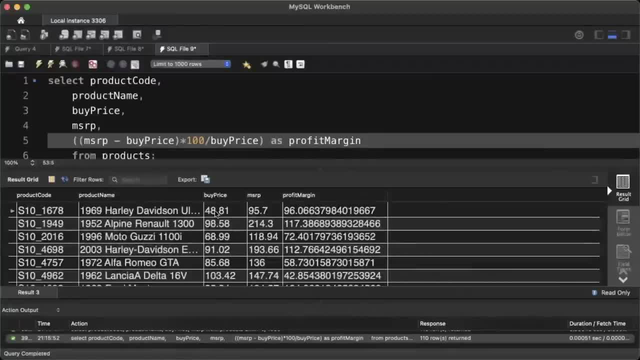 And you can see that the profit margin for this product, since we buy it at $48 and sell it at $95, is 96%. That is the amount of money that we've made On top of the. And what are we going to do with the profit margin? 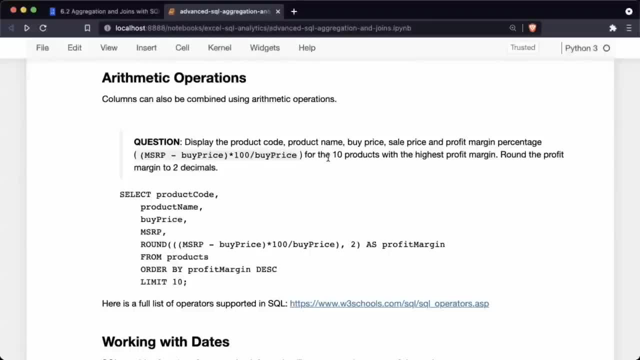 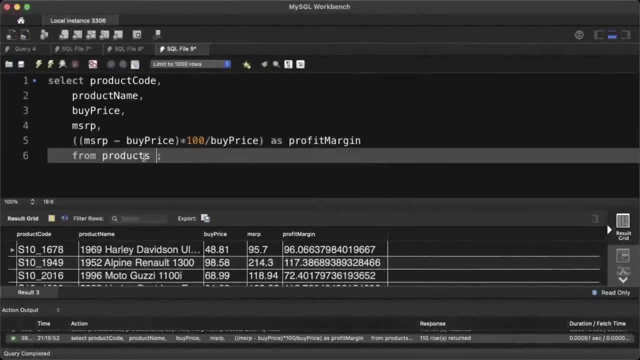 Well, we want to show the 10 products with the highest profit margin, So let's add that, So that will be a sort or an order by order by and now, once we've created this column, we can use it here, So we can call ordered by profit margin and you want to limit it to 10 and you want to see the highest profit margin. 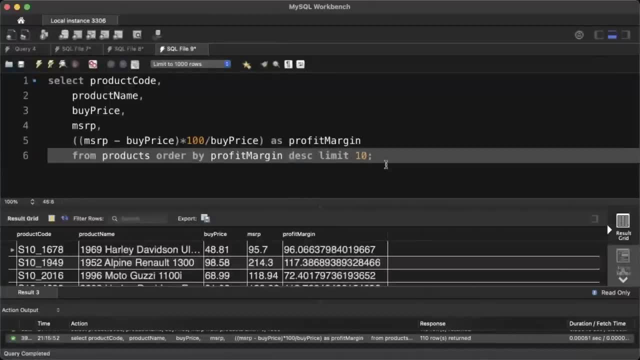 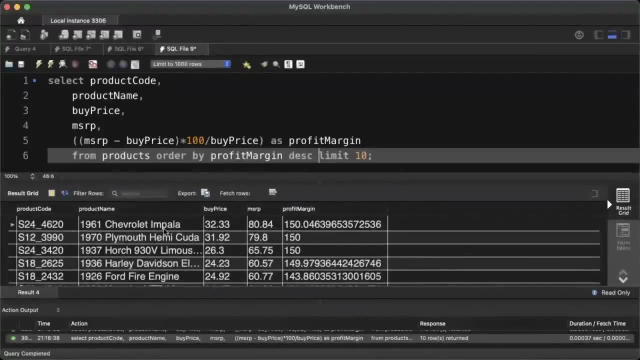 So we say D E S C Descending limit 10.. Let's check that great. So now we have this product, the Chevrolet Impala, on this product We are making a huge profit margin. We're buying it for $32,, selling it for 80.. 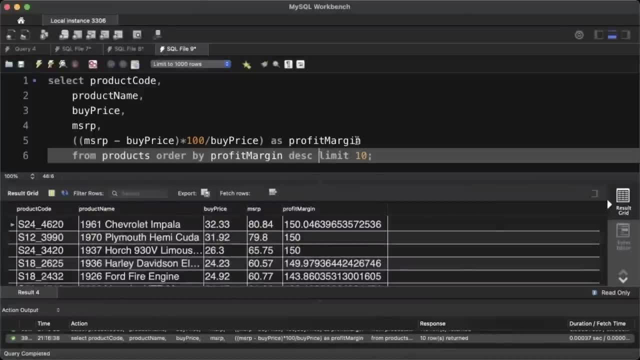 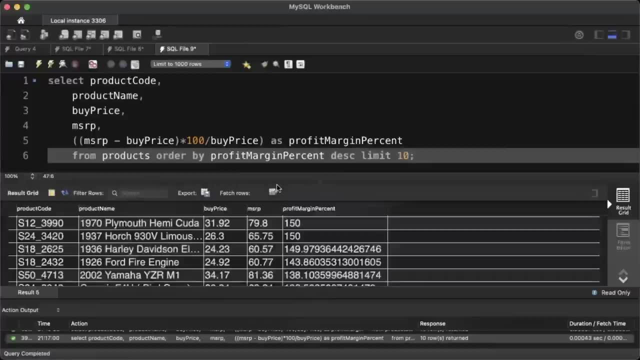 So 1: 50% profit. actually, maybe let me just call this profit margin percent, so that it's not confusing with the actual number. Yup, Now, the last thing we want to do is round the Profit Margin to two decimals, and that's easy. 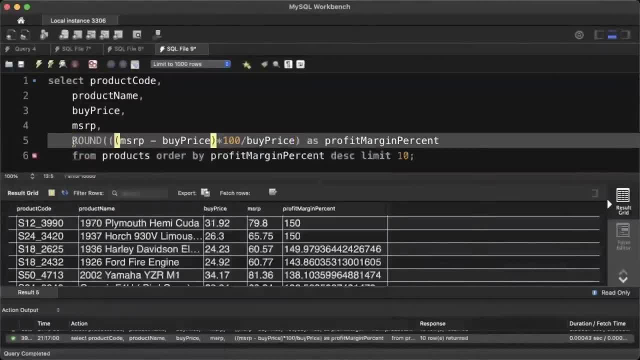 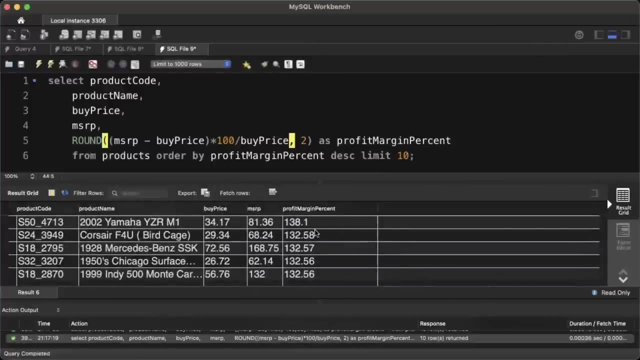 We just type around here and another bracket here. Well, I guess we don't. let's see, we probably don't need that bracket, Um, and we want to round it to two decimals. So there you go. Now we have the profit margin rounded to two decimals and these are the 10 products with the highest profit margin percentage. 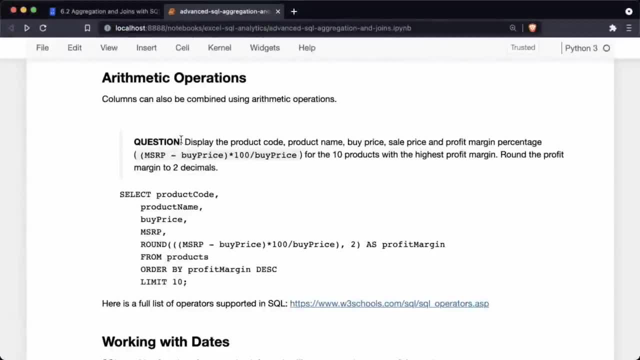 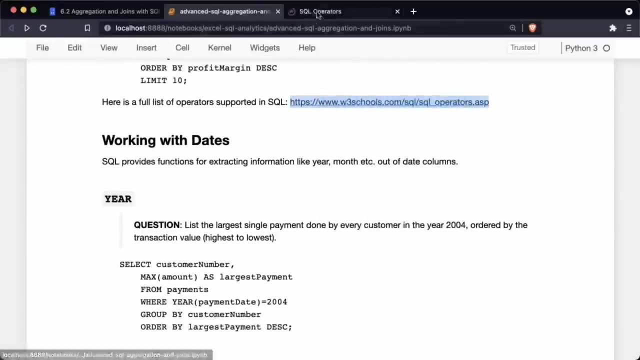 So these are the kinds of queries that you should be able to answer by using arithmetic operations. by using sorting, grouping and aggregation and mapping functions, You can check out what other operators are supported in SQL. It's not just a Yuhan arithmetic. 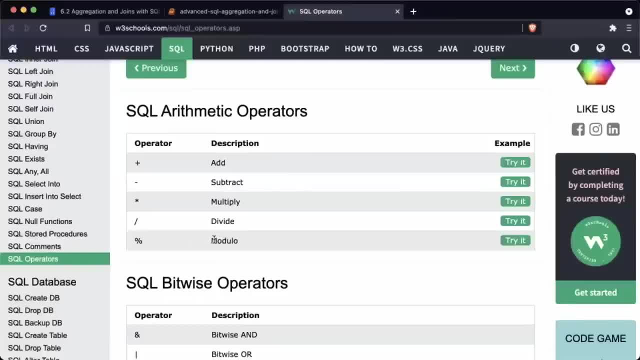 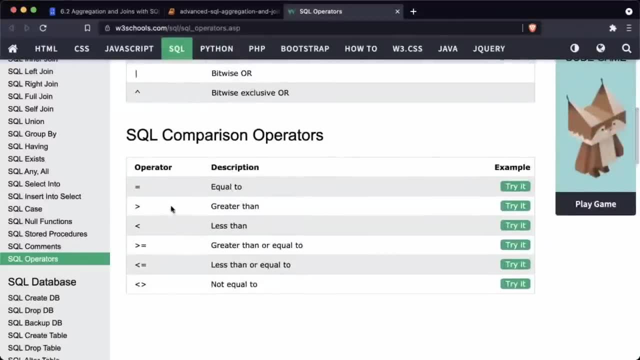 You have add, subtract, multiply, divide- You can divide, And you also have this modular function which is to compute the remainder, So you can do that as well. And then you have some bitwise operations, and you're already familiar with comparison operations as well. 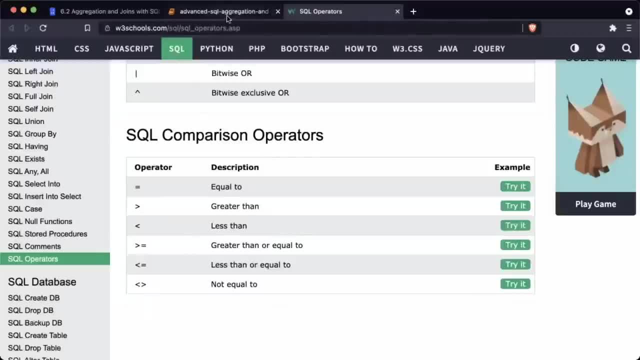 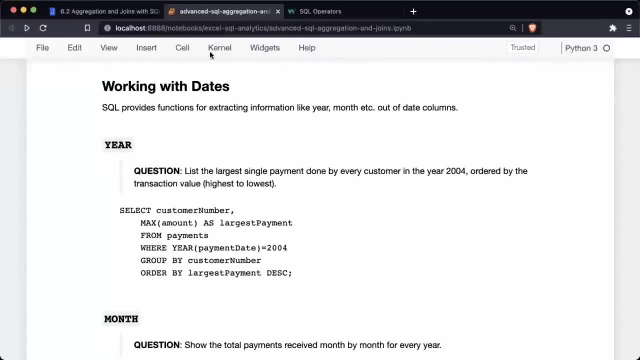 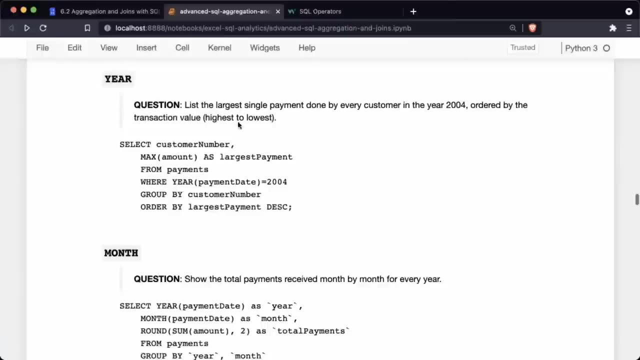 So comparison operations are typically used in the where clause, As we saw with the date. talking about dates, SQL also provides several functions for extracting information like the year, month et cetera, out of date columns. So let's look at an example list: the largest single payment done by every customer in the year 2004, ordered by the: 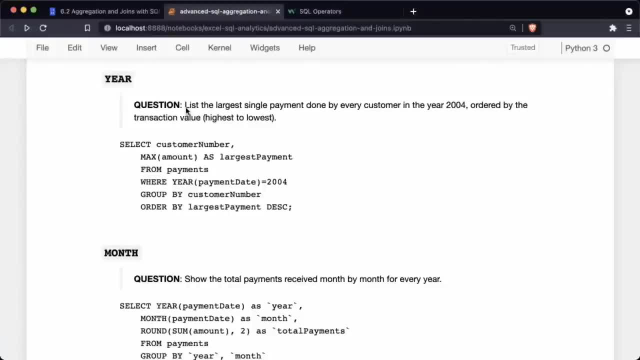 transaction value: highest to lowest. Okay, Again, it seems complex, but let's break it down. We are interested in payments. That's what I can gather here, List the largest single payment. So I'm just going to go here and first of all just to select star from payments. 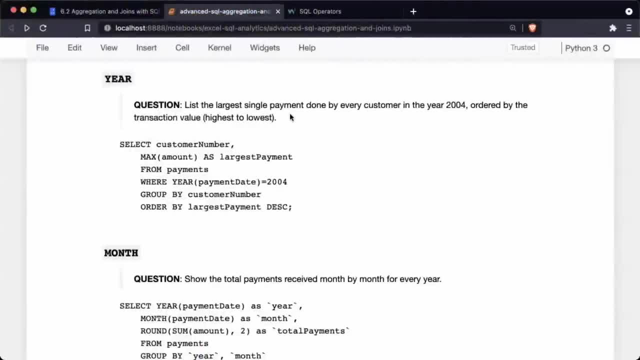 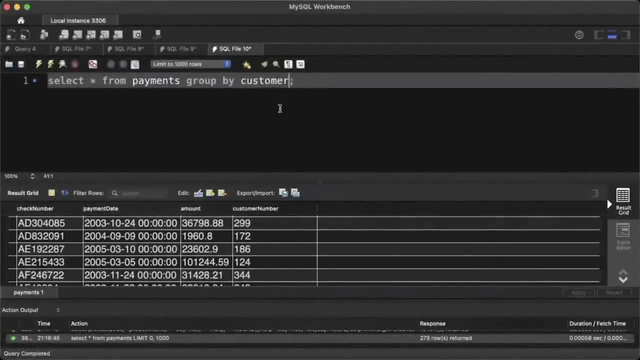 Okay, We have payments now. Next, we want the largest payment by each customer. Okay, So we want basically the maximum payment by each customer. So we can probably do a group by Customer number and then for each group of rows, for each customer, we want the maximum payment that they've done. 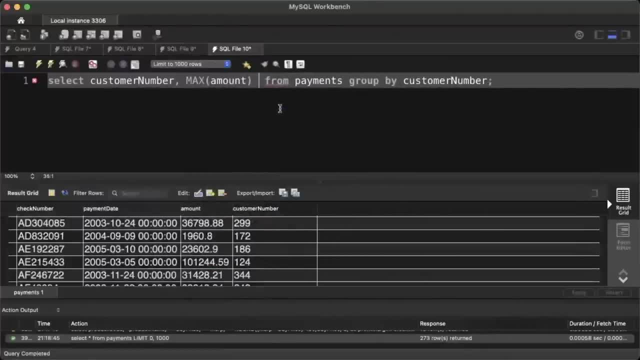 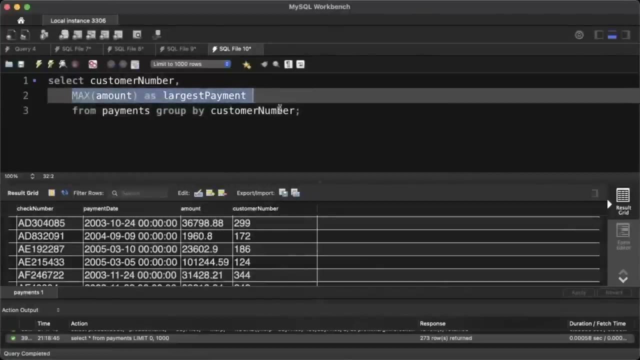 So let's call amount, max amount, and let's rename that to largest payment. Okay, All right, So start starting to make sense now. So we have, we select customer number, We select the maximum amount. So for each customer we look at all the payment. 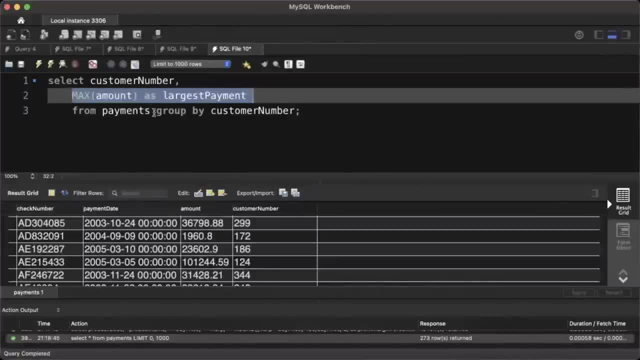 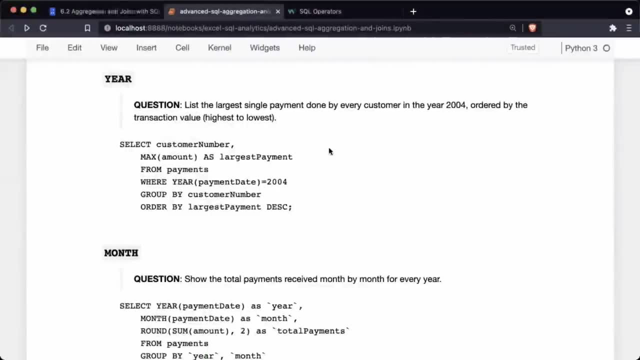 We've made and pick the one with the maximum amount or pick the maximum amount among those, And of course for that we have to do a group by customer number. but we want to look at this in the year 2004.. How do we do that? 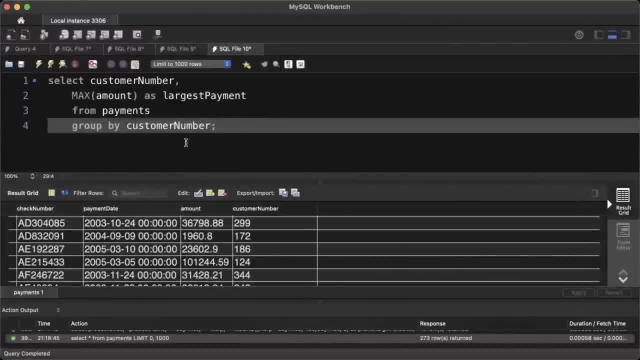 Well, we have a payment date and we could check if the payment date is greater than Jan 1st 2004, and less than Jan 1st 2005,, and things like that. Or we could Simply do where and we could use this year function. 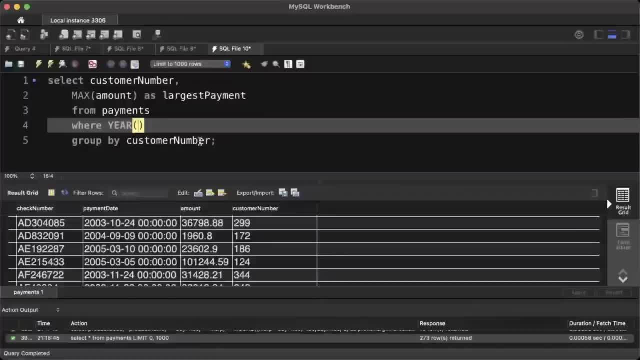 So here is a year as a function, just like other mapping functions, and into the year function, pass in payment date and just check if the year of the payment date is 2004.. Okay, So that's our query right here: select customer number, max amount as largest payment from payments where year of the payment date is 2004 and group by customer number. 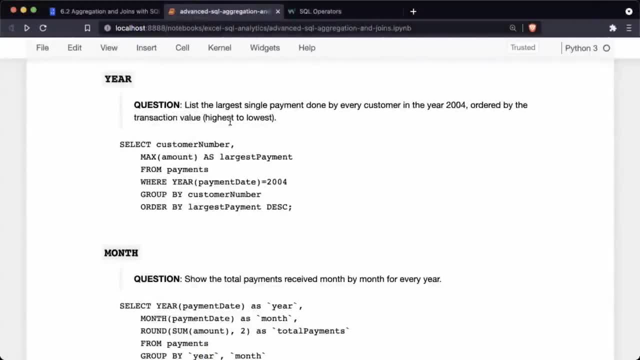 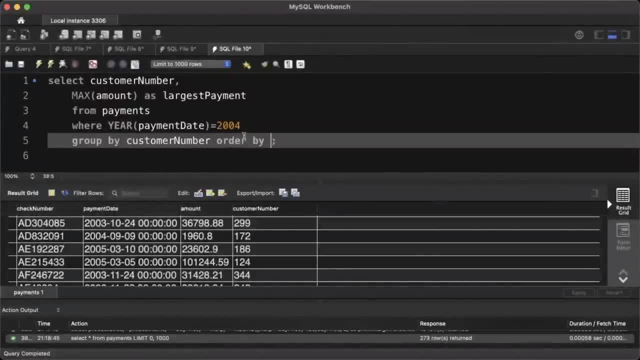 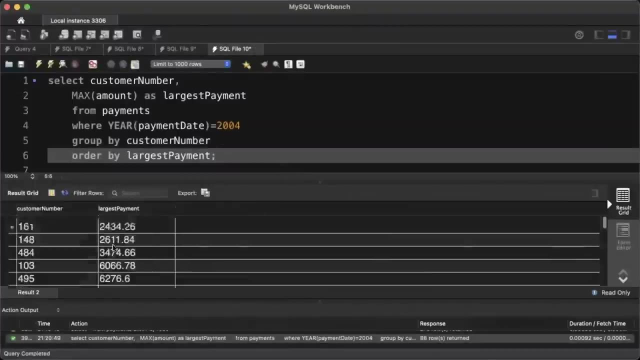 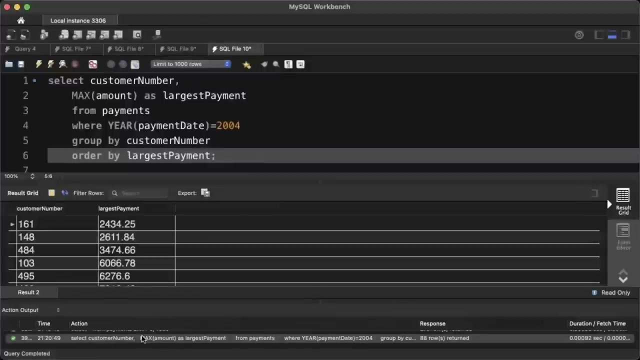 And ordered by transaction value, right? So we want to order that by transaction value. So we should also probably put in order by largest payment and let's run that. So it turns out that customer number one 61, it turns out that customer number one 61 made the largest payment in the year. 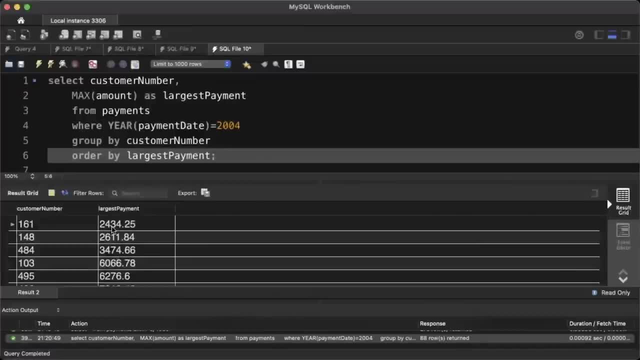 2004 and that payment was $2,434.. Oh well, no, we want to sort it in descending order. Yeah, So customer number one 41,. the loyal customer made $116,200 in a single payment And that was the highest payment in 2004 by a huge margin. 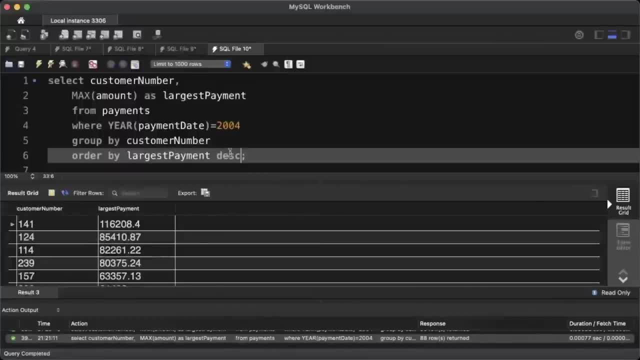 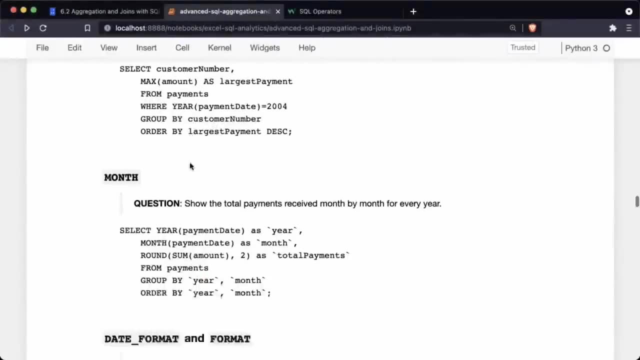 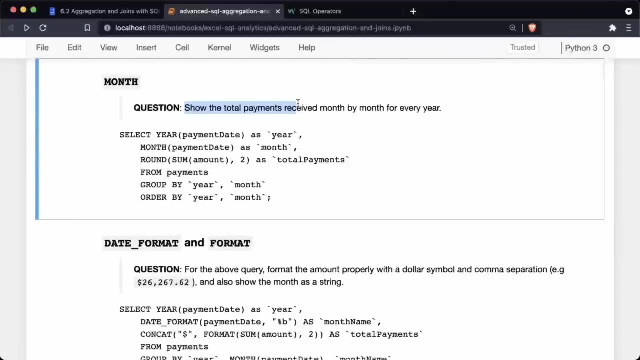 Actually, you had to 84,410 after that. Okay, So that's how you pick out information from A year, from a date. Here's another example: show the total payments received month by month for every year. Okay, This is interesting. 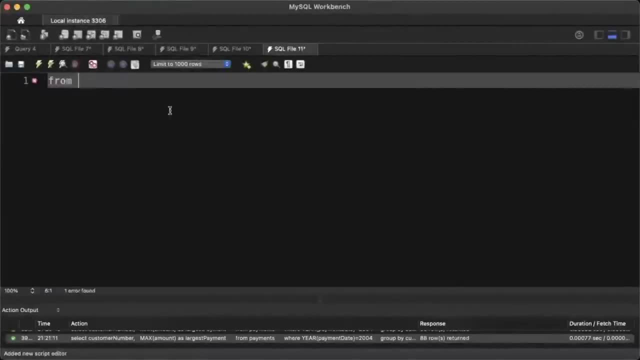 So you want to show the total payments month by month for every year. So you want to see January 2003,, February 2003,, March 2004, and so on. So let's once again start with payments. select start from select, star from payments. 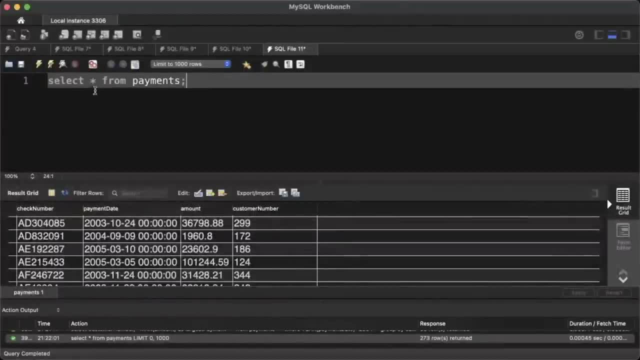 We have the data. Now we are interested in year and month, So we have a payment date. If we can just create a new column for year and a new column for month, I think that should just get us started. So I'm just going to create a new column for year. 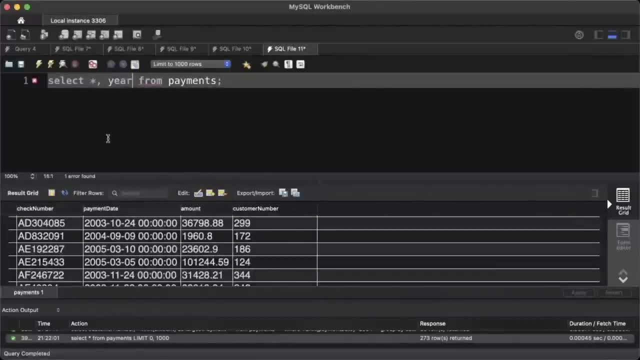 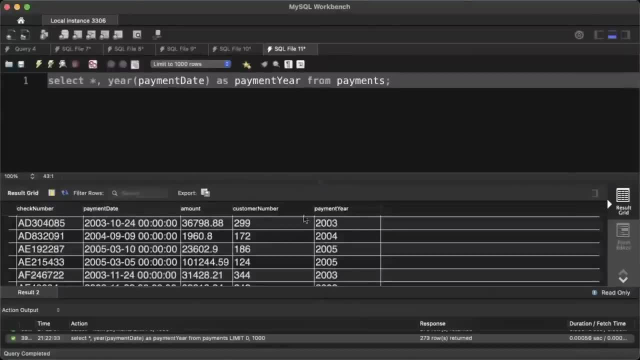 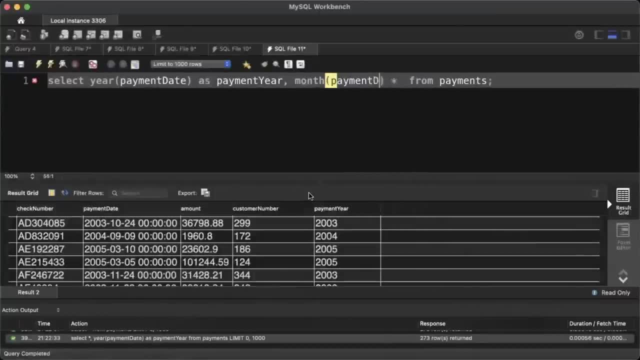 So we just type month and we type payment date. So from the payment date we get the month and we call that payment month. So let's put that on a new line here, comma star. So we still want the other columns, or you know what. maybe let's just keep the amounts now. 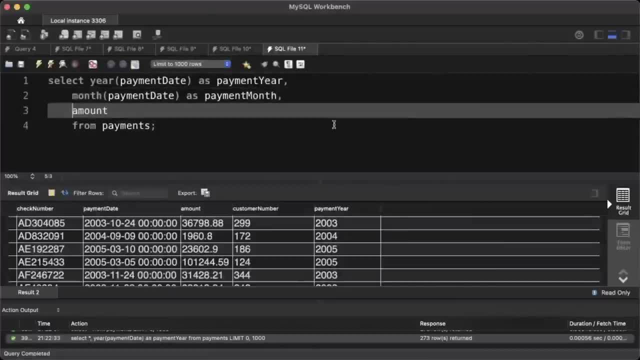 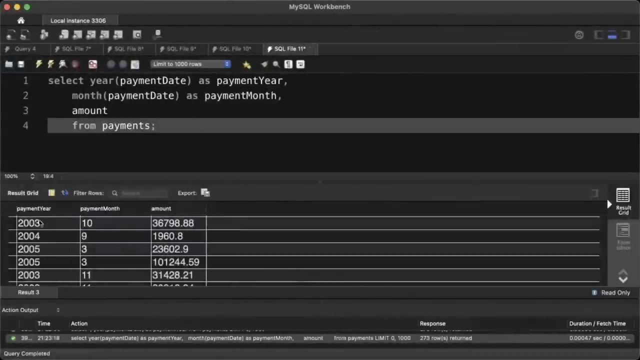 Or maybe you don't need the other information. So select payment date: year as payment year, month of payment: date as payment month and then the amount from payments: Yup. So now it tells us of for every single payment, we now have a year and a date and the amount. 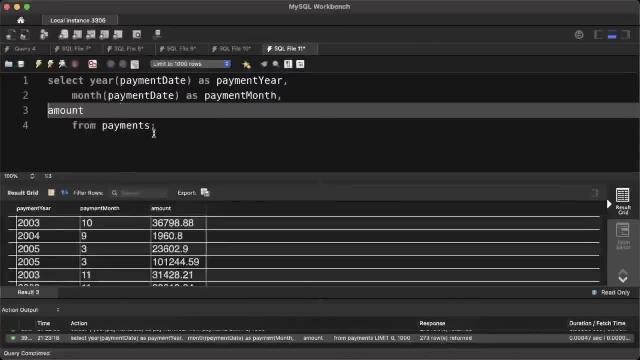 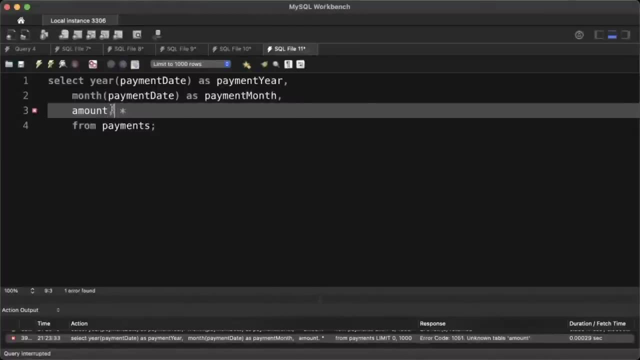 but of course we don't want, uh, of course we don't want, uh, like this is still. It's showing us every individual payment, Like if I put a comma star here, you will see that we're still looking at, if I just, instead of the amount, if I put star here. 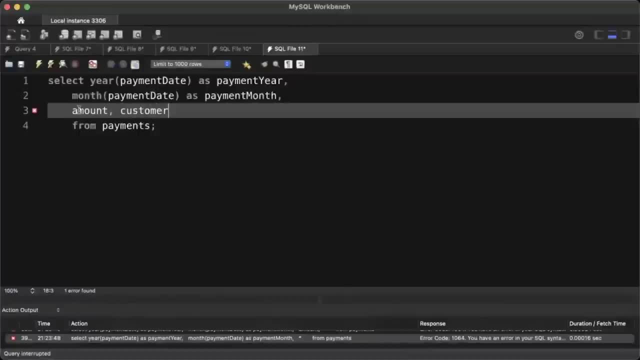 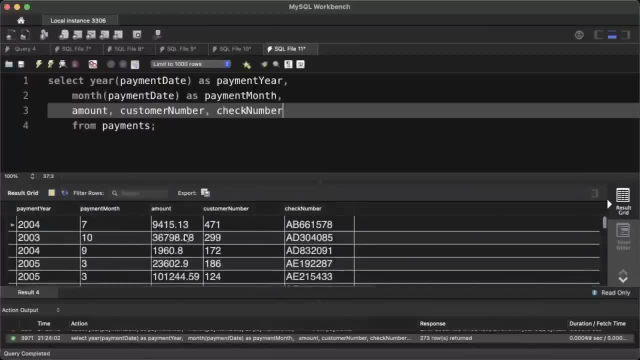 Okay, Okay, Okay, Okay, Yeah. So you can see that we're still looking at every single payment. even though we've created a payment year column and we've created a payment month column, we are still looking at every single payment individually. 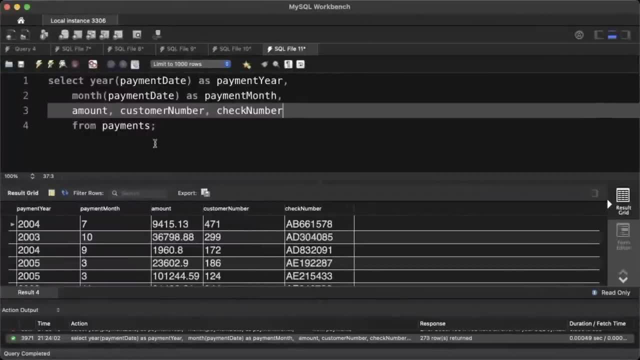 What we want is the totals for each month and for each year. So how do we do that? Well, you guessed it: We want to total up the amounts. So let's get rid of these other columns and let's just do a sum, and we want to get the sum of the. 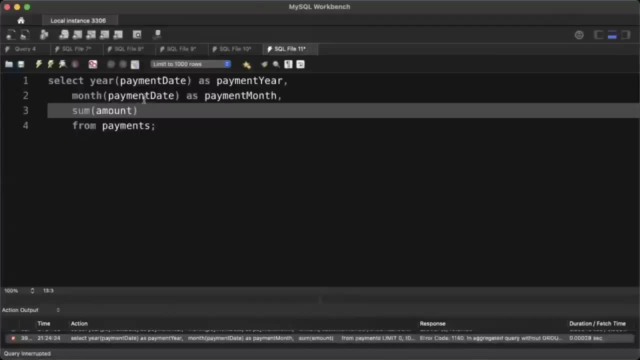 amount Okay, But of course just doing a sum is not enough, because we also need to do a group by right, Because we want to first define groups. So for each month, comma, year, we want to get a group of columns. 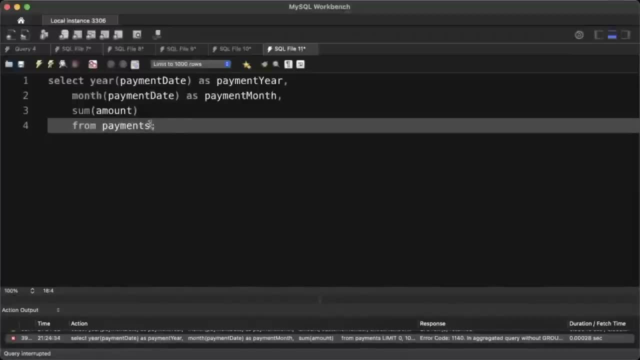 You want to get the group a group of rules. So you want to get all the rules which were which belong to January of 2003,, all the rules which belong to February of 2003, and then sum up each group. 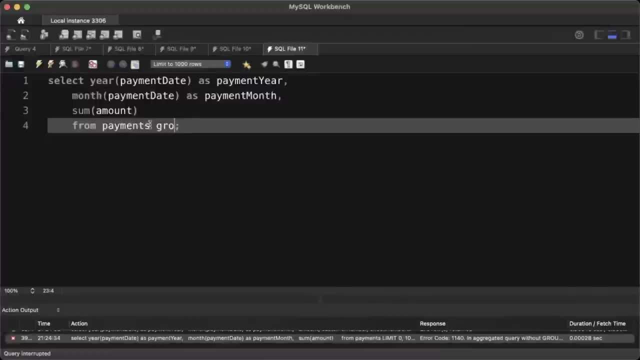 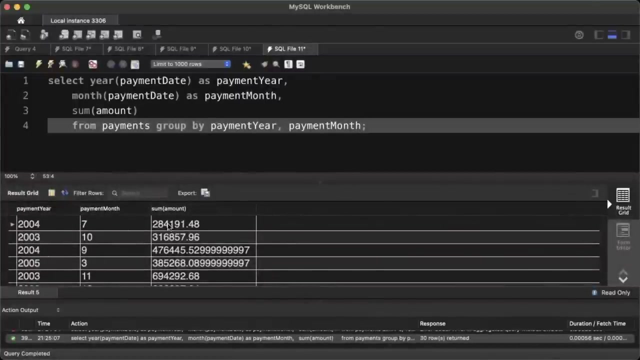 So we type here group by, group by and then group by. you can actually provide multiple Columns. So we have this payment year column and we have this payment month column. So now we have a payment year, We have a payment month and we have the total sum. 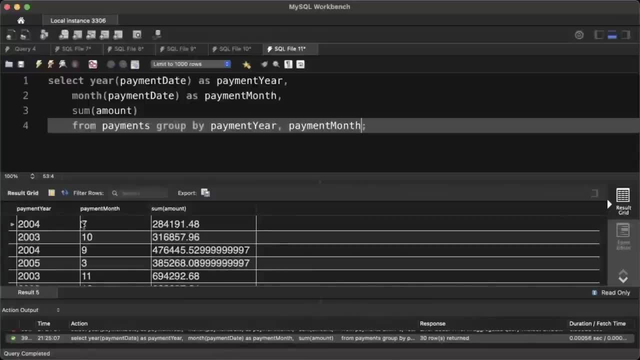 So this is the sum of the amount of all the payments made in that particular month of that particular year, And maybe we also want to order by the same criteria so that we can see it in a more understandable format. So we also ordered by payment year and payment month. 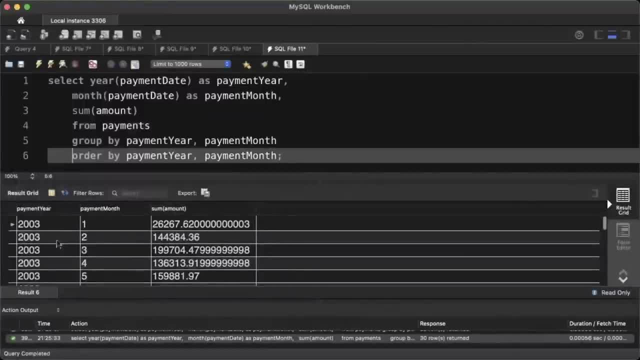 And you don't need this comma here. Yeah, So now we have 2003 one, and the sum is $26,000, and then 2003, two, which is February of 2003.. And the summer is $144,000.. 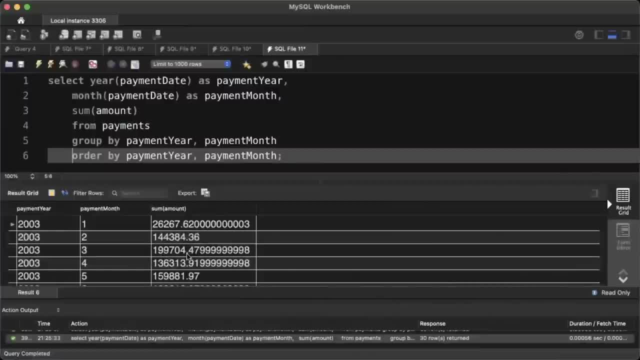 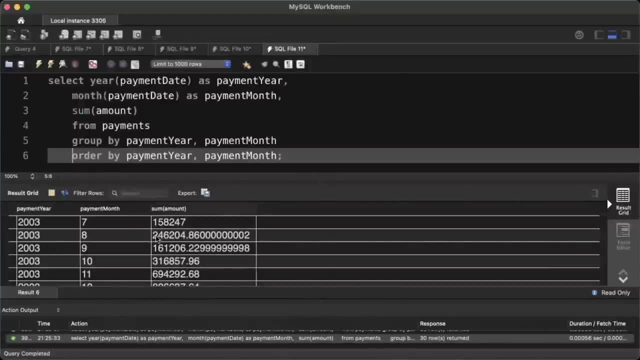 And then 2003,. March is $199,000. And so on seems like what is this? August, September of 2003 was pretty good, So this is how you can now start doing some basic analysis and interpretation. So this is: 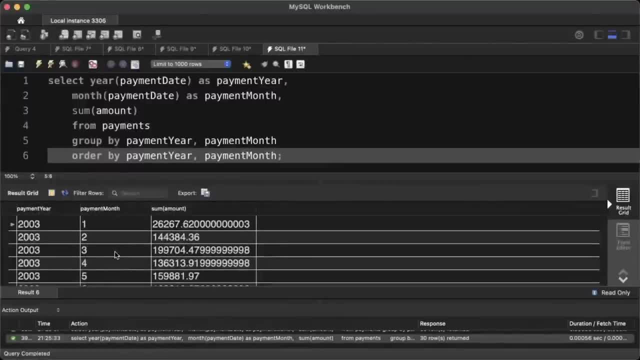 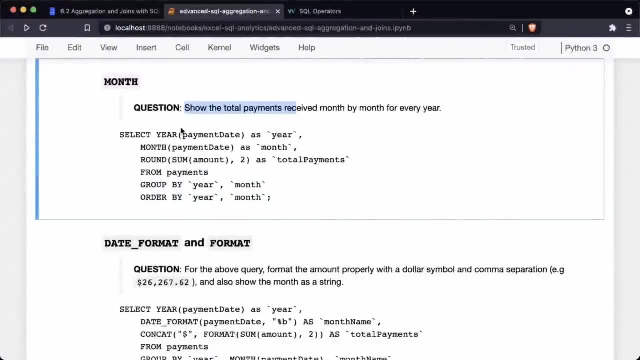 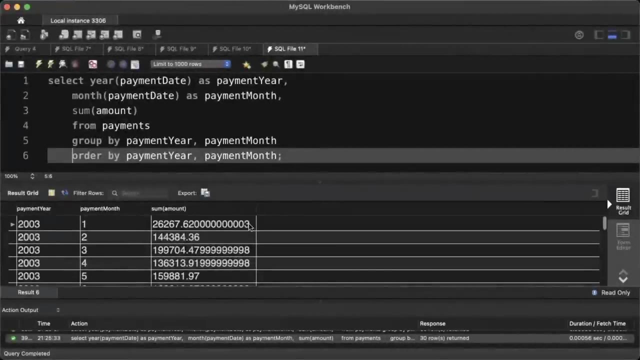 Your revenue growth or this is your revenue table. So if your boss asks for a month, why is revenue table? This is what you give them. but of course, you probably don't want to show these numbers like this, Like it doesn't make sense to look at this. 0, 0, 0, 0, 3 here. 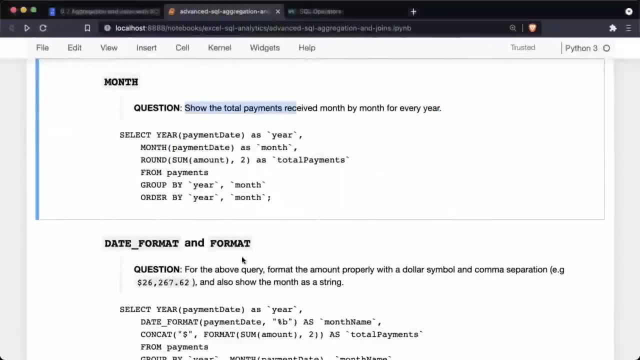 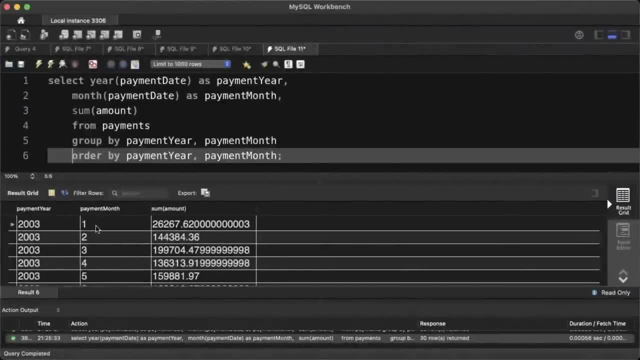 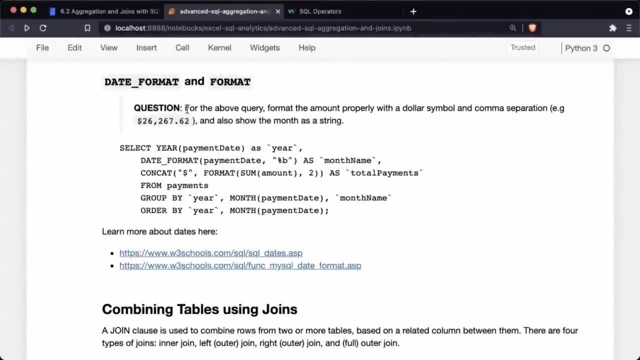 And it's probably a floating point or a rounding error somewhere, So let's make these a little prettier. and here again, it's a bit difficult to guess the month from month number. going to the actual month can be a bit difficult, So let's make this a little prettier. now for the above query, the query that we just looked at, let's format the amount. 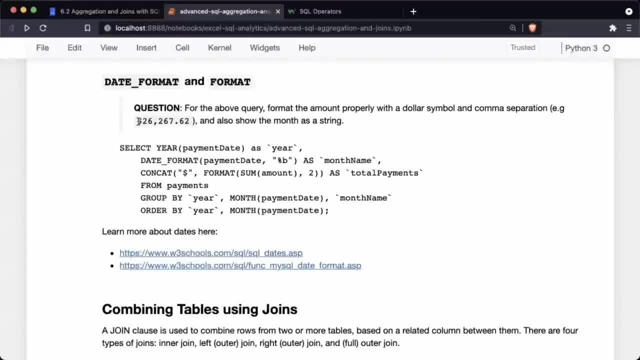 properly with a dollar symbol and comma separation. Maybe show it something like this: 26,267.6, two and just two, two decimal places, And let's also show the month as a string. Okay, So now we're in the territory of printing things nicely. 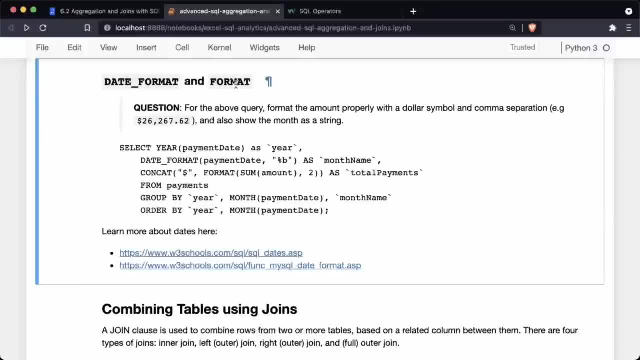 Well, well, Of making things look good. So that's where you need these formatting functions. There are two numbers, two functions. One is the format function for numbers and then the date format function for dates. So let's first look at the format function for numbers. 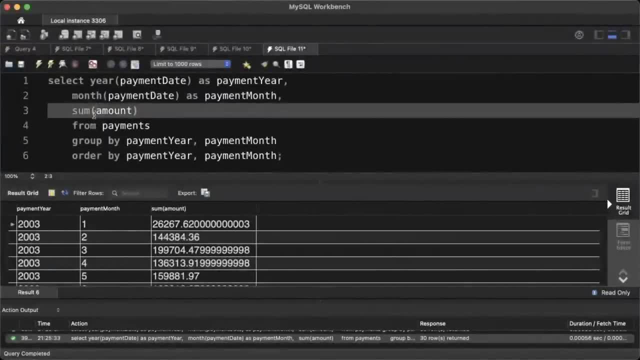 Now, instead of showing the sum, just the sum of amount, I am going to call format here and I'm simply going to put in. I think you can. to format, you can mention how many decimal digits you want. So I'm just going to put in two here and format is automatically going to add commas here. 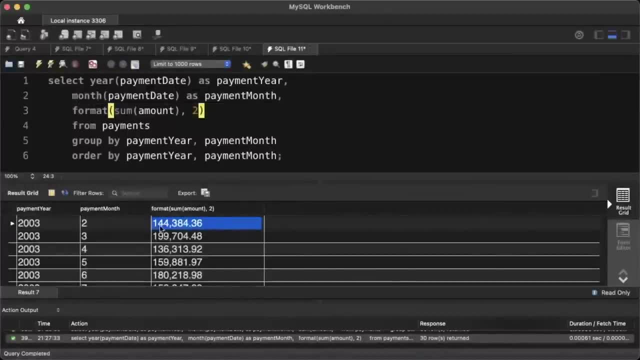 So now you can see that you have 1,, 4,, 4 comma, 3,, 8,, 4.36,. just by adding this format keyword here, And of course, now it's no longer number, Now it has become a string and let us also rename this column as revenue. 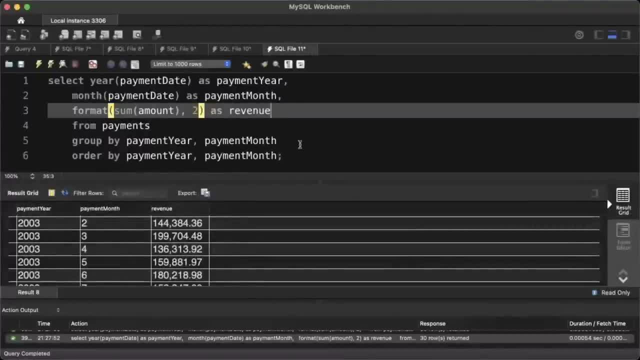 So now we have revenues 1,, 4,, 4, 3,, 8,, 4.36.. Maybe let's go step further. Let us add a dollar Symbol here. How do we add a dollar symbol? Well, this is a string and we want to add a dollar symbol at the beginning of the string. 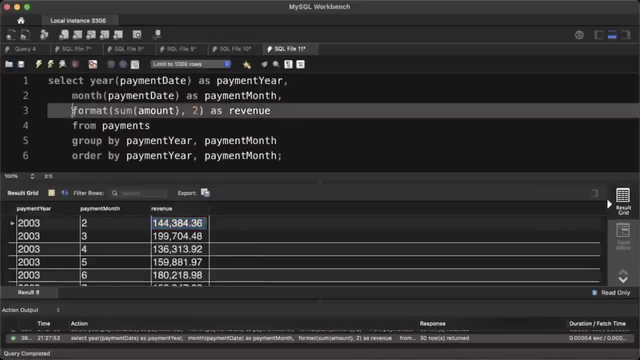 How do we combine two strings? that is done using concatenation, So let's call concat the concat function that we saw earlier, but this time, instead of concatenating two columns, we are concatenating a string- the dollar symbol- with the column. 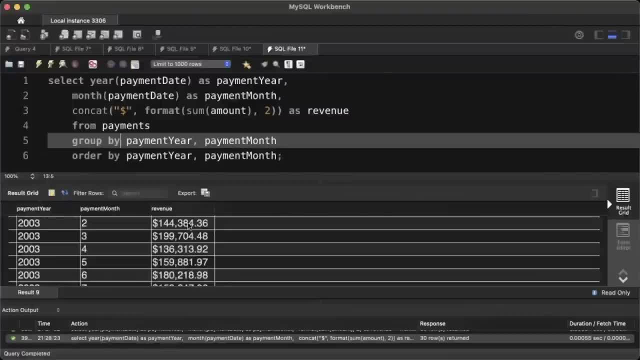 So now, when we call concat, we have dollar 1,, 4,, 4,, 3,, 8,, 4.36.. And that is called the revenue. So that's how we format the numbers: A small, a little other, a small cleanup that you can do here, especially if you're sending it out to somebody. this result is maybe. 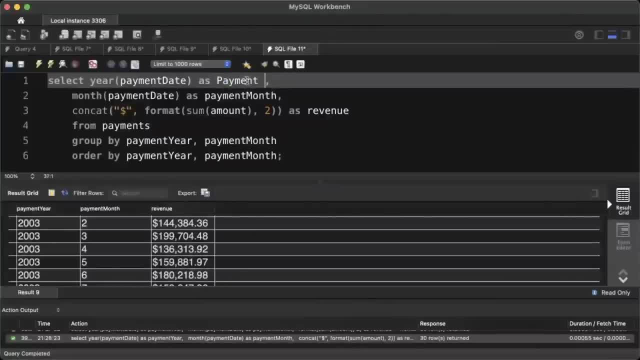 you want to just clean up these con call column names. So if you want to just call it payment year- but of course that's going to be a problem- So whenever you have spaces within column names you can use these back courts. So this is the court that is available on your 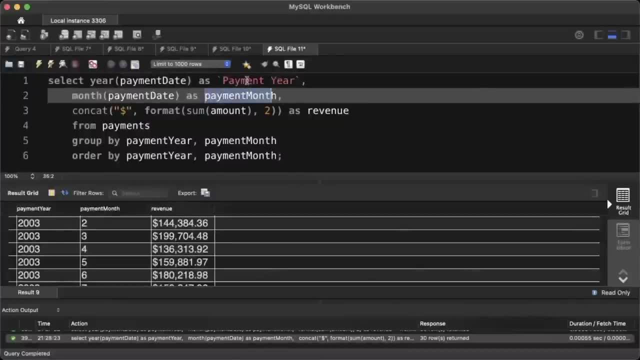 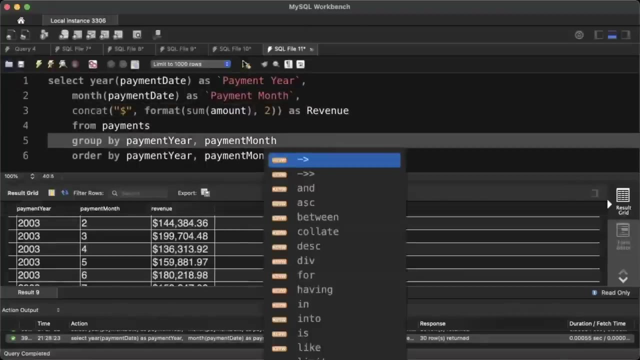 Key Board just below the escape key, and let's call this payment month, Okay, And then let's call this a revenue. I think this should be fine, just like this, And once again, let's just changed it here, just cleaning it up a little bit to make it look nicer, and then you can export. 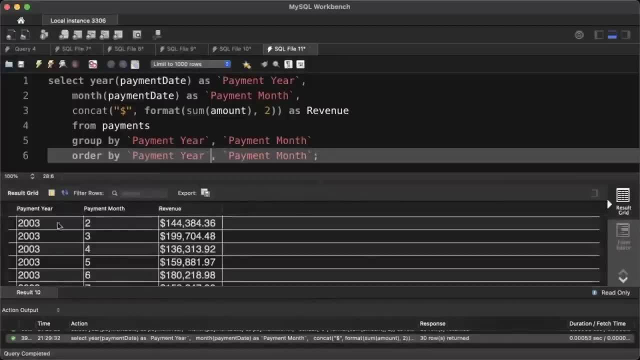 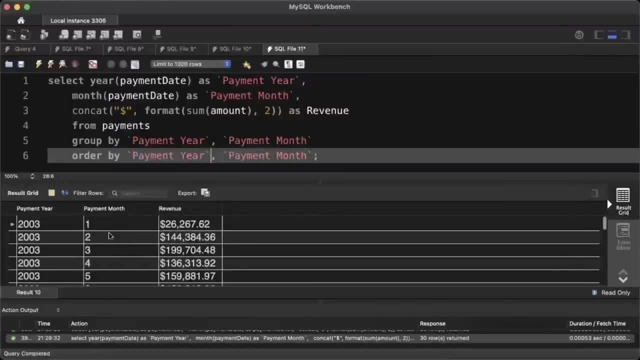 It and send it as a CSV or something. So now you have payment year, you have payment month, You have revenue with dollars looking good, but of course we still missing this piece. We want to show things like January, February, et cetera here. 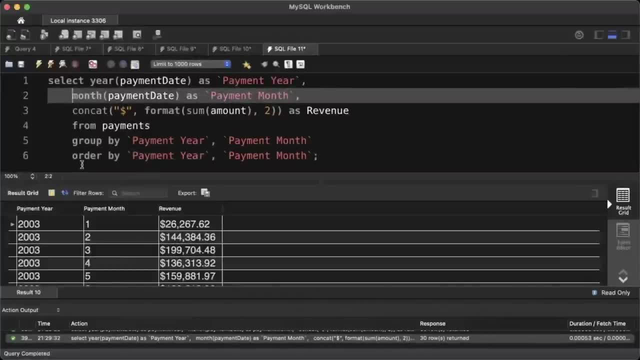 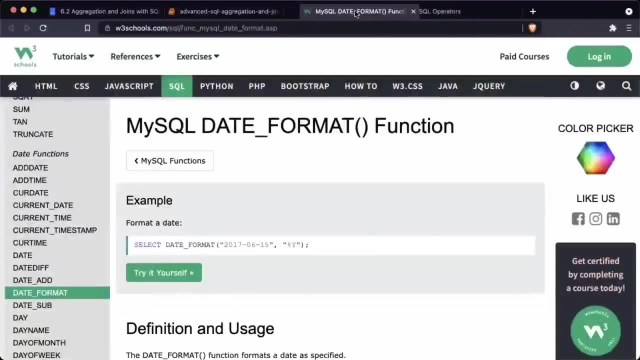 So if you want to show Jan, Feb, et cetera, here's what we can do. We can call it date format. So there is this function called date format, and date format is something you will most likely have to look up. 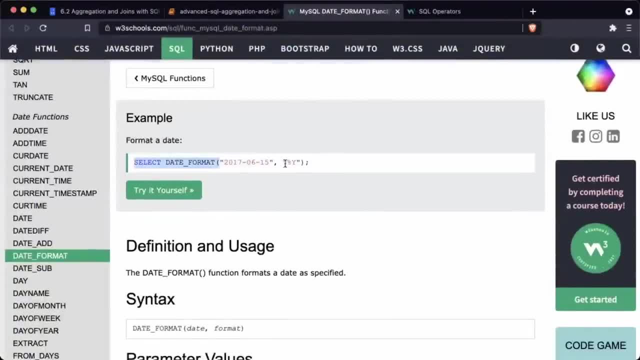 So date format takes a date as an input and then it takes us Certain format in which you want to see the date. For example, if you want to see the Y Y, M, M, DD format, then you put something like percentage Y hyphen. 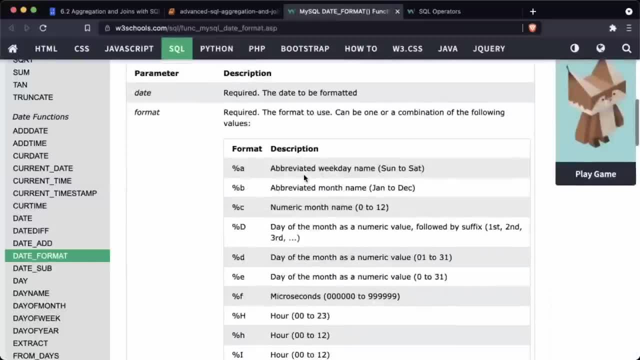 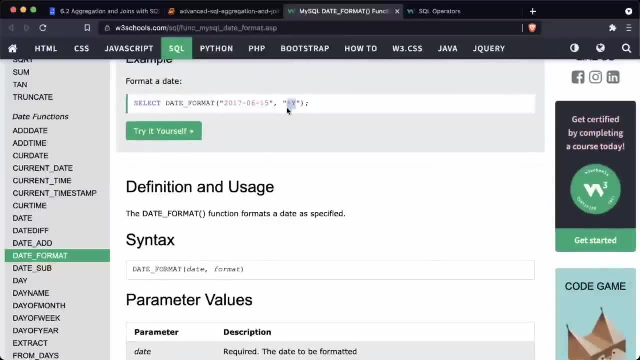 percentage M, hyphen, percentage D or or something, And here are all the variables that you put in. So, inside these courts, as a second argument, you provide all the variables that you want to show And, based on that, it is going to show you that information. 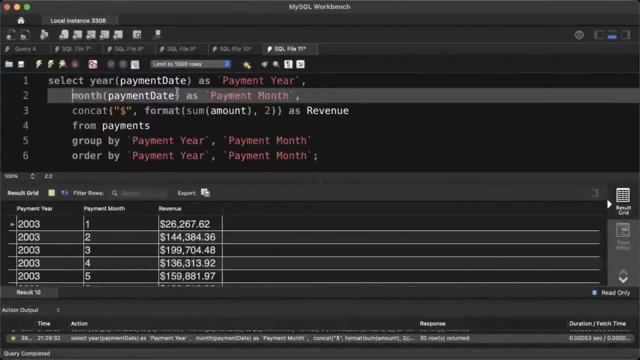 So we are interested in, we have a month here and we want to show that Month. Um, actually we we just want to show the payment date as a month. So I'm going to remove this month, I'm just going to call date format here. 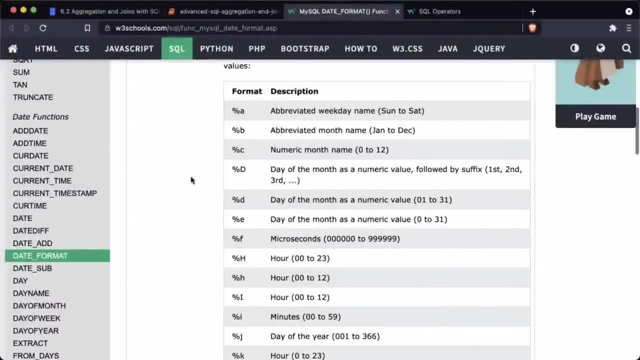 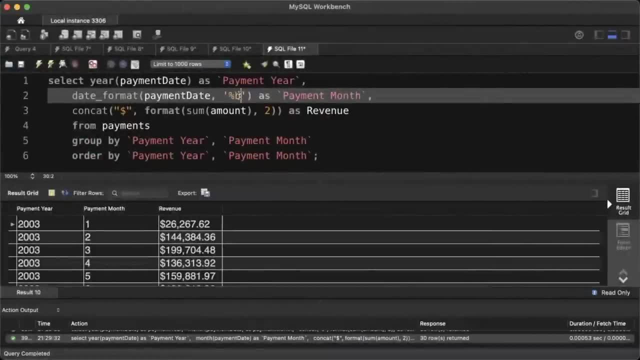 And how do I want to format it? Let's see, let's see what options we have. So there is this person be here, So I can take this person B, and if I just take this person be here, let's see what happens. 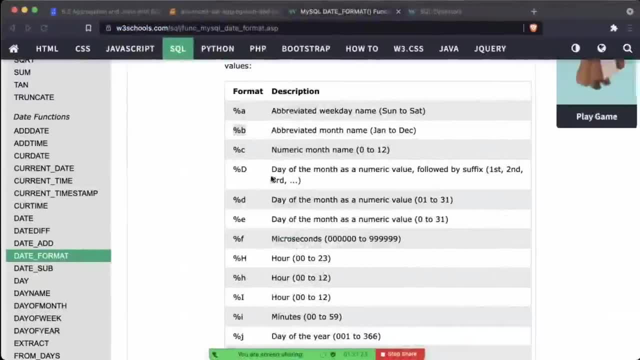 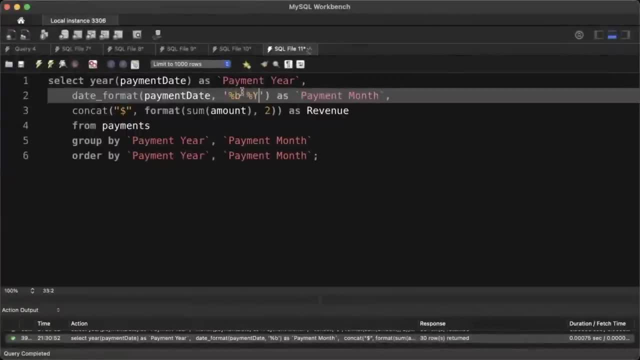 So you see here, now this has become August And in fact, if I want to get the year name, I think the year would be Y. So if I want to get the year name, I would maybe just put this: and now you can see August 2003,. 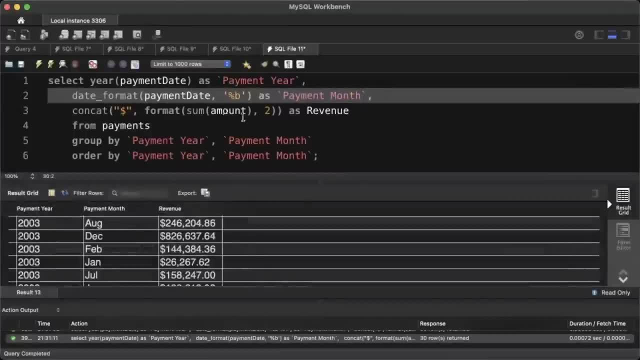 December 2003,. et cetera, but I just want to keep the month name here. So now we have the month name. So we took the date called date format on it, directly on the date, And we just extracted out the month using this person B. 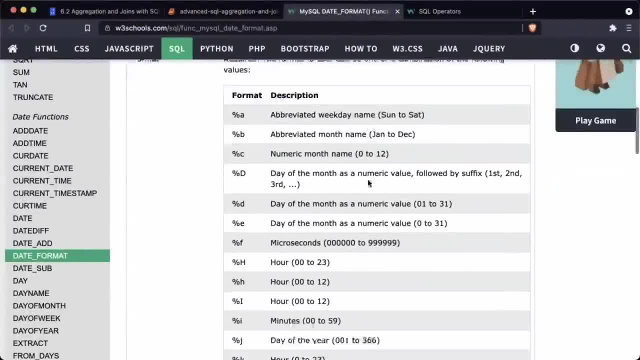 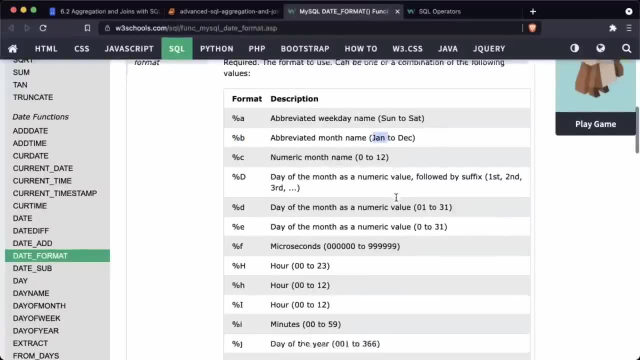 Um, and that is something that I looked up in this table- There's no way I can remember all of these, So I just have to look these up each time- And we saw that person B can give us the abbreviated month name. If you want the full month name, then we can use percent M. that can give us the full month name. 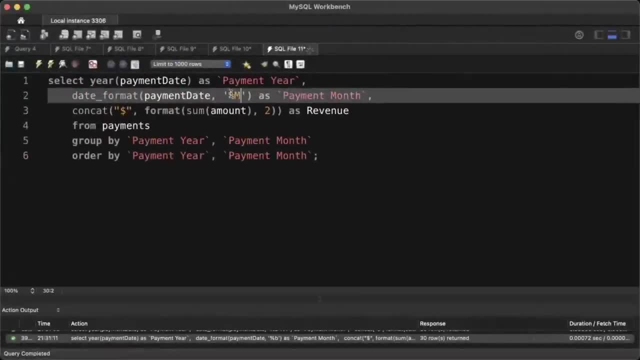 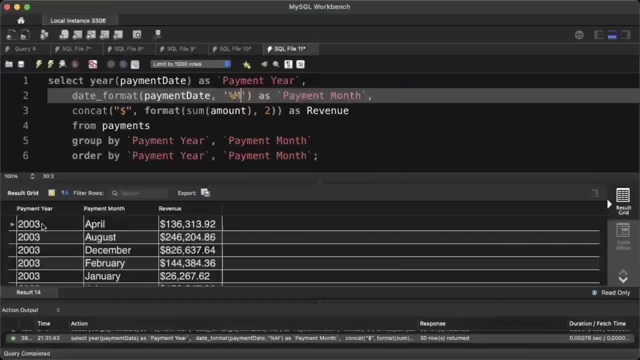 Let's try that too, Maybe, Okay, So, yeah, so now you have the full month name, but now we've run into a problem, because now we have payment year and we have payment month, but now because we are ordering by payment year and then 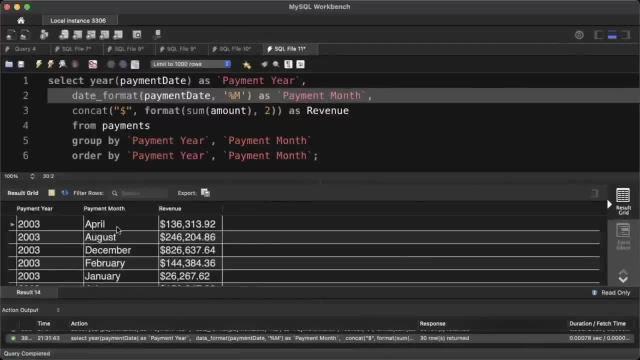 payment month: the ordering. the ordering becomes alphabet. Okay, So we want to display the number, We want to display the string, but we want to order by the number. How do we do that? Well, here's one idea. I create another column. 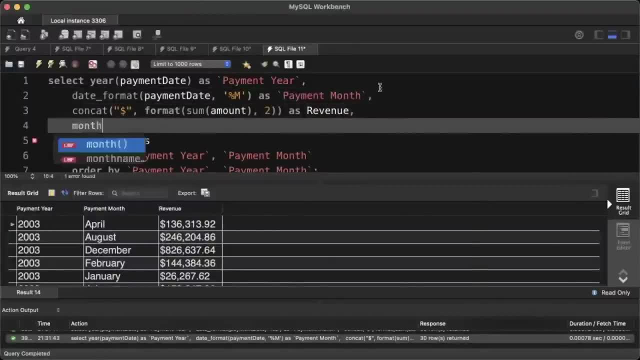 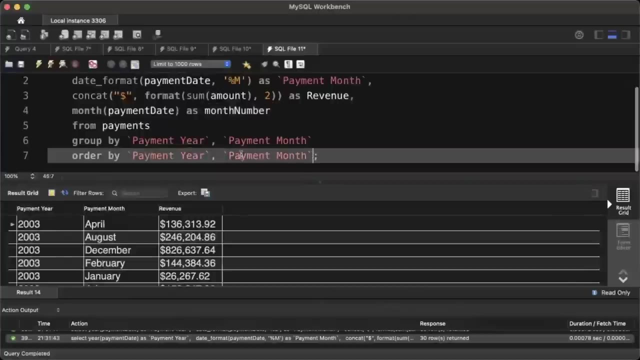 Let me just call that. uh, let's use month and payment date, So let's get the month from payment date and let's call this is called that as a month number and I'm just going I'm going to, instead of ordering by payment year and payment month, I'm going to order by month number. 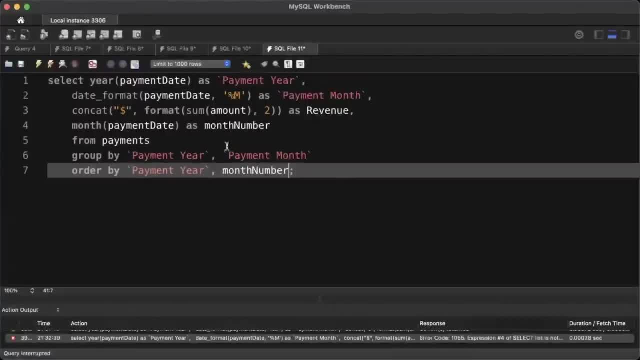 Okay, And let's try to run that. So that gives us an error, because Now, since I have this new column, month number, I should also be grouping by this column, Otherwise, anything other than- I'm sorry, anything other than the aggregation. 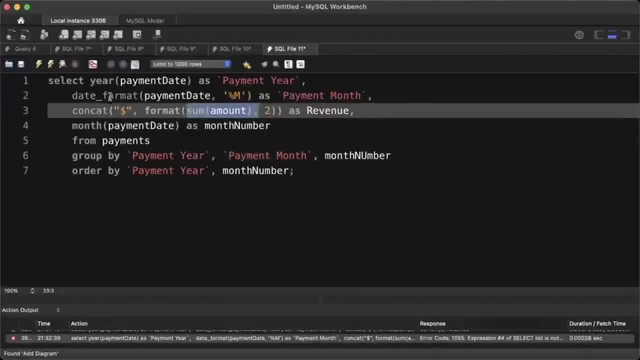 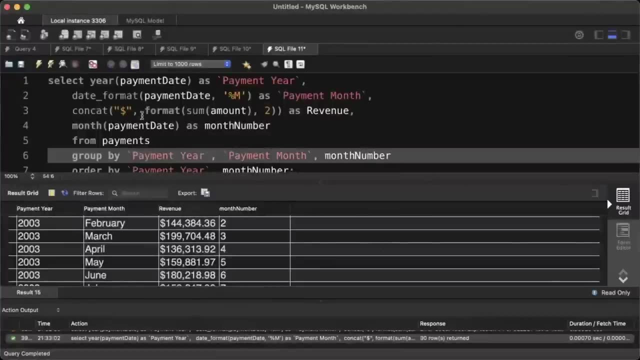 So here is where we are doing the aggregation: Anything other than the aggregation Sure In group by. so let me just put not month number here. Okay, So now we have three columns which we've created. We've created, created a payment year. 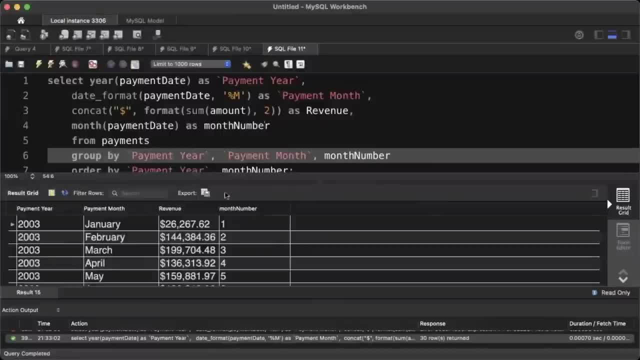 That's fine. And we've created a payment month- Great. And we've created a month number because we also want to track a month. We also want to track numbers here, and then we are grouping by payment year, payment month and month number. 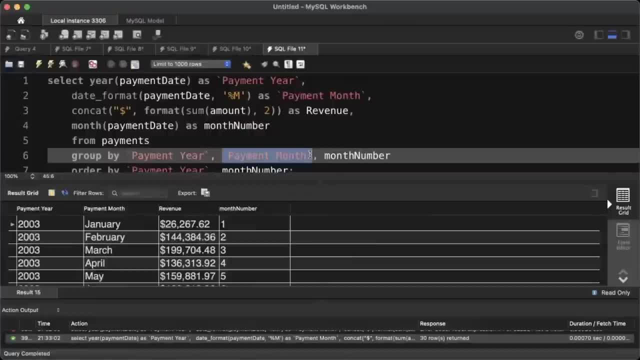 Of course, payment month and month number represent the same information, So the same groups would be formed. for Every month of every year we will get a group of rules And then we are taking the sum of those rows, some of those rows, to get the sum of the amount. 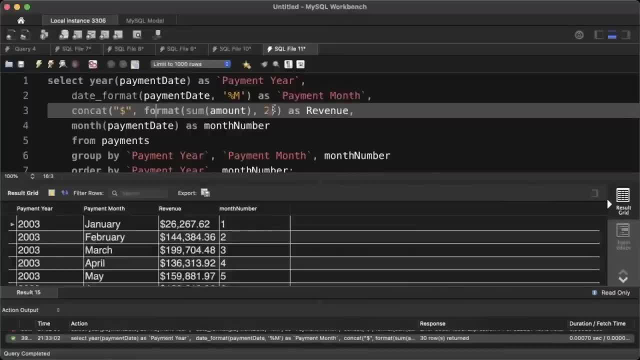 Then we are formatting it to add commas and show two decimals, And then we are adding the dollar symbol and we are calling that column revenue. Okay, So this is looking good. This is a pretty complex query at this point, but it's looking good. 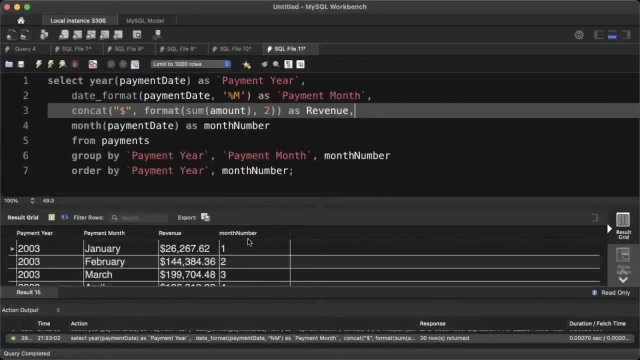 The only problem I have is that there is this last month number column here which I don't like. Uh, this is not something I want to send it to um, the person who's asking for this information. So how do we remove that? 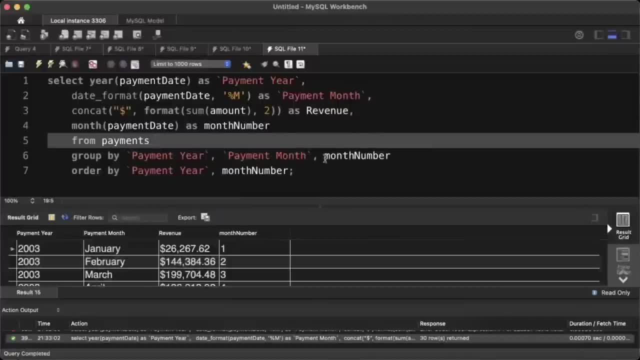 So in some sense we want to use this column month number for grouping and for ordering, but we don't want to display it. Here's how you can do it. So very simple trick here: just remove it from select. So you select payment, your payment, month payment, you select revenue. but you remove this from here. remove the month number, call. 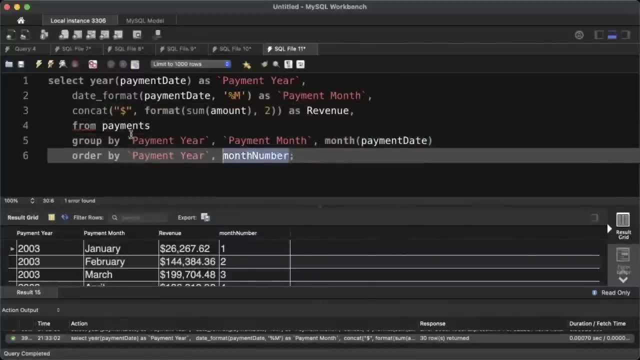 And just put that here. So just put it in group by and put it in order by. okay, So now we saying we select year and we select this payment month, which is nicely formatted, And we select this sum which is nicely formatted as revenue from payments. but in group by we're grouping by this additional condition, this sort of hidden column, which is the month payment date. 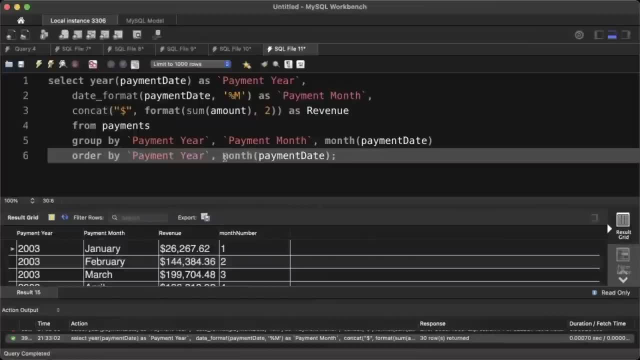 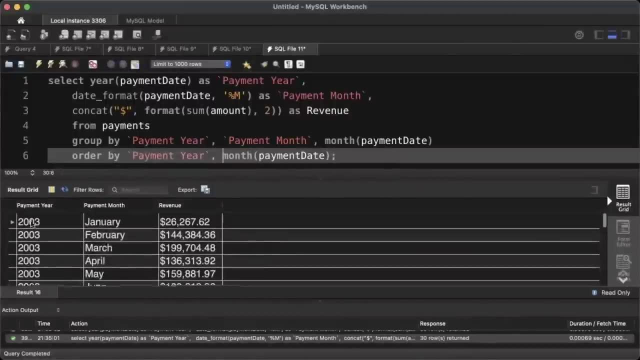 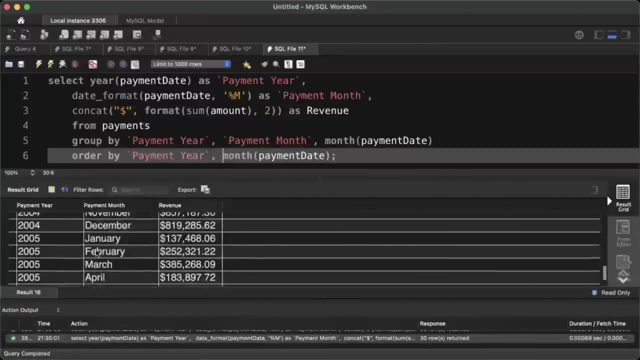 And we are also ordering by this additional hidden column, Which is a month payment date. Okay, And now we finally have 2003,. January 2003,, February 2003,, March 2004,. January February, March 2005,. January February March. 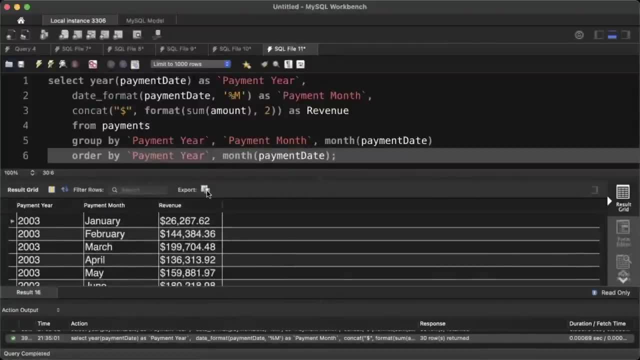 Okay, Now this is the perfectly formatted revenue column- uh revenue table. We export it, put it into Excel or, uh, send the CSV to whoever needs it. Okay, So that's the query. There's a lot going on here. 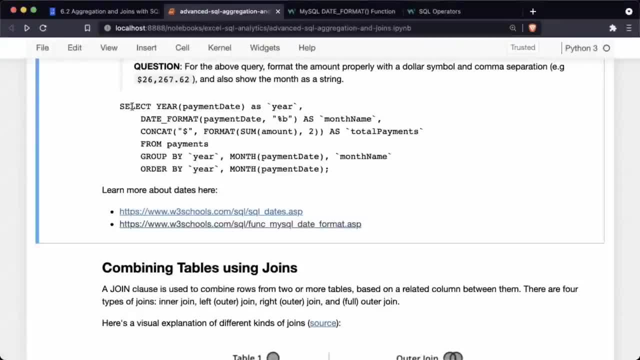 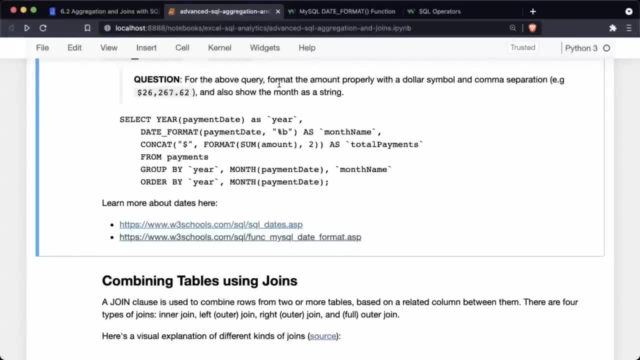 Suspend Your time with it, go through each step And, as I said, what do you want to do? is you want to start with the table? that seems the simplest. uh, just get all the data and keep adding in, keep embellishing the query step-by-step, to cover all the requirements and maybe also just make it look good. 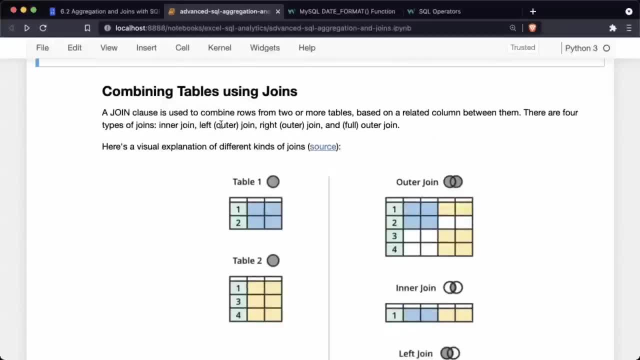 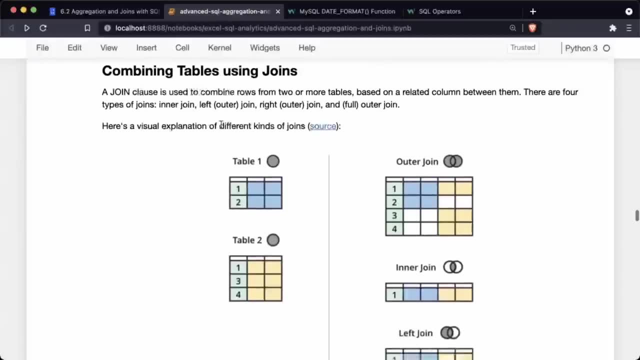 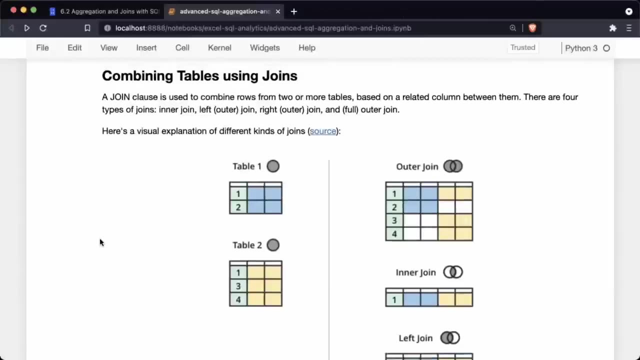 So that's all about aggregation and mapping functions and arithmetic operators And dates. So let's talk about combining tables using joins. A joint clause is used to combine rules from two or more tables based on a related column between them. So here, for example, you have table one which has three columns and you have table two which also has three columns and one of the columns. 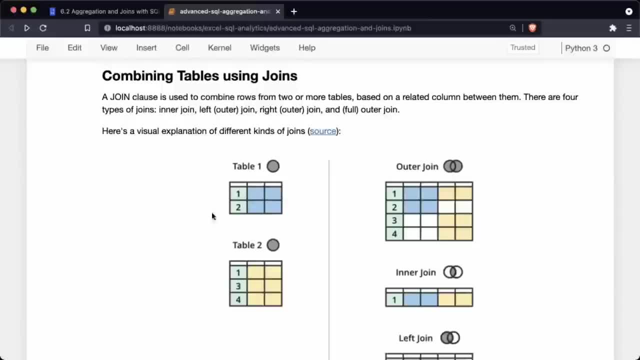 Let's say this is some sort of a shared column, So one of the columns has, uh, is related and has the same or similar set of values. So table one has one, two and table two has one, three, four. So what are you going to do is you can combine the two tables such that you have this one column and then, for this row, one, and then these two values. you also get the information. 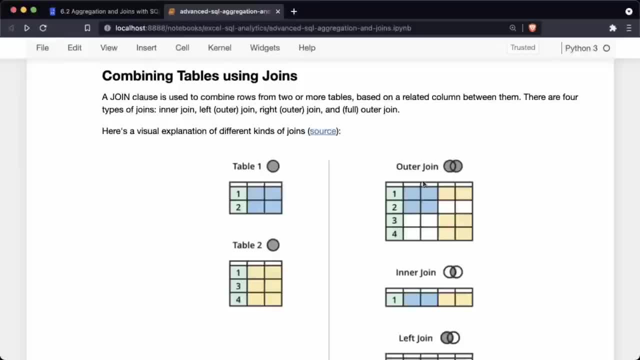 Okay, Okay, So you get the information from this table, these two values, and that creates like a one big room. So you can think of this like the result of the joint. So for the column for the value one, we get the information from table one and we get the information from table two. for the row with the value two, we get the information from table one. here. 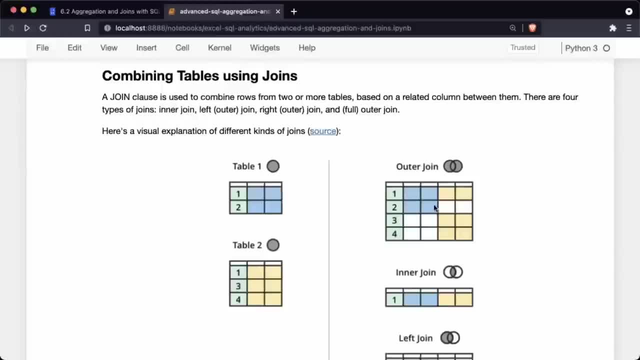 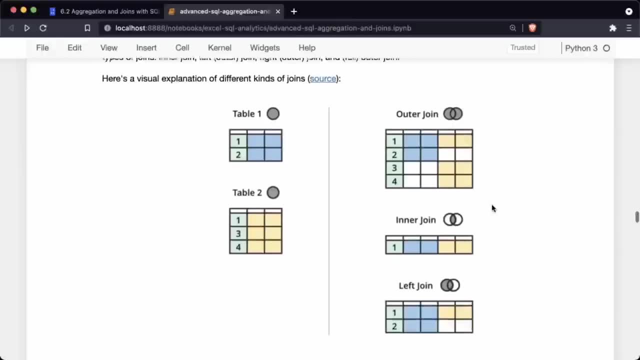 Okay, Okay, Okay. So there is no information in table two. So now what happens here? whether we put empty values or we don't show this row depends on the kind of joint. So if it is an outer joint, then we just show empty values here for these columns from table two. 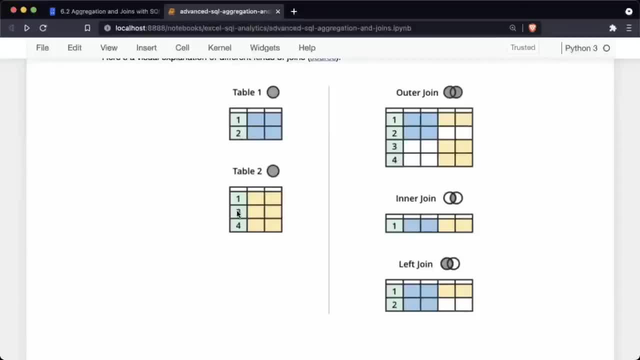 And then here there are no more values left in table one, So we go through table two, we pick these values and we just show empty values here. So we show empty values for uh three for table or for these two columns from table. 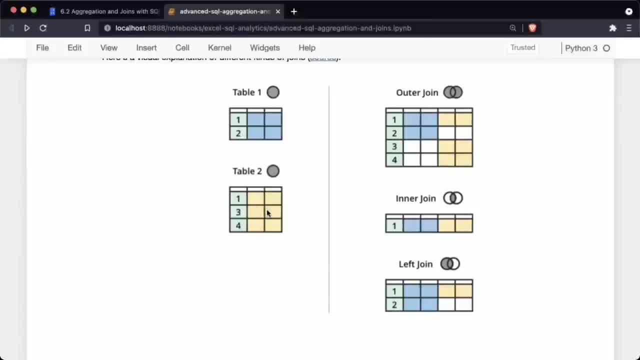 And for the columns from table two we show these values. And finally we have four for which we again show empty values from table one, And we show these two values here for table two. Okay, So that's outer joint, And then we have inner joint which picks just the intersection of the values. 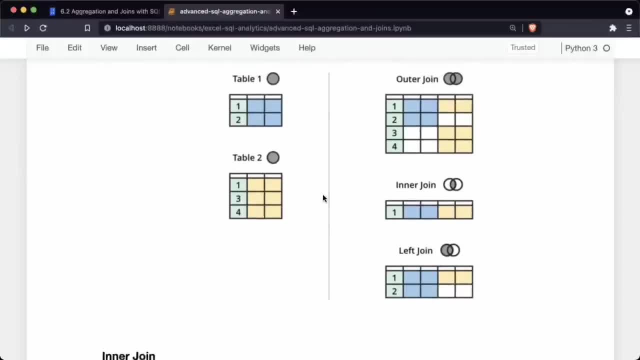 And then we have the left joint and right joint. So let's maybe look at some examples and this will become a lot clearer. The first thing we'll talk about is the inner joint, and this is the default join. Okay, Okay, Join in my SQL. 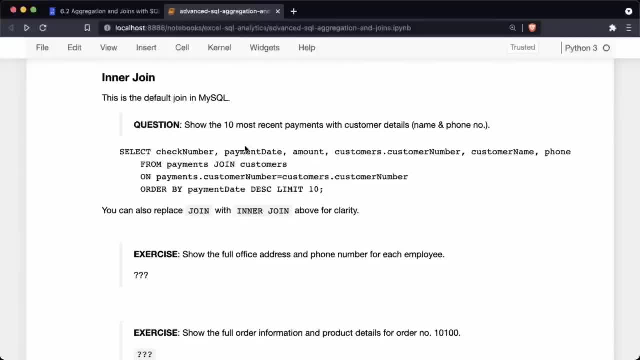 So whenever you type join, whenever you're trying to join two tables on a certain column, then by default it is going to be an inner joint and let's see it in the context of a problem And it'll make more sense. show the 10 most recent payments with customer details. 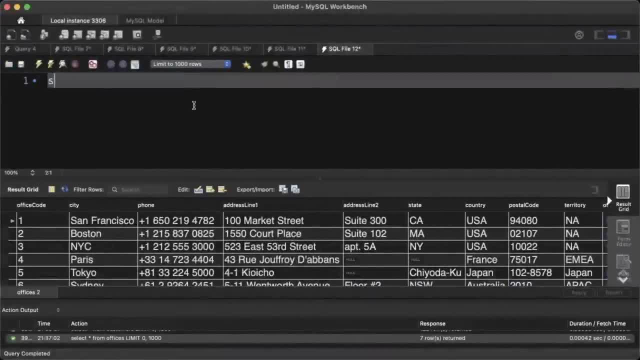 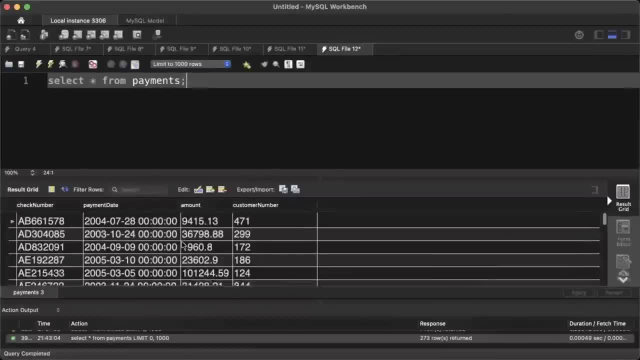 So name and phone number Okay. So let's go select star from payments. These are all the payments that have been made. Now, the trouble here is that in this result we only have the customer number. What we'd like to show is the customer details as well. 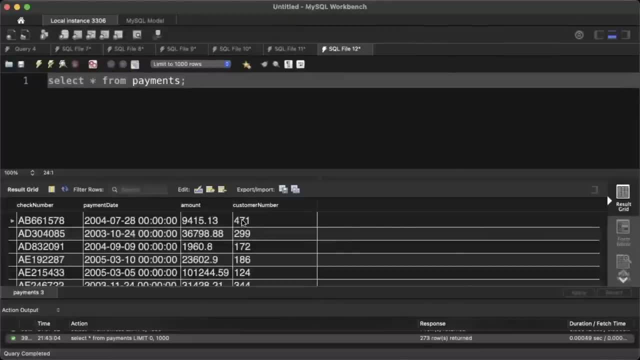 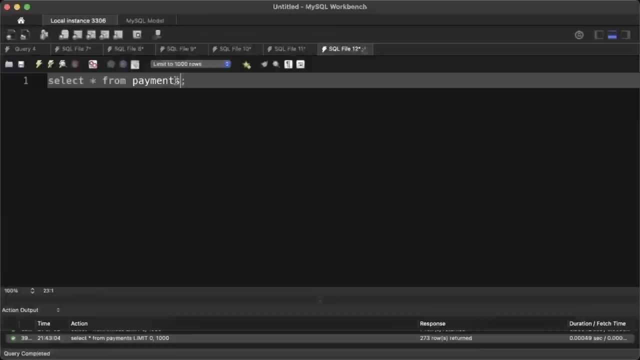 Who is this? customer number? 471, and we will look at the most recent payments. So let me just grab the most recent payments order by payment date, or maybe let's do that part at the end. Maybe first let's get the customer details. 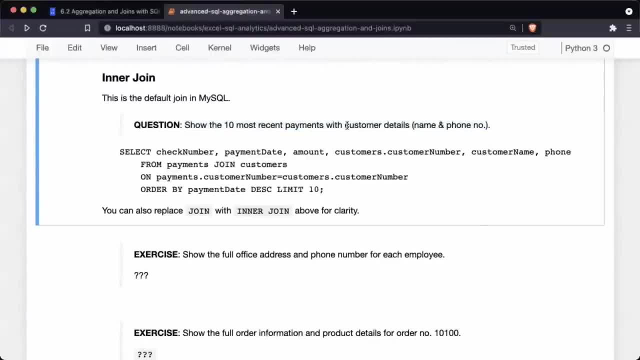 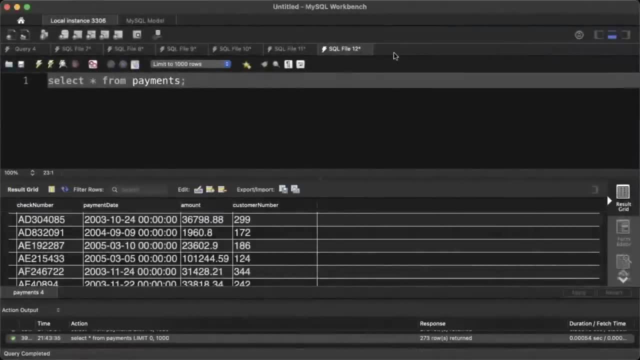 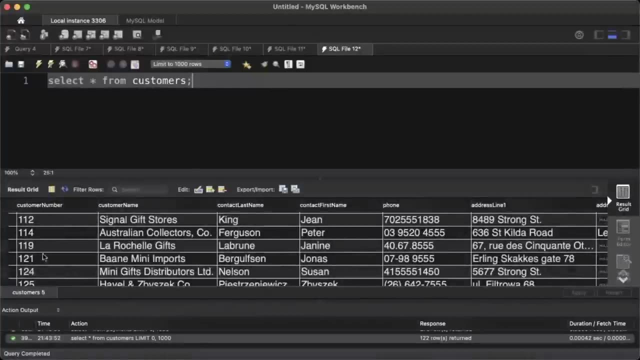 So we have selected Star from payments and we want to show customer details- name and phone number. How do we do that? I know that there is a customer number field in the customer's table as well. So if I do select star from customers, there's a customer number table. 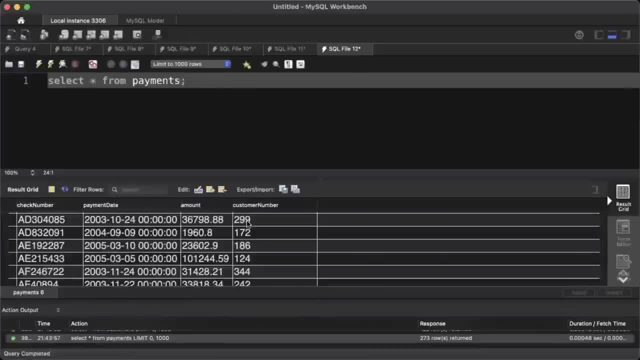 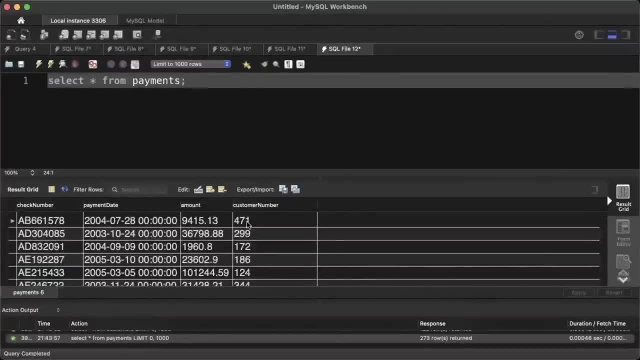 There's a customer number field or column. So what I really want to do is I want to fetch the information for customer number 471 from the customer table. How do I do that? I type select star from payments, join customer number. Okay. 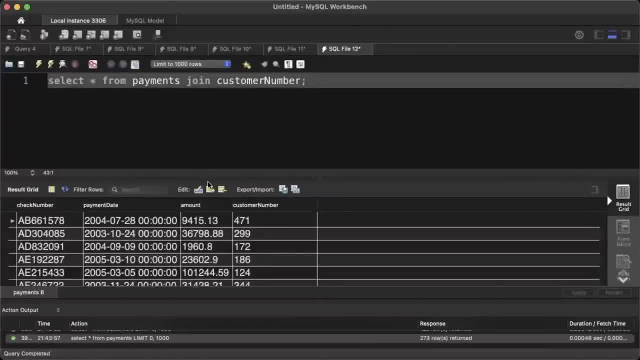 So what did we just do? We said that I want to get some information from the customer number table as well. but how do I decide which? how? how do I decide which rows are connected? Well, I want to use the customer number, right. 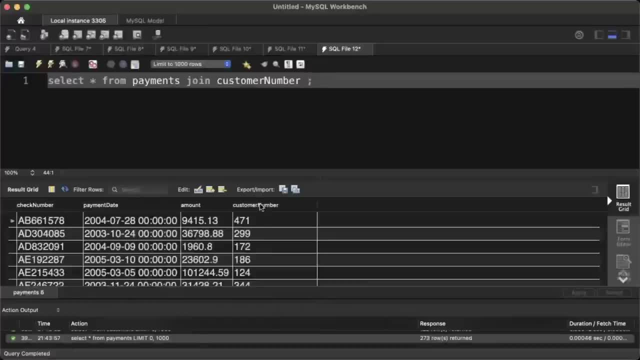 So by default, SQL doesn't guess. SQL requires you to provide How you want to match up the rows of the two different tables. So you say, join on on which column you want to join, and then you provide the column from this table and the column from this table. 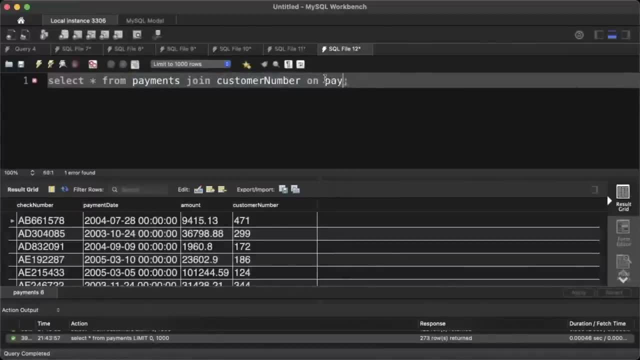 So you said payments join customer number. on payments dot, it's now because there are two tables involved, So that's where you have to specify the the table name before you specify the column name. So payments dot customer number Equals customers dot customer number. 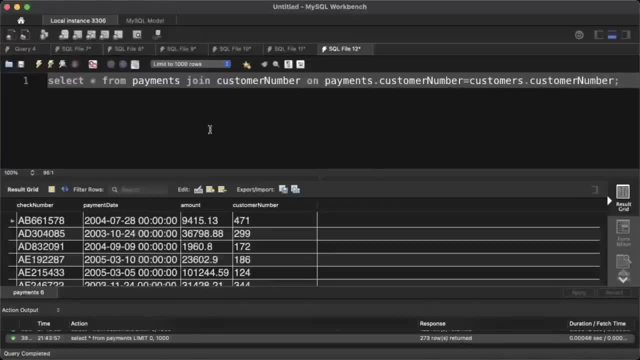 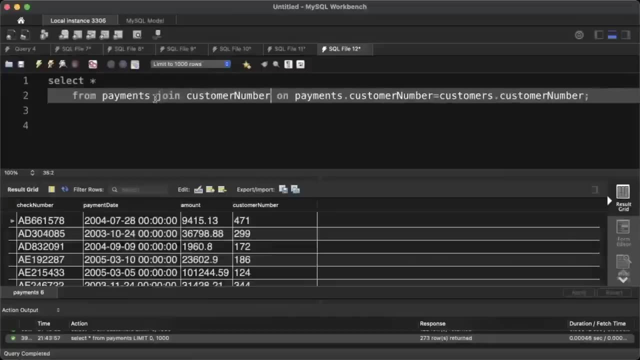 Okay. So let's just try and make sense of this And maybe let's put this on different lines. So we are saying that I'm not happy with the information that I have from the payments table. I also want to get information from the customer table. 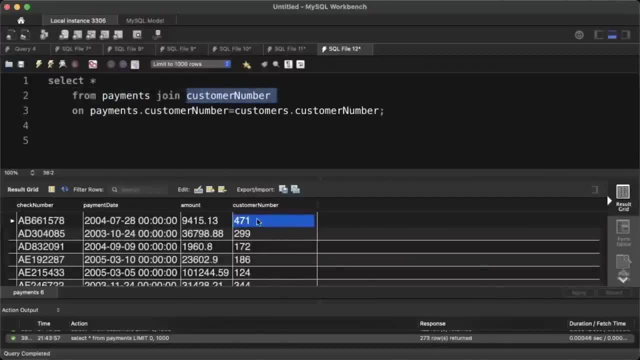 I want- Okay, want- to augment some information here for the customer using the customer table. And how do I want to augment that information? I want SQL on my database server to look at the customer number field in the payment table here. So for this row, look at the customer number field and find the row in the 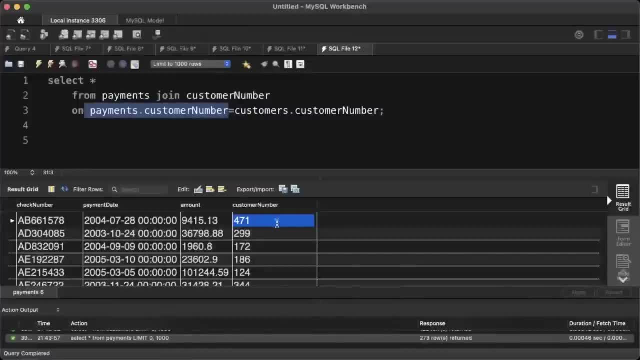 customer's table which has the same customer number. So find the row which has the customer number for 71, get all the information from that row and add it to this row. Okay, Similarly, we want the server to look at the second row and see that. 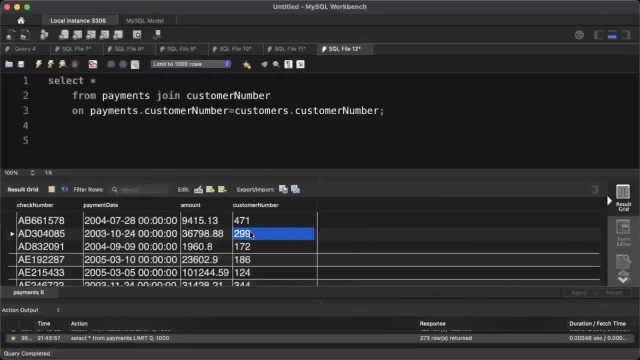 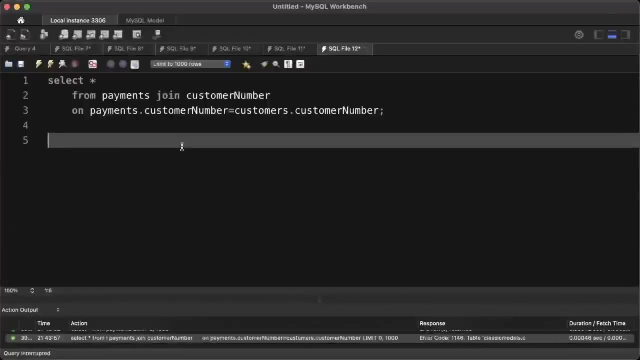 we have customer number 2: 99 here. Find the row in the customer's table which has the customer number set to 2: 99.. So because we're comparing the customer number columns, get all the information from that row and add it here and let's run that. 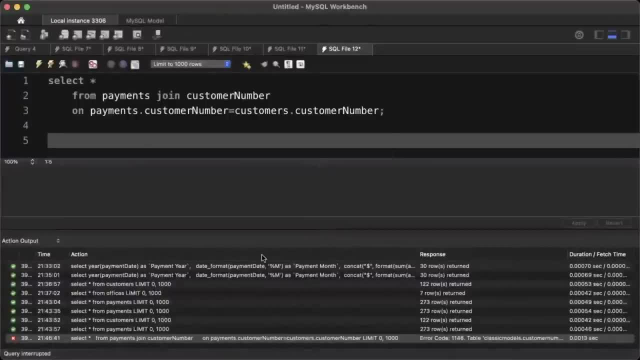 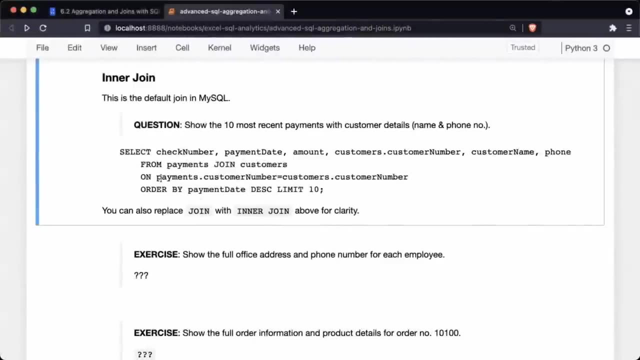 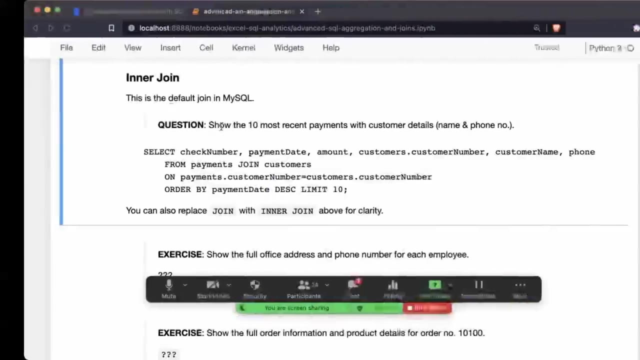 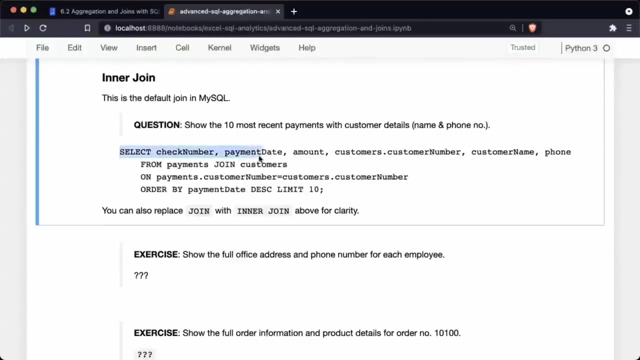 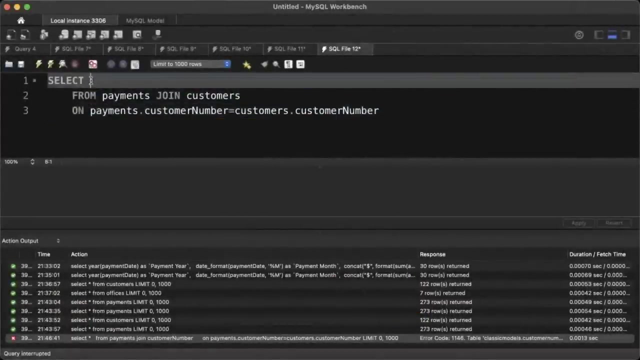 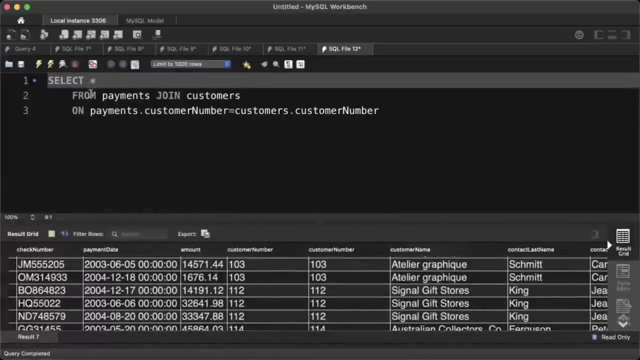 Okay, Did that lead to an error? Let me just check this. Um, maybe I have a, maybe I have a typo here somewhere. but yeah, sorry, I think I had a typo there. but yeah, just repeat: select star from payments. join customers. 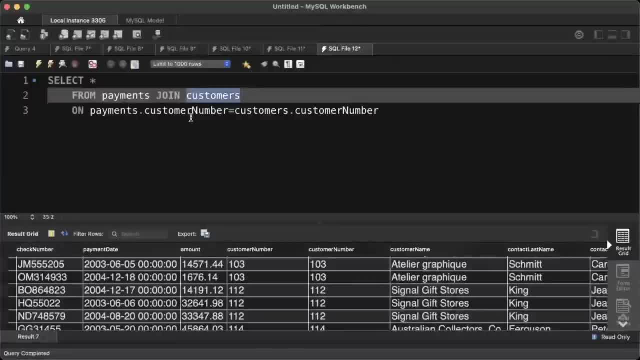 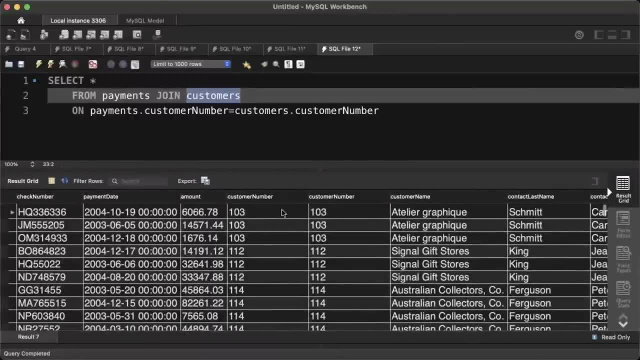 So you want to join payments with customers on the column customer number. And now what SQL is doing is it looks at a row in payments, It sees a customer number there, And when it sees a customer number from the payments column, it looks for a row within. 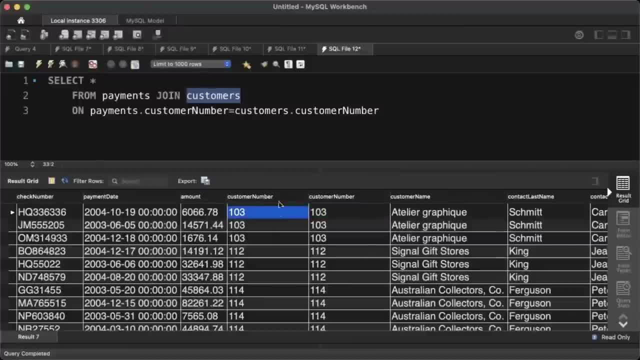 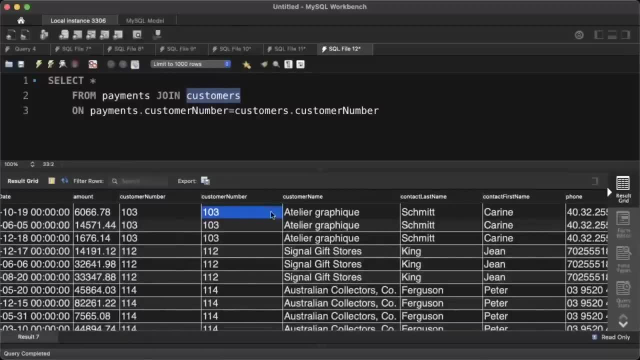 the customer's table with the same customer number. So this customer number comes from payments and this customer number comes from customers, And then it takes all the information for that row and it adds it to this row. So now we have not just the payment information, but we also have the customer. 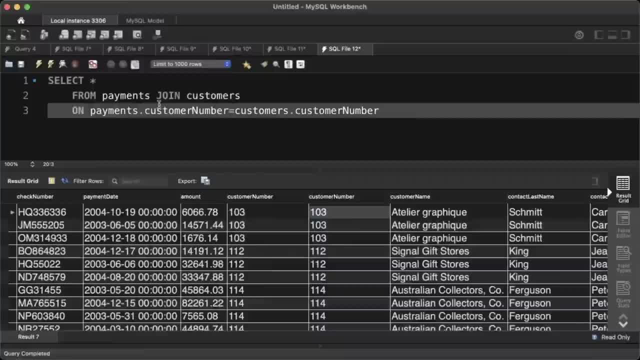 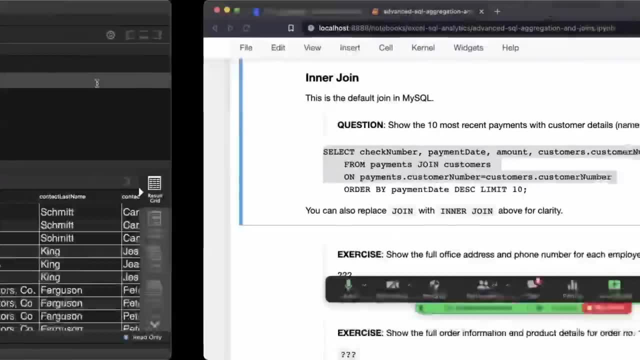 information attached with each payment. So that is join. Okay, Now we probably don't want all the rows here, So that's why we may want to just select some rows. So I'm just going to select check number, payment date, amount, um customer number. 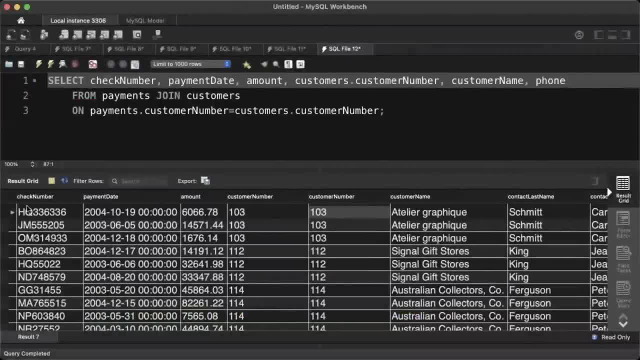 customer name and the phone number. So I just keep the check number, payment date, amount. And I just want to keep one of these columns, because these columns are a bit ambiguous, They come from both, So I'll just keep customers dot, customer number, which I know is going to be equal. 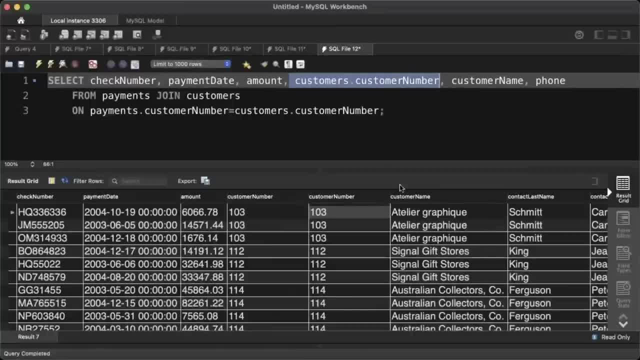 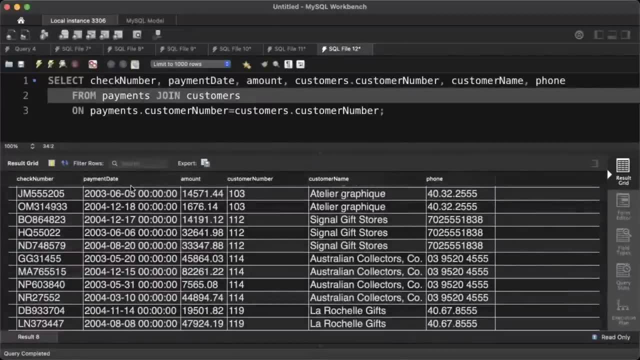 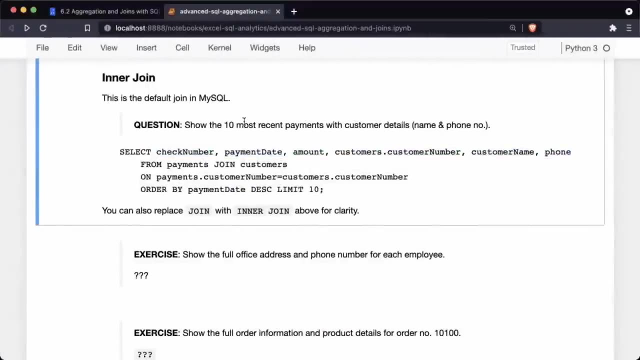 To equal to uh payments or customer numbers, And then I'm just going to keep the customer name and phone number. Okay, So now we have check number, payment date, amount, customer number, customer name, phone number, and then we can now cover the additional criteria, which is, we want to show just the 10. 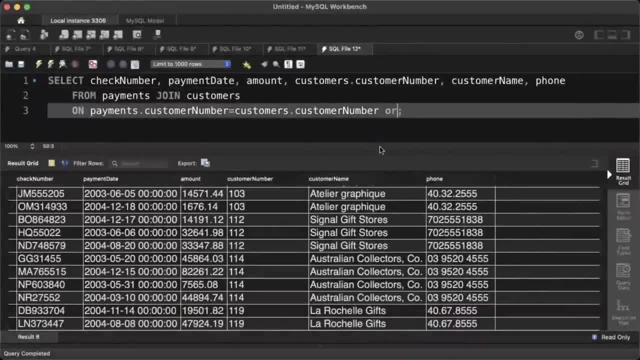 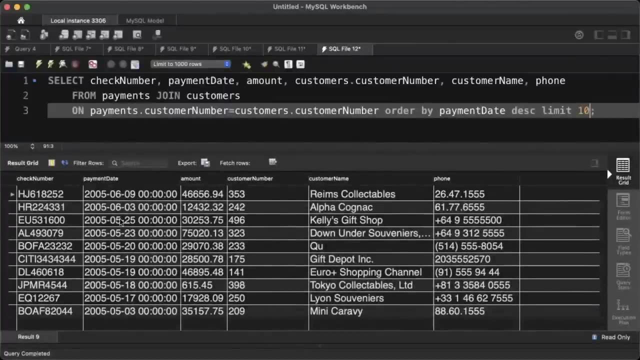 most recent payments. So we want to order by order by payment date descending and limited to 10.. Okay, So now we have just 10.. Now we have just 10 payments, the 10 most recent payments, and you can verify this that these are the most recent payments. 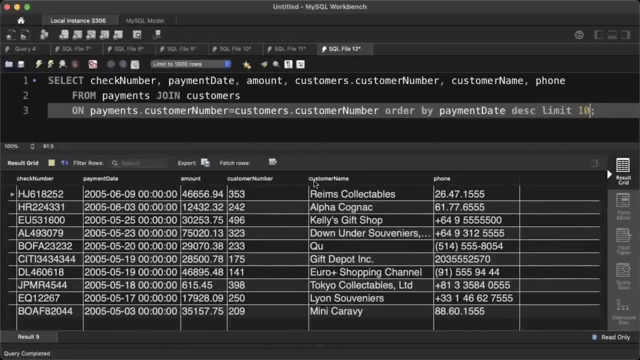 6 0, 9, 6 0, 3, 5, 25 and so on, And then we have the amount, customer number, customer name and the phone number. Okay, Now the key thing for you to understand here is the join: how it is, how it, how it works. 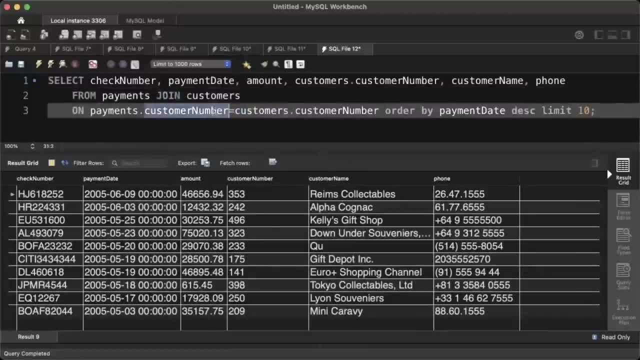 It looks good That payments looks at the value of customer number and it picks a row from customer number which matches it. Okay, And this is an inner join. What does that mean? Well, there are several customers who may not have made a payment in the last 10 days or who may not have made a payment at all. 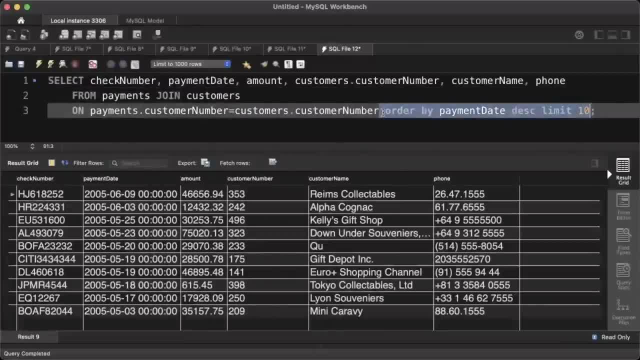 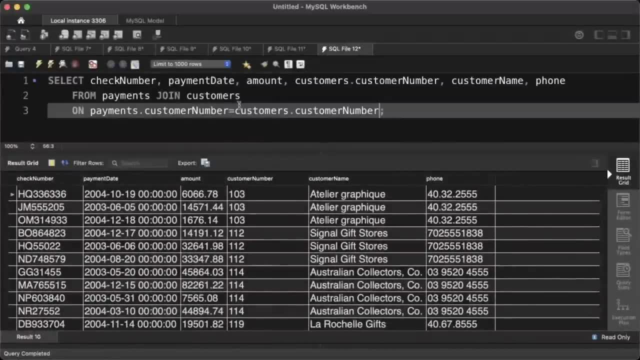 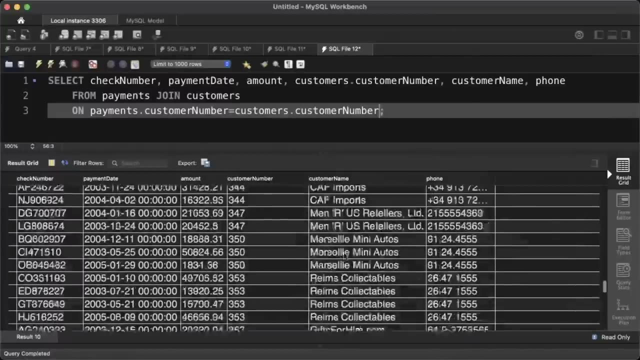 So if I remove this for a moment, order by et cetera, there are several customers who may not have Made any payments, So I probably don't want to show the information for those customers who have not made any payments right now, if I do this in a joint here, or if I do this: 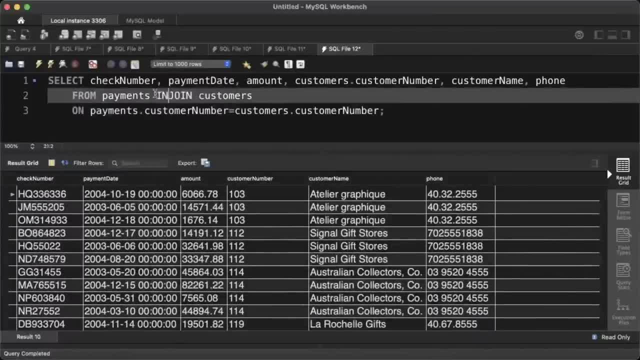 normal. this is the inner joint. I can also type inner. then what I'm telling SQL is: don't show me customers for which I don't have any payment information. But if I change this to outer joint now, we are telling SQL. 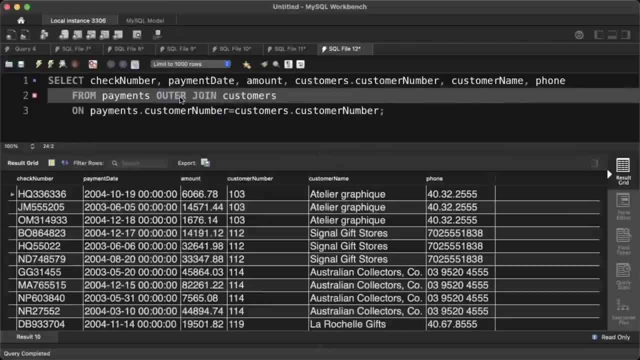 Okay, maybe it's like a full outer joint or that we look up the syntax, but if we change this to a outer joint, then we would get information for all the customers, right? So we would not only get information for customers who have made payments, but we would also get information for customers who have not made payments. 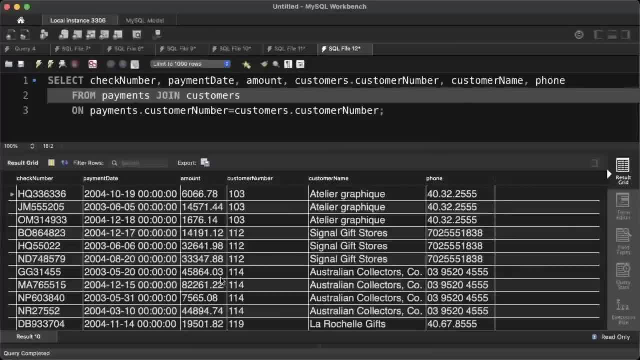 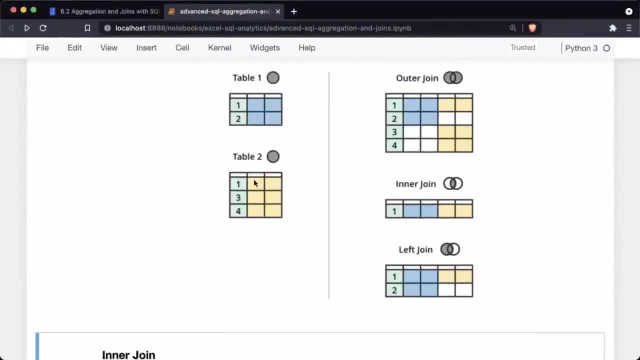 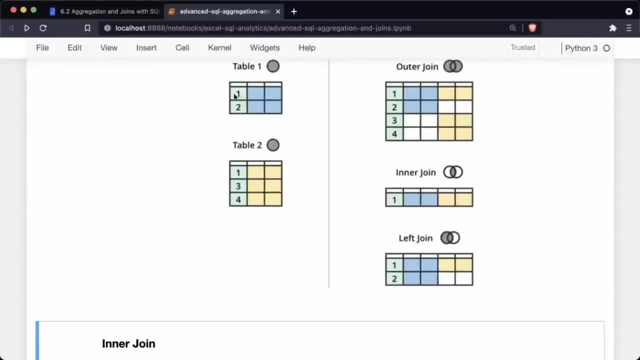 And what is going to be present in the check number, payment date and amount columns? Okay T, it's just going to be empty. So just going back here, if table one is payments and table two is customers, then when you do an inner joint, we only look at those rows where these values are present in both the columns. 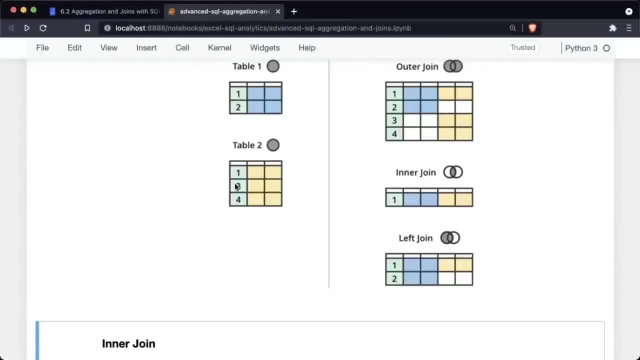 For example, if customer number one and two occur in payments and customer number one, three and four occur in customers, then we will only pick one, because that's the common column. And that's what happens when you do an inner joint: it just picks the common values on. 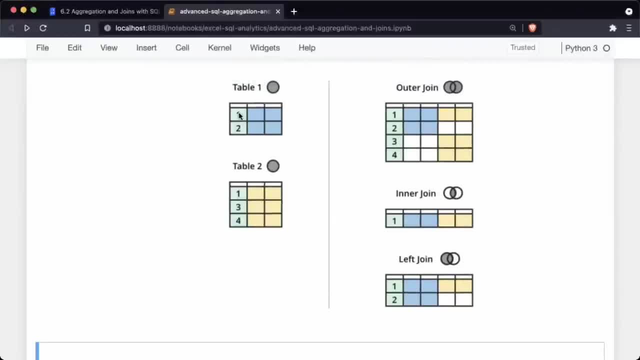 Yeah, On the other hand, if you do an outer joint, then we're going to pick. we're going to have a row of a row for customer one, We're going to have a row for customer two- These two are in payments- and we are going to have a have a row for customer three and four, which don't really show up in the customer's column in the payments table at all. 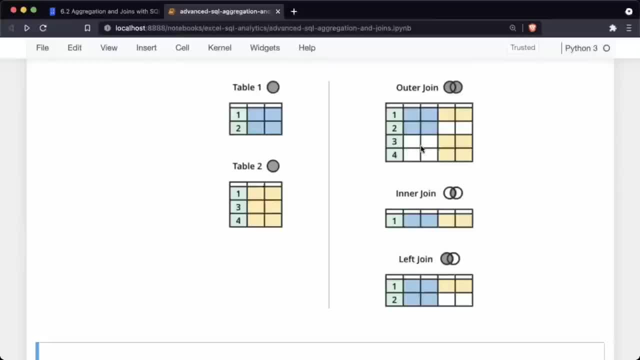 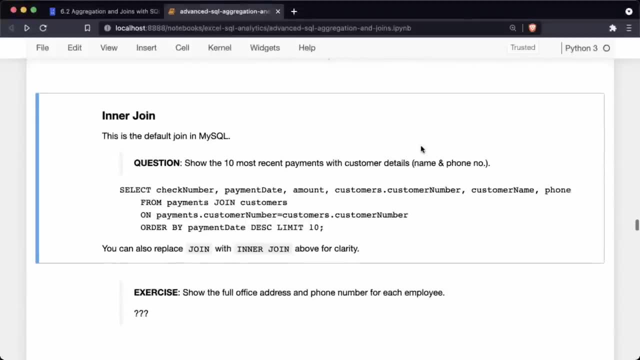 So this is what it's going to be, And there is just going to be empty data here, Okay, Um. then there is a left join and right join, So we look at these in a second too, Okay, Um. but 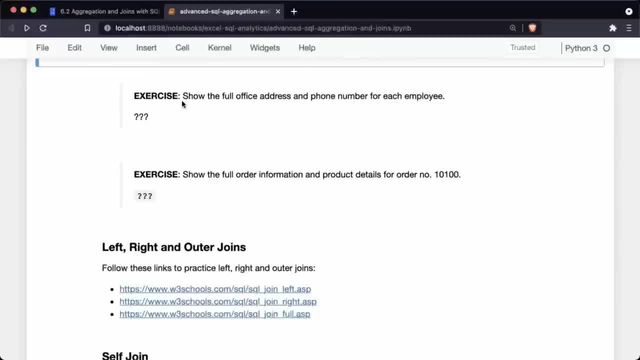 Before we look at left, right and outer joints, here are a couple of exercises for you. show the full office address and phone number for each employee, So once again you can guess what this will look like. You will say: select star from employees. 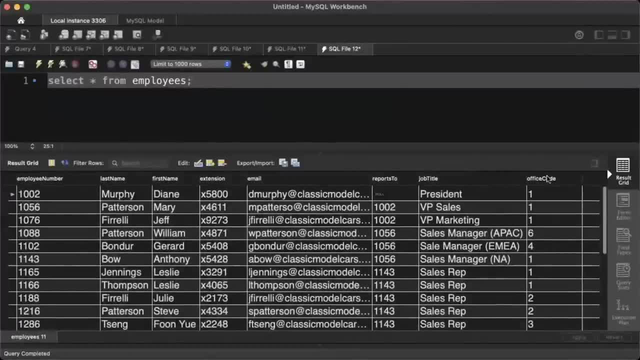 And of course, now you want the full office data, So you have an office code here. So you want to do join with offices on employees: Dot Office code equals offices, dot office code And maybe let's just put the employee number here. 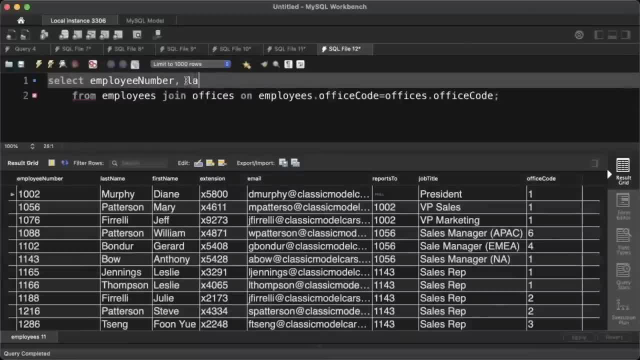 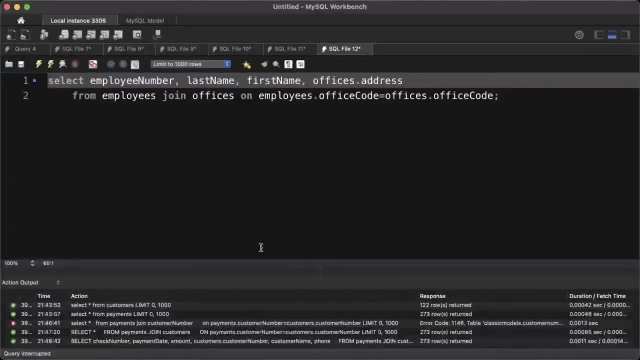 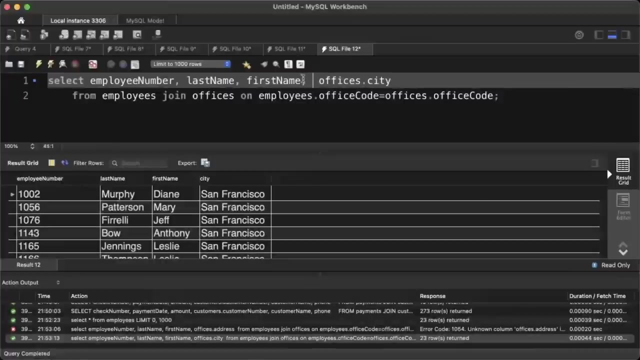 Let's just put employee number and let's put maybe the last name, first name and offices dot address. Let's just put city, right now, offices dot city. So now you have employee number, last name, first name. Let's maybe also put office code. 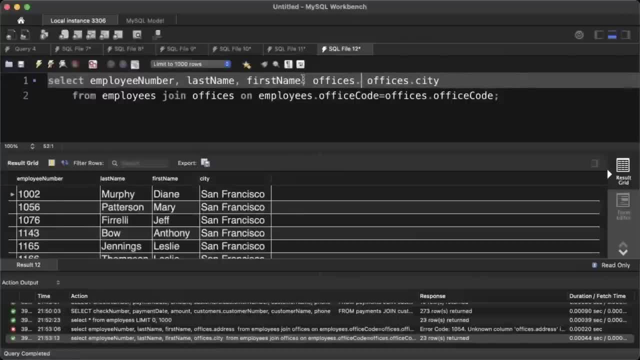 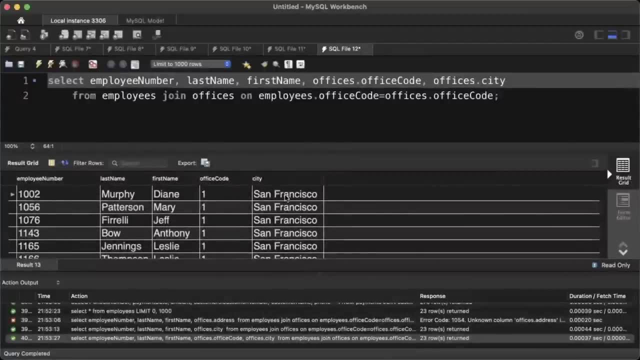 So office is dot office code. Okay, So now we have employee number, last name, first name, office code, city, city, San Francisco, And then we also want to show the full phone number. So office has a phone number. 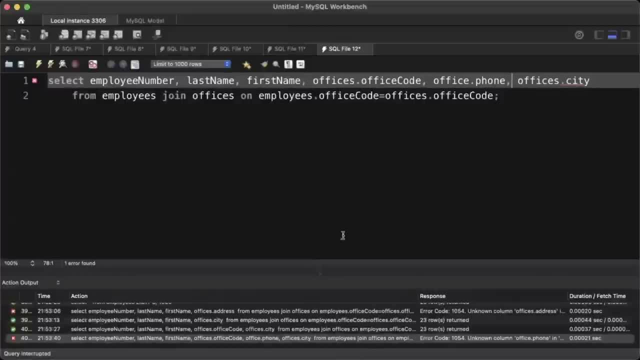 So office has a phone. Let's check what that is. Select star from. So office has a phone. Um, so we want to show the offices- offices dot- phone information as well. So now we have the phone and then every employee has an extension. 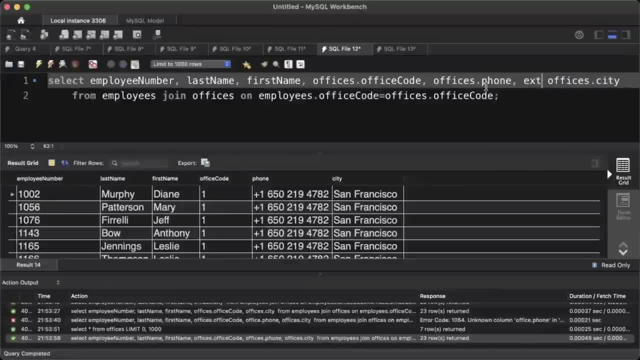 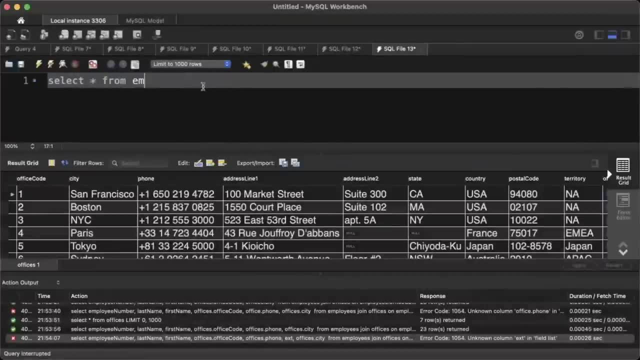 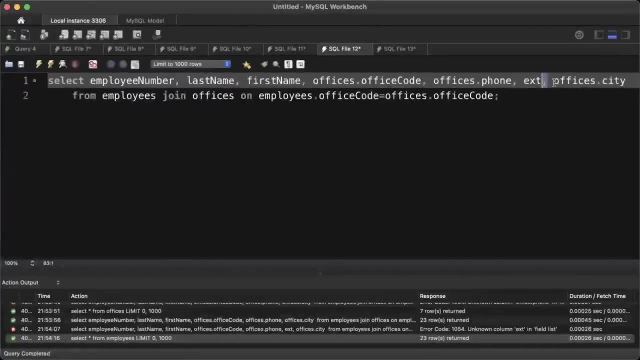 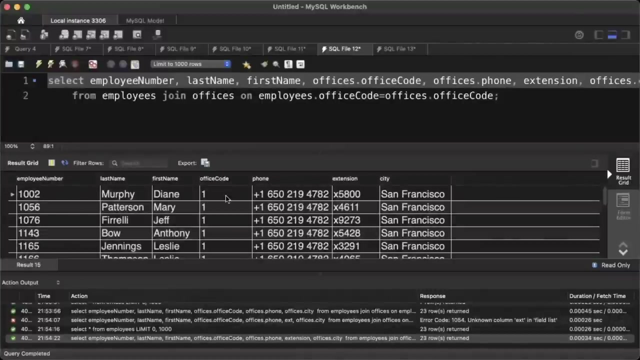 So we can get the ext column from employee. That is the extension. Let's just check that. select star from employees: extension. So every co, every employee, has an extension. So now we have employee number, last name, first name, office code. 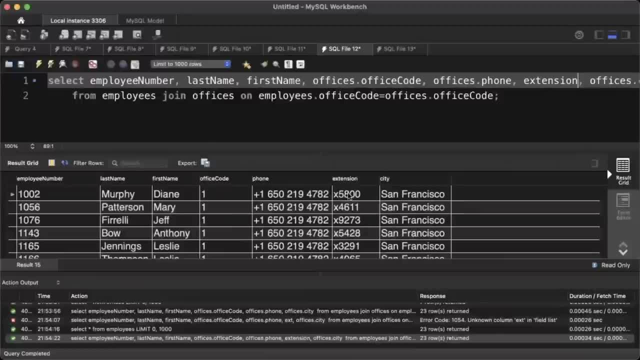 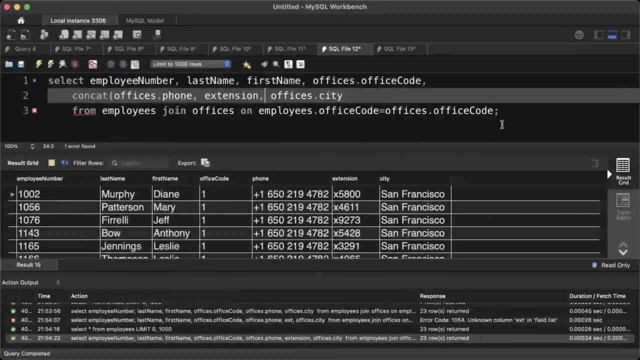 We have the phone number Um, we have the office city and we have this extension. We can combine these two so we can say concat, Let's get that here. so we can say concat, and we can concatenate the office phone with the extension. 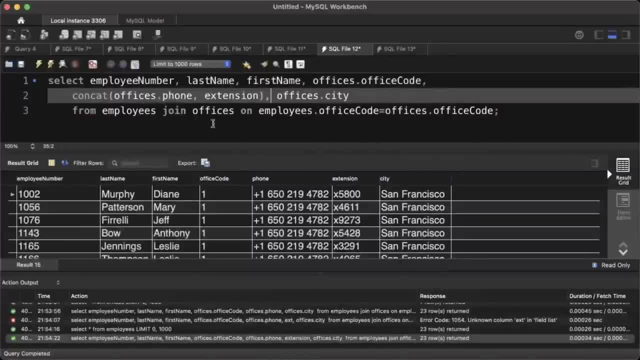 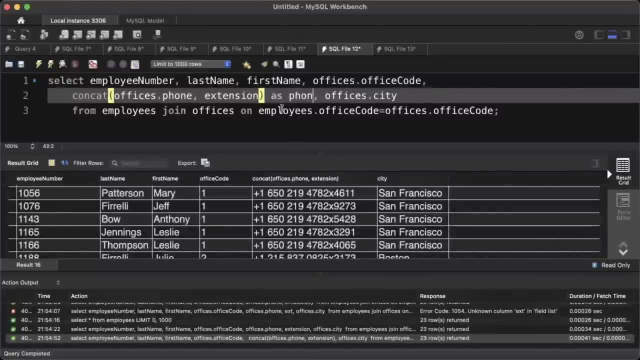 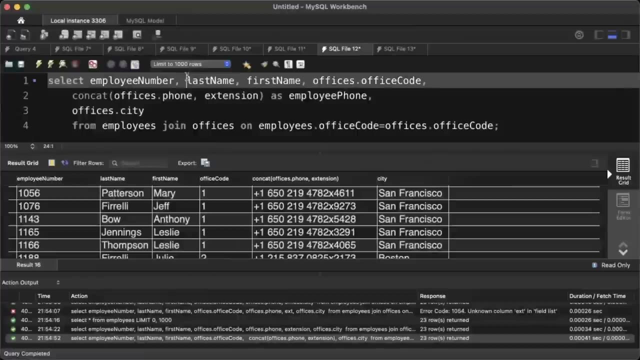 So now we are concatenating one column from the offices table and one column from the employee table and put those together And let's just call that um, employee phone number or employee phone. Okay, So now we have the employee number, Okay. 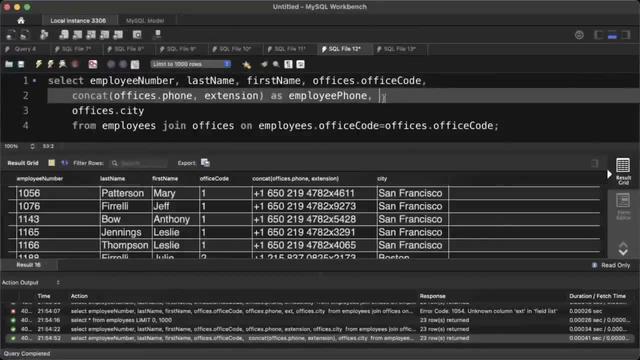 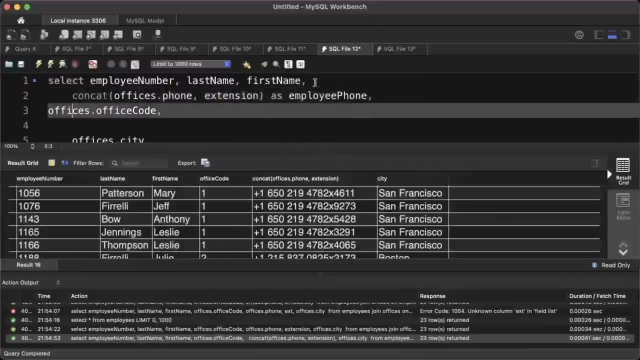 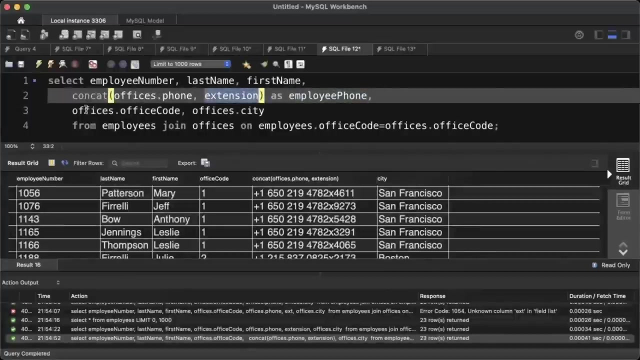 Last name, first name, office code and employee phone number. Maybe let's just put that here. Okay, So now we have an employee number- last name, first name- and then we have the employee phone number, which is a combination of the phone number from office and the extension from the employee table. 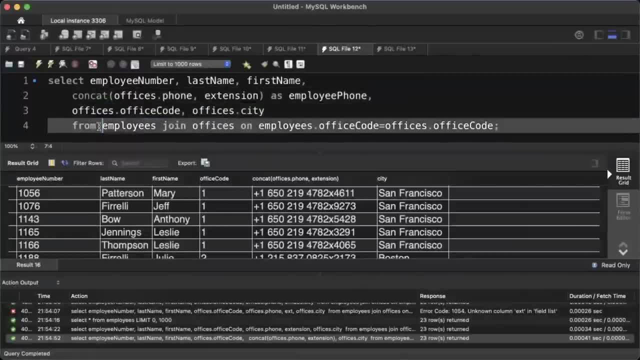 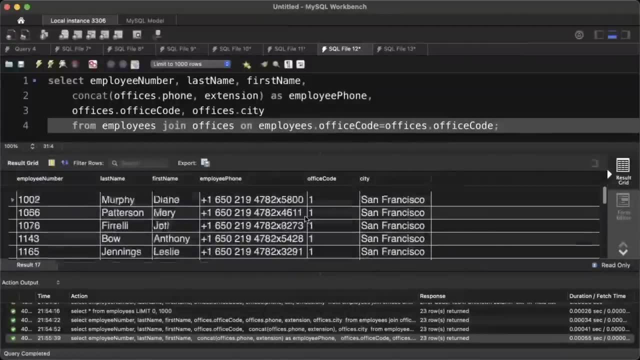 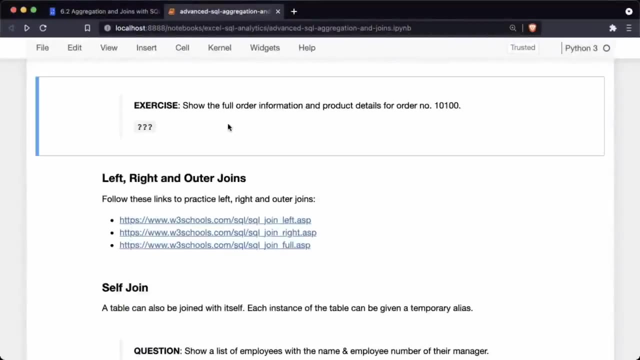 And then we have the office code and office city, and we've been able to do this because We've done a join between employees and offices. Okay, And that's what this looks like. Here's another example. show the full order information and product details for the order number one: zero, one, double zero. 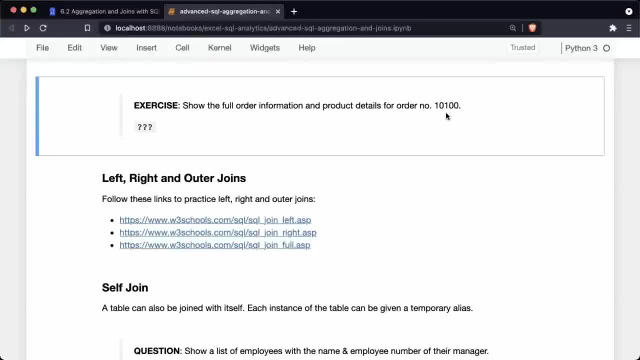 So here you would have to look up the order details common or the order details uh table and then from the order details table you would have to uh join it with the orders table to get information about orders, And you would have to join it with the product table to get information about the product. 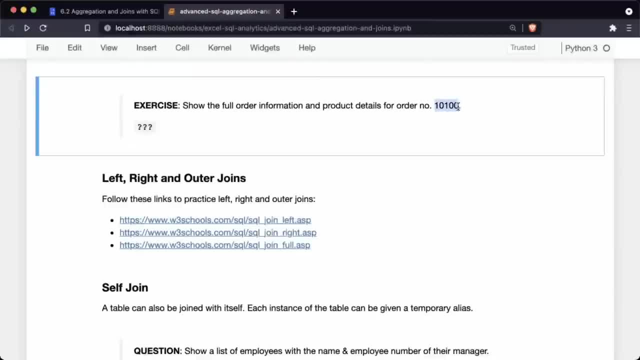 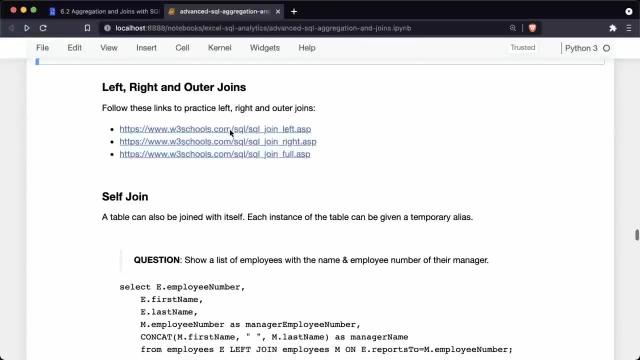 And then you would simply have to select the data for a specific order number. So here you are doing two joints or you're joining three tables. So I'll let you figure that out. It's not too difficult, It is just. it is just one more step removed from what we've done. 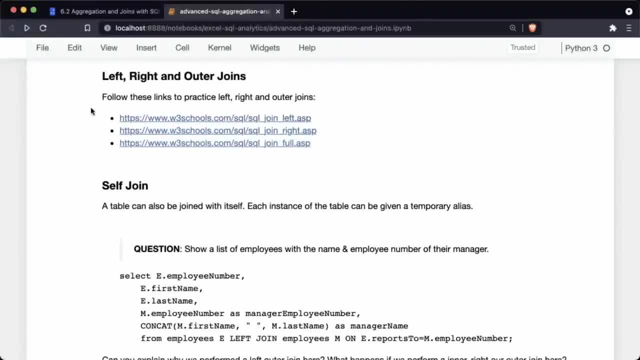 So that's basic joints and specifically that's inner joints. Now let's talk about left joint, right joint and full joints. unfortunately, in this data set there's not enough of an opportunity to demonstrate all three, So we're just going to look at some examples online and specifically, I recommend w three schools: 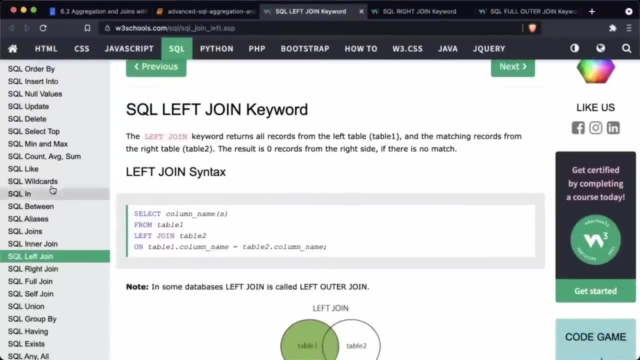 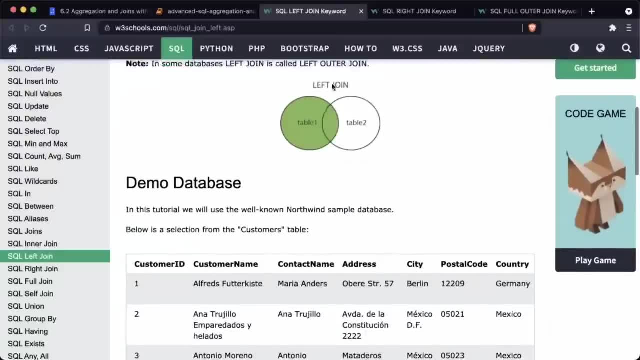 If you're just looking at some SQL syntax or need some help with SQL, they have pretty good documentation on all of these. So let's talk about left join, Okay. So here's how left join Okay, And you can look at this table and try, look at this picture and try to understand what's happening. but we have a demo database here. 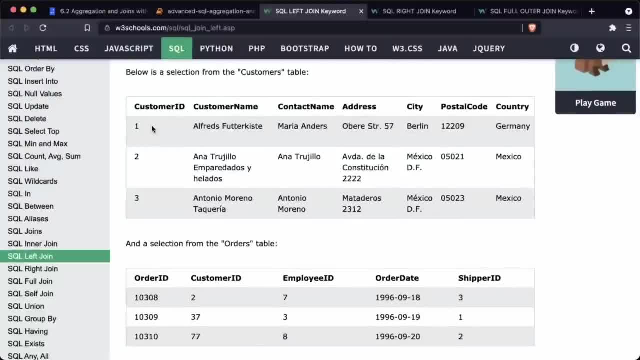 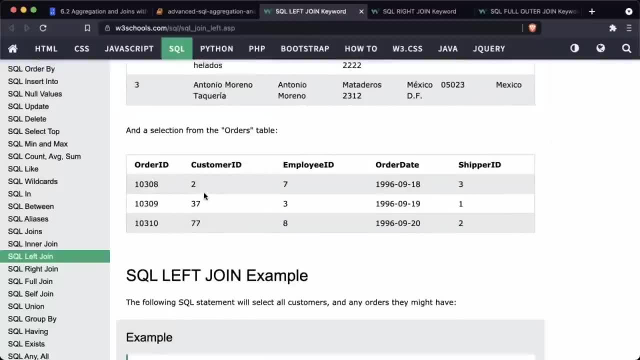 So we have this customer's table and in the customer's table we have a customer ID- one, two, three- and then we have a customer name, contact name, et cetera- And then we have an order stable. So the customer stable will be on the left. 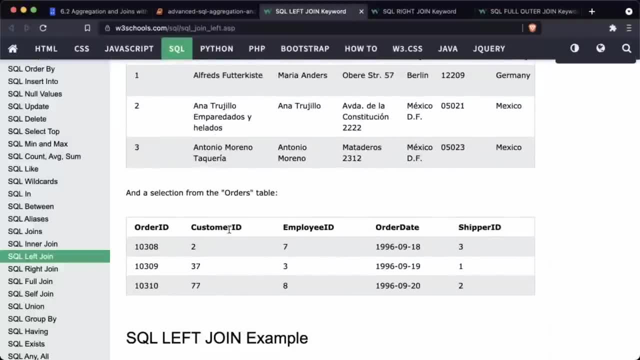 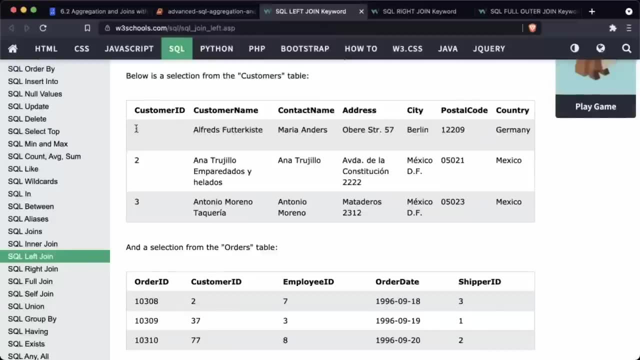 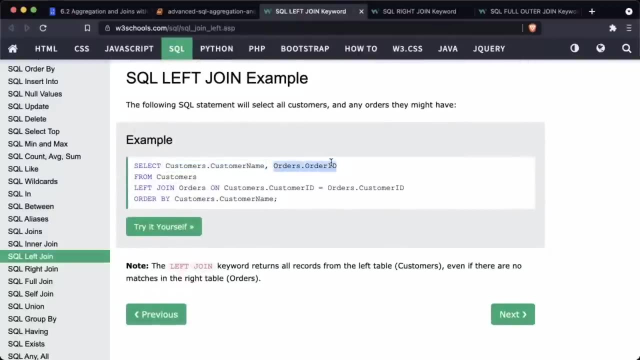 The customer stable will be on the left and the order stable will be on the right, And what we want to do is we want to join customer stable with the orders Stable on the customer ID column. So we say select customers dot customer name, comma orders dot order ID. 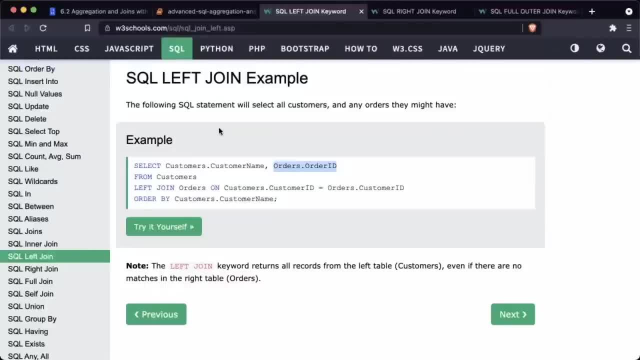 So we want to look at for each customer what are all the orders they've placed right. So we want to see customer name and we want to see the order ID from the customer stable left joined on orders on customers dot customer ID equals order dot- customer ID. 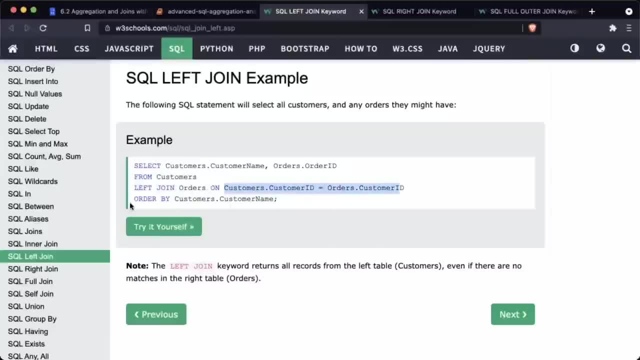 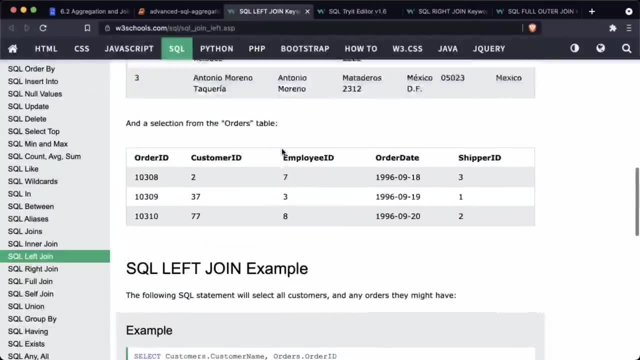 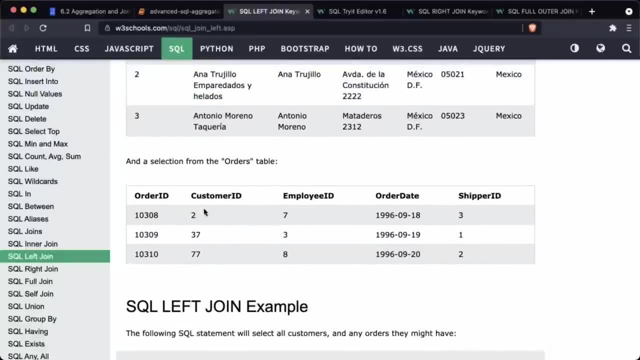 So we want to just combine on the customer ID column and we want to order by the customer name. So let's run this on. you can actually run this online and check. So here's our database. We have three customers and then we have three orders. of course, 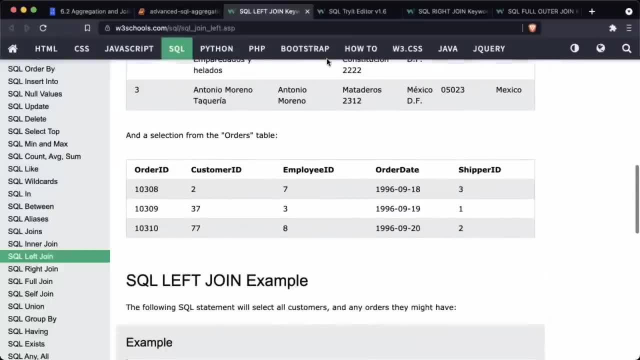 And okay, Actually there's. there's more than that. There are a bunch of customers and a bunch of orders, So let's just run this and let's see the result. Okay, In our database we have 90.. Okay. 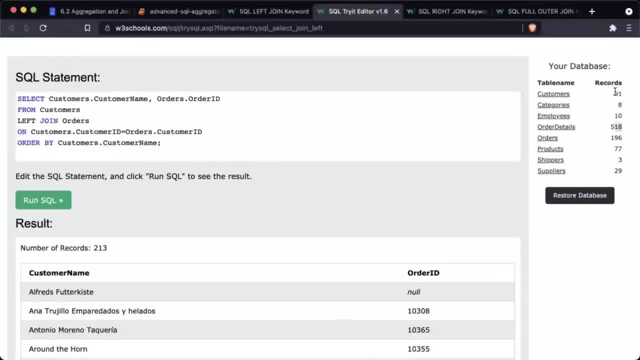 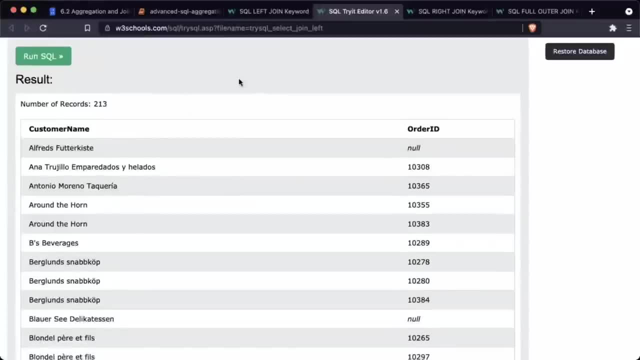 One customers and we have 518 orders and not every customer has placed an order. So when we do a left join between customers and orders, here's what we get: We get a customer name and then we get the order ID. So it turns out that Alfred F hasn't prayed, hasn't put, hasn't created any orders. 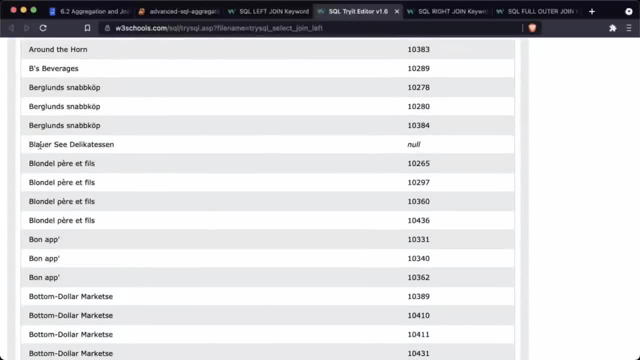 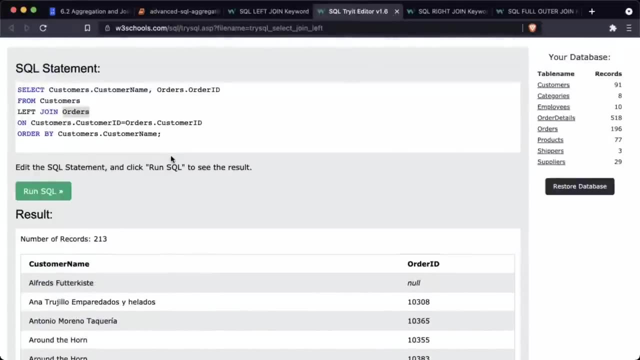 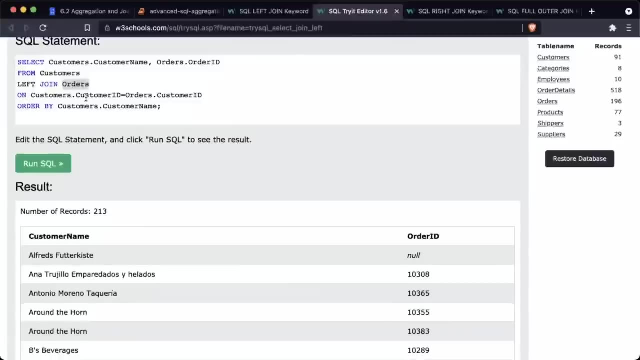 So that's why we have null here. And similarly, this person hasn't created any orders. That's why we have a null here. So For every customer and every order we could find, for every customer and order combination We could find where the orders customer ID matched with the customer's customer ID. 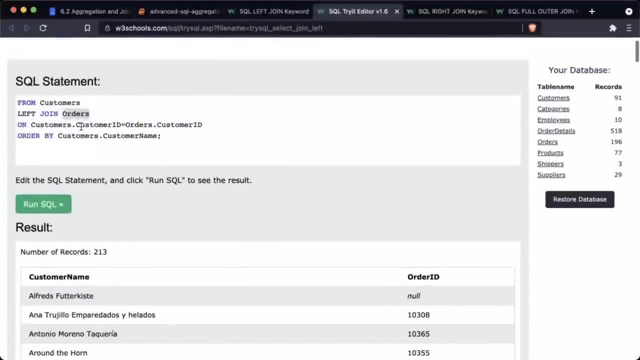 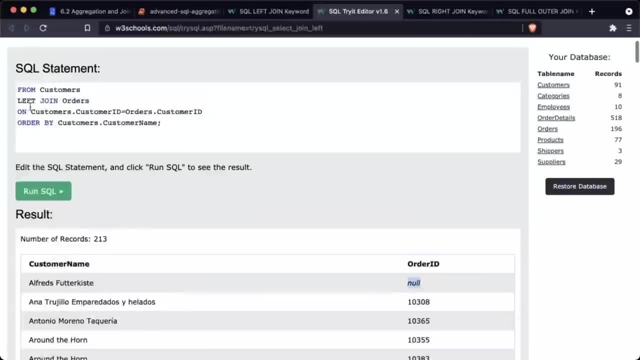 We have created a row and, because this is a left join, wherever there were certain customers for whom there were no orders, There is still a single row that has been kept. So Alfred has not ordered, but we still have this null here. Now, if we did not have this left joint, if we just had joined here, 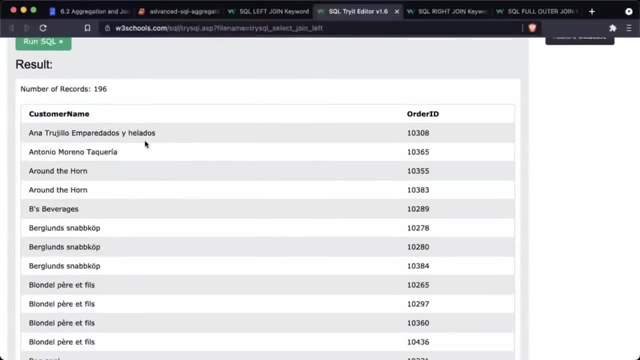 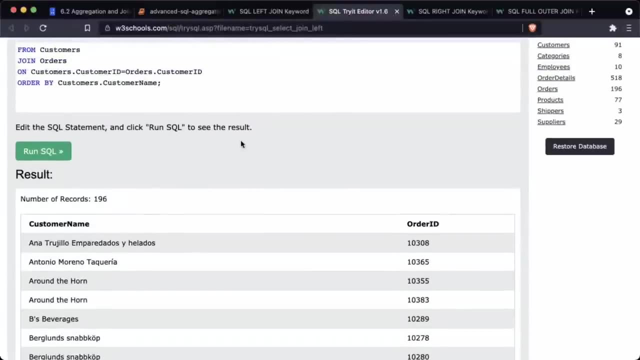 And let's run that. you would see that now you no longer have those null columns, So now you no longer have a customer name. So if a customer does not have a matching order, so if a customer- caller, customer row- does not have a matching order row, then that will be skipped. 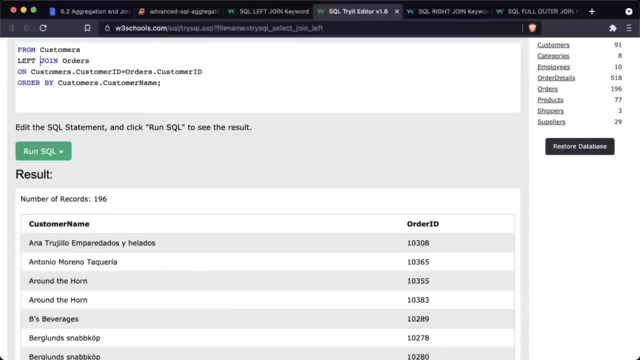 If you're doing a left joint, you are telling SQL that you want to keep all the rows from the left table, which is the customer's table, And you don't care about all the rows from the order table, but you do care about. 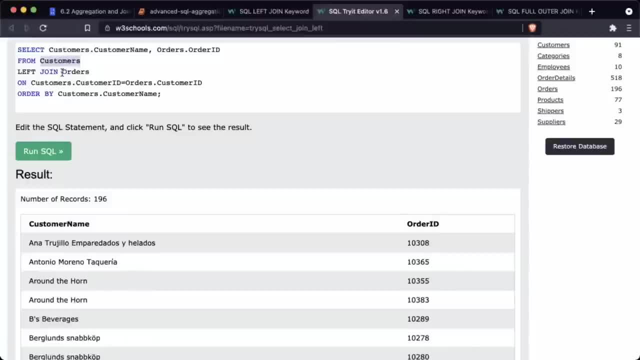 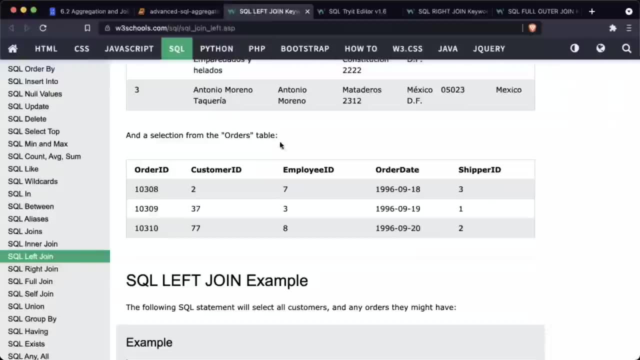 All the rows from the customer's table. So even if there is no matching row from the order's table, just show that customer name and then show a null there. Okay, So that's left join. Then maybe let's look at right join. 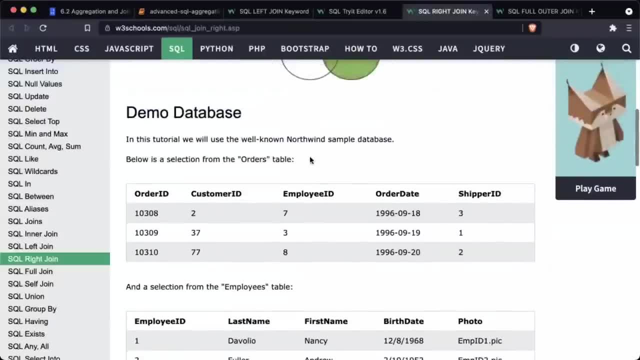 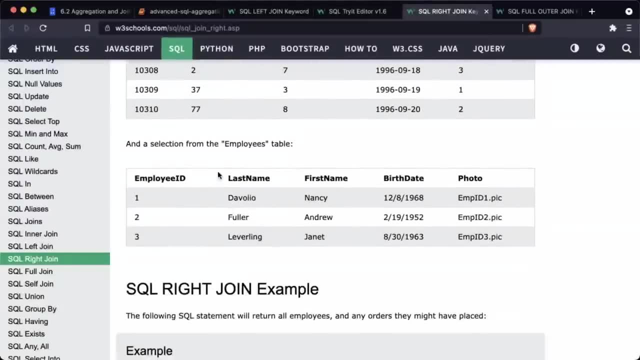 So here's an example of right join here. We have orders, So we have one table of orders, and then we have one table of employees. Okay, Now, For every order that is placed by a customer, there is also an employee that is assigned. 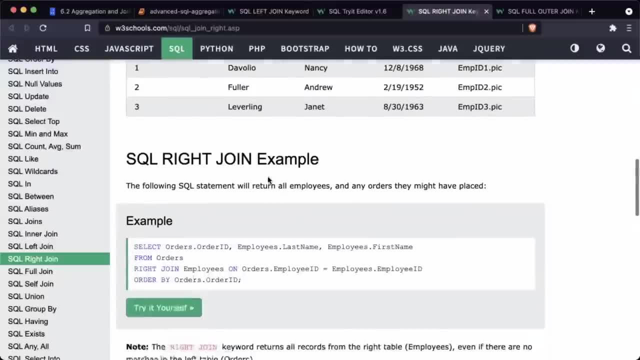 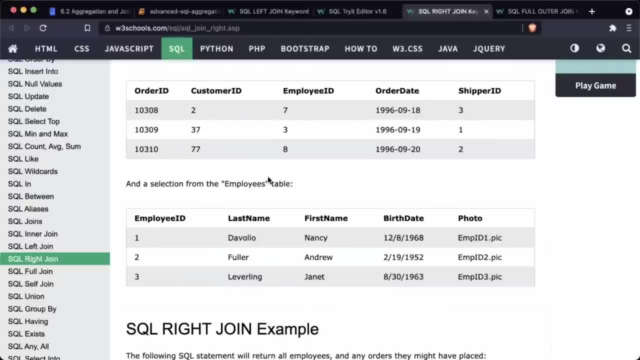 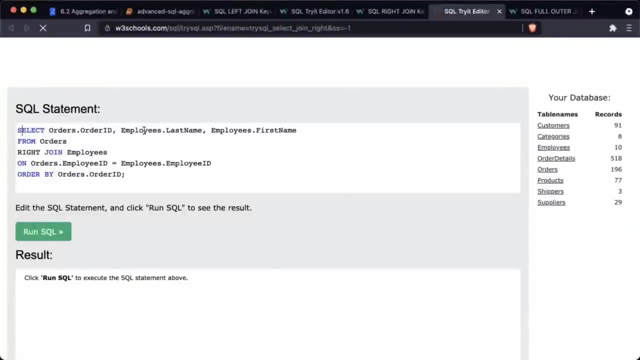 And then we have a table where we have details of employees. So let's say we want to get for each order the names of employees, who is assigned to that order and let's check it out. So this time we are saying select orders, start order ID and employee last name. employee first name from orders: 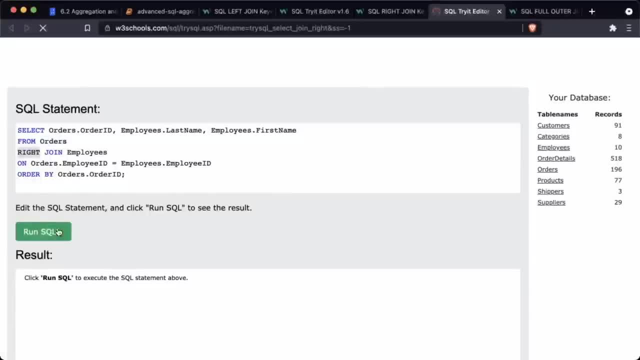 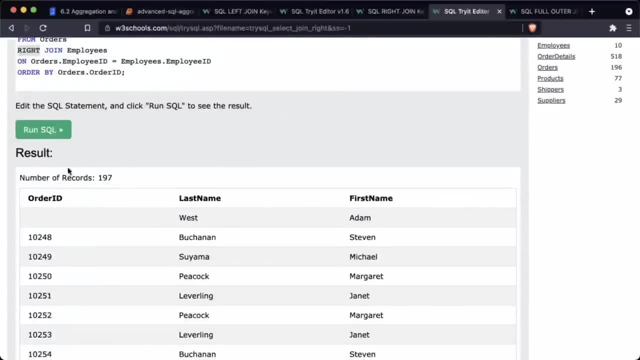 And we are saying, right, Join with employees. So let's run that and let's see what what happens. We are matching on the employee ID column So we get the order right, We get the order ID and we are also keeping the employee last name and first name. 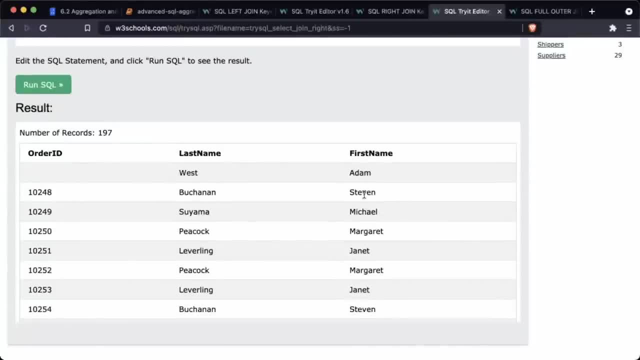 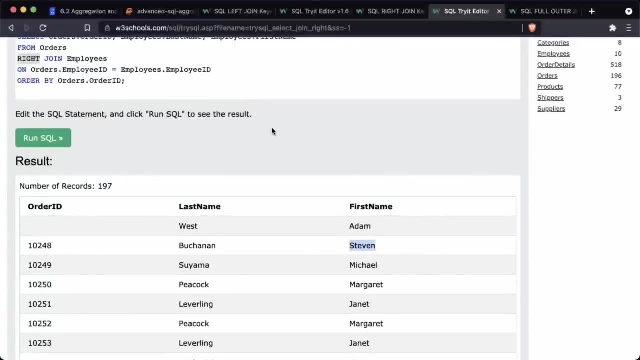 So we, for every order ID we get the last name and first name of an employee, But of course there are certain employees who may not have been assigned any orders. Maybe certain employees just don't deal with orders. They are into their managed people. 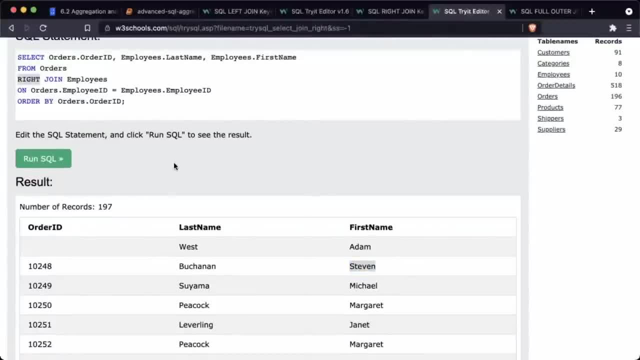 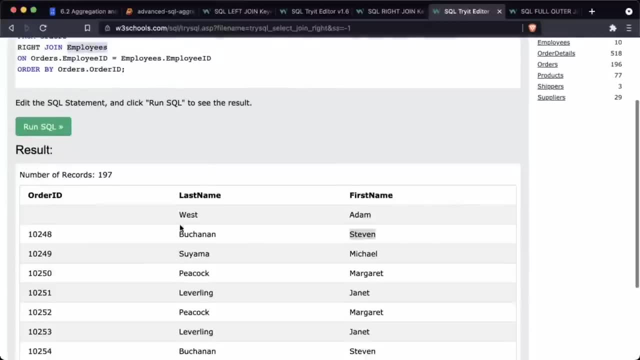 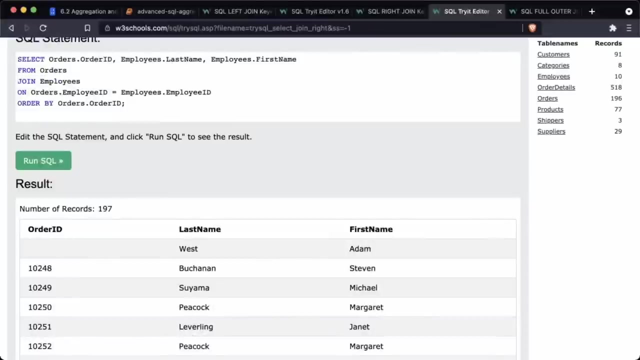 Because we have done a right join. we are telling SQL that you don't want to miss any rows from the right table, from the employees table, So you want to show employees even if they do not have any matching order columns. So now West Adam West does not have any orders, but we're still showing it here, which is showing a empty or null value here instead. of course, if we did not have joint right join here, then you can see. 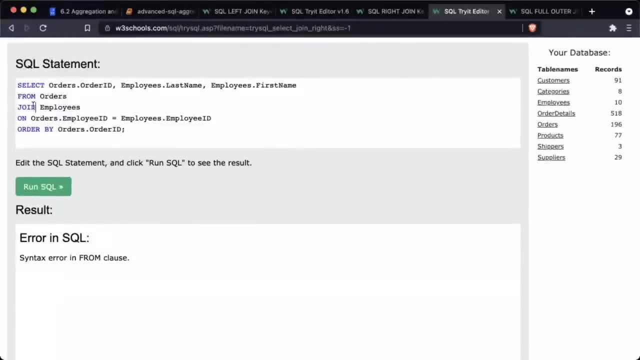 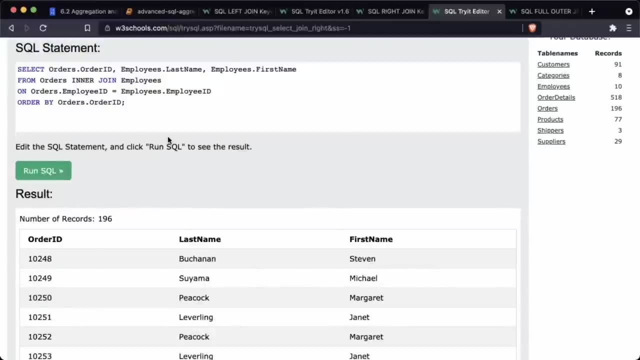 Okay, So we have done a right join. We are telling SQL that you don't want to miss any rows from the right table. single Save inner. Okay, Let's just do a inner join here. Yeah, If we just did an inner joint, which means we did not do a right joint. 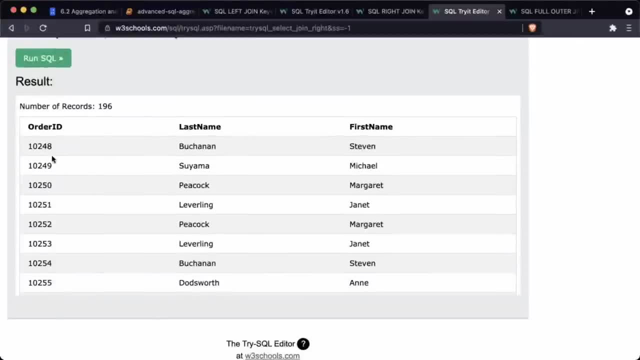 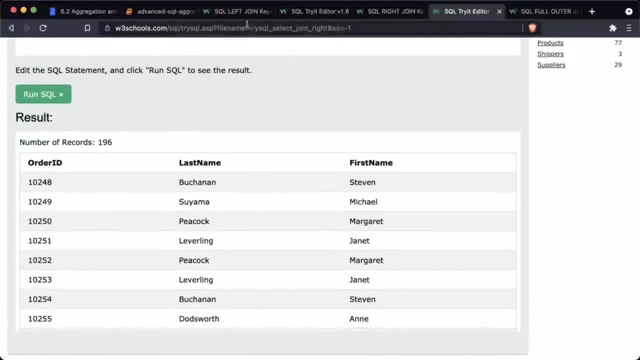 If we just did an inner joint here, then we would only get those employee names who have valid orders, right. So just try to remember this picture right, Where inner join means Okay the row must that, that value must exist in both columns, in both tables. 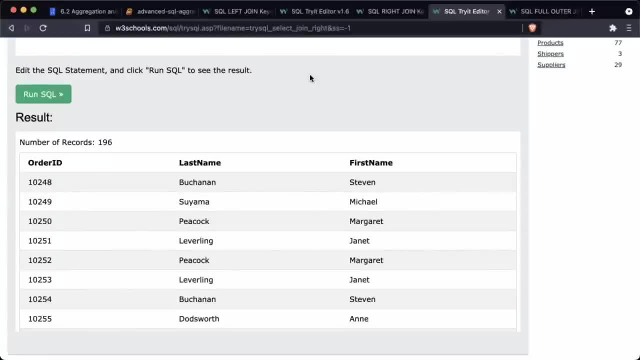 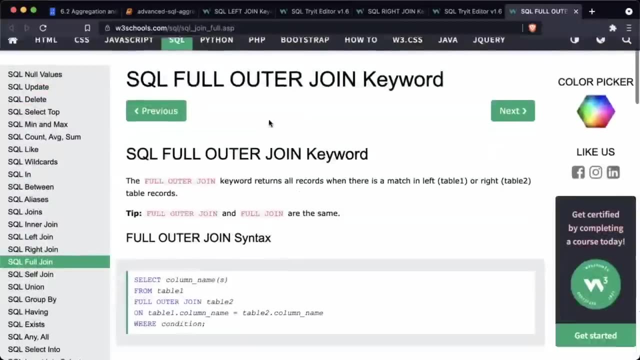 Left join means that all the values that exist in the left table show up. right Join means all the values that exist in the right table show up. and outer join- a full outer join- tells you that you want to maintain all the rows from the left left table. 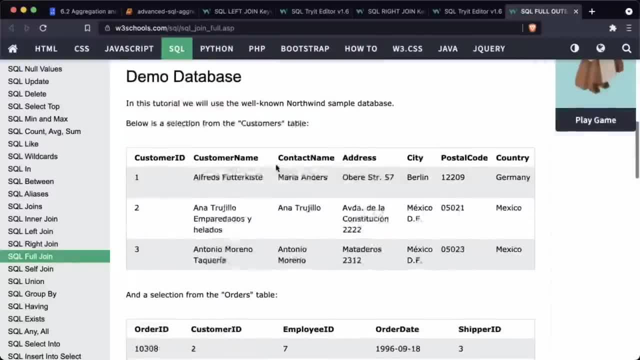 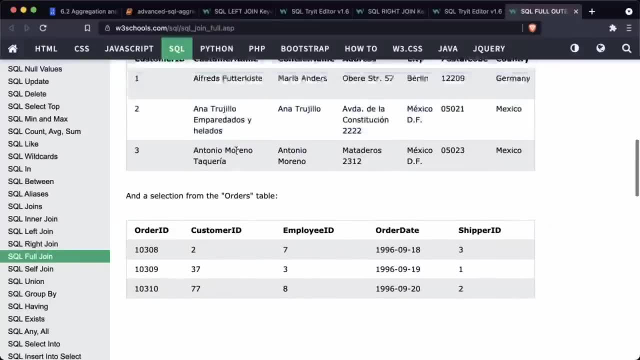 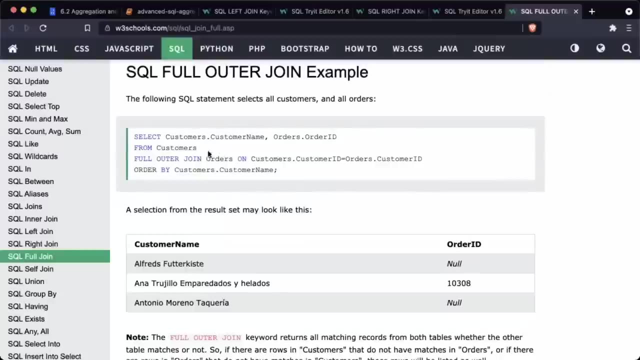 You want to maintain all the rows from the right table as well And you want to fill in nulls wherever possible. So here's an example: We have a customer stable and then we have an order stable and I believe you're doing a full outer join on customers and orders. 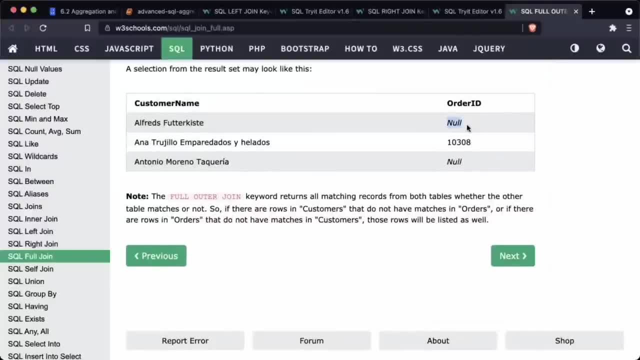 And this time you will see that there are certain order ID table, certain order IDs that may be null, and sometimes a certain customer name may be null, right, So that's how an outer join works. So just keep this picture in mind: this one outer join means you want to retain. 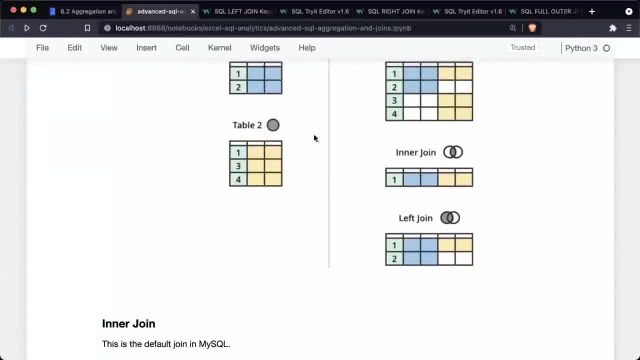 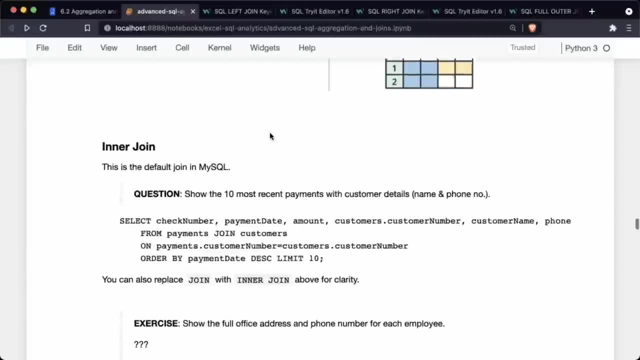 all the values. inner join means you want to retain just the intersection of the common values. left join means you want to retain all the values from the left table. right: Join me as you want to retain all the values from the right table. Okay. 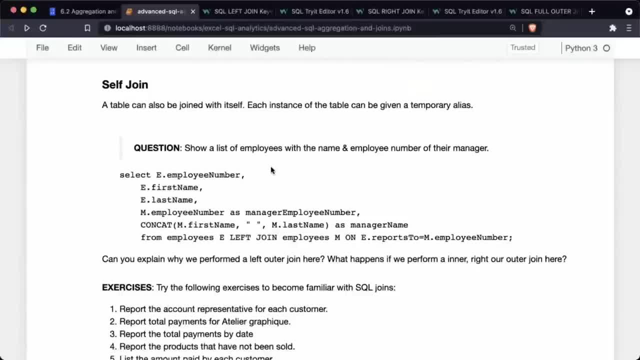 And one last thing: a table can also be joined with itself. You don't have to do a join between multiple tables and each instance of the table can be given a temporary alias. So you need to rename those tables because otherwise, if you're just joining a table, 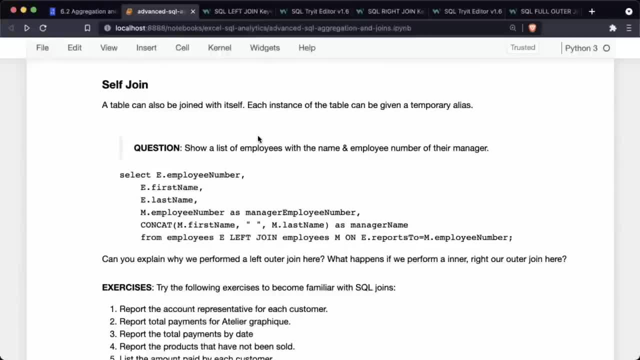 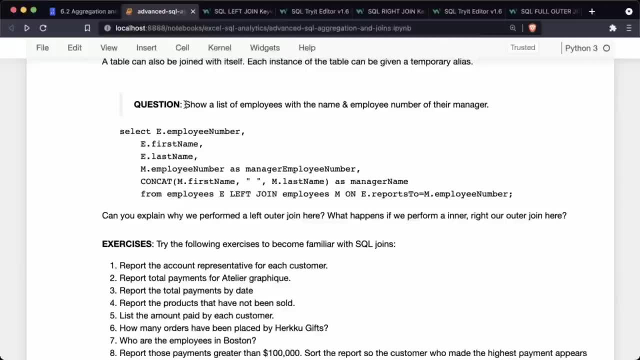 with itself. it may get confusing When you're explaining which columns to join on. So here's an example. remember employees. employees have this reports to field which reflect refers to another employee. So let's say we want to show a list of employees with the name. 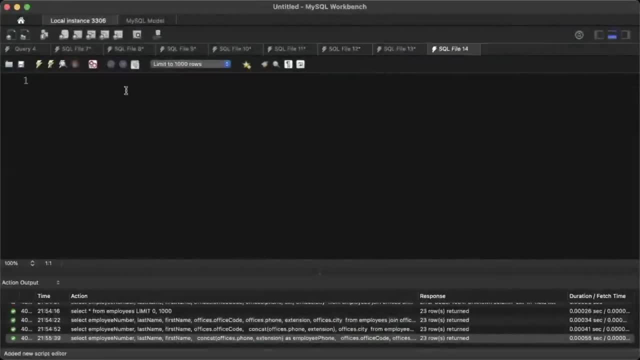 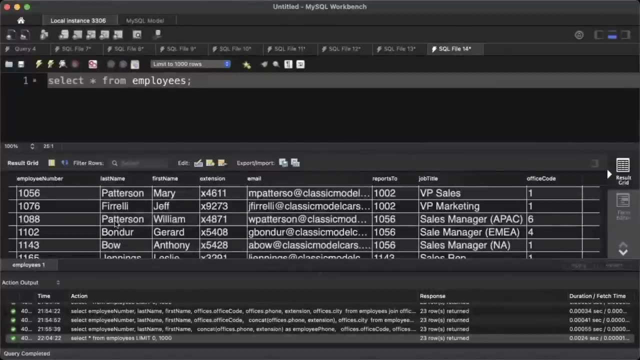 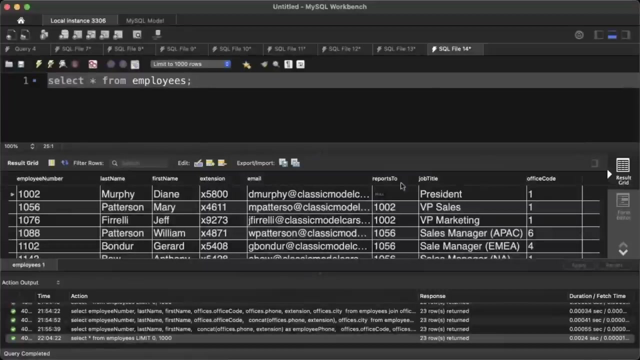 and employee number of their manager. So let's do select star from employees, Okay, So now we have all this information. We have employee number: I'm a employee, Okay, Okay. Okay. Last name, employee first name and then a bunch of information. 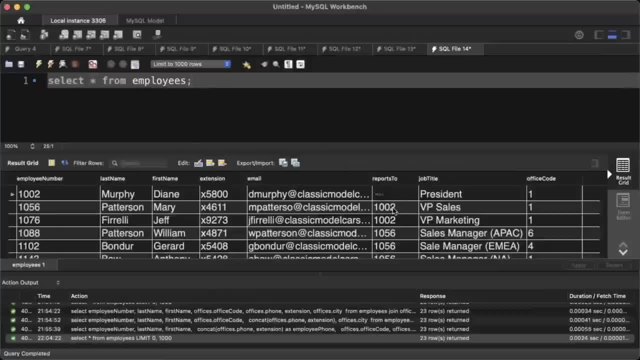 And then we have this thing called reports too. So every employee on most employees, except the president, I believe most employees report to another employee. So now, if you want to show who they report to, we want to get information about who they report to. what do we do? 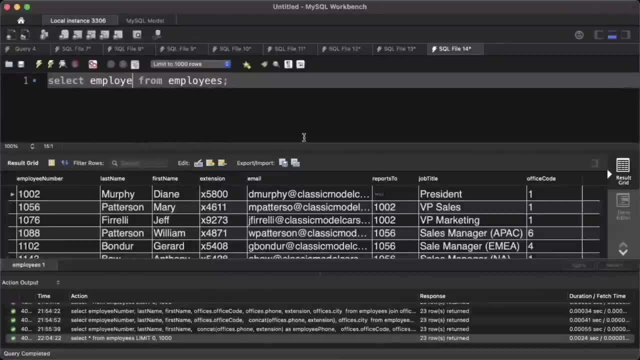 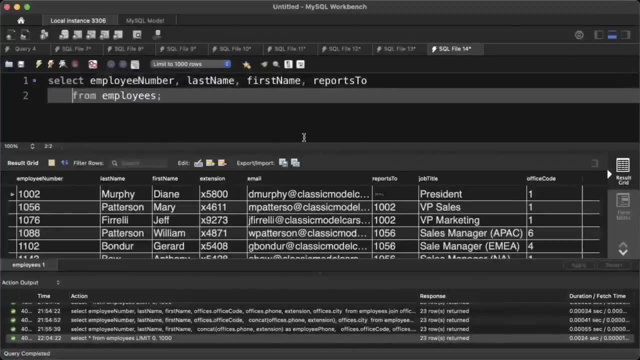 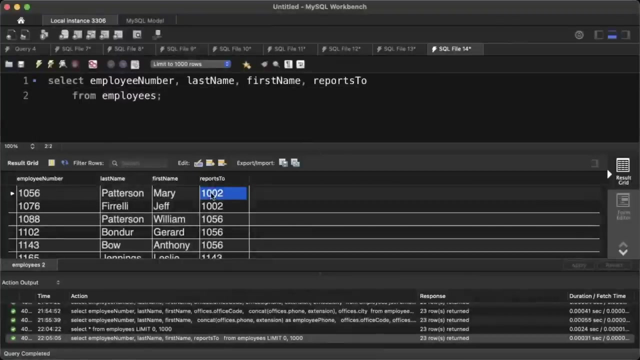 Well, first let me just simplify this output a little bit. Let me just put in employee number and let me put in last name and first name And reports too, so that we just have this information that we really need. Okay, Now I want to take the reports to number and get information from the employee table and insert that information here as new rows. 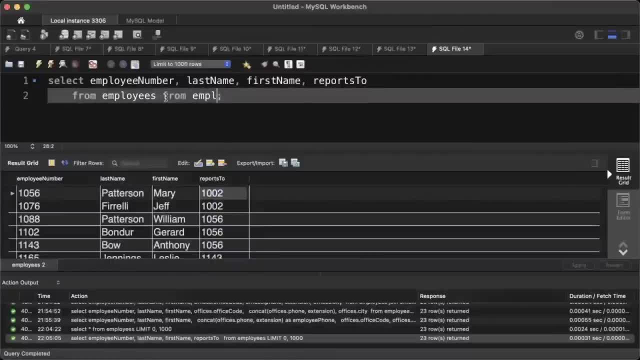 So we say from: employees join employees, but of course- and this is an inner joint, of course by default. So first let's do an inner joint and then we'll see if this needs to be a different joint. So we say: employees join employees, and now this can get confusing because you, both of these are called employees. 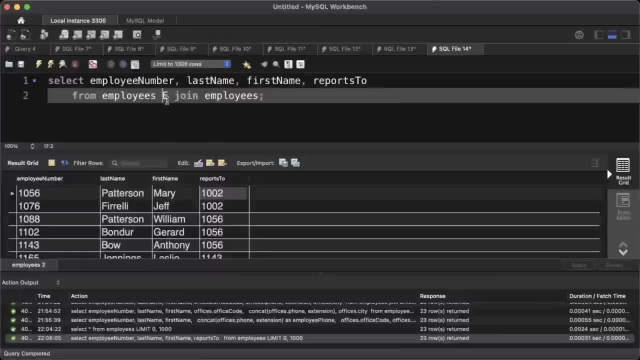 So let's call call one of these E, so you just give a space and then type a temporary name You don't put as here, you just put a space and let's call this M. so E for employees and M for manager, Okay. 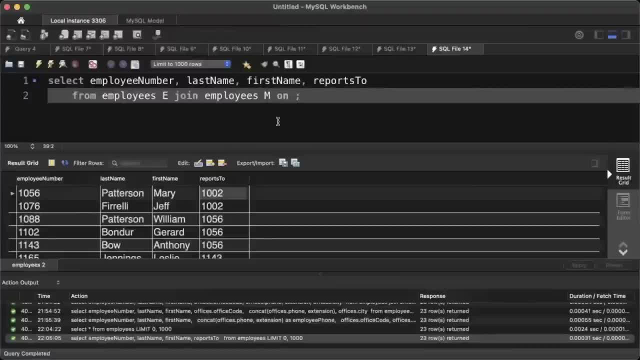 So now we are joining, and How are we joining? We want to join. now. This gets interesting here from E, from the first, from the left table, we want to look at reports too. And from the right table M, we want to look at the employee number. 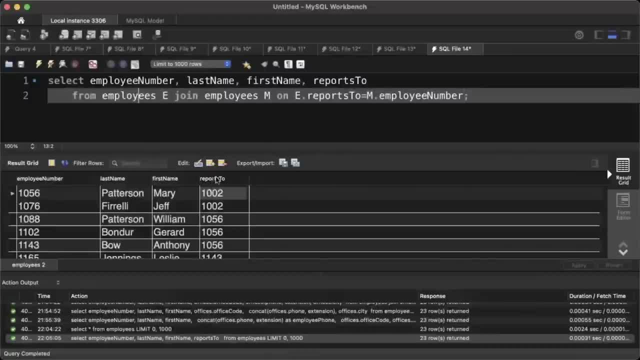 Okay, So from the employees table we want to take the reports to information and we want to find The Core Corresponding column where the employee number matches this reports to number. Okay, So think of employees and managers as different tables. 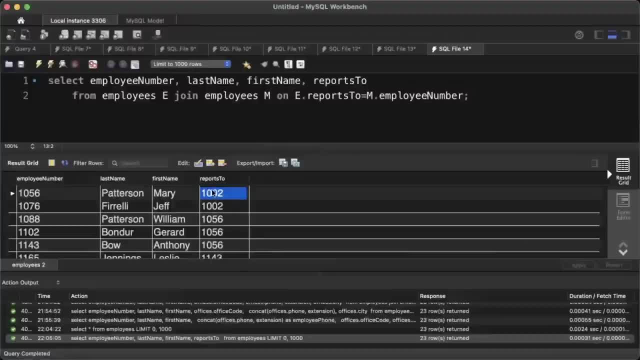 They are the same table, but think of them conceptually as different tables. We capture this number and we get that information from the M table, So that's why we have reports to equals employee number and let's grab some information here from the other side as well. 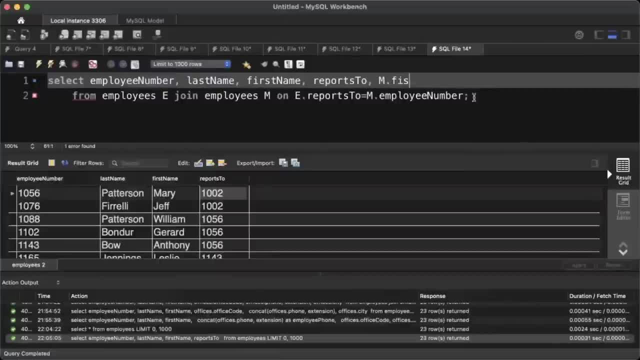 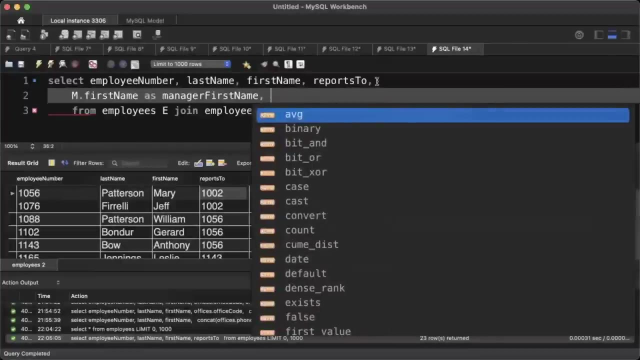 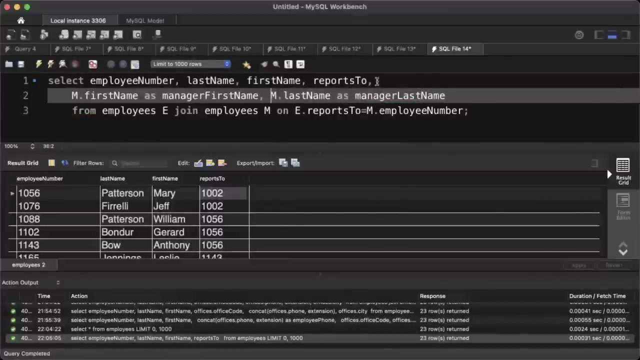 So from M let's grab the first name, Okay, And let's just call that manager first name. and from M let us grab the last name as well: M dot, last name, and let's call that manager last name. and from M let's also grab the employee number. 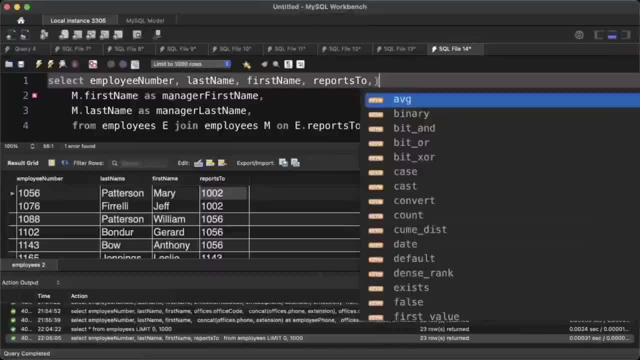 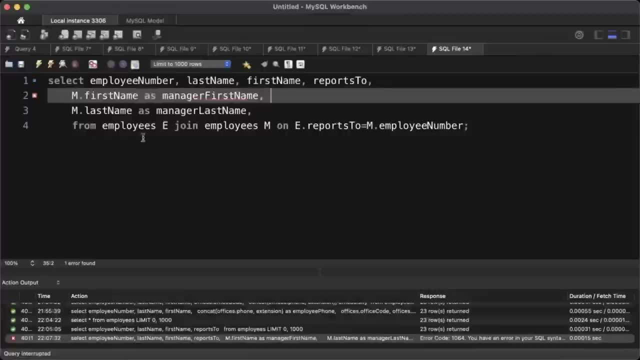 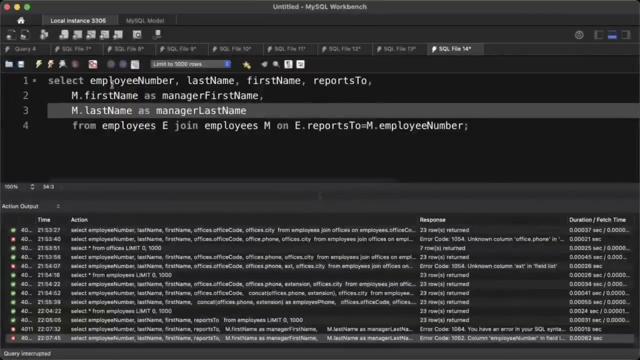 Well, actually we have that already. We have reports too, Okay, Okay, We have reports too. So that's that, there we go. So we have select employee number, first name reports too, And we want to select. okay, Now, reports too. 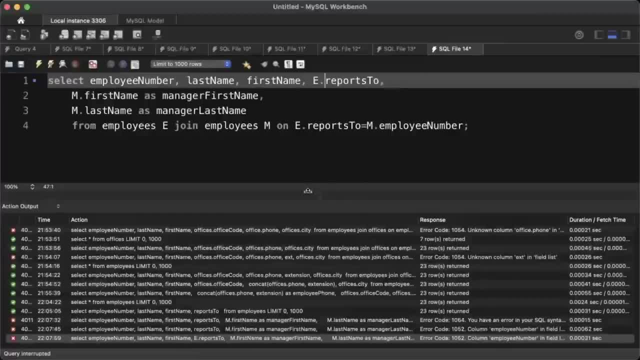 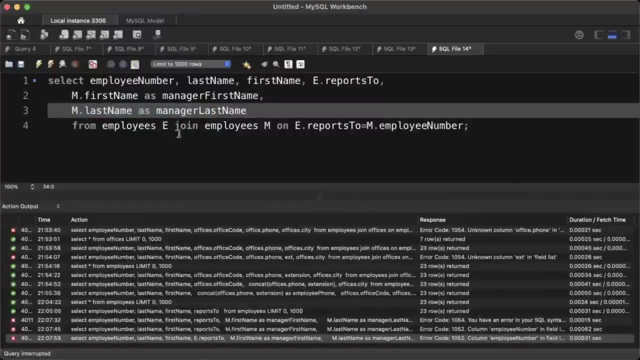 Let's just put in M dot, because this is going to get confusing otherwise for SQL and you want to select M dot first name and we want to select M dot last name as manager, last name from the employee's table. I think I may have a typo here. 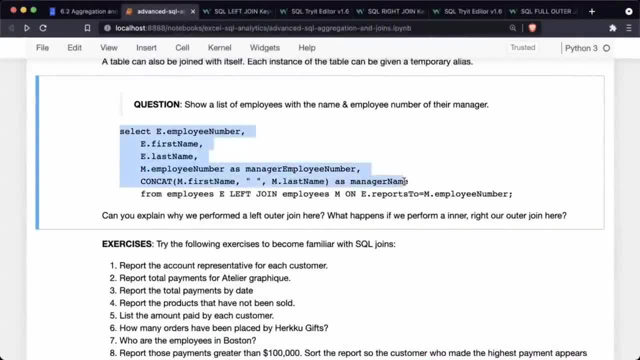 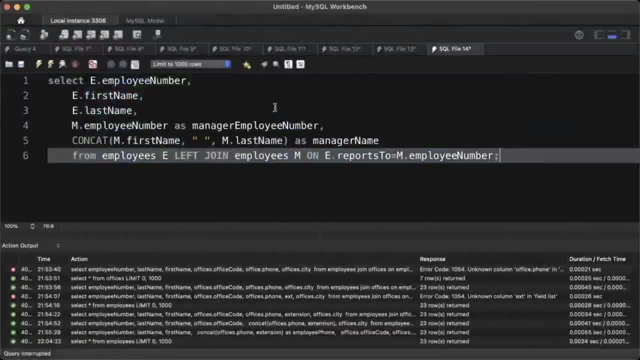 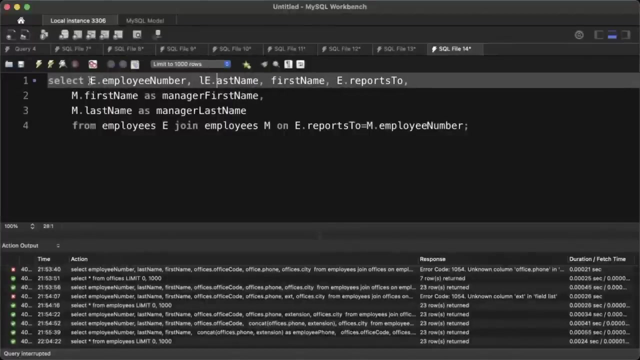 Let me just grab this. Okay, I think I may have a typo here, so I'm just going to fix this right now. But yeah, so we have E dot employee number and we have E dot first name, and we have. I see what the issue was, because we have all these columns in each of the tables. 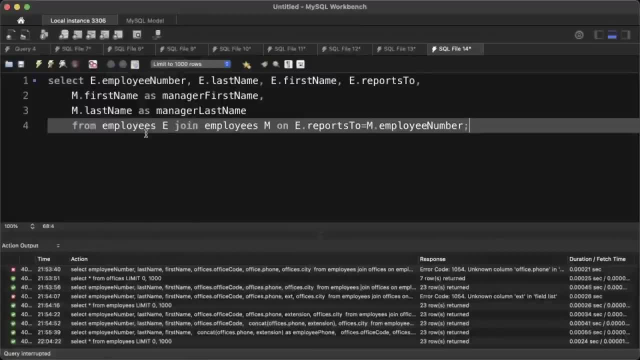 So we just need to add E dot. So we say we have an employee stable joined with the employee stable. One is called E, one is called M, So we have E dot employee number. E dot last name. E dot first name. reports to M dot first name. M dot last name. 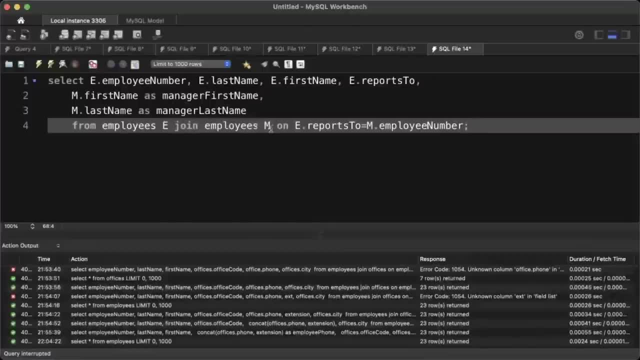 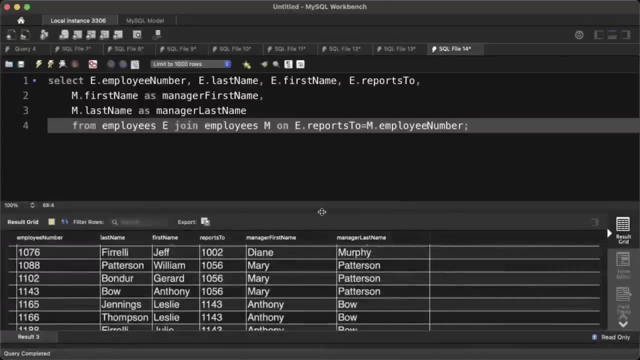 From employees join employees on the reports to column, joined with the employee number, column. Okay, So this is probably the most confusing part of it all. So now for every single employee who has a manager, because this is an inner joint, remember. 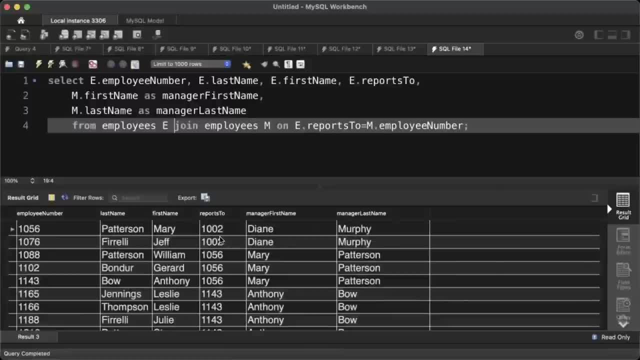 So for every single employee who has a manager, we get their employee, we get their manager information as well, So we get the name and last name of their manager. Maybe we can concatenate this, So let's maybe just do Concat M dot first name and M dot last name as manager name. 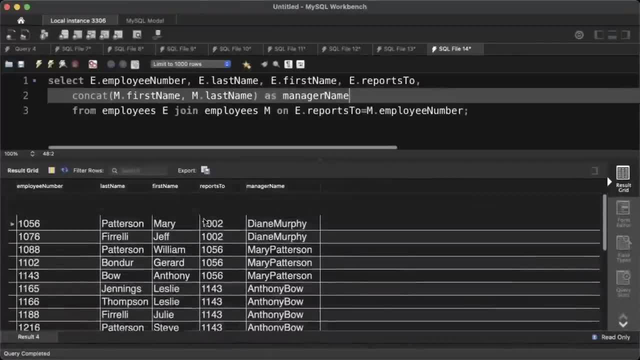 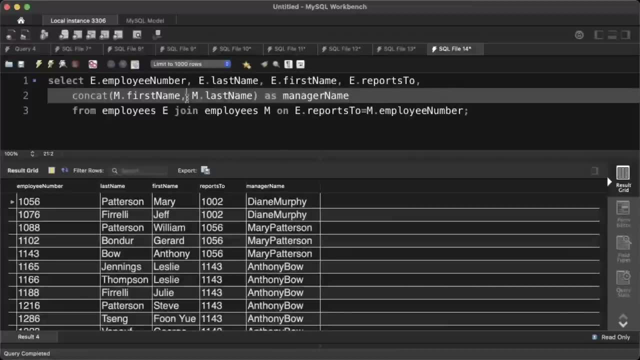 So now we have this information about each employee: They we have their last name, first name, employee number, and then we have the employee number they report to and we have the name of the their manager. Let's just add a space here as well. 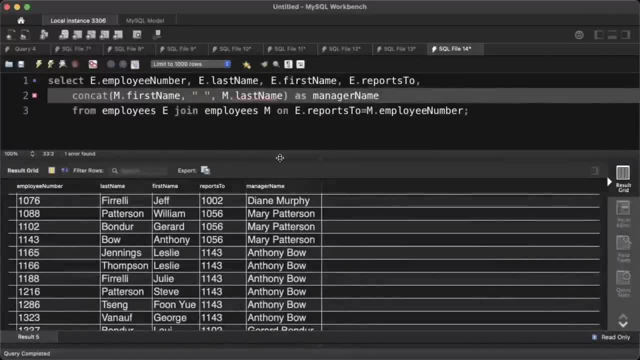 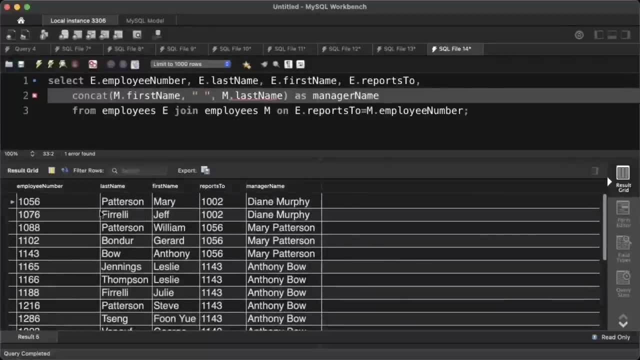 Okay Now, one last thing here that We Would want to just cover is there is a certain employee, the president, who does not report to anyone, And we have not shown that information here because we are doing an inner joint, So because the president, Diane Murphy, does not report to anybody. 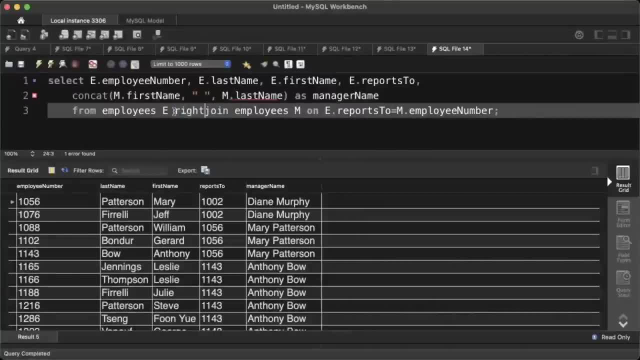 So that row gets skipped. but instead, if we do a right- sorry, if we do a left- joint, what we're telling SQL is: we want to maintain the list of all the Employees from the left table E, even if they do not have a person that they report to. 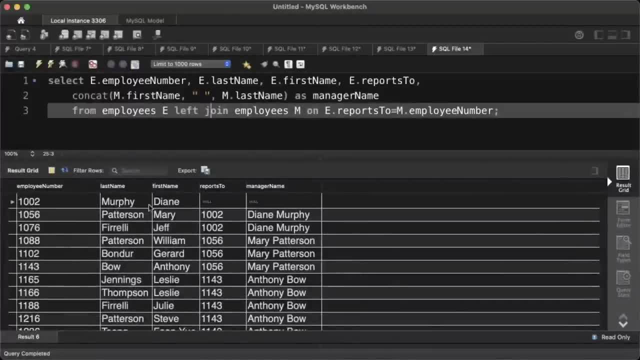 So now, if you check, you have an employee number 1, 0, 0, 2, Murphy Diane, and for them reports to his null, And of course null value doesn't show up in the other table, So their manager name is also null. 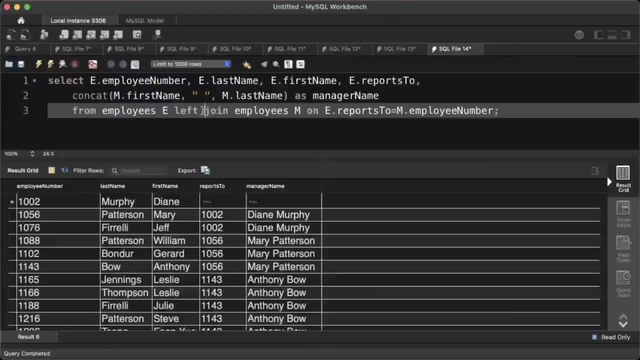 Okay, So now you see that this is supposed to be a left joint. and why this is supposed to be a left turn left join and not an inner joint? because you want to show all The employee numbers even if they don't have a manager. now suppose, instead of a left joint, you had done a right joint. 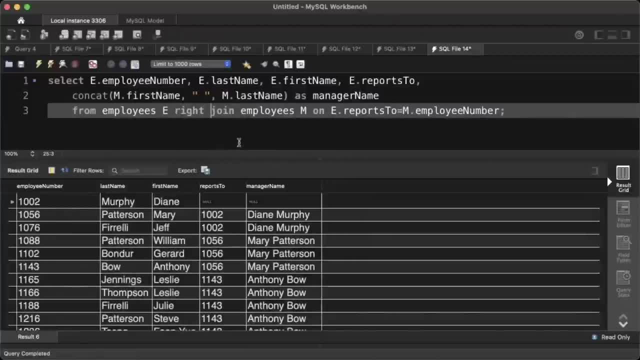 What would happen now? So now we're telling SQL that only show me employees from the left table who have a manager, but on the other side, on the right side, if there are certain employees In the M table which do not feature in the reports, to call. 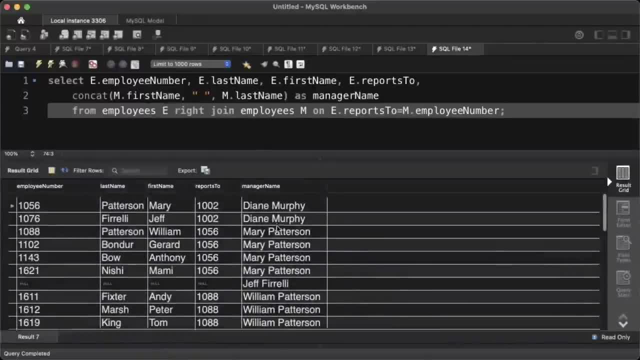 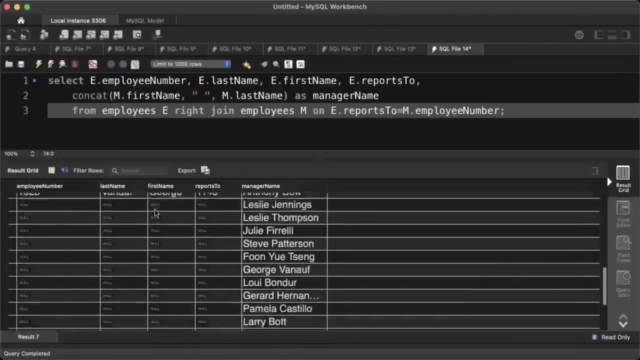 You should still show them. So let me run that and let me show you the result. So it seems like the result hasn't changed. So one thing that has happened is Diane Murphy has gone away, but if I scroll down here, you will see that now I have Leslie Jennings, Leslie Thompson, Julie, 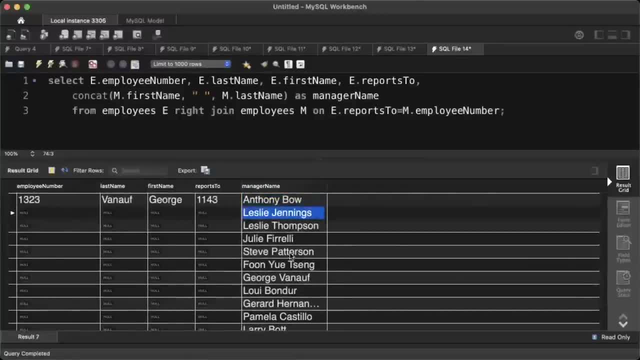 for Ellie, all these people who do not have any reportees still show up. This is because we are doing the right journey. We are saying that every row from the M table should be represented, even if they don't have any matching information in the E table. 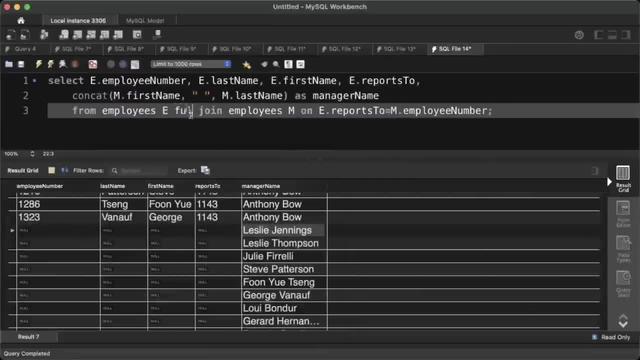 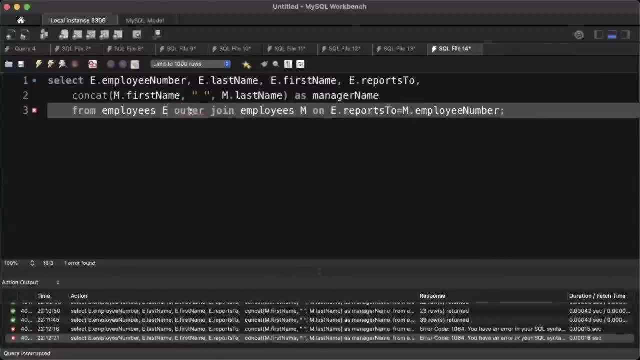 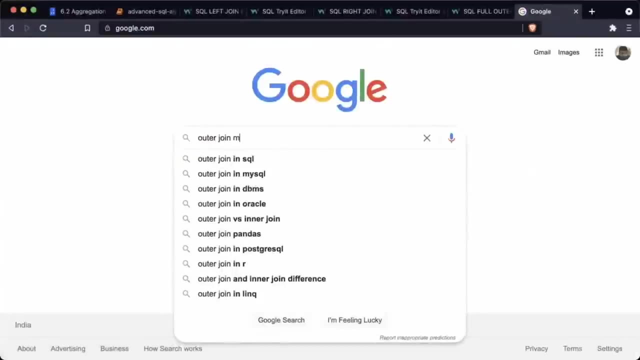 So that's So. that's the issue with the right joint. And if we did a full outer joint or I think it's just called an outer joint, okay, I'm not sure what the outer join in my sequel is. I guess it's just called full outer joint. 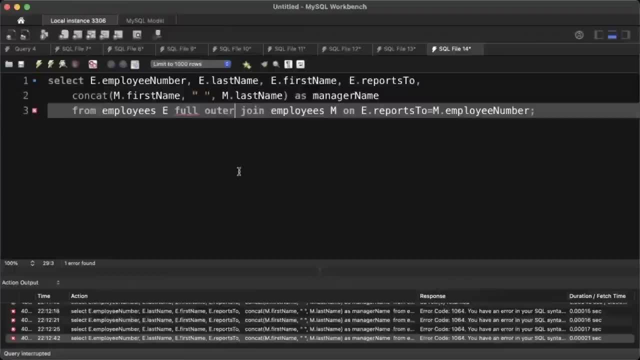 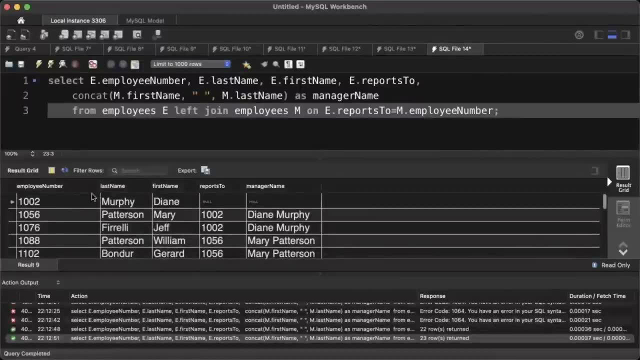 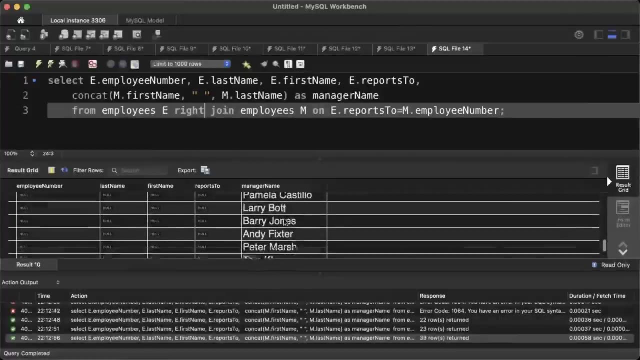 I think I'll have to look it up, but if we did the full outer joint, then we would see this, we would see Diane Murphy and we would also see all this information: Pamela Castillo, Larry bolt et Cetera. 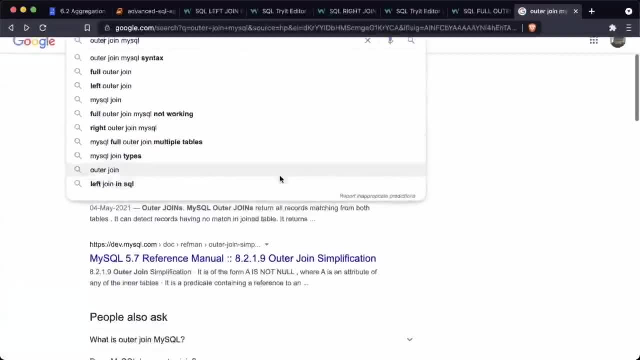 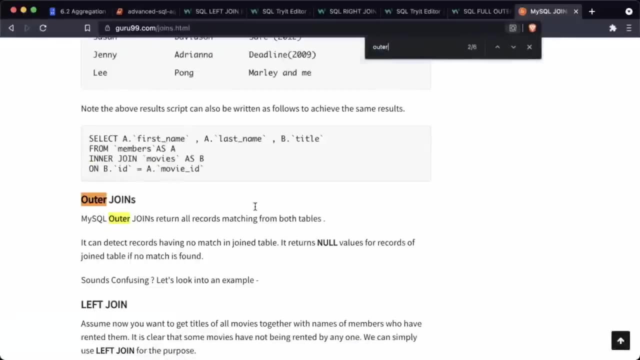 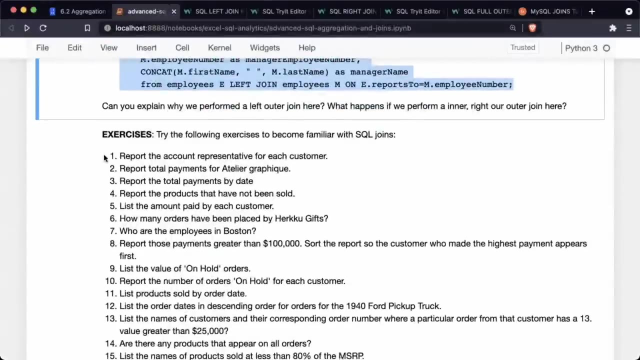 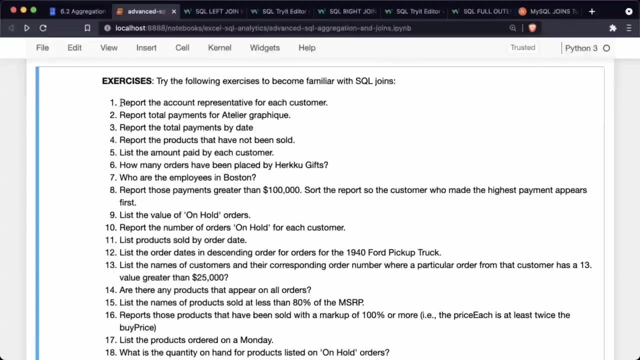 Okay, We'll check this out. What: how do you create a outer join in? Okay, We'll check this out. What In my sequel? Okay, Nevermind. So that's joints, And here are some exercises for you to try out to become familiar with SQL. joins: the report: the account representative for each customer: uh, report the total payments for the atelier graphic. 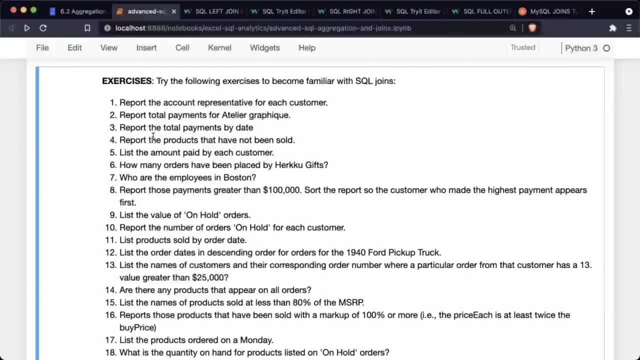 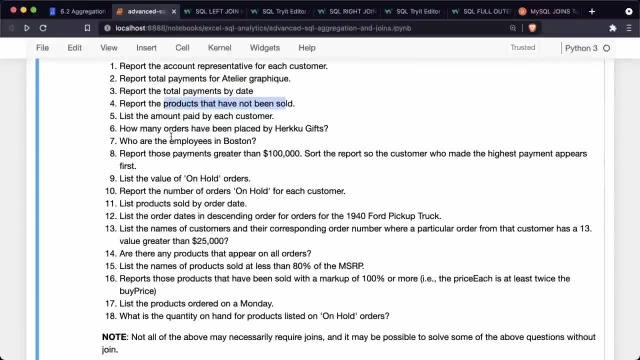 This is one of the- uh, I think this is one of the customers. Okay, Report the total payments by date. report the products that have not been sold ever, list the amount paid by each customer, and so on. So each of these will require a certain joint. 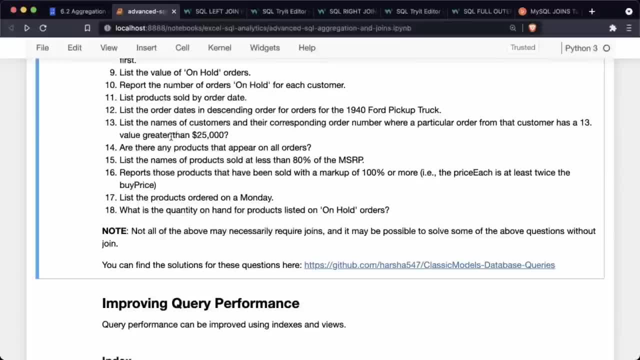 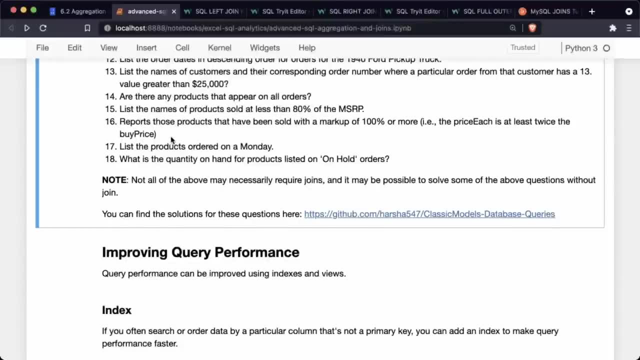 Not all of them may require joints, And for some of these it's possible that you can do them without joints. In some cases, you will also have to do some other things, like arithmetic operations, et Cetera. For example, list the names of products sold at less than 80% of the MSRP. 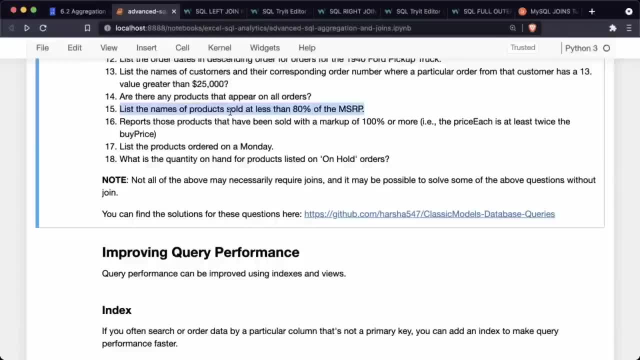 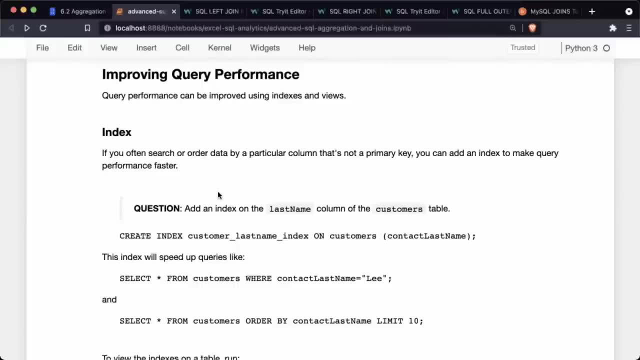 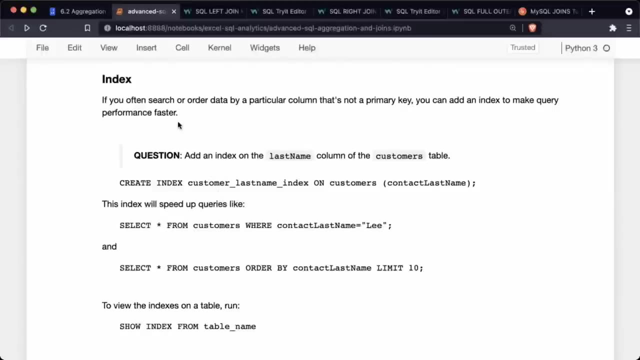 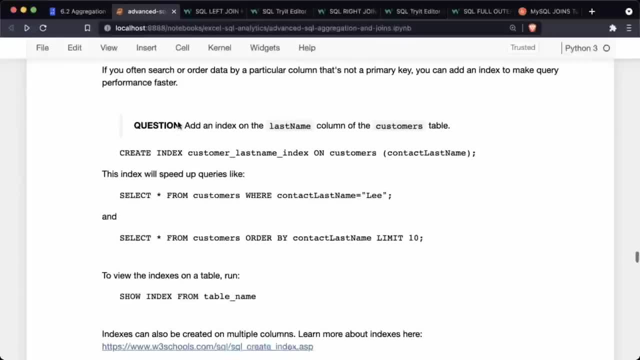 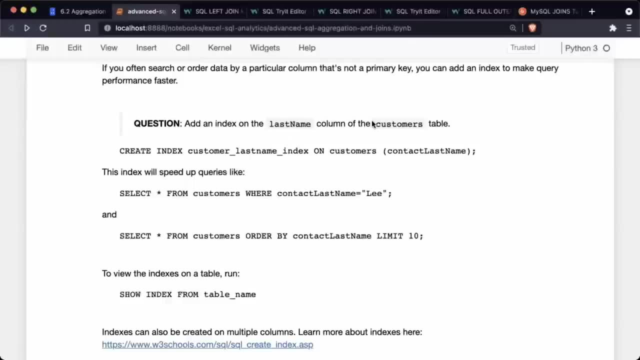 Then you can add an index to make the query performance faster. For example, if you search by customer's last name a lot or if you order by customer's last name a lot, then you should do this. You should run this command: create index customer last name and give it whatever name. 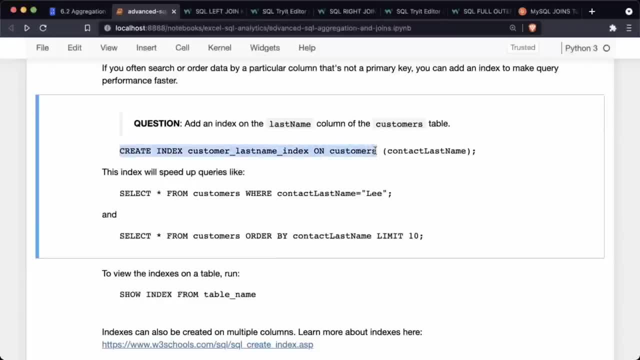 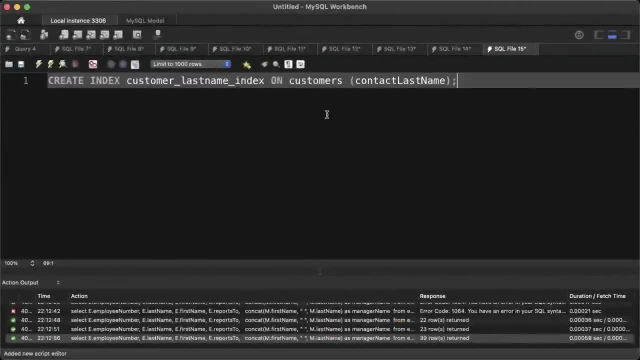 you want. So you say create index so-and-so on the table customers using the column contact last name. So if we do this, if we just run create index customer last name index on customers, what we're telling SQL is that we want SQL to track the contact last name information, the contact. 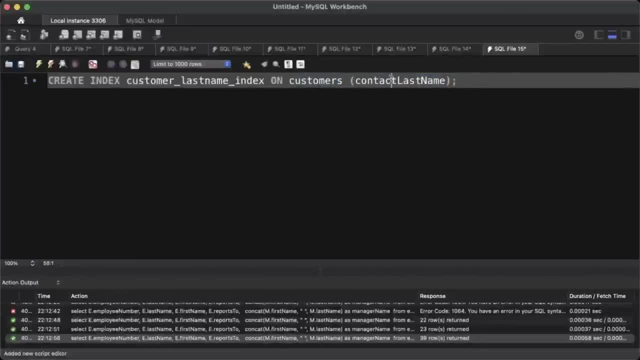 last name column In the customer's table and set up a way for us to efficiently do queries on that column. So what does this mean? Well, the next time we do a query on the last name, let's say we do something like this: 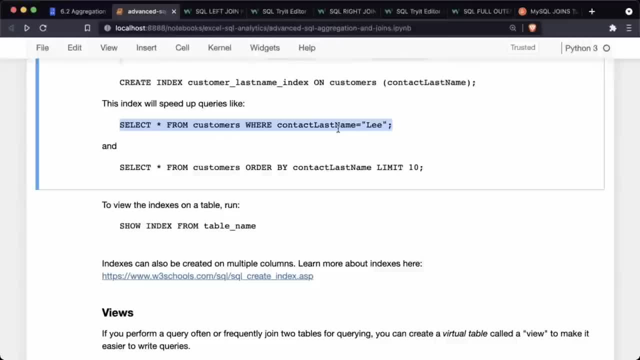 select star from customers where contact last name equals Lee, because contact last name has an index, This query will be very fast. If the contact last name did not have an index, then this query would be fairly slow And the difference would be. 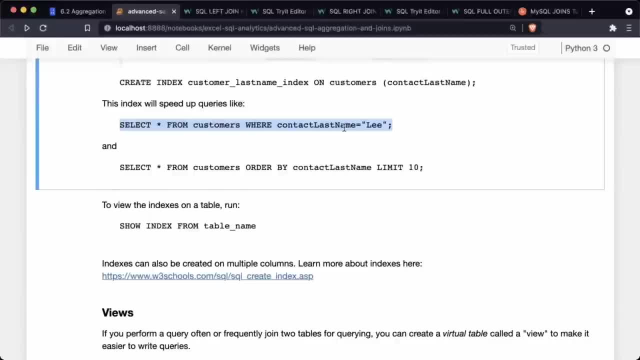 Um, If the contact last name did not have an index, then SQL would have to search through all the rules. But if the contact last name does have an index, then SQL can actually avoid searching because it has set up some ways to, uh, efficiently track information and search information from. 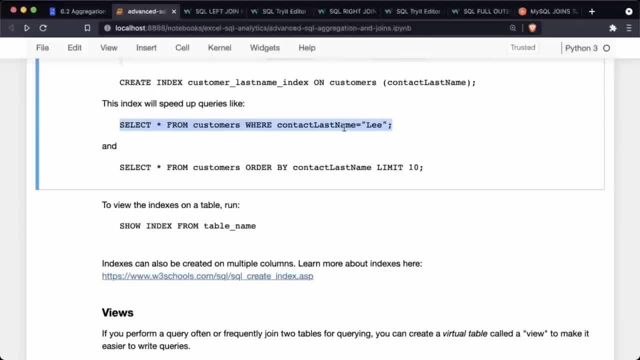 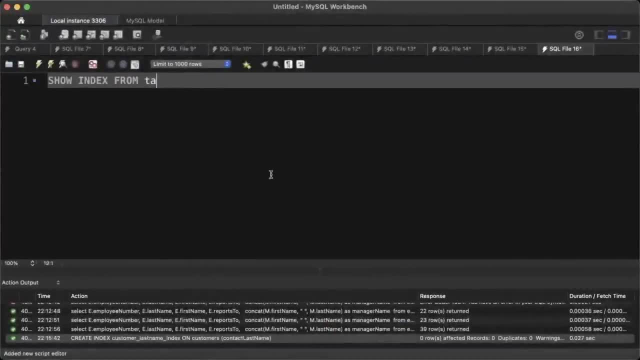 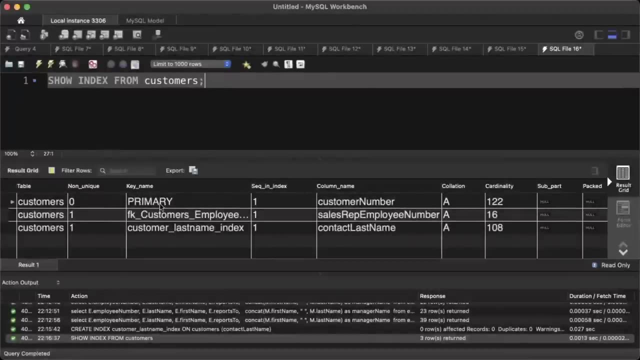 the contact last name column. In fact, it is using a data structure called a B tree and you can see what kind of index is created or what kind of indexes you have on a table simply by typing. So you can see that we have a primary key which is tracked using an index, because typically 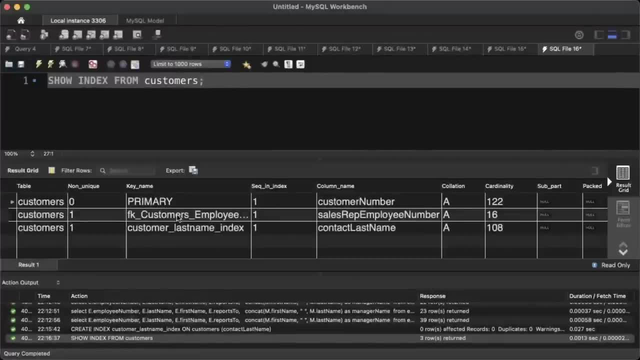 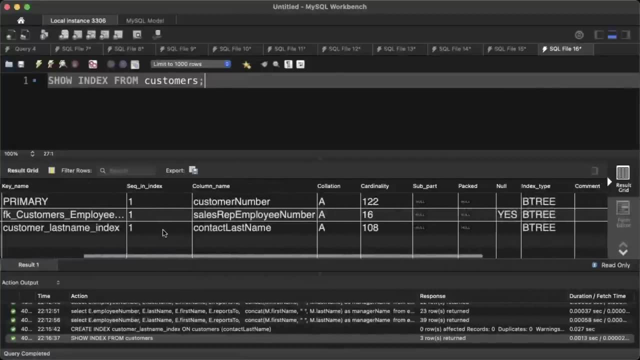 you extract information using finite primary key. We have a foreign key, So every foreign key also creates an index. but then we also have this customer last name index, which we just just created, And this index is represented as a B tree, which is a data structure and efficient data. 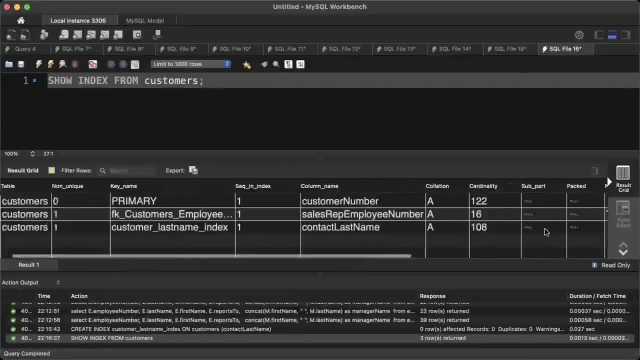 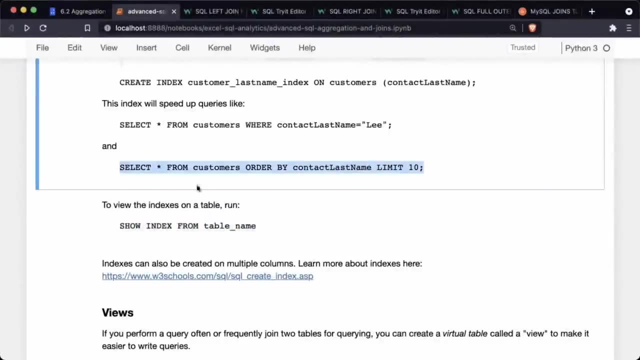 structure optimized for querying, So So whenever you query by last name, that is very efficient. not only querying, but ordering by last name is also efficient. So you could do something like this: select star from customers ordered by contact. last name limit 10.. 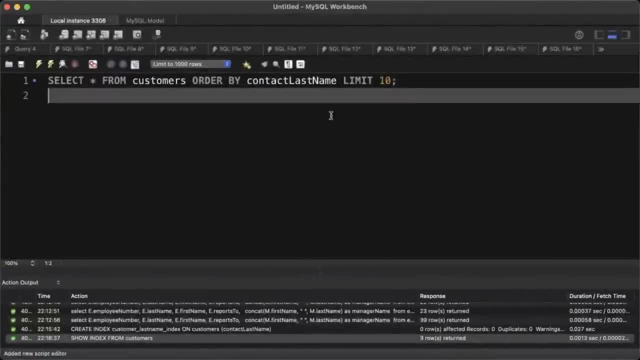 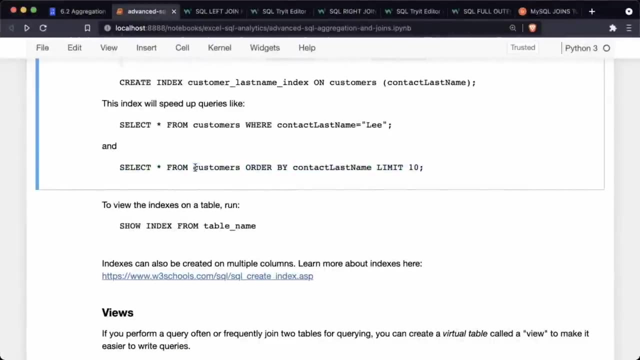 Again, if you have an index, this is going to be fairly efficient. If you don't have an index, it's going to be slow. It's not going to make a difference for this database that we are working with right now, But when you have a really large data set, a really large database with millions of rows, 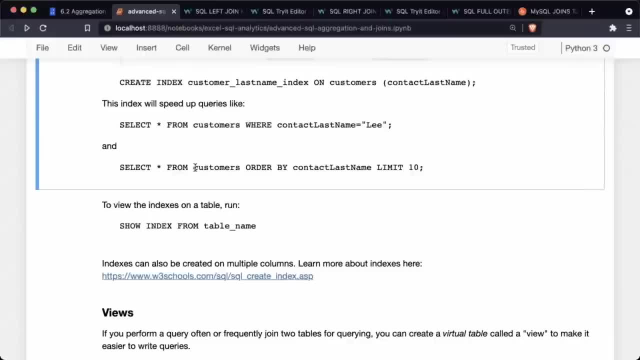 then this will start to make More sense. So if you are doing some queries and those queries seem to be taking a long time, maybe consider creating an index, or maybe consider asking the database administrator to create indexes on the columns that you are ordering by or searching by most frequently. 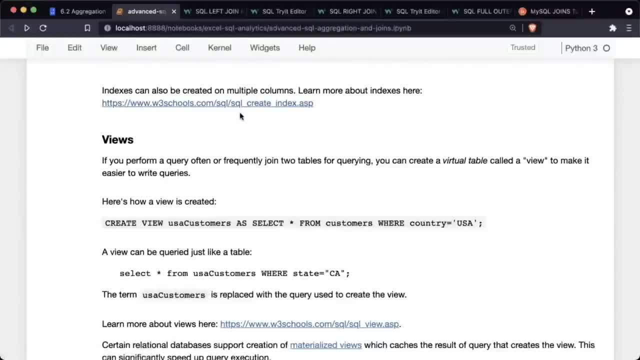 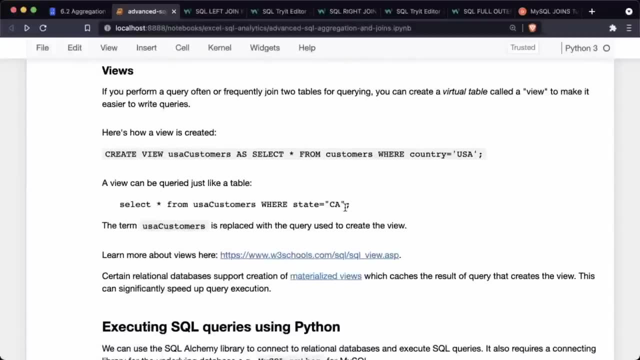 Okay, And indexes can also be created on multiple columns. If you put conditions on multiple columns frequently so you can check that out, Then another thing that you can do is create something called a view. So if you perform a query- Okay. 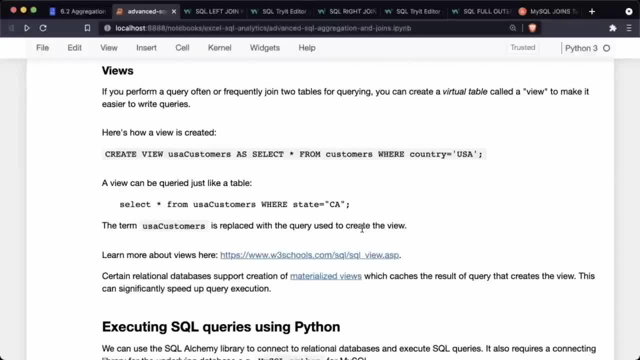 Or if you perform a query very often, or if you very frequently joined tables for querying, then you can create a virtual table out of that query And this virtual table is called a view. So here is how a view is created. So we'll see how views created and how it's used. 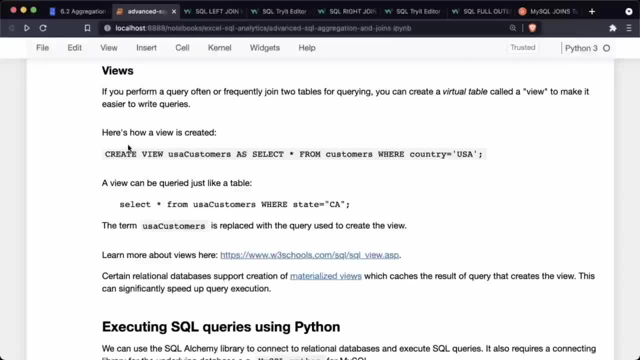 And then you probably see more, learn more about how it works. So to create a view, you say, create view USA customers, as you type the name of the view And you type as, and then you type a query like you normally do. 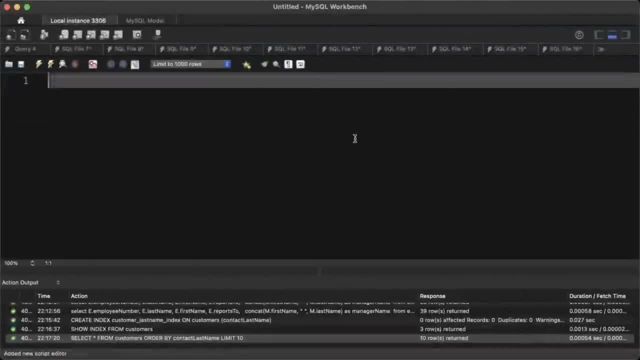 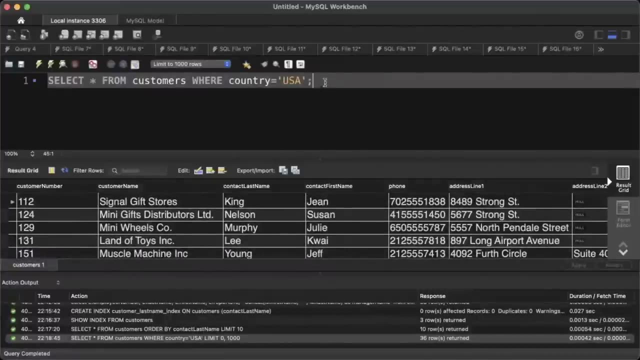 So, instead of doing, select star from customers where country equals USA, So this is all. this is the information about all the American customers. What we want to do is we want to take this query and we want to give it a name: USA customers. 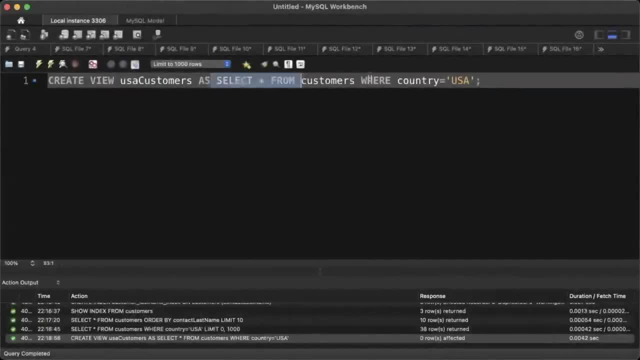 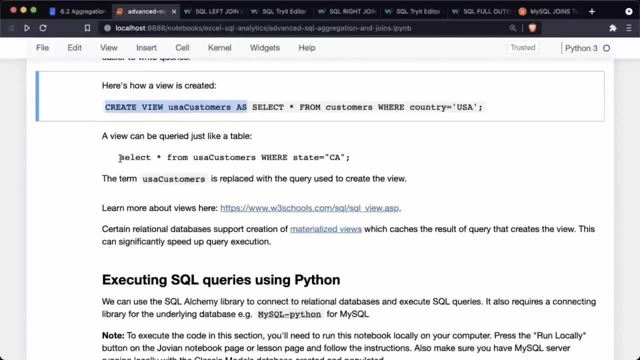 So let's say: let's say create view USA customers, and that is now going to represent this query. the word USA customers: How do we use it? We use it just like a normal table. Now let's say we want to get just the customers who are in California. 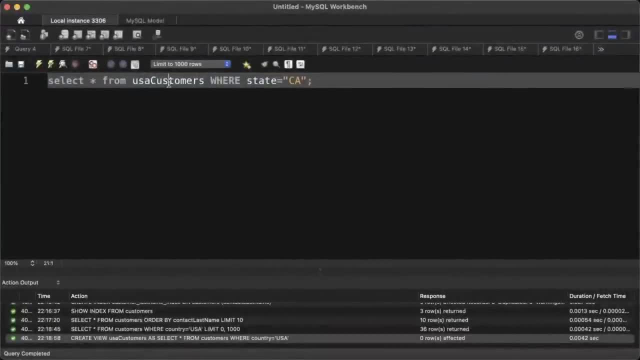 So we can do this: select star from USA customers. So now we refer to this view which we have created already. It's saved in the in the database that view. So select star from USA customers: customers who are from the USA where state equals CA. 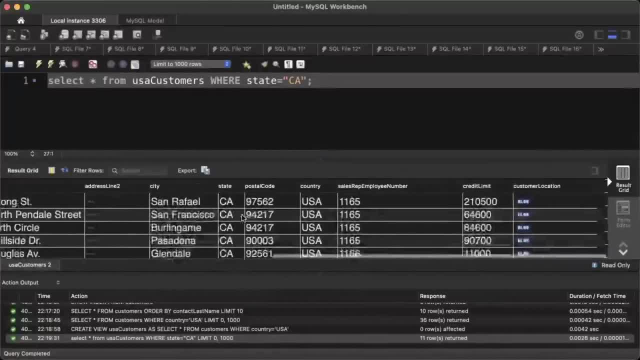 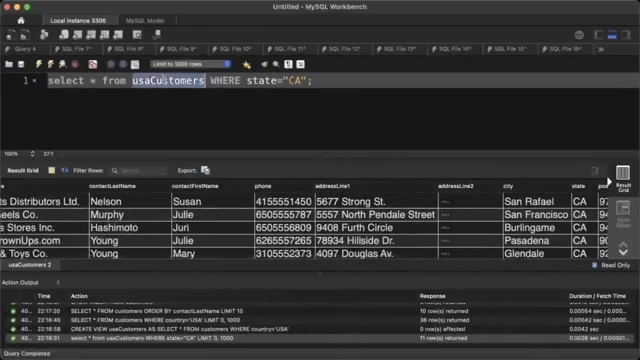 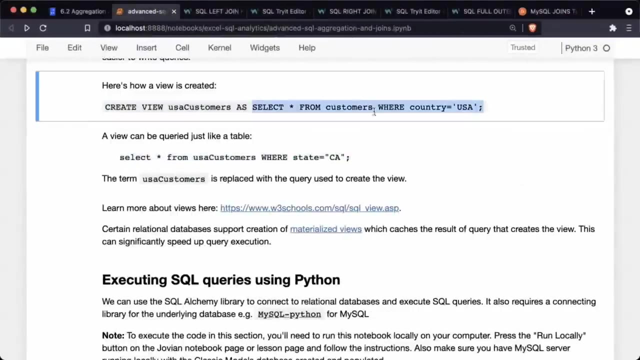 And when we run this, You can now see that we only have customers from USA. Of course, that's because this the state is a CA, but you can see that USA customers actually used information from this query that we had defined earlier. Okay, 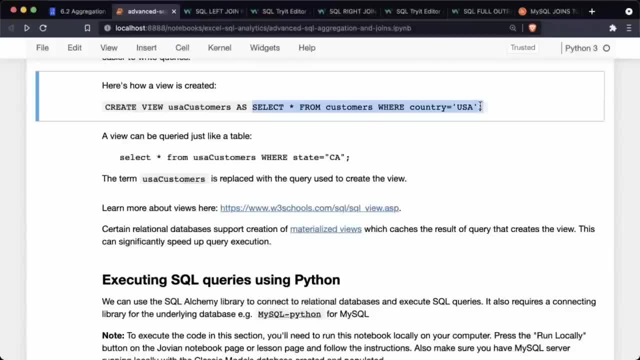 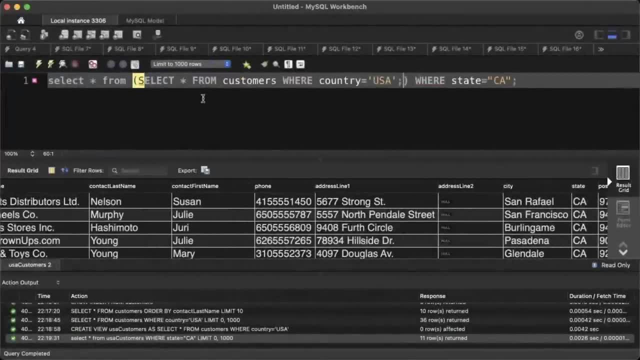 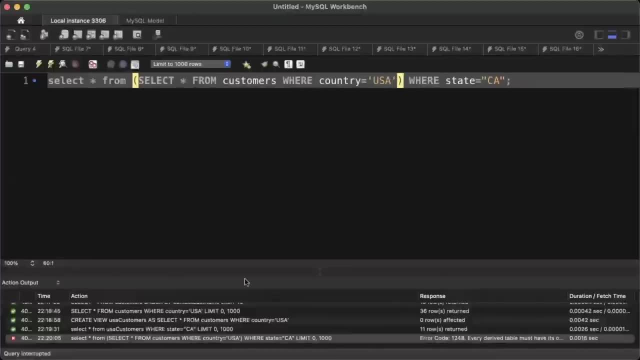 So, conceptually, what's happening is, wherever the SQL server sees USA customers, it's simply going to replace this with this select star from customers where country equals USA. Okay, And in fact you can also run this. Okay, This is not going to work directly, but, yeah, you need, once you create a view and use the 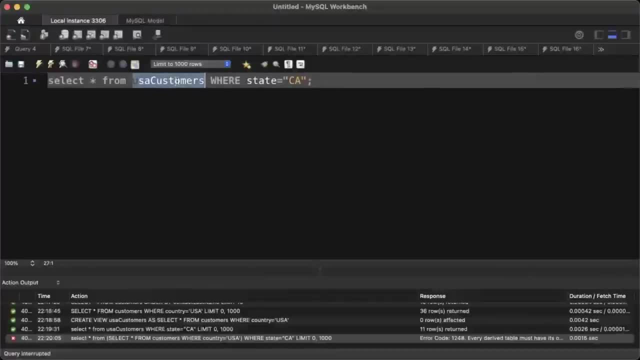 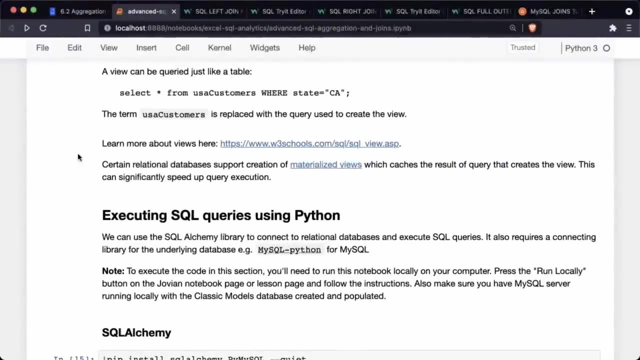 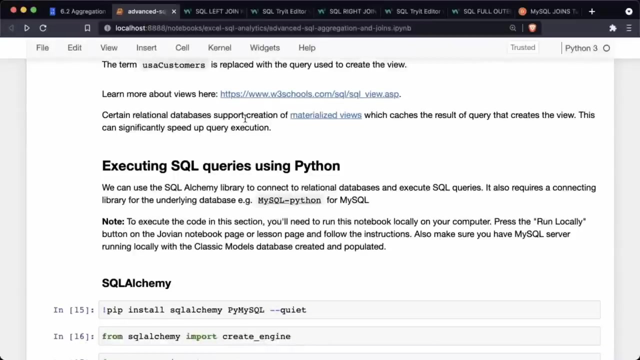 view. So SQL is going to replace the view name with the actual query that you have provided. Now, typically, when you create a view, no new data gets created. It's simply that information that is tracked, Which query The view represents. but certain relational databases also support creation of materialized 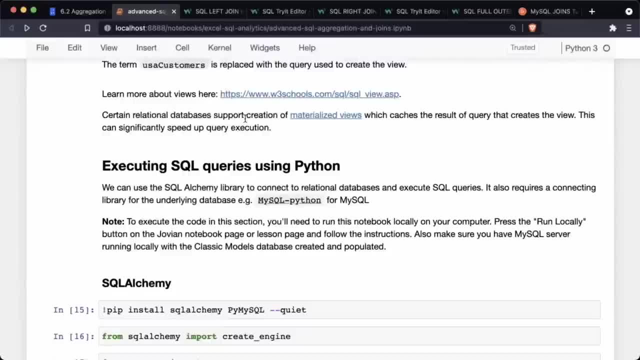 views. So let's say you're doing joins between certain tables very often and then you are getting information about that from that joined table, from that joined query. Then you can create a materialized view which is going to contain the joined version of. 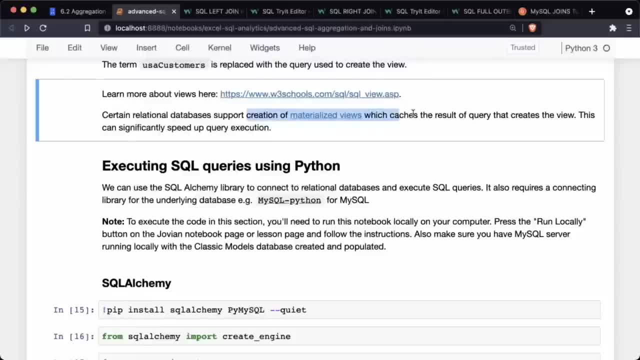 the two tables So that whenever any of those two tables is updated, the view gets recreated And that is Like a separate table that is always tracking the latest version of the joins of the two tables And that takes up more space but that makes it very efficient to query. 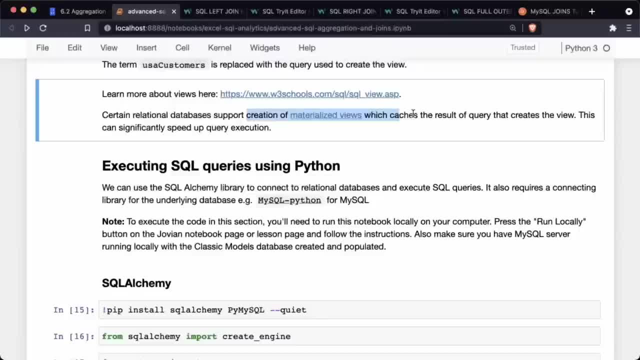 So now, whenever you make queries on that view, instead of rerunning the query that creates the view, it will have the view already as a table saved within the database and all that information will be cashed. So you can get that. You can get the result out of the view very easily. 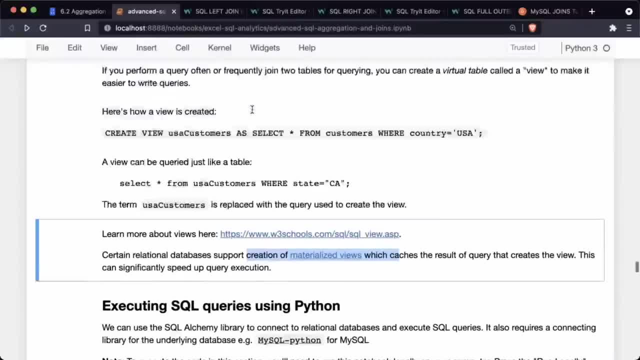 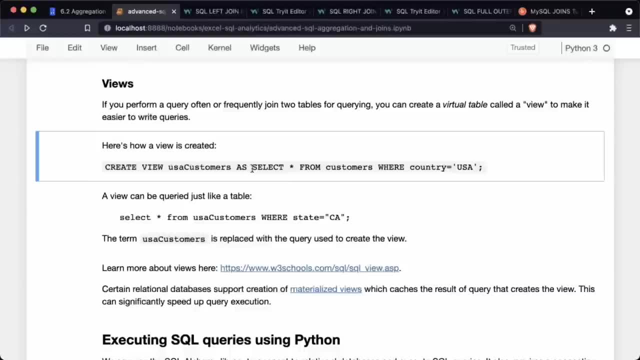 Okay, So now by default, we are not actually creating a table- USA customers. but if you make this a materialized view, then the database is actually going to set up this table called USA customers somewhere And that is going to be kept up to date with the list of customers from the USA. 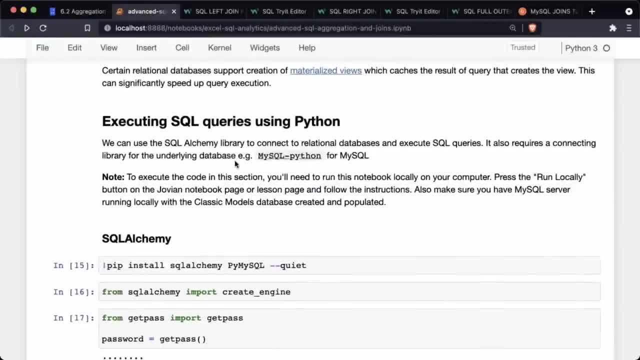 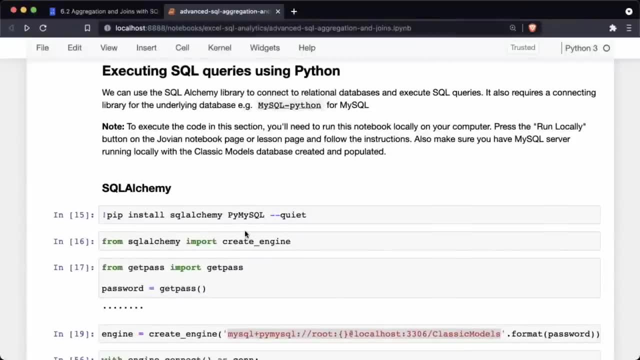 Okay, So that's materialized views, not something you'll have to worry about or work with often, but in case you come across the term, that's what it means. Okay, So let's talk about executing SQL queries using Python. One way we've seen how to execute SQL queries is using the MySQL command line interface. 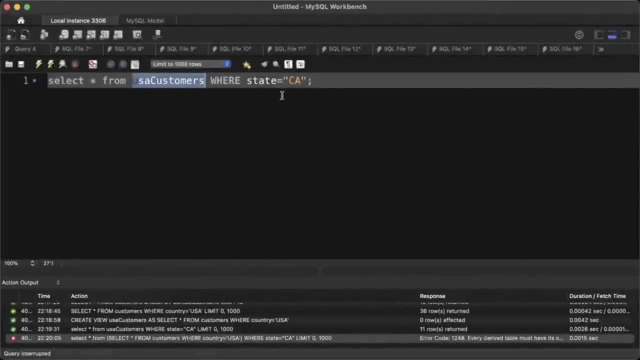 Another way we've seen how to execute SQL queries is using the MySQL workbench, And the common thread here is: all you need is to connect to your SQL server, your database server. That could be running locally. That could be running on the cloud. 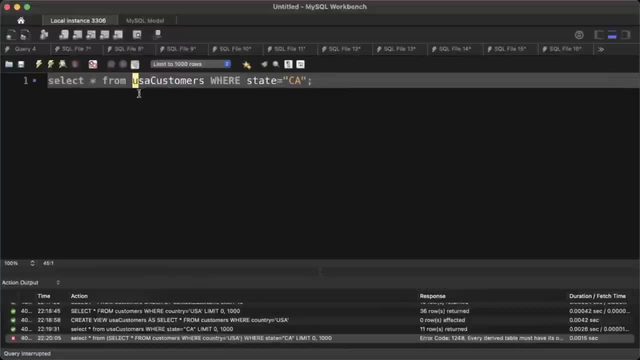 Okay, And once you have connect, connected to that server, you need to be able to send instructions to the server, the queries that you want to, that you want to send, that, that you want to perform, And then the database server is going to give you back the results and you should be able. 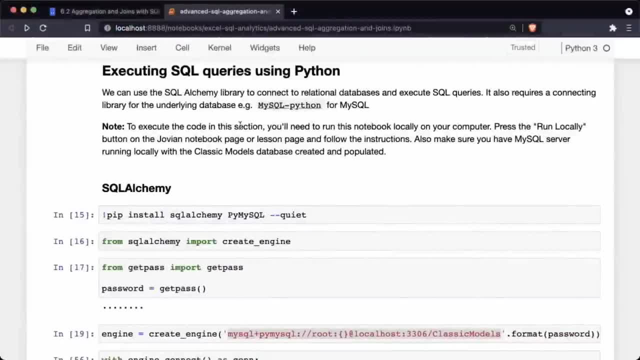 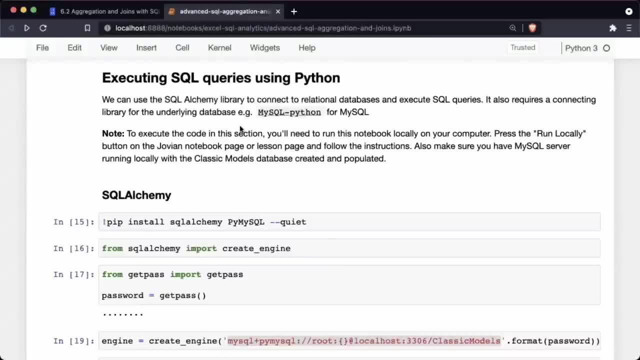 to understand the results. So this is something that you can do from any language. Every language has some libraries for working with SQL relational databases. in Python, One of the most popular libraries is the SQL alchemy library. Okay, So you can look it up. 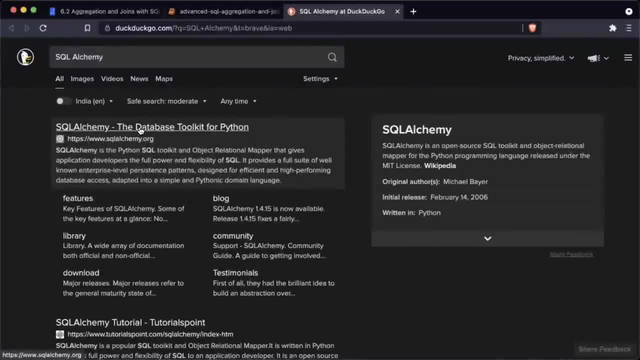 This is SQL alchemy or SQL alchemy, And it's a very powerful toolkit for Python that pretty much everybody who uses SQL databases and does some programming in Python uses this library. In fact, we use it on Jovian. When you open your profile page to get the information for your profile, we use the SQL. 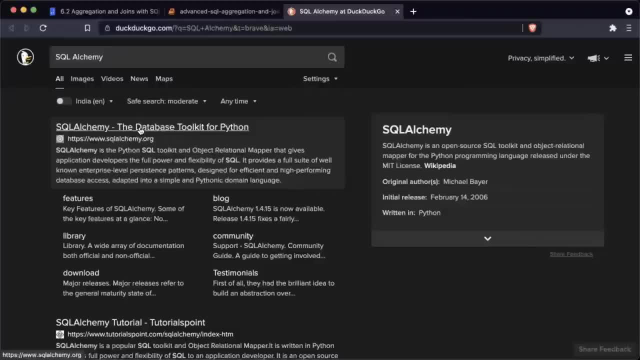 alchemy library to get information out of My SQL database And then we display that information to you on the profile page. Okay, So it's a very powerful and a very efficient library as well. It's as as it says here: it provides enterprise level persistent patterns designed for efficient. 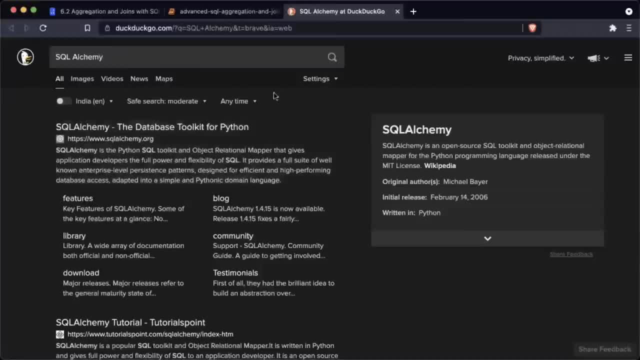 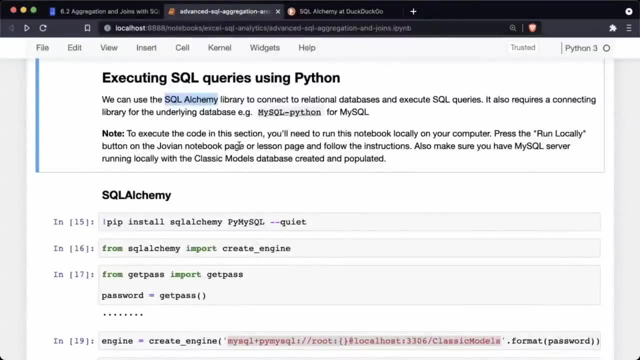 and high performing database access, adapted into a simple Pythonic domain language. Okay, So that's the library we are going to use. Okay, Now here's the other thing. that is not just a single relational database. There are many, in fact. here are some: 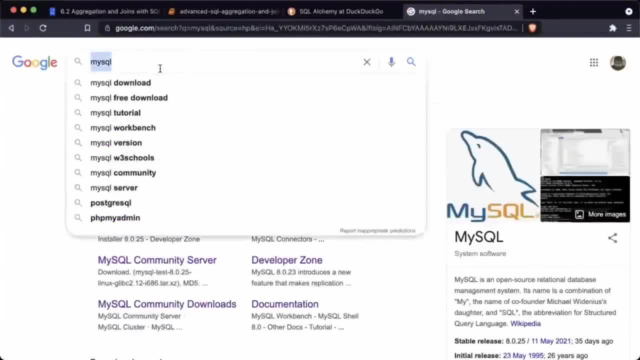 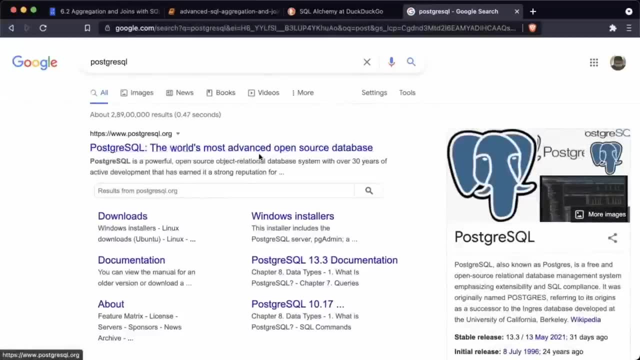 So my SQL is one that we've looked at. apart from that, there is something called postgres, So this is sort of a slightly more advanced version of my SQL, where it also supports latitudes and longitudes. is also supports like a Jason column type. 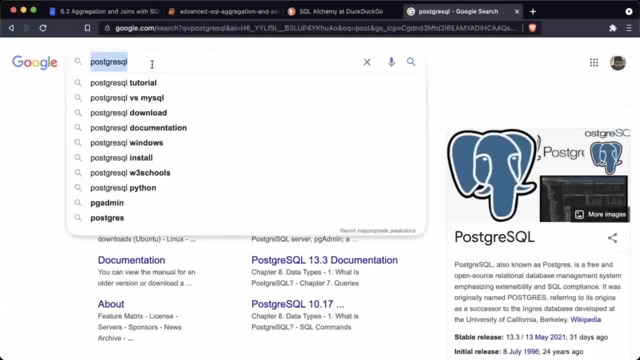 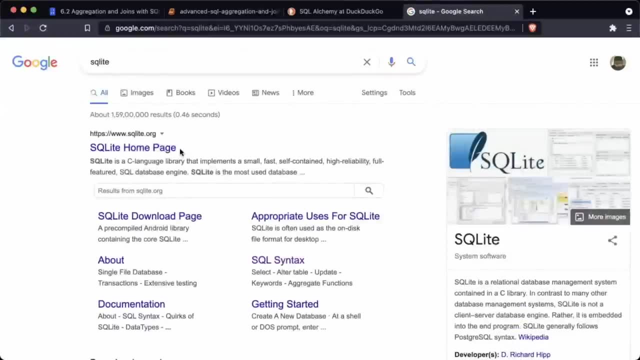 It has more column types. Um then there is something called a SQL light. So SQL light is a less- uh is a limited version of my SQL, and SQL light is typically used for situations where you can possibly- you possibly cannot- set up a entire server and 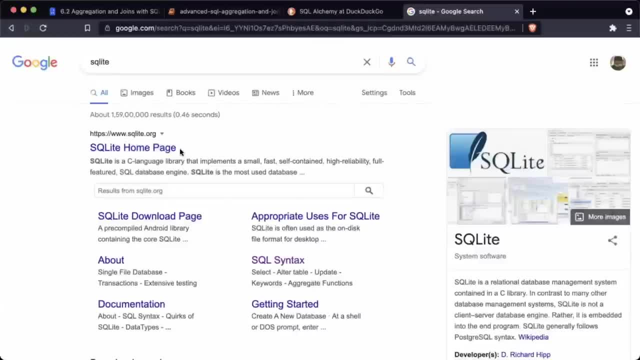 you just have to maybe work with something very light. So SQL light, instead of setting up a proper database server et cetera, simply uses a file on the disc and that file just works as a database. Uh, of course everybody uses the disc, but SQL it just makes it very efficient and very fast and very small. 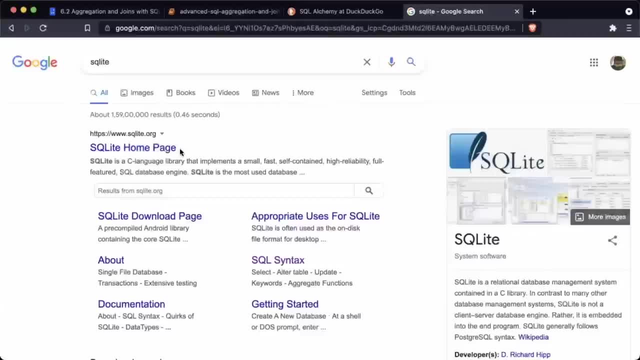 So typically this is used in um, let's say in in your phones. So any Android app or any iOS app that you use, uh is if it stores any information on your device, typically that store that information will be stored in a SQL light uh database because it has very low memory and CPU requirements. 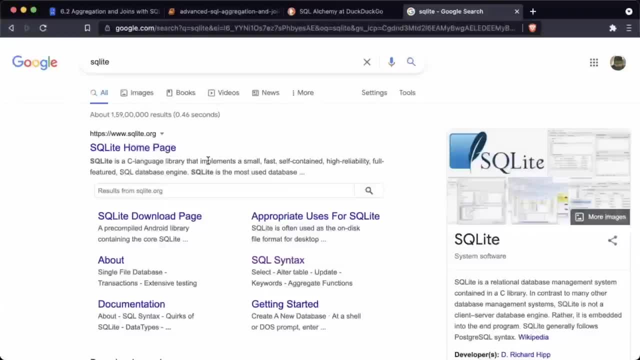 Of course it is. It does not implement the entire SQL language, It only implements parts of it And it sort of cuts corners here and there to make it possible to use SQL in a very low memory setting. In fact, in your, in your assignment, you will be using SQL light, so that that is something that can run easily on binders. 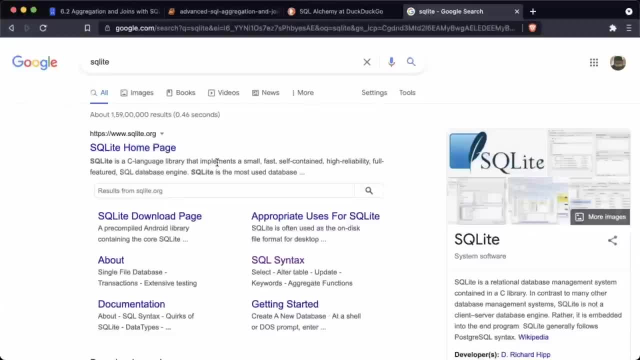 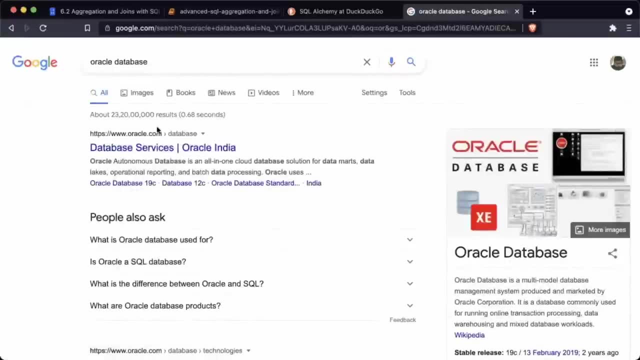 Setting up my SQL and binder is a big challenge, So we're just going to use SQL light. apart from that, you have You have some proprietary databases like Oracle, So Oracle has its own database. uh, again, that has its own flavor of SQL. 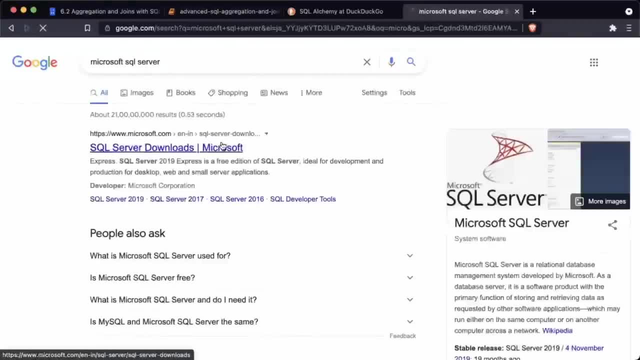 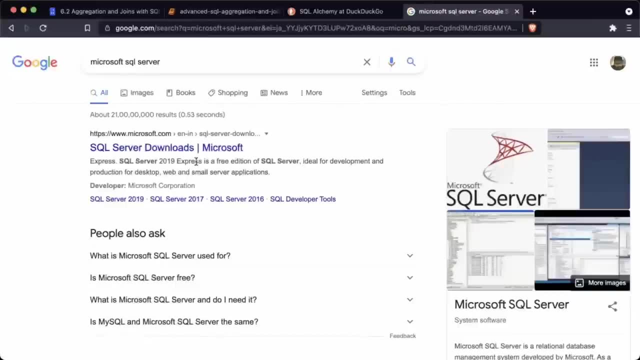 Uh, then you have the Microsoft SQL server, So that has again its own version of SQL. There are some changes. not all the commands work work exactly the same way And in fact if you look up any SQL tutorial, they will tell you what the differences between the different flavors of SQL are. 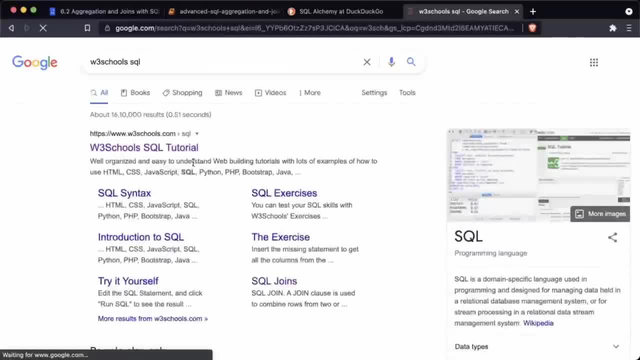 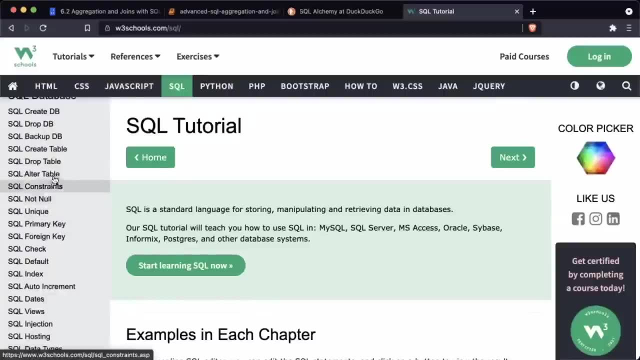 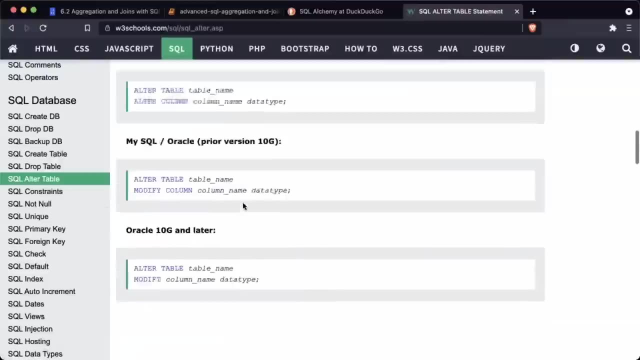 Right. For example, W3 schools Is The one that I would recommend, And here on the side you can see all the possible different um things that you do that you can do with SQL, And if you open any specific example here, like alter table, you will see how these are different across different SQL databases. 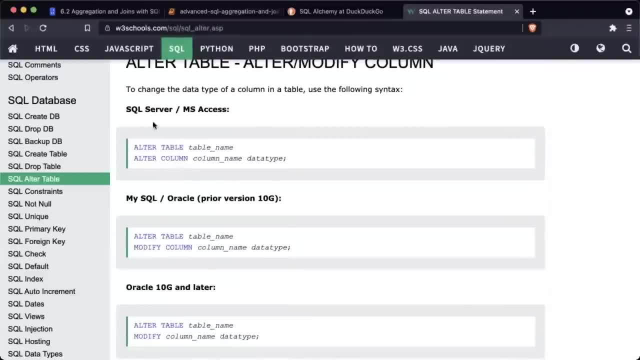 So alter table, which is to change the column name, et cetera. This is how it works on SQL server. This is how it works on my SQL. This is how it works on Oracle. In this case, I think they look the same. 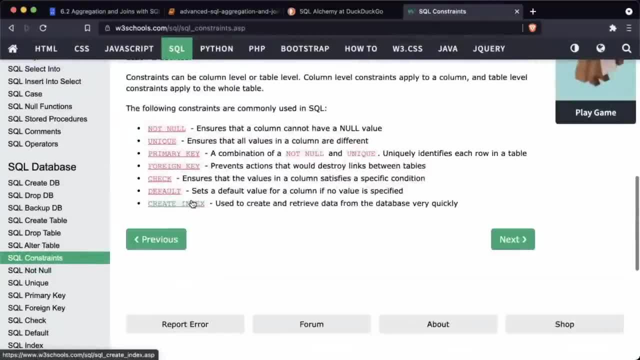 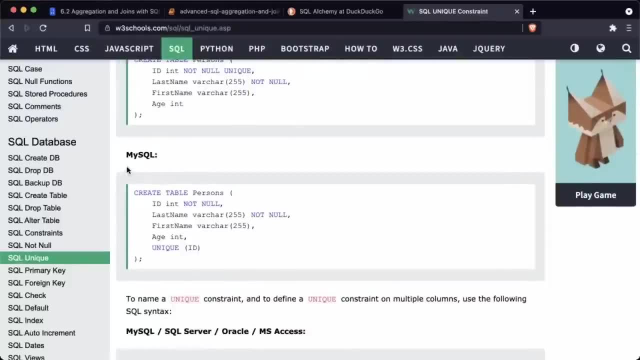 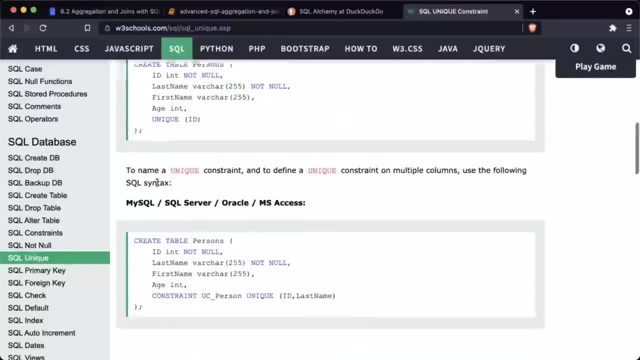 There's no change here, but there are other things, probably with constraints, where things would be different. Yeah, So you see here, this is how it works with SQL server, This is how it works with my SQL. So if you're putting some sort of a unique constraint in SQL server, you put it here in my SQL, you put it at the end, and so on. 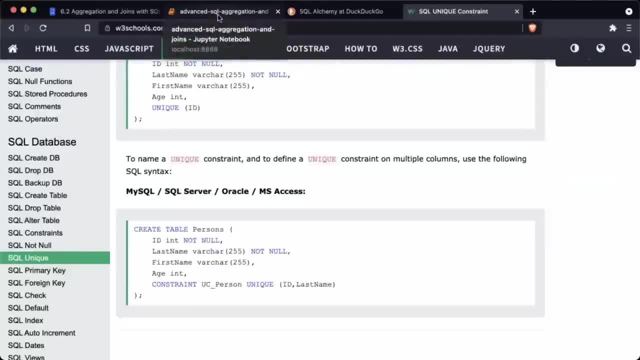 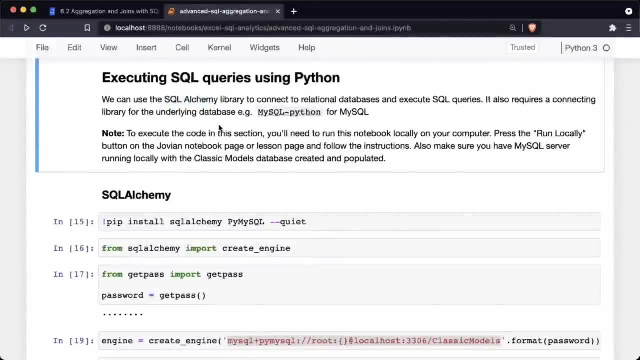 So just look things up. Don't worry about um knowing all the different variants of SQL, but the way it is relevant for us here is SQL alchemy does not include all of these connectors to all of the different types of relational databases. 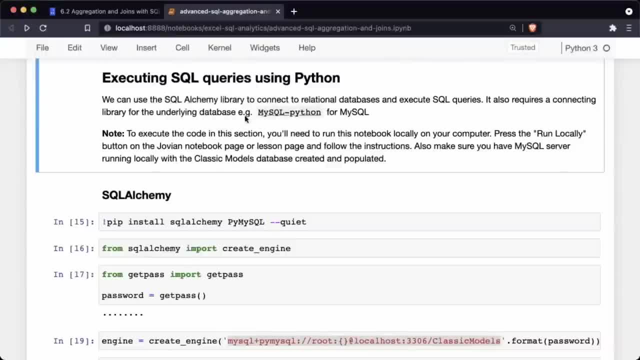 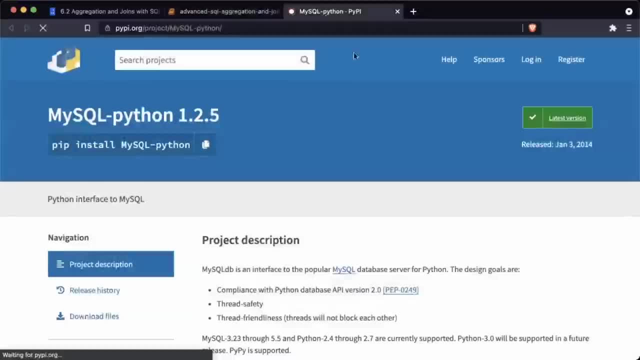 So what you'll have to do is maybe you will have to use some kind of a connector, a connecting library. So, for example, if you're connecting to my SQL, then my SQL Python is a commonly used connector. So you will have to either use my SQL Python or there's another connector called PI, my SQL. 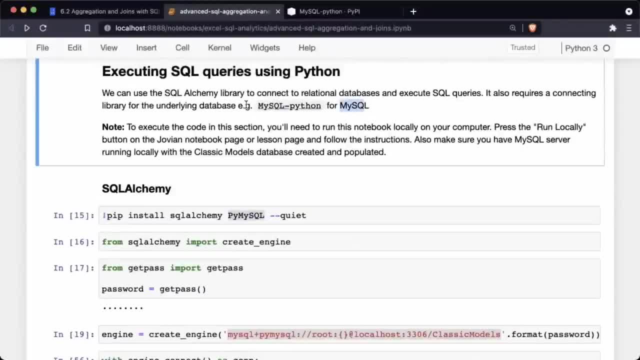 Uh, so there are several characters for my SQL right. So SQL alchemy Gives us the Python interface for writing SQL queries And then internally it uses one of these libraries to connect to the specific kind of database that you want to work with. 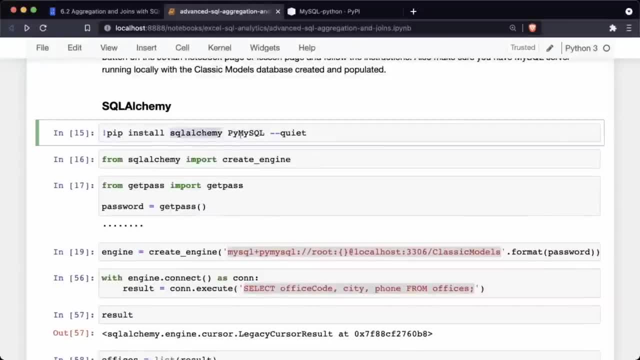 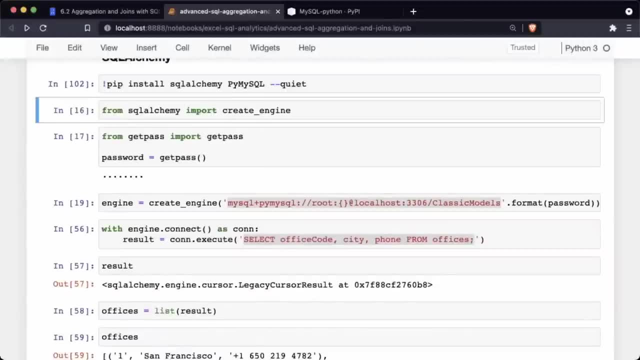 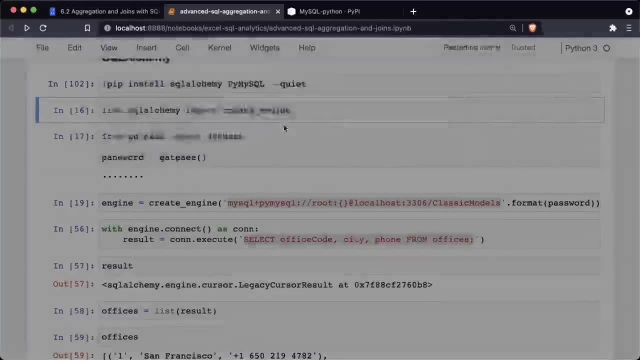 So you'll need to install both. So now we are going to install SQL alchemy and we are going to install PI- my SQL, So let's install both of them. SQL alchemy handles the Python side by. my SQL handles the my SQL side, and I'm just going to create clear output here. 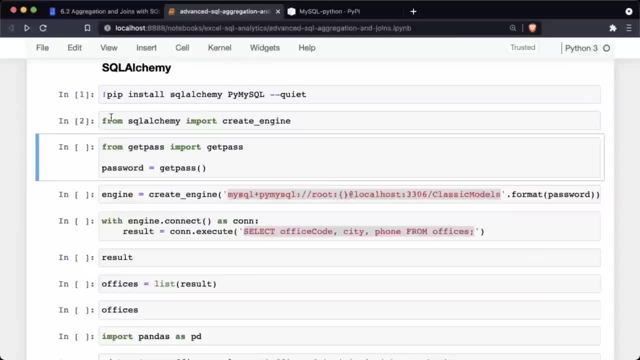 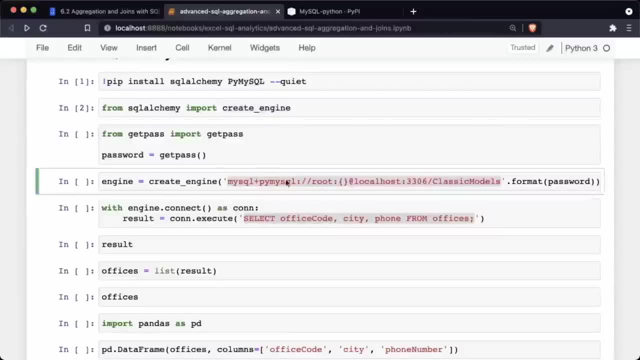 And let's import. see here's how you connect to a SQL database. The first thing you do is you say from SQL alchemy, import, create engine. So import, create engine and create engine takes a string, a connection string. 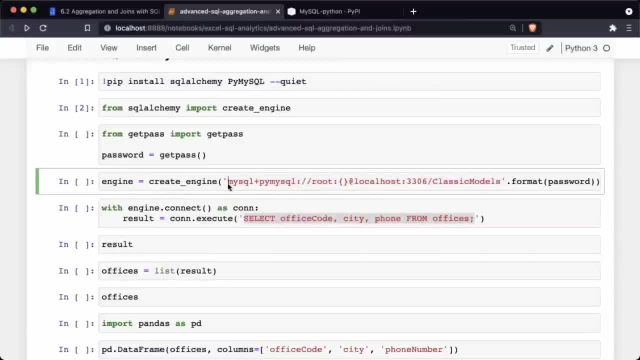 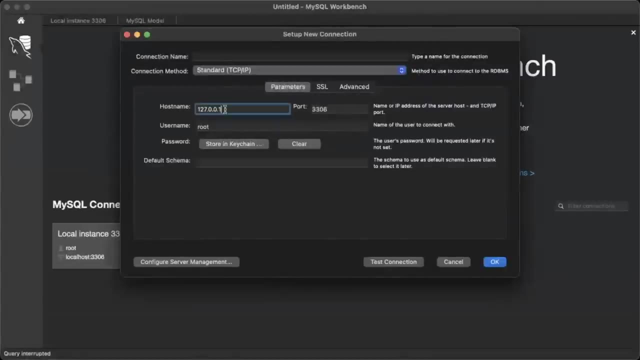 So what do you do is you say create engine and then you give it this string, this database connection string, which contains all the information required to connect to the database. Now remember my SQL workbench. Here, when we try to connect to a new database, we would have to provide a host name. 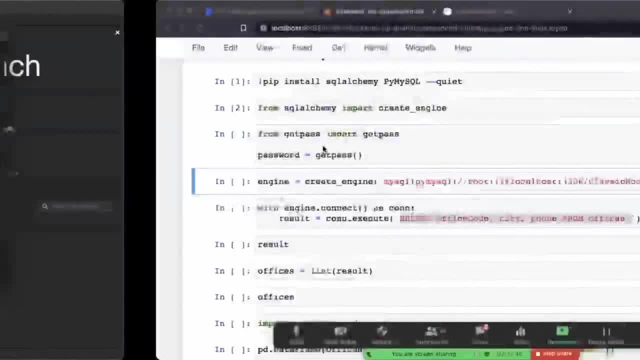 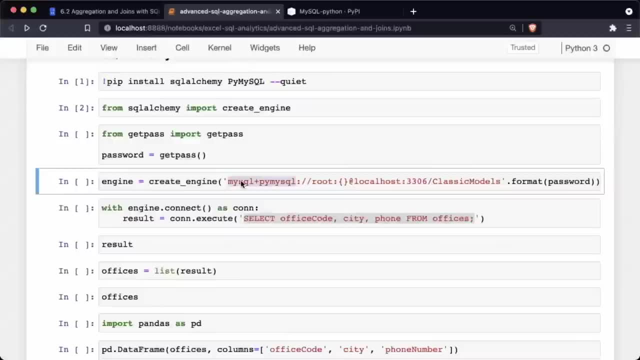 You would have to provide a port, We would have to provide a username and a password. So it works exactly the same way here. We say, uh, what kind of database we want to connect to? So we want to connect to a my SQL database. 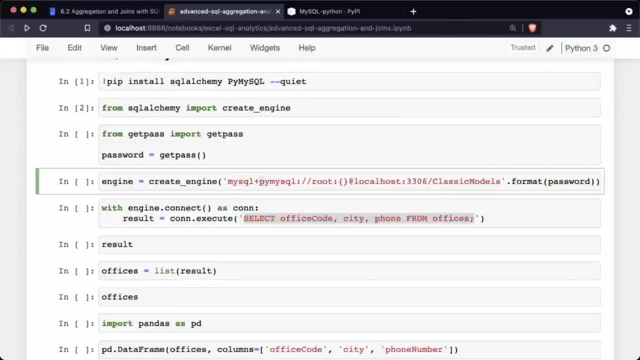 So that's why we have my SQL here We say what connector we are using. now, even for my SQL, there are several connectors that people have written for SQL alchemy. So we w we are using the PI, My SQL connector. 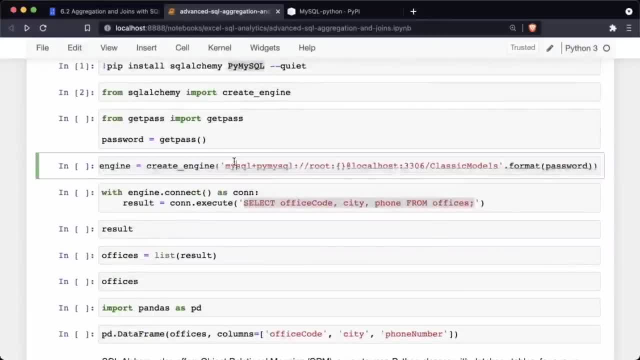 If you were using the my SQL Python connector, then this value would be different. Um, but in any case, we want to use the my SQL database, So this is the kind of database that we are using. Plus, this is the kind of connector we are using by my SQL. 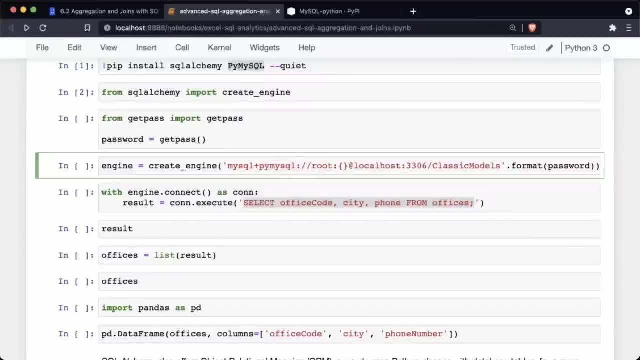 Then we say colon, dot, dot, and this is just a standard syntax. Then we provide the username and after the username you provide the password. So normally you shouldn't type passwords out, but let's say if you wanted to provide the password. 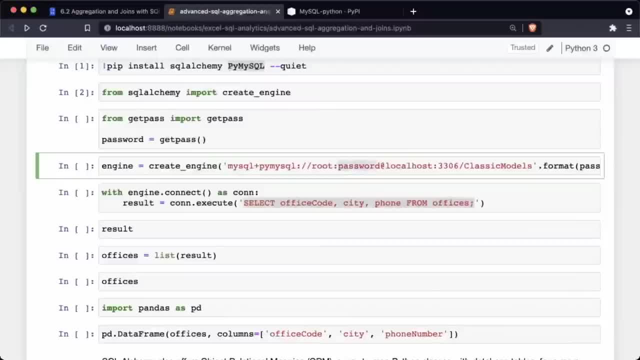 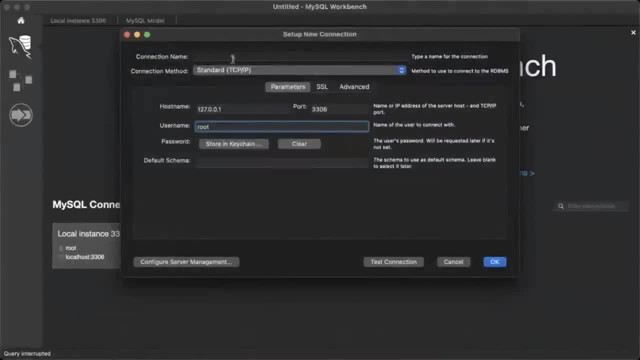 Directly you would say: uh, username, colon, password, then you pro, then you type at and then you type the server. So the host name that you put here, 1, 27.0 0.0 0.1, which means the local computer. 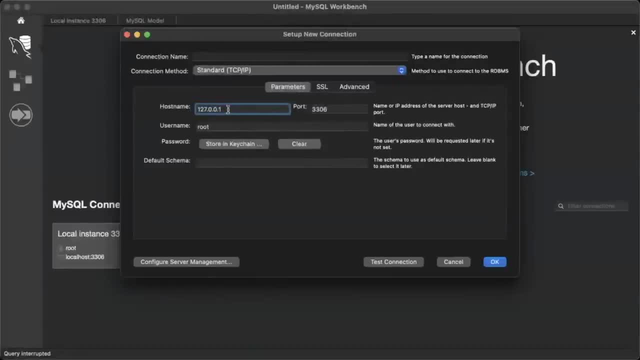 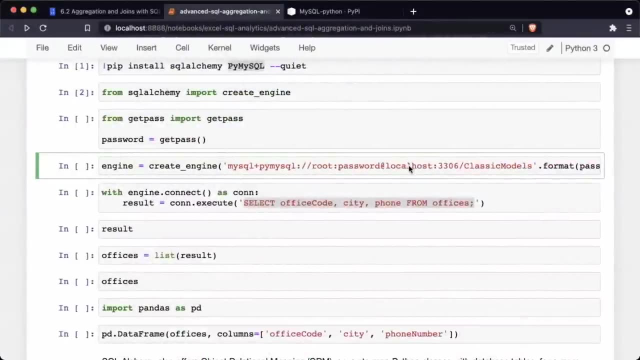 This is just short, for the local computer is a standard host name, Um, and that is also known as local host. So this could be 1, 27,, 0, 0, 1, or this could be local host. Both of those mean connect to a database on this computer. 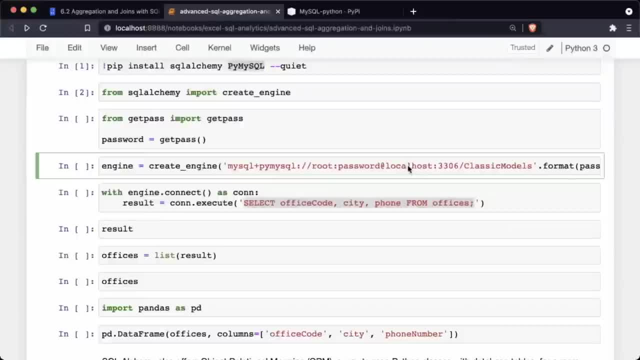 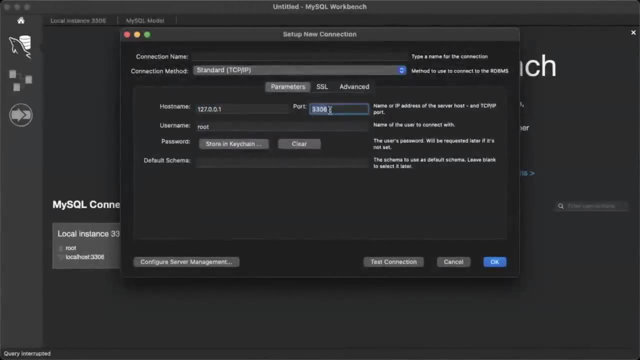 But if you are connecting to a database somewhere on the cloud, then you should get the username and the password and the host name for that cloud database. Next you provide the port. So for every database there are certain port that you connect at. 3, 3, 0, 6 is the default port that is used in most databases. 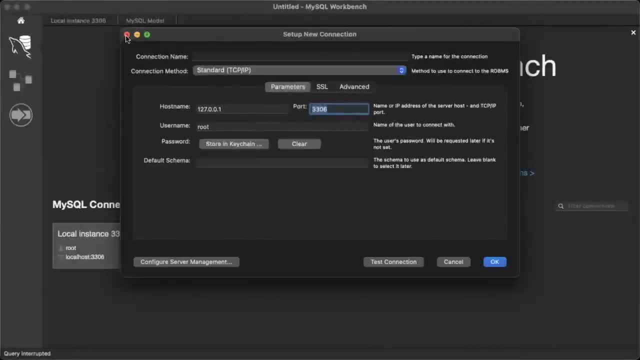 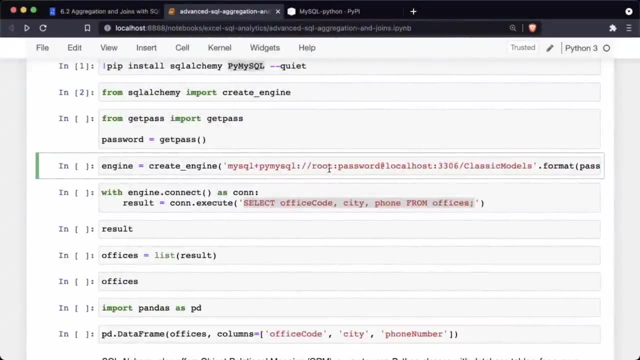 But if there is a different port, then you can ask your database admin to give you the port. So once again you get the type of database that you're connecting to, the type of vector you're using. colon: slash- slash the username password at local host. colon: the port: slash the name of the database that you're connecting to. 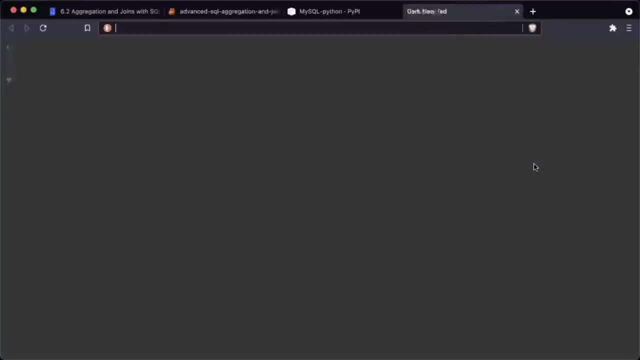 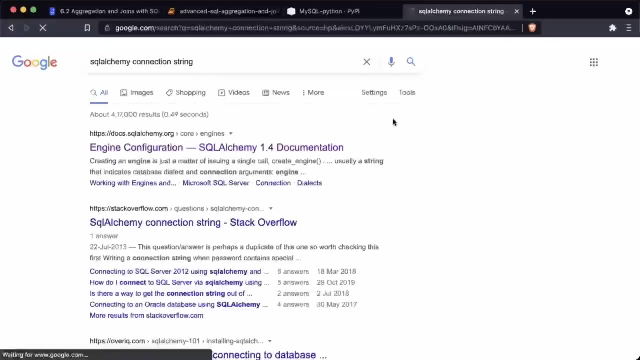 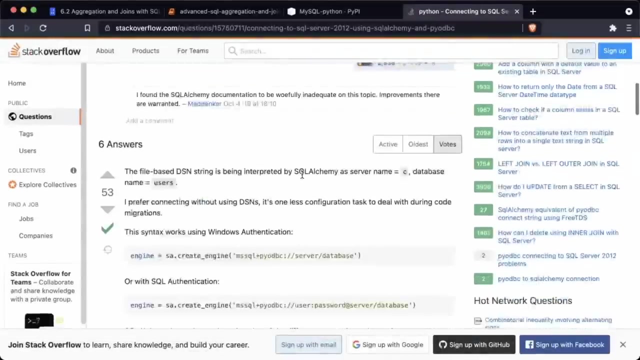 Okay, This is not something you have to remember. You can always just look up SQL alchemy connection string and let's say you want to look it up for SQL server. So you can just search connection string for SQL server and you can see what that connection string will look like. 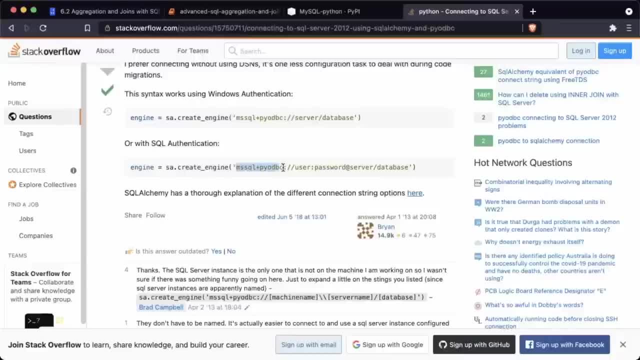 So for SQL Server this is what it will look like: My C M S SQL plus P Y O DBC. So the P Y O DBC is the connector and then username password at server. So server would be local host colon 3, 3, 0, 6, or some other online server slash database. 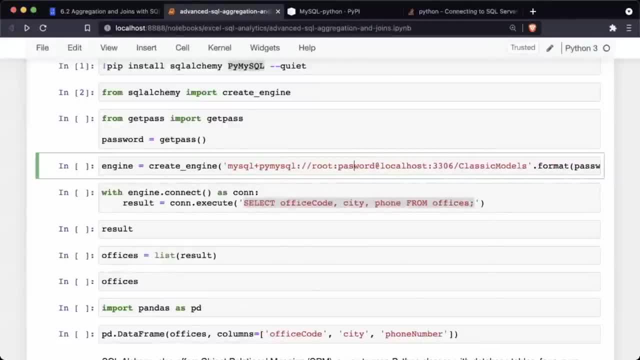 Okay. Now, one thing I've done here is, instead of putting the password I want, I don't want to type my password into a Jupiter notebook, So I have just imported get pass and I'm going to run get pass. 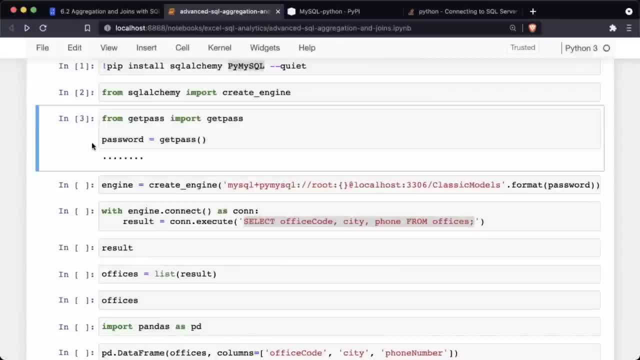 I'm going to type the password here. So now the variable password contains the value of the password that I just typed in, but I'm not going to display it in front of you because I don't want you to show you. I don't want to show you, I don't want you to see my password. 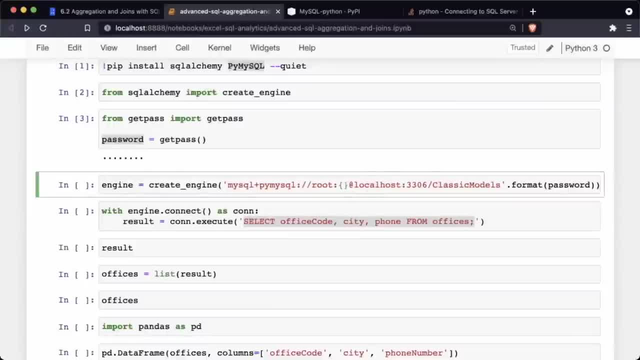 So what I'm then going to do is use string formatting to insert the password into this string. So now I have the connection string inside which I have this gap, using these quotations are using these brackets, Okay, And then I'm going dot format password and that's going to put the password into that gap. 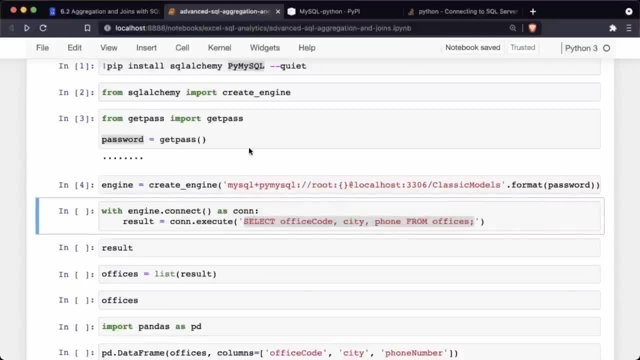 Okay, So never put your password directly into your Jupiter notebook, especially at work, because that's going to be very bad, because then anybody who has your Jupiter notebook will be able to use your account. Always use, get, pass. So just put the password into a variable and then pass that variable, using string formatting, into the connection. 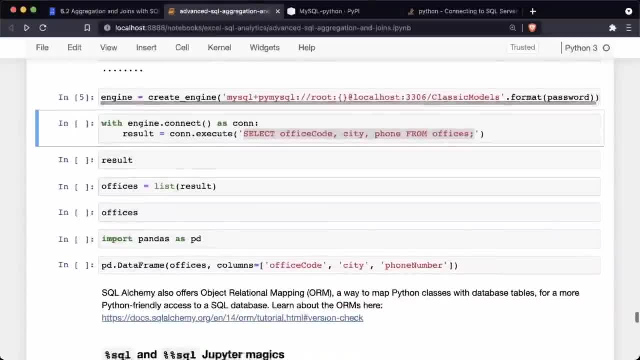 string and that then creates this engine. Okay, So now we've created this engine. So what has happened so far? Nothing, really. we've just set up this object and we've given all this information to SQL alchemy. Then we actually connect to the engine. 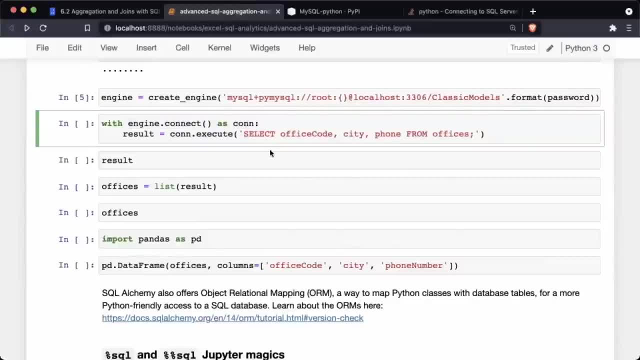 We say, with engine dot, connect as con, C O, N, N, and then we can execute SQL queries. Okay, So we connect to the engine as con. and why do we have this with? Well, this automatically takes care of closing the connection once we get the result. 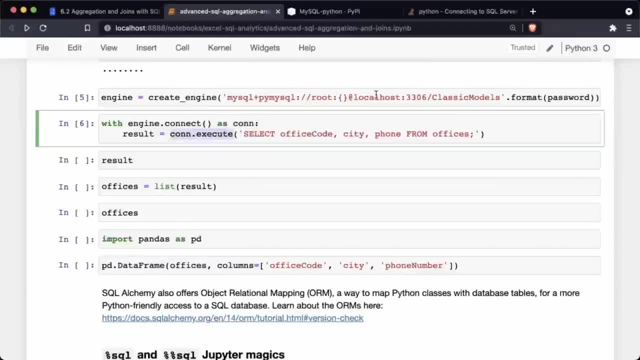 So we say C O N N dot execute. and now I'm connecting to my local database. So make sure that if you're running this on your computer you have the SQL server, my SQL server, running, And if you're running this on binder, obviously it's not going to be able to connect to your local computer. 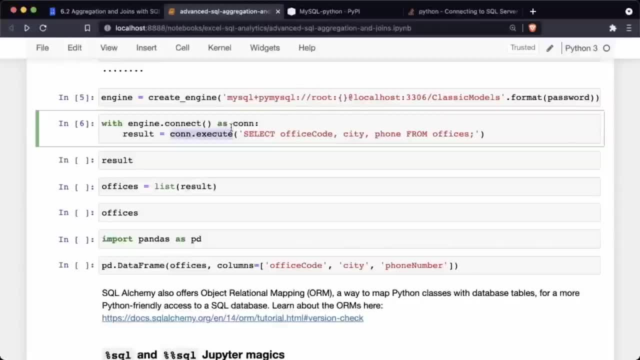 So make sure that you're running this locally on your computer. Okay, So now we say connection, dot execute and we have a query. So we have select office code, Comma city, comma phone from offices. So let's see what this query gives us in the SQL work bench. 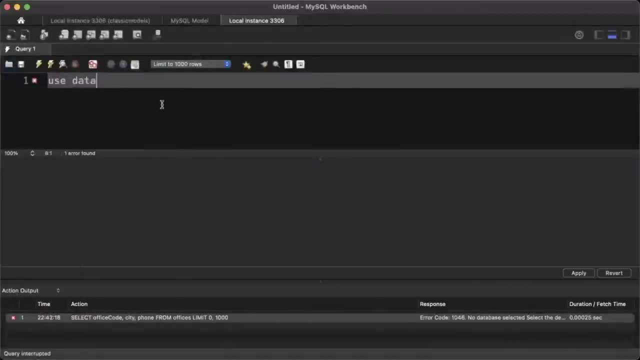 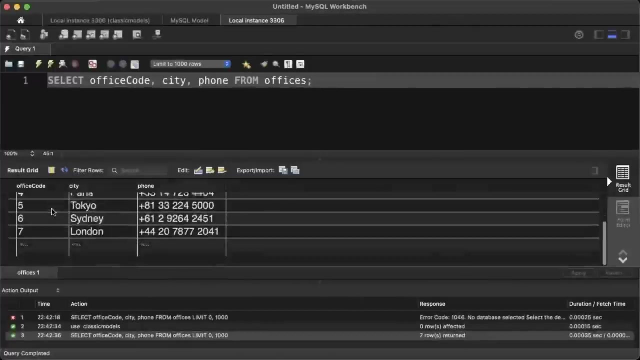 Okay, Maybe first I should do use database classic models, or just use classic models, Yup, And now I can select office code, city, phone number. So I expect to see it. Information like this: seven office codes and then the city and phone number. 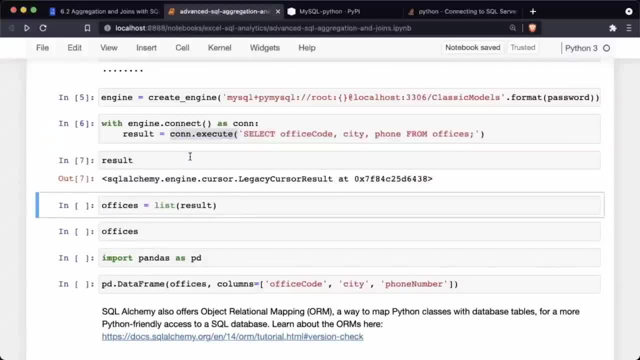 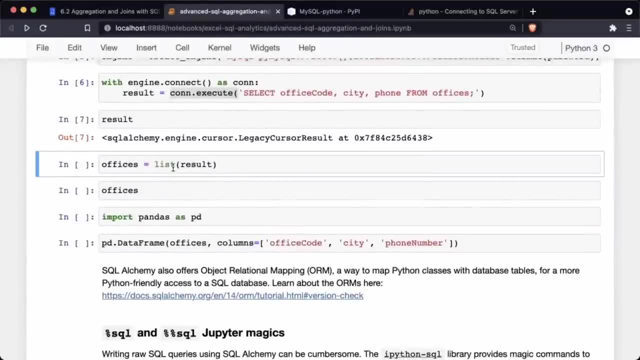 So I get the result from corn dot execute and let's look at the result. The result is this: legacy cursor result. It doesn't give me much, but you can convert that result into a list, So you just call list on it. 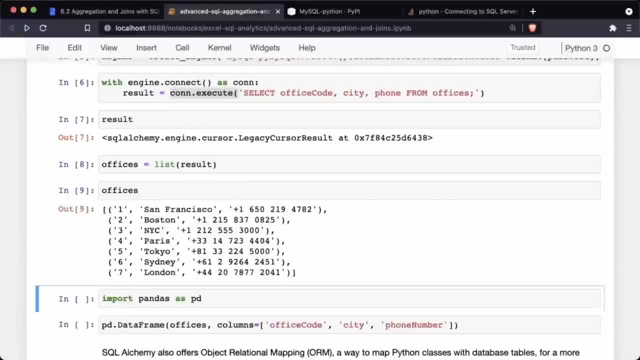 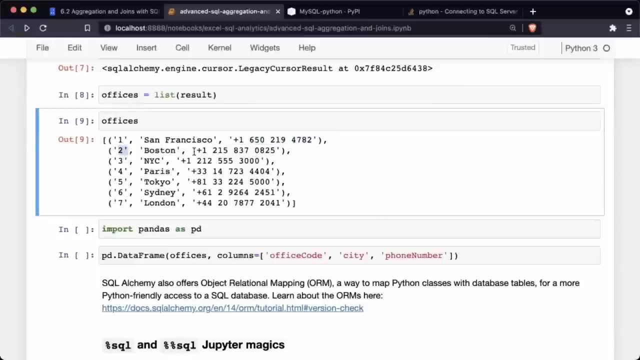 And that gives you this list of offices or list of results, And let's check that. So here now you get one San Francisco plus one six by zero, two, one Nine. Two Boston plus one two one five, and you can match that information up here. 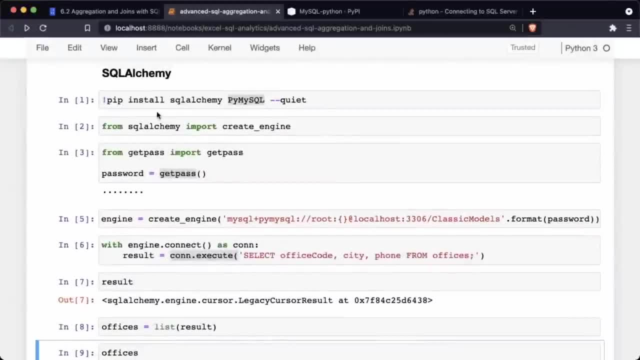 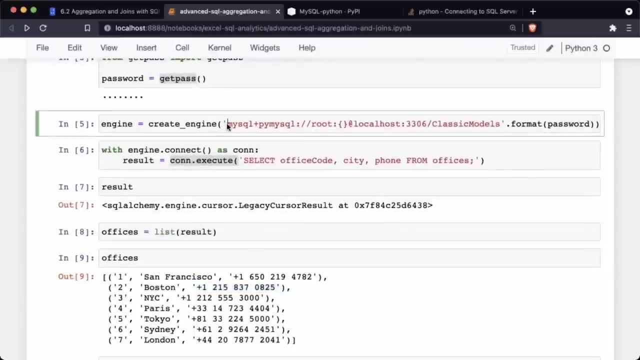 Okay, So quick recap: install SQL alchemy, install the connector, import, create engine. then create the engine using this connection string which contains information about the kind of server, the kind of database you're using, the kind of connector you're using, the username, password, host name and port and database name. 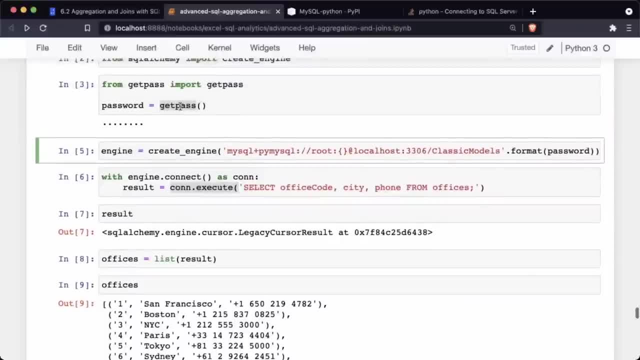 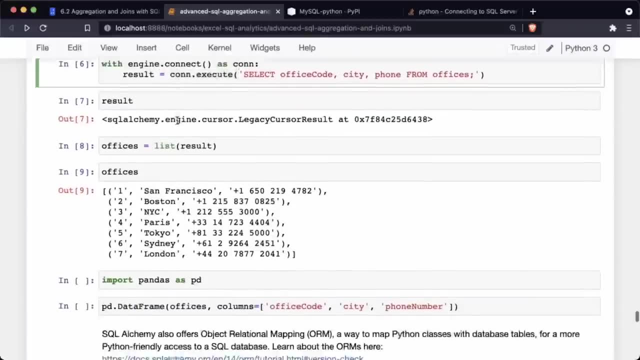 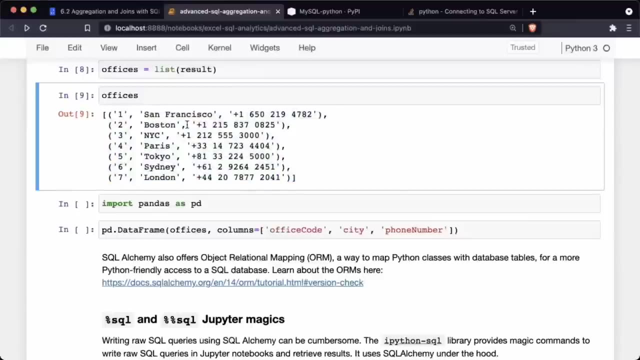 Of course, Or don't type your password directly. get it using get pass, Once the engine is created, connect like this and then get the result. And now you have this result here. So now, once you have this result, this is a Python list and it's a list of tuples. 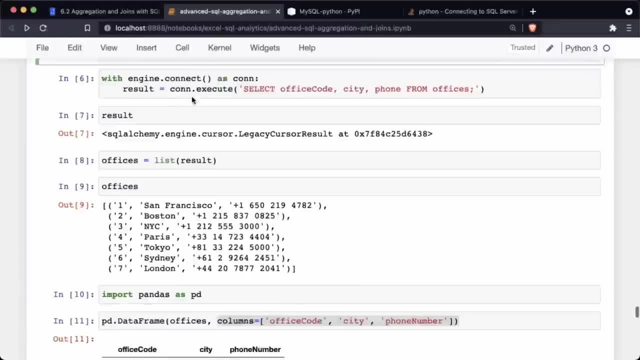 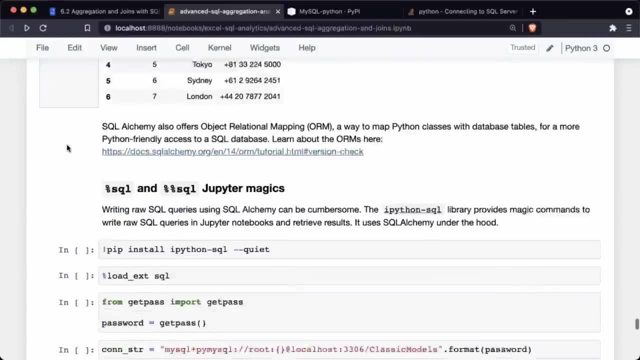 The idea I want you to take away is that you can create this engine, create a connection and then get data out of a SQL database using Python. Now, of course, this is a lot of work, And that is where you have this nice, neat little library called I Python SQL. 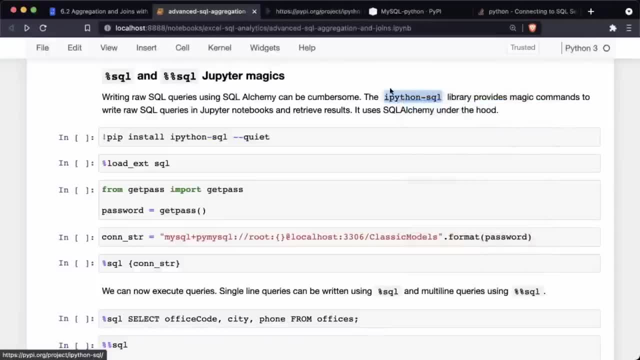 It's probably one of the most wonderful libraries I've come across because it takes away so much of the complexity that you have to take care of when you're connecting to SQL databases. So the IPython SQL library provides something called magic commands to write raw SQL queries in Jupyter. 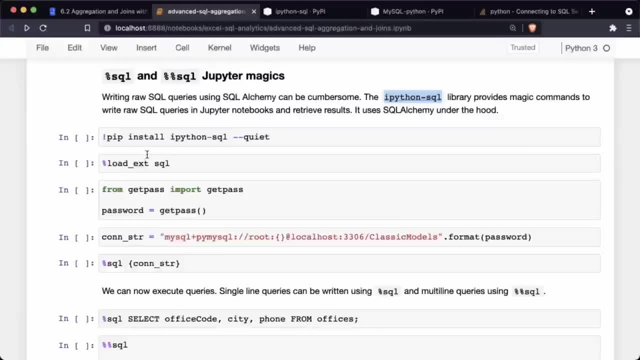 So you just type raw, you just type a SQL query within Jupyter And That Will execute and that will get you the results. and it'll give you the results in a nice tabular format, something that you can use within Python. 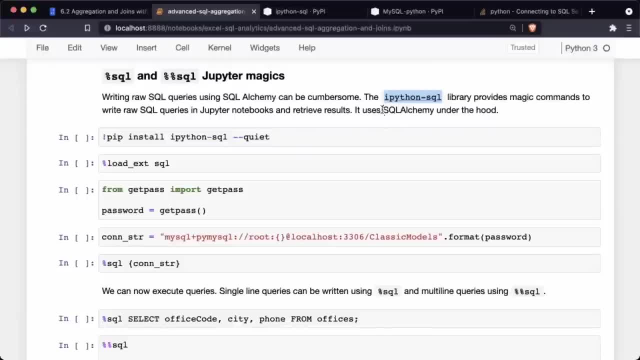 And in fact it uses SQL alchemy under the hood. So you want to have SQL alchemy installed and you want to have the right connector installed. So, for example, in this case I'm using PI, my SQL, So I have SQL alchemy installed. 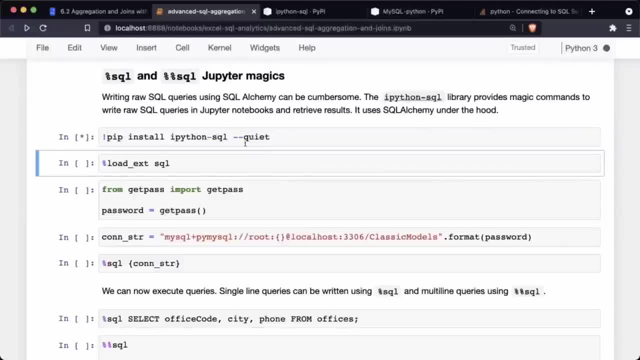 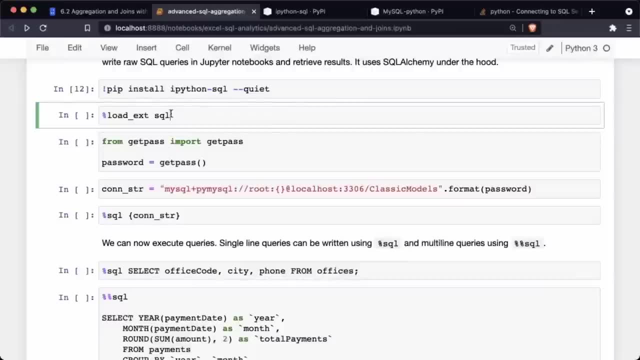 I have PI, my SQL, installed and now I'm going to install IPython SQL. So I installed the IPython SQL library And now it. It really is magic, because- and these are called magic commands- The first thing you do is you have to load this extension within the Jupyter notebook. 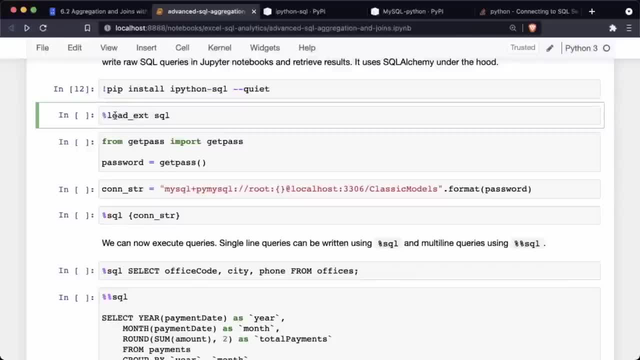 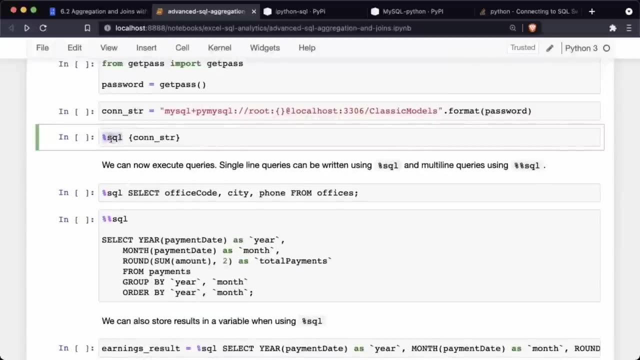 So you say load EXT. Uh, so you type this percentage symbol, you type load EXT, and then the extension that we're loading in is called SQL. And once you type this, once you run the cell load EXT SQL, then you will be able to start using this new command called SQL. 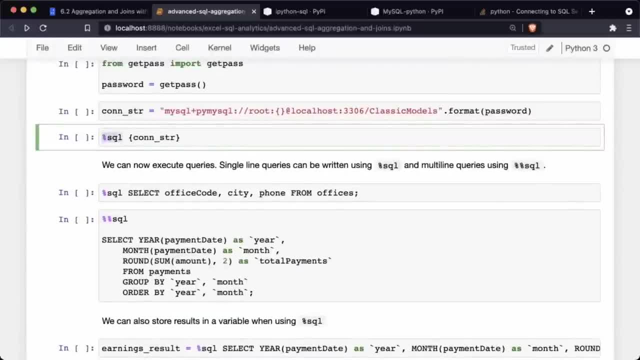 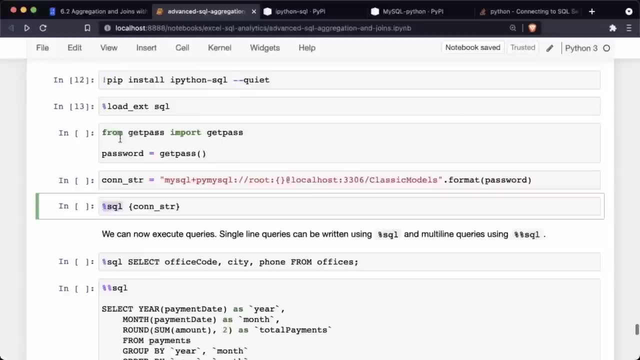 So anything that starts with a percentage is called a magic command in Jupyter. This is no longer plain Python. Now, this is some instruction that we are sending to Jupyter, So here's what you can do. You can type percentage SQL, Okay. 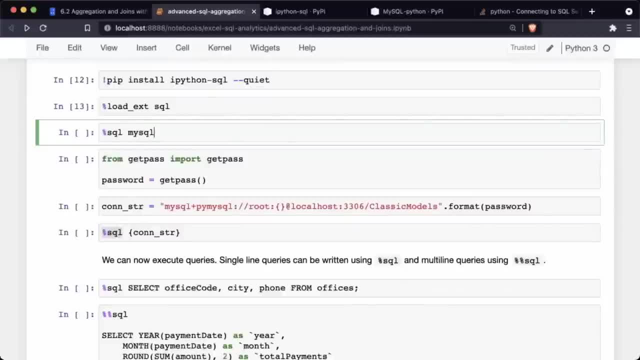 And then you give it a connection string. So for example, if you give it my SQL plus PI, my SQL colon, slash, slash, root colon, and then you put in the password here, let's say the password is just password at local host. 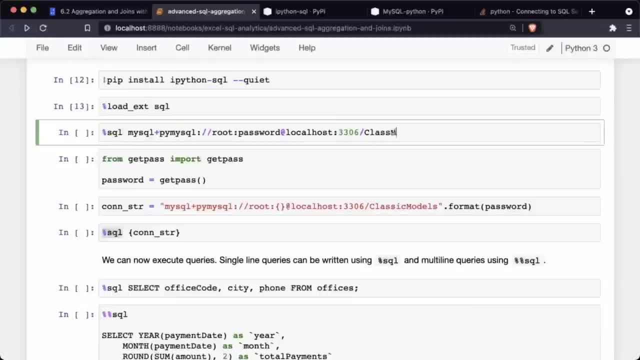 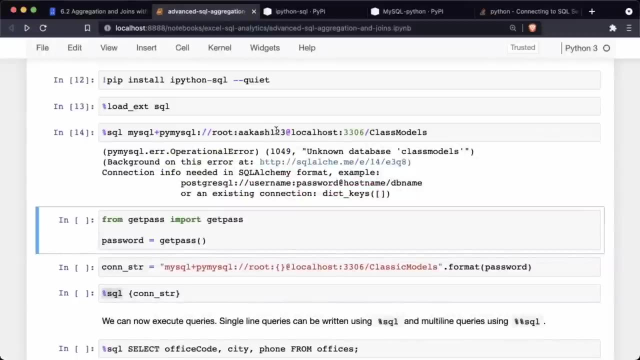 Cool In three Zero six and slash classic models. Okay, And I'm just going to reveal my password here for a second. So I'm just going to. the password is. well, it's Akash one to three. So if I run this, classic models. 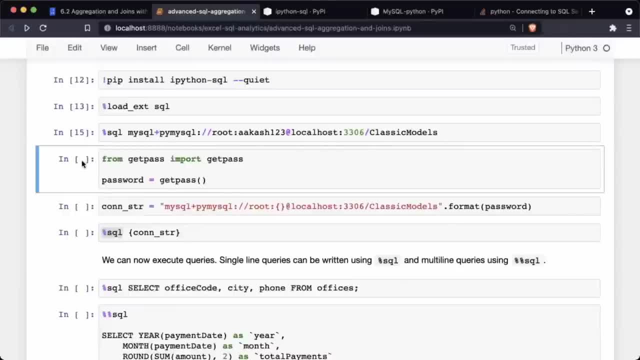 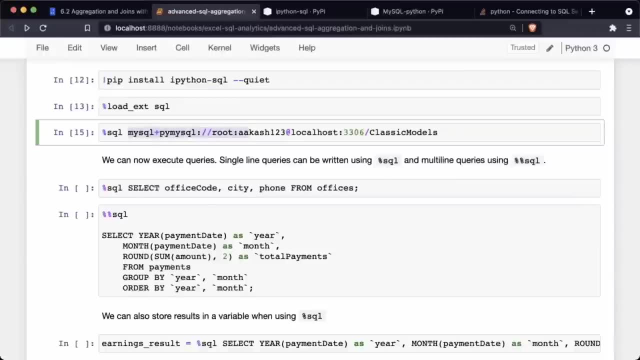 Yeah, So if I run this, now I'm connected to the, now I'm connected to them, to the database. right, I've just typed my SQL plus PI, my SQL colon Root, So username slash password. So this is a SQL alchemy connection string. 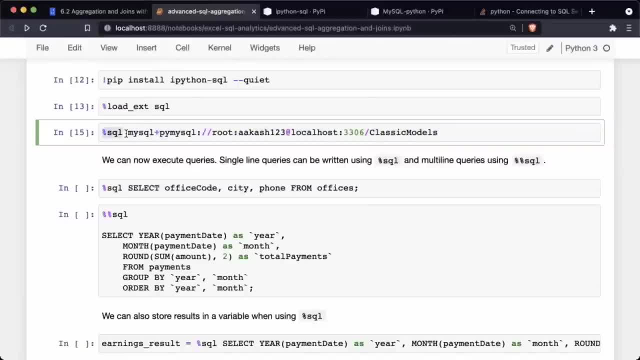 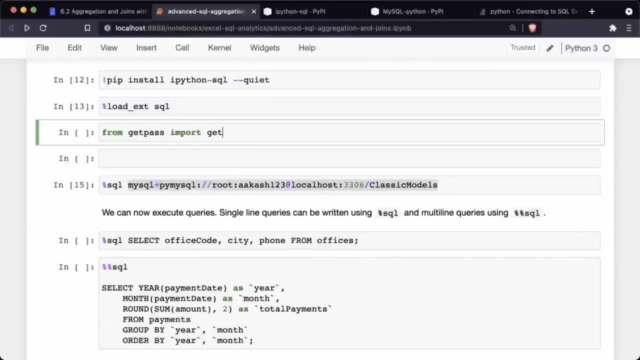 Now, instead of having to do import engine, create engine, et cetera, et cetera, I can just type colon SQL, give it the connection string And that is just going to connect to the, to the database. Now what to do. if I don't want to reveal my password, I would do from a get pass, import, get pass and then I would run get pass and okay. 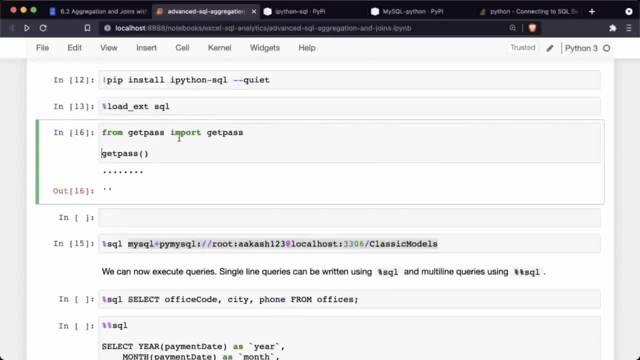 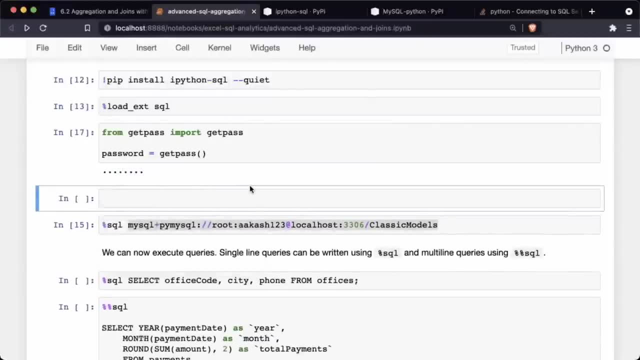 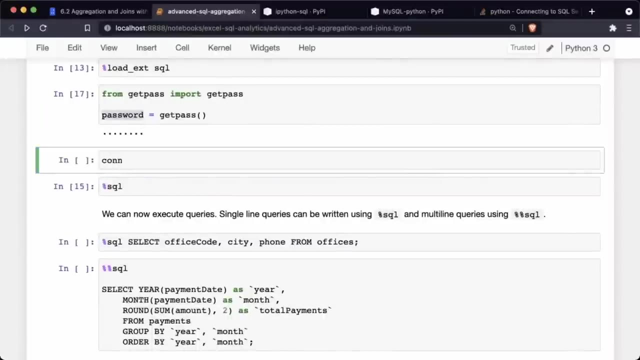 Maybe I should Put the result into password, Okay, And then I type my password. So now this variable password has my password and then I can take this and this, put it into a string. So I create a normal connections STR, I create a normal Python variable and I just insert the password here. 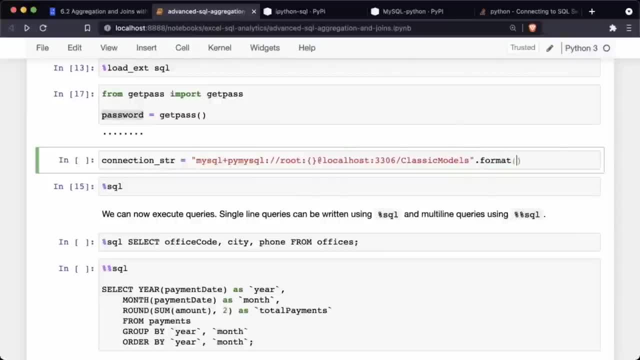 So I do dot format Password. and now I've created this connection string. So now I want to, instead of typing out the full connection string, I want to pass the variable connection string. And we do that by: in magic commands, We pass value from variables using these brackets. 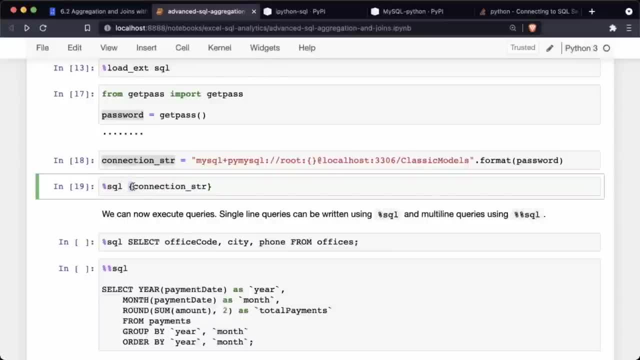 Okay. So when we type this, when, when we have, when Jupiter sees this bracket, it says okay, let me take the value of connection STR, Which is all of this with the password replaced here, And let me replace this with that value. 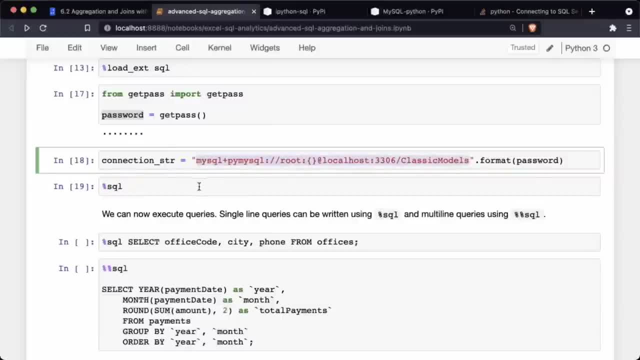 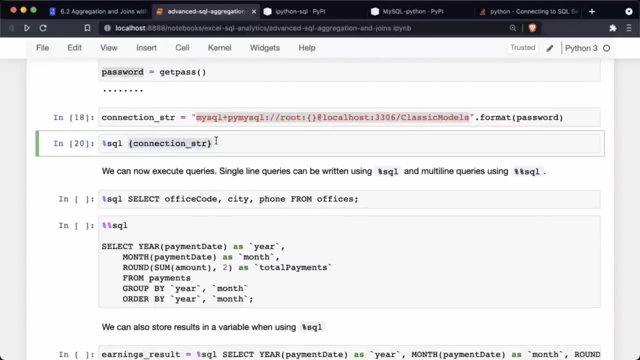 Uh, sorry, with with all of this stuff. Okay, So this is all around about way of hiding my password, but in any case, the the point being you just provide the connection string. Either you type out the entire string, including your password, or you put the connection string into a variable and you pass it using this bracket. 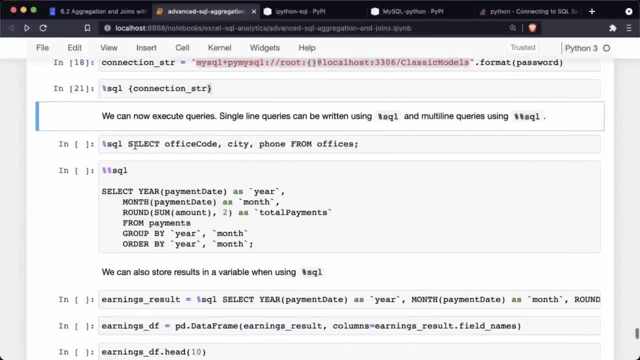 But just with this one line of code we are now connected to, To the database, and we can now execute queries. And here's how you execute queries: You type percentage SQL and then you just type the query like select office code, city phone from offices. 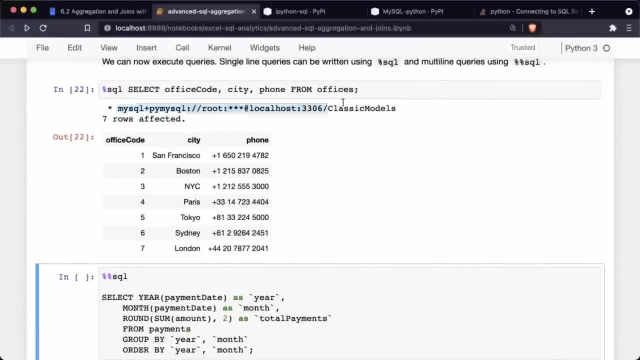 So there you go. So now you can see that it's telling me that I'm connected on uh using this connection route, and it hides a password, thankfully, Uh so, yeah, so we've typed this query and here is the result of the query: 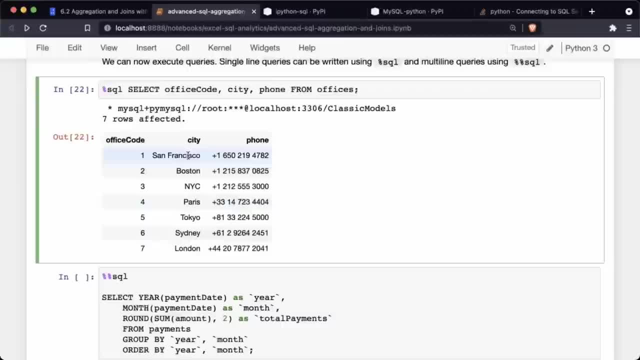 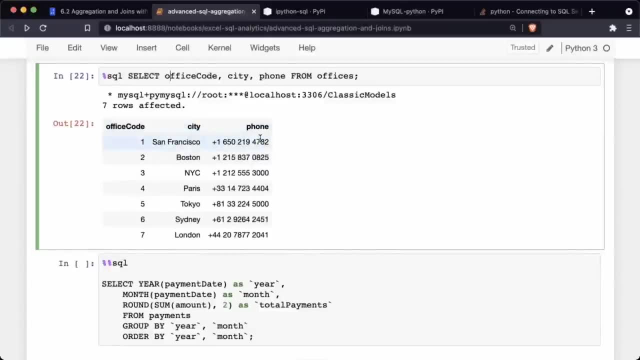 So the result is office code, city phone One, two, three, four, five, six, seven, San Francisco, Boston, et cetera, And the phone numbers. If you have a multi line query, something that you need to split across multiple lines, then just put a double percentage. 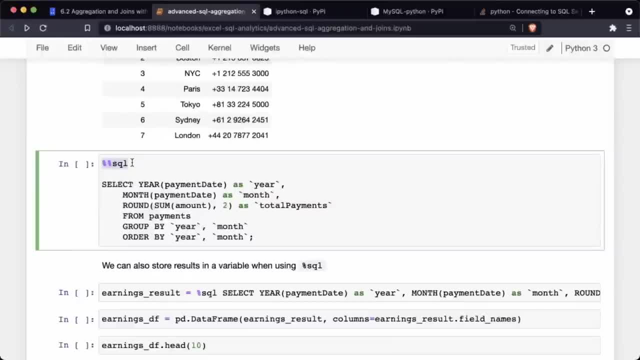 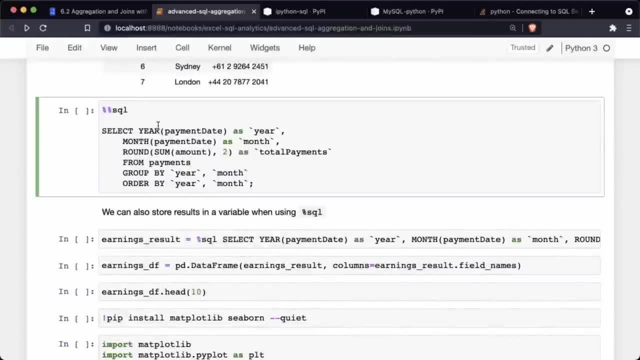 And when you put a double percentage, then this entire cell is passed to this magic command. When you put a single percentage, that just works for a line. the double percentage works for an entire cell. So let's run that. So now, here we are, doing the same thing. 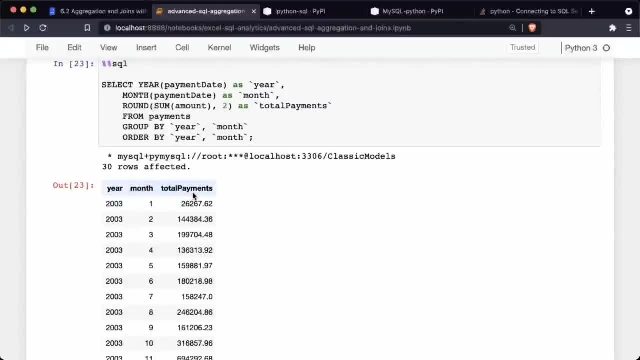 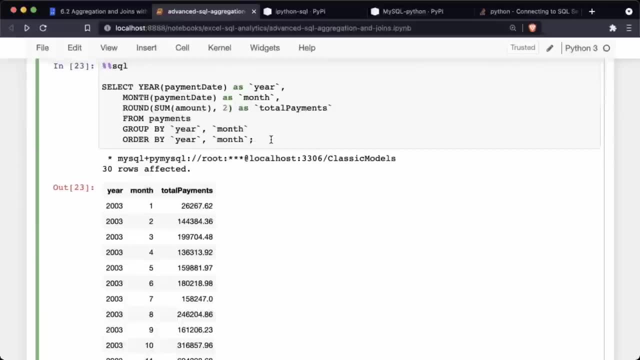 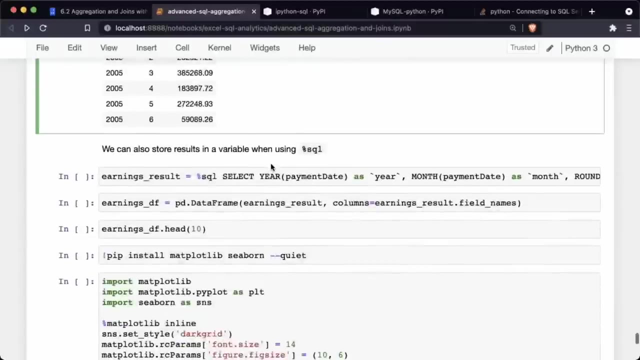 Remember, for every year and every month we want to get the total payments. So that's what we have here: year, month total payments by, as a result of this complex SQL query, percentage percentage SQL- and then you type the name, they type the query and that's the data. here's when it gets even more interesting. 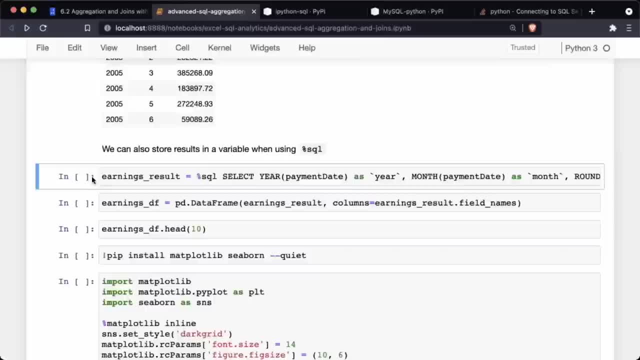 You can actually combine Python code and SQL code. So here's what I'm doing: I'm seeing earnings result equals And then, from this point on, once I type percentage SQL, Yeah, Jupiter detects that this is a magic command and it's going to read all of this as SQL code. 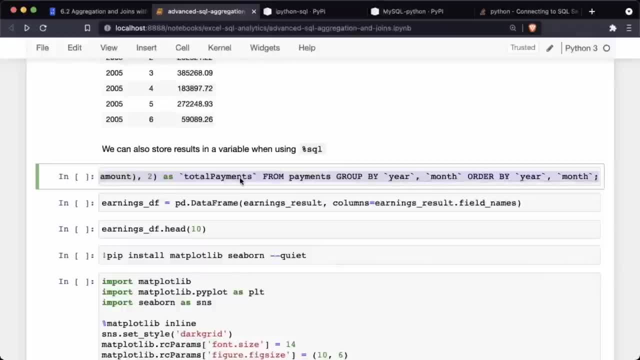 Okay. So what's happening is that all of this is being passed into this magic command, percentage SQL, and that magic command is going to, under the hood, use SQL alchemy, create a connection using the connection string that we had set up and pass this SQL query to that connection. 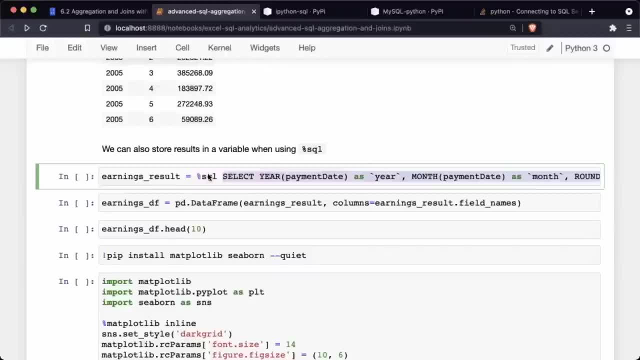 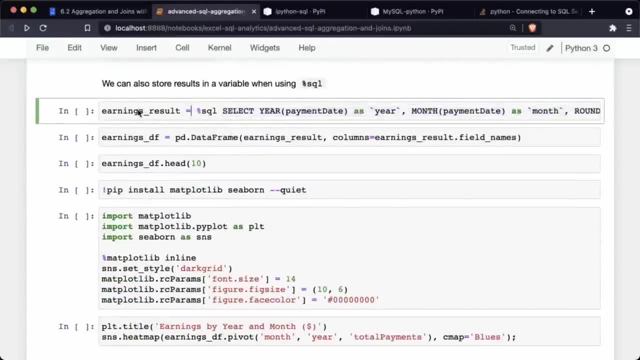 And from that connection get some results and then take those results and convert that into this format. Okay, And then that data frame kind of format is going to be put into this variable earnings result. So you type the variable name, you type equals, and then you type percent SQL and then you simply type the query. 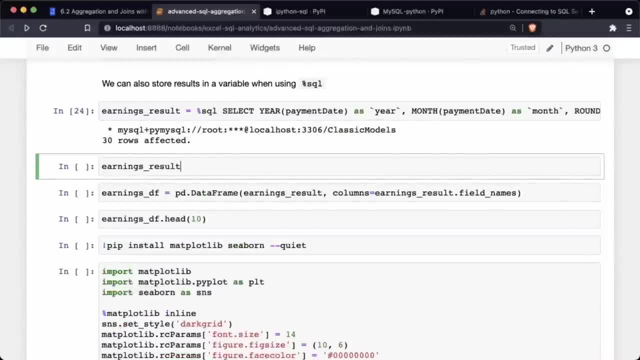 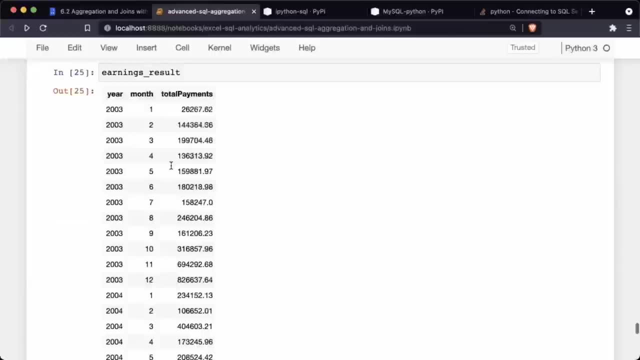 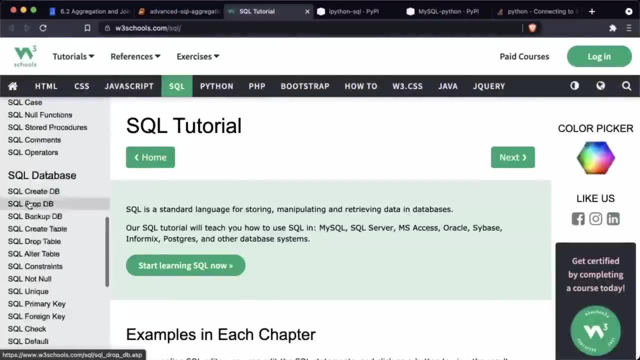 And now you have earnings result: That was the topic for today. as I've said, w three schools is a good resource and I would just go through all of these just to get a sense of everything SQL has to offer and use this notebook to 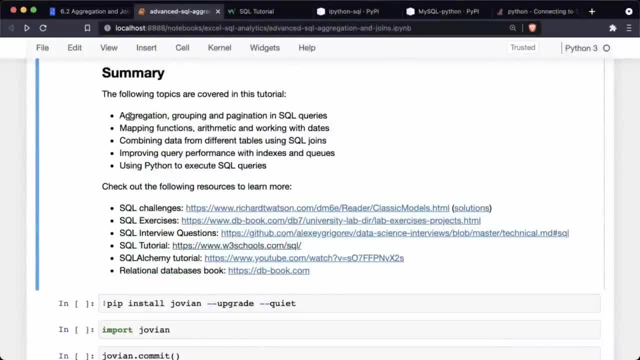 learn how all of these things fit together. So we looked at aggregation, grouping, pagination in SQL queries. We looked at mapping functions, arithmetic and working with dates. We looked at how to combine data from different tables using SQL joints. We looked at improving query performance with indexes and queues. 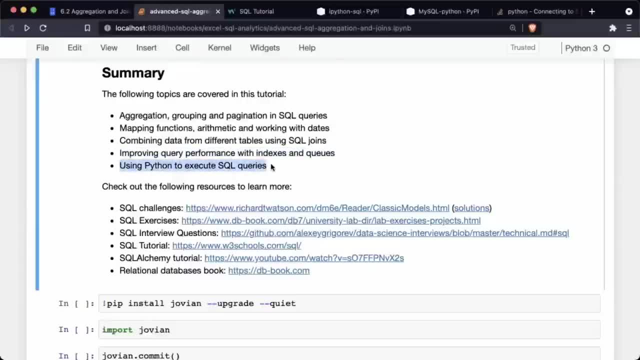 We looked at how to use by thin to execute SQL queries, which is to Get SQL alchemy, get a connector, create a connection string pass, put the password into it securely, create an engine runs queries. or we could just use the IPython SQL magic commands and simply use direct raw SQL statements inside a Jupiter notebook. 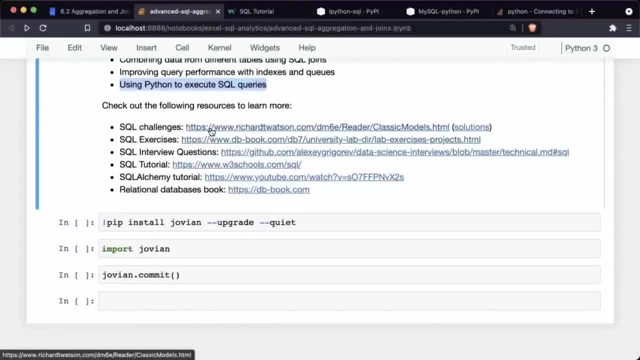 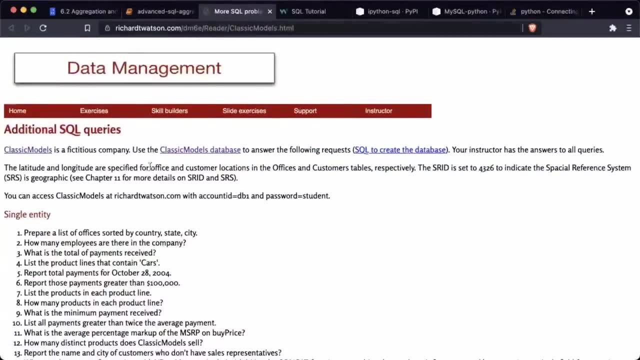 So what should you do next? You should definitely check out some of these other challenges. on the classic models database, This is from This professor. his name is Richard T Watson. It's a great database And he has also given you a lot of questions to solve. 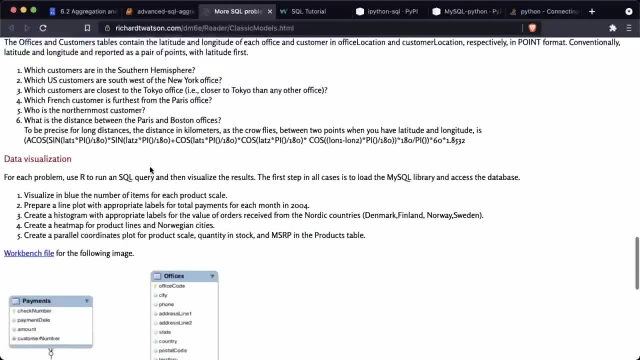 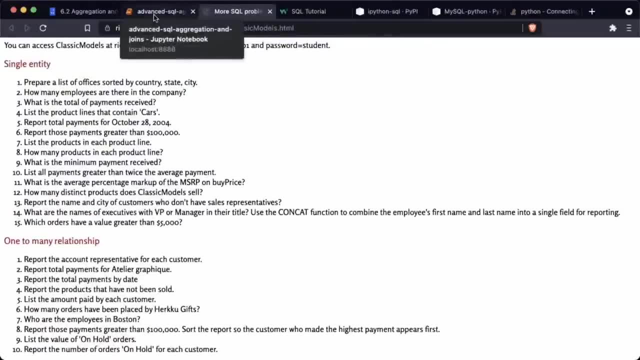 So there are about a hundred or 120 questions that you could try and solve, So the more it's all about exercise SQL. there's no other way to become an expert at SQL, And I wouldn't say I am because I haven't done enough exercises. 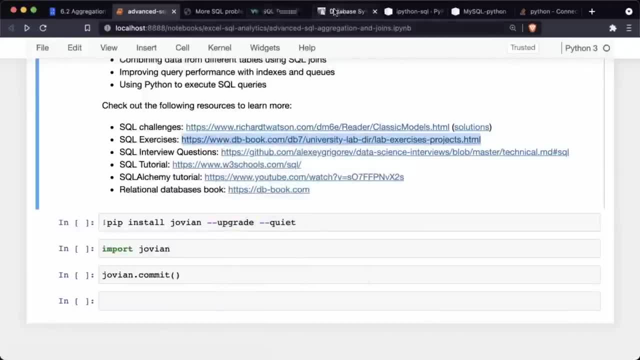 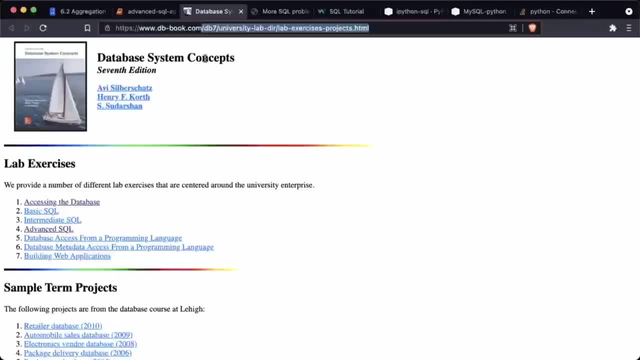 Here's one more set. a different database that you should look at is the Database system concepts book. in on this book page on dbbookcom You have a bunch of exercises so you can check here. Sam, sample lab exercises and term projects. 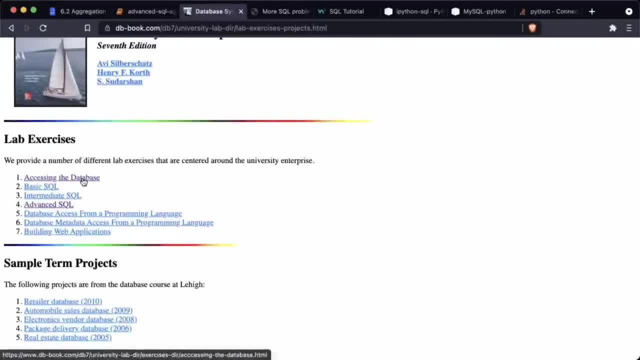 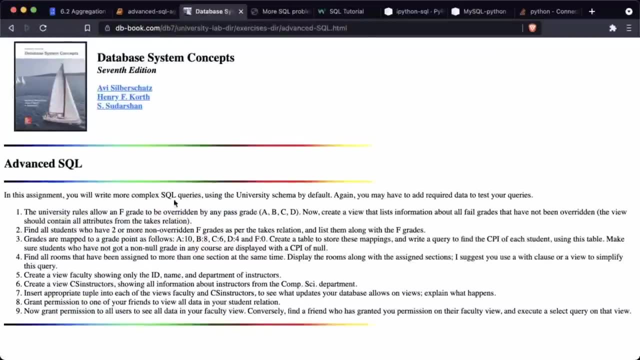 So here you can figure out, there is a basic SQL file, just like the classic models database, And there are a bunch of exercises like: here are some advanced SQL exercises, and this is all based on a university database. So here you have all these. 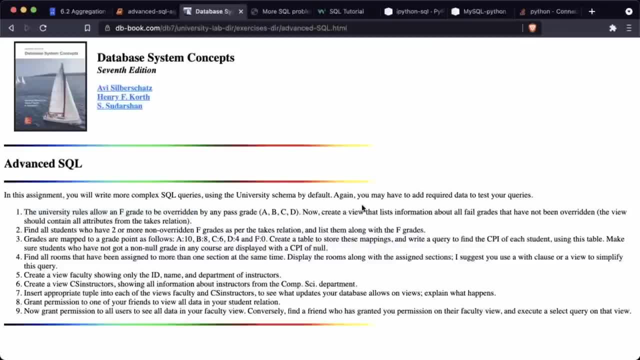 Questions. The university allows an F grade to be overridden by any pass grade. create a view that lists information about all field grades that have not been overridden, and the view should contain all attributes from all the tech, all the takes from the takes relation right. 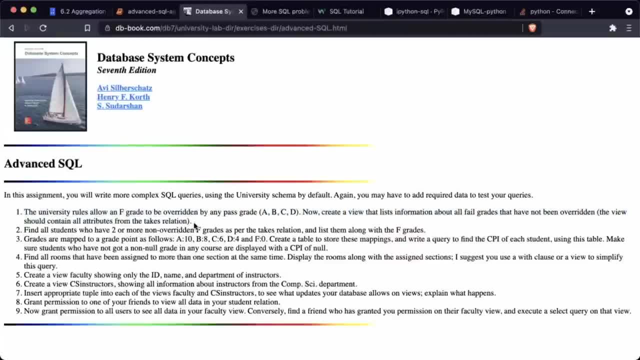 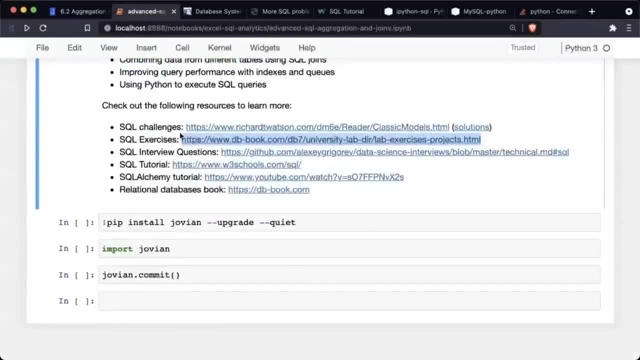 So there's a lot going on here, And, of course, this is more advanced, and then you have some more basic and intermediate questions as well. Right, So these are two good databases: the classic models database and then the student university database. You also have a solutions for the classic models database. 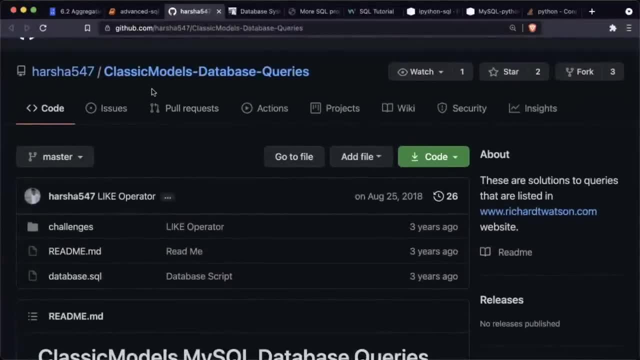 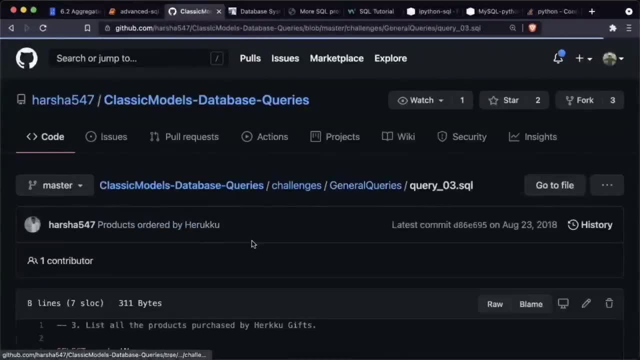 So if you want to check out solutions, this person has a very kindly put up their solutions So you can look up the solutions to the different challenges here. Yeah, So these are some of the solutions for the classic models database. Try that out. 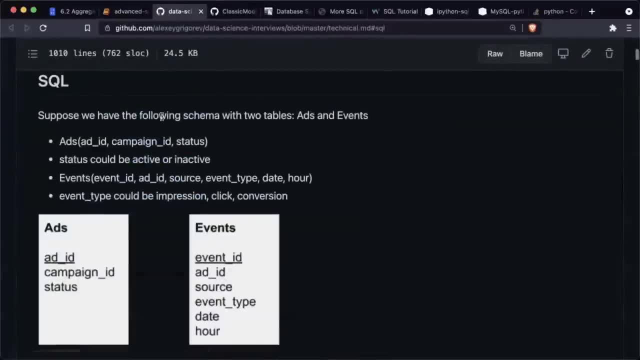 Then you have these interview questions with SQL. This is: uh. this repository has been created by Alexei Grigoryev. He actually did a webinar recently, a few weeks ago with us webinar on machine learning, but he has created this repository called data science interviews. 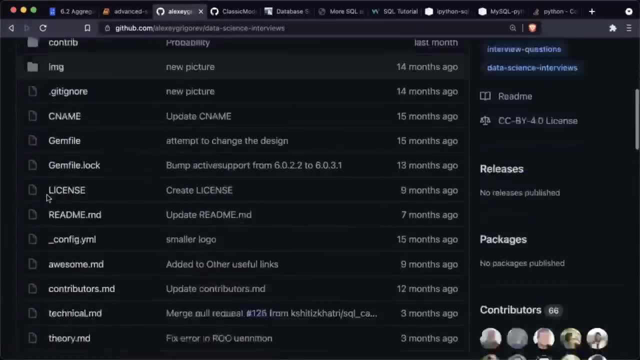 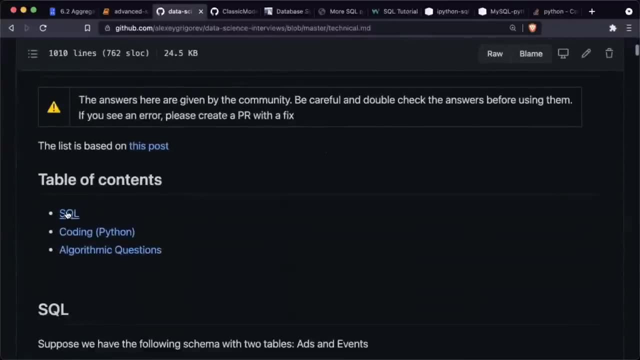 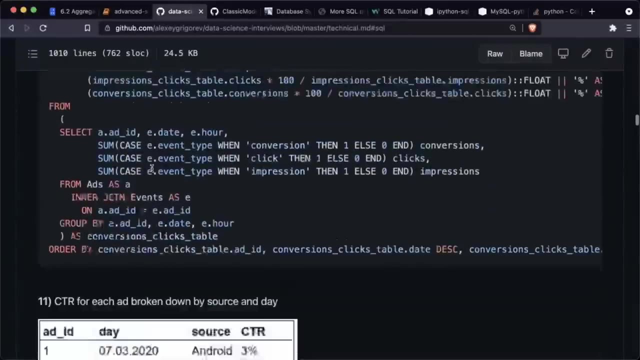 And specifically in this repository you have under technical questions, Yeah, Under technical or MD you have SQL. So just check out a SQL and here you have a bunch of questions. I think probably over 50 or 60 questions, and you can see some of these get pretty big. but the 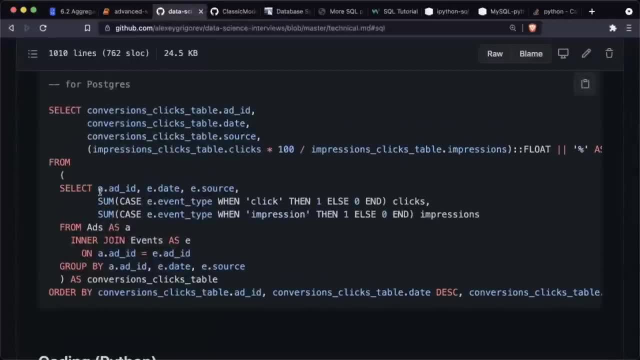 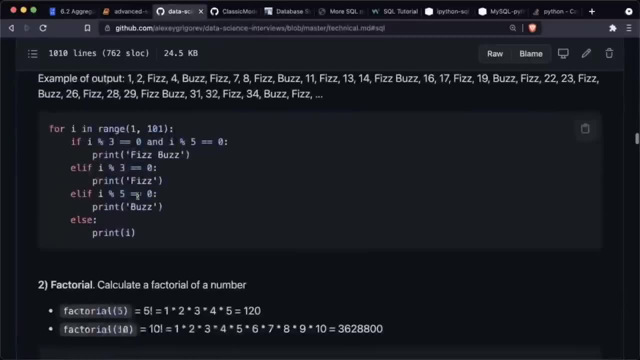 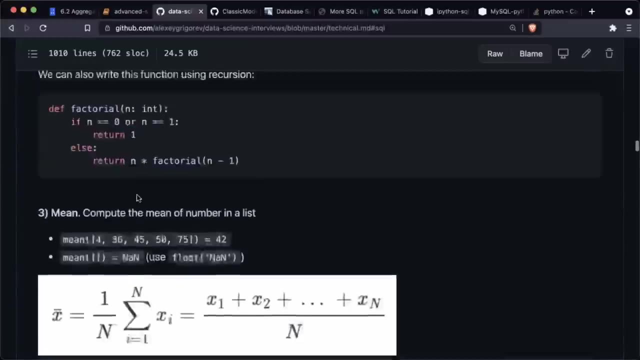 concepts are the same. you see select order by join, and then you're taking the result of one query and then using that as a table in another query, and so on. Okay, So that's SQL for you. Yeah, I think there are, about what's this, 11 questions here, but they cover a lot of different use cases. 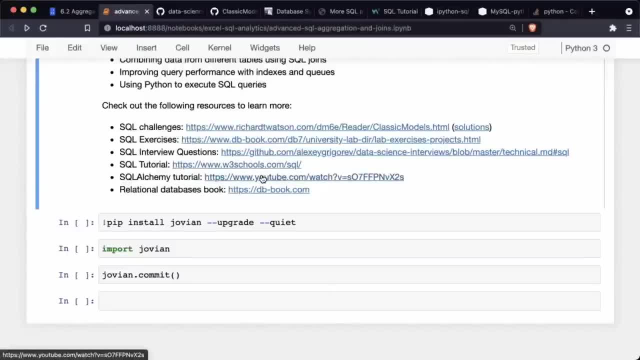 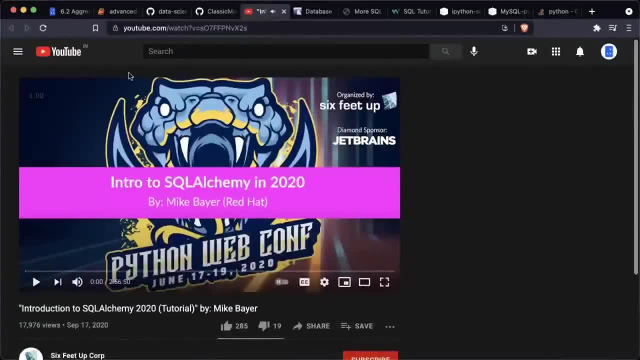 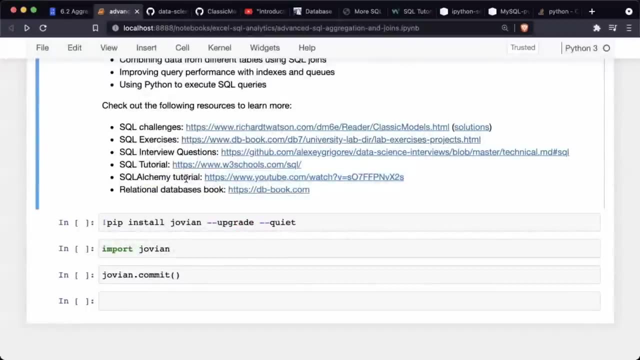 Then W3 schools is a great place to learn. SQL. alchemy is Okay Again if you want to learn more about SQL alchemy, the object relationship mapping- here's one tutorial that I found and went through. It seemed good. Otherwise, reading the official documentation is always the best way in the most comprehensive resource. 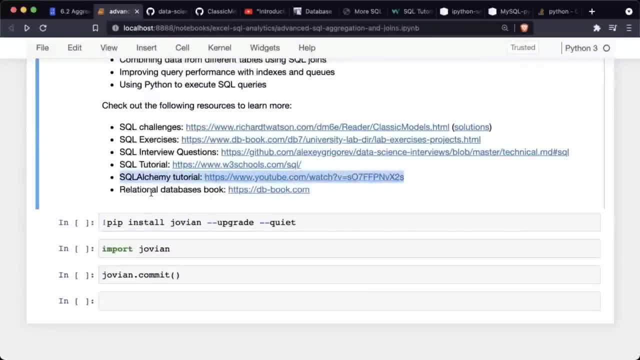 I wouldn't worry too much about this right now. as long as you can just connect to databases and make some queries, you should be fine. And finally, if you'd really want to get a book, then the business book I would recommend. this is the book. 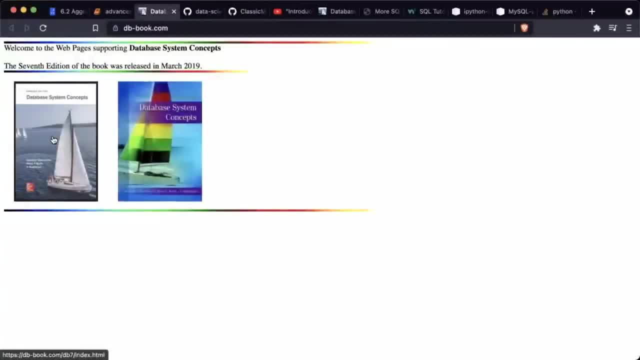 Um, so one of the authors is The professor who I learned SQL under. he was my college professor. but yeah, this book overall is still great And even if you don't want to get the book, I would definitely check out the slides. 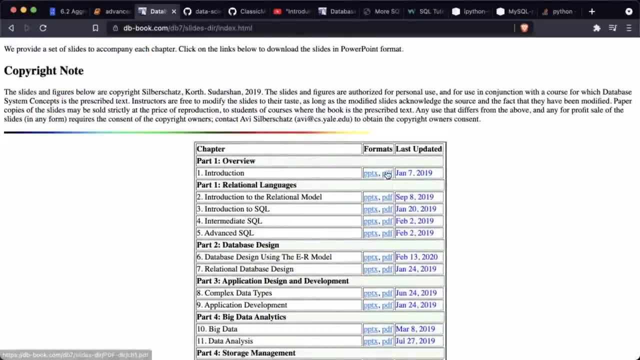 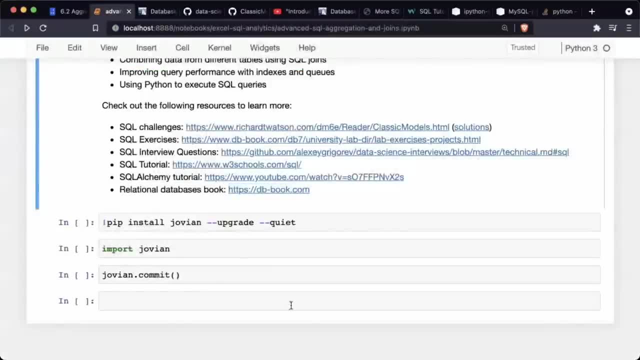 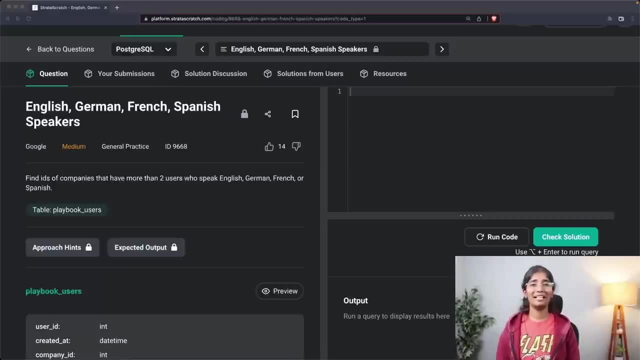 Whenever you want to get deeper into SQL, I would definitely encourage you to check out the slides on this book for sure. Hello everyone, This is someone with a and welcome to the CD solving SQL interview questions, and the CDs will be covering for SQL interview questions that were. 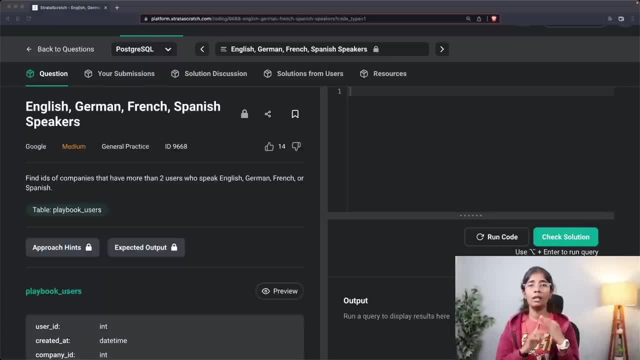 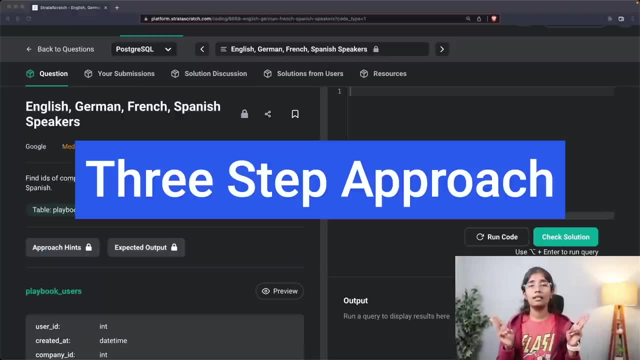 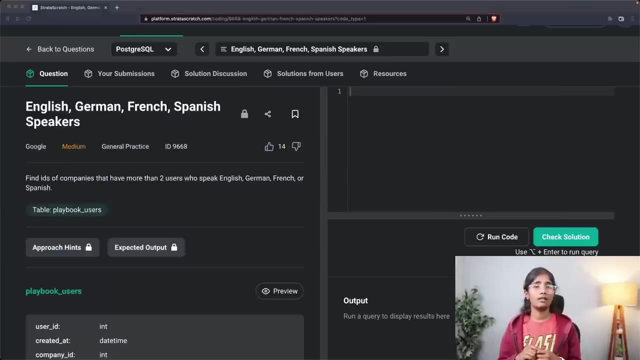 asked that Amazon, Netflix, Uber and Google. before we go ahead and start solving these SQL interview questions, There's something that I'd like to introduce you to first, and that is three-step approach for solving any SQL interview questions. Generally, in an interview, you're not always expected to give the correct answer, but the interview would like to know what is the approach that you have. 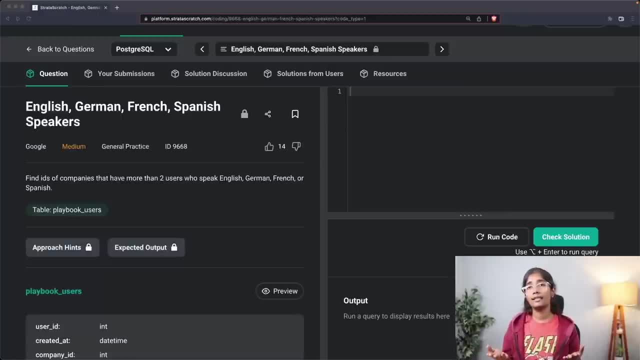 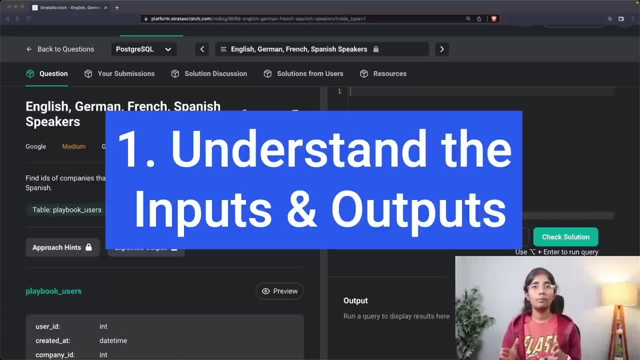 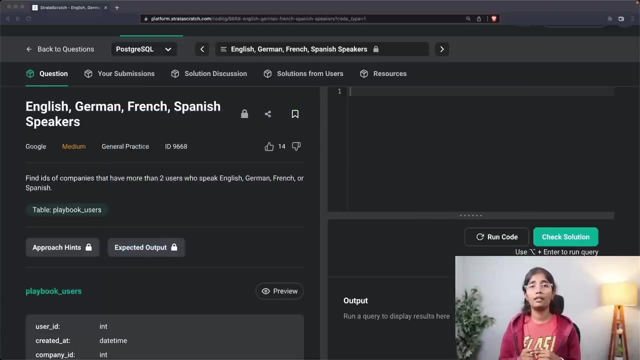 tried for solving a problem, And this is where our three-step approach might help you. step one of our approach is understanding the inputs and the outputs. do not jump into solving the query. As soon as you see the question, understand what are the inputs that you should be using and what are the outputs that your final results should be. 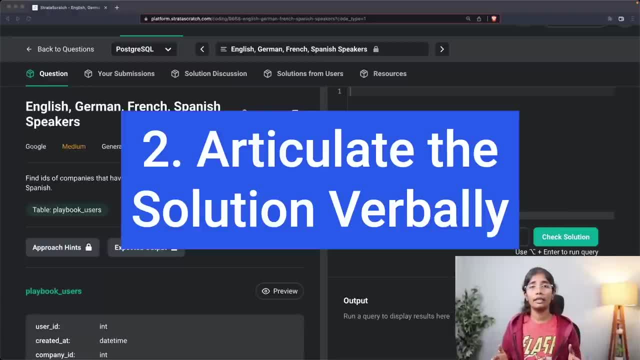 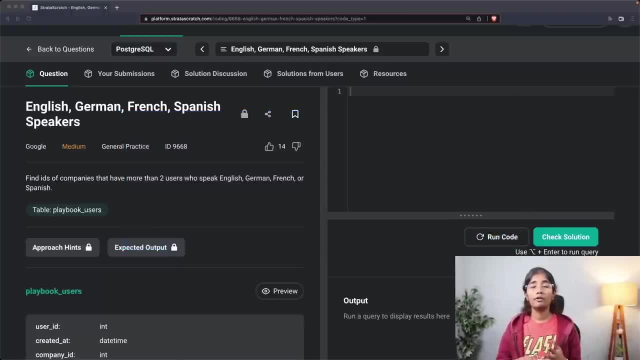 containing step two: articulate your solution verbally. Once you've decided what are the inputs and the outputs, explain your interviewer What is the approach verbally, get a confirmation of your understanding and then start writing: Okay, Your query. step three: construct the query step by step. 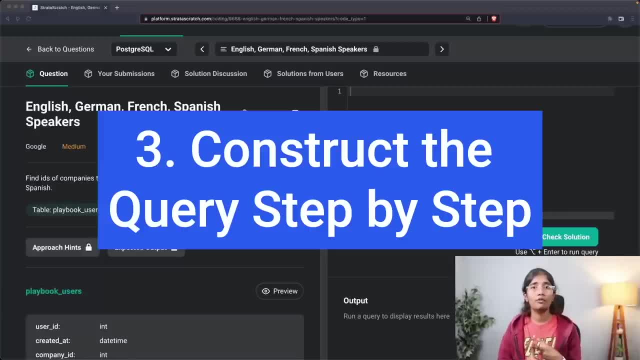 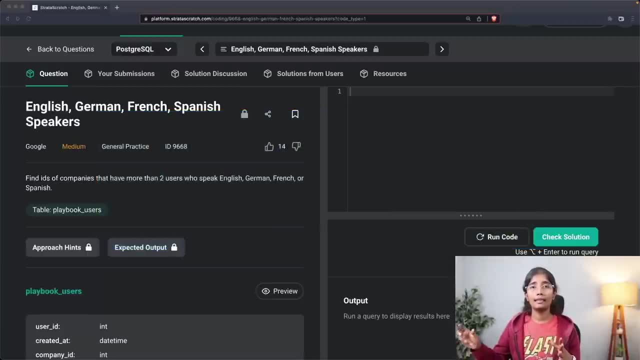 Once you've decided what are the inputs and the outputs, once you've gotten a confirmation of your approach, break down your SQL query into steps and print out the results of these intermediate queries and then improve your final result. So now that you've gotten an idea on how to approach an SQL interview question, let's go ahead and solve one. 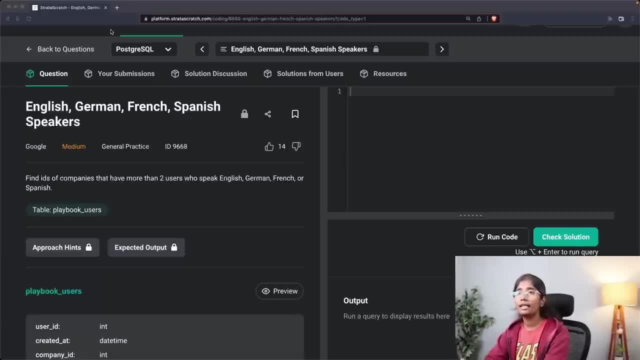 As you can see on the screen, the platform that we'll be using in the entire series for solving the interview Questions is known as the status scratch, And if you look at the screen on the left side, you can see the questions and all the required information that you need to know. 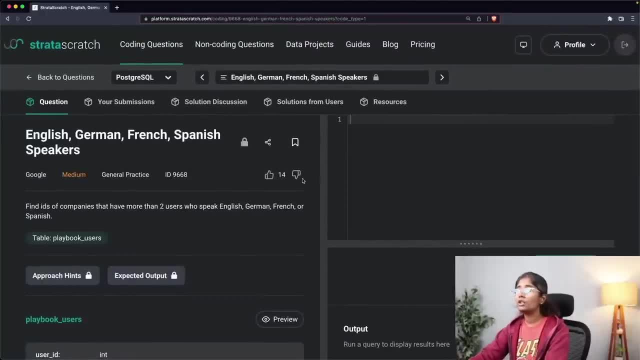 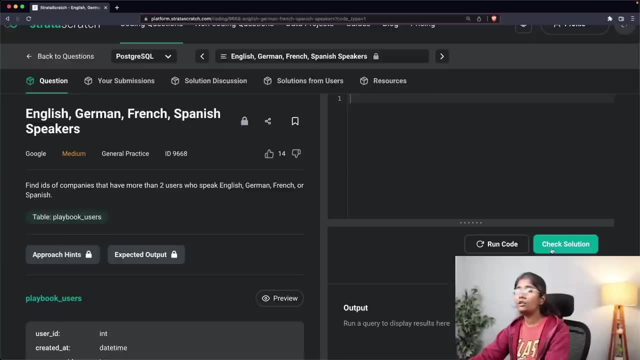 And on the right side you can start writing the query. Now make sure that you're signed into stratascratchcom before you actually run the code, or else you'll not be able to run the code. Unfortunately, you'll not be able to check whether the solution is correct or wrong, but we'll be sharing all the required links for practice and to 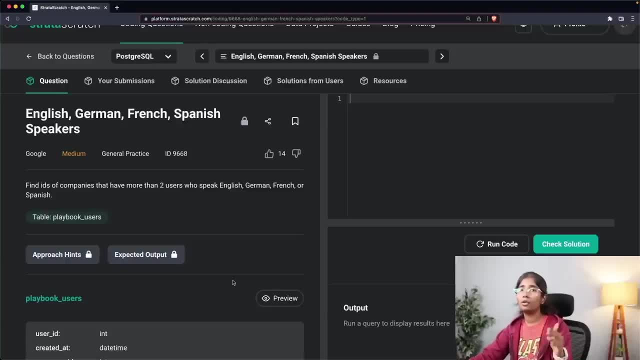 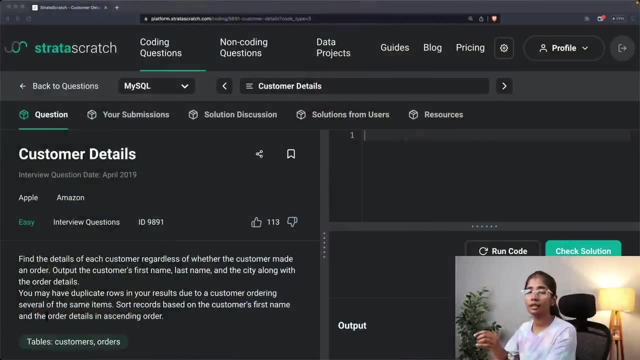 check whether your solution is correct or wrong down in the description, So do not Worry much about it. In this video, we'll be solving an SQL interview question asked at Apple. As you can see on the screen, the problem that we'll be solving today is customer details. 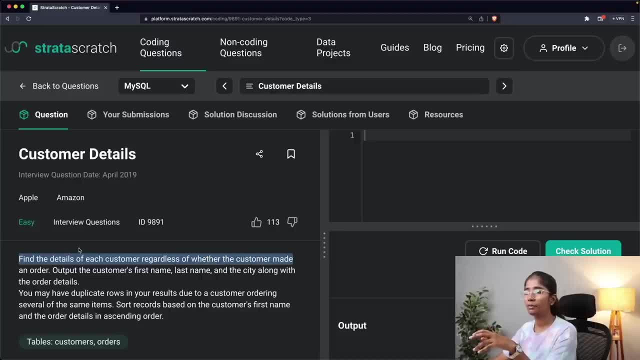 Find the details of each customer, regardless of whether the customer made an order. Output the customer's first name, last name and the city, along with the order details. You may have duplicate rows in your results due to a customer ordering several of the same items. 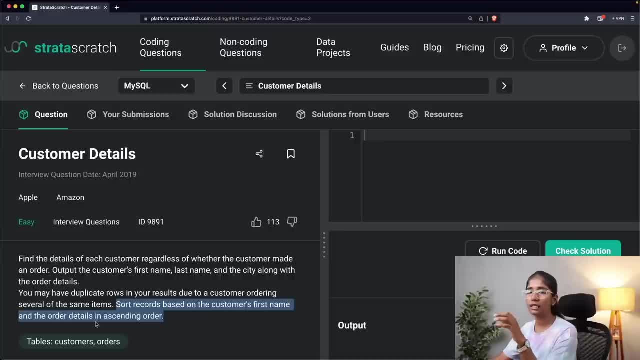 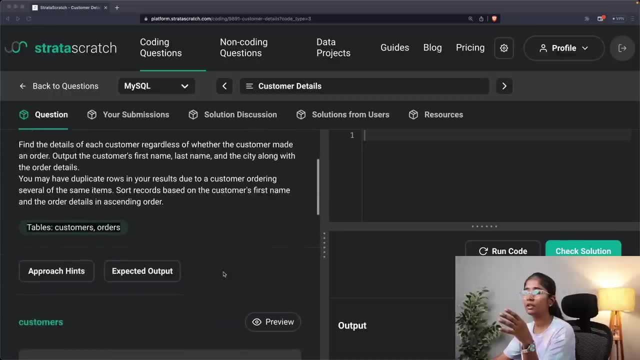 Sort records based on the customer's first name and the order details In S Sending order. As you can see, we have two tables: customers and orders. Let me just quickly have a look at all the columns that are present in both the tables. 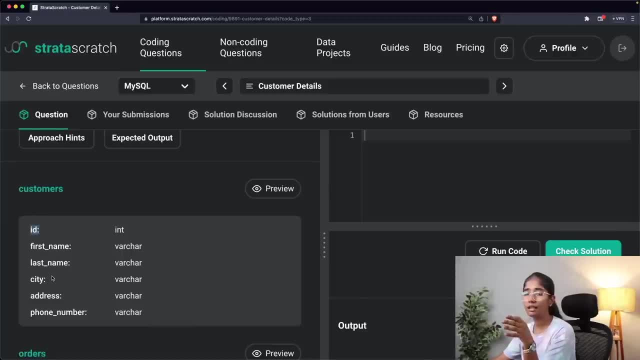 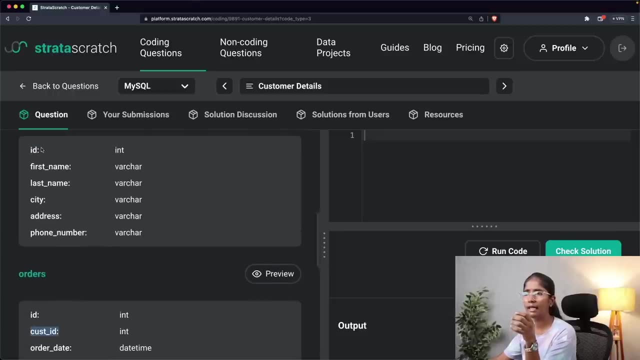 Customers table contains ID- the first name, last name, city, which we want- and the orders table contains ID- customer ID, which I believe this customer ID is the same as the ID present in the customers table- and order date and order details, which, again, is something that we want. 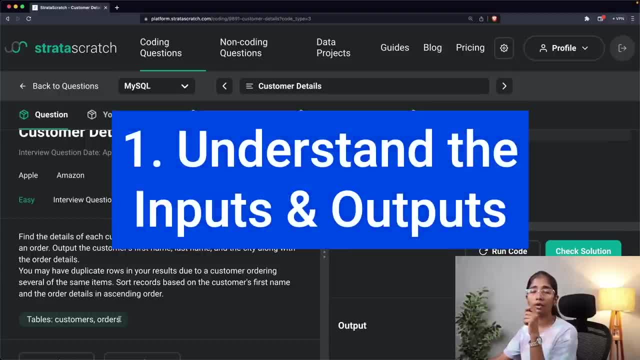 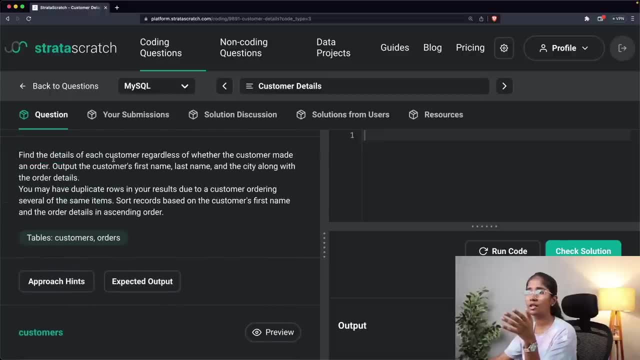 According to our approach, the first step of solving an interview Question is understanding the inputs and the outputs. Now, what are our inputs? Since, I said, find the details for each customer, regardless of whether the customer made an order, I'm going to use the customer ID as one of the inputs. 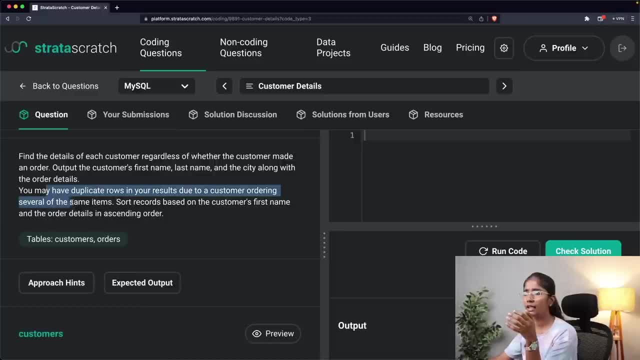 And they have mentioned what the output should contain, And they've mentioned that it will contain some duplicates. Now they also said to sort records based on the customer's first name and the order details, So my inputs will also contain customer's first name and order details to perform the sorting. and the output should contain: 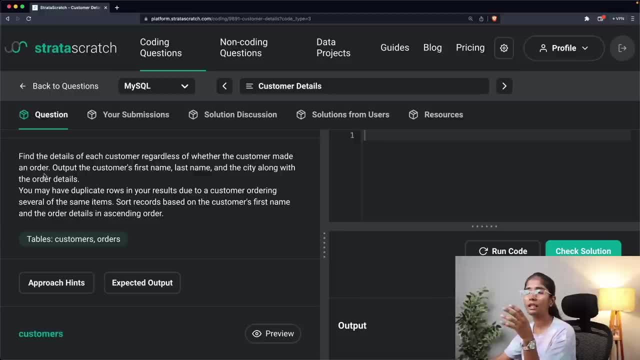 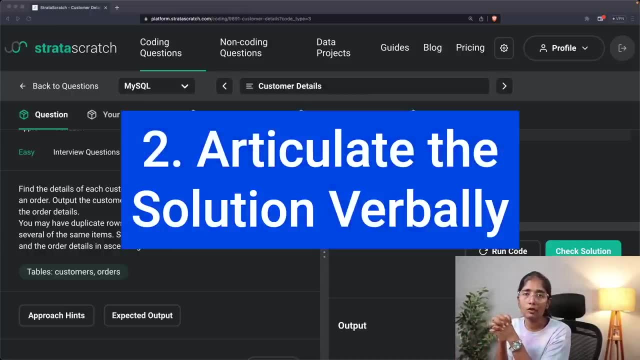 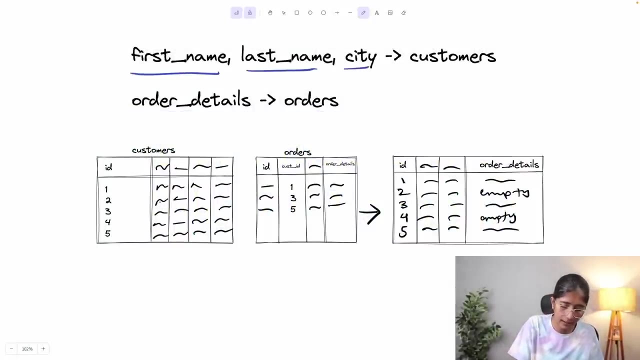 Customer's first name, last name and the city, along with the order details. So these are going to be my inputs and the outputs. The second step of our approach is articulating the solution verbally to the interviewer. In our approach, we have established that the output should contain first name, last name, city, which is coming from the customer's table. 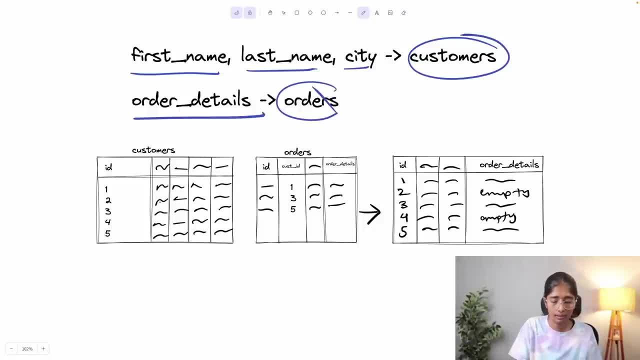 And it should also contain order details, which is coming from the orders table, which means we have to combine both of the table results to get the final output, And for that I can Perform a joint. Now, what joint do I have to perform? 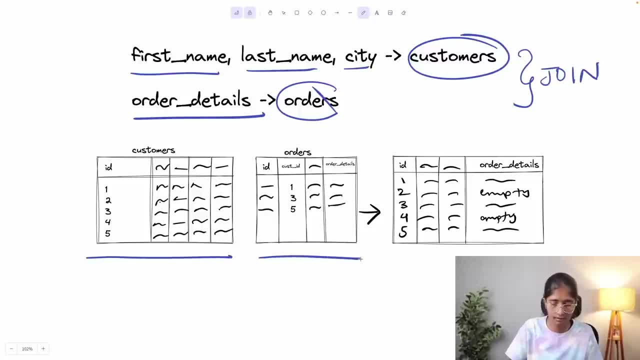 Given that I'm joining customer's table on the orders table, I'll have to use a left joint so that I'll get all the customer details present in the customer's table, irrespective of whether they've made an order or not. And that's what the question states. 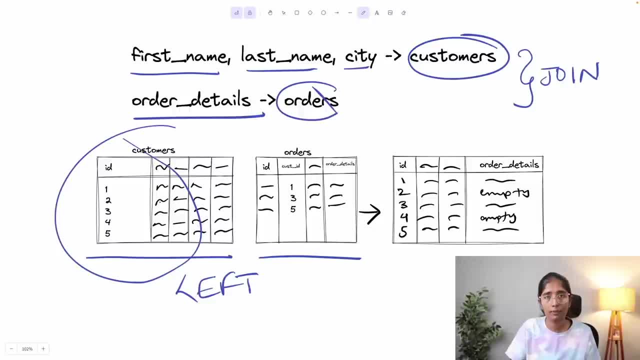 So I'll be performing a left joint on the customer's tables with respect to the orders table to get the final output result. Finally, they've also mentioned that we have to order it by first name And also order details. So this is going to be my approach. 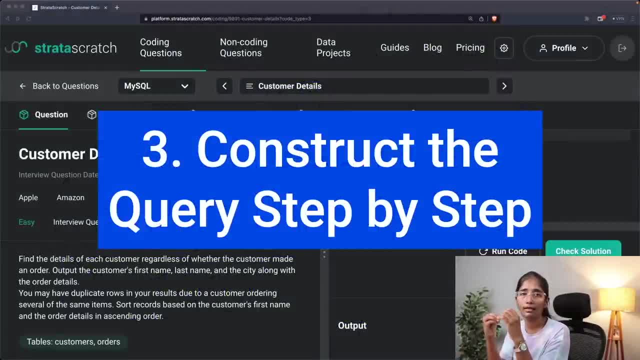 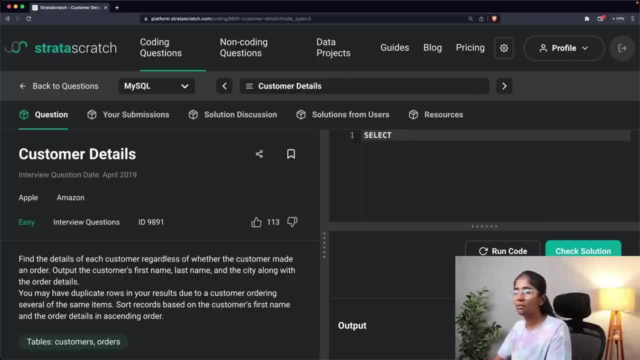 Now the third step of our approach is constructing the query step by step, And the first part of our query construction is performing the joint Select, since my output should contain first name, last name, city and the order details. These are the column names that will be present in the select statement. 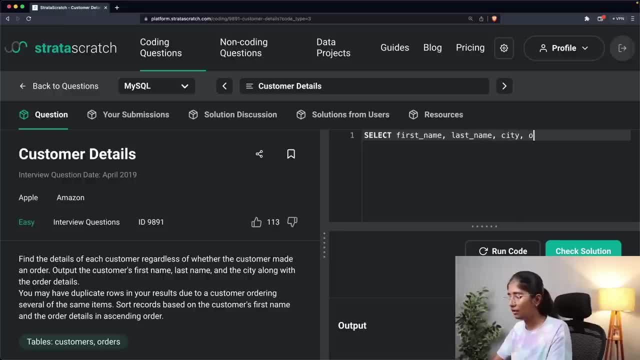 First name, last name, city order Details from customers left join orders on customersid is equal to orderscustid, because we have established that customer ID is the ID that is common and similar to the ID in the customer's table. So let me just run this. 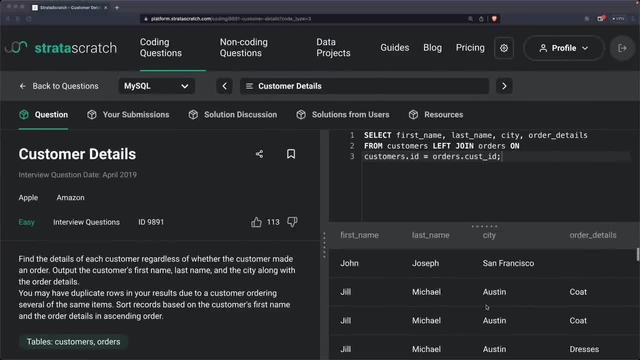 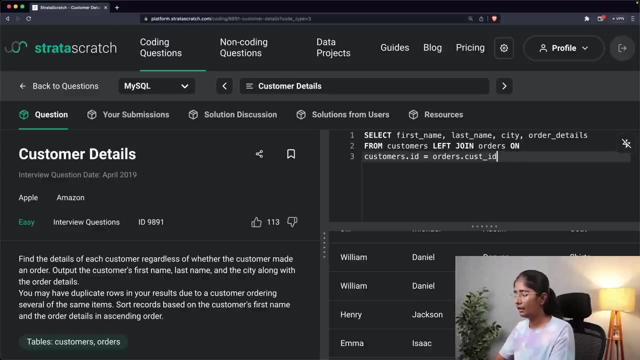 As you can see, the left join has been perfected And whenever there is a customer who made an order, the order details value is filled, And if that customer has not made any order, that order details section is empty. Now the second part of our query construction is ordering this by order details and the customer's first name. 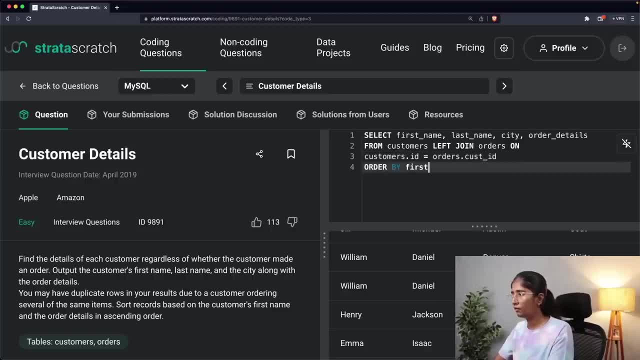 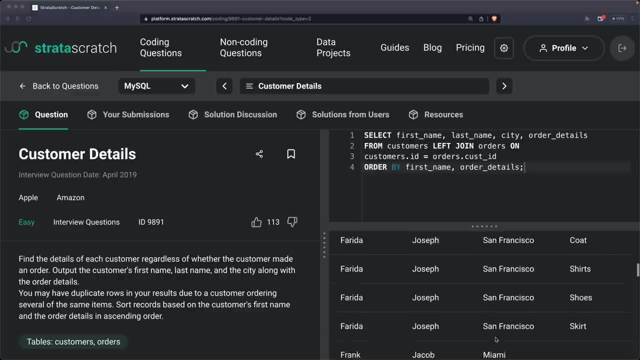 So I'm just going to say order by first name, order details, And I'm going to run this. As you can see, the order details has been ordered according to the first name and then followed by the order details. So yeah, that's what they've been asking us in the question. 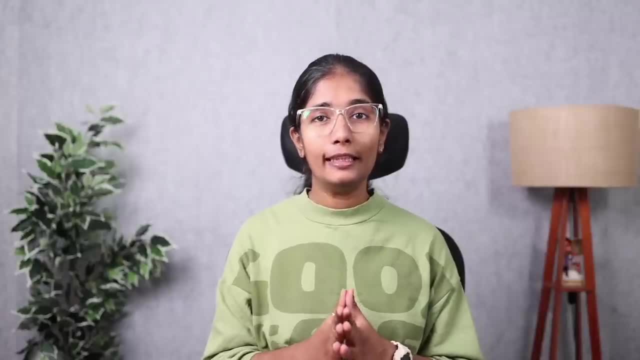 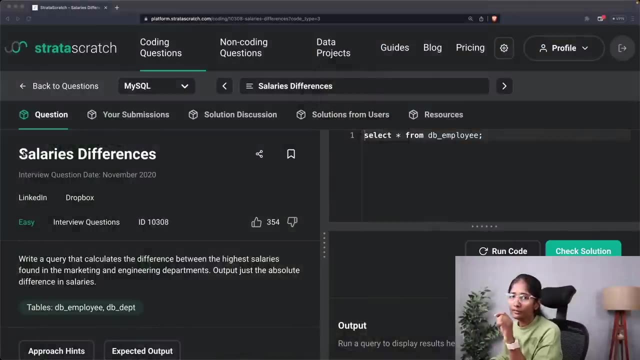 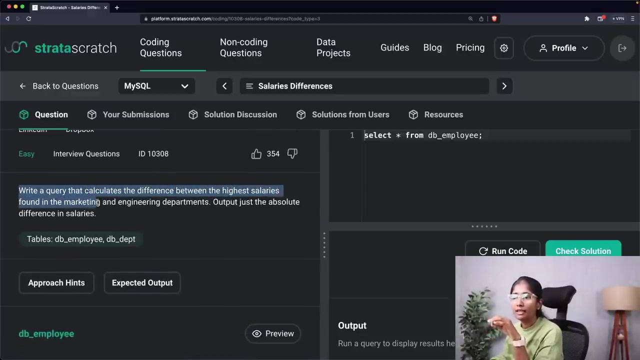 Thank you so much for watching. Welcome to the series solving SQL interview questions. In this video we'll be solving an SQL interview question asked at LinkedIn. The problem that we're solving today is salaries differences. Write a query that calculates the difference between the highest salaries found in the marketing and engineering departments. 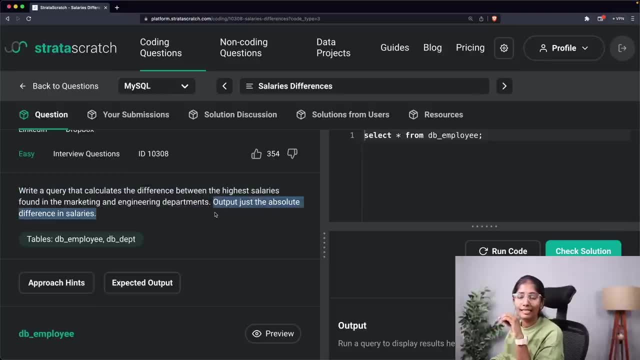 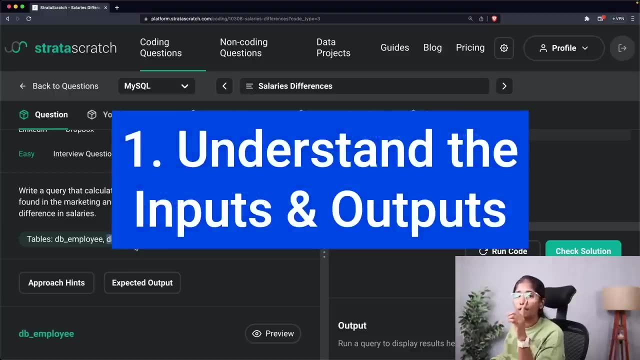 engineering departments Output just the absolute difference in salaries, and the tables that are given to us are DB employee and DB department. According to our approach, the first step of solving the SQL question is understanding the inputs and the outputs. For that I quickly just 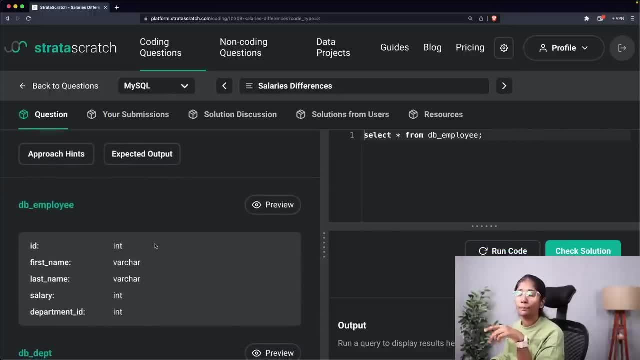 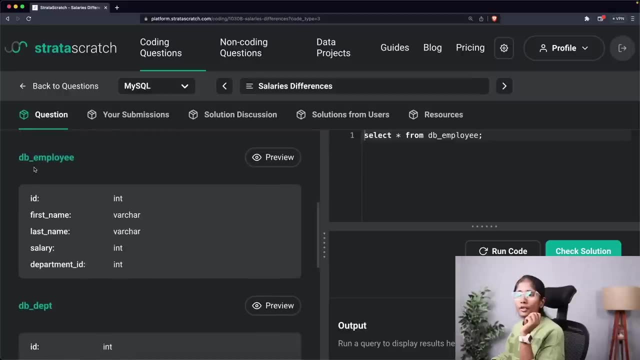 want to have a look at all the columns that are present in these two tables so that I'll know what inputs I have to give to the table to get the salaries difference output. As you can see, it contains ID, first name, last name, salary. So since they asked us to calculate the highest, 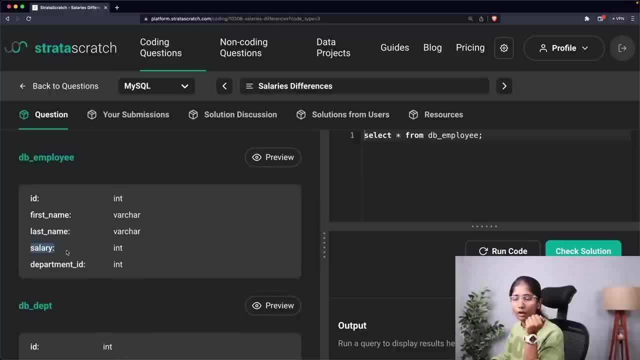 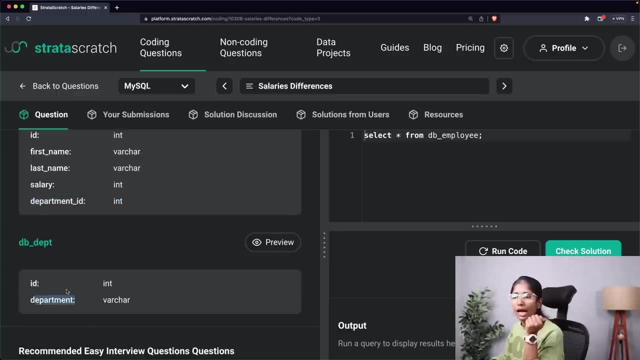 difference between the salaries. I'm going to use the salary column as my input and there's department ID and in the DB department table I have ID and the department. I believe this ID is similar to the department ID present in the employees table and, as they mentioned in the 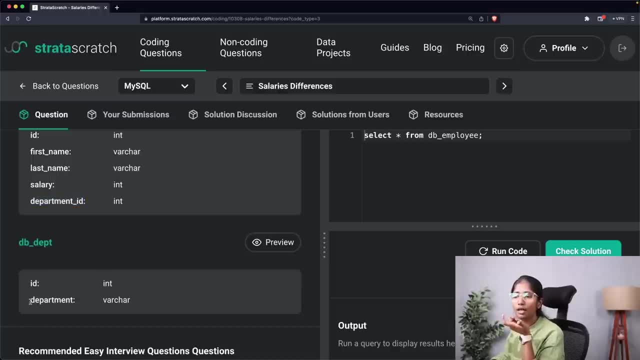 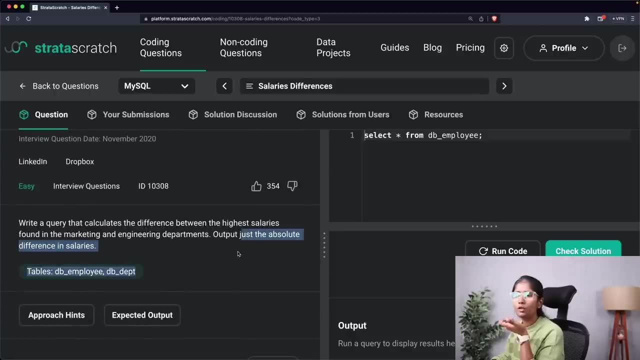 question they want specifically for marketing and engineering departments. department is going to be my other input. What is going to be my other input? I'm going to be my other input. I'm going to be my output Output just the absolute difference in salaries. So these are my inputs. 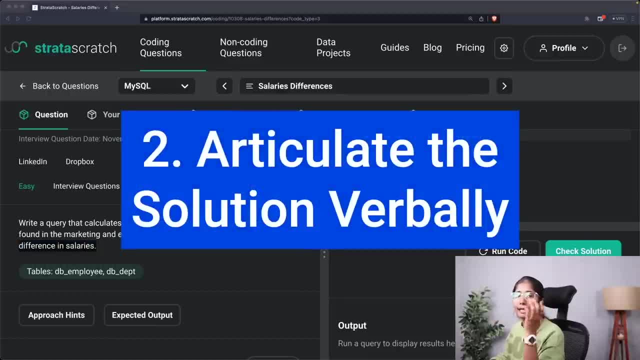 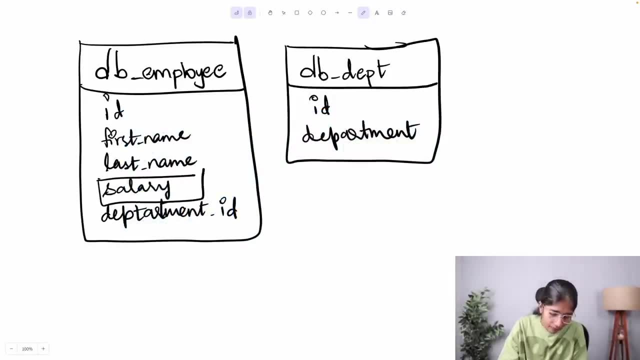 and the outputs. Now the second step of our approach is articulating a solution verbally to the interviewer, As we've discussed that, the columns that we'll be using are salary and the department, and what they've asked us to calculate is the highest difference of the salaries between 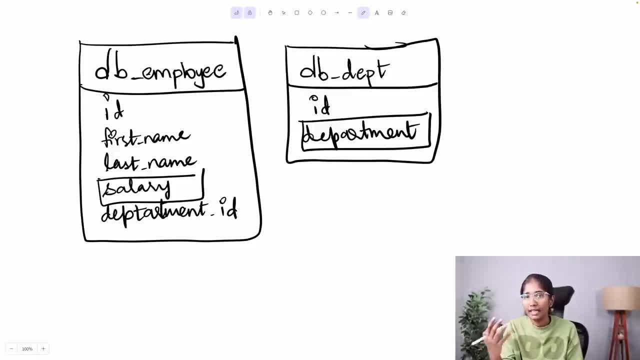 the departments marketing and engineering. So when they're saying highest, you probably are expected to use the highest difference between the salaries. So when they're saying highest, the aggregation function max in the each department and calculate the difference between them. So 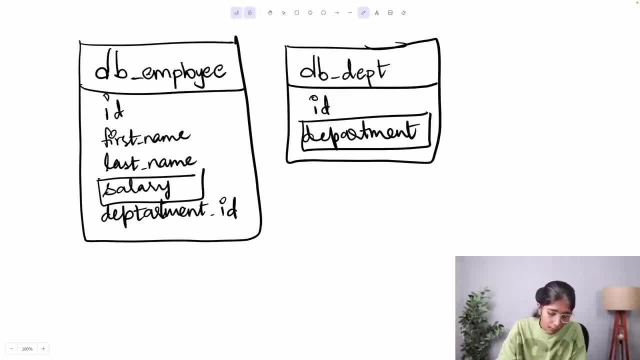 my approach is probably going to be. first thing, I'll perform a join between the DB employee and DB department so that I can get the department name, and the first thing I'll do is write a select statement which will get me the maximum salary from the department marketing, and I'll write. 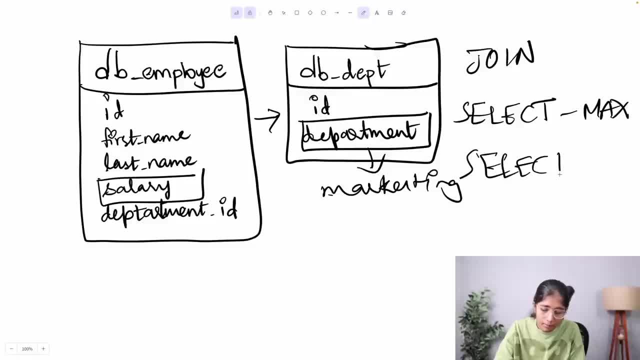 another select statement which will get me the maximum salary from the department engineering, and then I'll calculate the difference between this select statement and the other select statement. get the absolute difference, and that's what they're looking for. There's also another way that you can approach this problem. 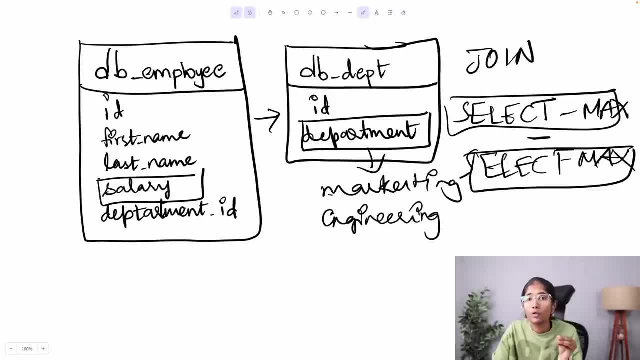 without having to use two select statements, and that is by using a self-join with the help of table aliases. Now, right now, we're performing a join of DB employee with DB department so that we can get the department name. Okay, what if we know what is the department ID of the department names? marketing and engineering. 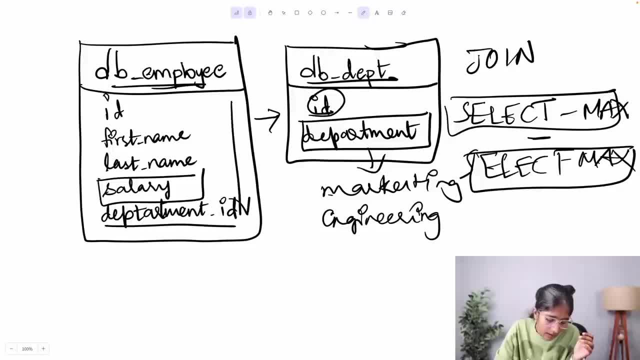 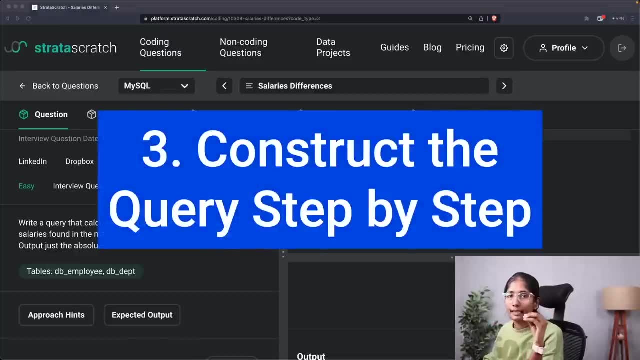 we can simply just use this department ID within this table, calculate the maximum salary of that particular department and minus it with the maximum salary of the other department by performing a self-join. Now the third step of our approach is constructing the query step by step. 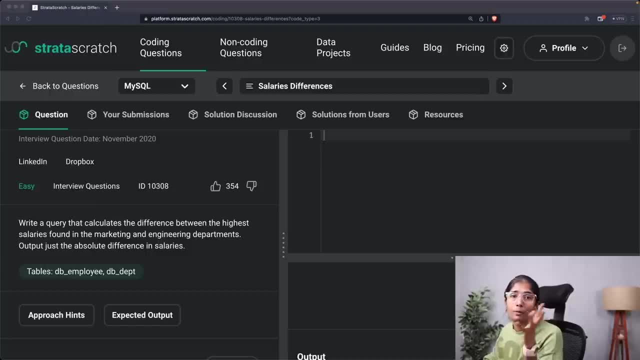 and the first part of our query construction is calculating the maximum salary for the department's marketing and engineering. So for that I'm just going to say: select max of salary from DB employee join with DB department on dbemployeedepartmentid is equal to dbdepartmentid and I'm going to give 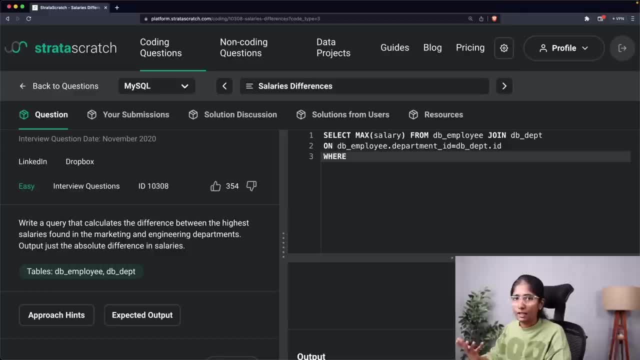 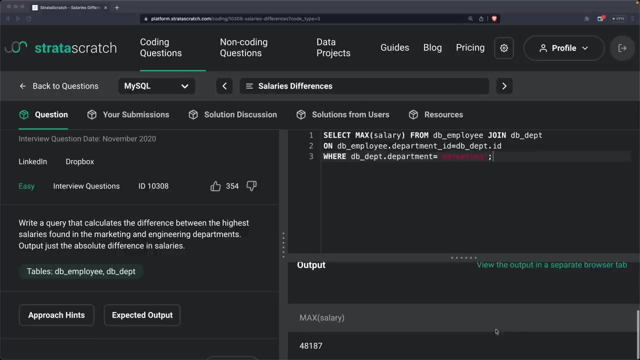 the where clause for the department. So I'll get that specific department maximum salary where dbdepartment is a code. Okay, so I think I should say dbdepartmentdepartment is equal to marketing. So let me just execute this And, as you can see, I 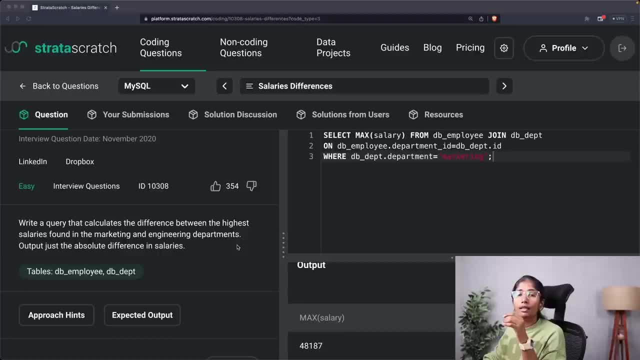 now have got the maximum salary for the department marketing. Similarly, I'll also be calculating the maximum salary of the department engineering, and then I'll get the absolute difference between these two select statements. So for that, what I'm going to do is I'm going to put this entire statement in one bracket, then I'm going to 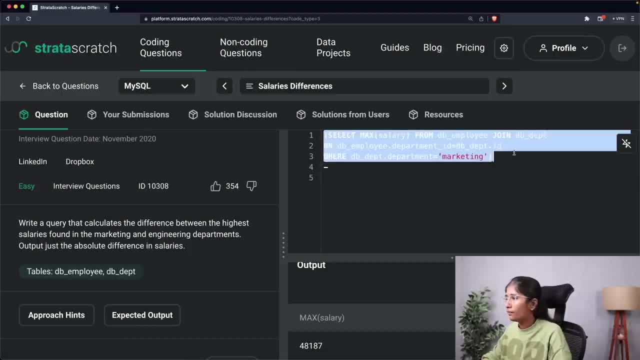 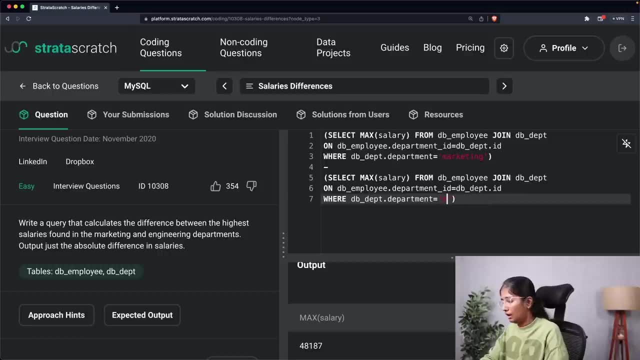 do minus and I'm going to copy paste the same syntax here, because it's almost the same thing except for the marketing name. Instead I'm going to say engineering. So these are the two style statements and i'm going to perform absolute difference between these select statements. 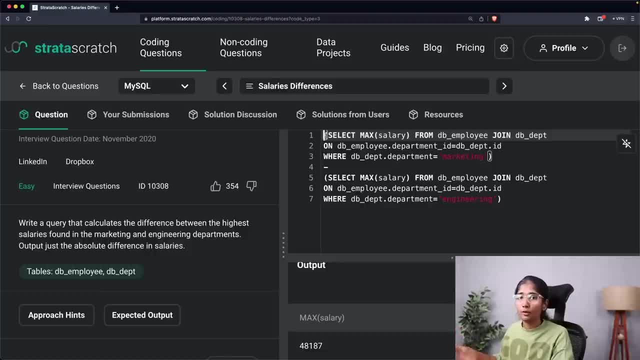 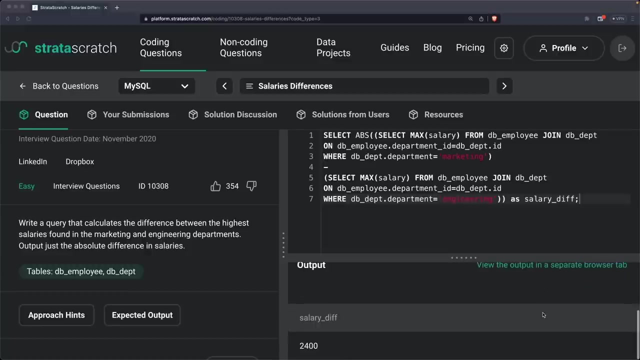 so that i will get the difference between the highest salaries of the departments. so i'm going to say select absolute difference of these and i'm going to give this an alias name as salary tiff and then i'm going to execute this. as you can see, we now got the absolute highest salary difference of the departments. 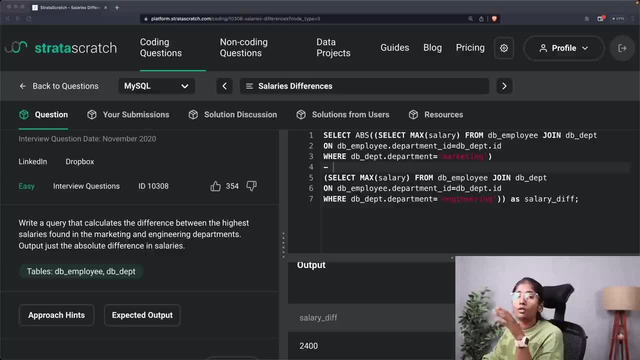 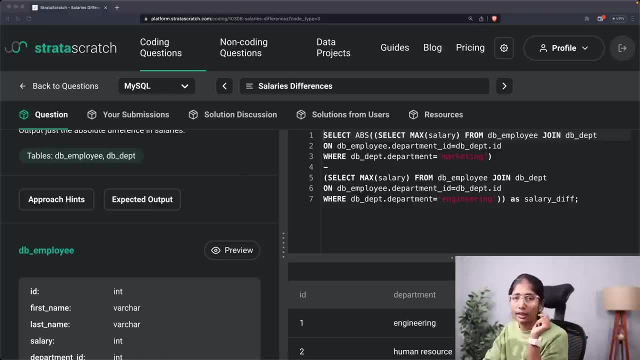 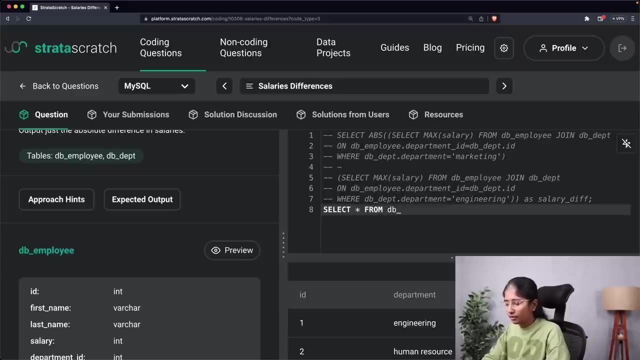 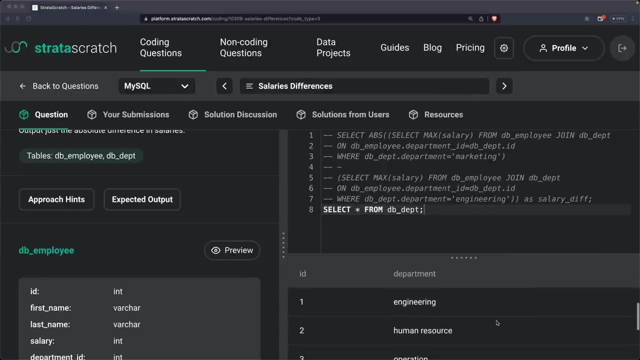 marketing and engineering. so this is one way of our approach. as we've discussed, there's another way of approaching the same problem, which is by using a self-join. first, let me just see what are the department ids for. the department names marketing and engineering. so i am just simply going to run this and, as you can see, engineering is having the department id1. 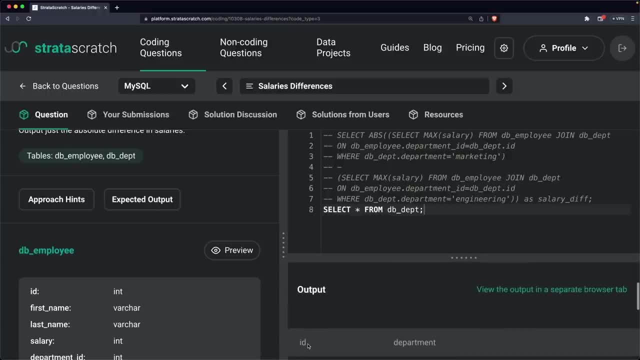 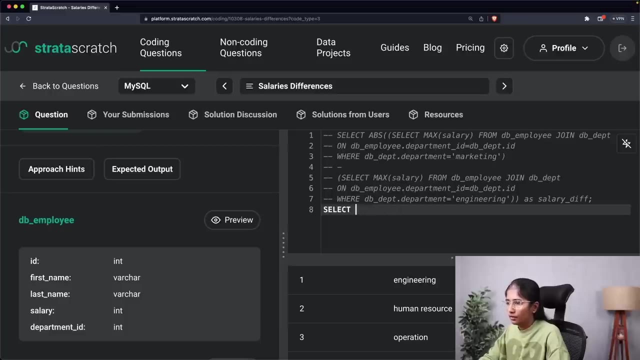 and marketing is having the department id4. so using these numbers in the department id column of the db employee i will perform a self-join to calculate the highest difference. so for that i am going to say select max of a dot salary minus max of b dot salary and i'm going to give this as salary difference. 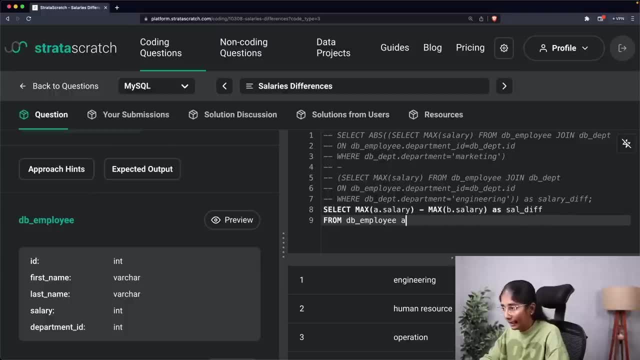 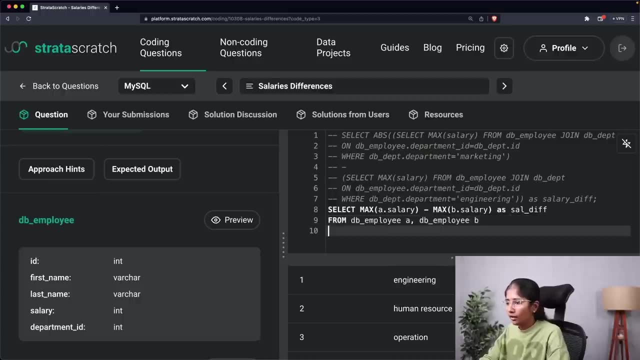 from db employee a and i'm performing the self. join here db employee b using table aliases: where a dot department id which is equal to 1.. where a dot department id which is equal to 1.. one and b dot department id is equal to four, one is for engineering and four is for marketing. 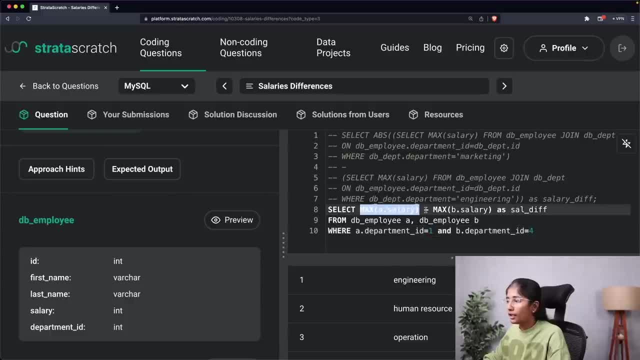 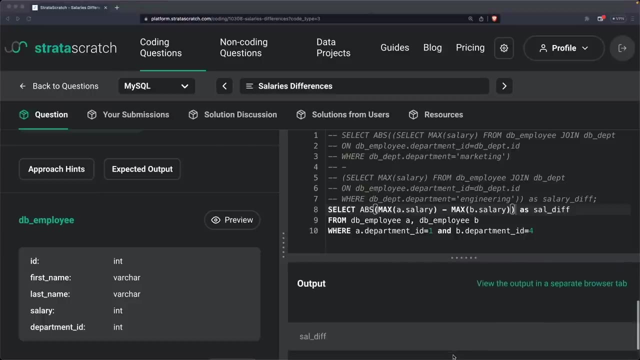 and i'm calculating the maximum salary of the engineering and maximum salary of the marketing and i'm performing the difference and since they said they want the absolute difference, i'm going to say absolute of this and then run the score and, as you can see, we got the same answers. so yeah, that is how you approach these kind of sql interview questions. 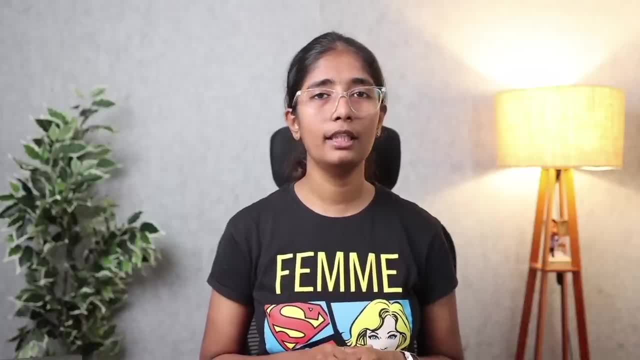 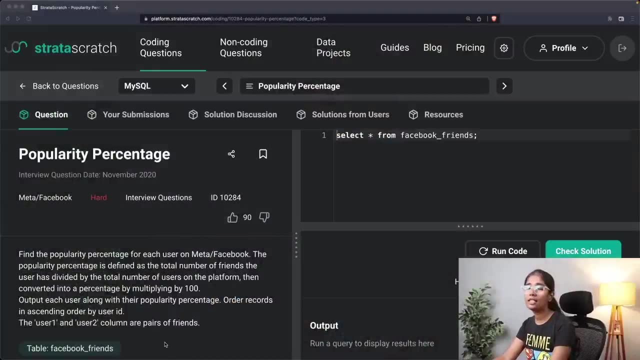 thank you so much for watching. in this video we'll be solving an sql interview question asked at facebook, which is a part of meta. let's go ahead and start solving. as you can see on the screen, the problem that we'll be solving today is popularity percentage. 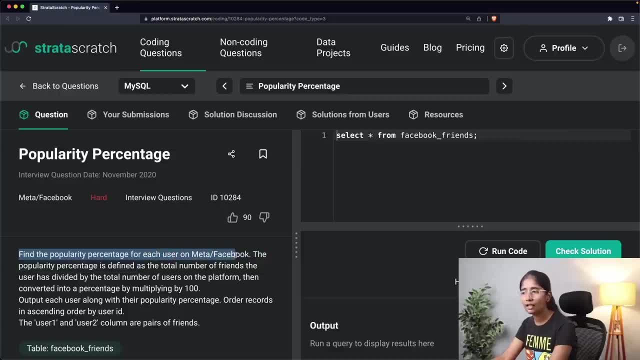 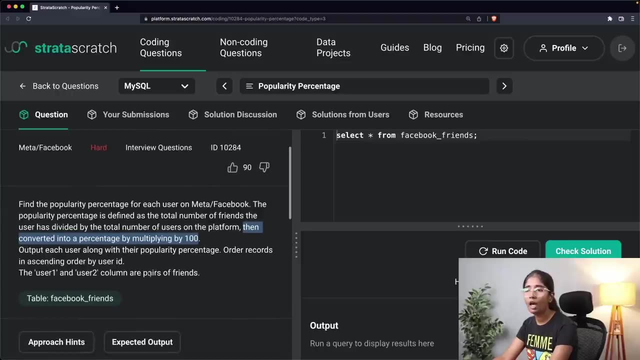 find the popularity percentage for each user on meta facebook. the popularity percentage is defined as the total number of friends the user has divided by the total number of users on the platform, then converted into percentage by multiplying by 100. output: each user with their popularity percentage. order records and ascending order by user id. 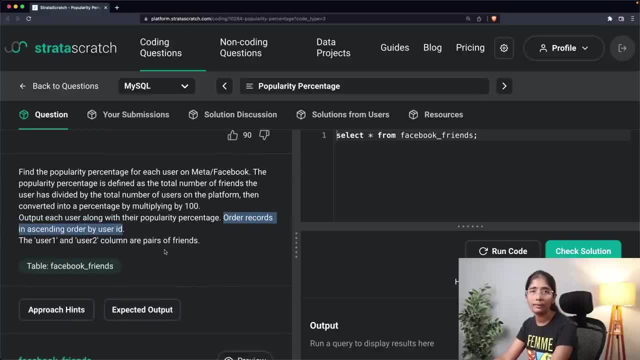 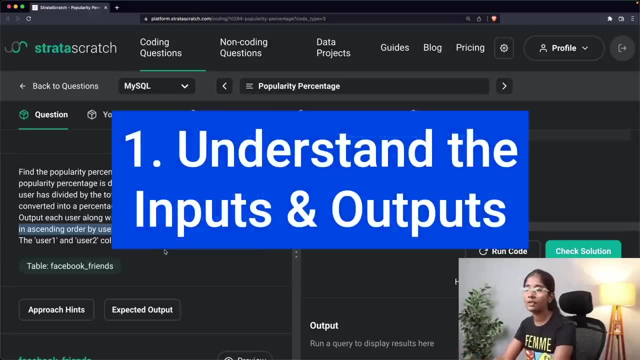 the user one and user to column are pays of friends. so, according to our approach, the first step of our query construction is understanding the inputs and the outputs. let's go ahead and take a quick look at the table and we can see that it is user 1 and user 2. 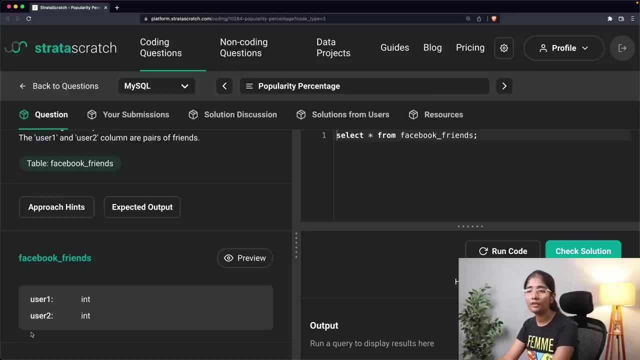 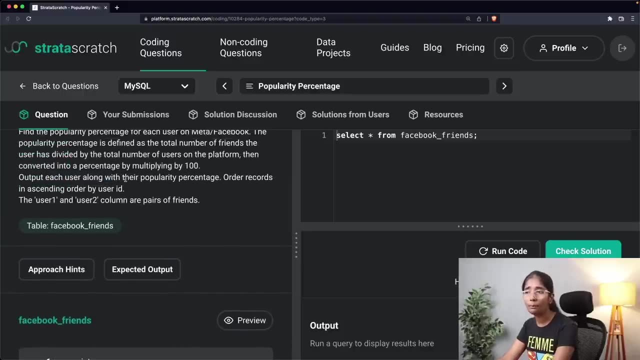 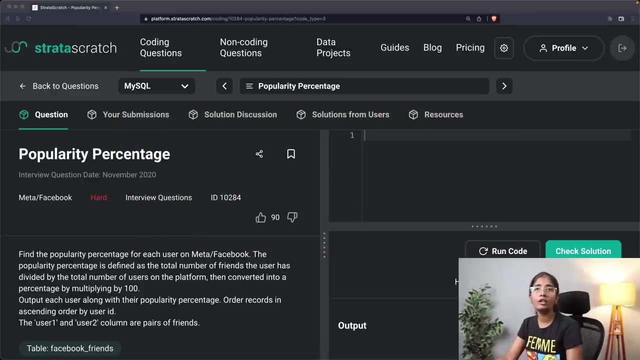 and these user 1 and user 2 columns are pairs of friends, so we have to use both user 1 and user 2 as our input columns, and the output should be each user along with their popularity percentage. now the second step of our approach is articulating a solution verbally to the interviewer, according 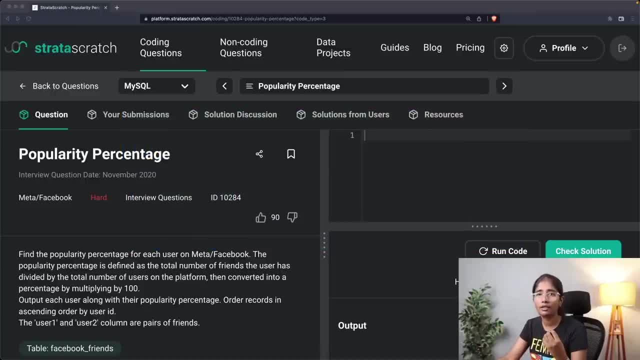 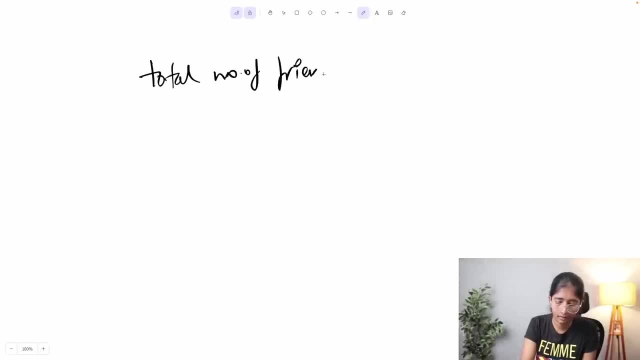 our approach. they've asked us to calculate the popularity percentage right, which is basically total number of friends a user has divided by total number of users on the platform into 100. before we actually multiply with 100 and get the percentage, we first need to figure out how to calculate the total number of friends a user has and also the total number of users on. 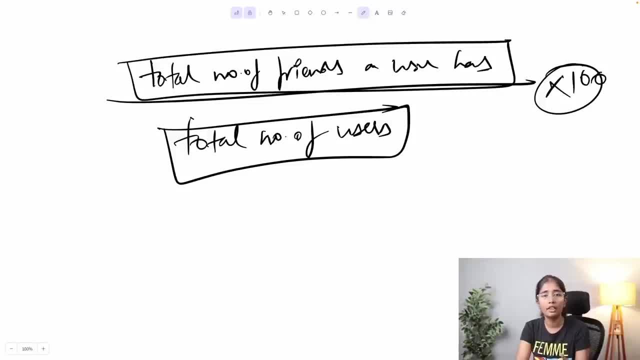 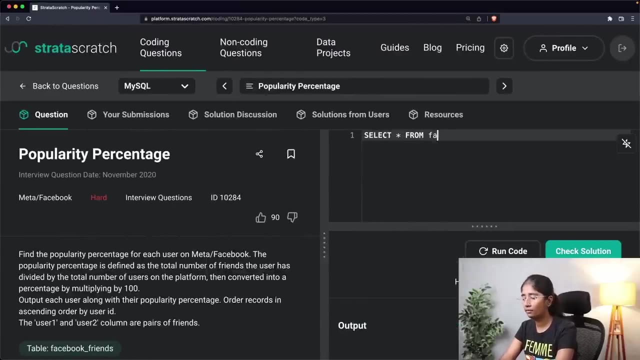 the platform. before i figure out what method or function i need to use to calculate the total number of friends a user has or the total number of users, i just want to have a quick look at how the data is in the table for that. i'm just going to come back here and see select star from facebook. 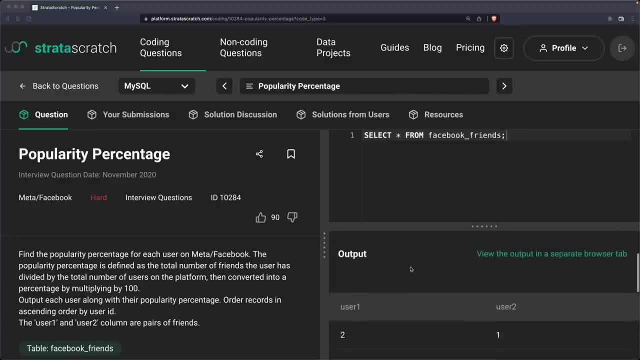 i'm going to run this and i'll. you can see there is user 1 and user 2, where user 1, 2 is friends with user 2, 1 and 1 is friends with 3 and 4 is friends with 1. this seems to be a little confusing for me to calculate a total. 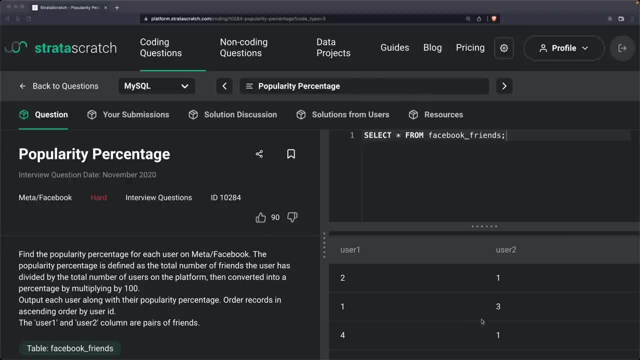 number of friends a user has, because seems like one is spread across both the columns and i can understand that the rest of the you know users are also spread across like that. so for my better understanding, what i want is if i can have all the ones on the left side and their friends on the 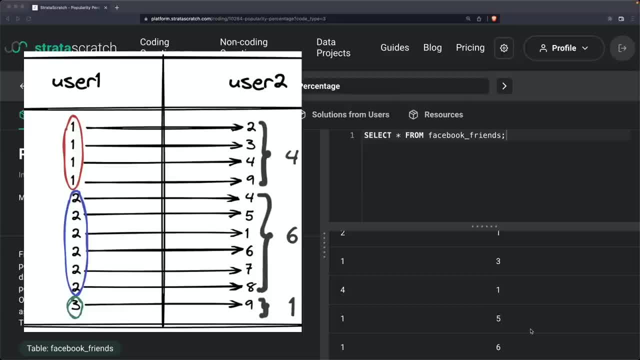 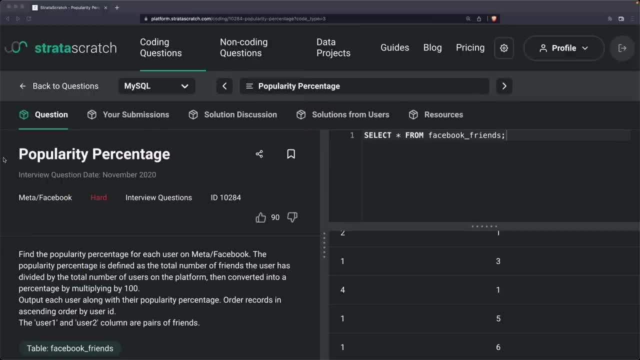 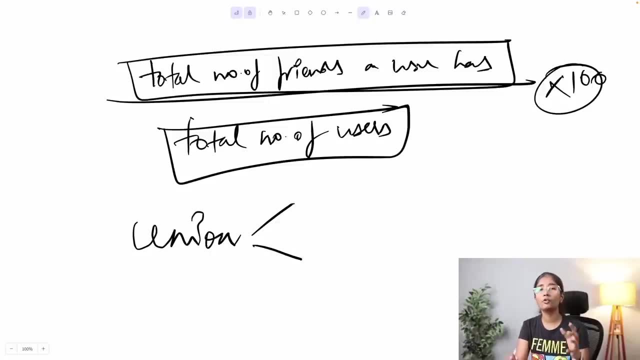 right side and all the twos on the left side and their friends at the right side, it is easier for me to calculate the total number of friends a user has, and for that the thing that comes to my head is union. so union is basically a method used for you to combine the results of two select 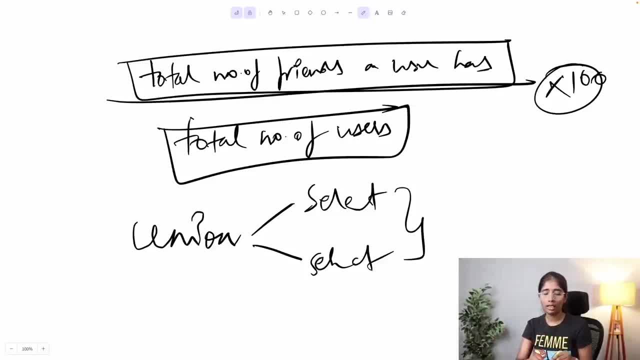 statements and removes any duplicates present in it. so that's how union works. so that is going to be my approach for calculating the total number of friends a user has. now the second step should is calculating the total number of users. so if i'm having all the users on the left side and 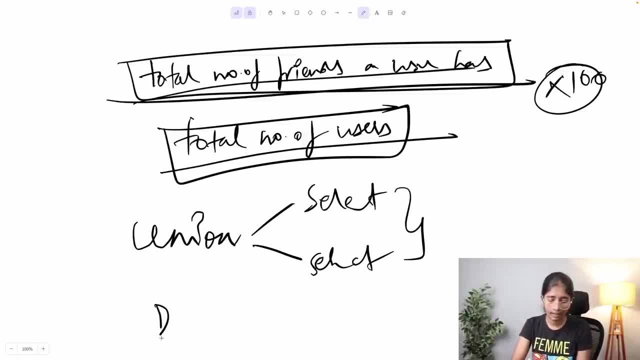 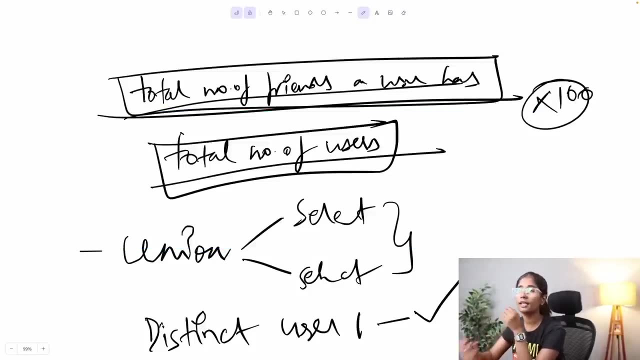 their friends on the right side. i can just simply say distinct of user one right that should probably give me the all existing users on the platform. now the third step of our approach is constructing the query step by step, and the first part of our query construction is calculating the total number of. 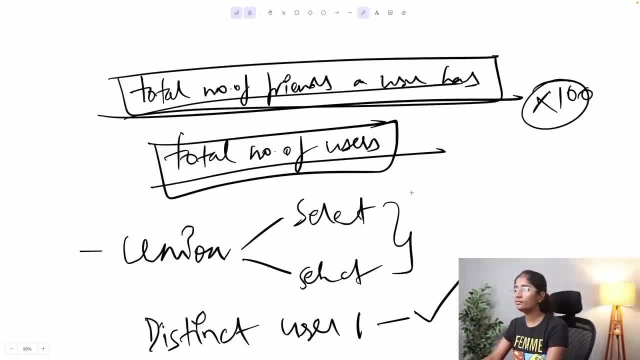 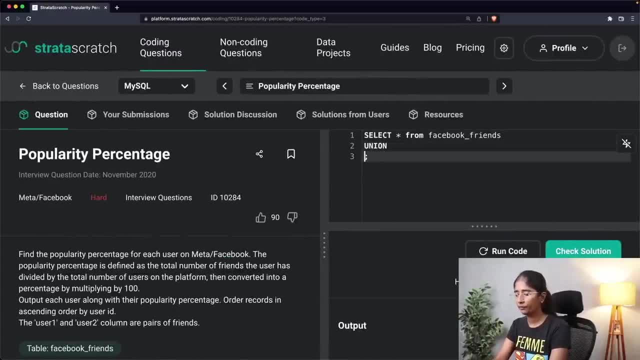 friends a user has. let me just go back to my query editor to write that query. first, i already have select staff from facebook friends. i'm going to say union set user2 as user2. i'm going to order this by user1 because they wanted the final result to be ordered by the. 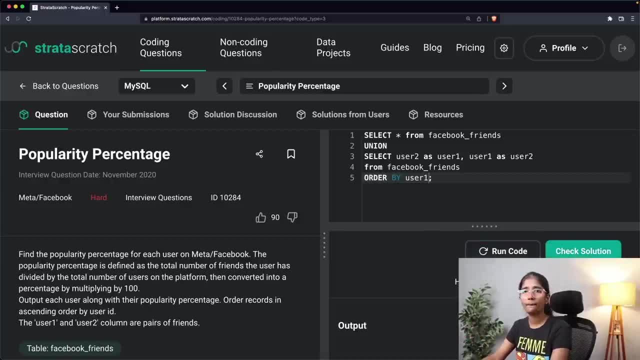 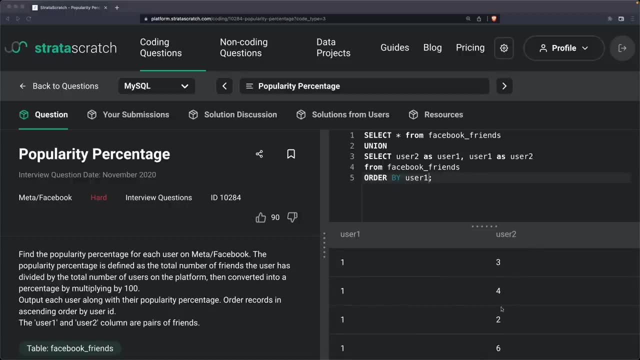 the user. i'm just going to run this query. as you can see, we are now having it in the format of all the one on the left side and its friends on the right side, all twos on the left side and its friends on the right. this is how that union is working, but what exactly is happening here? so 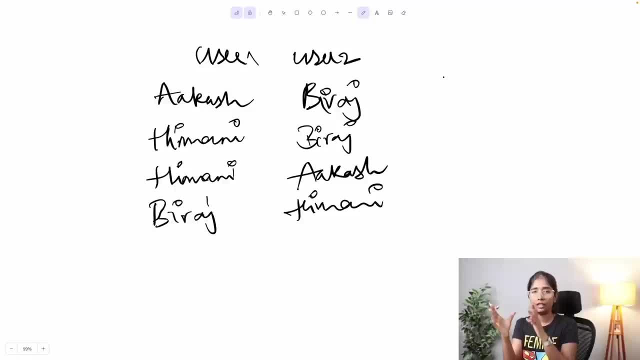 when you see, the first part of a query was: select staff from facebook friends, right, and this is the result. now the second part is we are saying: use user 2 as user 1 and user 1 as user 2. so now this column will become user 1 and this column will become as user 2, so the union basically combines. 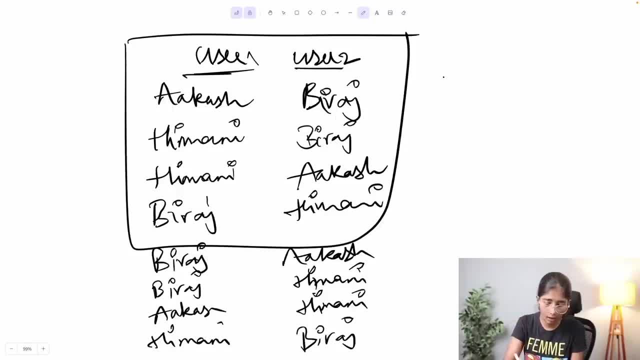 these two results and removes if there are any duplicates present here. so let's just see if there are any duplicates or not, as i can see. is there any barrage and akash no, and then we are saying barrage and himani. so there's already a barrage and himani here, so we can remove. 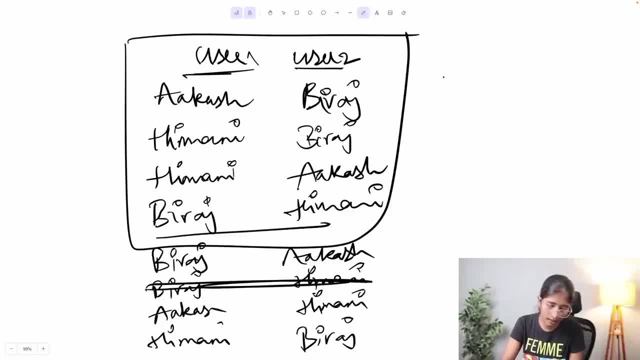 this, and i'm also looking at akash and himani. is there any akash and himani somewhere here? no, so it's going to stay. and there's also something called as himani and barrage. there's himani and barrage already here. i'm just simply going to exclude this, so it is now in the 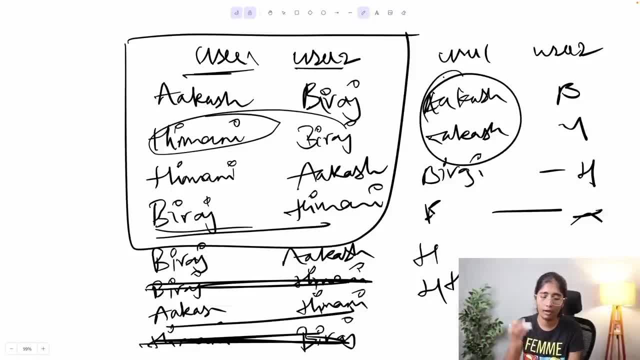 format right on how we wanted it, which is all the users on the left side and their respective friends on the right side. now this explains the first part of our approach, which is calculating the total number of friends a user has. now all i have to do is just group it by the user one. 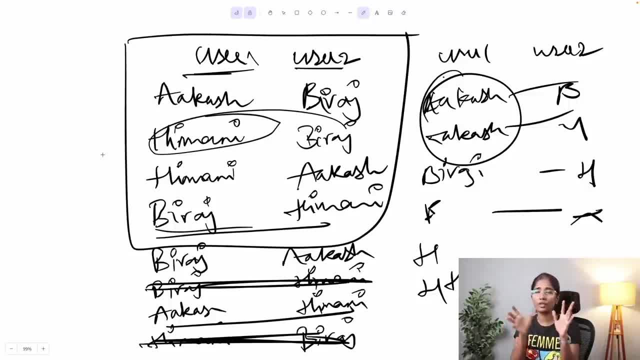 and then i'm going to remove this and i'm also looking at akash and himani. is there any akash and himani? and do the count of the user two to get how many friends each user has. so the second step is of our query construction is calculating the total number of users on the platform. so for that, 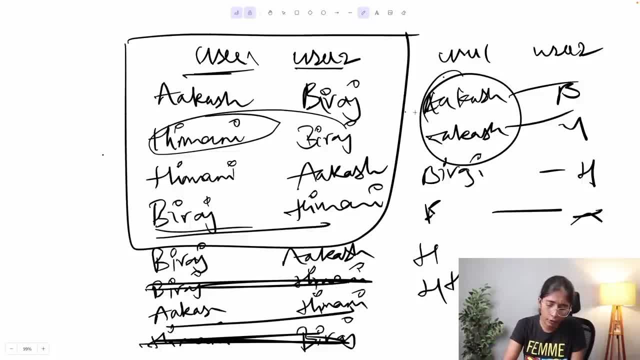 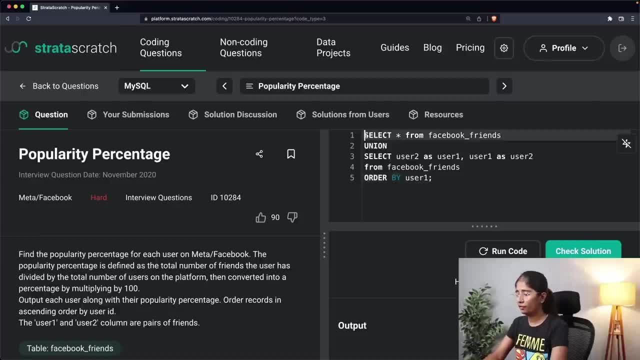 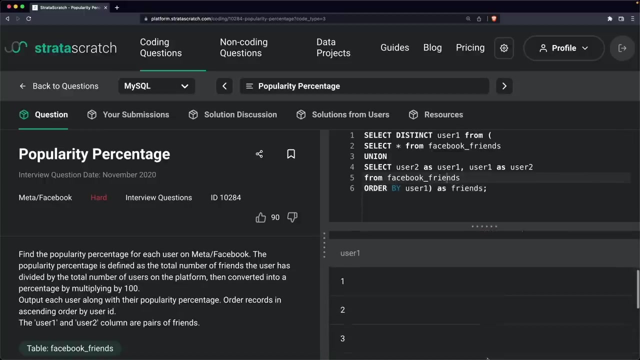 what i can do is i can just simply calculate the unique entry of each user one in this table, right? all i have to now do is use this as the input for select distinct user one from this subquery. i'm going to give this table result. friends, i run this as you can see. now. these are all the distinct users. now i just have to say: 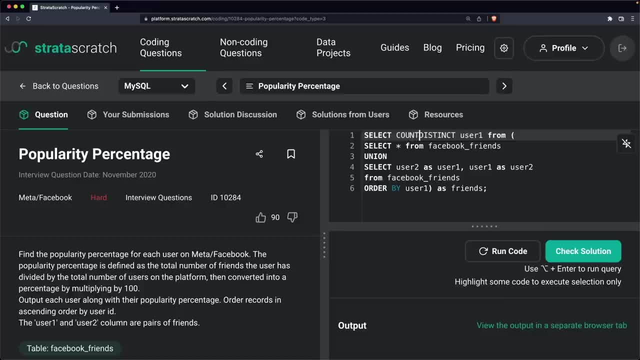 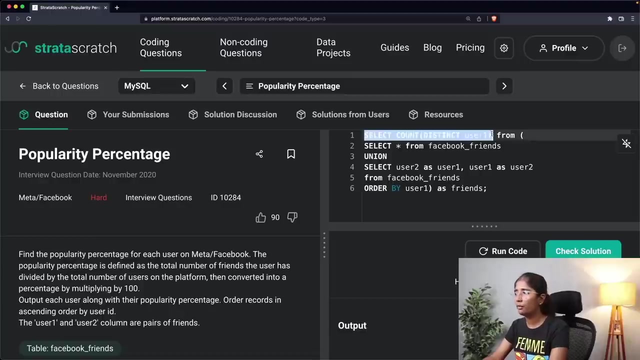 i can see there are a total of nine distinct uses on the platform. i just now have to divide the count of each user's number of friends by this into 100 to get the popularity personalty. but as you notice here, the total number of users on a platform is using this as the input for it to 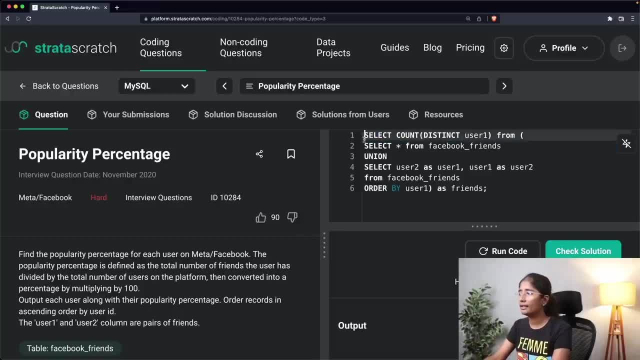 this. now for me to divide this by this, i have to store this result in something so that i can use this as the input for this, to calculate the popularity percentage. so for that i'm going to use a common table expression. width is the keyword which indicates that you're writing. 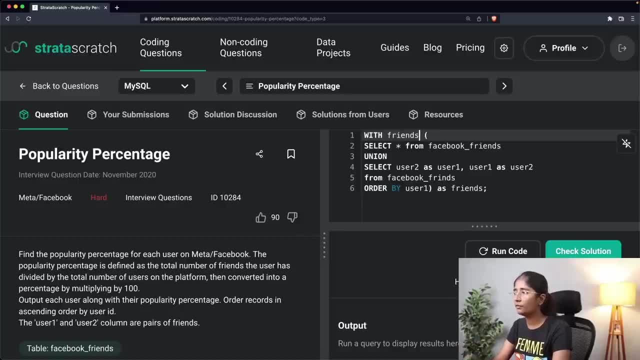 a common table expression and i'm going to give this common table expression name with friends as this. let me just there's a contributor, i'm going to remove this. this is my common table expression and i'm going to use this as the input for my next query, which 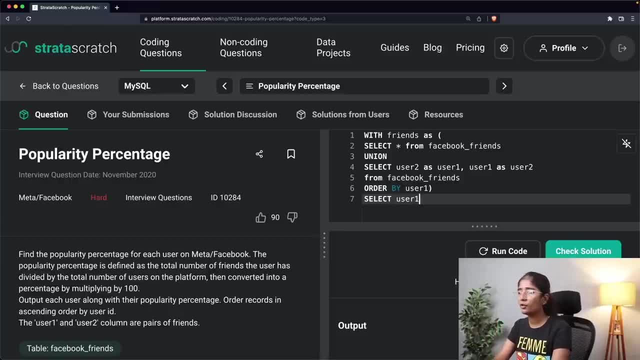 is calculating the popularity person. i'm going to say select user one, which is basically they want for each user the popularity percentage. so i'm going to select user one and i'm going to say count of user two, because count of user two is the one which will tell you the total number. 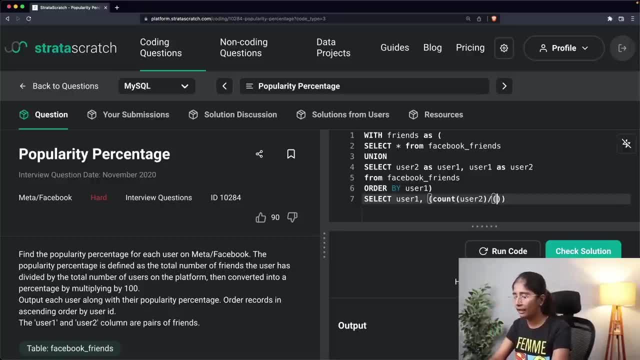 of friends a user has. i'm going to divide this by you: select count of distinct user one, because that is the section which will give us the total number of users on the platform. and this entire data is from the friends common table. expression. group it by user one because we want it for each. 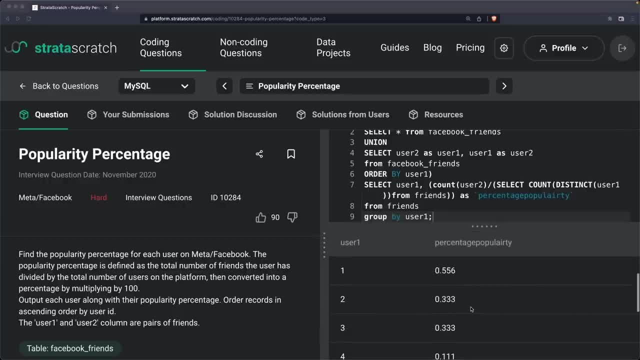 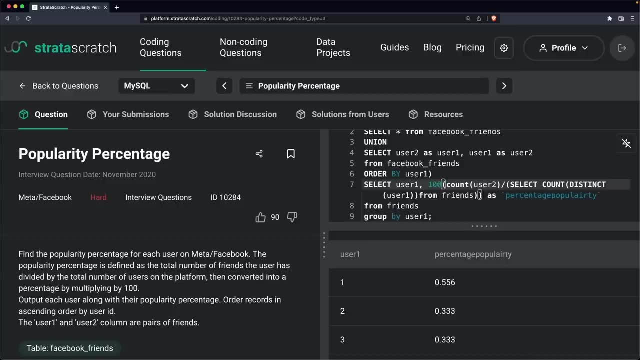 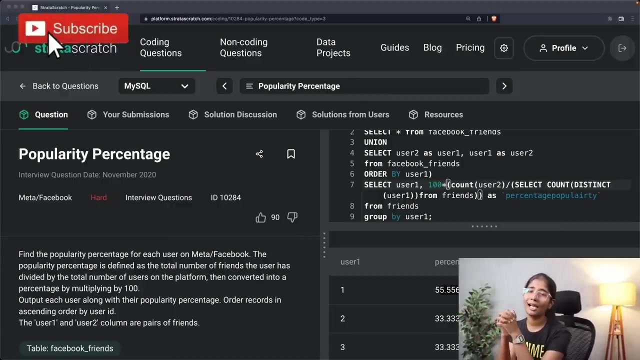 as you can see, we now have the popularity. now i just simply have to write this with hundred: this is the popularity percentage of each user. so, yeah, that is basically how you solve this popularity percentage question. thank you so much for watching. i will see you guys next time. bye. in this video, we'll be covering an sql interview question as a whole, so i'm going to 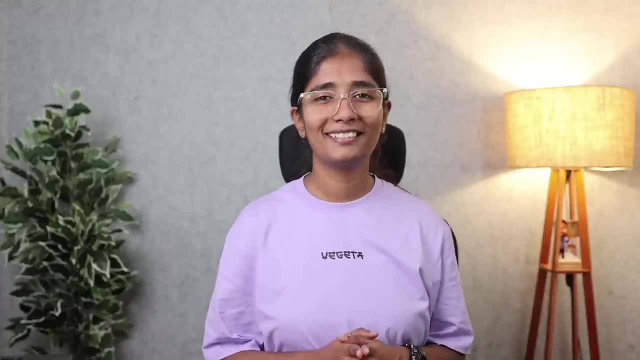 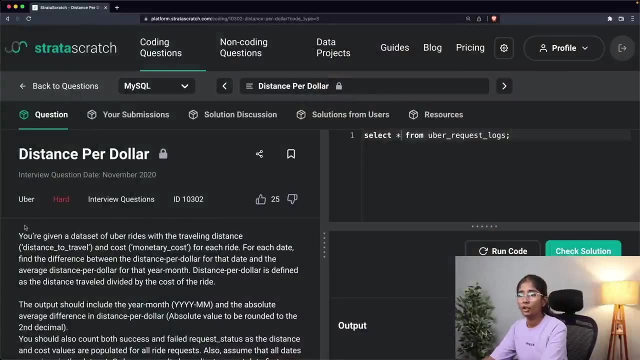 go ahead and start solving. the problem that we'll be solving today is distance per dollar. as you can look at the screen, you're given a data set of uber rights with the traveling distance, distance to travel column and cost- monetary cost column for each right, for each date. find the difference. 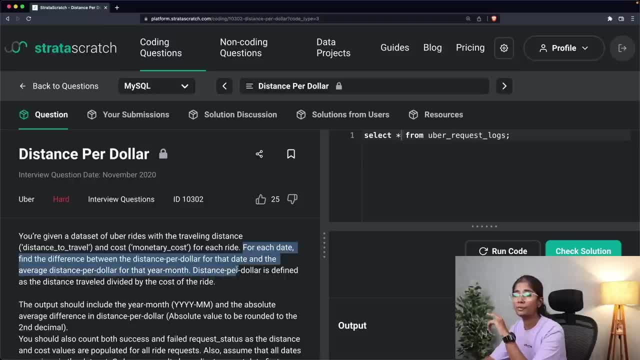 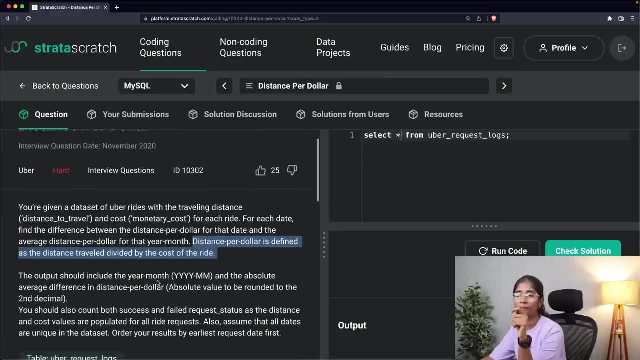 between the distance per dollar for that date and the average distance per dollar for that year, month. distance per dollar is defined as the distance traveled divided by the cost of the right. the output should include the year, month and the absolute average difference in the distance per dollar, absolute value to be rounded to the second decimal you should: 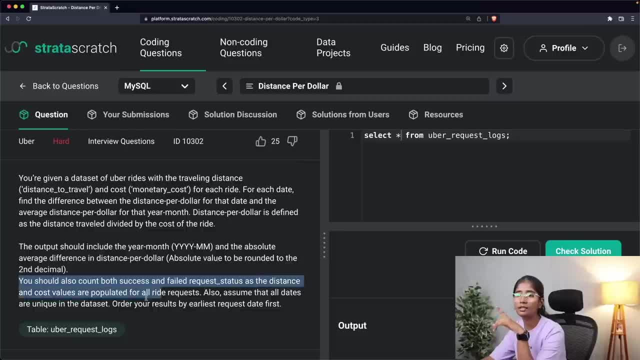 also count both sexes and failed request status, as the distance and the cost values are populated for all the requests. also assume that all the dates are unique in the data set order your result by the earliest request date first. so this is our question and according to our 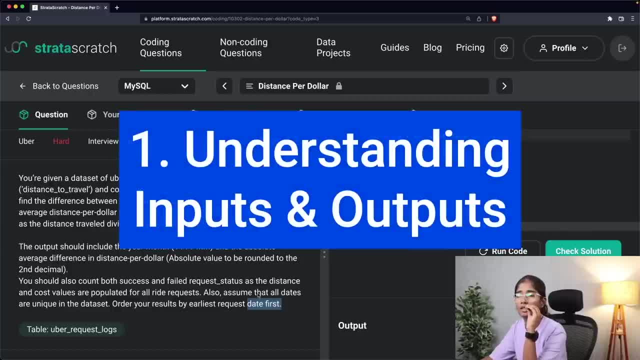 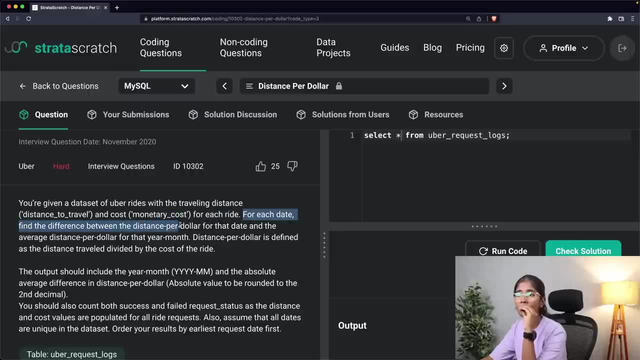 approach. the first step is understanding the inputs and the outputs. so for that i'm just going back to the question again and they're saying: for each state, find the difference between the distance per dollar for that date and the average distance per dollar for that year month. so i see that they're asking us to calculate something called. 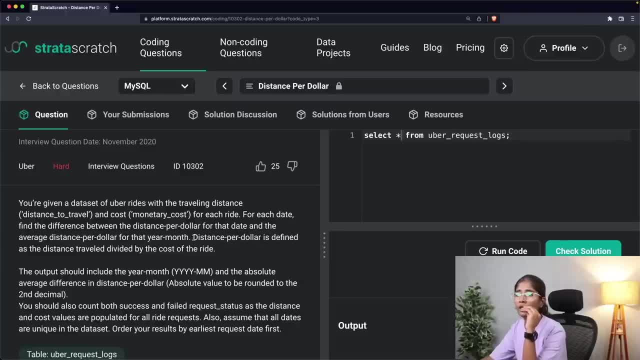 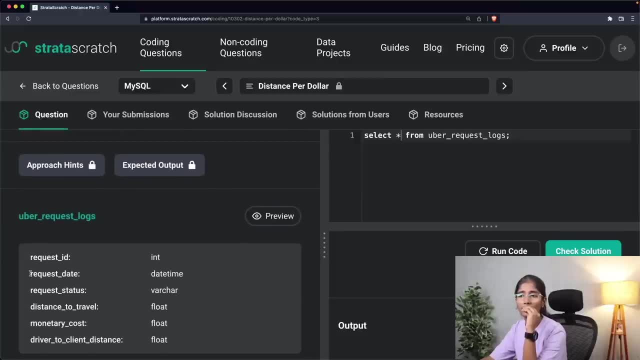 as the distance per dollar per each date. so i see that we have to use a date time column, which i know by looking at the table. it has something called as the request date, so my input is going to be request date and for calculating the distance per dollar i need to divide the distance. 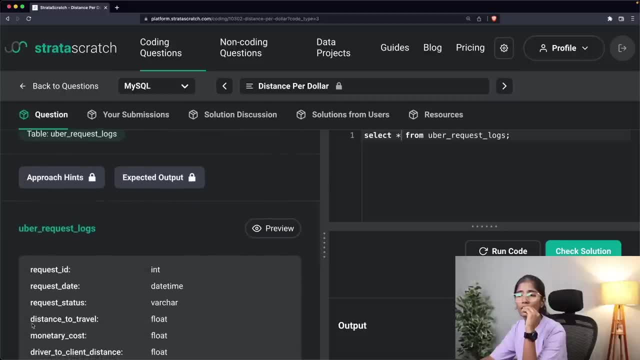 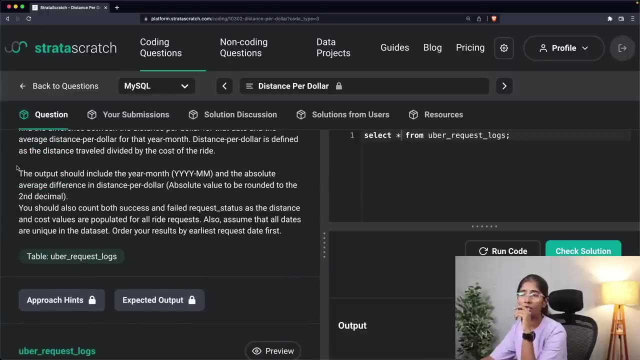 traveled by the cost of the right. so i'm going to use the columns distance to travel and monetary cost now. so my inputs are going to be these three: request, date, distance to travel and monetary cost. now my outputs are going to be as they explicitly mentioned in the question. the output should: 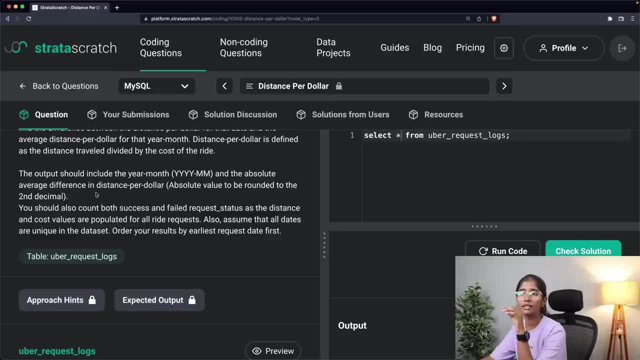 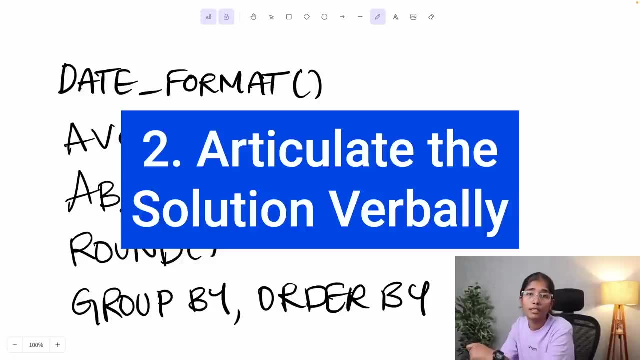 include year, month and the absolute average difference in the distance per dollar and the absolute value to be equal to the average distance per dollar. so i'm going to use the rounded of two decimals. now the second step of our approach is going to be articulating our solution. 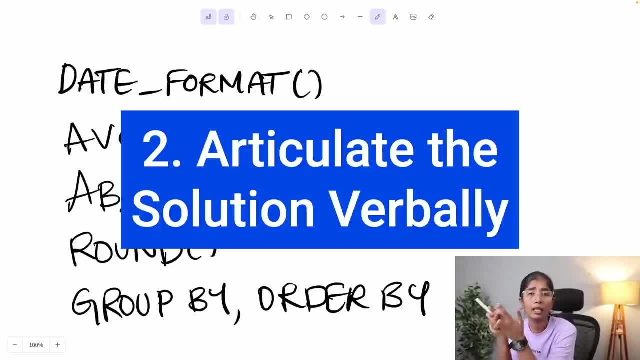 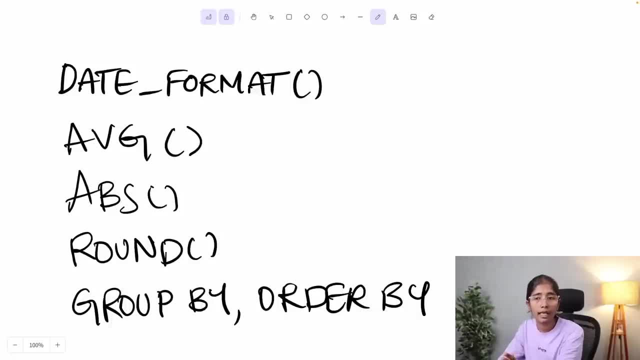 verbally to the interviewer, which is basically explaining our approach and getting a confirmation of our understanding. so from the question we understand that they want us to include the year and month, which means we are basically expected to extract the year and month from the date time column which is requested. so for that i'm going to use the date format. 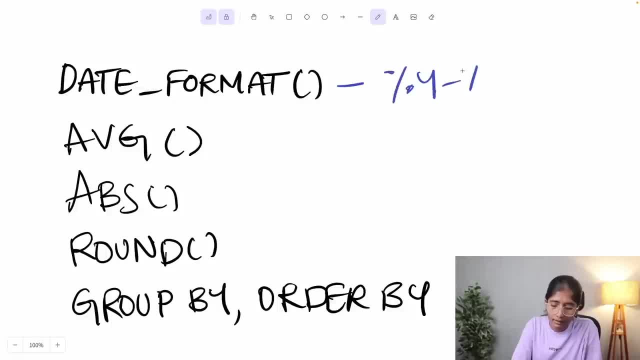 in this way, so that it will extract the year and month for me. and the second thing they want from us is the absolute average difference in the distance per dollar. so for actually calculating the difference first, you need to calculate the average, right? so i'm going to use the average. 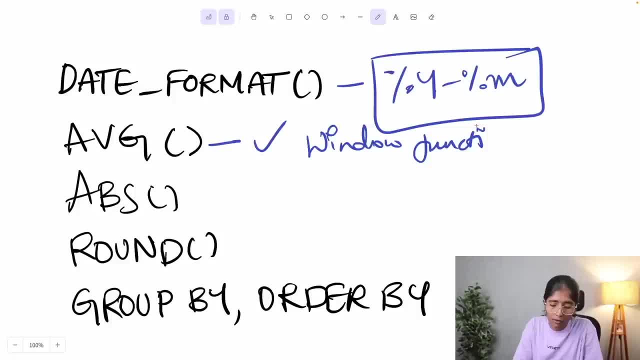 window function so that it is calculated for each and every row. then i'm going to use the absolute function so that i'll get the absolute value of the difference that i'm getting. then i'm going to use the round with the average value of the difference that i'm getting, and then i'm going 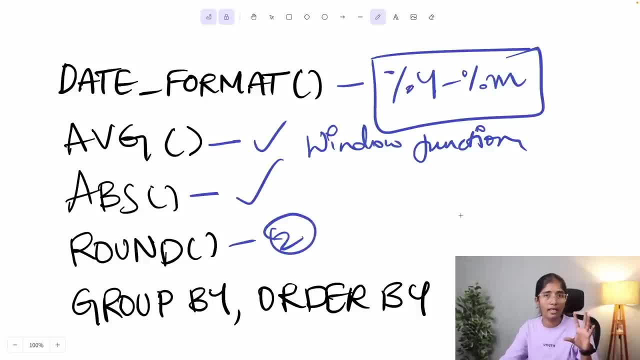 to use the period for the year and month which is in theуз value, which is left at table 2. so you'd be doing a good job of benefitting in this process as a way of calculating theished from from formal plan, and it's also very useful when it comes to senate. it will actually tell you. 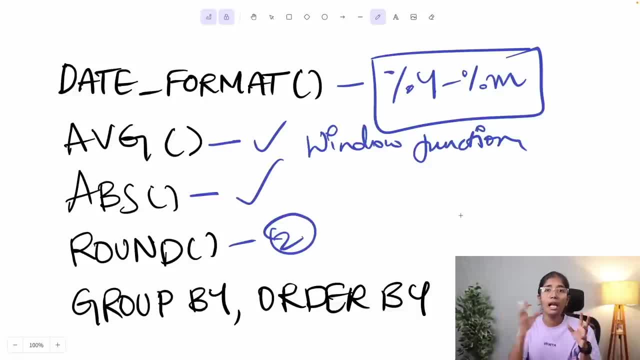 exactly how many extra passes you get if you clear out some issues, your questions, and you want to make sure you give them in your review box that you already did always do so as a survey, which iset nope, it wasn't the issue. by the way, you write a comment. please comment at the end of the video, if you are. 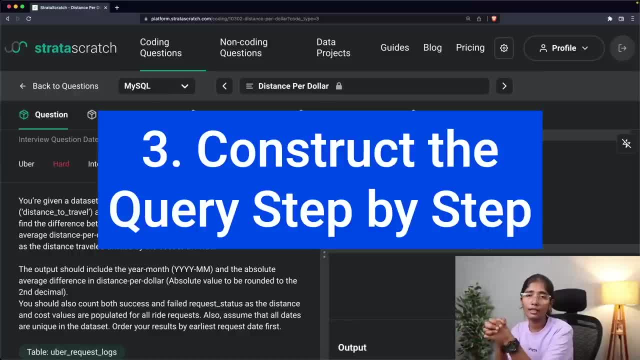 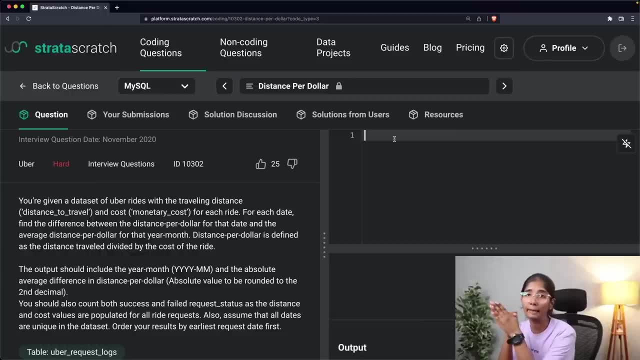 already satisfied with. anything you'll like to know, let me know in the comments section. approach Now. the third step of our approach is constructing the query step by step, And the first part of our query construction is extracting the year and month out of the daytime column. 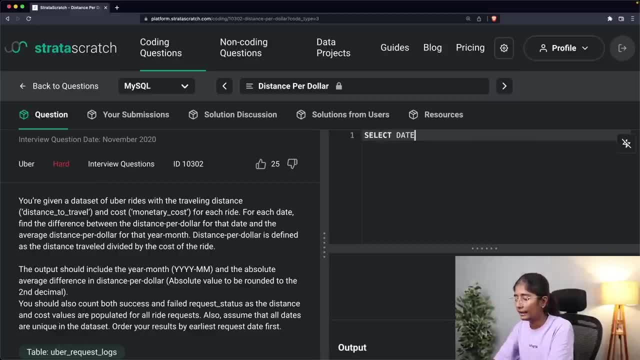 So I'm going to say select date format and our column name is request date And the format that we want is year and month, Sorry, And I'm going to give this entire extracted column a name, probably year, month, And I'm getting this entire data from the uber request logs table. 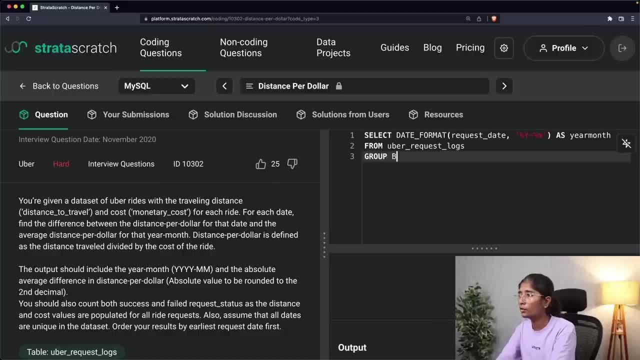 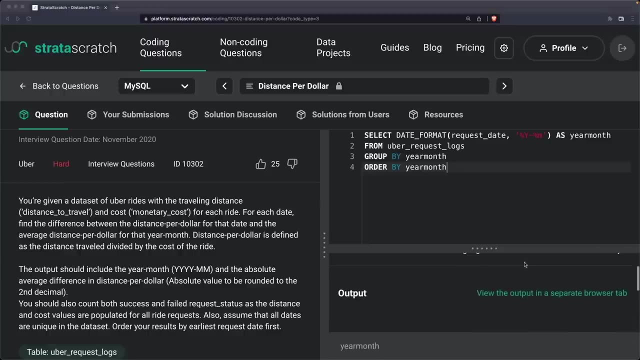 And since they want this for each year month, I'm going to group by year month And I'm going to order by Year month. So this is our code. I'm going to execute now And, as you can see on the screen, we can now see the output for each and every year and month. 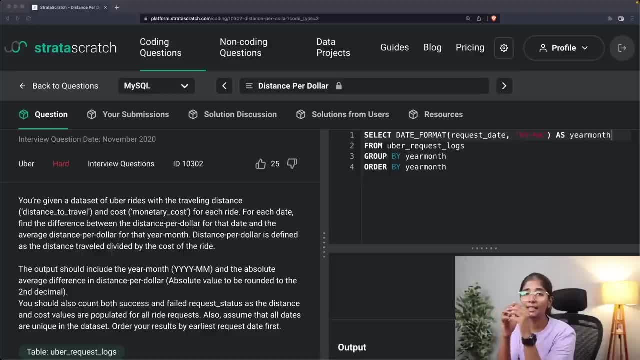 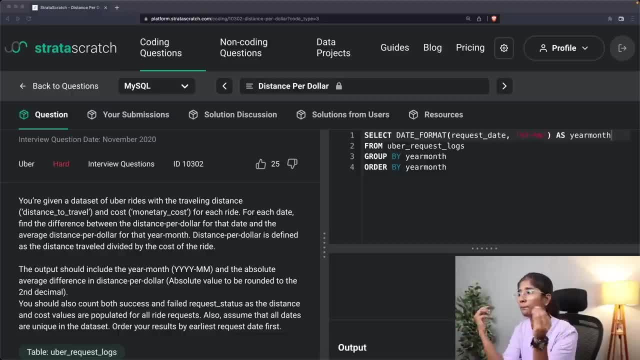 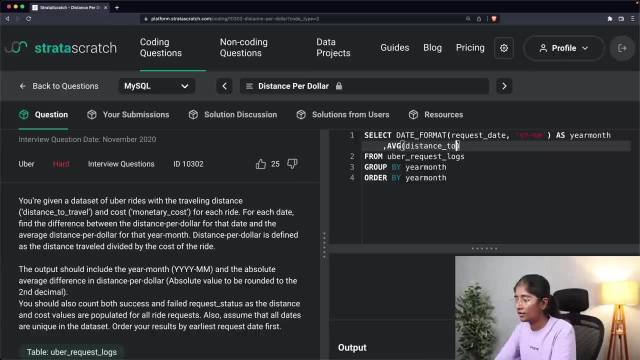 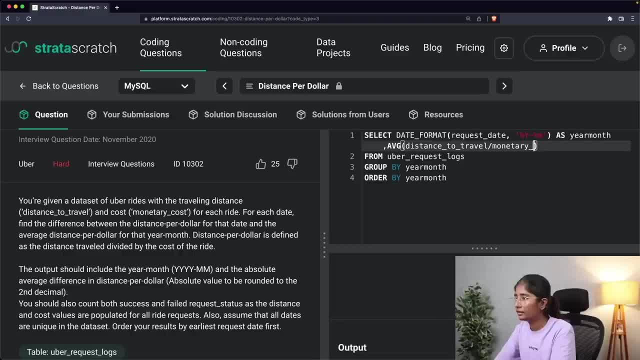 monetary cost. So they've mentioned in a question that the distance for calculating the distance per dollar it is distance to travel divided by the cost. So I've given that Now I'm going to minus this by average of distance to travel divided by monetary cost. 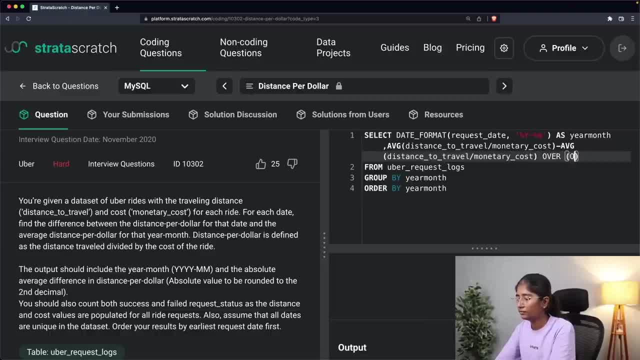 over partition by, Since they want this to be partitioned by the year and month, which is our date format. request date of this year month. So the reason why we're using this year month column directly instead of giving it a column name which is year, month window function will. 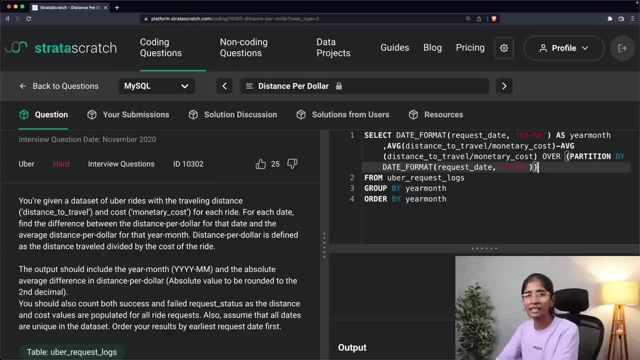 not be able to identify this prior, So we need to specify the entire thing. So this is done. Now I'm going to give this entire column name a function which is probably called as the average difference. So this entire thing is again coming from. 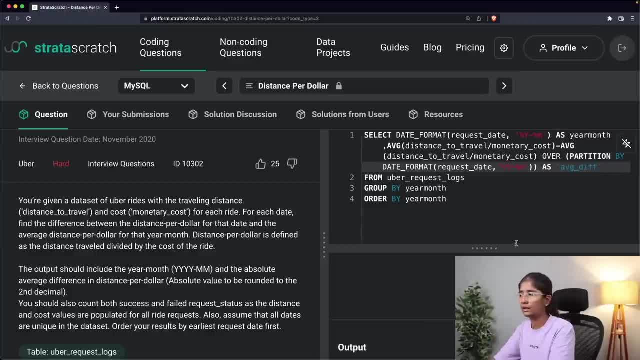 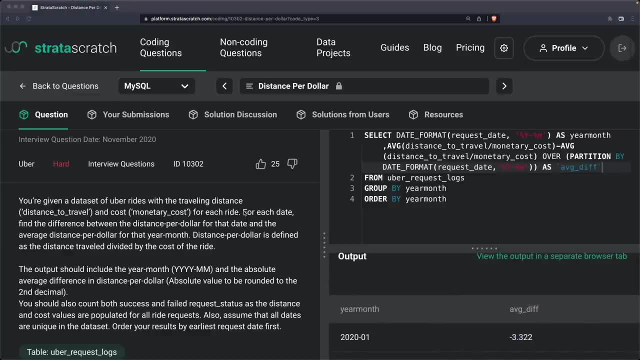 the uber request logs and order by year month. group by year month. So I'm simply going to run this query now. As you can see, you now have the year, month and the average difference, But in the question that specified that they wanted explicitly as the absolute value. So 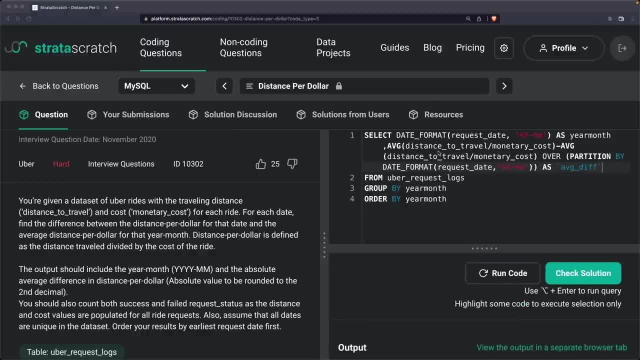 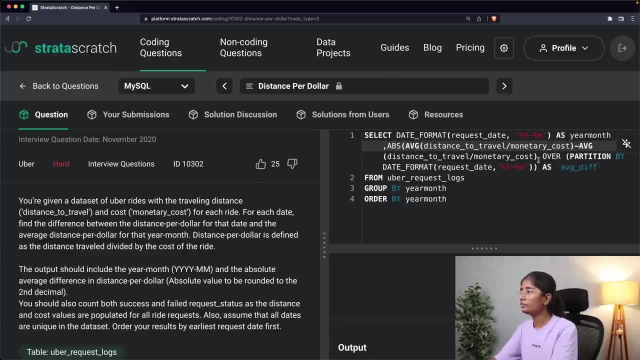 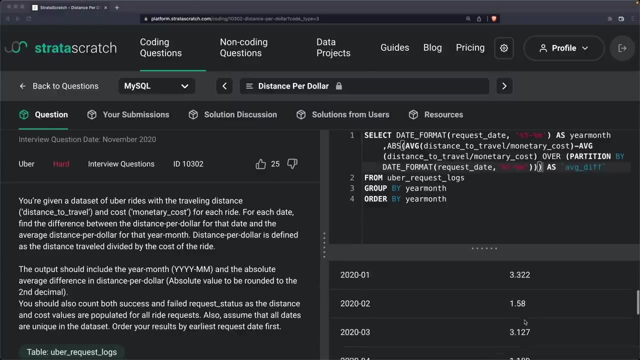 you now have to use the absolute function, and that's what I'm going to do now. So I'm going to see absolute value of this entire thing and I'm going to run it. As you can see, this has been rounded off to absolute value. So let's say I wanted to say absolute. 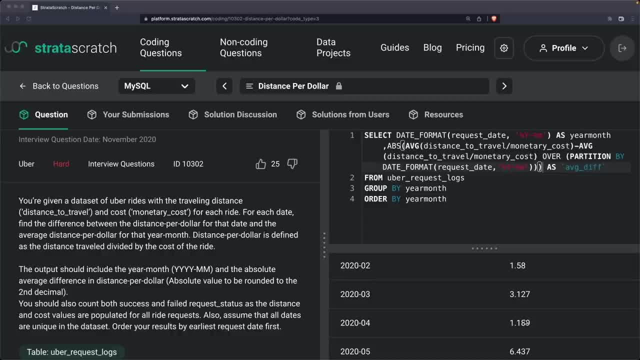 no, that's not the absolute value. See, I haven't earned it yet, But you can see it's absolute value, which is basically it's returning you a positive value. now they also want this to be rounded off to two decimals, so i'm now also going to use round method. so i'm going to say: 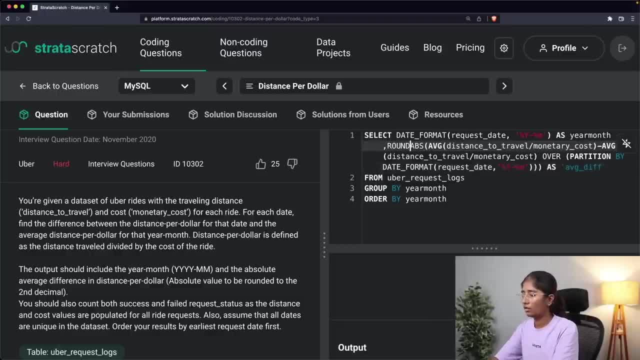 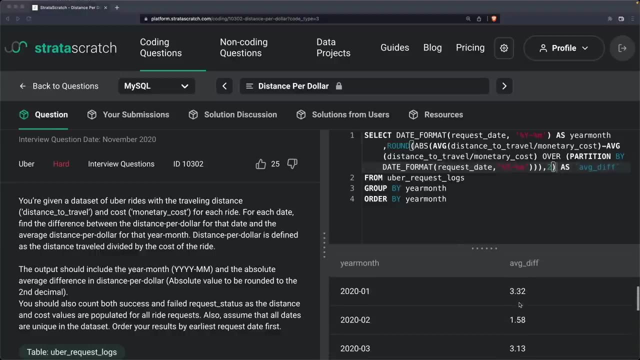 round, and then i'm going to come back here and say two, and then i'm going to run the code. as you can see now this is rounded off to two decimals. so that's basically what they're looking for. the output should contain the year, month and the average difference between the distance per 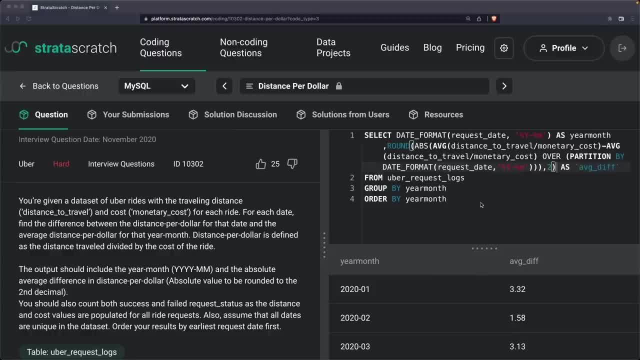 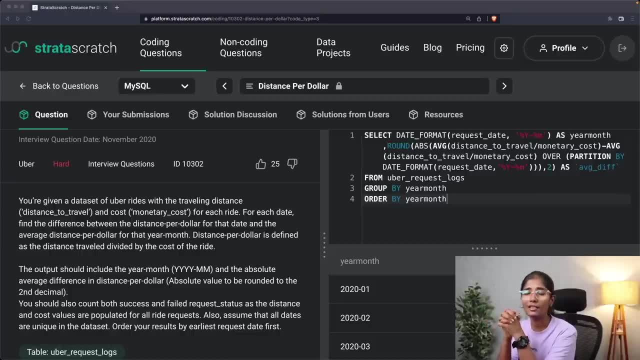 dollar, the absolute value rounded off to two decimals. so yeah, that's how you solve these kind of sql interview questions. thank you so much for watching. i'll see you guys next time. bye in this video. we'll be covering an sql interview for you in the next video, so until then, bye, bye. question asked at amazon. so let's go ahead and start solving the problem that we'll be solving today is monthly percentage difference. given a table of purchases by date, calculate the month over month percentage change in revenue. the output should include the year, month date in this particular format and percentage change rounded to the second decimal point and sorted from the. 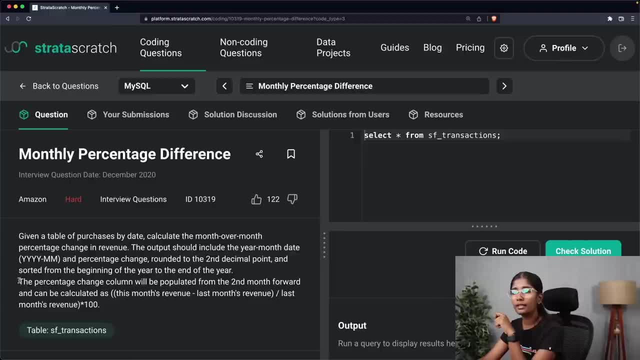 beginning of the year to the end of the year. the percentage change column will be populated from the beginning of the year to the end of the year. the percentage change column will be calculated from the second month forward and can be calculated as this month's revenue minus last. 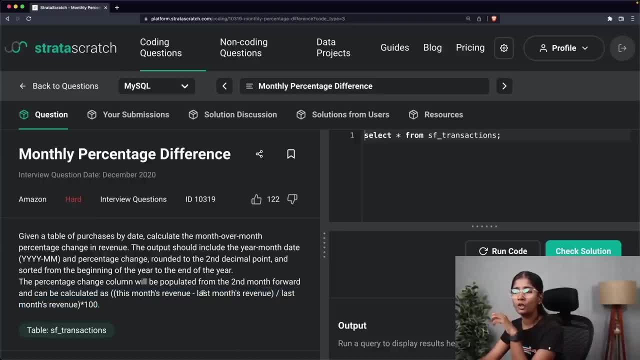 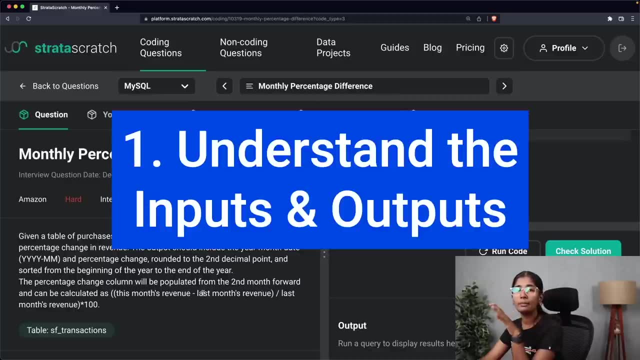 month's revenue divided by last month's revenue into 100. so they're also giving an idea on how to calculate this percentage change column. according to our approach, the first step is to understand the inputs and the outputs, and we can do that by reading the question clearly once. 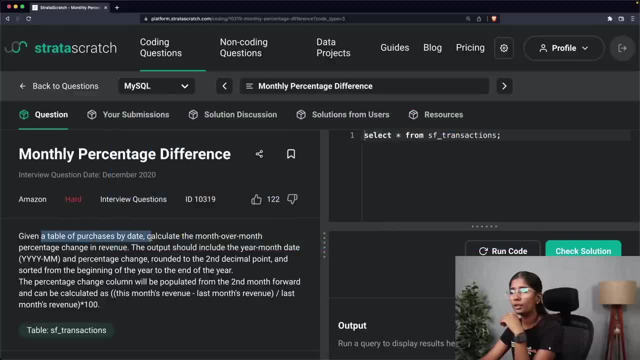 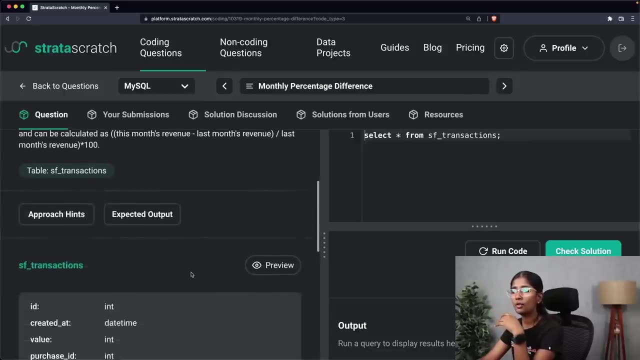 again, since they're saying: given a table of purchases by date, calculate month over month percentage change in revenue. there is some daytime column involved here. so for me to confirm whether we have a daytime column or not, i need to have a closer look at all the columns in the table. so if i scroll down i can see all the available columns. 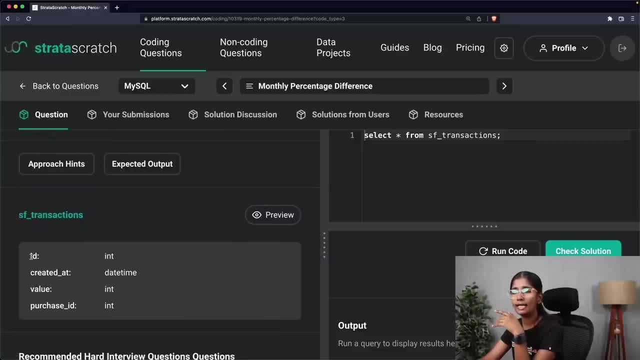 in that particular table which is named as the sf transaction. so i see id created at value purchase id. so my input is going to be the daytime column which is created at, and since they are wanting the percentage change in the revenue, i'm guessing the value is the one which contains the revenue number. 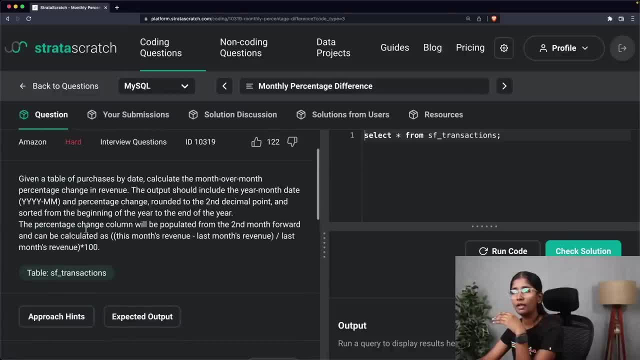 so my inputs are going to be created at value and they said the output should include the month, year, date and percentage change. so my output is simply going to be that month- year column and also the percentage change column. that will be calculating using the formula that they have. 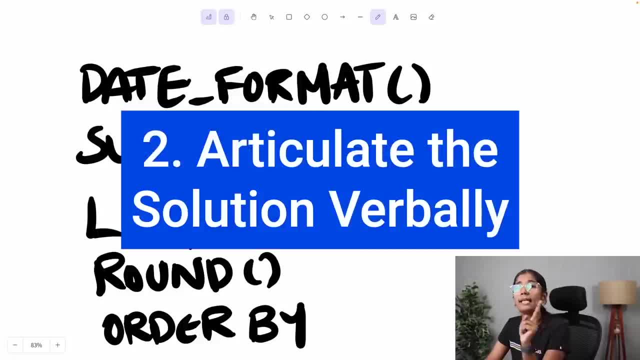 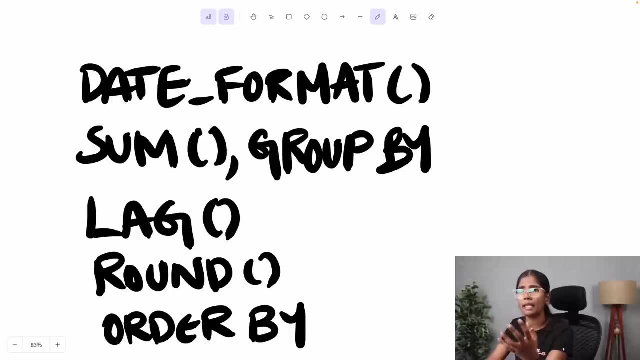 mentioned in the question. so the second step of our approach is articulating a solution verbally to the interviewer which is basically explaining our approach and getting a confirmation of our understanding in our question. the output should contain the date time column in a particular format, which is basically in the year and month. i'm going to use the date format function in mysql which will 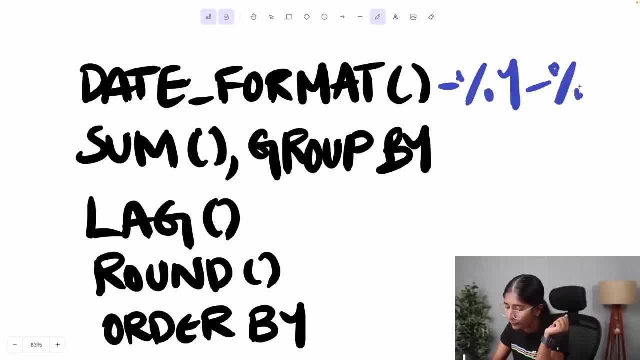 help me extract the year and also the month for that particular output column. and they are also asking us to calculate the percentage change in the revenue. before we calculate the percentage change in the revenue, we first need to calculate the revenue right, and for that i'm going to use 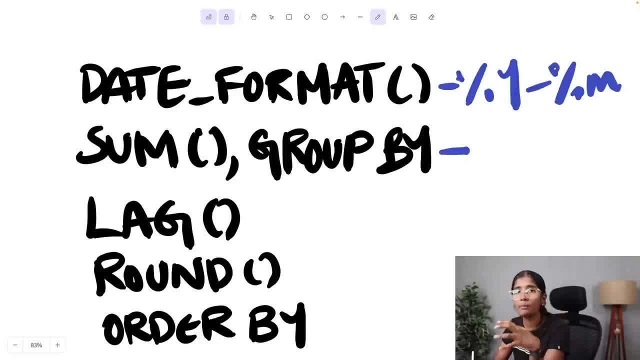 the sum for the entire value column and group it by the month and year column that we are extracting so that we can get the month wise revenue and this will generate the revenue for us. so once the revenue is generated, i'm going to now calculate the percentage change. 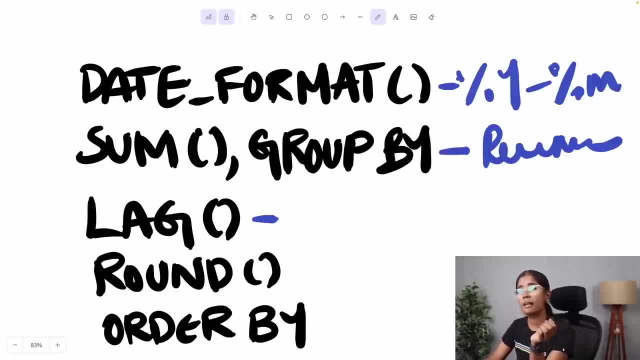 in the revenue using the formula described in the question. so in that question they're using the terms such as previous month and current month, and one function that comes to my head for calculating the percentage change in the revenue is the percentage change in the revenue, which is a window function, and i'm going to use the lag for that. now they've also explicitly 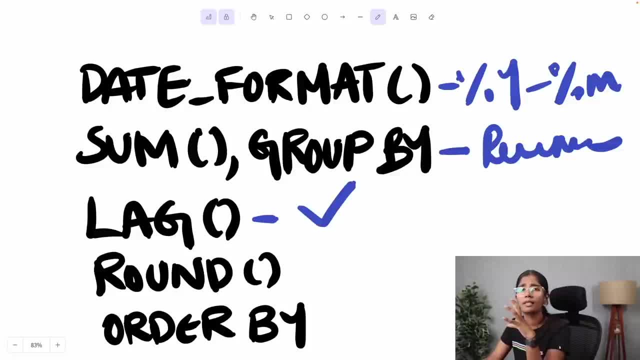 mentioned that they want us to round off the entire percentage change to two decimal points, and for that i'm going to use the round function with the input as two, so that the decimal points are rounded off at two. and finally, they want us to order this as per the starting year. so i'm going 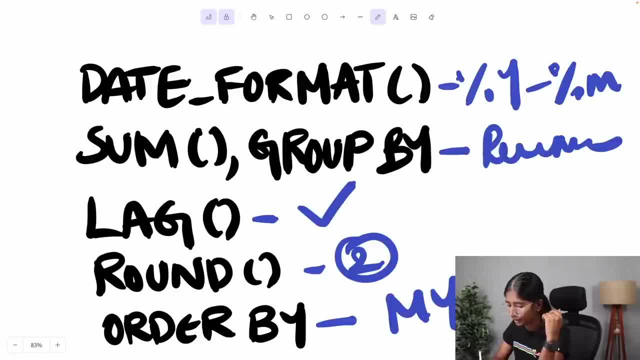 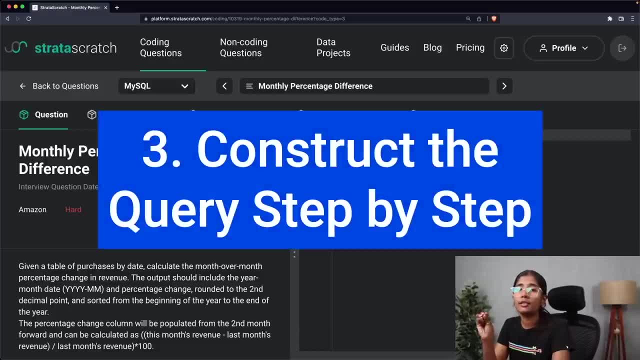 to order it by the month year column that we are generating. so this is basically the way that we are going to do it. so this is basically going to be my approach. now the third step of our approach is constructing the query step by step. the first step of our query was extracting the month and 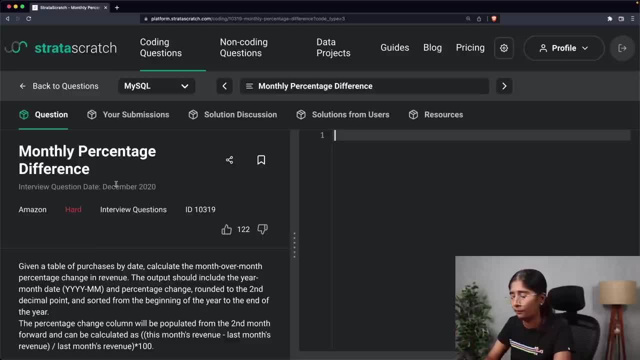 the year from the date time column using the date format function. so select date format from the created at column. it has to be in the format percentage y, percentage m, and i'm going to select the date format and i'm going to select the date format and i'm going to. 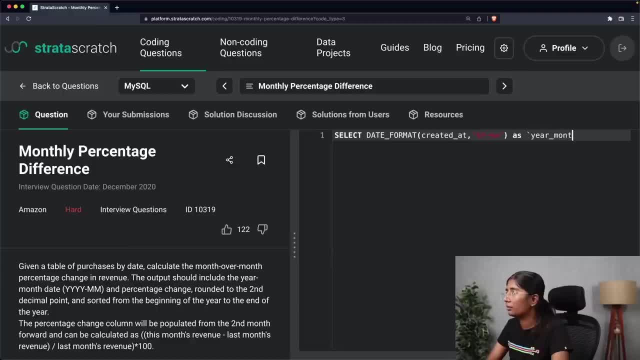 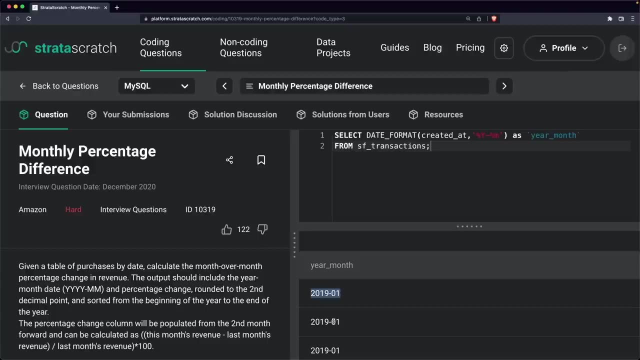 give this column a name as your month, and this data is coming from sf transactions. so i'm going to now run the query. as you can see on the screen, we have extracted the year and month column using the date format. now the second step is calculating the total revenue. so for that i'm just going to check. 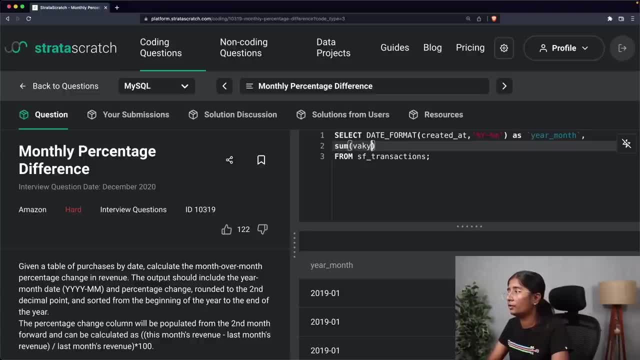 sum of value and give this a revenue name, and i'm going to group it by this column year month so that i get the monthly revenue. so i'm now going to run the query again. as you can see in the output, we now have the monthly revenue. 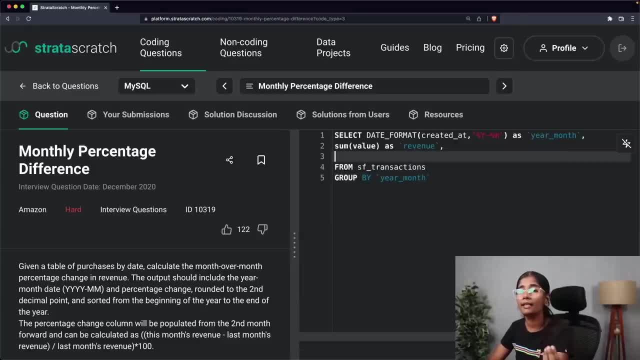 now our next step is to run the query. as you can see in the output, we now have the monthly revenue. now our next step in constructing our query is calculating the percentage change in the revenue using the lag window function, and we are going to use the formula that has been described in the question. 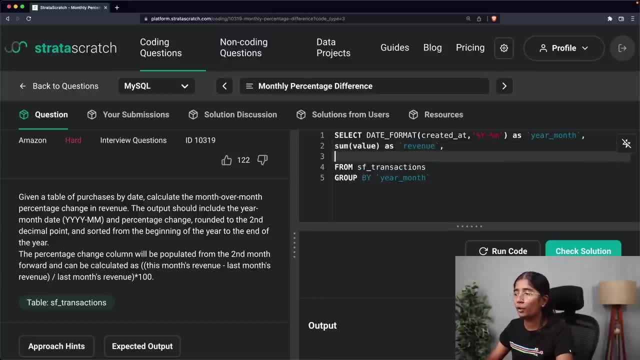 so, as described in the question, i am going to first use the formula this month's revenue minus last month's revenue, which is for this month's revenue i'm simply just going to say sum of value and for last month's revenue is where i'm going to use lag of sum of. 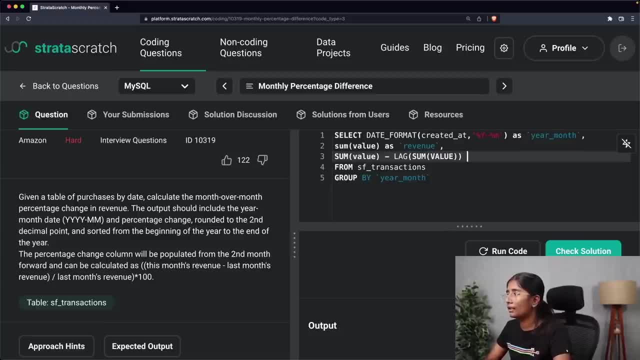 value. okay, and since this is a window function, to indicate the SQL that this is a window function, i'm going to use the over clause and i'm going to put this entire thing in brackets and divide this entire thing pi last month's revenue again, which is: 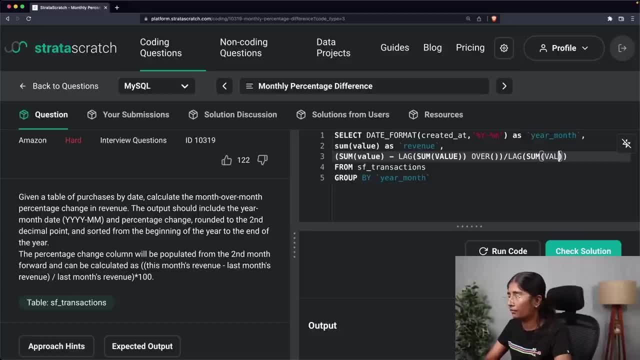 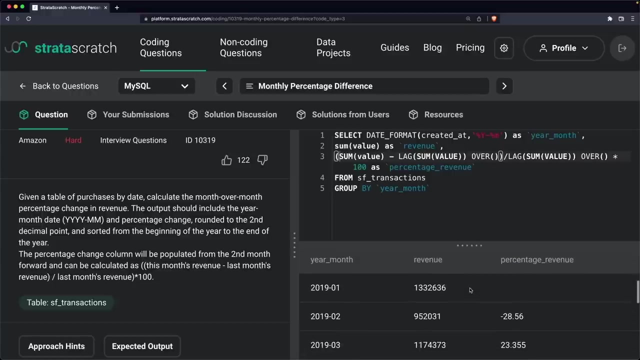 where i'm going to use the lag sum of value and i'm going to indicate that this is a window function and i'm going to multiply this with 100. and i'm going to give this column name: percentage revenue. i'm going to run this as you can see the output. now we have the. 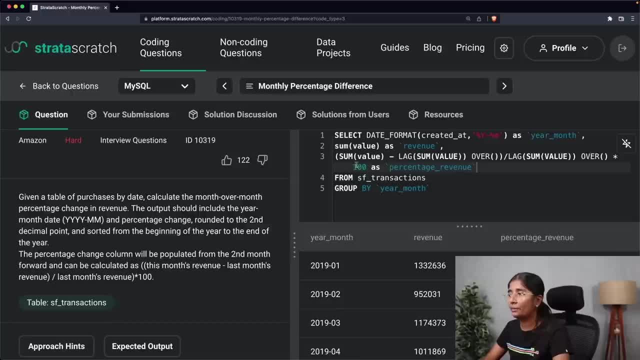 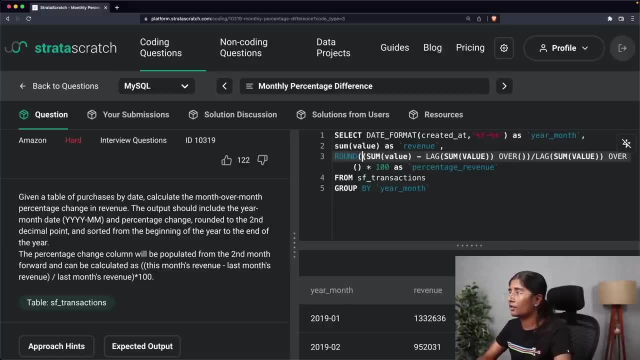 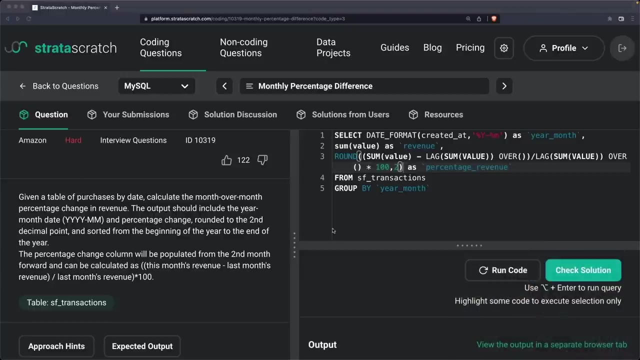 year, month revenue and percentage revenue. now this next step is rounding of this entire thing to two decimals. so i'm now going to use round function and then comma it by two and then going to run this code again and you should be able to see that this is. 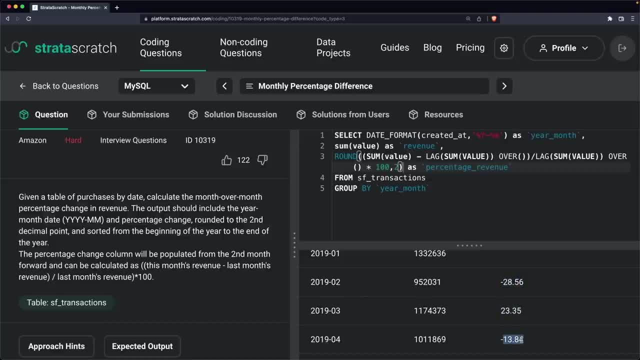 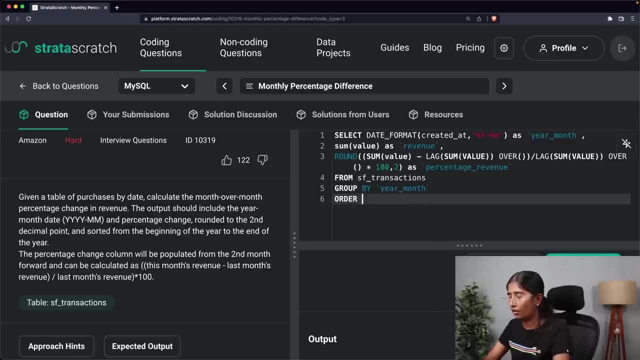 now rounded off into two decimals. now the last step that we need to do is basically ordering this by the year month. i'm now just simply going to say order by year month, and then i'm going to run and you can see that again, this has been ordered. 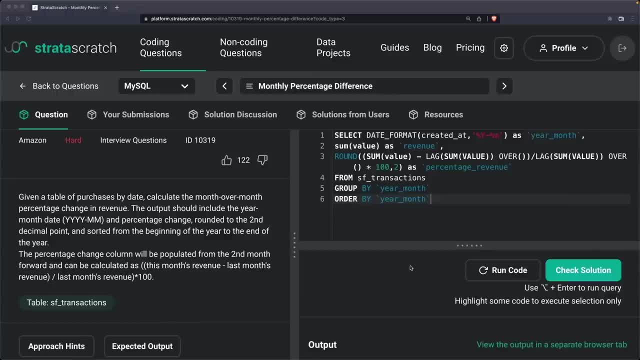 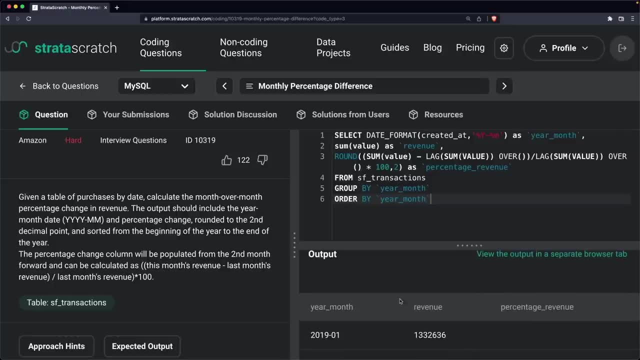 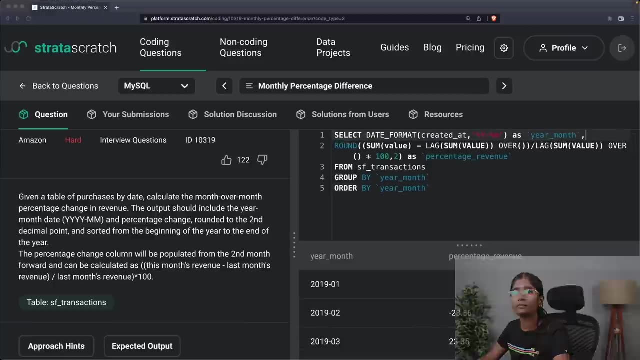 so this is our output. since our question says that the output should only include the year, date, month and the percentage change, i no longer need to show this revenue column, so i'm just simply going to remove this, or you just simply have the year and the percentage revenue. 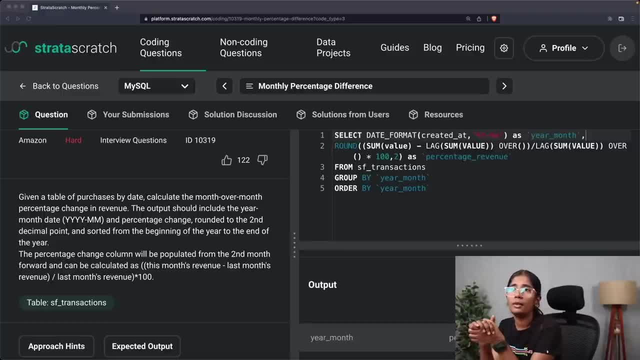 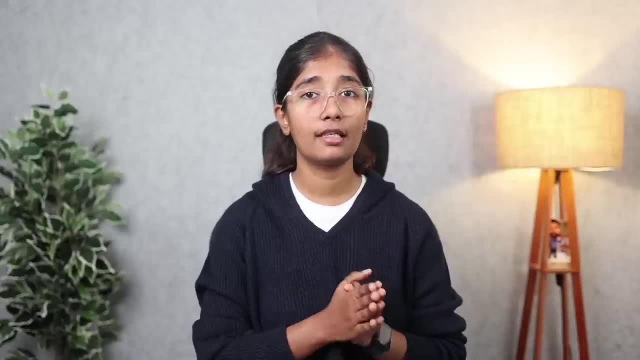 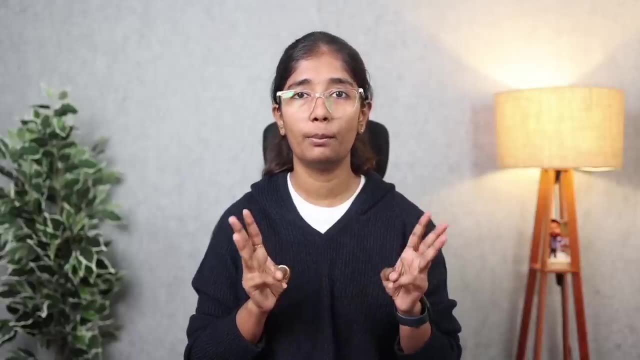 so, yeah, that's how we operate the revenue column. now the next step is in regard to the ratings that i want to give is that number one marginality, which is just the number one marginality of a number, and, for example, of my marginality is size, population, because 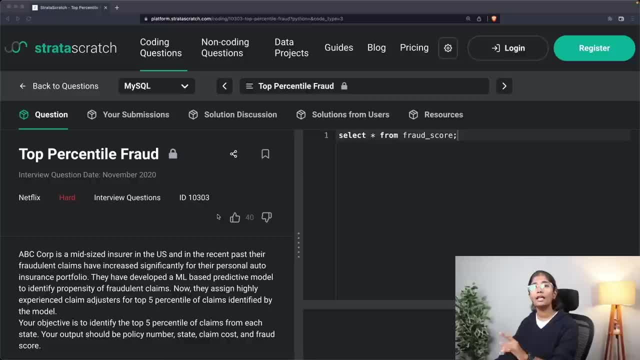 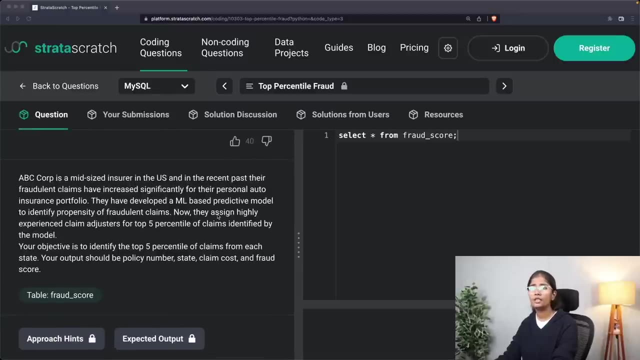 let's say under the eleven sixteen. you want to give yourself a formula versus the縛, as jean is reading from the current formula. so this is the current Очень risk this series. let's take a look at the question now. abc corp is a mid-sized insurer in the us. 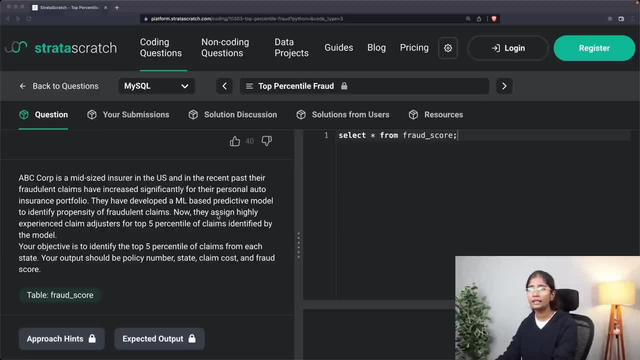 and in the recent past the fraudulent claims have increased significantly for their personal auto insurance portfolio. they have developed a ml based predictive model to identify propensity of fraudulent claims. now they assign highly experienced claim adjusters for top five percentile of claims identified by the model. your objective is to identify the top five percentile. 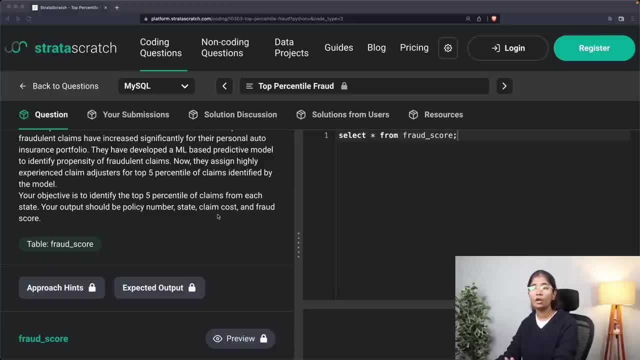 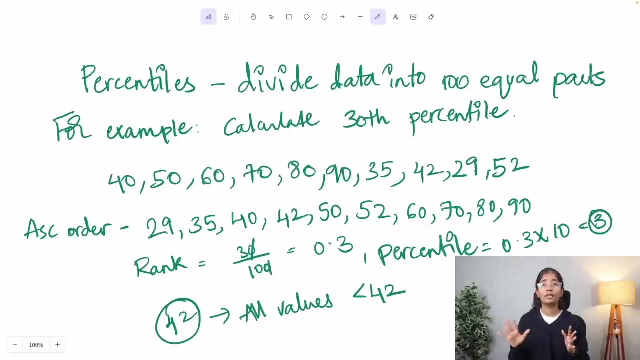 of claims for each state. your output should be policy number, state claim cost and fraud score. but before we get into that, i'm seeing terms such as percentile. so what exactly does this percentile mean? percentile is simply a value under which a percentage of data falls into. so if you look, 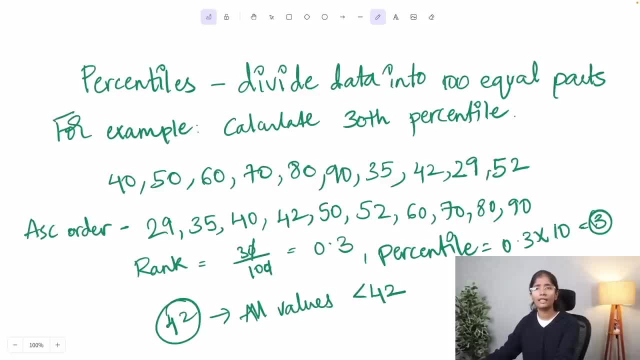 at the screen. we have data points such as 40, 50, 60 so on- total 10 data points, and we are being asked to calculate the 30th percentile. the first step of calculating a percentile is arranging the data points in ascending order, that is, from lowest to the highest. the next step of calculating that particular value under which? 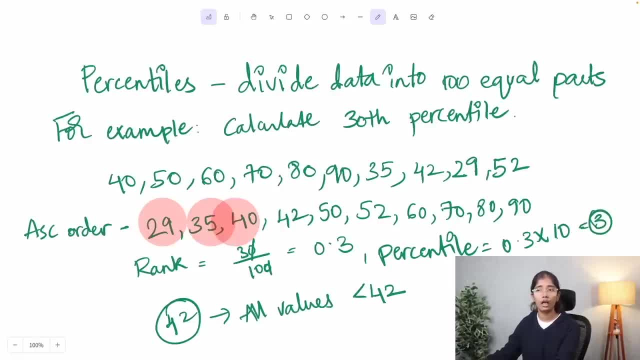 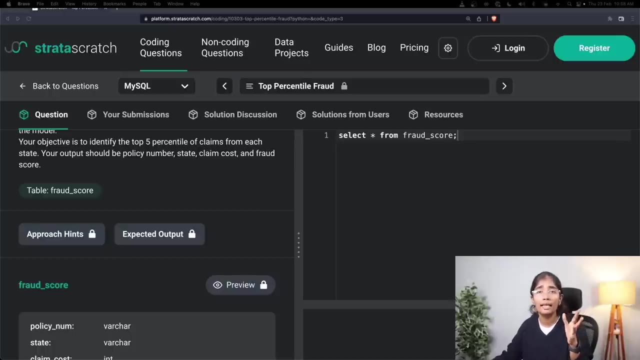 30 percent of the data falls is. you have to count the numbers from left to right. 42 is the number under which 30 percent of the data falls into. now, coming back to our question, where they asked us to identify the top five percentile, what they meant is basically finding all the data that falls into. 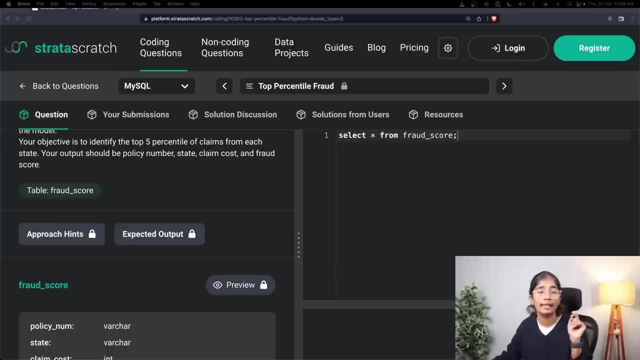 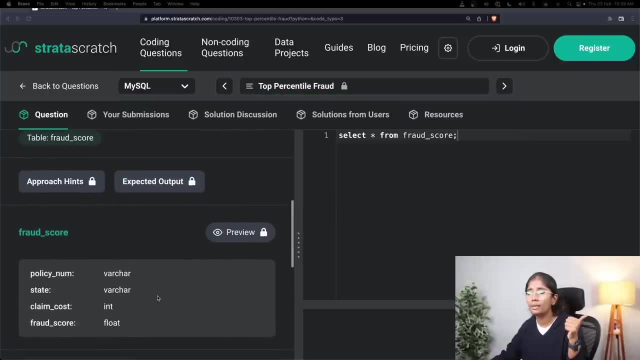 all the values that fall under the top five percent of the fraudulent claims. the first step of our solution is identifying the inputs and the outputs. so let me take a look at all the columns that are present in the table to see which will give me the fraud claim. so i can see that there's 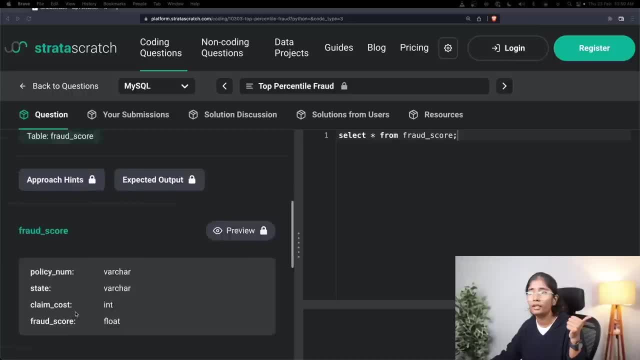 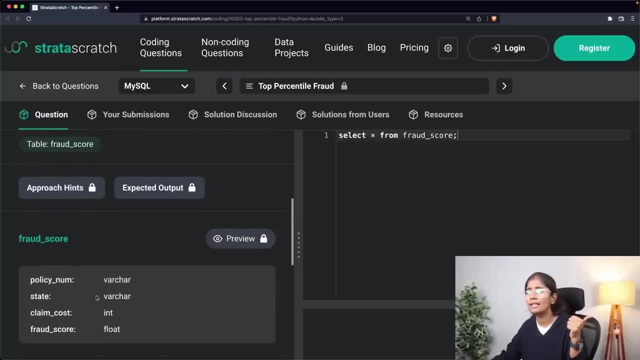 a column called as fraud score. so i'm going to use this as the input for calculating the fraud claim. and since they're saying that they want it for each state, i'm going to use the column called as state, as mentioned here. so my inputs are going to be fraud score and 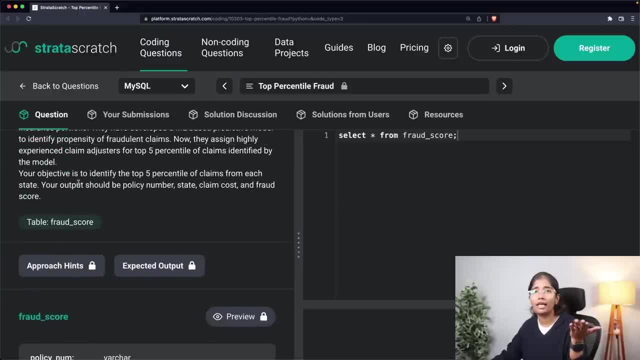 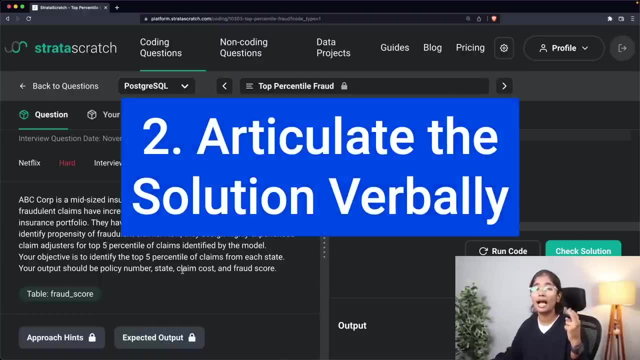 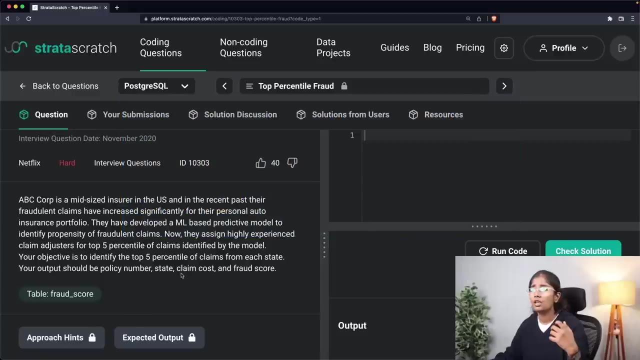 and state what are my outputs going to be here? they explicitly mentioned that it should contain policy number, state, claim, cost and fraud score. now the second step of our approach is articulating a solution verbally, which is basically explaining your approach to your interviewer and getting your confirmation so in our questions, since they're asking us to identify the top five. 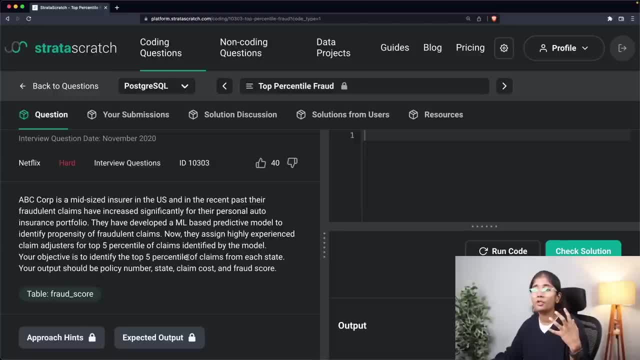 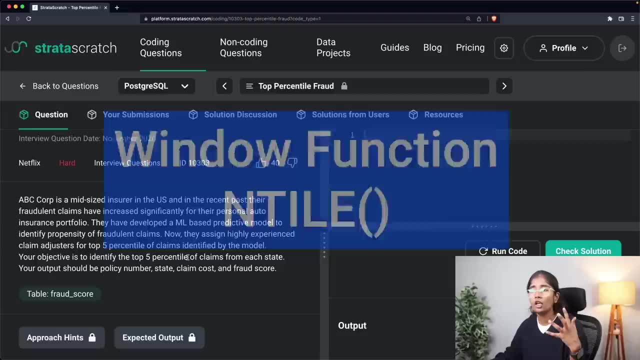 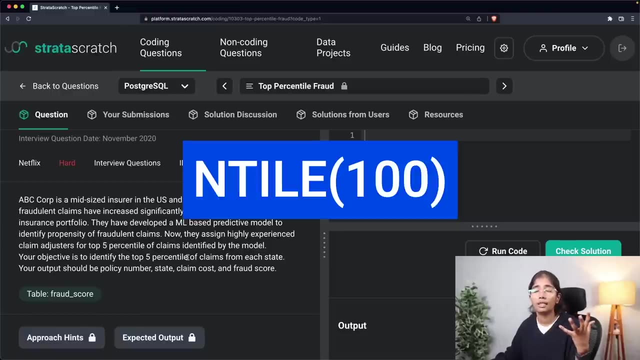 percentile of claims from each state. the thing that comes to my head for calculating the percentile is a window function, end tile, which will help you calculate percent tiles, quartiles, etc. so my input for the entire function is going to be 100, so that it divides the entire data into 100 equal parts, which is what percentile is, and then i'm going to use a filtering. 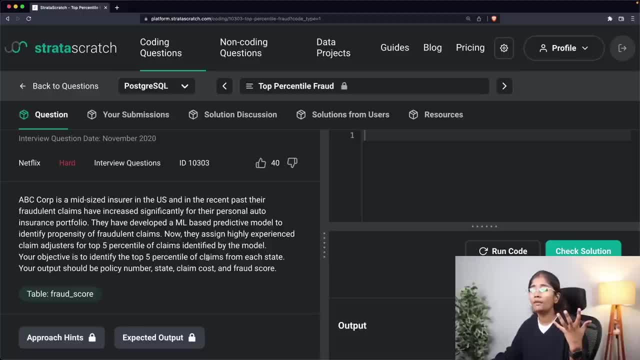 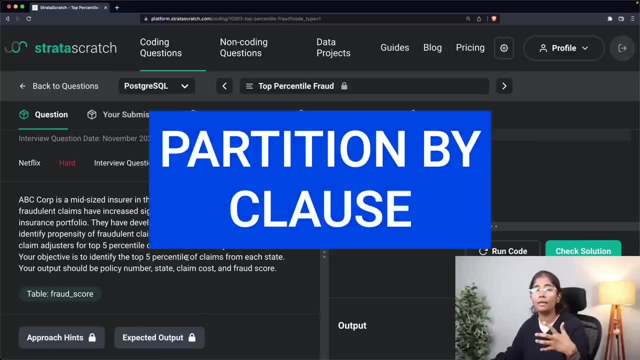 technique for filtering out the top five percentile. now, when they said from each state. i'm using a window function here. right, and in window function you have a clause called as partition, by which will help you create windows, as per the column that you mention in it, and since the question. 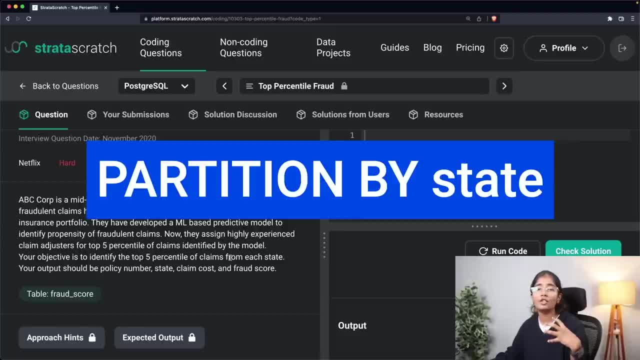 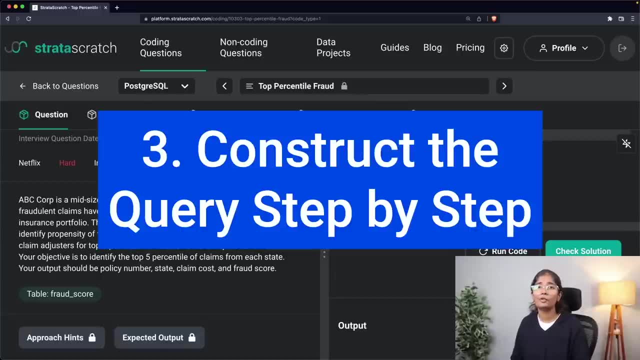 says from each state. i'm going to say partition by each state in my window function so that for each state i'm going to get the top five percentile. now the third step of our approach is constructing the query step by step. i'm going to say select. 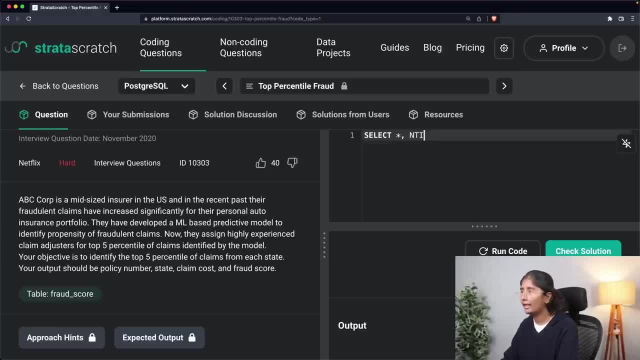 stars, since they want almost all the columns in the output, and tile is the function that i'm using to calculate the percentile with the input as 100, so that the data is divided into 100 equal parts. i'm going to use the over clause used to indicate that you're using a window function. 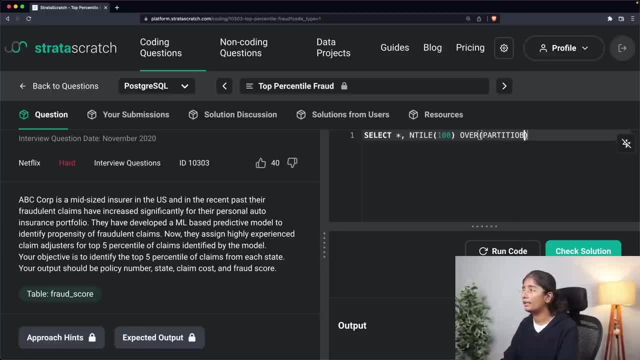 and i want each of this window to be partitioned by state, since the question states they want it from each state, and i'm going to order this by fraud score- the column which contains the fraudulent claims. and since they want top five percent, i'm going to order this by descending order and i'm going to give this entire, entire function. 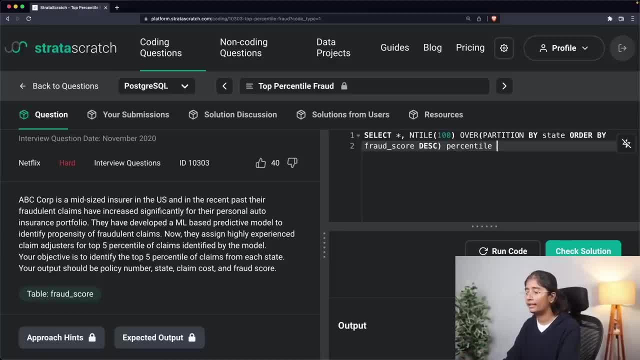 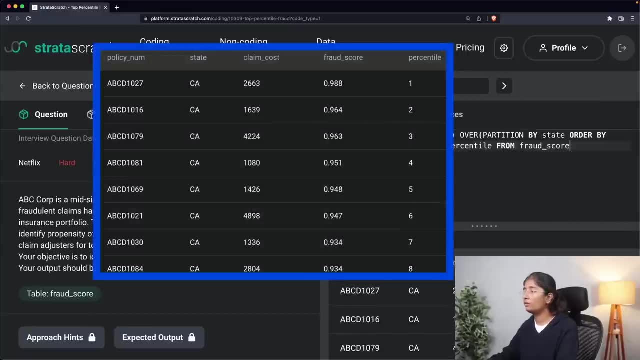 column a name which is percentile, since that's what we are calculating, and this entire data is coming from the fraud score table, so i'm running it okay. great, i now can see that it is ordered by the fraud score and divided into 100 equal parts. now the next step. 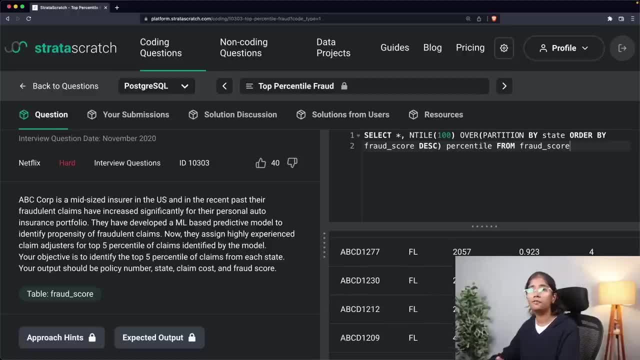 is for me to filter out the top five percentile from this entire query. so this table has to be an input for another table so that i can filter it out using the where clause. so that's what i'm going to do now. this table is going to be one and i'm going to select star from this table. 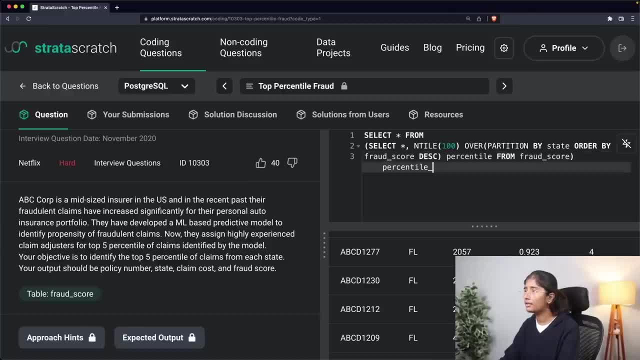 i'm going to give this table a name called as percentile table and filter out where percentile is less than or equal to five, because we are looking for the top five percentile. so i'm going to run this query now and there you go. you now have, as stated, it should contain policy numbers. state. 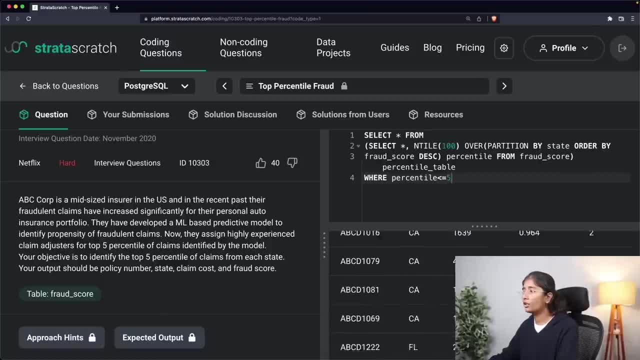 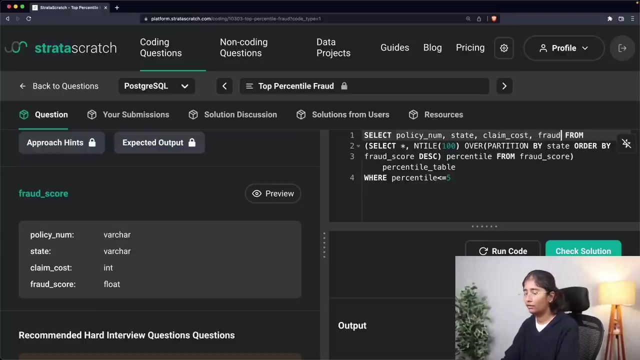 claim, cost, fraud score, percentile. and then you're containing top five percentile for the each state. since they said the output should only contain these and you don't want it to show the percentile, you can explicitly mention here what are the column names that you're looking for. so i can simply say policy num, state, claim, cost, comma, fraud score from this table. 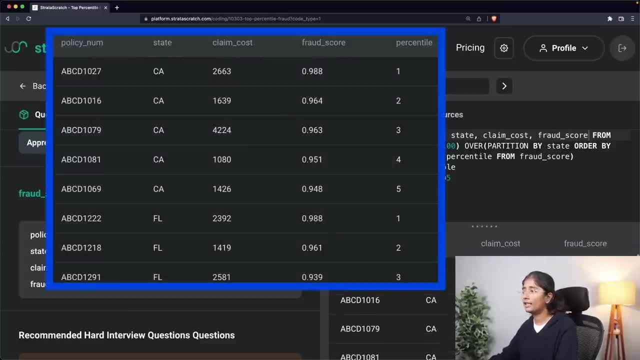 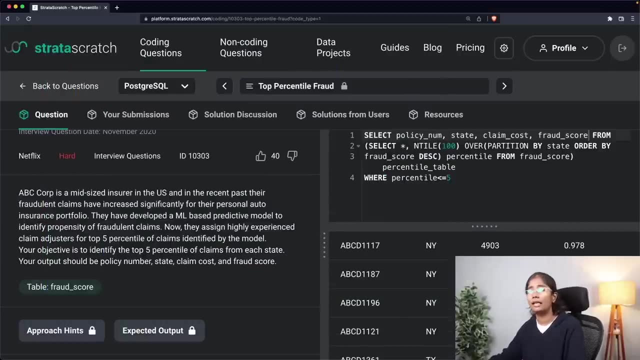 and then i'm going to run it. so there you go: policy number state. so these are the top five percentileiano each state. yeah, that's how you go ahead and solve this particular kind of questions. i will see you guys next time. bye, let's take a look at the question now. find ids of companies that have. 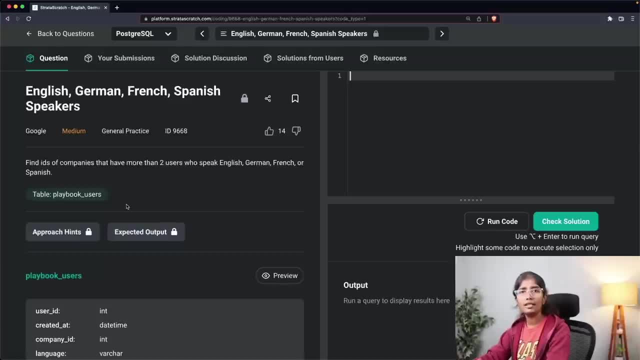 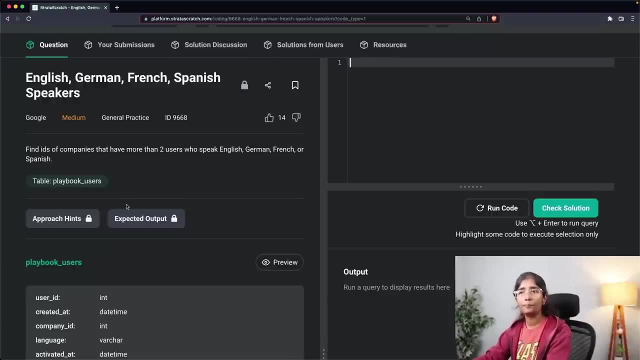 more than two users who speak english, german, french or spanish. so, according to our approach, our first step is to understand the inputs and the outputs clearly. now for me to understand the inputs clearly, i need to know what are the columns present in the table. playbook users. if you scroll. 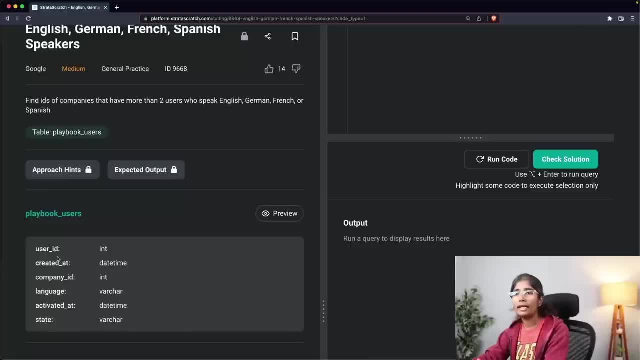 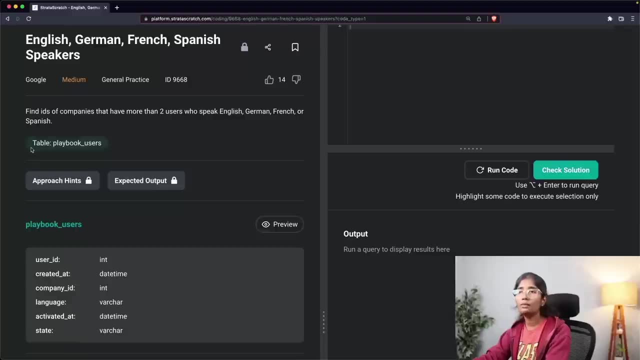 down you will see the inputs that are given to you, which is user id created at company id, language activated. and state now among these what should be my inputs and how will i know that? by reading the question clearly, which is find ids of the companies. so i need to use the company id that have more. 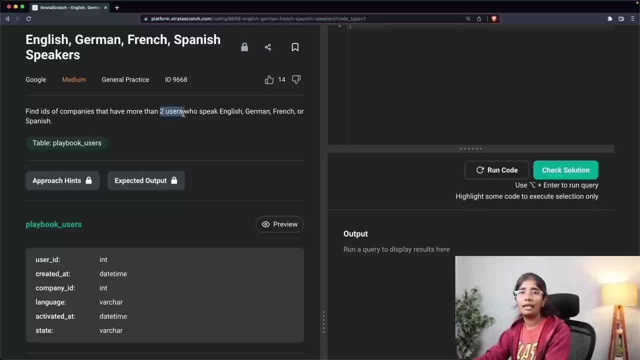 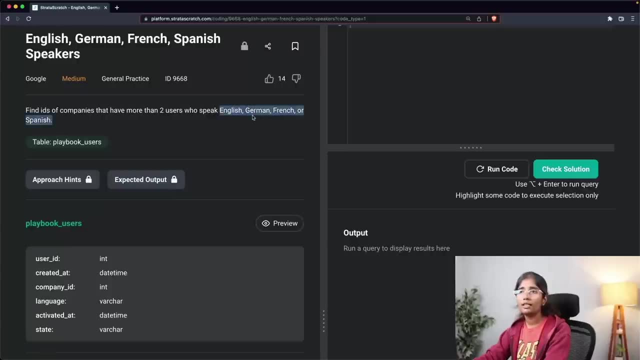 than two users. so when they're talking about users- which means i'll also have to use user id- who speak english, german, french and spanish. so i don't see any columns with respect to this. but i can see that there is a column known as user id, and i can see that there is a column known as user id, and 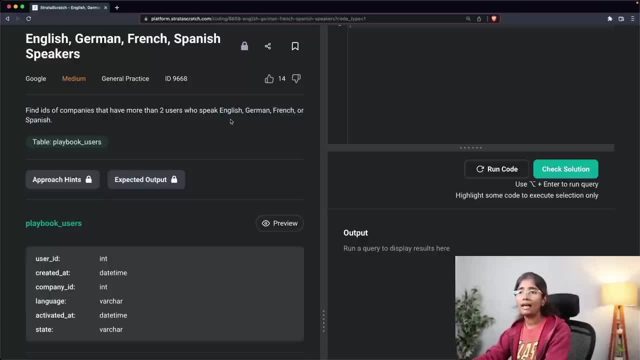 as language. so i now need to filter out these languages from the column language. so what are my inputs? company id, user id and the language. now what are my outputs? since the questions only simply states find the ids of the companies, my output will only simply be company id. so my inputs: 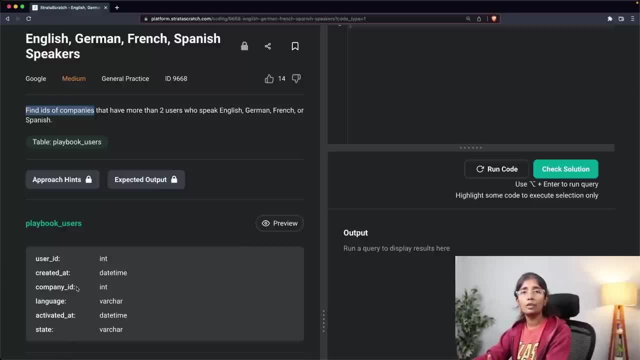 are company id, user id, language and my output is only simply company id. now step two of our approach is explain your approach verbally. now that you've understood what are the inputs and the outputs, you now have to explain to your interviewer what is the approach. if you look at the question, it says: find the ids of the company. 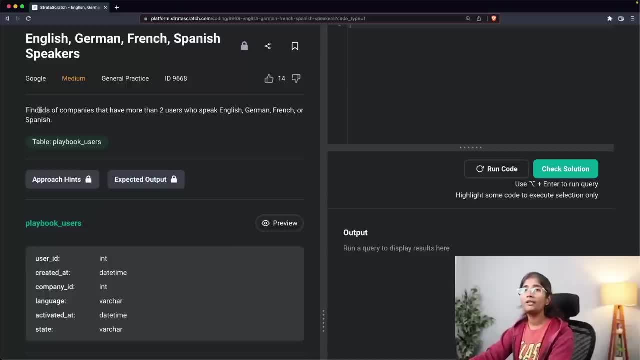 so they want you to find for each company, which means you have to use a group by clause, known as company id, and then, since they're talking about that, have more than two users. they want to perform some aggregation function, in this case, which is count. so you're going to. 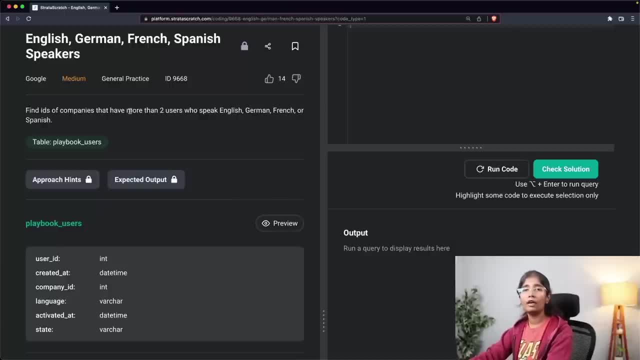 have to perform an aggregation function count for finding out more than two users and since they want it for each company, you'll have to do something called as group by, for each company who speak xyz languages. so you now need to filter out these languages from the column language. 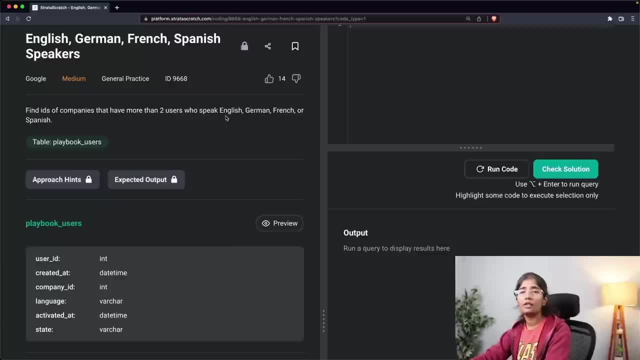 so one operator that comes to my mind as soon as i am checking for a string value is in, so i'm going to check whether this particular language is present in the language column or not for that particular user. now that i've explained my approach to my interviewer verbally, the third: 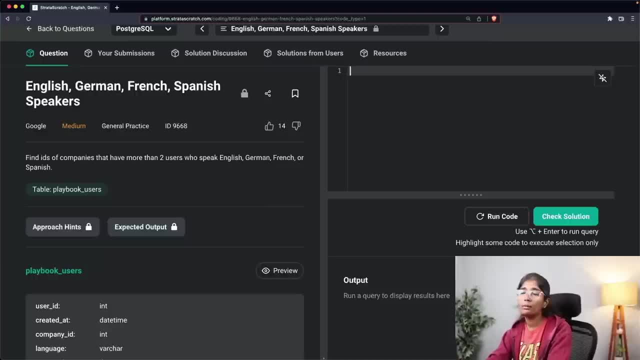 step is basically constructing my query step by step, and that's what i'm going to do now. the first step of constructing my query is filtering out the users who are speaking the languages xyz select. since my output should only contain company id, i'm only going to give company. 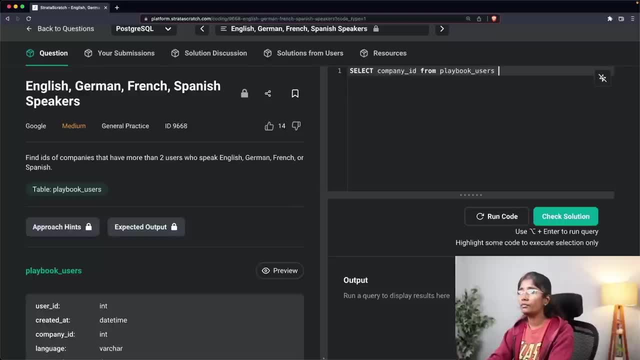 id from the table playbook users where language in. i'm going to give english, german, french and spanish, so i'm just going to run this code. okay, now it's showing me all the company ids where these languages are presenting. but since i want for each company id, i'm going to do group by. 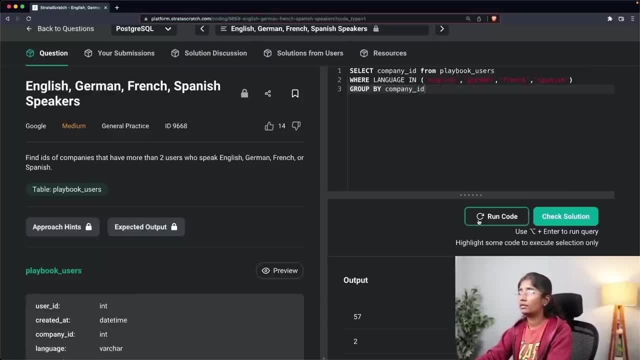 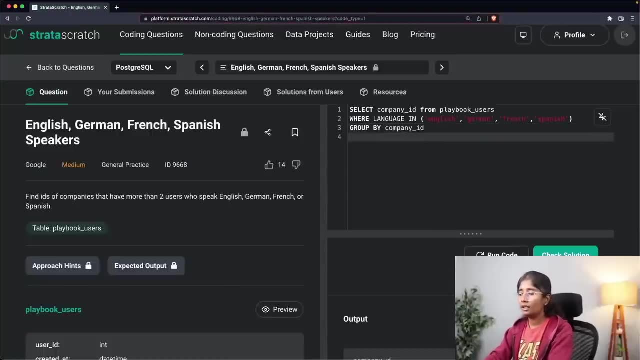 company id. great, now the class is, they want the users who are more than two in number. this is where i'm going to use my having clause, having count or user id greater than two, and now a company might contain, like multiple entries, i want distinct user id, unique user id, and i'm going to say: 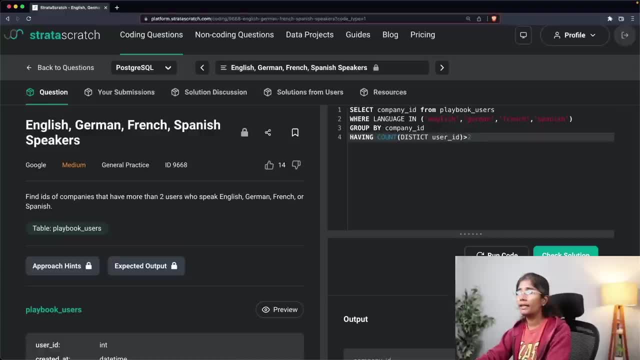 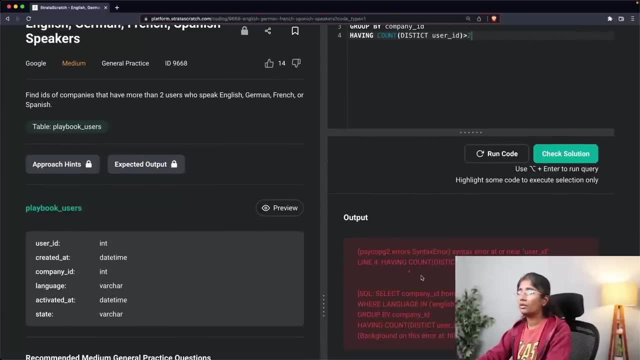 since this said it has to have more than two, i'm saying greater than two and then executing my query. who is going to be my example from that general looking query? so i'm going to give our shell code and it says there is some error which says having count. oh, it seems like i have a typo here. 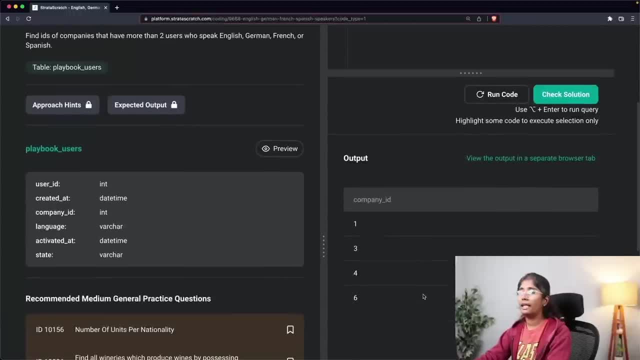 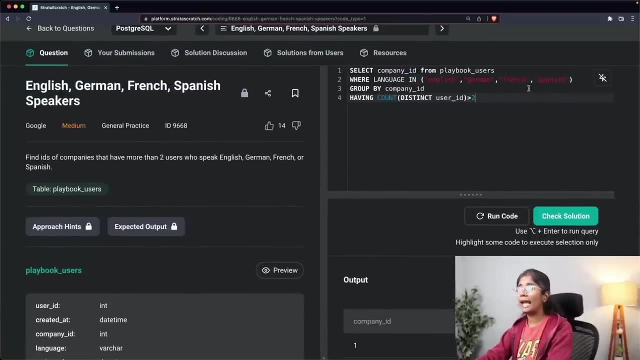 so i'm going to say this: tink, and then i'm going to run my code and there you go. so these are the companies where there are more than two users who speak the languages english, german, french and spanish. so this is how we approach in solving an sql query. so keep three things in mind, which is: 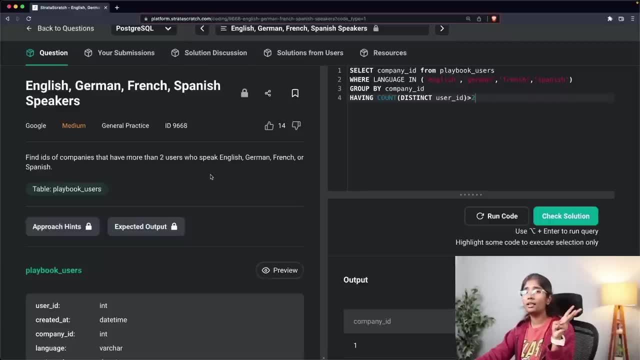 and outputs explaining your approach verbally. third thing is constructing your query step by step. that's it for this video, guys. i will see you next time. bye.